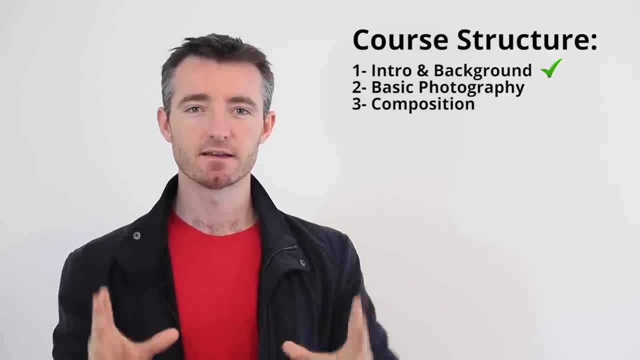 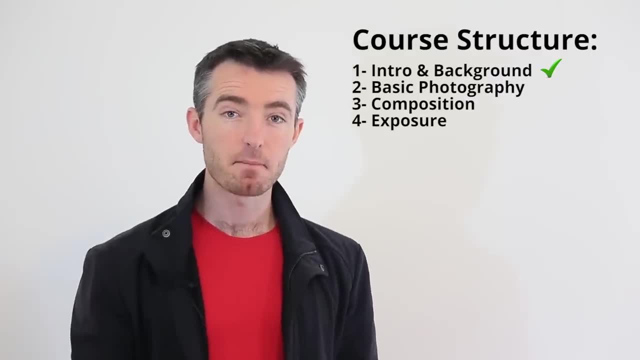 your photos so that it just feels more balanced or just more aesthetic. Then we look at exposure. You know, sometimes the photos come out a bit too bright or a bit too dark. Why does that happen? How do you fix it up? Quickly: look at histogram graphs and things like that. 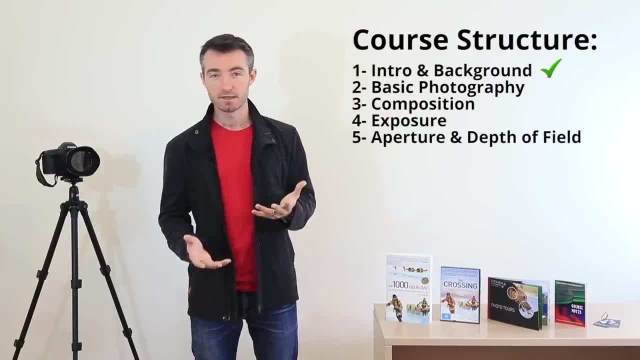 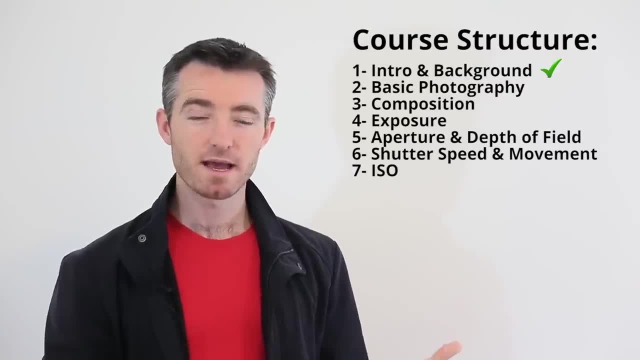 Then we look at aperture And what that does to your depth of field, And then shutter speed and how that affects things that are moving in your photos, And then we look at ISO. What's that all about? Lighting- Lighting, of course. there's so much to learn about lighting in photography. 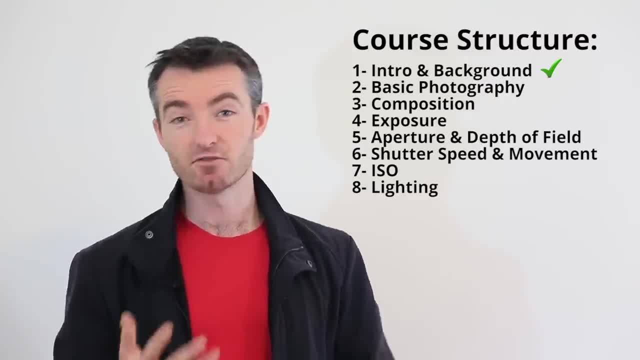 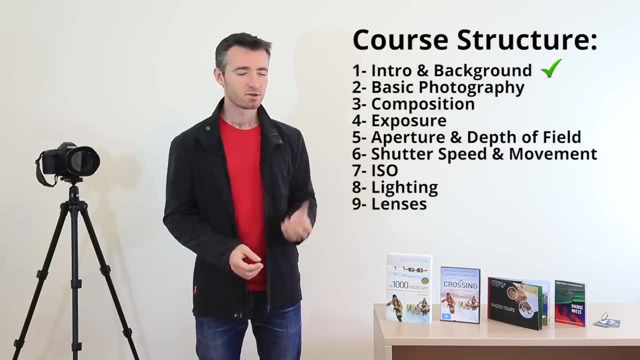 but just understanding the basics of it, like the different types of lighting and the different directions of lighting, that can be an enormous improvement to your photography Lenses. There's obviously so many different types of lenses in the world. Good to have a bit of a handle. 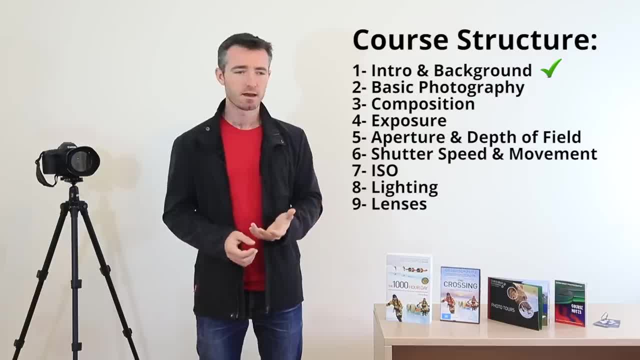 on how you categorise them, how you know what they do, what you need to know about them, what you need to know about them and how you can use them in your photography, And then we'll finish up with a lecture on just practical advice, Just bits and pieces. 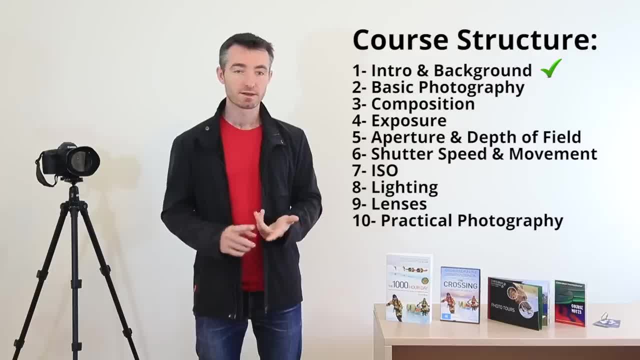 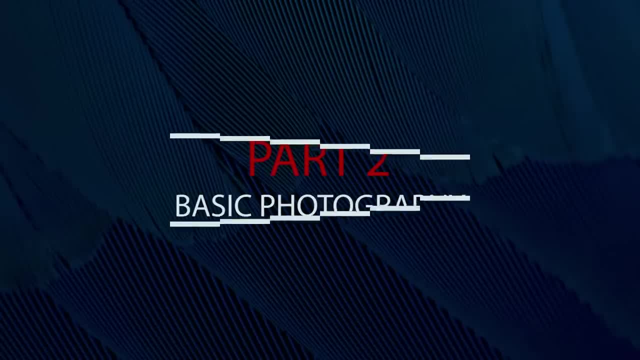 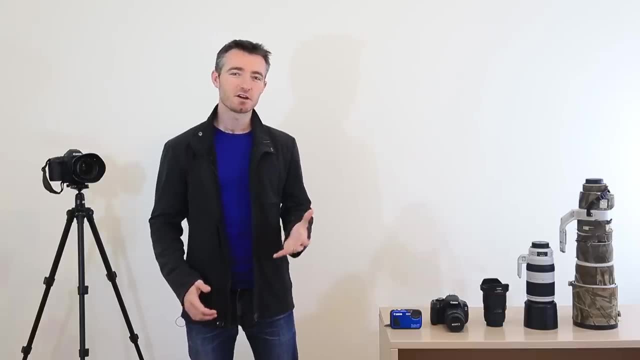 I'd hate for someone to be able to do a photography course and not be told Everything from a little bit on post-production to keeping your camera clean and where to from here and that sort of thing. Okay so, basic photography. In this lecture we're just going to look at some very simple 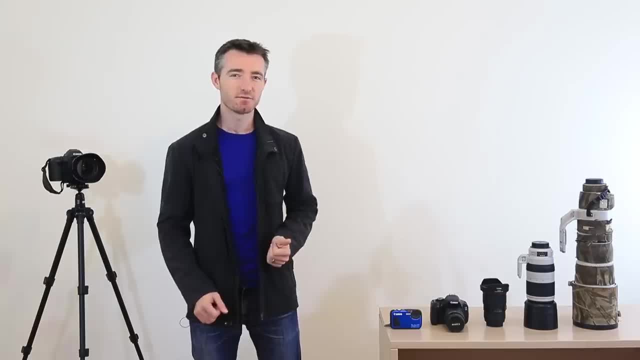 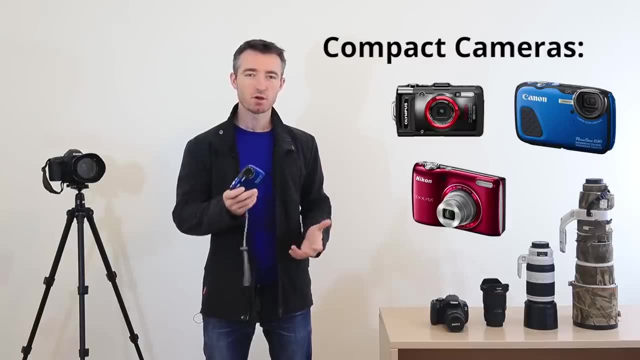 things like how the camera works and how to set it up ready to start taking photos. You've got three different types of cameras, really. You've got compact cameras like these ones, and the beauty of them is obviously just that they're so compact You can take. 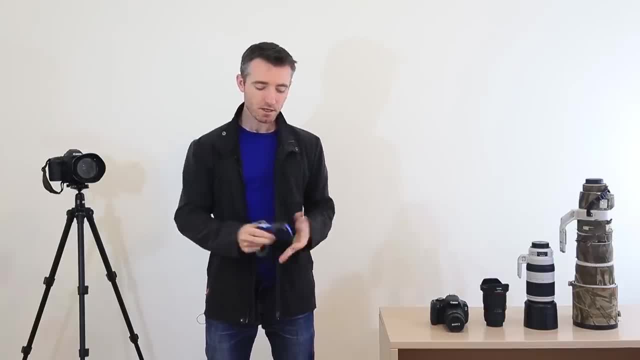 them with you wherever you go, and you can always get some kind of photo. Sure, it might not be quite as high quality or have quite the same amount of creative control as a big DSLR camera or something, but at least you can get a picture, And obviously the best. 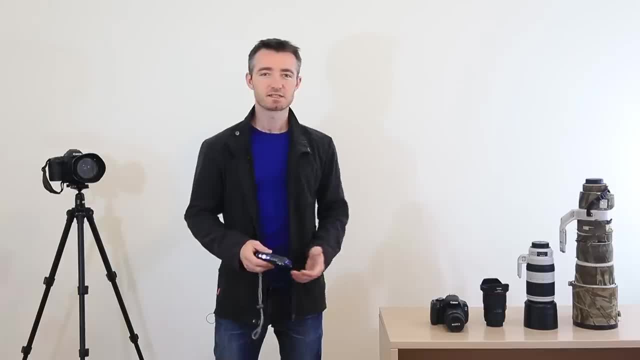 camera is the one you have with you at the time. Sometimes, when people buy their big DSLR camera, they start to dismiss the compact camera and sort of think, huh, that's only for social photography or you'd never take a picture like that. But that's not the case. 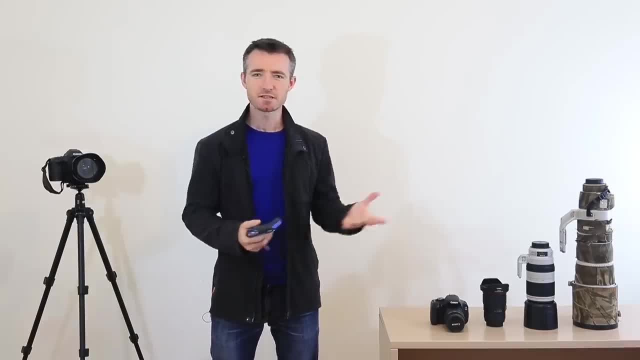 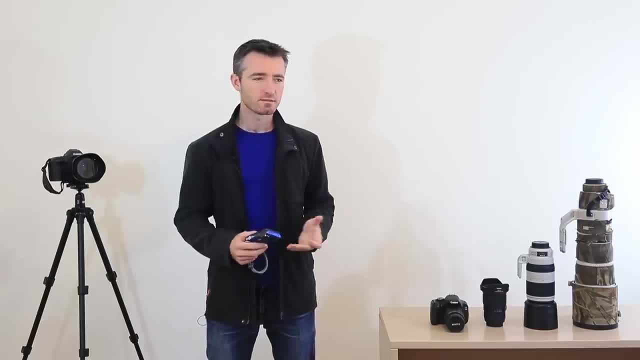 especially if they're waterproof, shockproof. little jobs like this thing where you can bring it out in situations where, even if you had your big DSLR with you, you're not going to bring it out if it's pouring with rain or if it's really dusty or something At least. 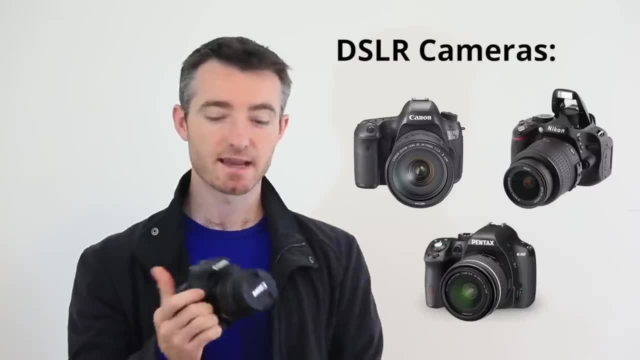 these kind of cameras you can always get a shot. Then you've got DSLR cameras like this one, bristling with all these buttons and dials to bring out that creative control to your fingertips so you can set up the photo to. 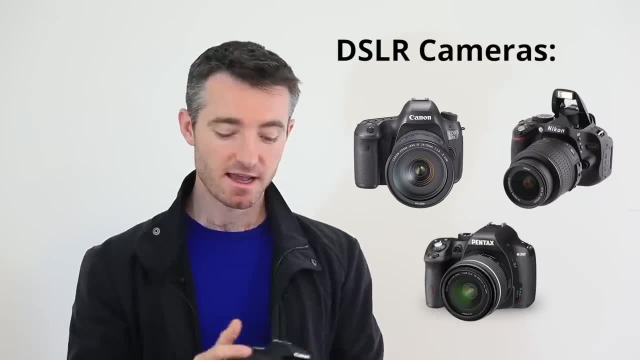 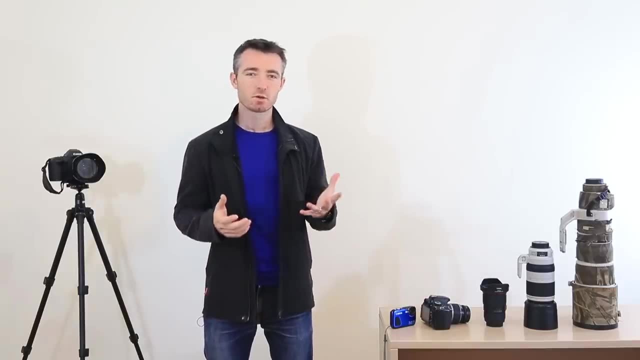 come out the way you want. You can use interchangeable lenses and in general you just have a lot more control and you can get much higher quality photos. Then you've got sort of in between cameras, mirrorless, micro, four thirds bridge cameras. 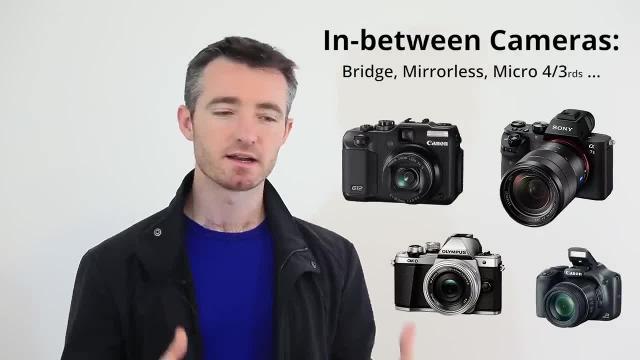 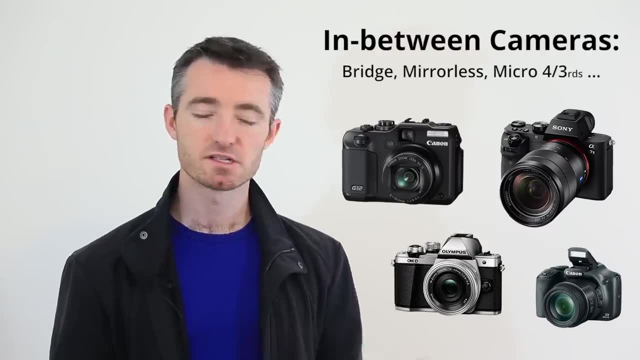 They still have all the same theory, all the same aperture and shutter speed and all that kind of stuff, but they're just often smaller. Sometimes you can change lenses, sometimes you can't. They're just more convenient, more portable and increasingly they're doing better. 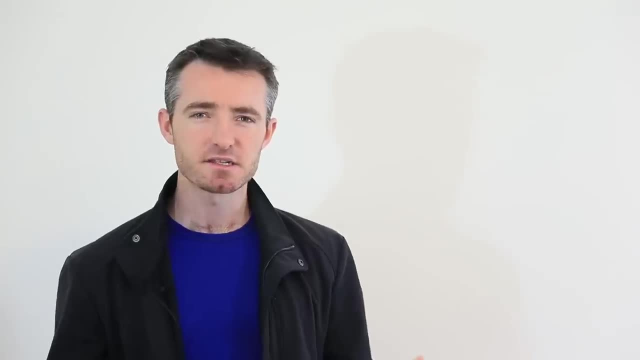 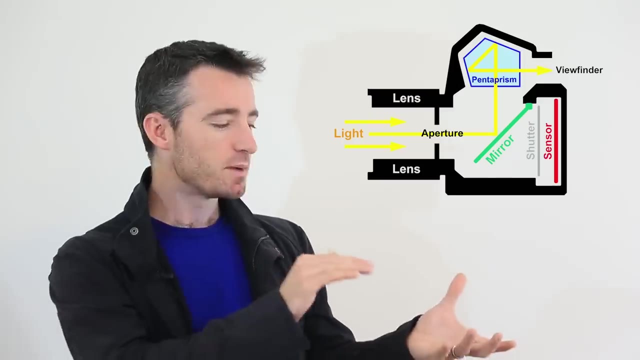 and better jobs at taking incredibly high quality photos. Okay, so how do these things actually work? Well, just simply, Light comes in through the lens. obviously, That's where you're doing your zooming and your focusing and so on. but importantly, 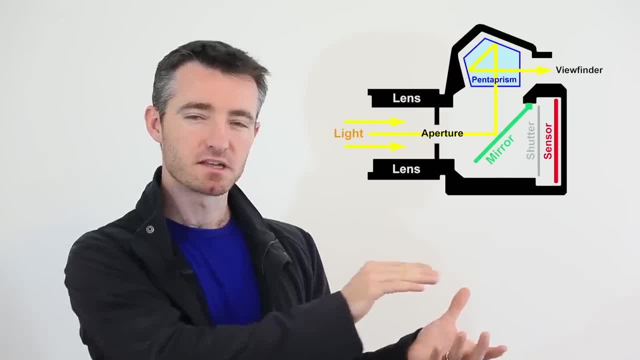 the light has to pass through a variable sized hole in the back of the lens and that's called your aperture, And you can set that hole to be whatever size you want. You just tell the camera: hey, I want the hole to be this big, I want the hole to be. 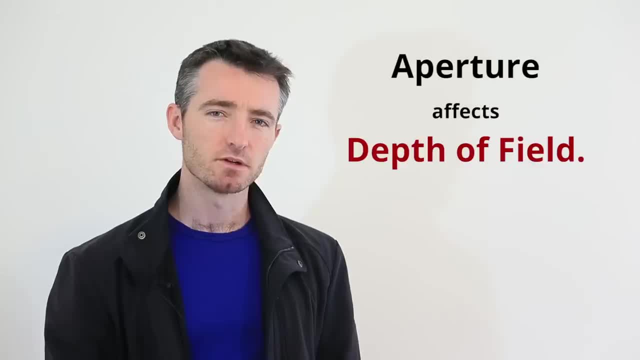 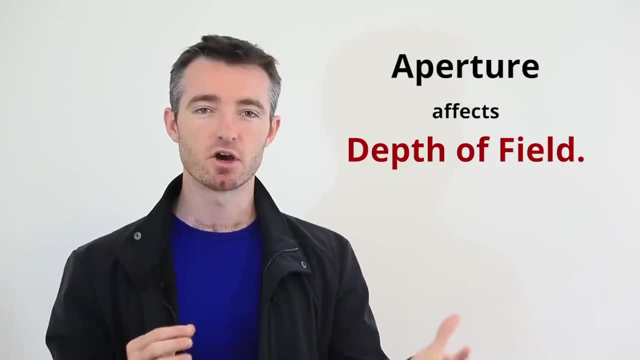 this big and the size that you set that hole at controls- what's called your depth of field in the photo. Now, depth of field is just the amount of stuff that's nice and sharp and in focus in your shot in front of and behind the point that you focused on. 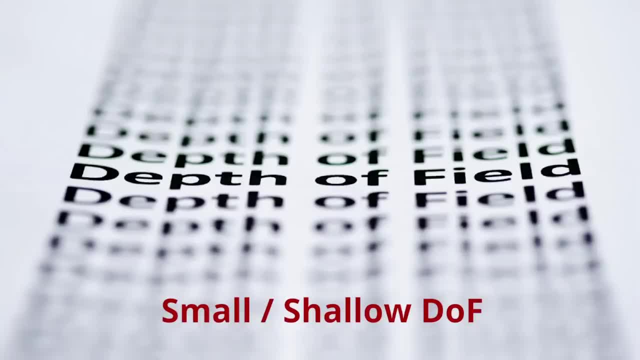 So you can see If you used a small or shallow depth of field. you know we've focused the camera here, but very quickly the background becomes blurry and anything in the front becomes blurry, Whereas if you used a different sized aperture hole, maybe you'd end up with a big depth. 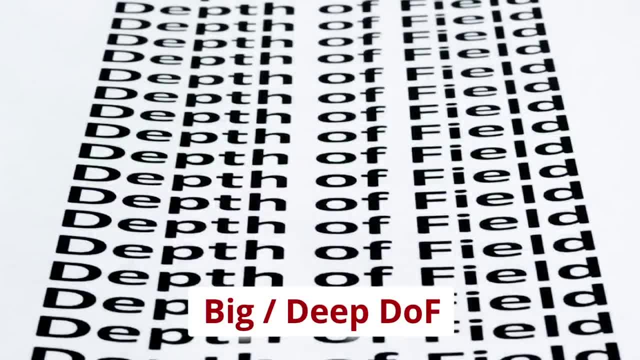 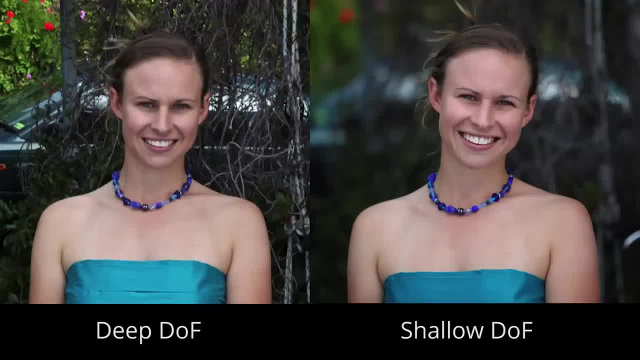 of field or a deep depth of field, And you can see here that much closer it's still in focus and much further away it's still sharp And you can see the effect that has on your photos. For a photo of a person, obviously the one with the nice soft background looks a whole. 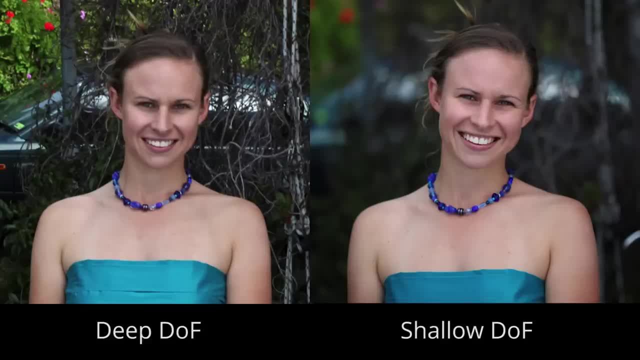 lot more professional because the model stands out against that soft blurry background, looks more 3D, Whereas on the other photo, where there's a larger depth of field, you kind of lose your subject against the background. It kind of feels very flat and two-dimensional. 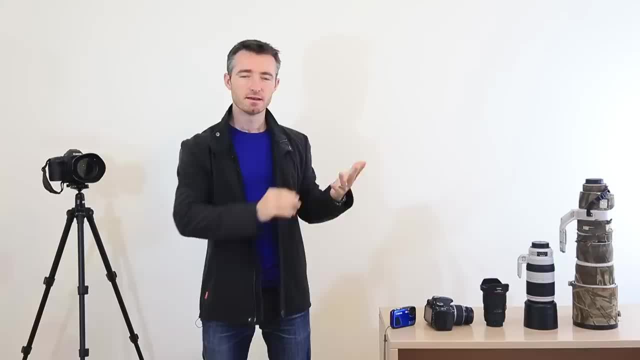 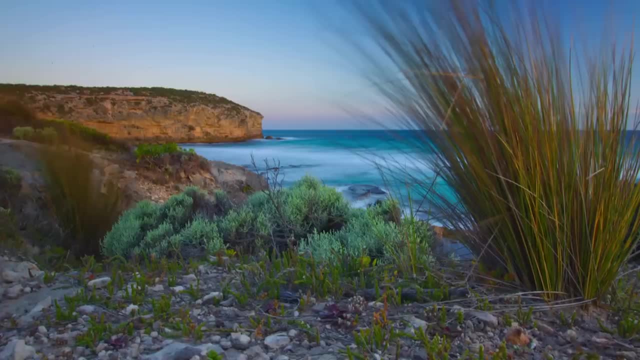 You can't really see where the hair finishes and the sticks in the background begin. It's all very kind of flat. But that's actually what you'd want: a big depth of field for a landscape photo, if you think about it, Because for a landscape shot you want your close-up rocks and flowers to be nice and 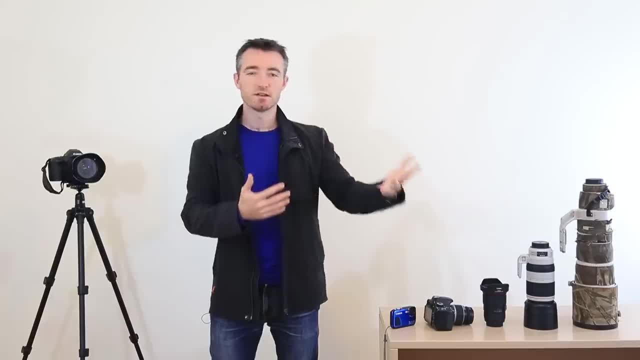 sharp, but also the distant mountains and clouds, because everything is interesting in a landscape scene. Now, obviously, if you leave your camera in auto mode, your camera has no auto mode, So you can't really see what's going on in the background, So you can't really see where the hair finishes and the sticks in the background begin. 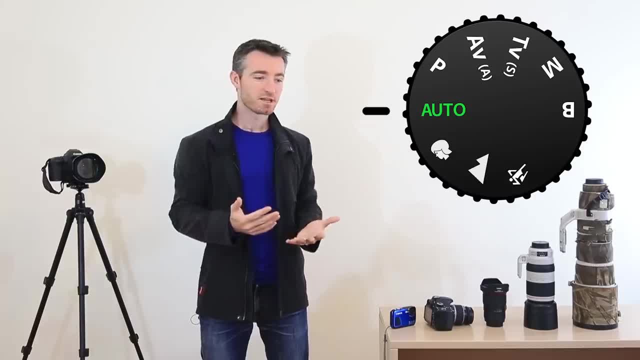 Your camera has no idea what kind of photo you're trying to take. It'll just pick a value somewhere in the middle, and it won't give you a very good job at either situation. So you can see how much creative control you're going to have just by playing with your aperture. 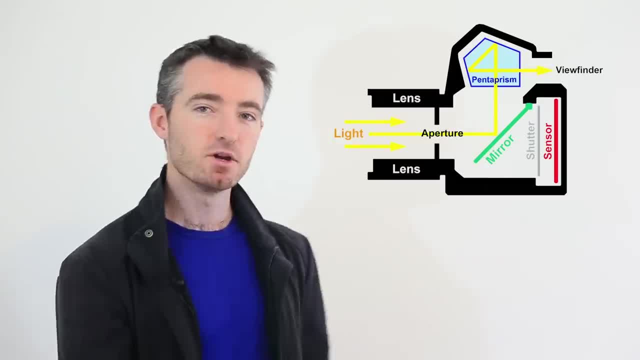 And it's really not that difficult at all. When you actually take the photo, the mirror kicks up out of the way. There's still a shutter in the way, though. The shutter will then open and close for a very precise amount of time to collect all. 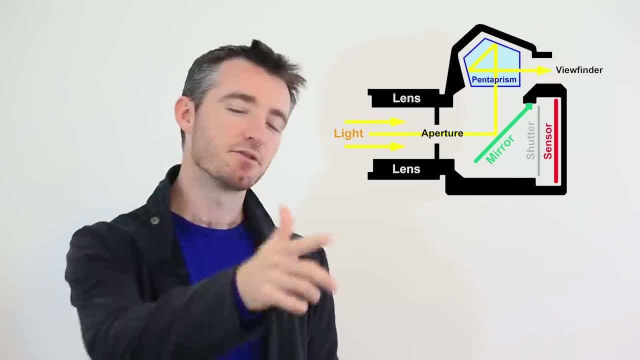 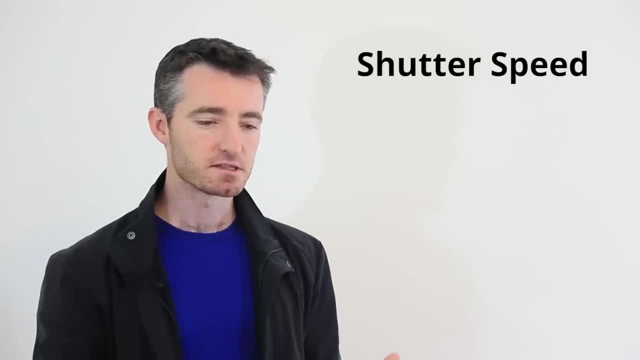 that light for your image And then the mirror will fall back down and you'll be able to see through the camera again. But the amount of time that that shutter stays open for that's called your shutter speed, and that affects how things that are moving end up looking in your photo. 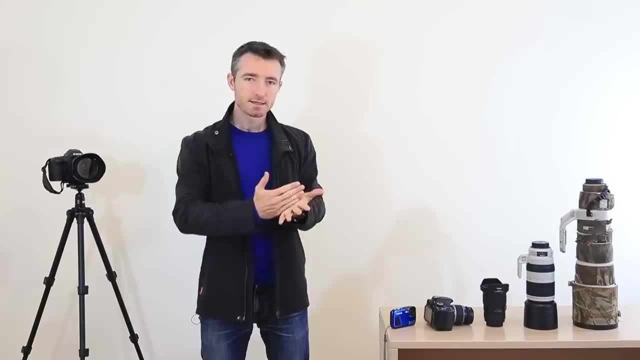 Obviously, if that shutter has only been open for a very brief amount of time, nothing's had a chance to move anywhere while the photo is being captured, So you end up being able to freeze even quite fast movement. But if the shutter is open for a long time, then anything that moves while that photo 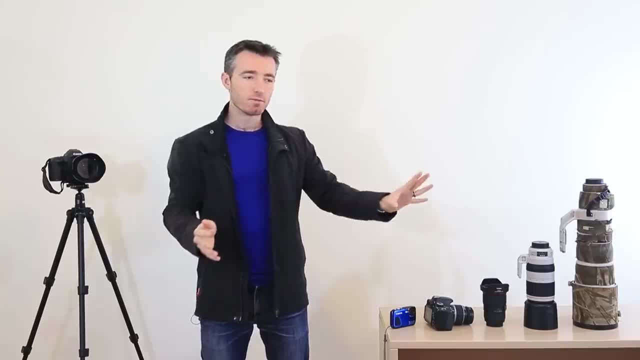 is being captured ends up being smeared through your image and you kind of end up with movement blur, Which can look really nice in a lot of situations, Not only waterfalls and classic shots like that, But anything that's moving. It can just add a bit of life if you let the shutter drag a little bit. 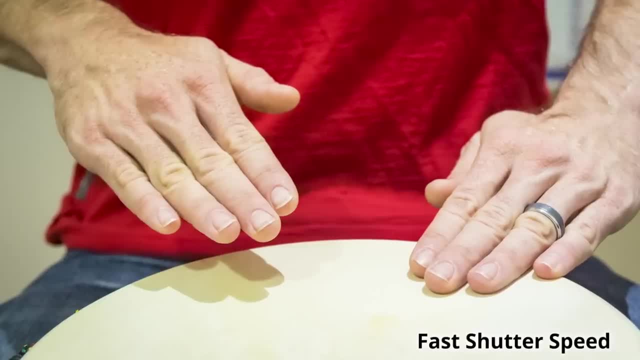 Let's say you're photographing someone hitting a big drum In auto mode. you probably end up with a pretty fast photo and the guy's hand is just going to be frozen there and you can't really tell is he hitting the drum or is he just standing. 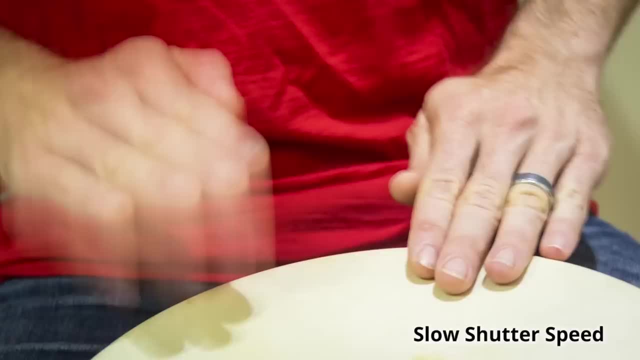 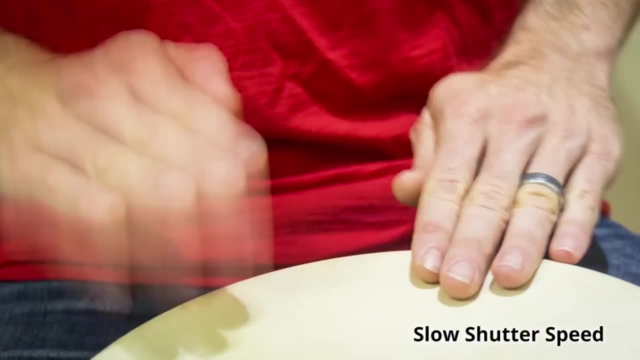 there or what, But if you allowed your shutter speed to be just long enough that the guy's hand could move from here to here while you were taking the picture, you'd end up with this streaky, blurry hand moving towards the drum. that might just add a whole lot of life. 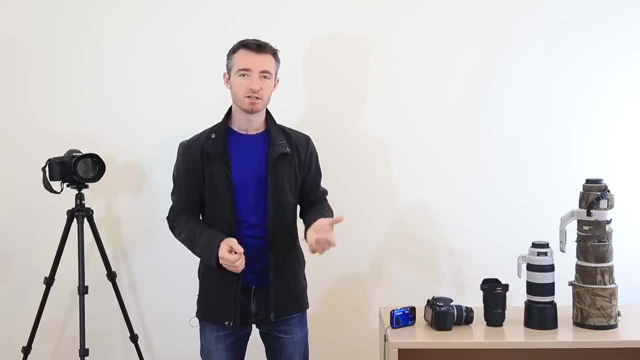 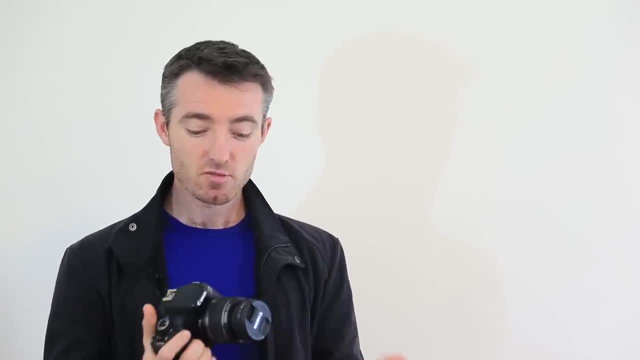 So there's a lot of situations where having a longer or a shorter shutter speed can really change the effect in your picture. Okay, starting at the real basics, Hopefully at least you know how to turn your camera on Zooming in and out. Obviously, you just twist the barrel of the lens and you see the image get more zoomed. 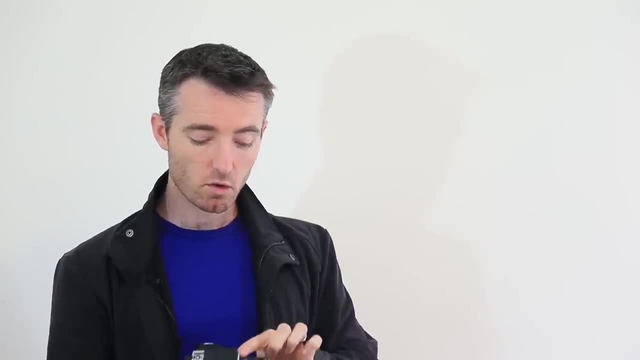 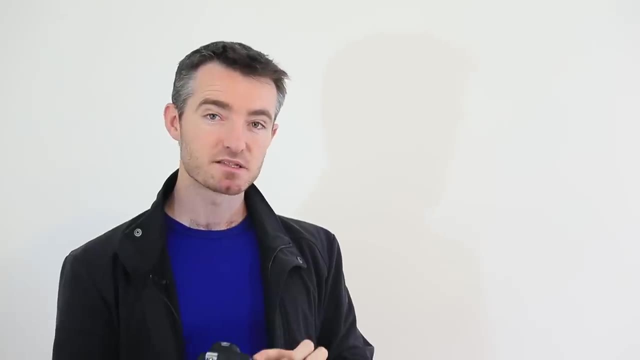 in and more zoomed out. Worth double checking. if you've got an auto focus, manual focus switch on the side of your lens, Good idea to make sure that's set to auto focus. If you've got a stabiliser, may as well turn that on. 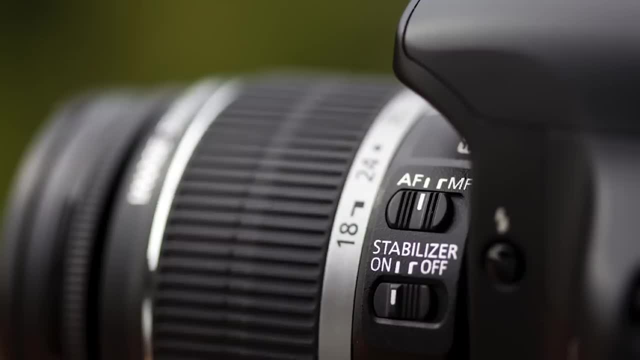 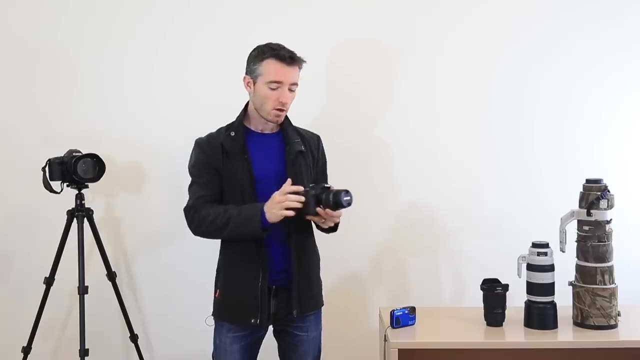 Different brands call it different things Could be optically stabilised. OS VR IS. If you've got any switch on your lens for now, you may as well turn it on Now. I'm sure you're all aware all shutter buttons work the same way, in that they're 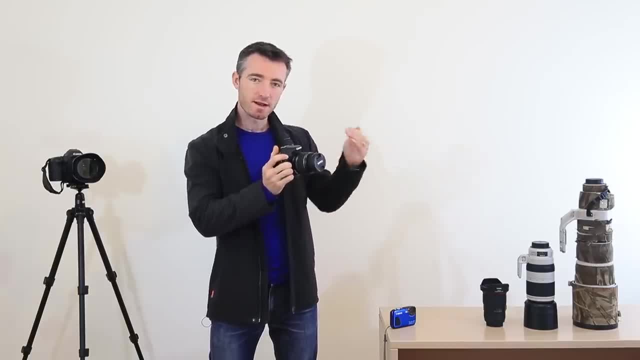 a two stage button. You know you can push them half way down and they come to a natural stop, and that's when the camera is trying to find something to focus on. zzzz beep. hopefully it does, But it won't actually take the picture until you press the button all the way down. 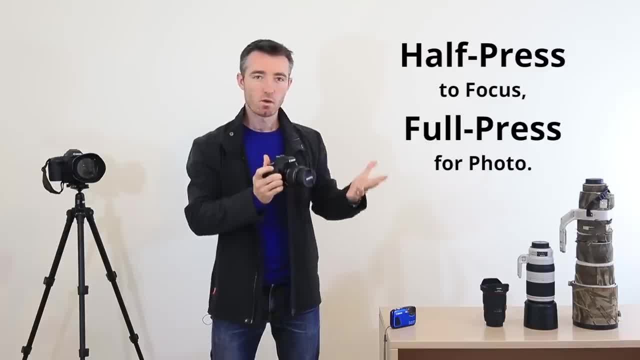 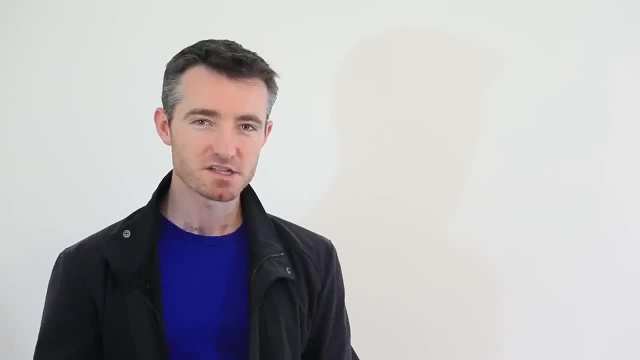 So it's supposed to be that two stage step? don't just plunge it all the way and then wonder why it didn't get the photo Half until it finds it beep, and then press the button carefully- Camera for the first time. I think the first thing we're always told is hold the camera. 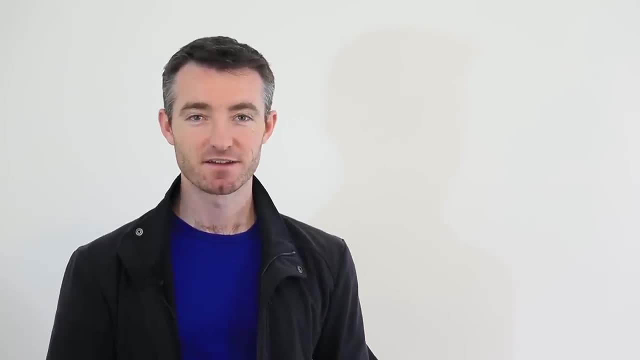 really steady And most people just think, yeah, I know all that kind of stuff. But actually you'd be surprised. I took a photo of the word shake when I was designing these lecture slides and it was late at night. it was a classic long, slow exposure. gonna have a lot of camera shake. 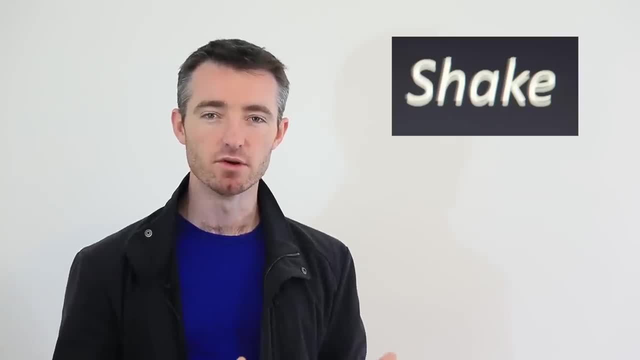 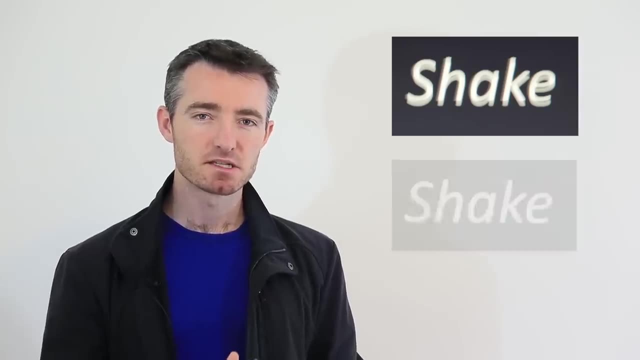 in there And this was holding the camera as steady as I possibly could, but just doing a few basic techniques wrong, like holding the camera the wrong way, the way I see a lot of people hold cameras, And then this is taking the same photo again. 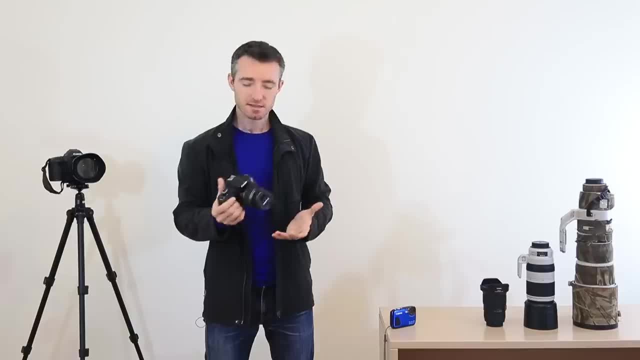 Doing a few basic things right, like hanging onto the camera correctly. So let's take a look at even how you're supposed to hang onto the thing With your right hand. it's pretty obvious. there's a giant grip there. you can't go wrong. 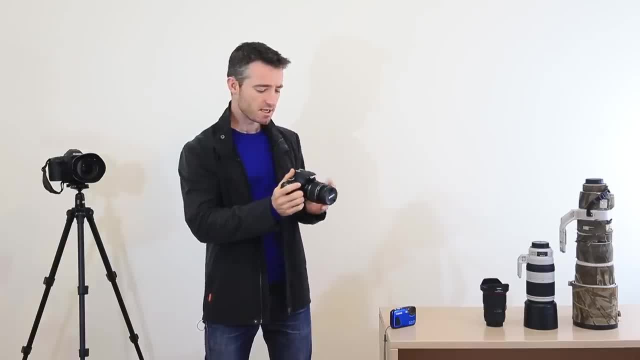 But with your left hand you see all kinds of awkward things happening, just cause there is nowhere really obvious to hang onto it and people end up just clasping the side of the camera often And that just means you're pressing all these buttons here without meaning to. but the worst 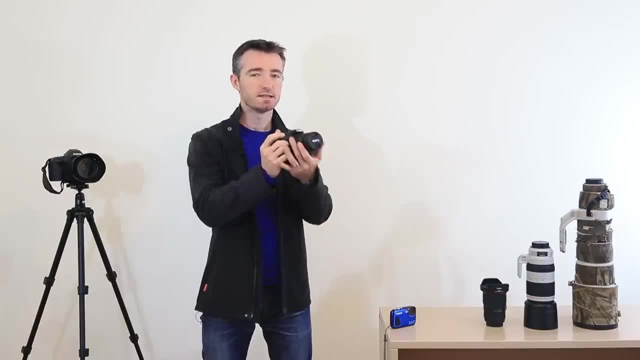 thing is you're not supporting the camera. Your left hand is supposed to be underneath the lens and in fact the further out along the lens it is- if it's a big lens, the steadier the shot will be, rather than all the way. 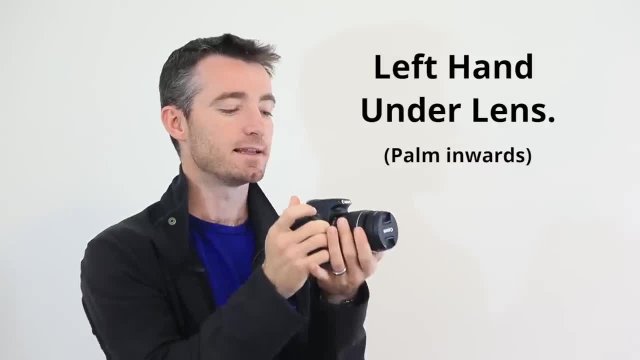 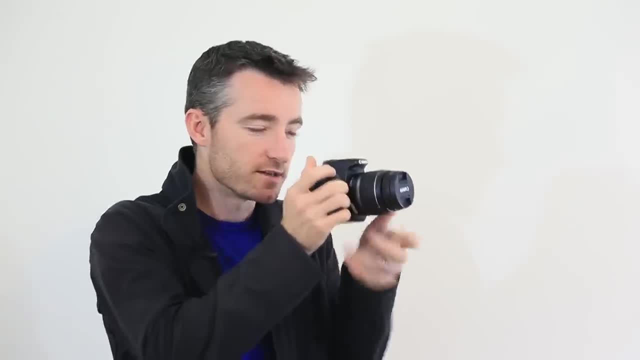 back here just clasping the side, So your left hand underneath the lens supporting it. That also means you're able to recompose the shot, zoom in and out all the time. You don't have to kind of change it and then come back and hang onto it and then that's. 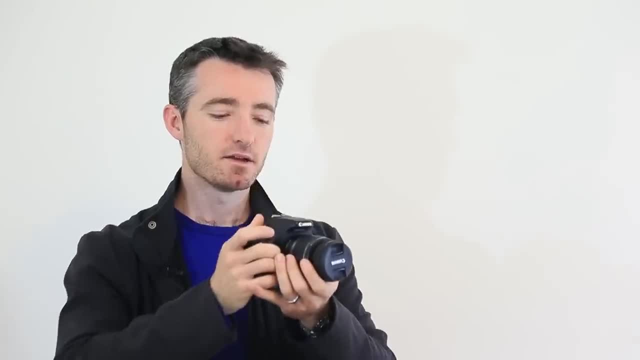 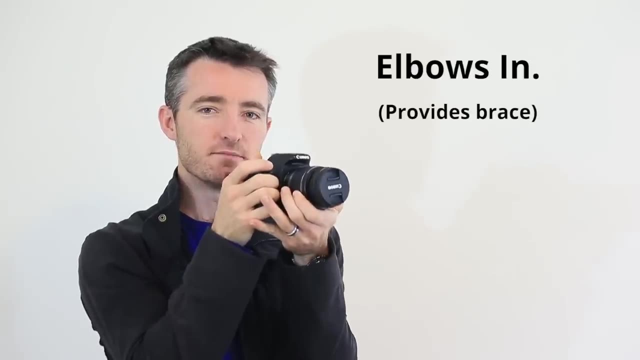 all very awkward. You should put your elbows in. that keeps it steady. So if you just hang onto a camera like that, it's able to wobble around wherever it wants to be. but if you pull your elbows in, you've just got a nice inbuilt rest and it just 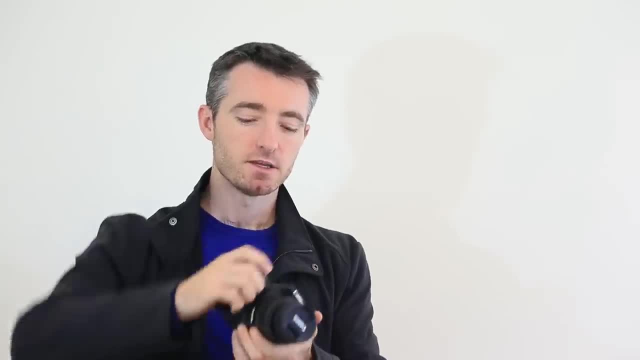 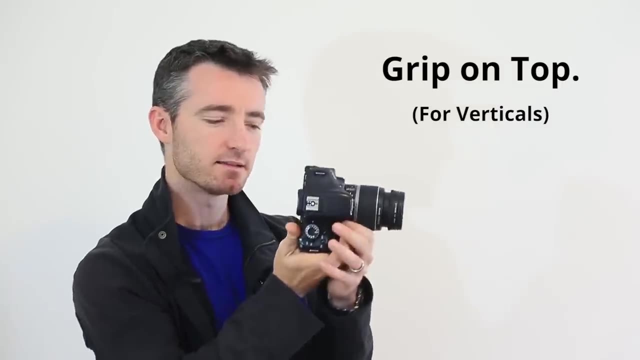 keeps it really steady, And if you're taking a vertical shot, you should actually have the grip on the top of the camera, not the bottom, Because if you have the grip on the bottom, then your other hand ends up tangled underneath here as well and you can't get to any of these settings on the top, and it's just kind. 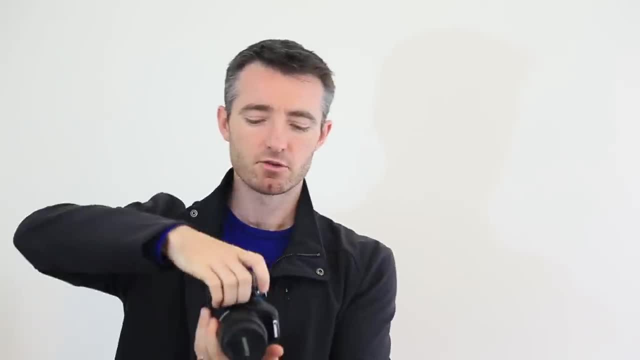 of top heavy. it's just propped up there like that. But if you have your grip on the top, your other hand comes underneath. you can still put your elbow in your chest, keep it really steady and you can get to all of your settings. 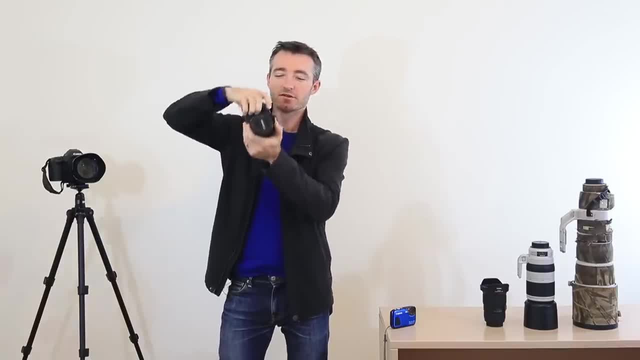 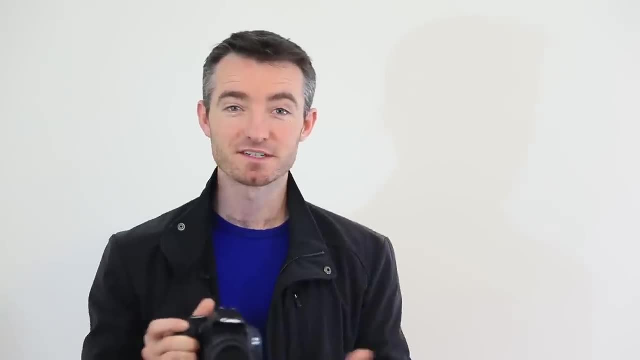 at once. Yeah, it means everyone can see you've got a sweaty underarm, but that's kind of the way it goes. Don't do these ones, Yeah. So pulling it down, keep it really steady. And probably the most important tip is don't press a button too hard, because it just shakes. 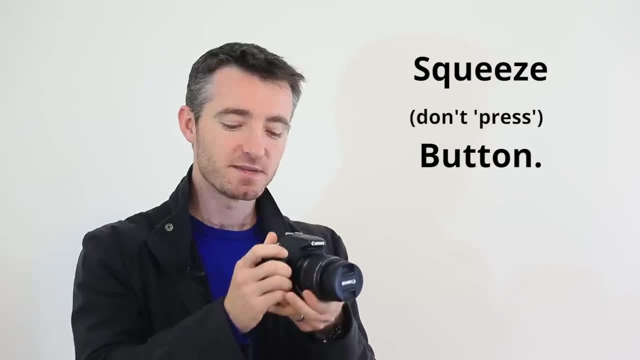 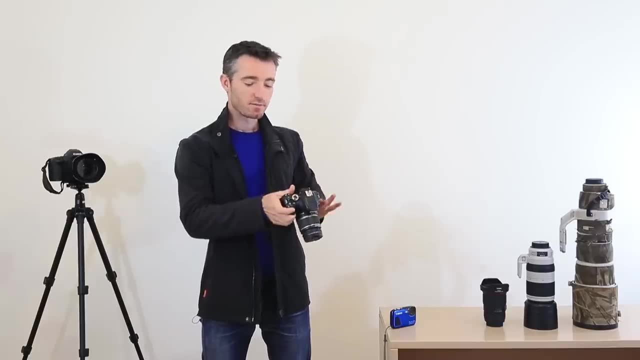 the camera at that critical moment when it's trying to take a picture. It should just be a case of gently squeezing it until it takes the shot. Obviously, one of the huge advantages of digital photography is that you can now look at the picture as soon as you've taken it and check that it worked out. 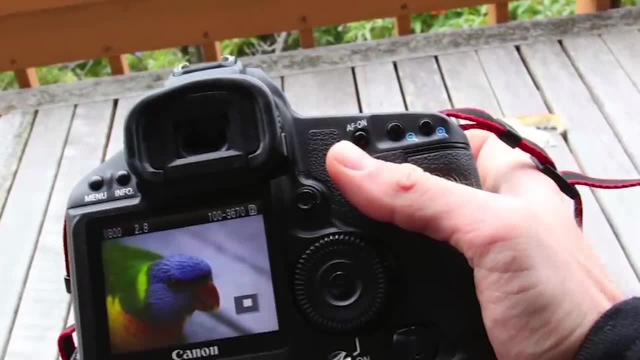 And if it didn't, you can quickly change the settings and take the photo again before your subject's gone. Gone are the days where you come back from the chemist two weeks later and then you're flicking through your photos and then you're like ugh. 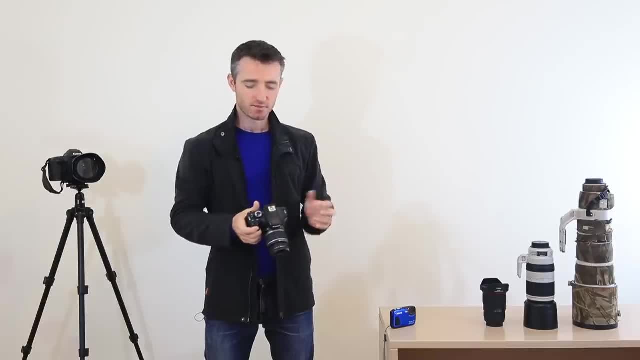 I had the lens cap on or something, But sometimes you need to remind yourself to do that check. You know, when you take a picture and it comes up for two seconds on the back, That's because you're supposed to look at it. 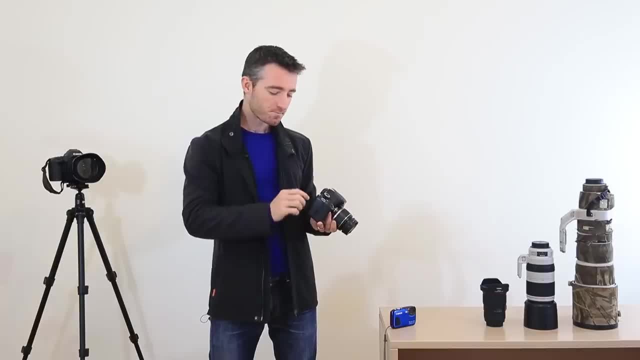 It's worth your time just having a quick glance, seeing if it seems about the right brightness, Maybe zooming in digitally on the little magnifying glass plus minus. zoom in on the picture you've taken. go right in and check that the detail is still nice and sharp. 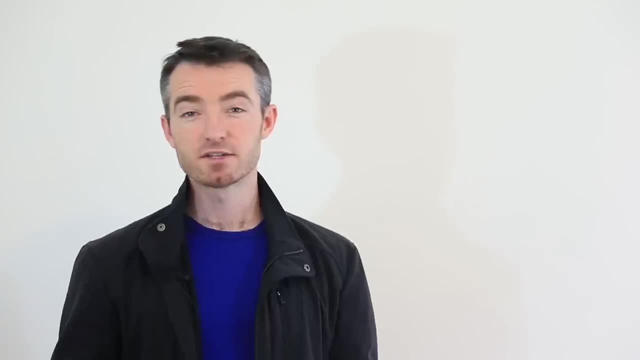 If not quick, change your settings and take it again while you still can. So, having taught this course a couple of times, there's a few things we've learnt that it's a good idea to try and catch early on. This might not be a problem for you- you might already have it set up- but it's still. 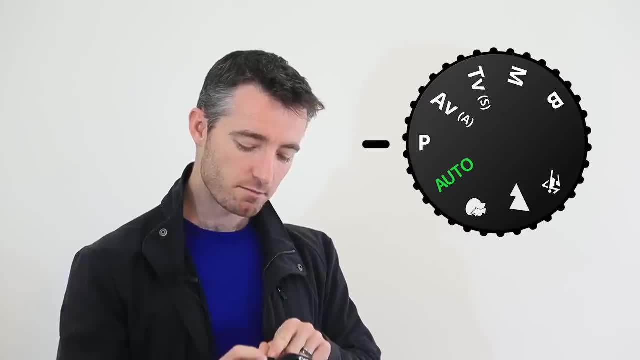 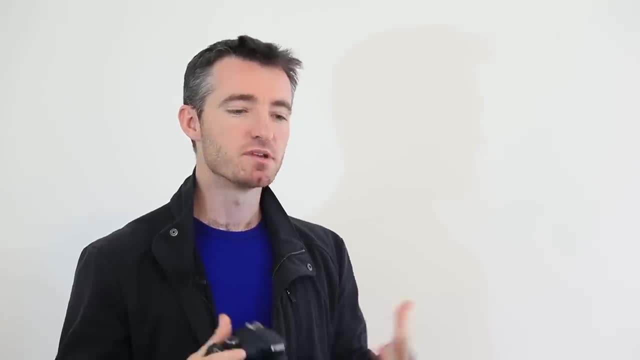 worth checking. So when you pick up your camera, make sure that it's on P mode to start with. on your big mode dial P for program. We'll just sort of use that as a stepping stone from here. It opens up some more options for us, but then we'll move on to using things like aperture. 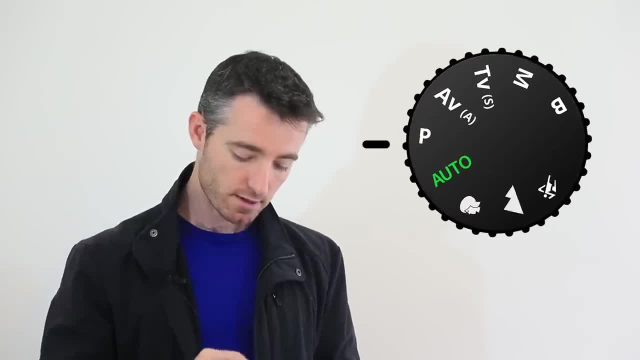 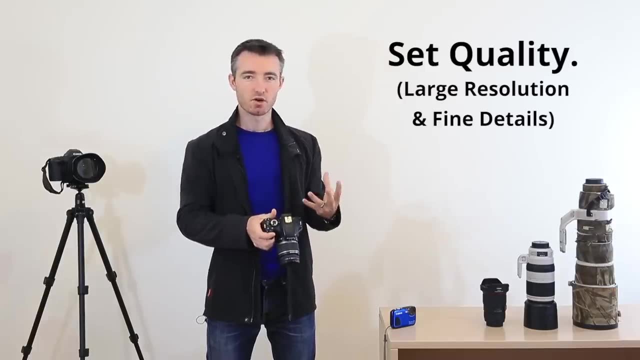 mode and shutter speed mode. But for now you've got to at least get off auto and go to P mode. You want to make sure you've got the right quality setting on your camera as well. Not much good taking low resolution or heavily compressed pictures. 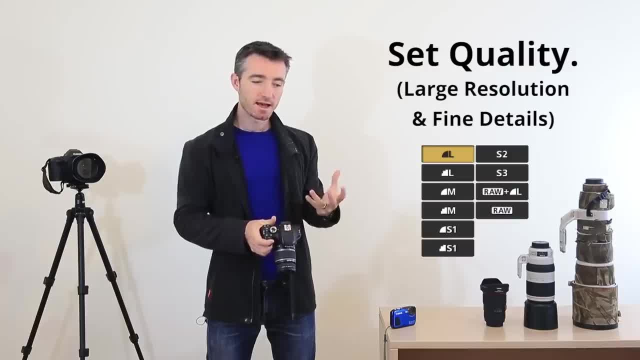 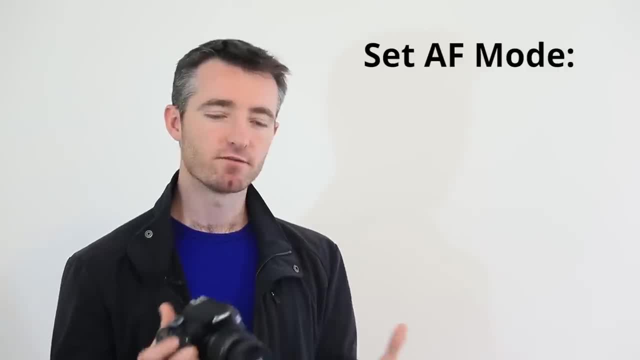 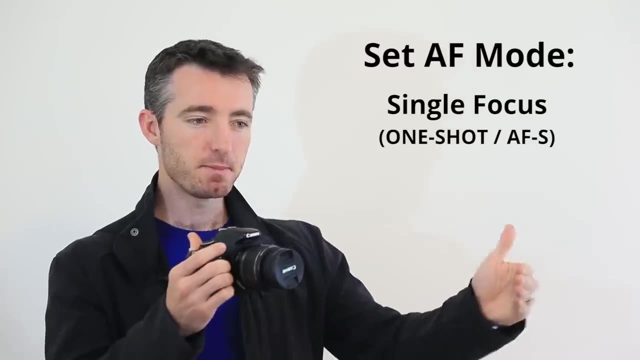 So go into your menu, Find your quality, Make sure you're on large, fine quality JPEG or a raw file if you're interested in doing that. Now, the auto focus in your camera can actually work in one of two different ways. It can either just do a single focus, so AF-S, or one shot, and that's when it focuses. find. 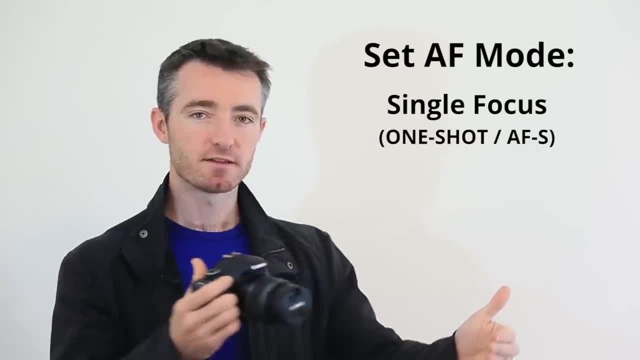 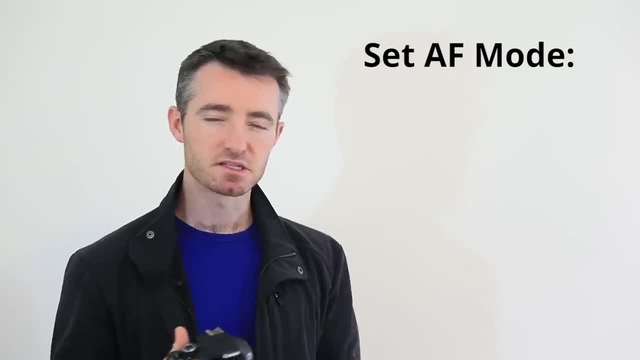 something, And as long as you keep your finger half pressed, if you move the camera around after that, it doesn't shift the focus, So it only focuses once. or you can change your camera focusing mode to AI servo, which other brands call AF-C for continuous. 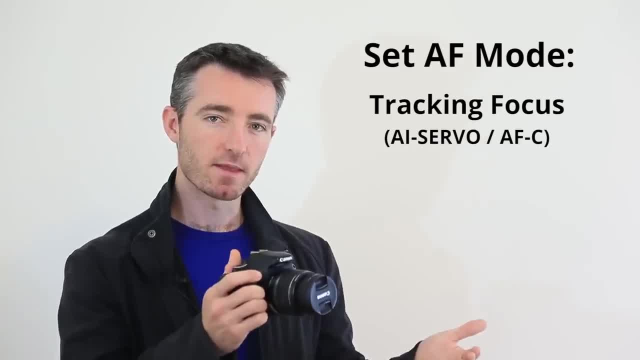 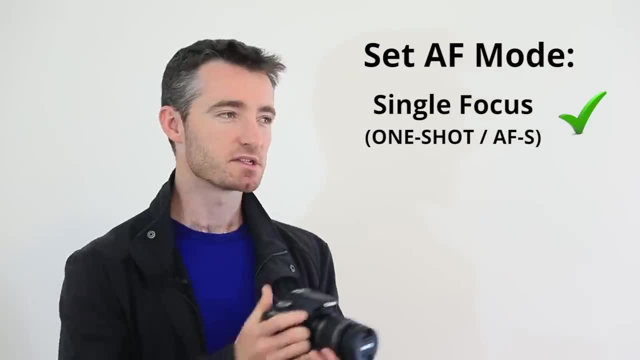 And that's a tracking focus. so as long as you hold your finger down halfway on that shutter button, it's constantly updating the focus wherever you point the camera. Most of the time you want to be on one shot- AF-S, the single focus, so you can carefully. 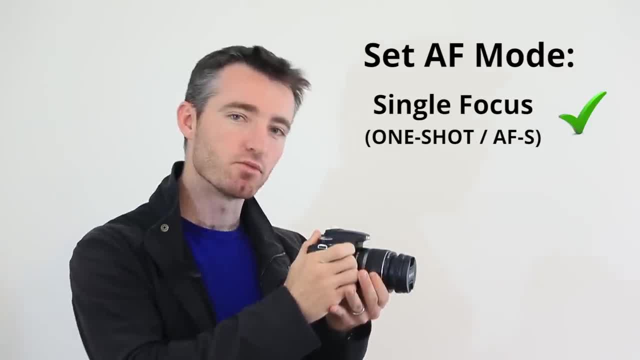 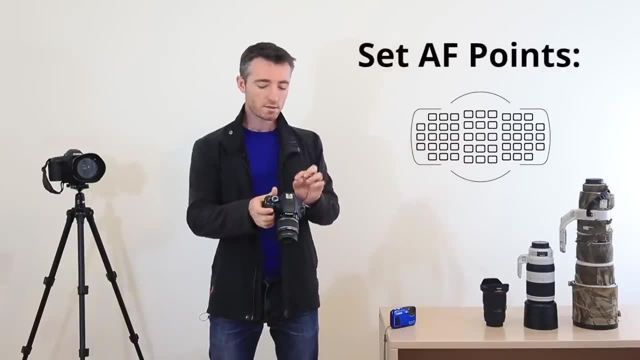 focus on something and then maybe recompose your shot a little bit before you press the button all the way down to get the shot. You've probably also noticed that a lot of cameras these days have a lot of auto focus points on them. These are all the different points that when you try and focus, these are all independently. 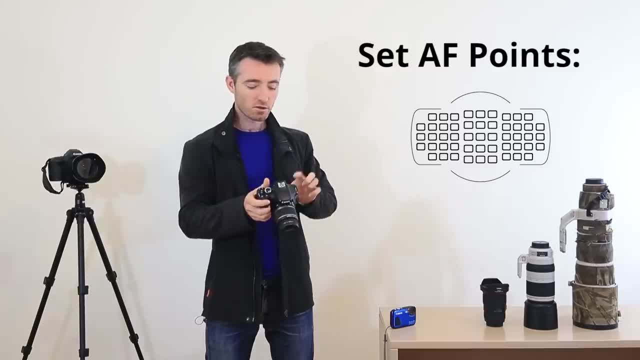 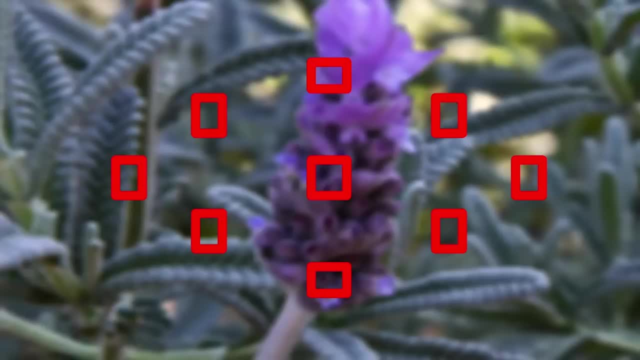 trying to find something And by default, all of these points are turned on, so they're all active, which means you have absolutely no control over where the camera is going to focus. it'll just find the first thing that's brightest or has the most contrast, and often it's not what you're. 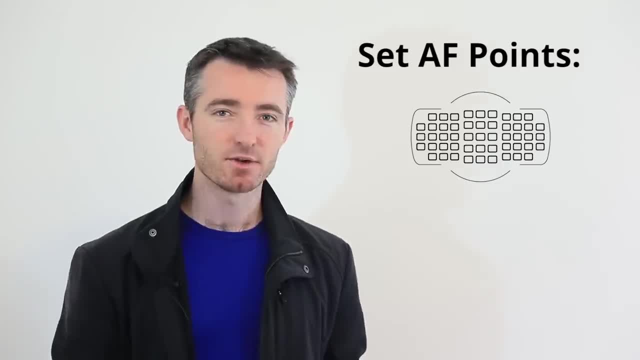 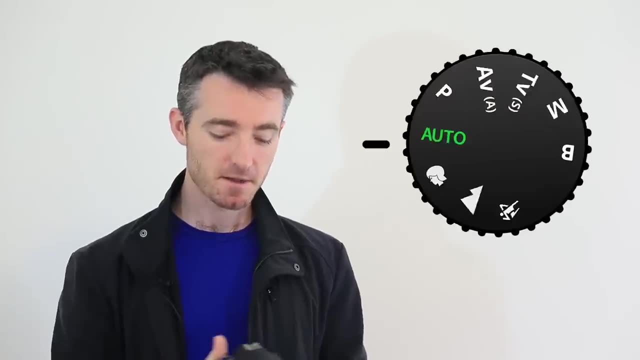 interested in. Now, in auto mode all of those points are turned on and you can't do anything about that. that's one of the big problems of auto mode: you can't even tell it where to focus, But thankfully in all the camera modes we're going to be using on this course. so that's. 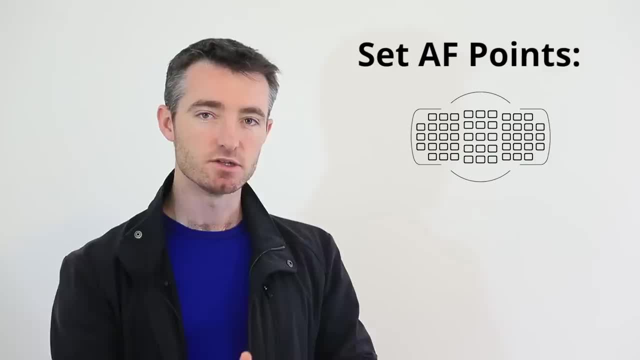 P mode and anything better than that. you can choose exactly which point to use and set it to the centre auto focus point. that's honestly the most useful point to set it on for 99% of your photography, and then it's very easy for you to accurately choose exactly. 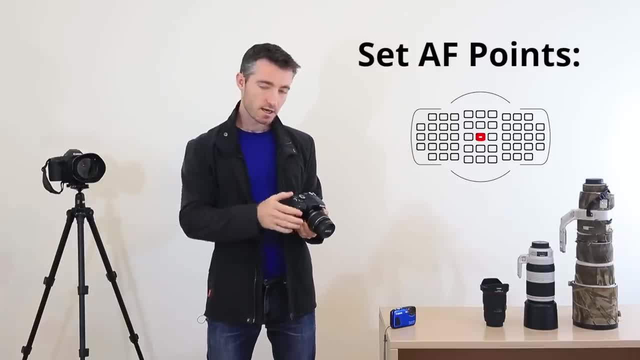 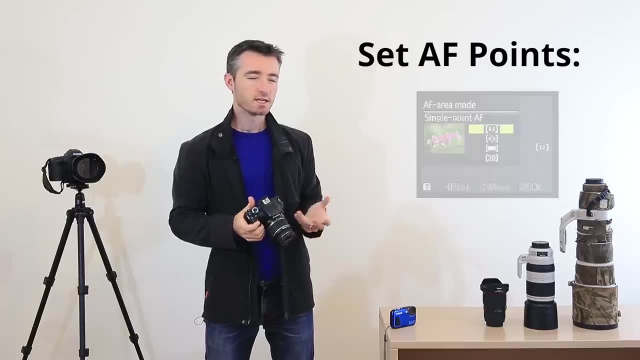 what you want to focus on, To change which auto focus points you're using different brands, different things- but Canon has a little button on it there. you press that and then you can choose between your different points. Nikon in through the menu auto focus area mode and you can just go. 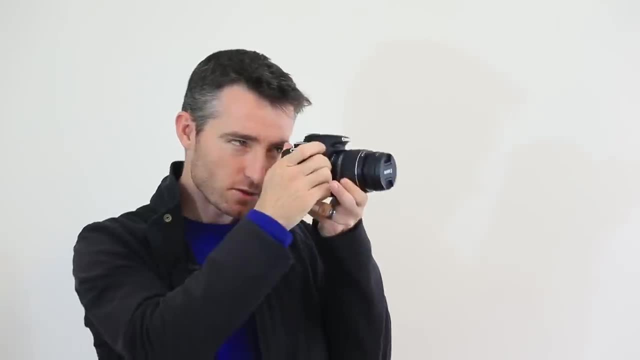 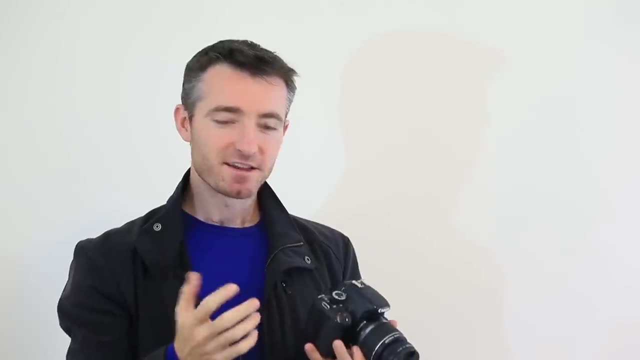 to single point and you can move that wherever you want. Also, if you've ever noticed, as you're looking through your viewfinder, if everything just always looks a bit blurry, That's not your eyes or anything. you've just got to change this little diopter adjustment. 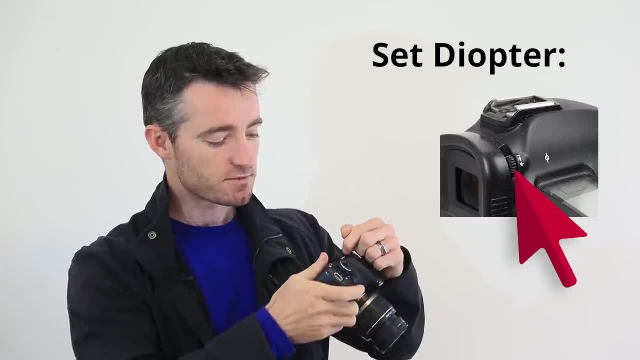 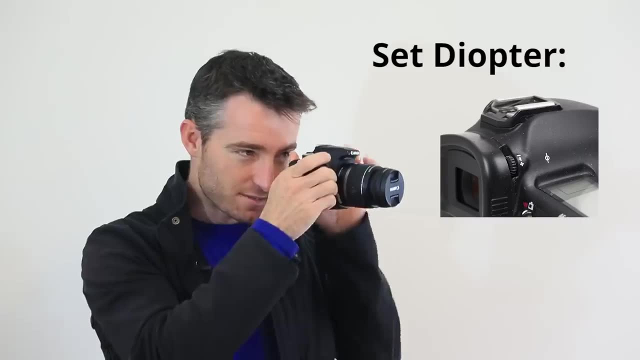 it's like setting the right pair of glasses for you. If you bump this little diopter adjustment off, everything always looks a bit blurry. But not a bad idea to go outside and wake the camera up, press the button a little bit so there's some numbers and things displaying in there. deliberately squiggle that thing. 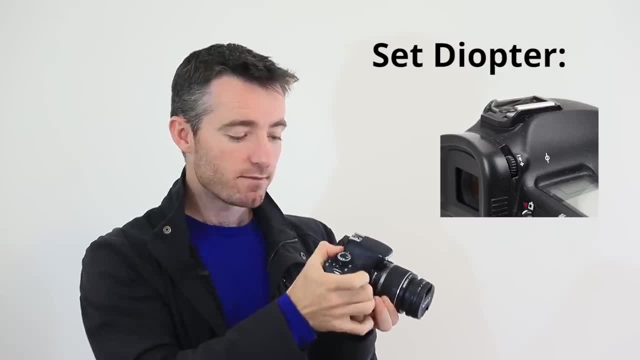 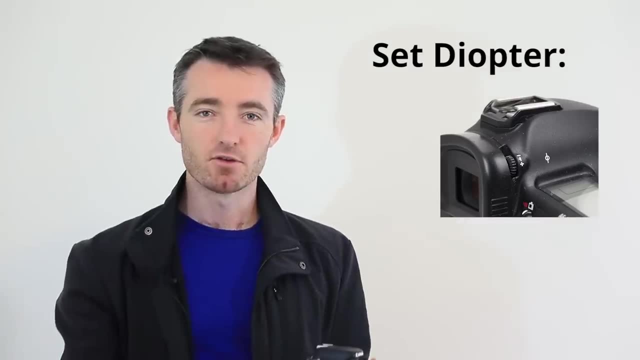 way out of whack and it will all go blurry, and then just move it back and forth until it just becomes the easiest to see and you might find that suddenly it's just so much natural to look through. you don't need to force your eyes to focus on stuff anymore. 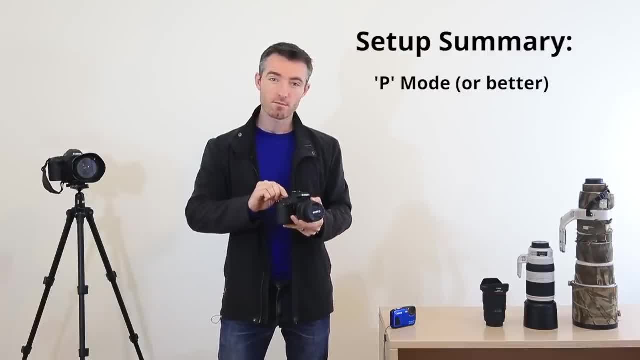 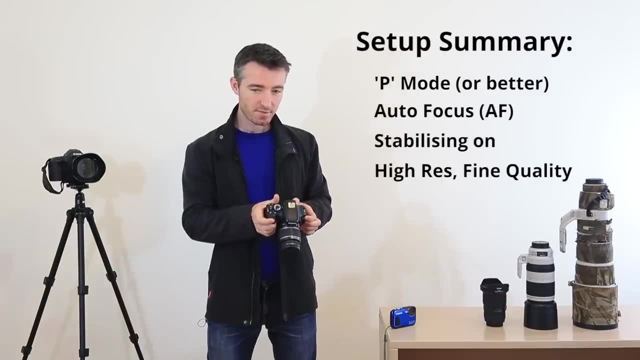 So, in summary, if you're about to start shooting, pick up your camera, check you're in program mode or something better: auto focus on stabilizing, on check you're on the right quality, high quality JPEG. your focus system maybe have one shot, rather than the tracking, and then 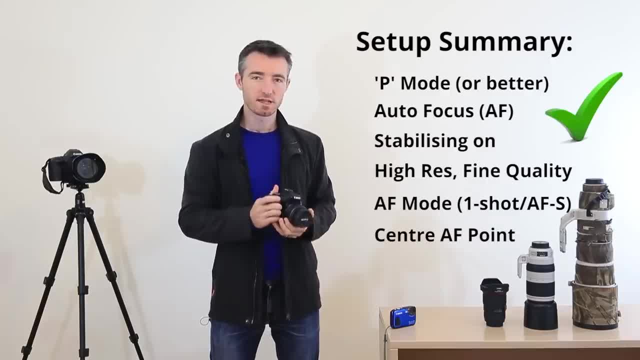 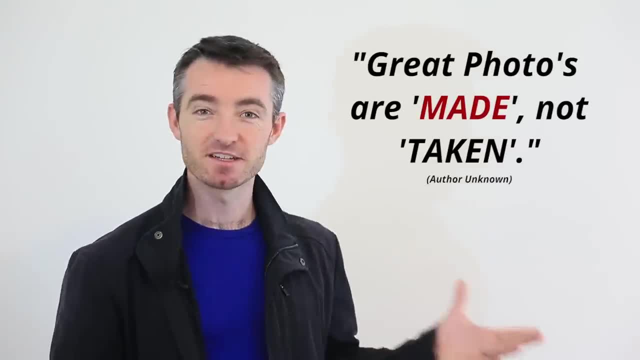 change yourself to the center auto focus point. That's a good place to start. Okay, now that you're all set up and ready to go, the next lecture is on composition, but before we go, I just wanted to leave you with this really tacky, cliche, great photos. 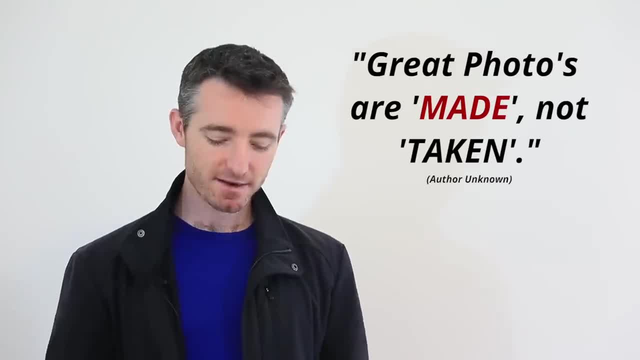 are made, not taken, which is kind of true, though, because you'll find a lot of the best photos aren't just auto mode. they've had a lot of thought put into them. do you want it to be brighter or darker composition? do you put your subject off on the side? do 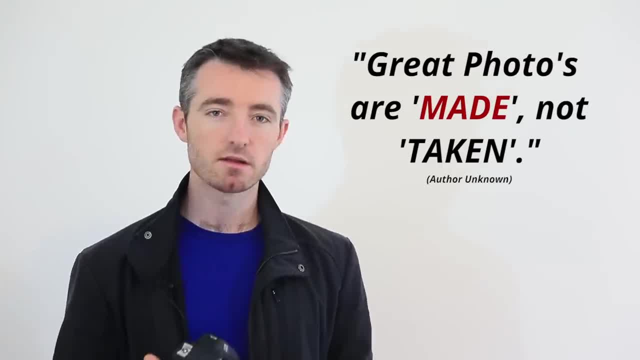 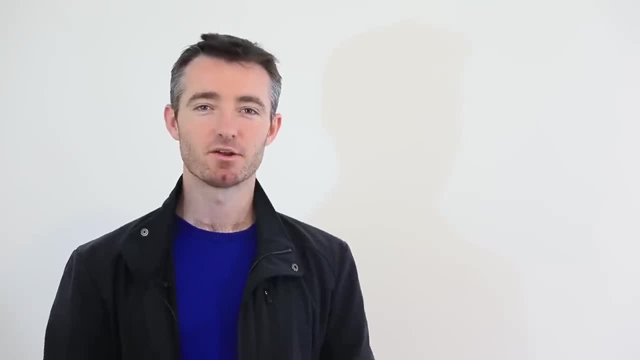 you want the blurry background or not. there's a whole array of different things under your control to make the photo come out the way you want, rather than the way auto mode gives it to you. So that's what we're going to look at from now on. 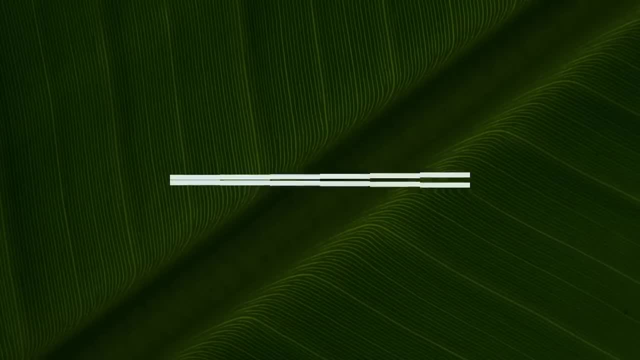 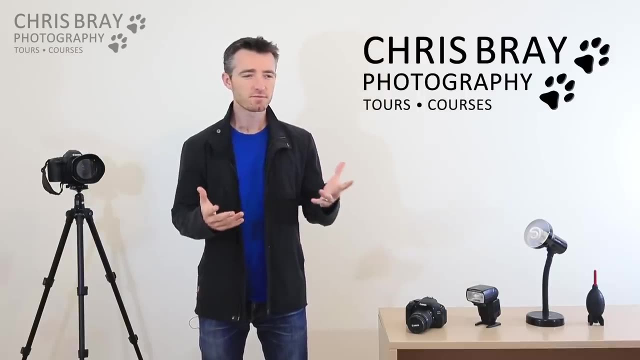 Composition. in this lecture, we're going to have a look at how you organize things in your photo, just so that it feels more balanced or complete. So we're going to have a look at my top 10 composition tips, starting with what you think. 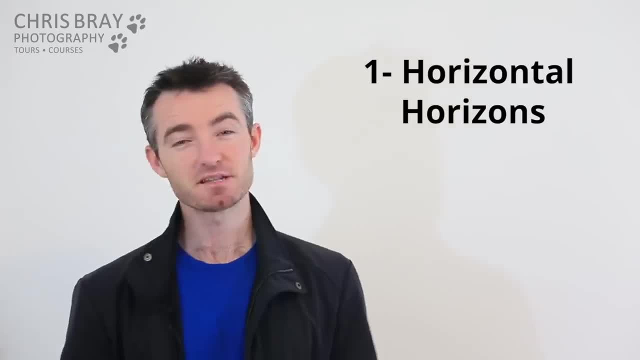 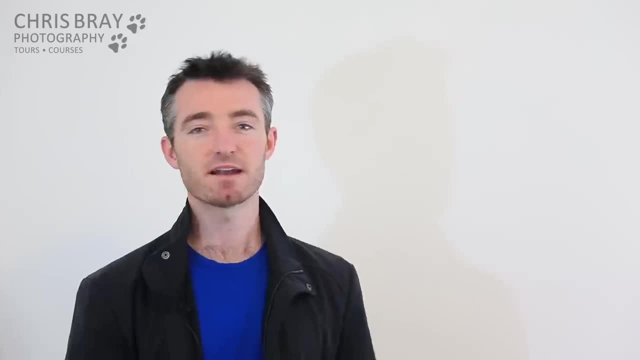 would be an obvious one. try to make sure your horizons are horizontal. but some people just have an inability to hold the camera square and every single photo they take is just a little bit wonky. Sometimes they say, oh, it doesn't matter, it's digital, surely we can just rotate it. 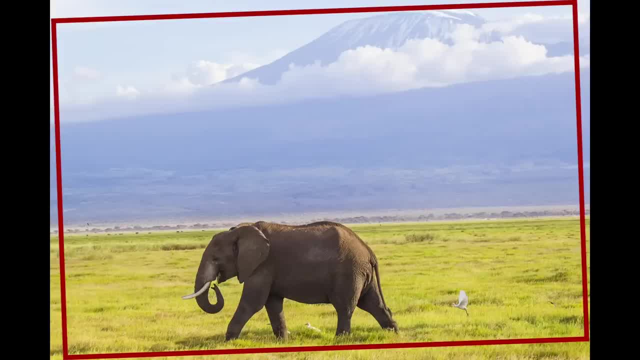 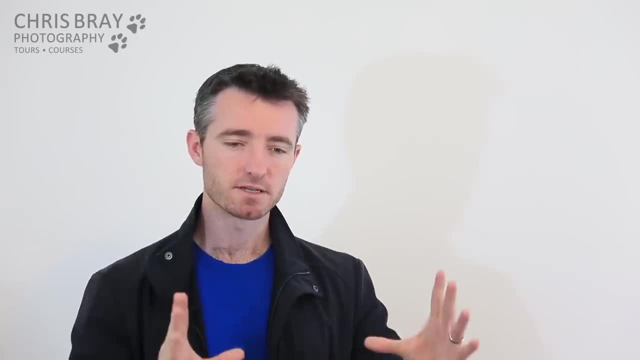 and crop it later on. but you'd be surprised how much you lose in a picture when you rotate it and crop it. Just because it was all in there when it was wonky doesn't mean it'll be all in there or look any good by the time you've cropped it. you lose huge wedges off every corner. 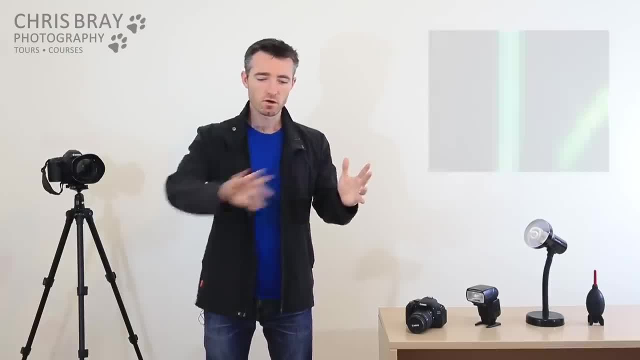 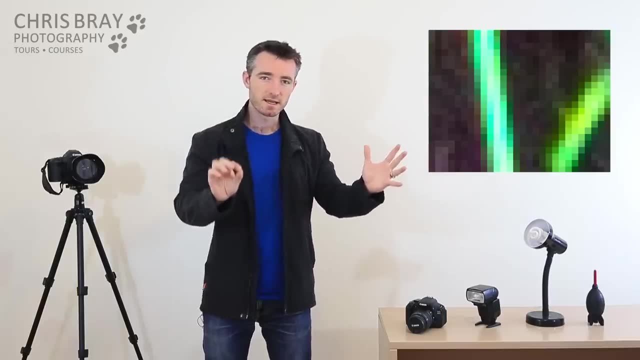 You also lose quality on your image. obviously, photos are horizontal and vertical rows of pixels and if you have to rotate it a little bit and then save it back into horizontal and vertical rows, of course some pixels get smeared from here to here and you just lose. 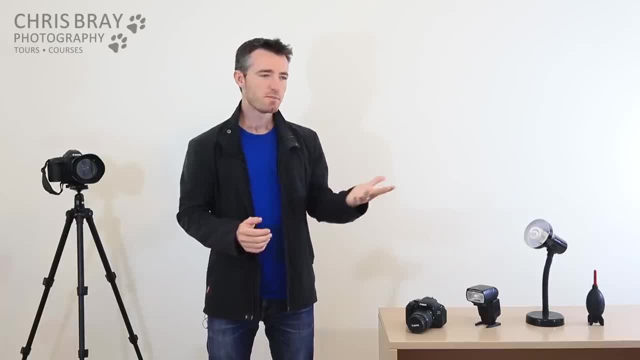 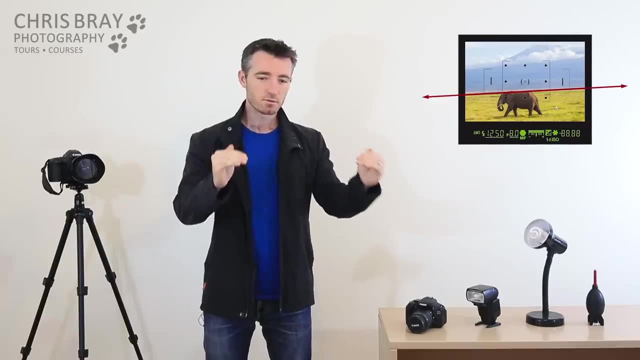 a bit of clarity, So you're better off getting it right in shot. Basically, just look for something that's supposed to be horizontal, like a horizon, and then try and just check that it's parallel with the bottom of your viewfinder, just match. 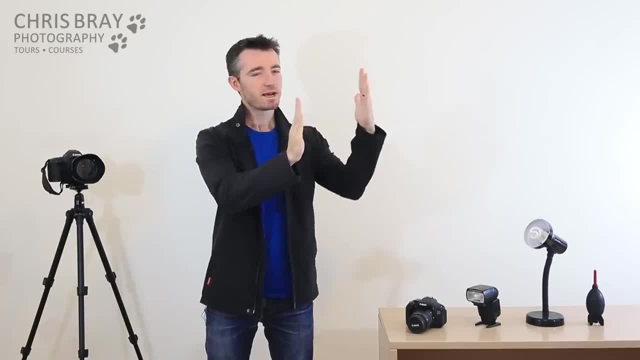 it up just to check it's parallel. or a building that's supposed to be vertical, just check it matches up with the side of your viewfinder. A lot of cameras these days have that inbuilt digital level, which is handy as well. but 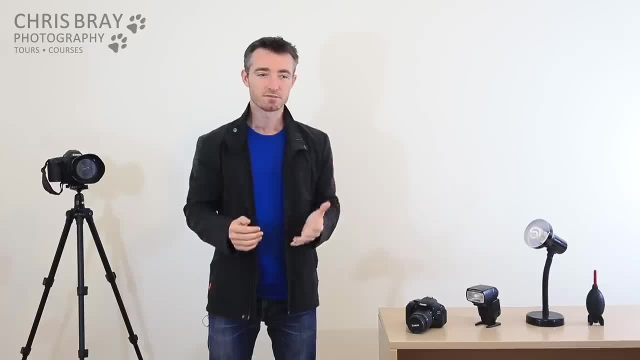 the main thing is just spend a couple of seconds to make sure your photo is square, because it ruins a lot of photos and you don't want to have to try and fix it later. Rule of thirds: you've probably heard of this one before. it's a pretty important composition. 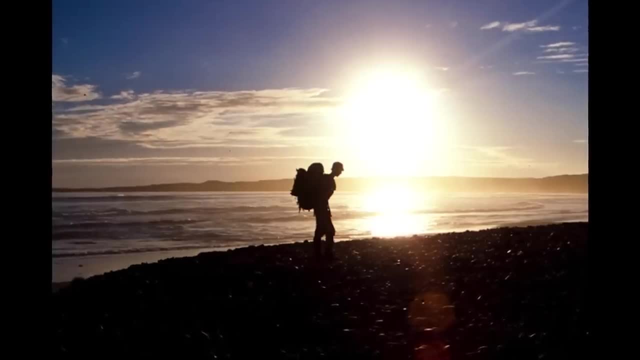 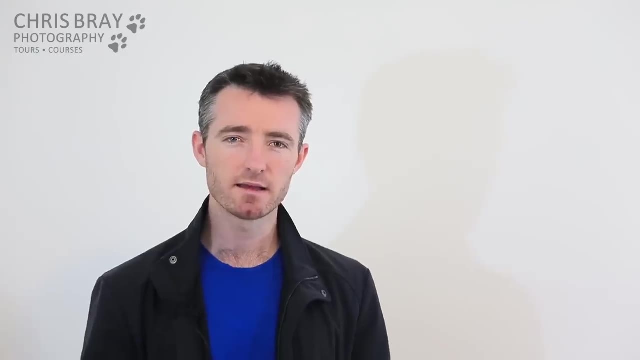 rule. It's basically saying that, yeah, here's a nice enough photo of a hiker walking along a beach, but for some reason this just feels a little bit nicer. it's a little more balanced. It's hard to work out exactly why, but in its simplest form, the rule of thirds is saying: 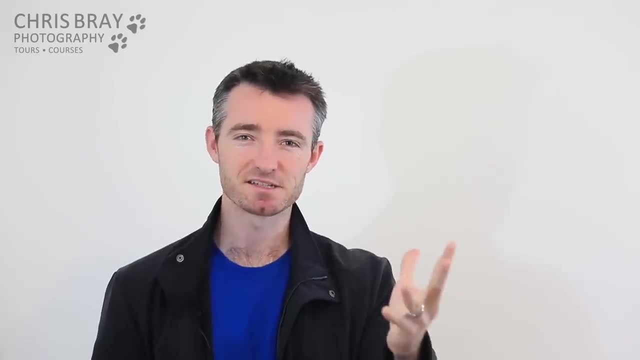 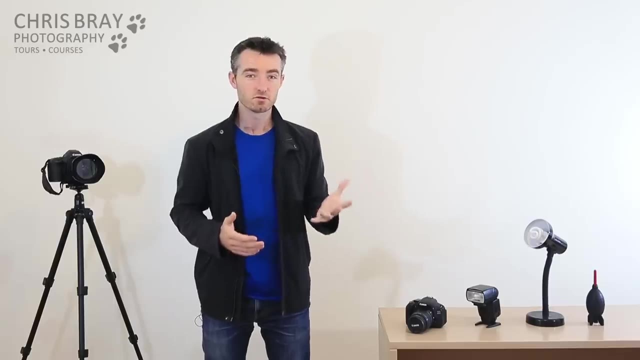 try not to just put your subject slap bang in the middle of the photo, as tempting as it is. It normally looks nicer if you can deliberately put your subject off on the side. give it some space in front of it. Now, what's actually going on here is the rule of thirds. that's just where in your head. 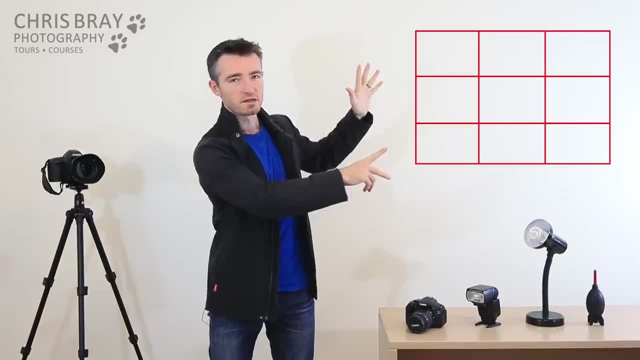 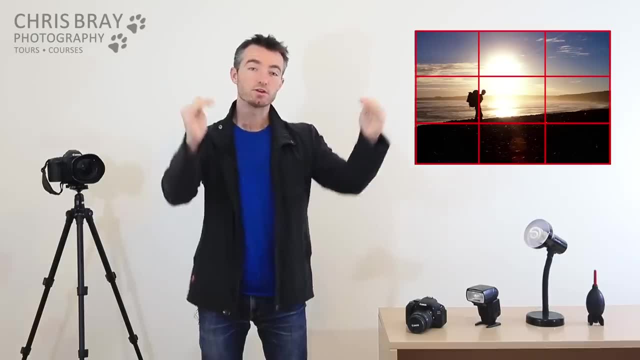 you mentally divide your viewfinder up into these vertical and horizontal thirds and just try and arrange as much as you can of your photo around those lines. So if you've got a strong horizon you might put that on the bottom third or the top third. 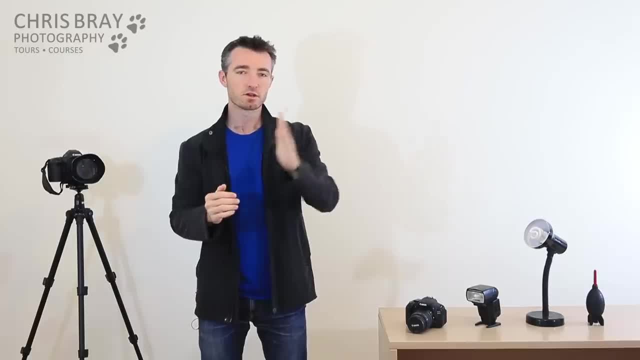 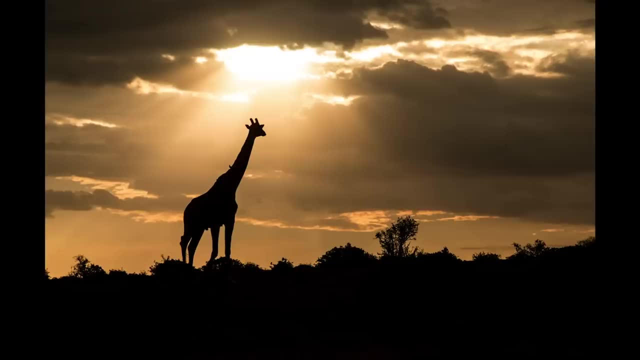 depending on which bit of the photo needed more space or if you're putting your subject off to the side, you might move them off to this third or the other third. Another example here. see, it's just in the middle. it doesn't look that exciting it. 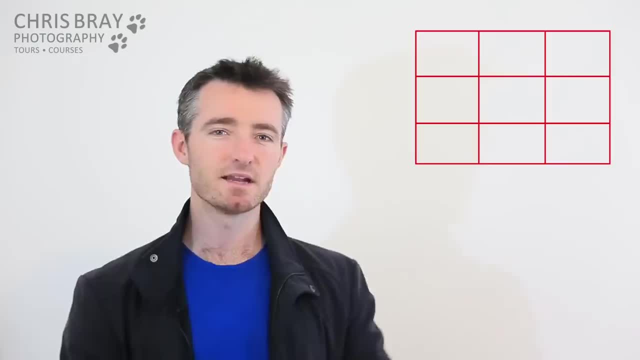 just looks a whole lot nicer when you pull it off to the side, In fact, where those third lines intersect. there's four points in a photo there, if you can put the key bit of your image, either your subject or the key bit of your subject. 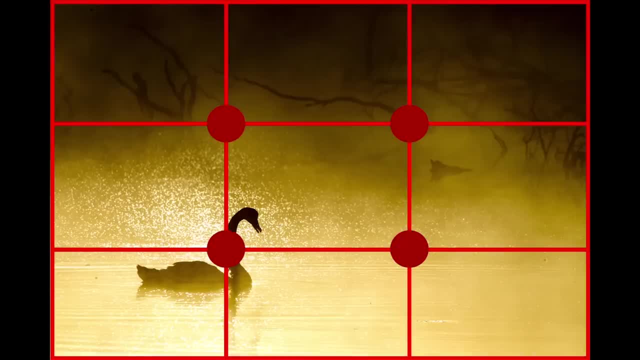 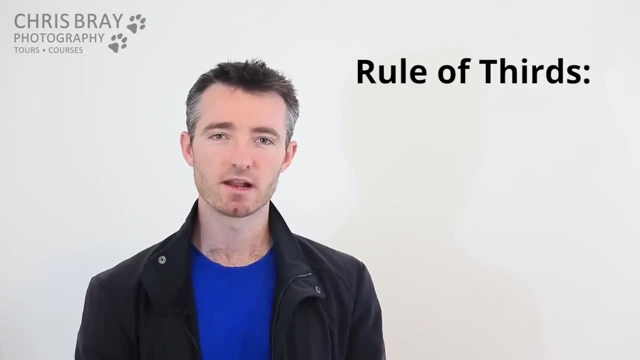 on those intersection points. That's a really powerful point in the photo and it looks really good. Sometimes you can have a bit of a dilemma as to which side of the photo do you put your subject on which third, and you can just try and remember it. as always, try and give. 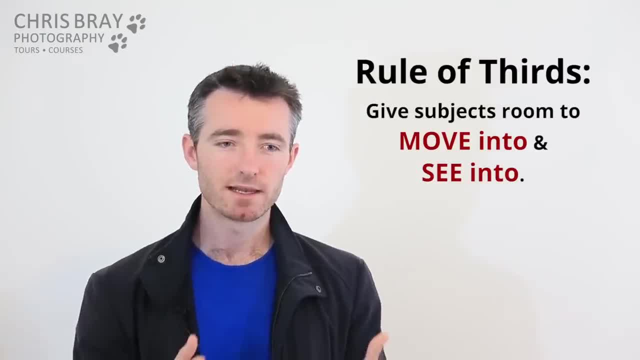 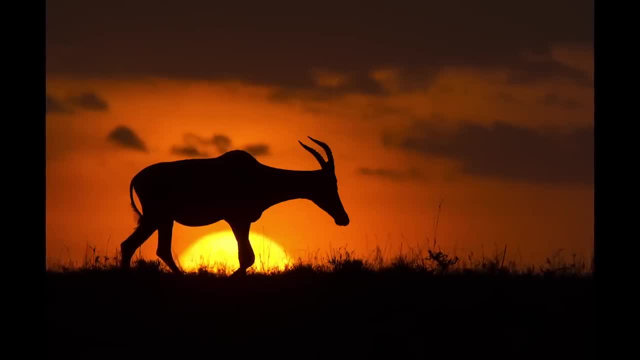 your subjects room to move into or see into. you know if they're looking or moving in a direction. no one cares about what's behind them, what's been and gone. they want to see forward. So you crop out all the stuff behind them. give them extra space in front. some people. 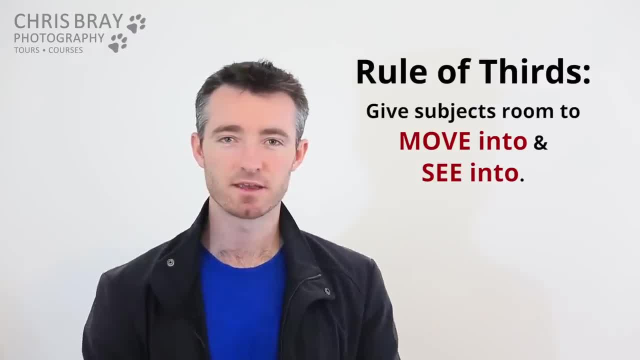 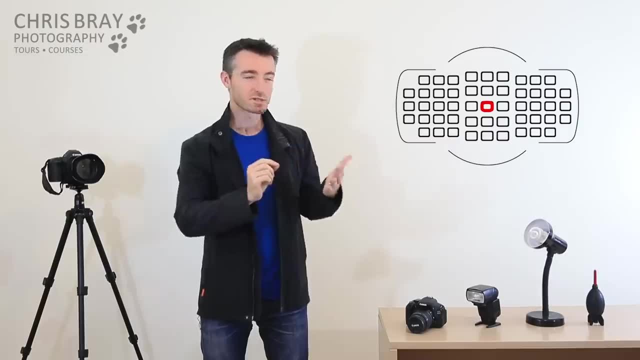 call that nose room. you're just giving space in front of things. that's the same thing as rule of thirds. Of course we all have a bit of a problem now because in the previous lecture we all went and put our centre autofocus point on, so the camera was only going to focus what's. 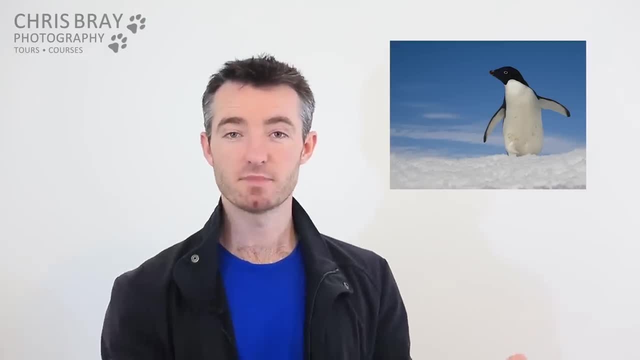 in the dead centre of the shot. Now here I am saying: oh, but it looks so much better if you put your penguin off on one third. Now, what that does mean is you do point directly at your subject, first of all, while you're. 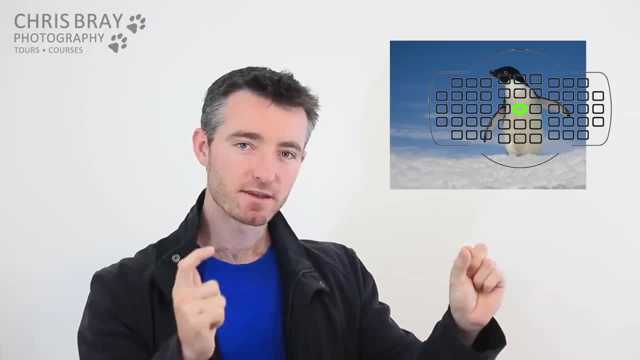 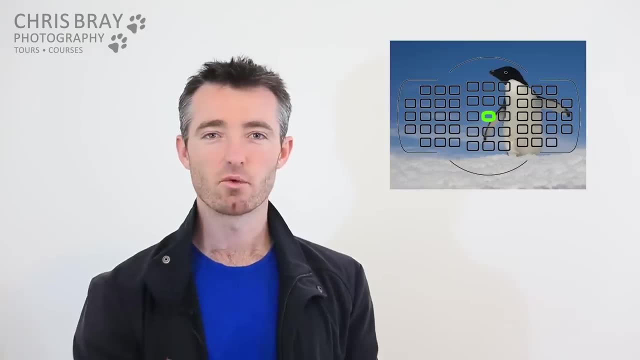 focusing beep and then, after it's found that focus lock, keep your finger half pressed and then you can reframe the shot and put your penguin off on the third or whatever you want for good composition before you depress the button all the way down to get. 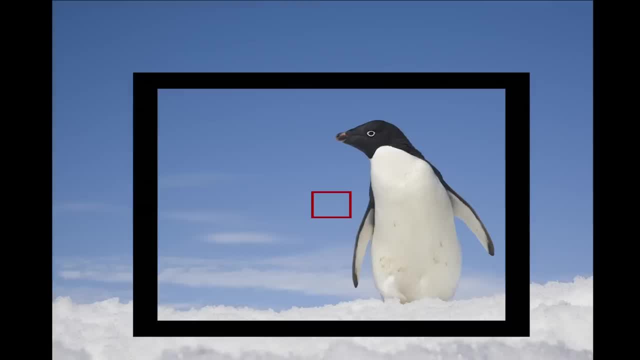 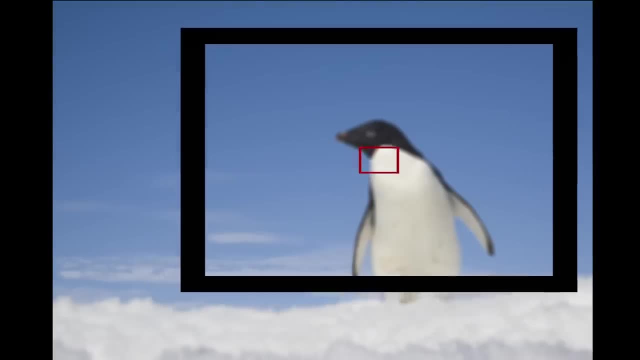 the shot. So if you go off with your penguin off on the side and you try and half press to focus, it's just going to focus on the sky behind the penguin and you end up with a blurry subject. So you point directly at your subject to start with, ideally focus on its eye. actually that's. 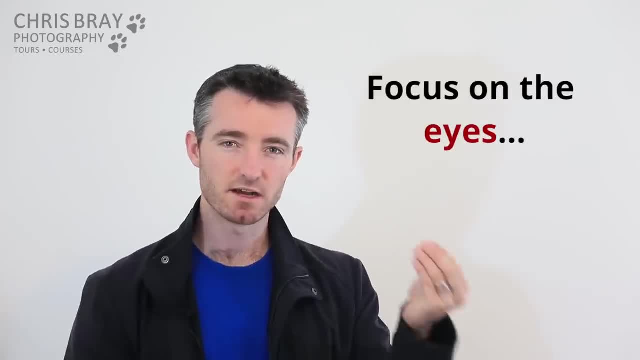 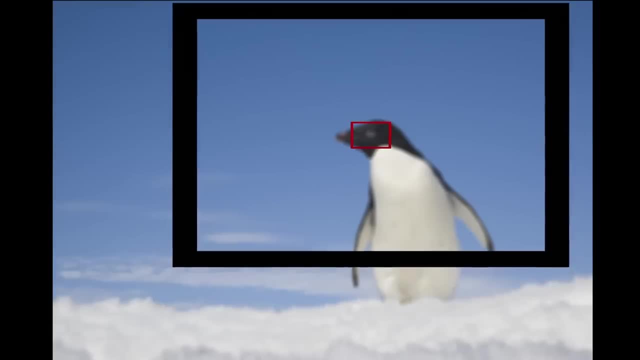 a good side tip. if you're ever photographing a person or an animal and you can see their eye in the shot, that's what you've got to focus on. that's the important part that has to be sharp. So here you'd just be focusing on the eye of the penguin. half press beep until it. 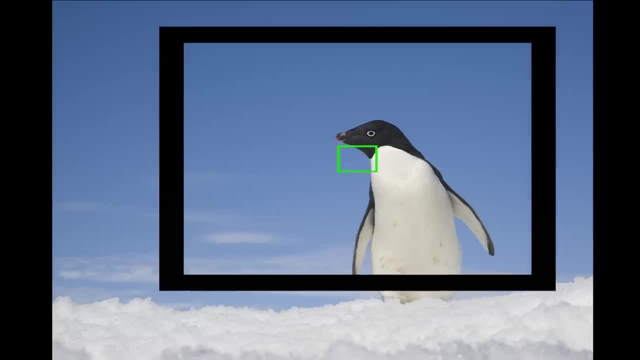 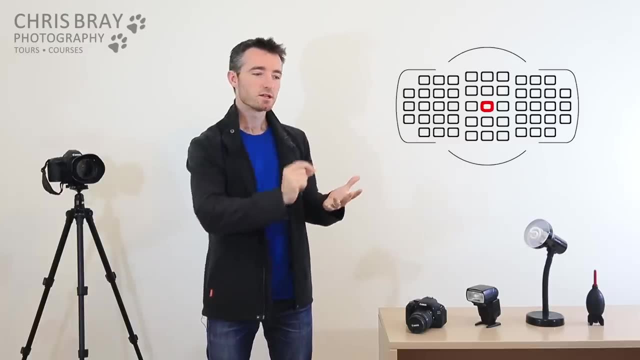 gets the focus, then you keep your finger half pressed while you reframe to the side rule of thirds, and then you depress the button all the way. perfect. So there you go. that's how you use that centre autofocus point to allow you to focus on exactly. 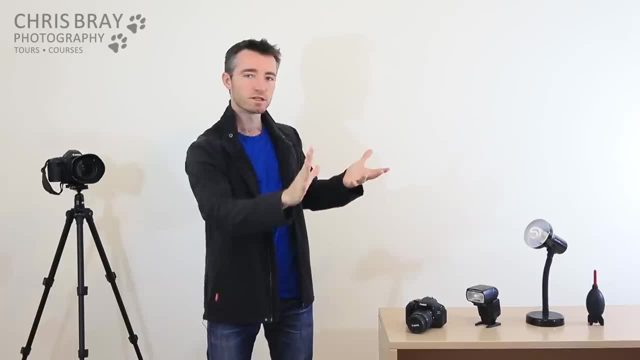 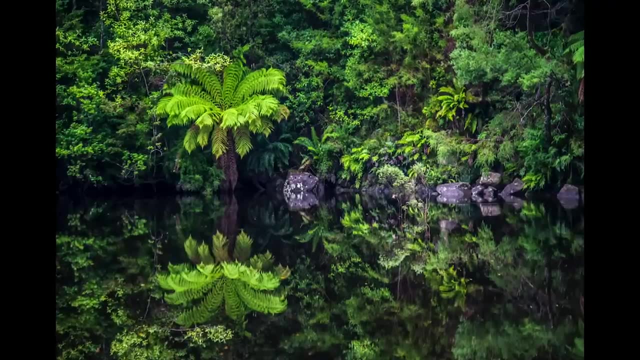 what you want in your image, but you can still then recompose and put it wherever you want in the photo before you take the shot. That's why you have that AF-S or single shot focus rather than the tracking system. I think about the only exception to the rule of thirds are reflection photos, where you 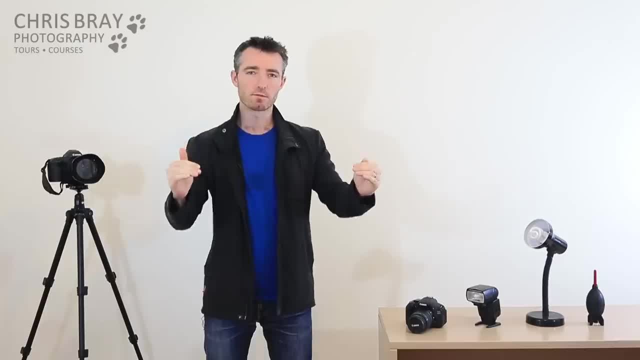 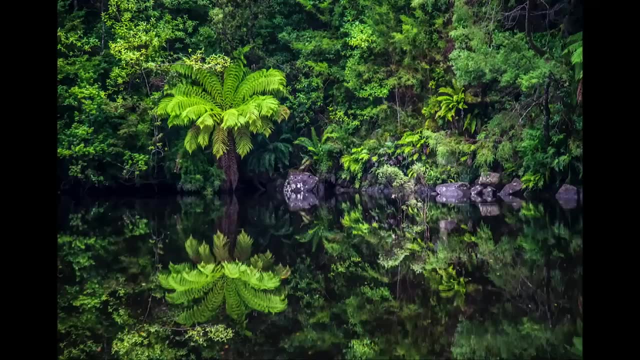 don't feel like you have to put that horizontal division on the top or bottom. third, because the symmetry of what's going on is what makes those photos beautiful anyway. but I think vertical plane still applies. But the key part of the photo where your eye is drawn to is obviously that tree fern. so 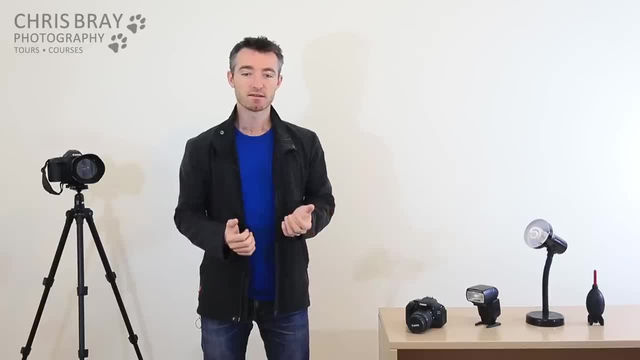 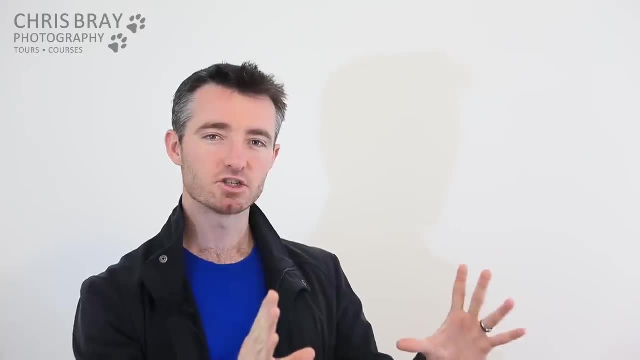 that's in the top third corner and bottom third corner kind of balances it out vaguely, still fitting the rule of thirds. So try and imagine this is a view out the back of a boat that you're on and you're trying to get a nice postcard shot of this bird and the sunset and things like that, using 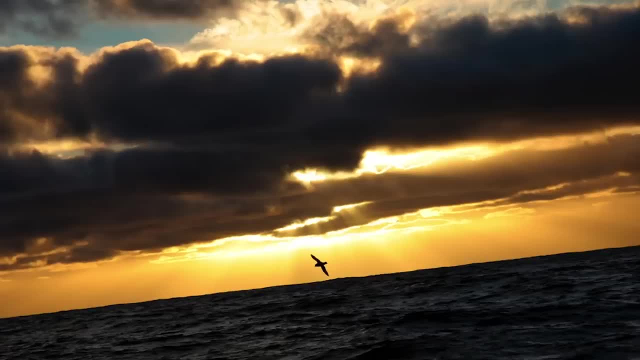 the rule of thirds. Have a think in your head how you might frame that up. Hopefully you're thinking something along the lines of that. You can see your horizon is obviously your strong bottom third, the clouds make the top third line. there's our little bird. he's the subject, he's moving into the shot. so 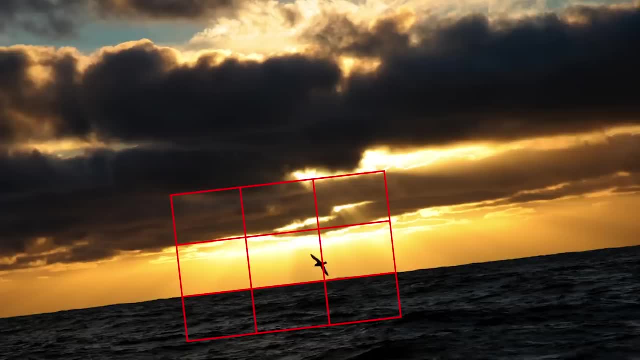 we want to give him space to move into, so we move him off to that right hand. third: But then you'll have some people jump up and down and say, oh, but you missed the lovely golden lighting over there and the blue sky at the top. what about that? 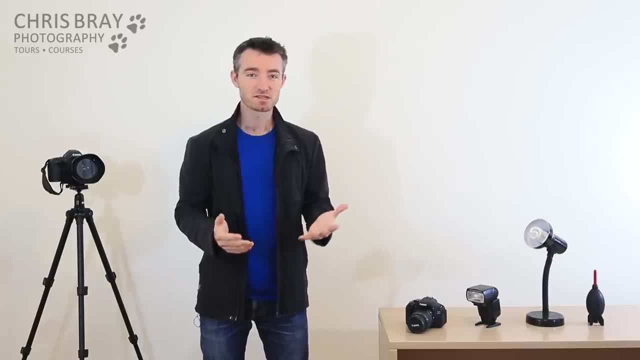 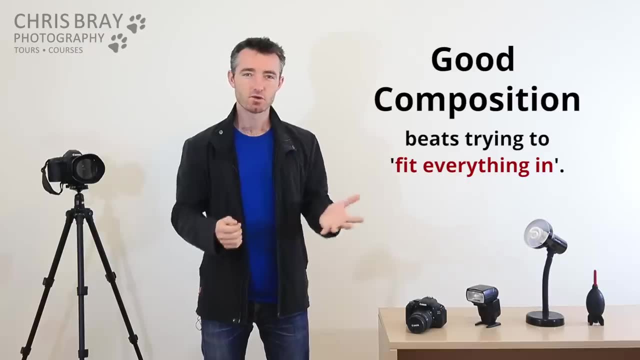 And it just goes to show that the world doesn't always fit into nine magic boxes and you've often got to make a call between good composition and trying to fit everything in, And I really think it's always important to try and have good composition. 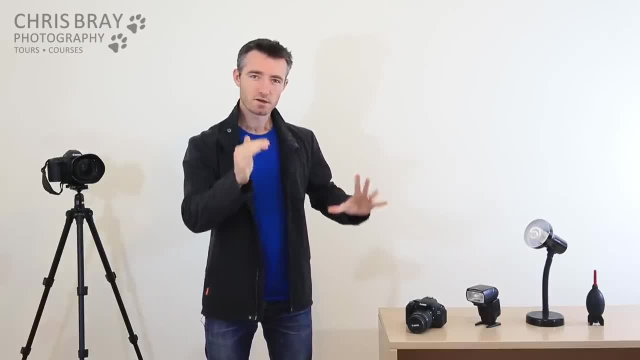 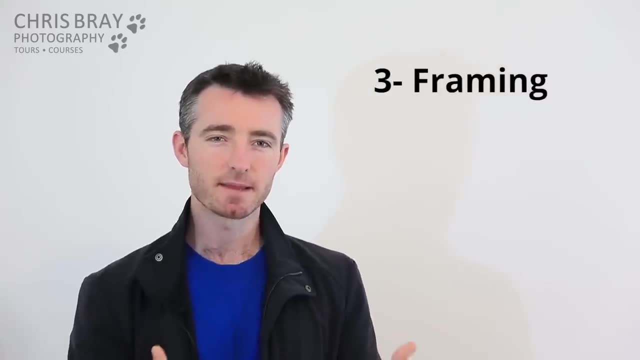 People don't know what they're missing if you don't include it in a photo. but what you include, It's got to look nice. Framing is another good tip. this is good for your landscape photos particularly. Framing is when you deliberately include something up close in your photo. it tends to make it. 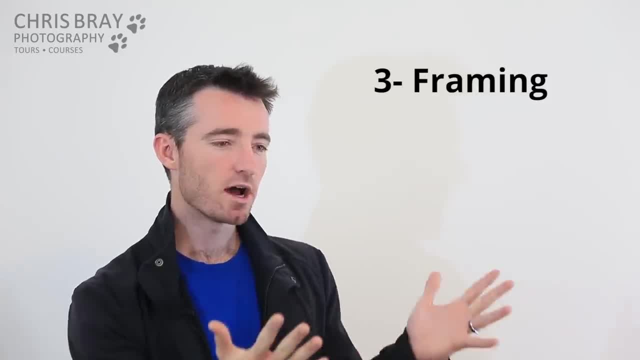 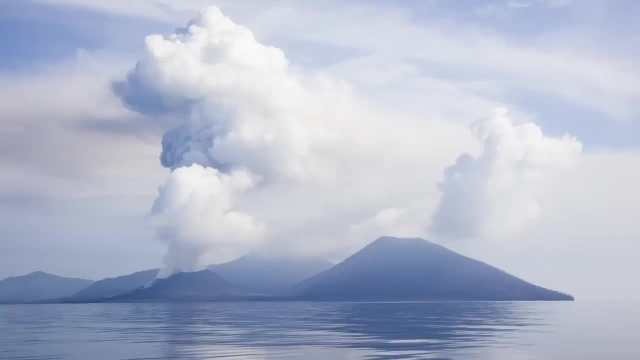 seem a bit more. 3D gives it a lot more depth. it also stops your eye falling off the edge of the photo. you kind of frame it or hem it in by putting something along the edges and the sides. Look at this example here. this was taken in Papua New Guinea. you can see some nice 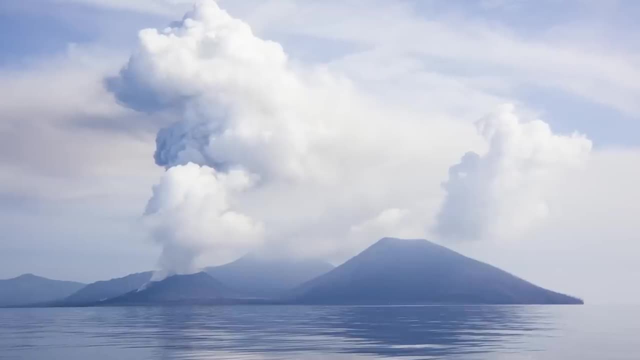 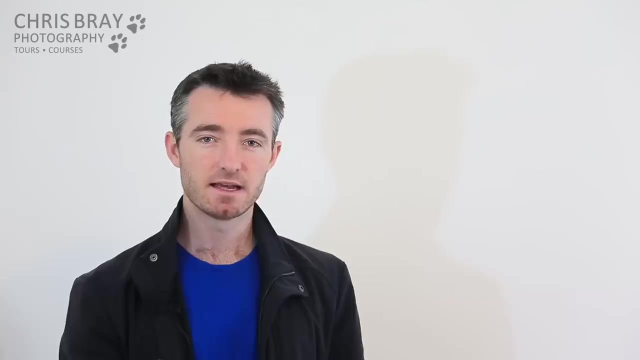 volcanoes puffing away, but it does look a little bit flat compared to this one, which just has so much more depth to it, And that's because I've deliberately got some close up foreground elements there. As you can see, it also tends to pull our attention back towards the middle of the photo again. 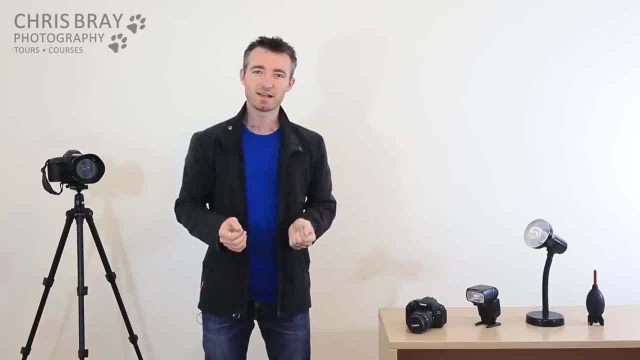 stops your eye just slipping off the edge- And you probably have to admit that a lot of people make this mistake with their landscape shots- where you know you get to a lookout and the first thing you do is you get everyone out of the way and if there's a fence there, you've got to get over the fence, because that's. 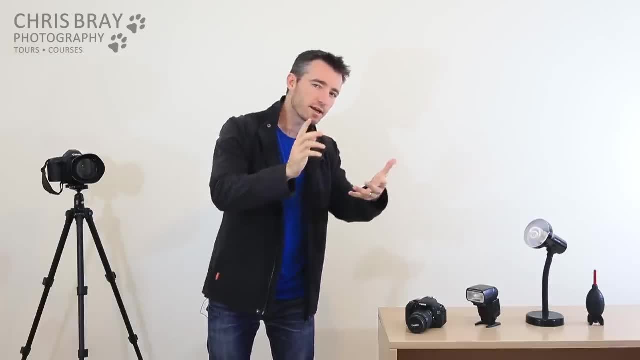 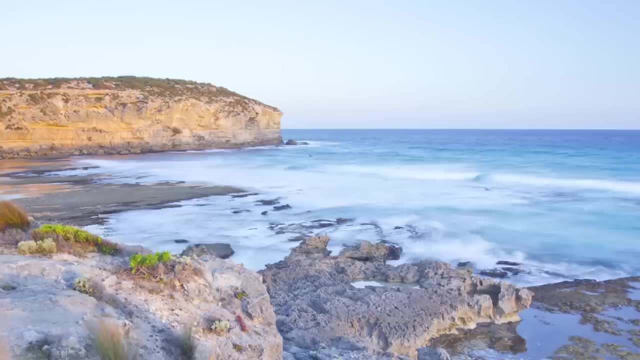 in the way and if there's a tree, you know you almost fall off the edge of the cliff trying to get away from the tree to cut that out. and you go to these great lengths to get an unobstructed view of the distant mountains. but then the problem is everything in your 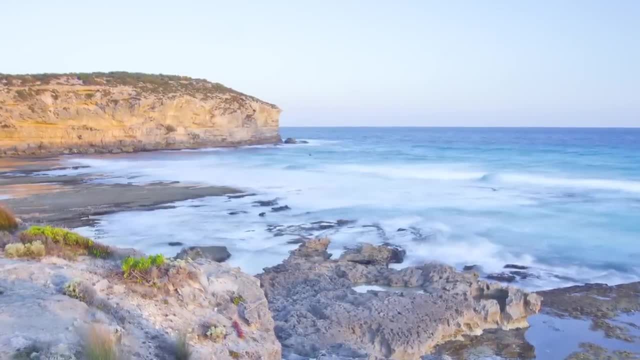 photo is a million miles away and it just looks flat. You're better off crouching down and trying to find a tussock of grass that you can pop up into that corner. or if there's a tree there, great, use that frame. half you shot. 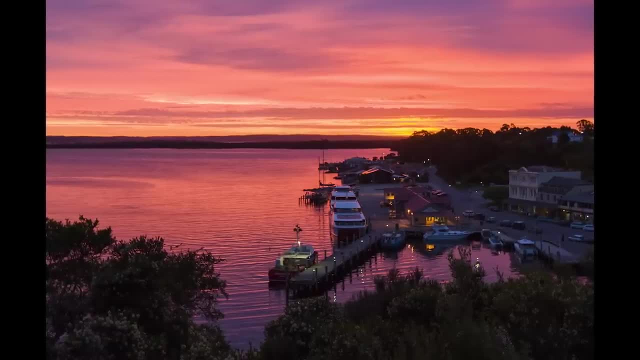 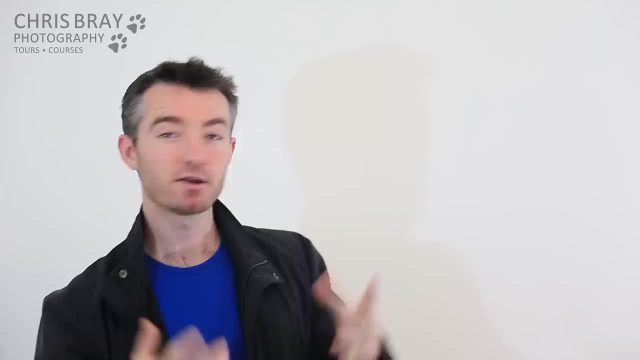 off with that, Same with this example sunset- not a particularly good photo, but it was a nice sunset. but there was this stupid tree that kept on putting branches in the left hand side of the shot and I had to keep on edging off to the right. I almost fell off the balcony trying to get. 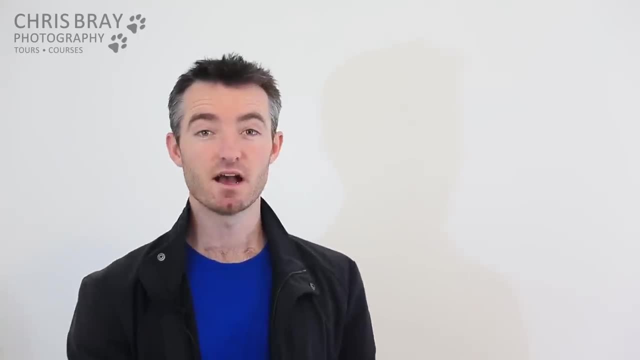 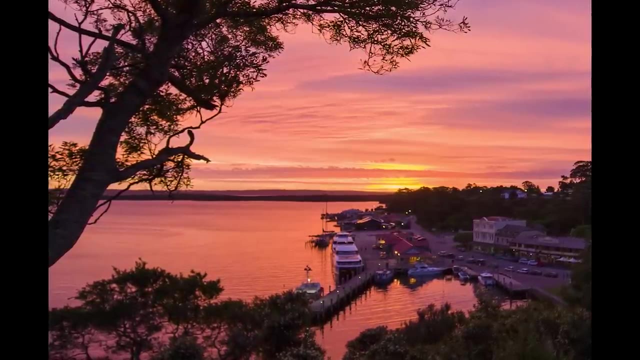 a clear view of the sky until it finally dawned on me that it's probably nicer to let that tree come into the shot. So it frames off that side of the shot, Looks at more 3D, pulls our attention into the sunset. looks a whole lot better. 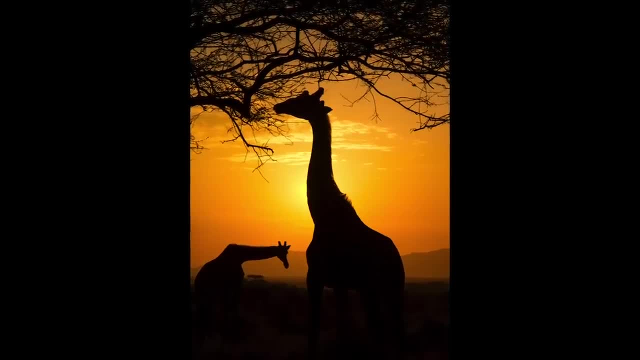 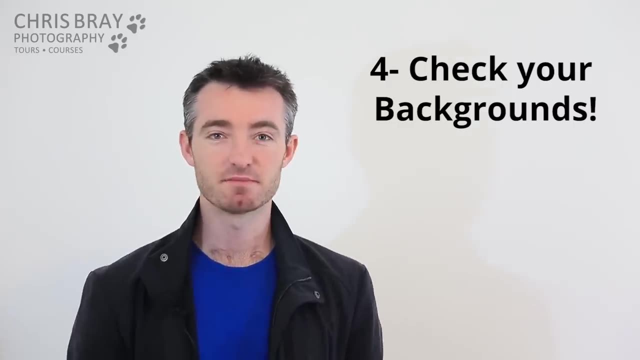 Another one here, including those bushes up the top, just frames off the top of the shot. Check your backgrounds. This is my favourite tip from the entire course. actually, it's the easiest way to make your photos just look 10 times better without having to do any kind of complex theory or anything. 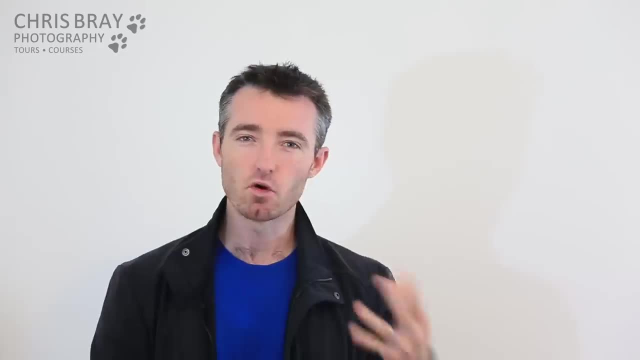 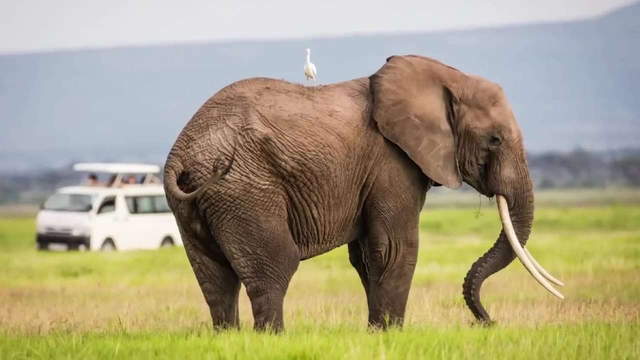 at all. The problem is, the human eye is really good at ignoring what's going on in the background of your photo. It's not until you get the picture back, and then you'll be like, ugh, really distracting element back there. 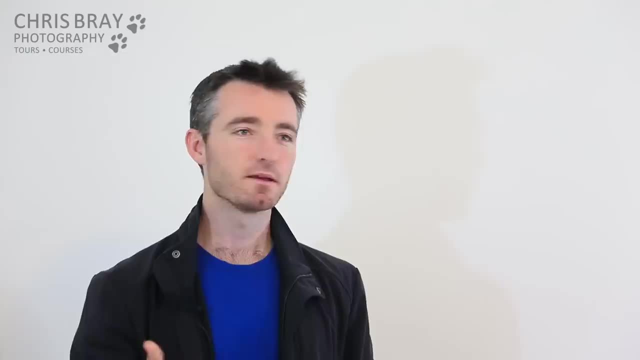 It can completely ruin the shot. the car coming out the back of the elephant, or it could be a power pole coming out of someone's head or a bright yellow car in the background. that's just really distracting. But the thing is it's like another whole level of consciousness you'll finally get. 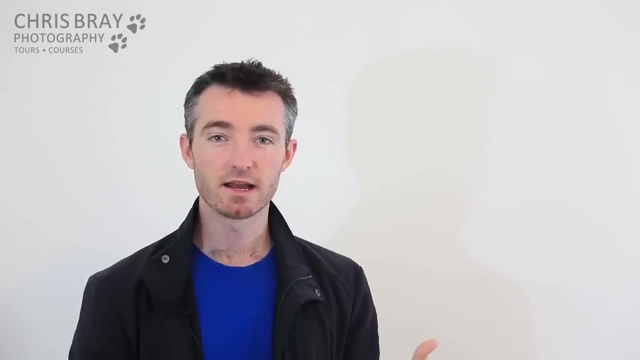 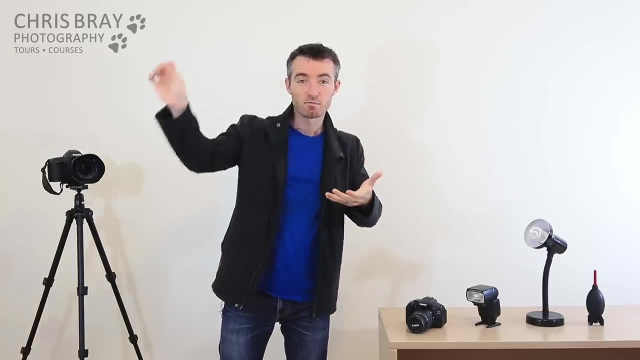 to with your photography, where the background is just one of the things you'll remember to check And you'll be like background, wow, that's really awkward. If I just move a little bit to the side, you don't have a telegraph pole coming out of. 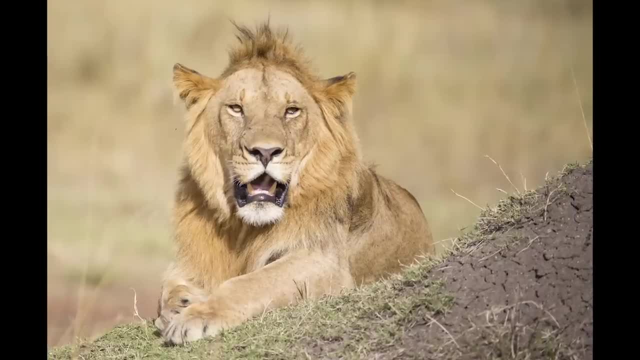 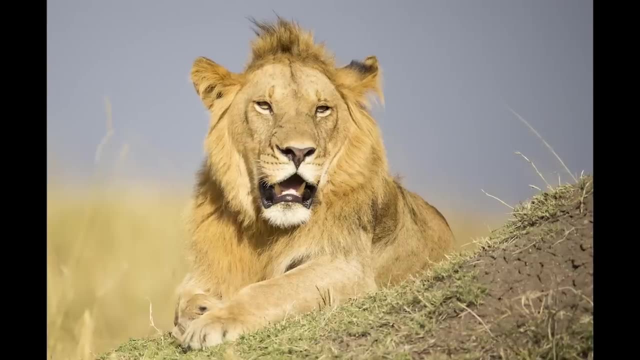 your head anymore, or whatever. it is Like this example with the lion. you know the lion just blends in too much with the background. you know it's the same color as the grass, But if you get down lower you can get him against a bit of the sky and he just pops. 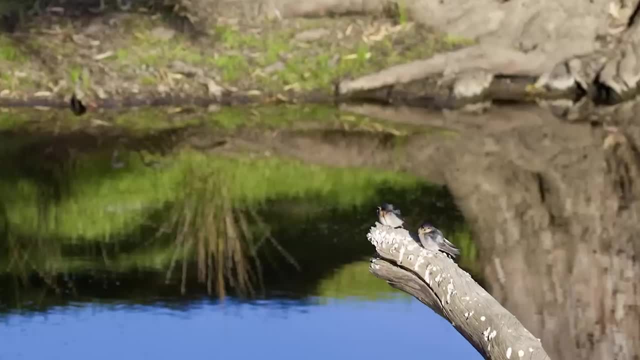 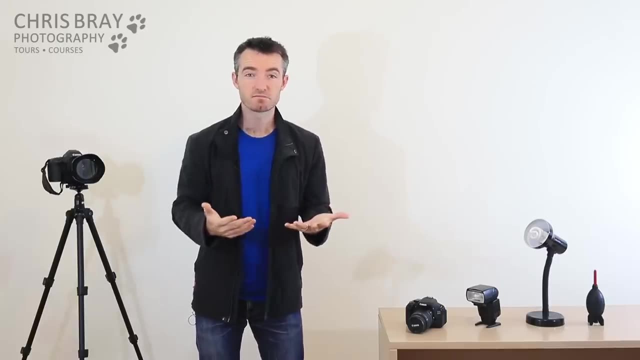 out there much nicer against that blue background. So what about this example? On Kangaroo Island? I was photographing these little birds on a stick and you kind of sneak up as close as you can get and you think that that's probably the best place to take. 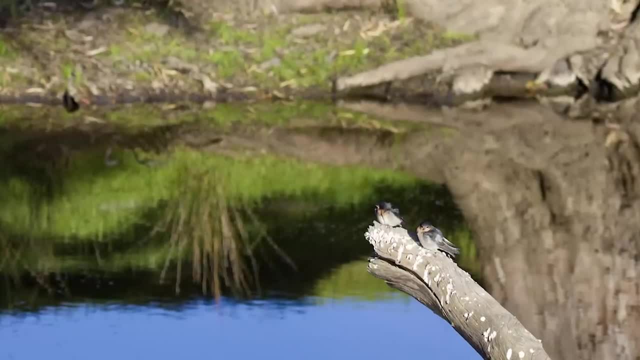 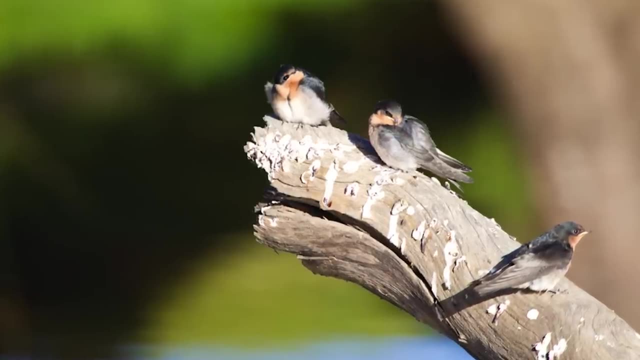 the photo from. But look at the background behind the birds. there You've got blue, brown, green. No matter how good your lens is at blurring it out, it's still a really terrible background. The birds are dark and the background just behind them is dark and they all blur. 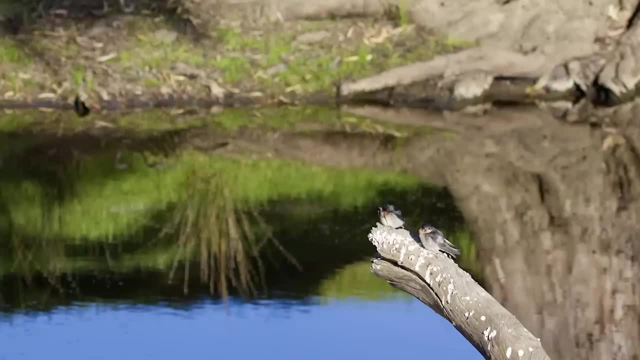 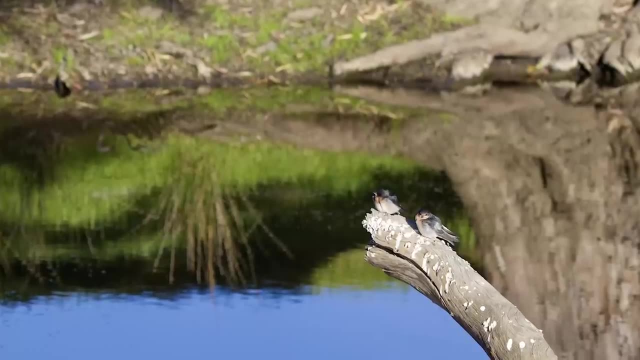 They all blend in. you can't really see them. You've got to look around and say: where can I find a nice, clean, contrasting color to use as a background here? What are our choices? Really, it's just the sky reflected onto the water. 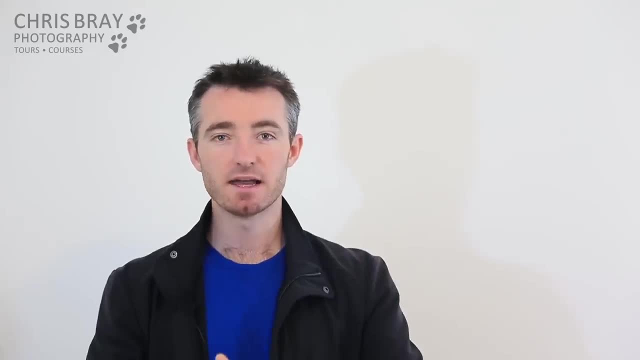 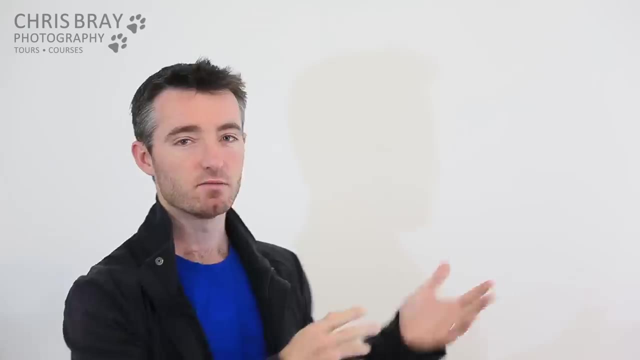 That nice blue color, That'd be fantastic. So you've somehow got to get that behind your subject. Could be a case of just getting a little higher, like tippy toe job, Or in this case I actually had to walk slightly back up the riverbank, which seemed kind of. 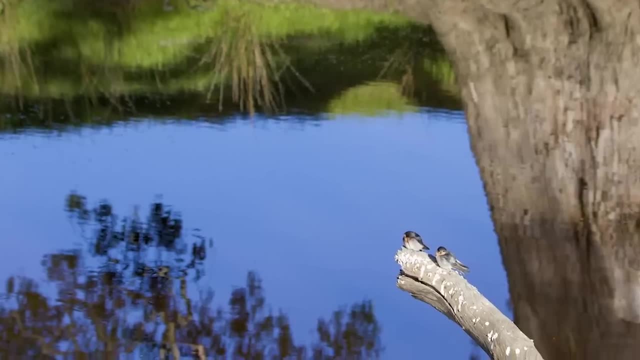 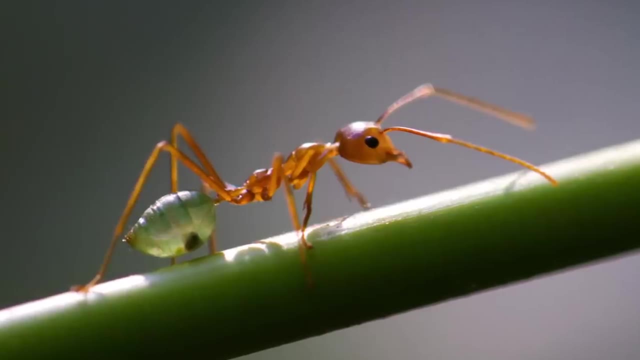 counterintuitive because I had to walk further away. but then you can get the most amazing blue uniform background that just looks spectacular. Well, That one, An ant on a stick, That grey background there, That's just the road, Like the asphalt on the road. 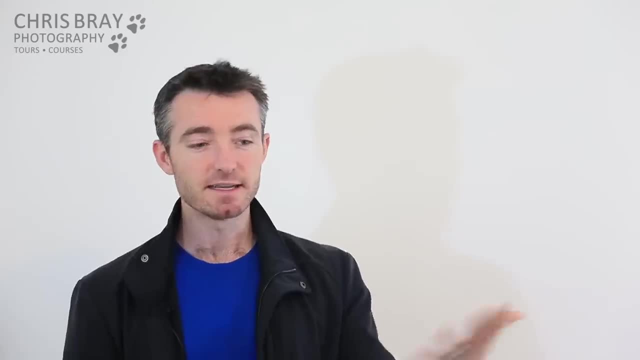 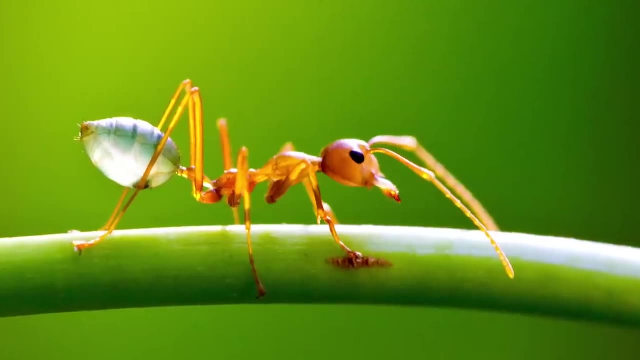 But you can see there is a bit of a green glow to the side there. That's actually a leaf just out of shot. So if I move the camera about a centimeter to the right, you can end up with a green background which looks so much more beautiful. 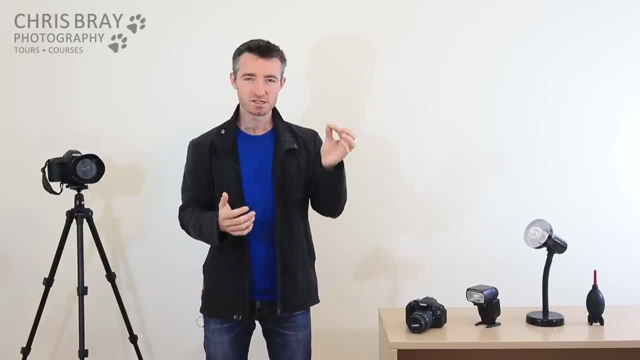 Honestly, if you can just remember to glance into your background when you're taking a picture and just check if there's any distracting elements there, or if you can just turn a bit and get a cleaner, contrasting color, it makes a world of difference to your photos. 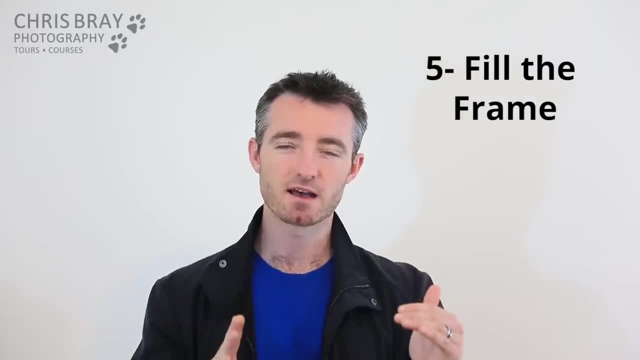 Fill the frame. Sometimes I think photos just could do with being cropped in A little bit tighter. People have this urge to try and fit everything in, all the extremities And often the most important part. if you could just concentrate on that, it's a much. 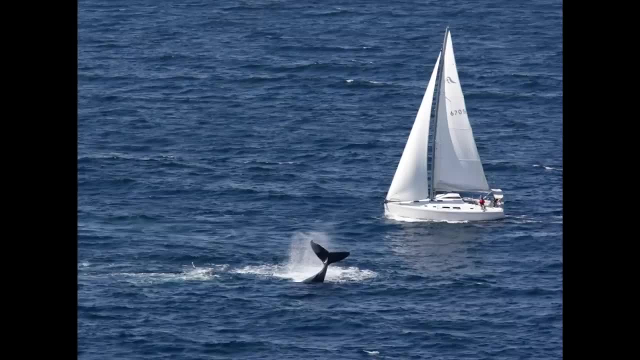 more usable photo. Look at this one. That might be the way you're tempted to take the photo because you want to fit it all in, but actually that's probably better. In fact, that is a far better composition for the shot. We all know that yachts have a big pointy bit at the top, and that's not what we're interested. 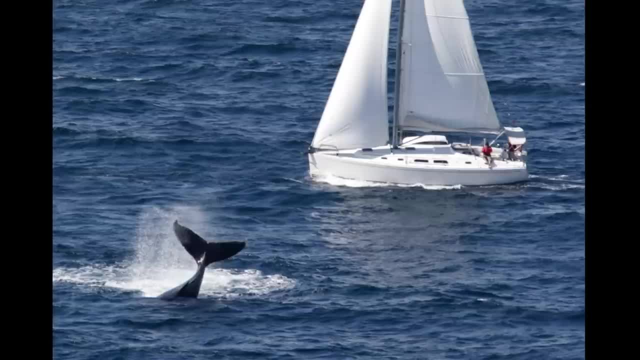 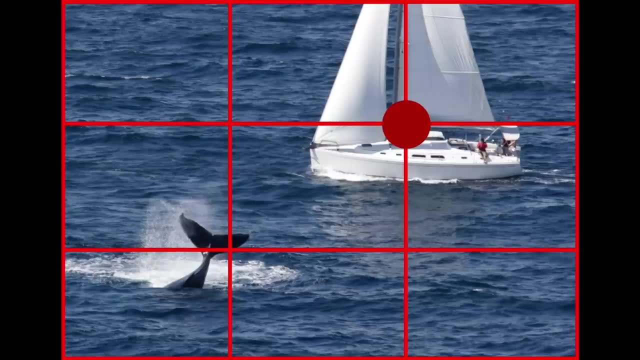 in this It's just the interaction between the whale and the yacht, And now that we've zoomed in more the subjects are bigger. it's more interesting. you can see the detail. It fits the rule of thirds. So we have the yacht on the top third intersection, whale on the bottom third, so they kind of. 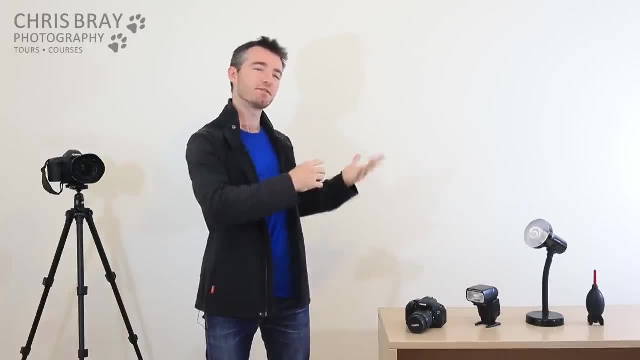 balance there. Or this example: I was trying to keep swimming as far ahead of this lady as I could so I could turn around and get her all in shot. but if you had to summarise that photo, you'd probably say that's a woman swimming with a blue starfish. 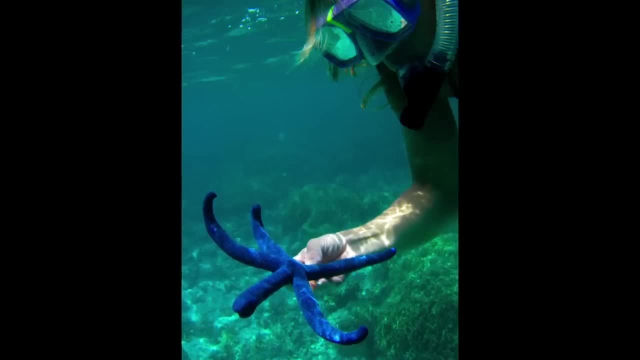 But really this is exactly the same thing- A woman swimming with a blue starfish- But it's a much simpler, cleaner sort of shot and it's probably more usable. You could imagine that in a little brochure on a local dive resort or something. 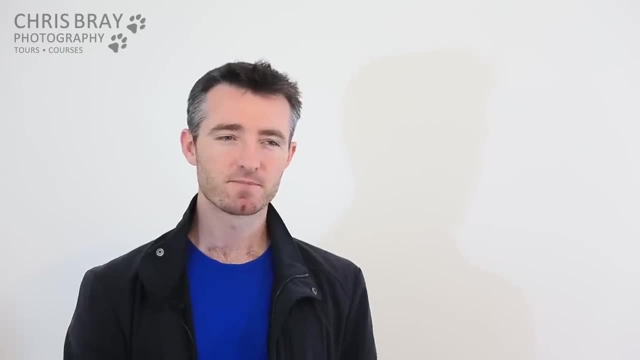 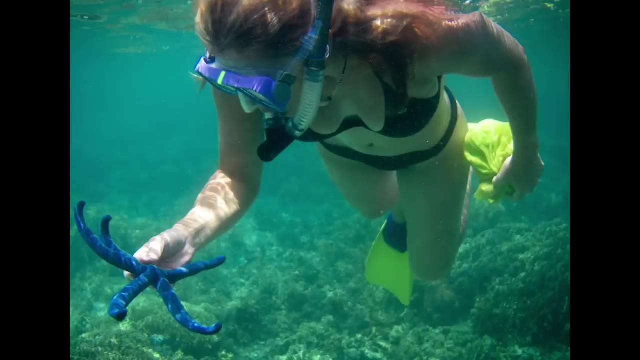 Not that she should be picking up starfish, But compared to the other photo, there's just too much stuff going on there, Too distracting. You're like: what is that yellow thing she's carrying? It's actually her shirt, but it looks like a bag. 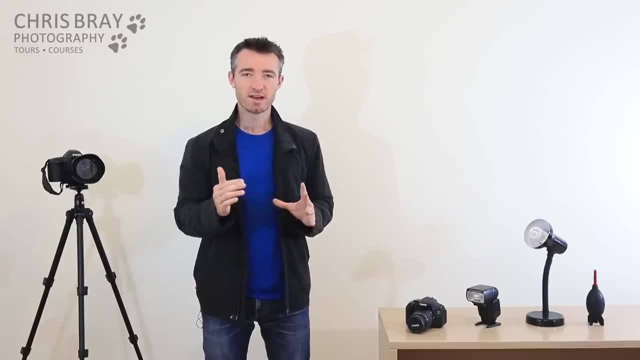 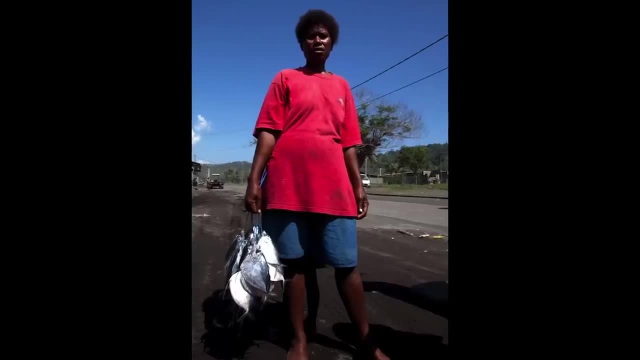 Is she stealing starfish? No, sometimes it's nicer to simplify your photo down just to the key parts, and they're often much more usable. Same with this one. I saw this lady walking down the street carrying a bunch of fish and I was like, oh that's. 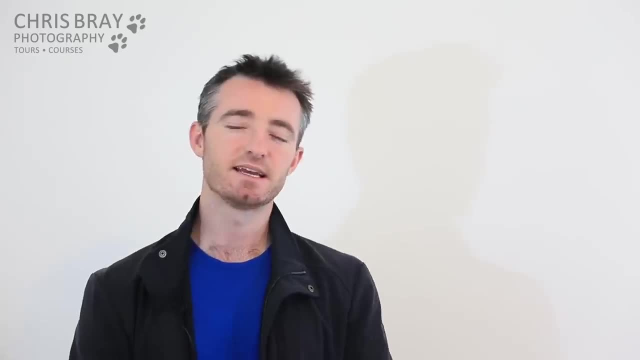 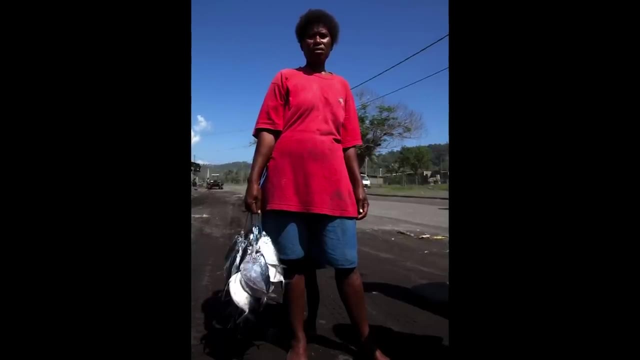 interesting, Get a photo of that. But then luckily, pretty quickly I realised: hang on a second. what is actually interesting here? Pretty sure it's not her wonderfully happy expression Or the fact that there's a tractor coming along. Oh, she's got no shoes on. 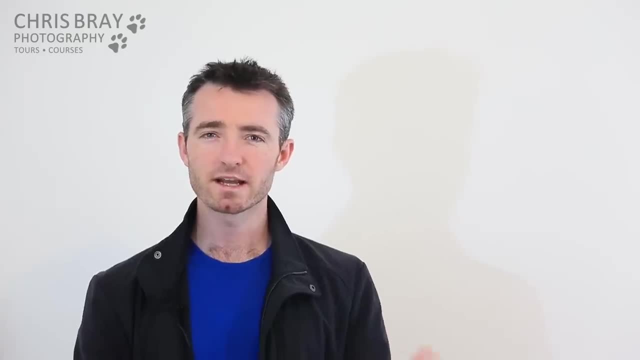 Or there's power lines coming out of her shoulder. You know, you've got to think. what actually caught my attention here was the fact that she was carrying fish, So maybe if I zoomed in and just took a photo of fish carrying, it would be a much more. 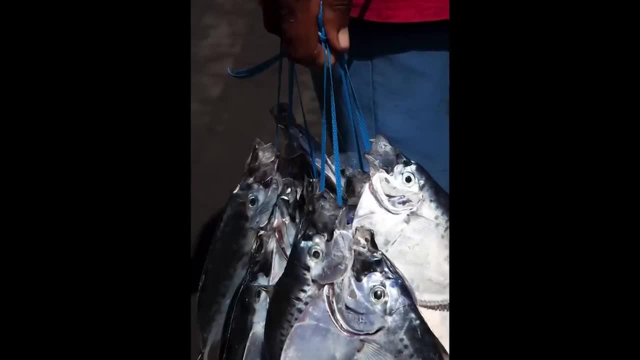 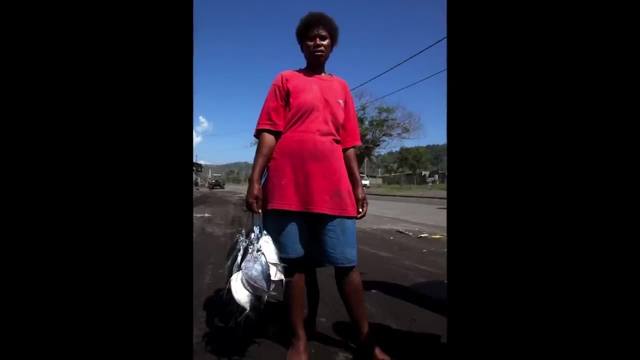 interesting shot. Even half the fish are cut out, But it doesn't matter, You can still tell they're fish. You can imagine a photo like that turning up in a little brochure about the local market place, Whereas that other photo, it's going to go nowhere. 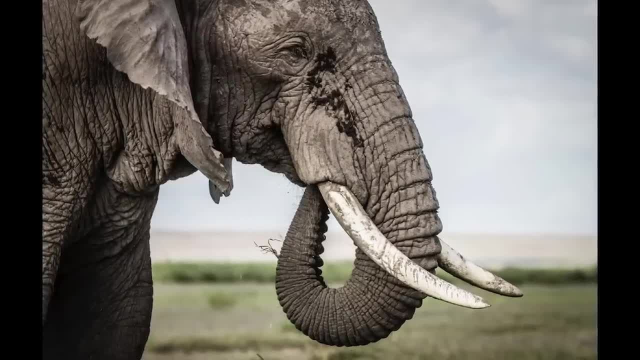 Even a photo like this. you don't need to fit the whole thing in. You don't even need his whole head in there. You can tell that it's a beautiful shot of an elephant works quite strongly. So just try and remember you don't always need to fit everything in. 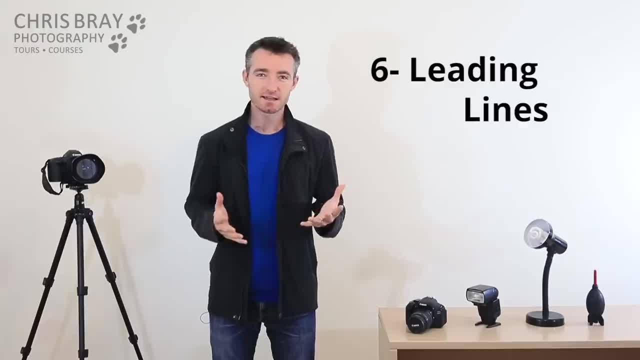 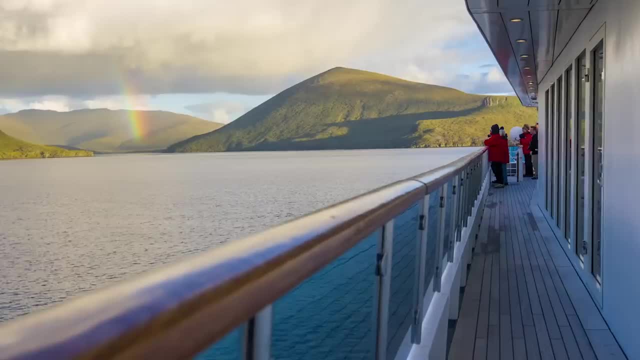 Crop in more, crop in tighter, often looks better. Leading lines: Now, a leading line is any line coming into your photo from the outside And it serves to guide your eye. through the photo Like this one, Your eye comes in along the railing and then it goes out to where the people are and you 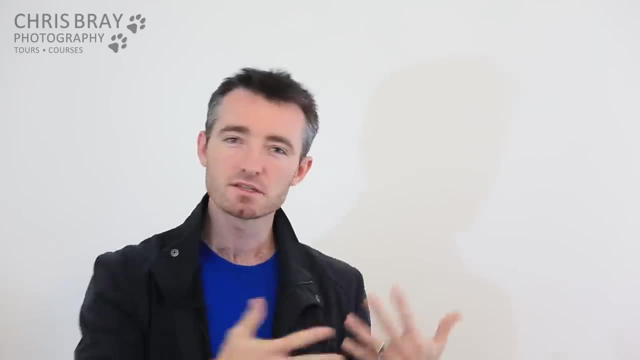 see that they're people and you gaze out along there and you see the rainbow And it all just ties together very neatly. Otherwise some photos can just feel a bit disjoint. You have to kind of look around for a while and then go. 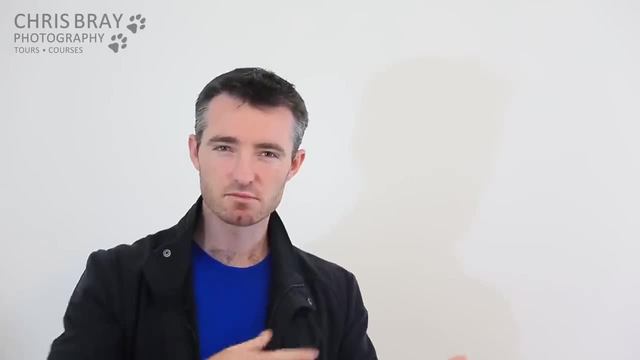 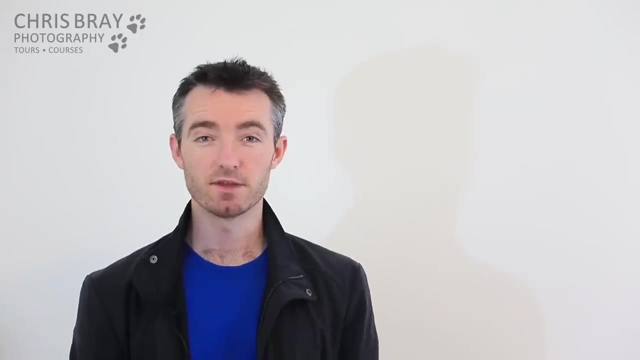 Oh, that's interesting, And oh that's interesting over there as well. It's just not as smooth. If you can link things up with a line, it often looks better. Sure, you don't always have convenient leading lines around, but if you look for them you. 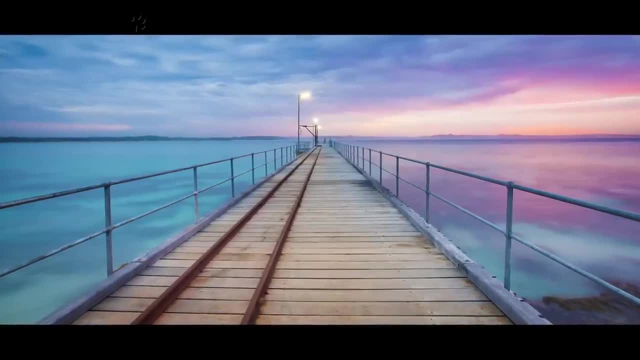 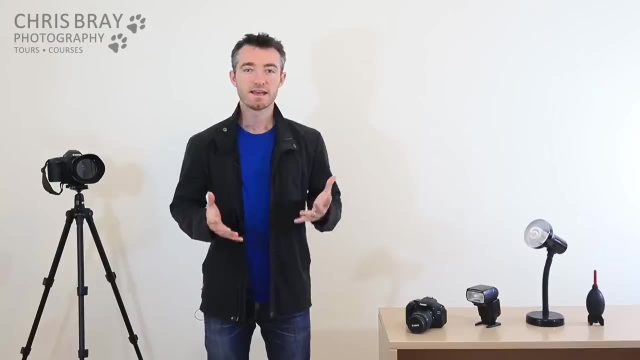 can often find them. And if you do have a leading line, a good tip is to make sure it comes in through the corner of your shot. Leading lines always look a lot more effective if they come in exactly from the corner. Anything but eye level. 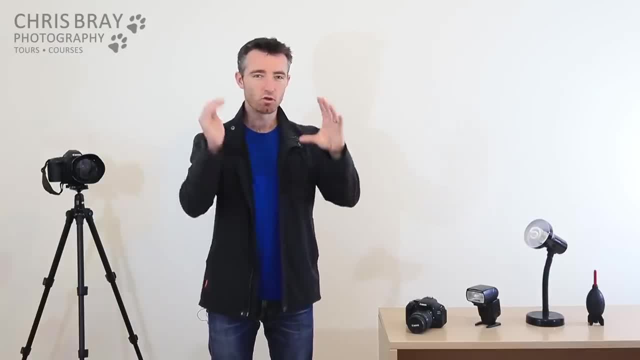 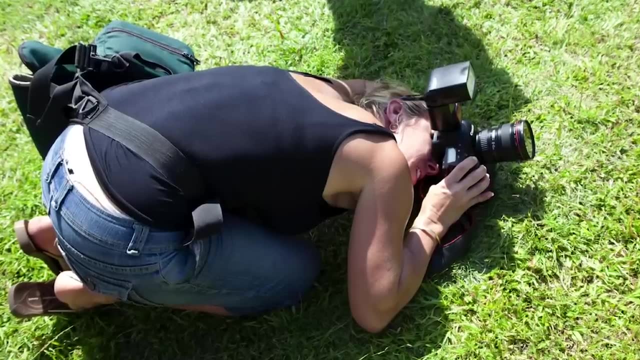 This composition tip is just saying: try not to take every single photo from just normal standing up height, because then everything always just looks the same. You know, Getting up high or getting down low can be a way to just add a whole new angle of interest. 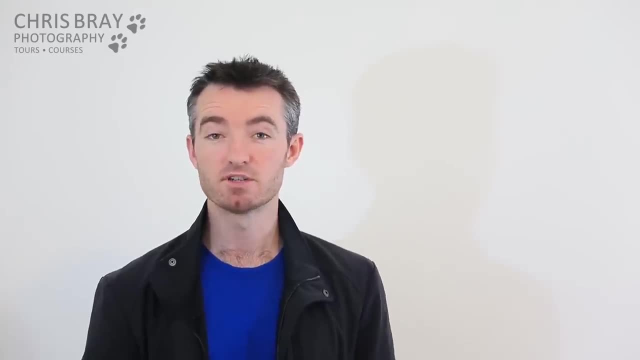 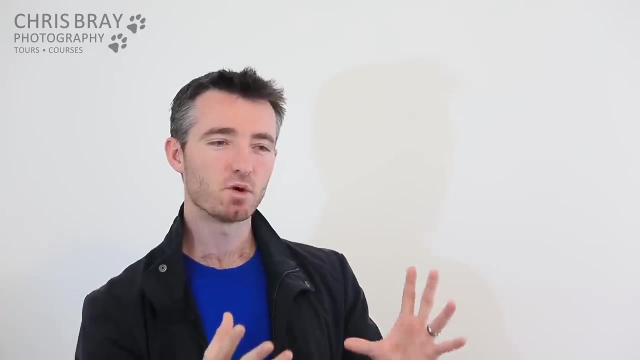 to a photo, A completely different perspective on an otherwise quite boring subject. perhaps You know that's just a photo of Jess on a bike, Not the most exciting subject in the world, But because it's taken from that really low vantage point. these are the kind of photos. 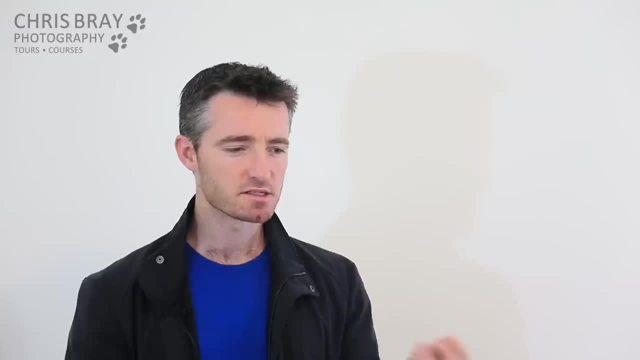 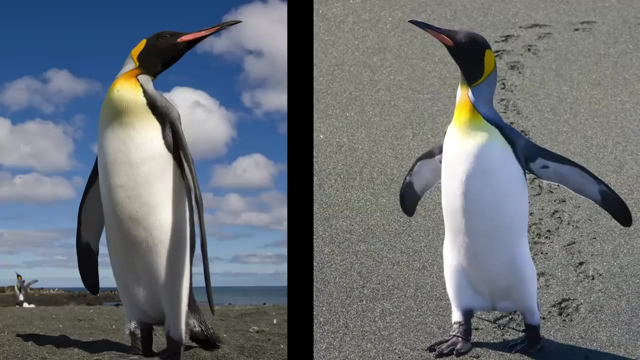 that stop you when you're flicking through a magazine, Because your brain basically goes: yeah, I know that that's a bike, but gee, that's weird. Oh, it's taken from down. Oh, I get it. Same photo of a penguin taken at two different heights. 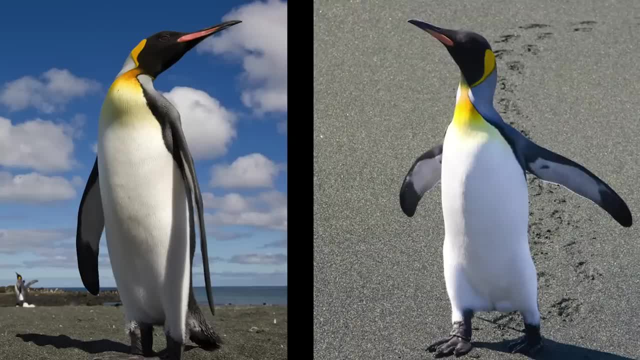 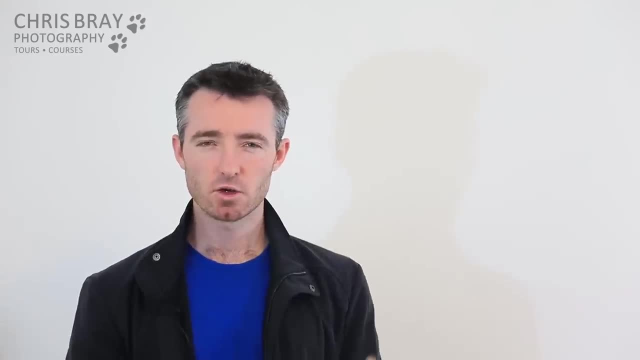 You can really feel a different vibe in those two photos. One feels quite tall and regal, the other one feels like a little penguin shuffling around on the ground. At the very least, though, if you're not trying to do some creative angle, you should always. 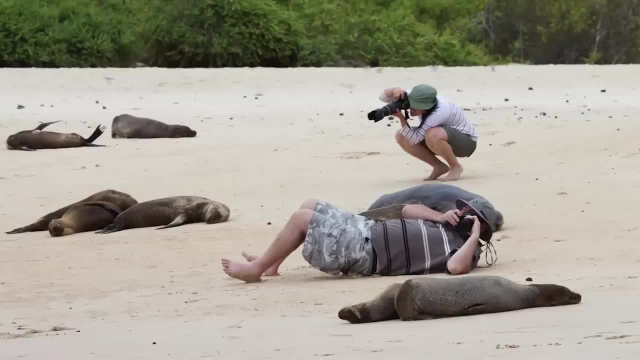 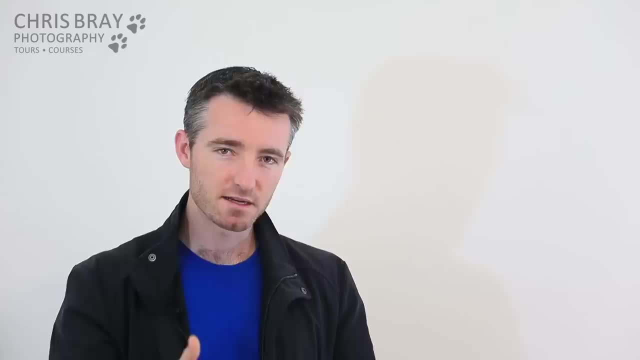 try to remember to get down to the same height as whatever it is you're photographing. So if you're photographing the family dog, get down to dog height Or kids, because you otherwise just end up with photos where the kids are kind of having. 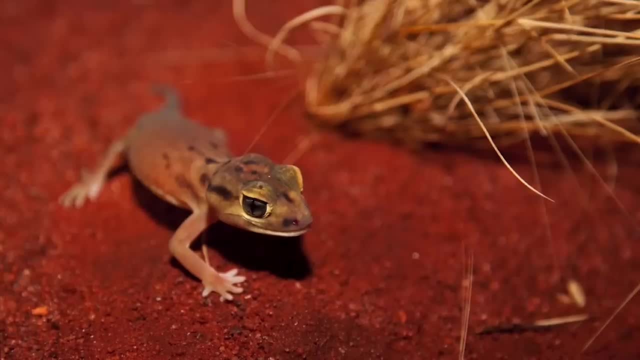 to look up into the photo and you feel very separated. So here's a photo of a gecko. Obviously that's taken down quite low, but it's not low enough As soon as you get down to the same height as whatever it is you're photographing you. 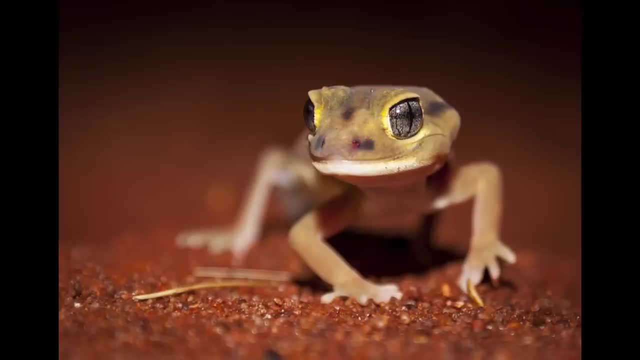 end up with a much more intimate connection there and it's just a much stronger photo. And you can see this photo is also a good example of rule of thirds, That gecko's eye, the key bit is in that top third intersection corner. 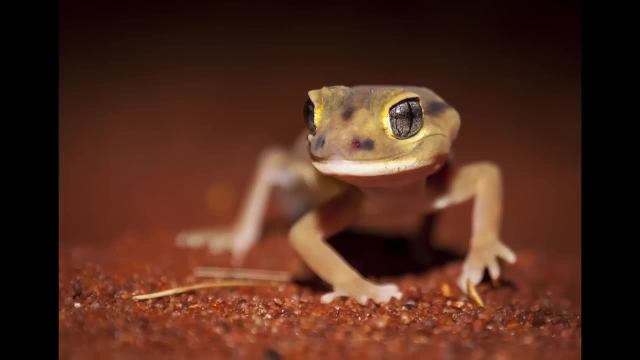 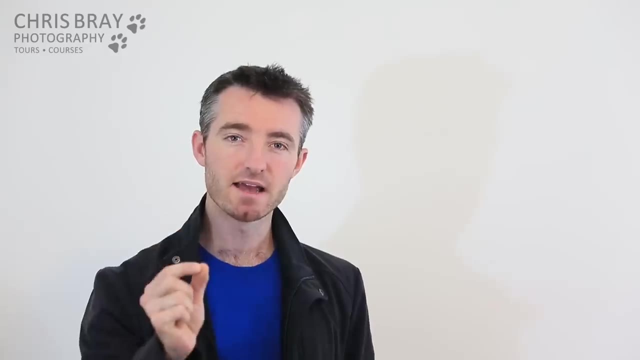 And you can see how important it is to focus on the eyes as well. So you can see, the front of his nose is blurry. everything behind the eye, the rest of the body, is completely blurry, very thin depth of field. but because the eye is sharp, that's. 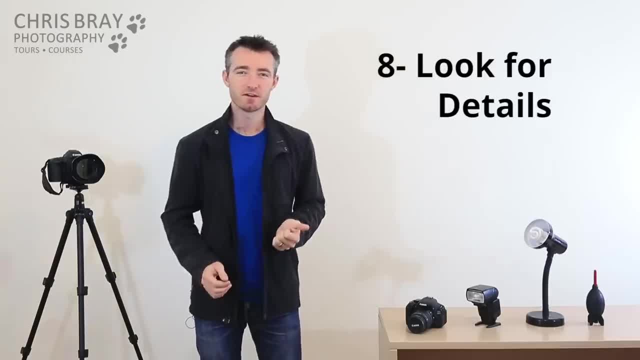 all that matters. when you look at the photo, Look for details. That's part of the fun of being a photographer. I think You start to spot little things that other people didn't even notice and then when you get a photo of it, it's amazing. 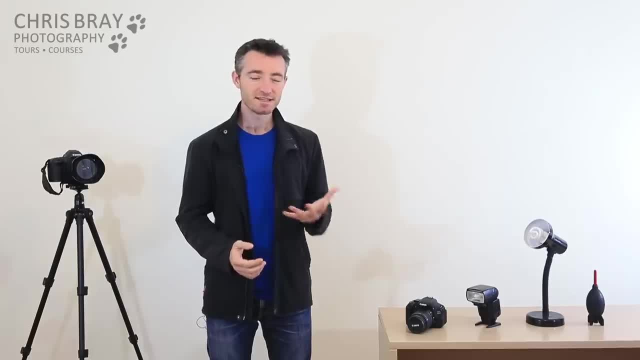 People just go. how did you even see that, let alone get a picture? It's very easy to get interesting photos if you start to look for the little details. You could just be walking through your garden or a jungle or something and find the way. 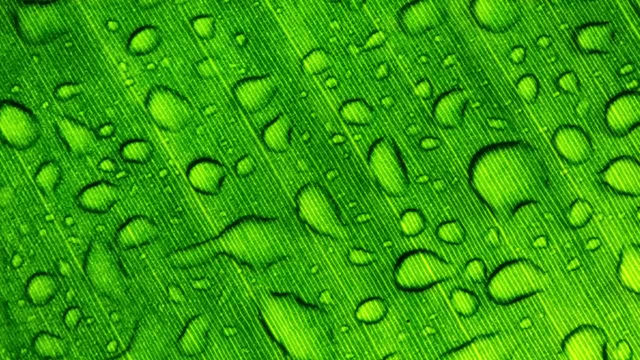 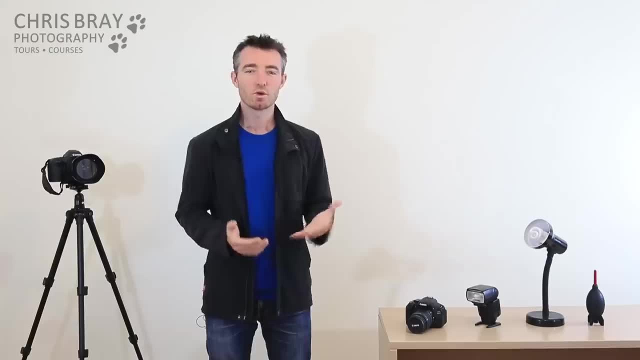 that beautiful little leaves have little curls on the end of them, or raindrops on the back of a leaf, or the way the spores grow on the back of a fern leaf. feather details. We were out photographing Uluru a couple of years ago and you know the sun went down. 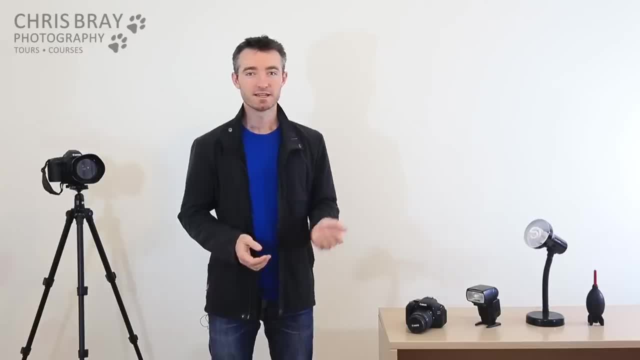 and we got some nice photos. and then we were just sort of thinking, what are we going to do now? And Jess actually spotted the reflection of Uluru in my eye- but she's got far more beautiful eyes than I do- so we swapped positions and I got a macro lens out and I took a photo. 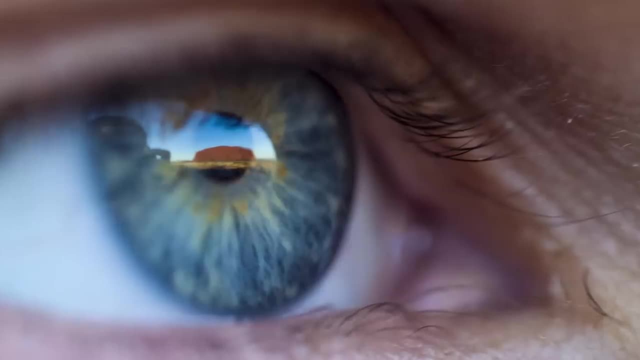 of Uluru reflected in her eye. People love this kind of photo. you know, technically it's a terrible photo, it's just about all blurry. but just because it's one of those little details that people go, wow, how did you even see that? 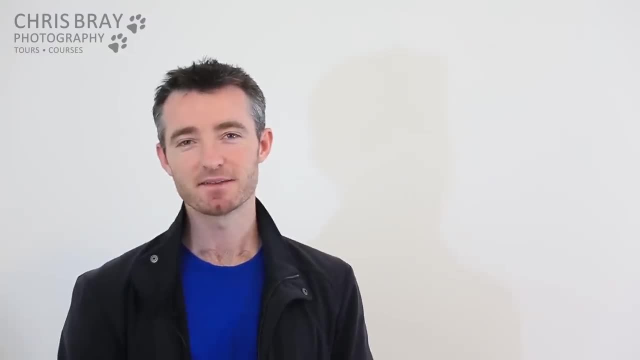 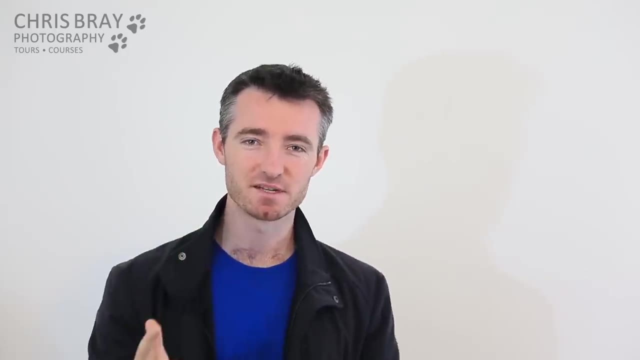 That's a great shot, So keep your eye out for little details and textures and things like that. they can be good photos. Okay, you've got to remember to take some vertical photos as well. A lot of us just only ever take horizontal photos, and that's a bit sad, because some 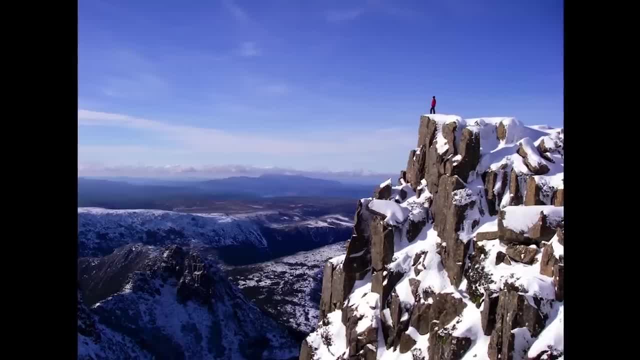 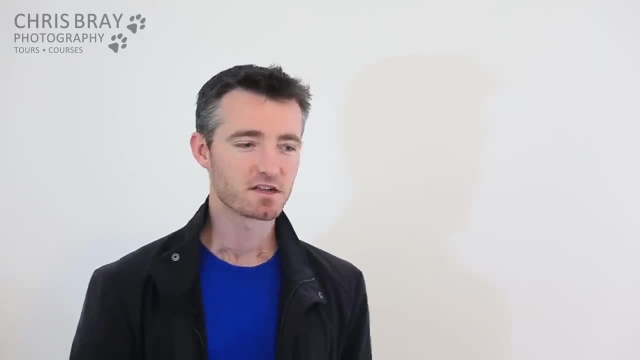 subjects just fit a vertical frame a whole lot better, Even long sweeping landscape shots like this one. you can still have a vertical version of that and it still works. Actually, when I went on my first Australian Geographic assignment, I was reading the contract. 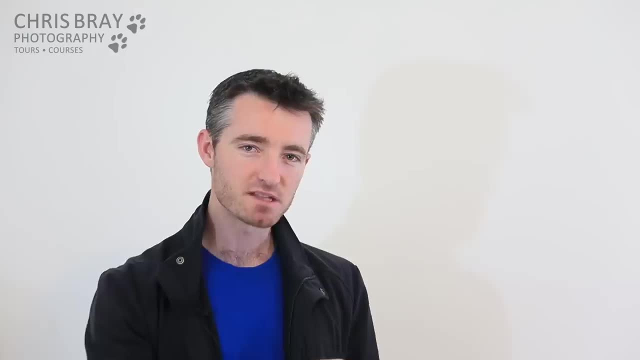 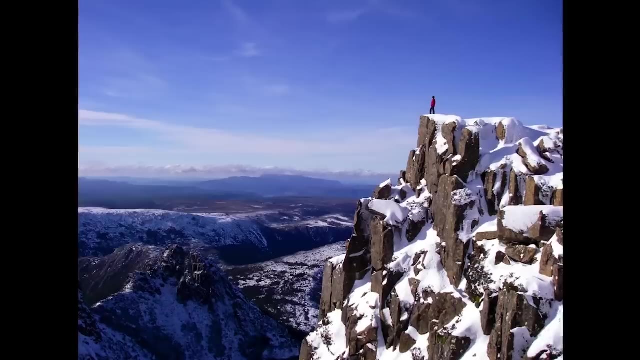 points, and one of them actually said: every single thing you photograph, you must take a horizontal and a vertical version of every single thing, and that blew me away. Often one of them might look better than the other. fair enough, but you can always take. 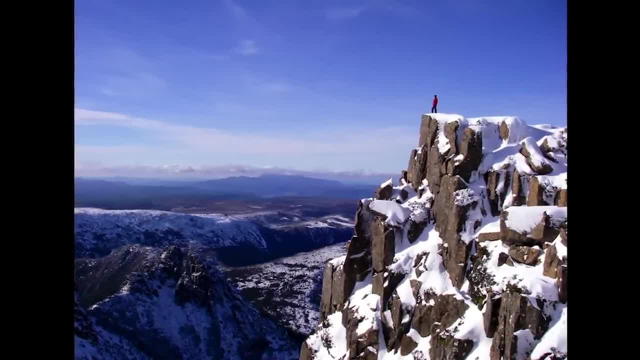 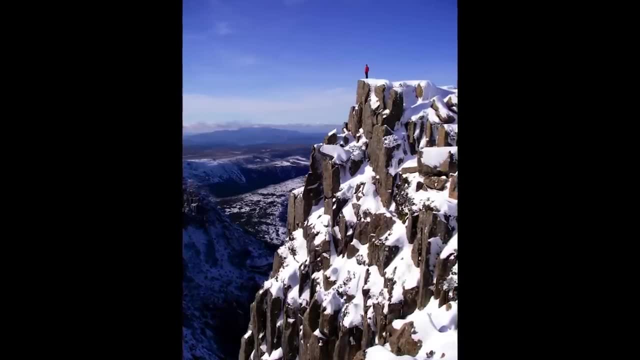 both and they always work. This one, the feeling is more: wow, what an amazing open view she has out that way. wow, wouldn't that be incredible. And the other photo is a bit more like: oh, don't stand so close to the edge, your eye. 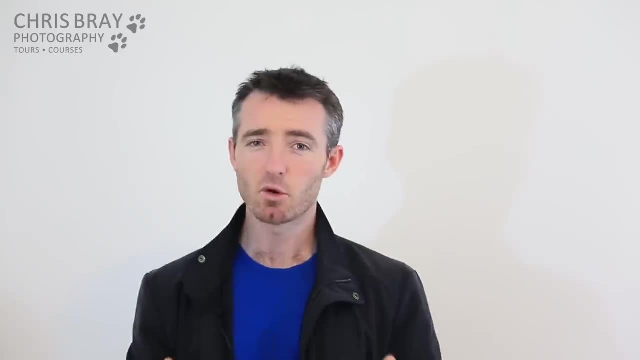 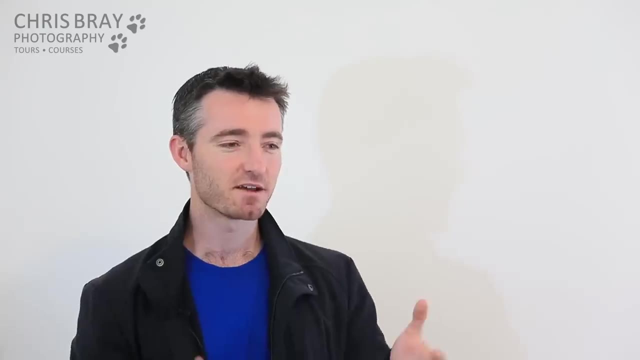 travels down the mountain and instead it feels taller. Now, if it feels awkward for you to take vertical photos, then that's a good sign that you're not taking enough of them. Maybe pretend you're on assignment for a while and next time you're taking a picture force. 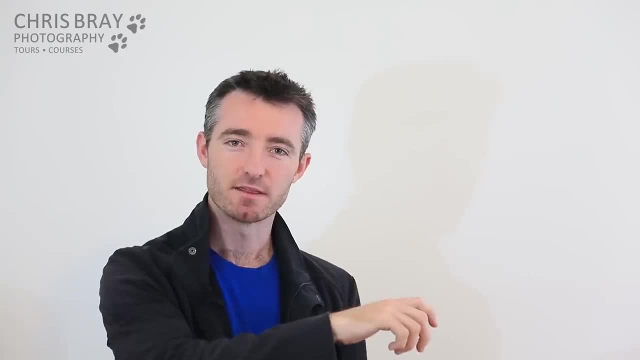 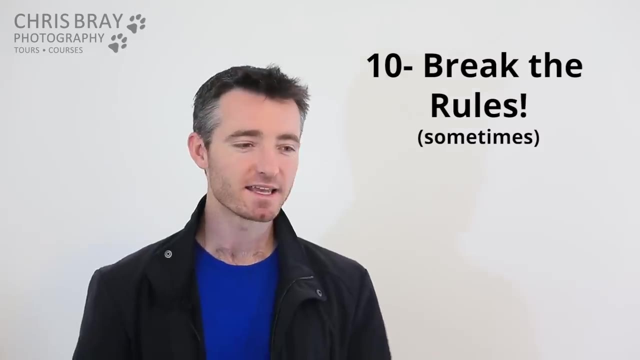 yourself to work out how to make it fit nice composition vertically. take some of that as well. it'll just be good practice for you. And the last one: break these rules. sometimes You know, photography is a creative outlet. it's not like engineering, where you've got. 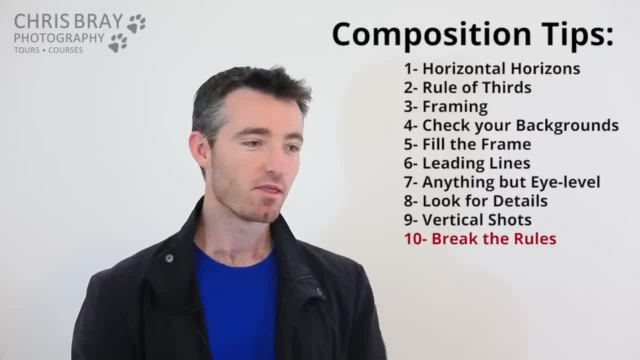 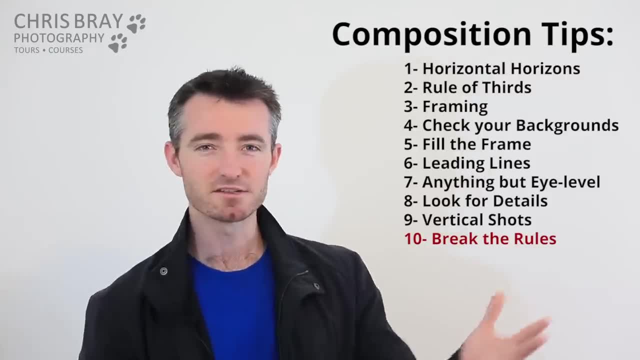 your top ten checklist and you better double check you've got every single one done, Otherwise the bridge is going to fall down and you're going to kill someone. Photography is fun, especially with digital. you can try all these different settings and weird angles that you're pretty sure aren't going to work at all, but sometimes they do. 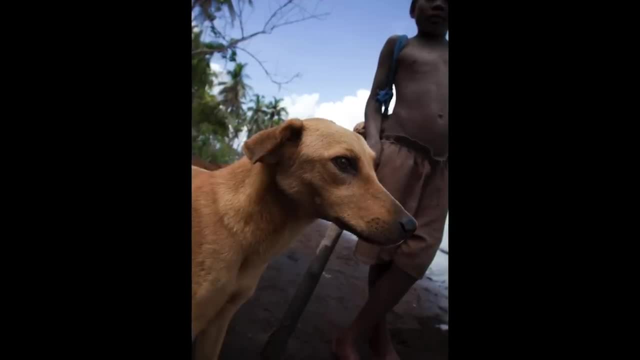 and you're like that looks cool. I don't know you might hate it. I don't mind it, though I can imagine it turning up in a magazine somewhere. But you know, I think it breaks every rule I can think of. 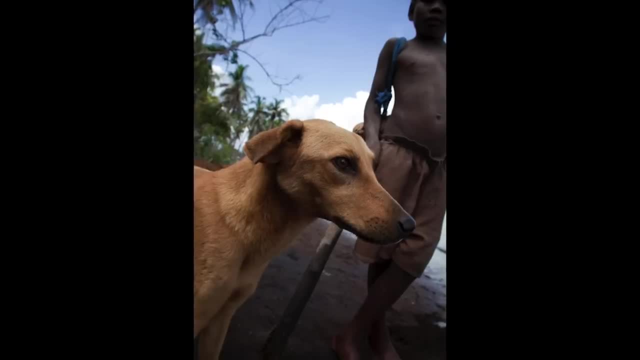 The dog's eye is probably the key bit in the photo and that's in the dead centre. there's no rule of thirds going on. it's probably about 30 degrees wonky and I know I say don't always try and fit everything in. 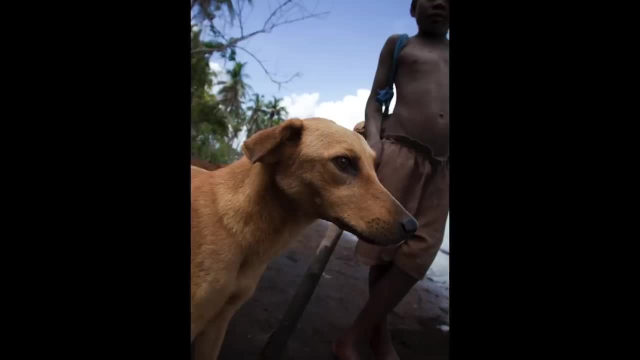 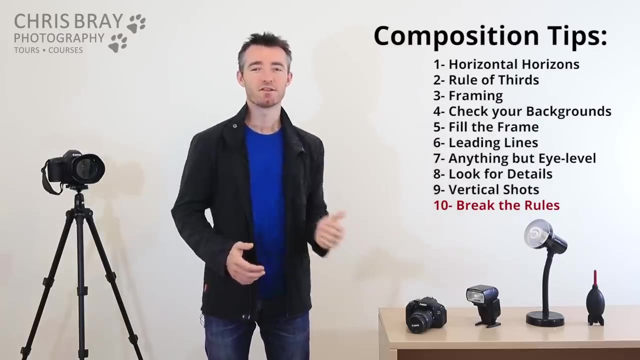 But I wouldn't normally just cut off a third of it, Cut someone's face and cut their toes off, But it sometimes still works. so feel free to break these rules. it's really just there as a scapegoat. If you've failed on all nine of those other points, you can just say you were concentrating. 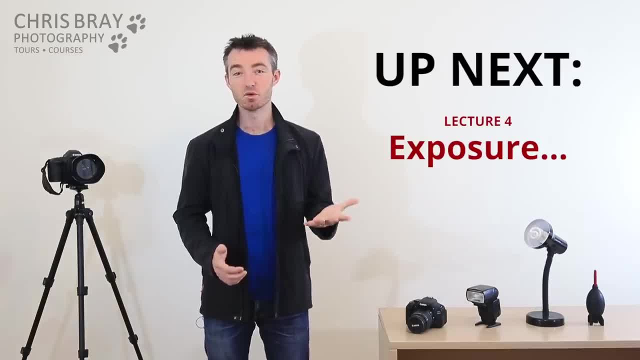 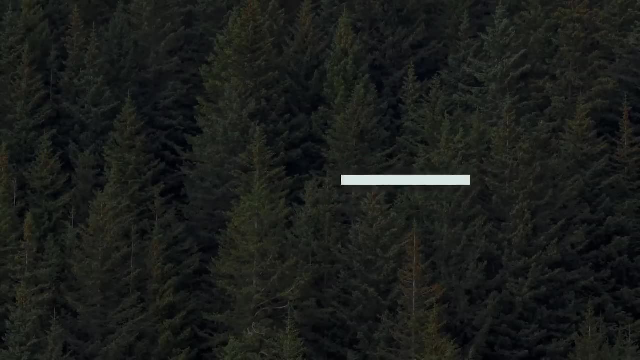 on the last one. So in the next lecture we're going to look at exposure. Sometimes the photos are a bit too bright, a bit too dark. how do you fix that? histograms, that kind of thing. You start to learn a lot more advanced stuff. 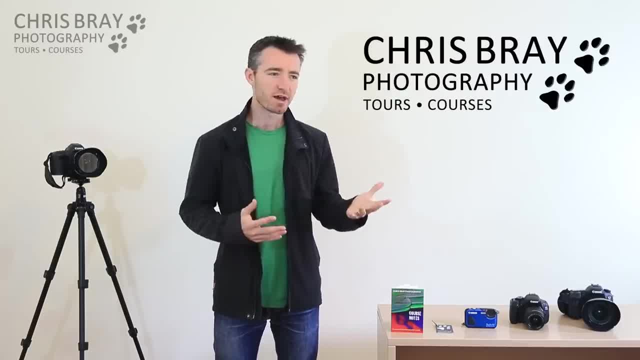 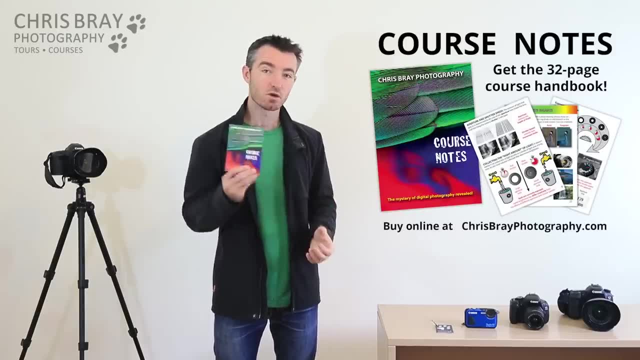 Exposure. In this section we're going to look at what makes your photos come out a bit too bright or a bit too dark. how do you control that? a bit of a look at histogram graphs as well, and just a reminder that this is all covered in the exposure section of the Course Notes. 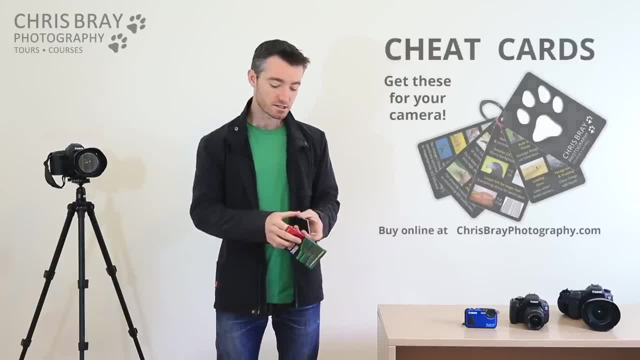 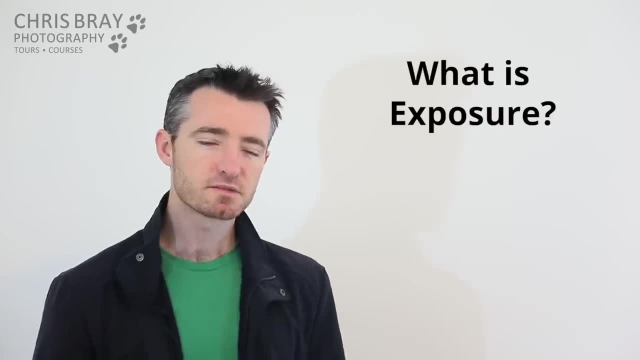 booklet that you can buy online and also there's little plastic summary cards. there's a little exposure section there just shows you how to change that brightness as well. But firstly, what actually is exposure? Well, exposure is light falling onto your image sensor and you can think of it as the entire. 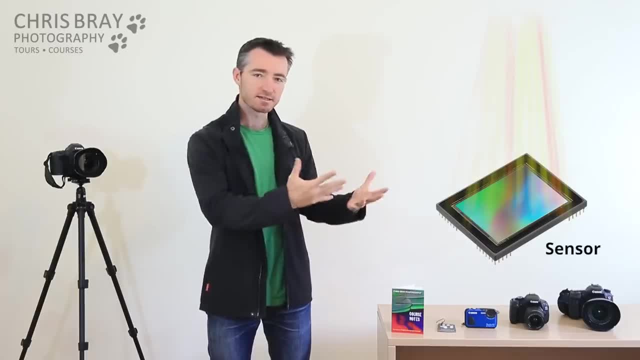 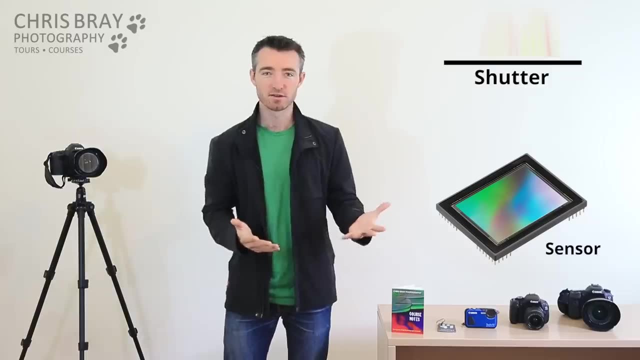 time the shutter is open, more and more light is landing on there and it's just collecting more and it's getting brighter and brighter and, hopefully, when the right amount of light has gone in there, your photo finishes and you end up with perfect exposure. 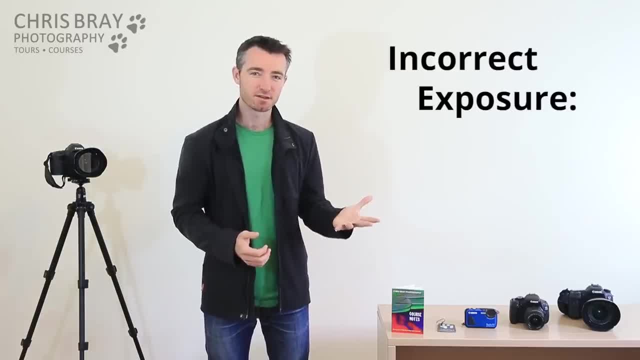 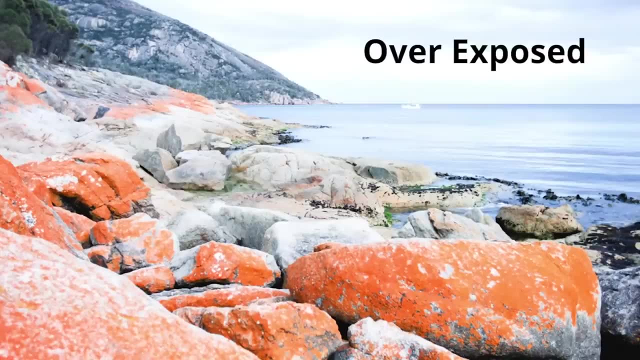 Obviously half the time that's not what happens and you end up with incorrect exposure. So underexposed, just not enough light got in there yet and everything's come out looking too dark. Overexposed- too much light got in there and everything just comes out looking too bright. 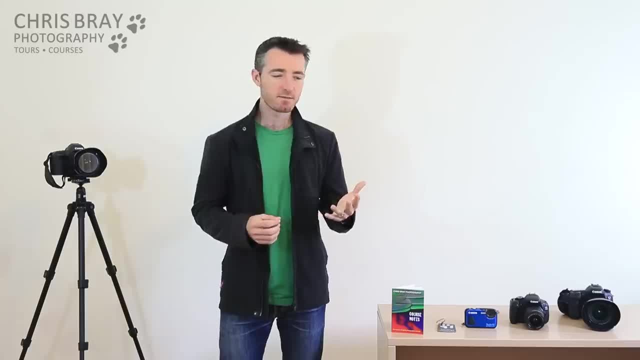 Correct exposure, just the right amount of light. But the problem can be that by the time you get you know this part of the photo looking correctly exposed. some other part will still be too dark or too bright And that's caused by what's called a contrast limitation. 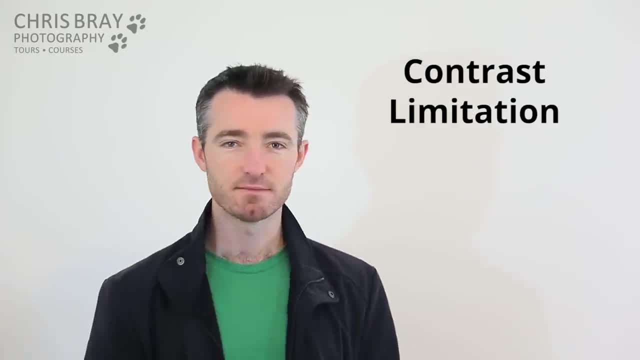 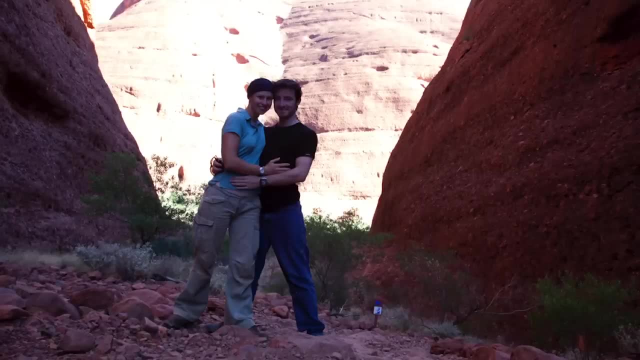 All cameras have this problem where they can't see into the bright and into the dark at the same time. So you've got a situation like this one perhaps, where we've got the foreground having correct exposure, but by then those background rocks in the brighter sun. they're now massively. 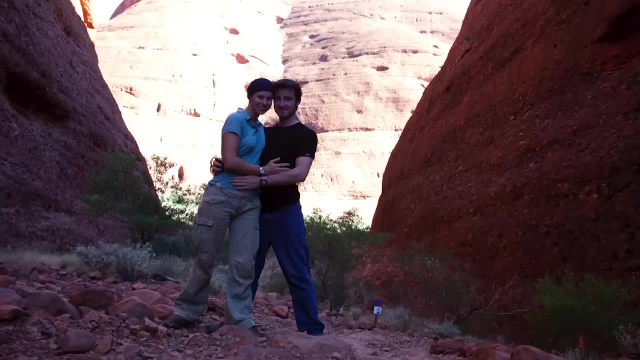 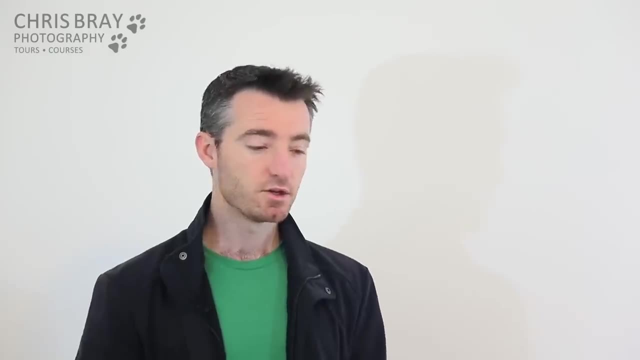 overexposed And you go. well, that doesn't look any good. maybe we'll set the camera up to get correct exposure for the background, But now of course the foreground is too dark And there's nothing you can do in the one picture to fix that up. 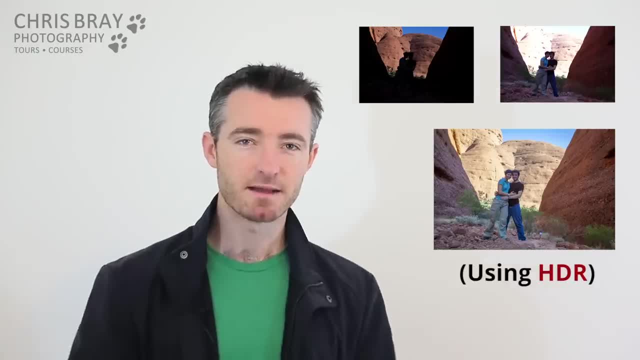 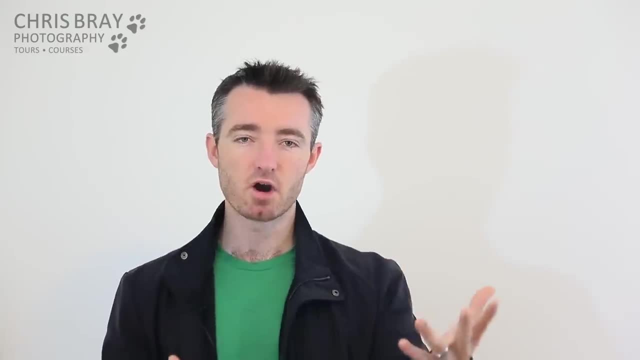 You could deliberately take both and merge them together using HDR, high dynamic range or something like that. There's just nothing you can do to get around that problem of really harsh lighting, having such a big difference between being in the bright and in the shadow. 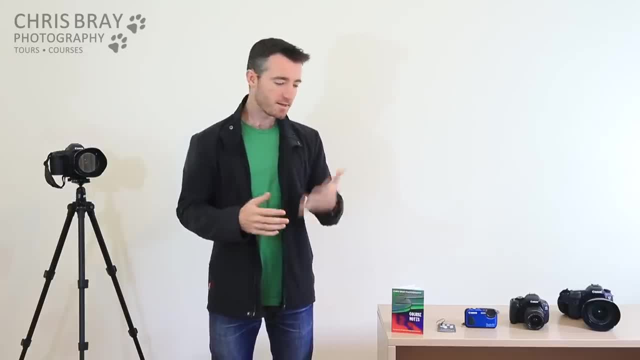 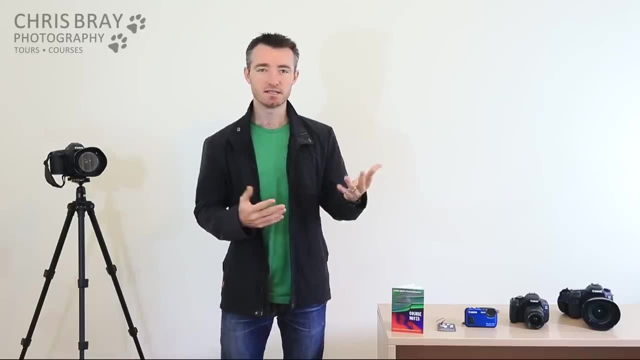 But the thing is, when I was standing there looking at that view myself, it looked great. And then you get a picture like that back and you're left wondering. you know what is wrong with the camera. It's not particularly that. the human eye has some incredible ability to see into the dark. 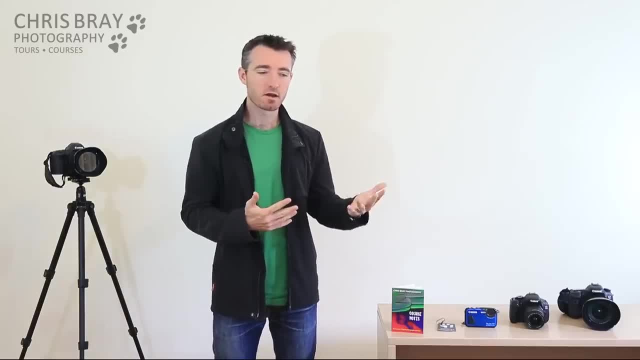 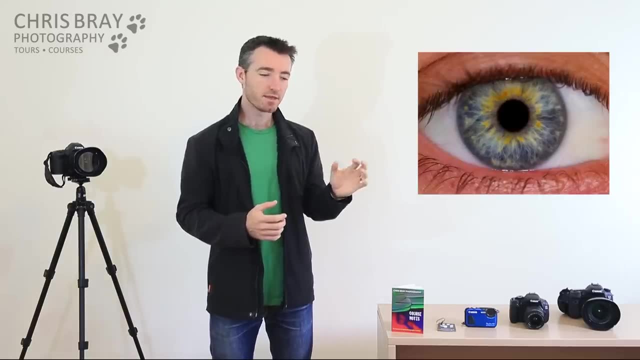 and the bright at the same time. It does have a better contrast range than a camera, But still the main thing to remember is that the camera has that variable sized aperture hole in the lens And your eye has exactly the same thing in your iris. 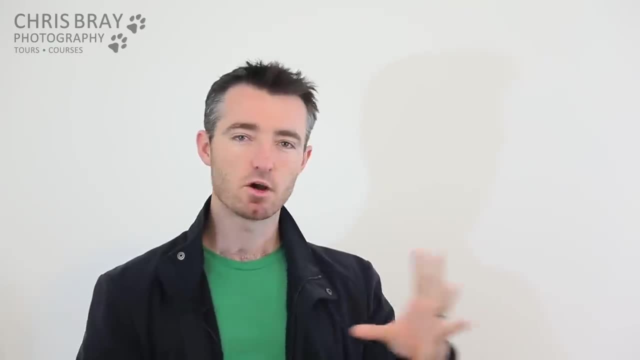 Or your pupil. The thing is, when you're looking at a scene, the pupil changes depending on where you're looking, so that everything looks correct for you. So when you look up here in the bright part of the scene, your pupil would shut right. 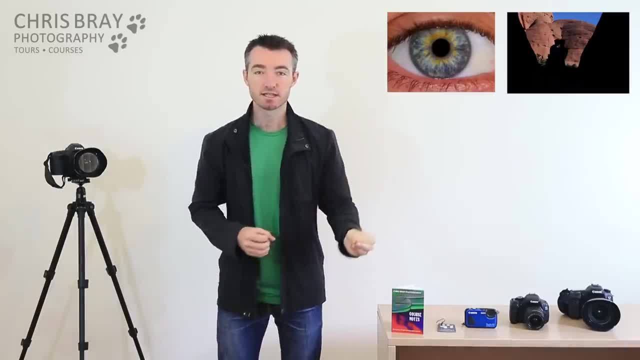 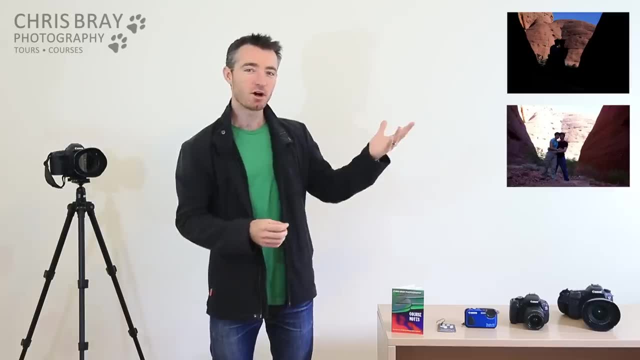 down and cut out all that light, So that would be correctly exposed. But then when you look down in the shadows, your pupil would open up and let more light in And then the shadows would look correctly exposed. But the thing is, you remember when you looked up to the top that's what it looked like. 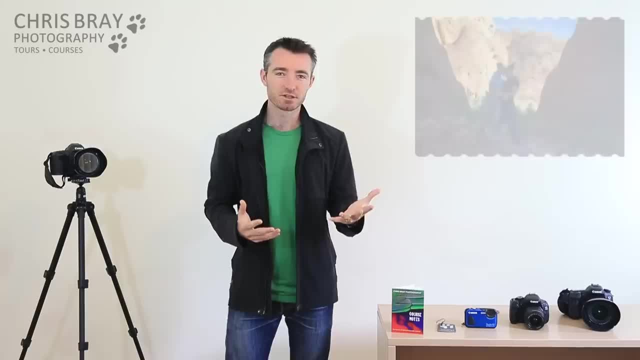 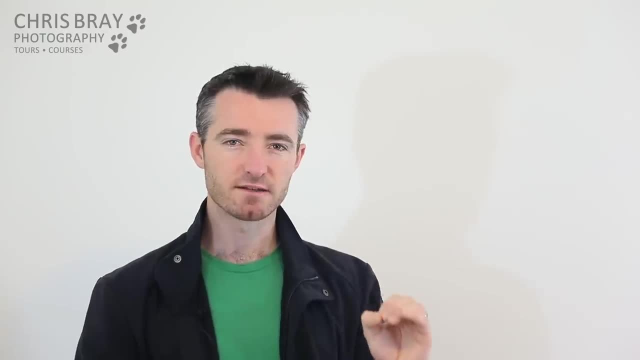 And when you look down in the shadows, that's what it looked like. You're kind of just building up a mental picture of the world that seems wonderfully exposed wherever you look, But it's because it's changing a lot. Of course, with a camera, though, you're stuck with the one setting for the entire shot. 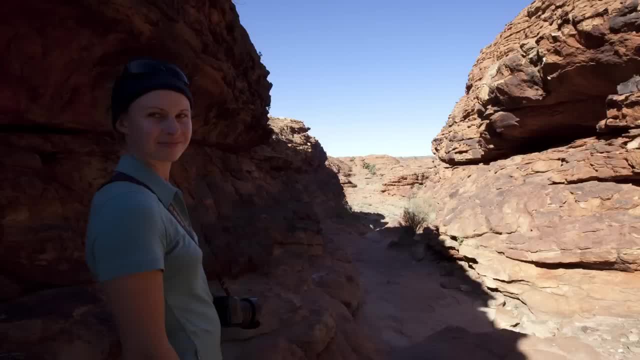 And there are just going to be some bits that are so much brighter that they become overexposed or underexposed, And there's just not a lot you can do. You've just got to remember that cameras can't cope well with scenes that differ too much. 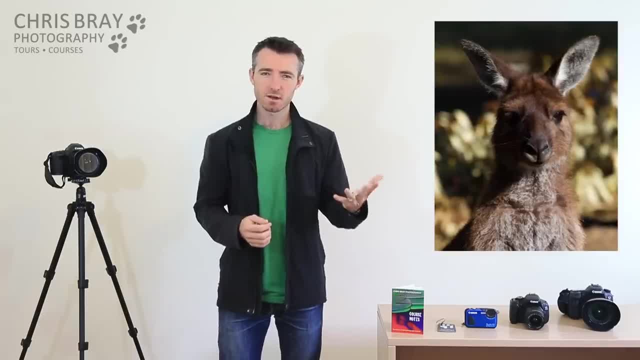 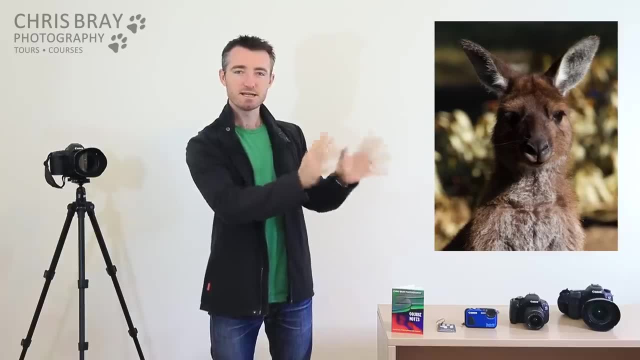 in their brightness, So really strong lighting, like mid-day lighting. that's why it's such a bad time to take photos, Because the difference of the side that's in the sun and the side that's in the shade just next to it, you know it's a million times different and the camera just can't. 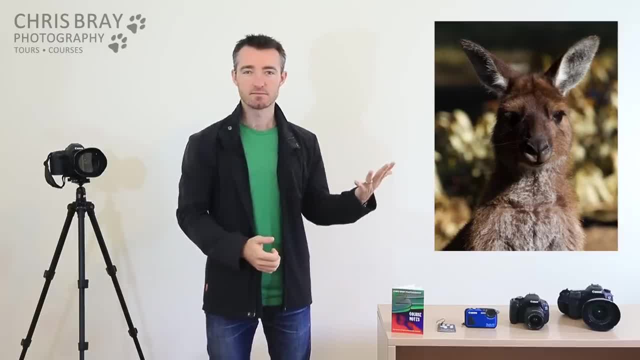 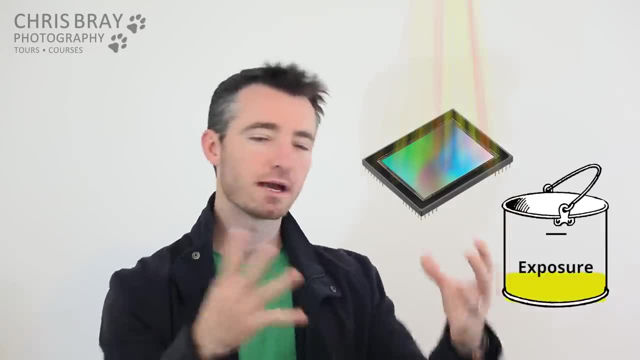 cope. You're going to end up with black shadows or overexposed highlights. So collecting the right amount of light- You can think of it as a volume of light you've got to get into your camera somehow, And it really doesn't matter whether it all comes in at once or if you just gradually. 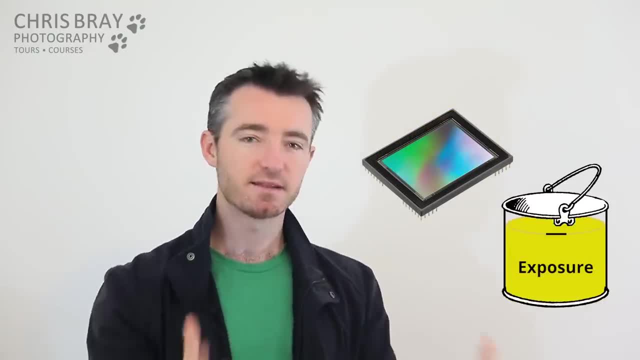 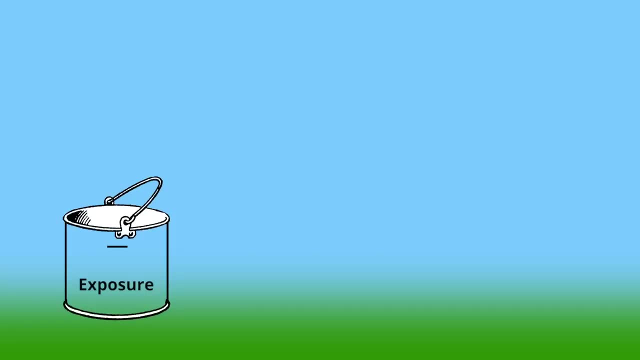 let the light trickle in as long as at the end of the shot you've collected that same total volume, Because that total amount of light is what determines how bright your photo is. That brings us to this useful little analogy. This is the size of your aperture hole here. 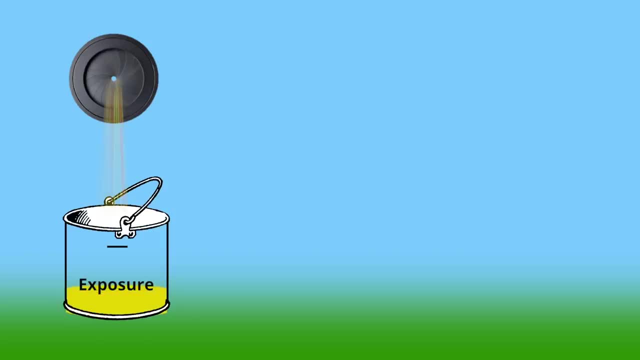 If you make that a really small hole, obviously the light can only gradually trickle in and it takes the camera quite a long time to collect the amount of light it needs for that correctly exposed photo. So you typically have quite long, slow shutter speeds associated with those tiny little holes. 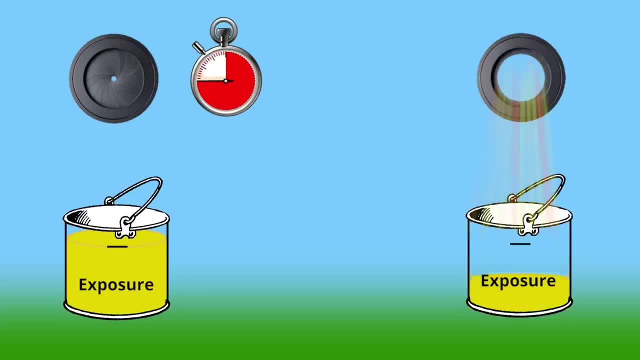 Conversely, if you open the aperture up to a really big hole like that, the light's able to rush in very quickly and you typically have quite fast shutter speeds associated with the large aperture holes. That makes sense to that level. But the key thing to realise here is that both of those photos are correctly exposed. 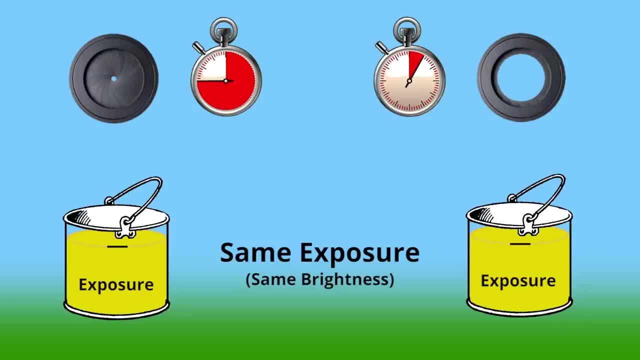 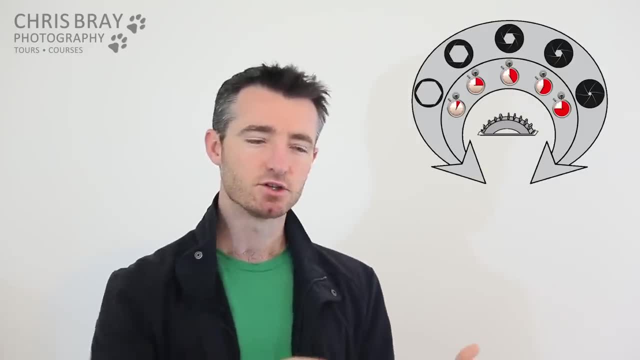 They both look exactly the same in terms of brightness, but they're creatively different due to the effects of having different shutter speeds and different apertures. So for any given scene There's actually a huge range, A whole bunch of different aperture, shutter speed pairs that will all end up with correct. 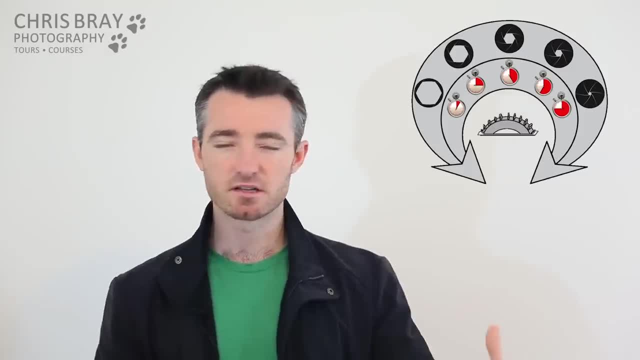 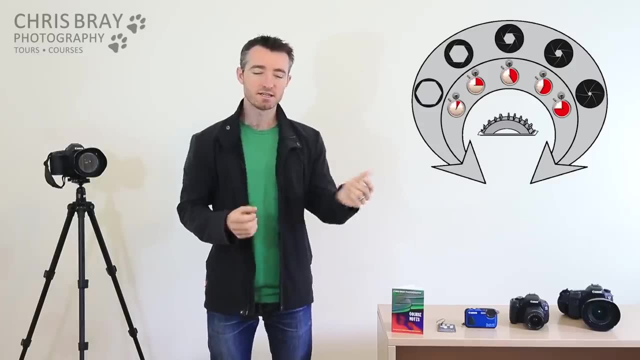 exposure and the photo will look fine. but you get to choose whether you want long shutter speeds or fast shutter speeds, or big aperture holes, small aperture holes to get the creative effect you want, Like if you wanted a really fast shutter speed to freeze an eagle coming past. well, you can. 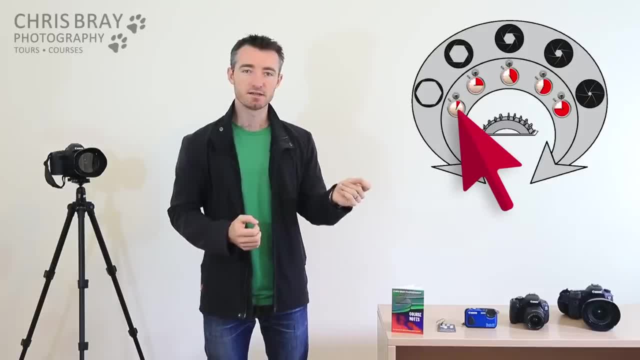 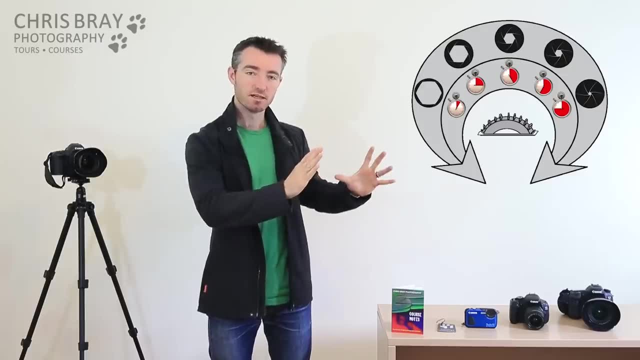 just tell the camera, hey, I want a thousandth of a second for the shutter speed, And the camera will work out and go: gee, I've got to get all that light in in a thousandth of a second. I'm going to have to open up that aperture hole really big. 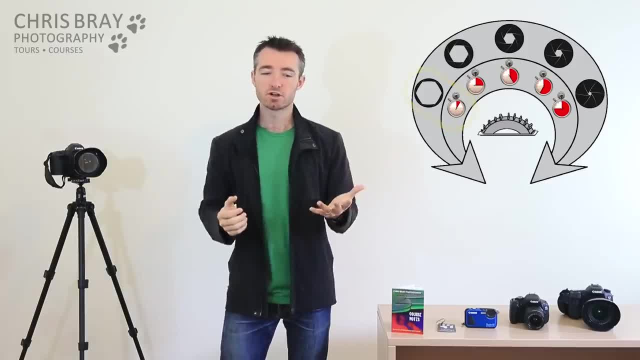 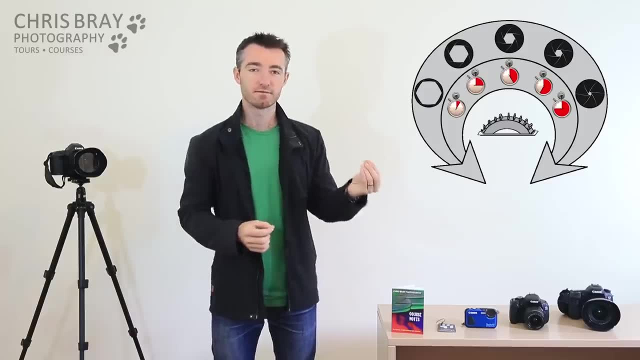 And it'll work out the size of the hole and set that for you. Or maybe you're interested in a long, slow shutter speed like of a waterfall. you want to see all that flowing movement, So you could just tell the camera. hey, I want a one second photo. 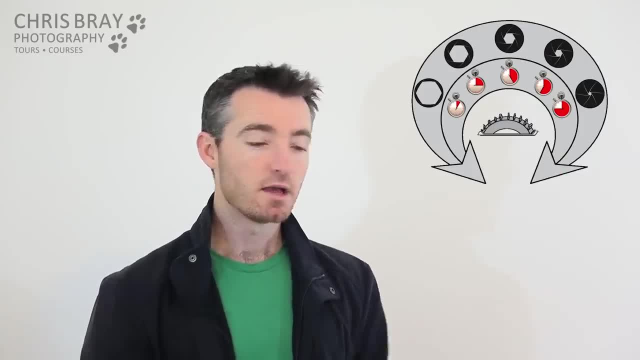 And the camera will then work out that it's going to have to let the light come in slowly through a little hole and it'll set the size of the hole for you. Or maybe you're not interested in shutter speed at all. You want a particular aperture. 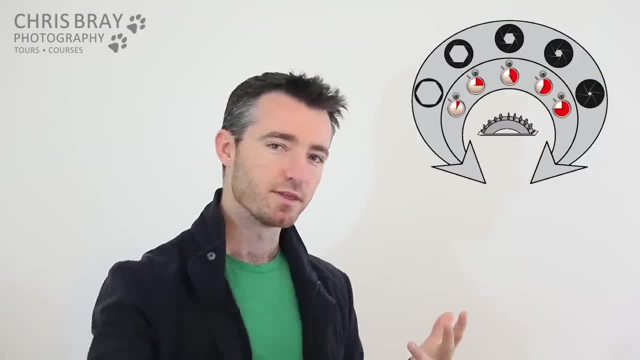 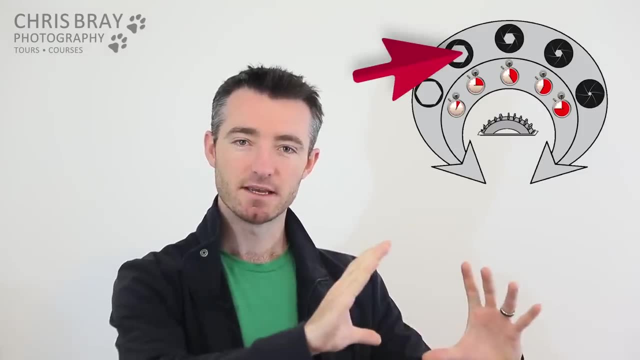 We'll learn in another lecture about how the actual aperture links into what's going on with your depth of field. but for now let's just say you wanted you know this much aperture. So If you've got a camera to make the aperture hole that big, it'll then work out the shutter. 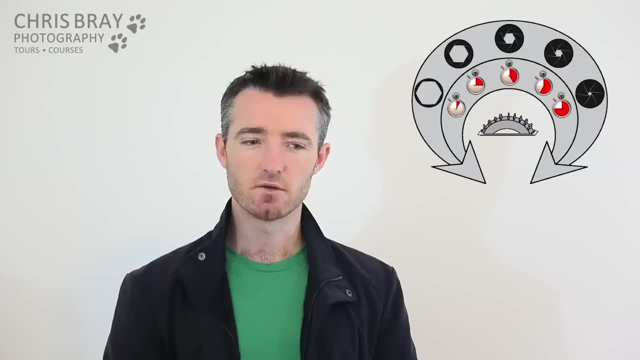 speed has to be this long to go with it. You don't need to try and balance these two things yourself unless you're in manual mode or something, And there's almost no call for that unless you're in a studio or a few other things. 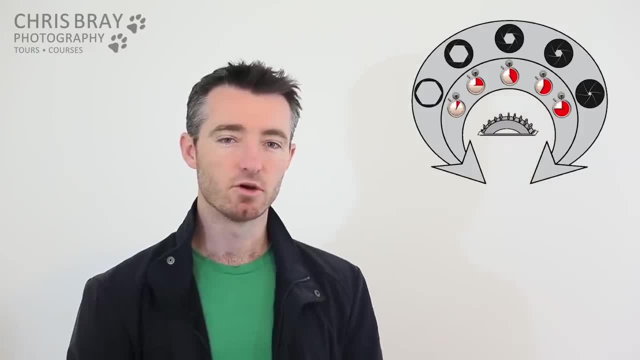 There's a bit of a misnomer around that you know to be a real photographer you need to use manual mode. Just, completely not true. So how do we actually start to shift this balance? How do we unlock some of that creative potential from the camera? 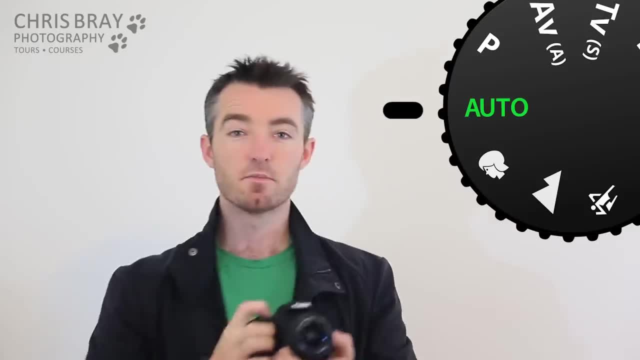 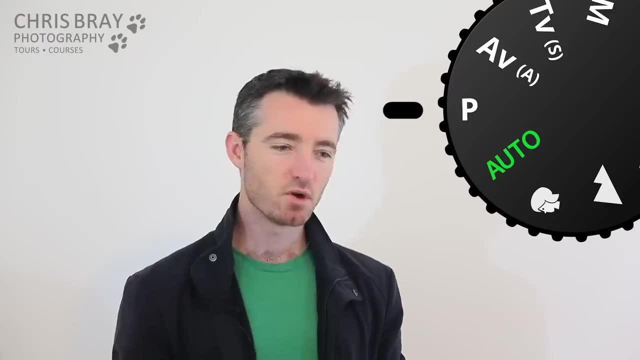 Well, yep, that's when you've got to step out of auto mode. So P mode or program mode, that's one step up from auto mode and, as you'll see that, some creative options for us. We use this mode as a stepping stone and sooner or later we'll end up not using P anymore. 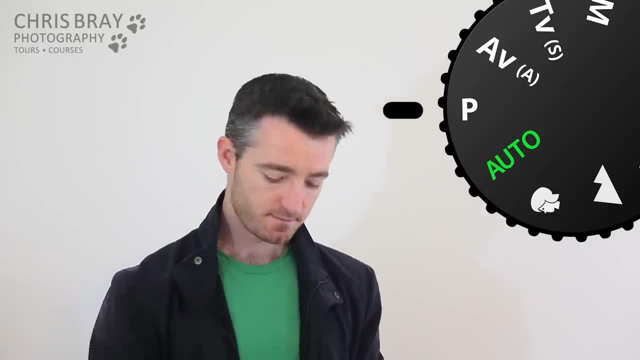 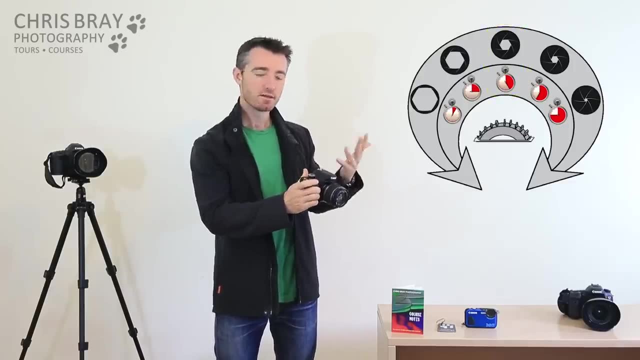 we'll just start using it in aperture or shutter speed, depending on what you're interested in. Now in program mode, when you go and take a picture, the camera automatically suggests a particular aperture- shutter speed combination for you that it thinks is about right. 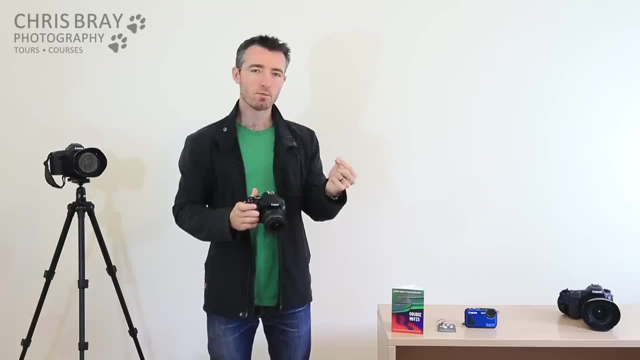 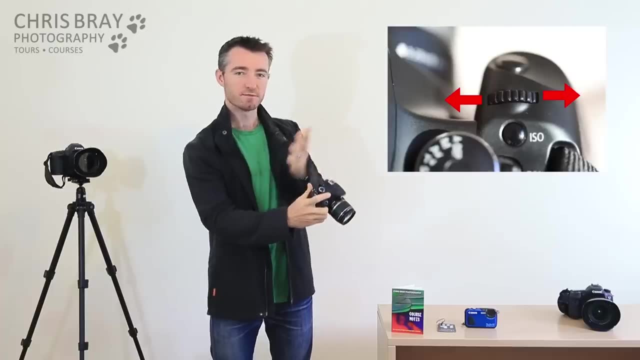 Interestingly, it's exactly the same set of values it would have given you in auto mode. normally, It's just that, if you wanted to, in P mode, if you're brave enough, you're allowed to start scrolling away from those default middle values. 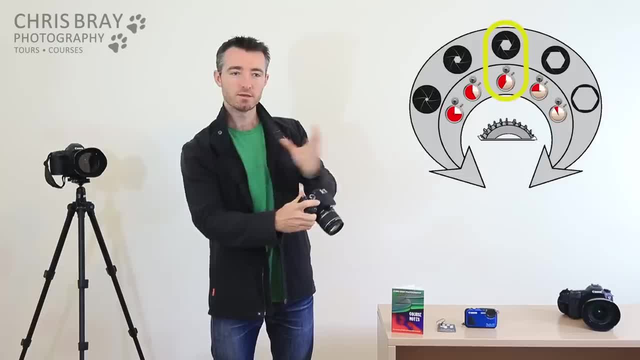 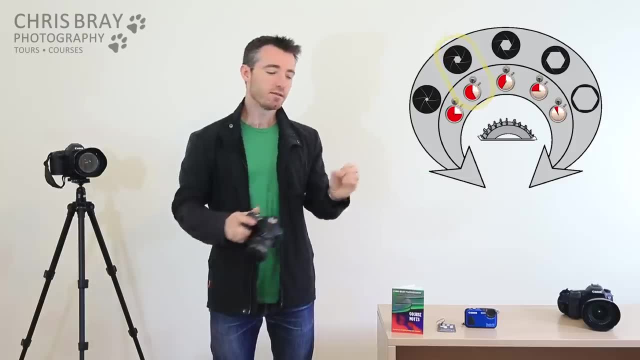 Okay, Let's do something more creative. So, as you scroll one way, you might find that the aperture hole is getting smaller and because it's getting smaller, the shutter speed will stay open longer for you. Or if you scroll the other way, the aperture might be getting bigger and therefore the 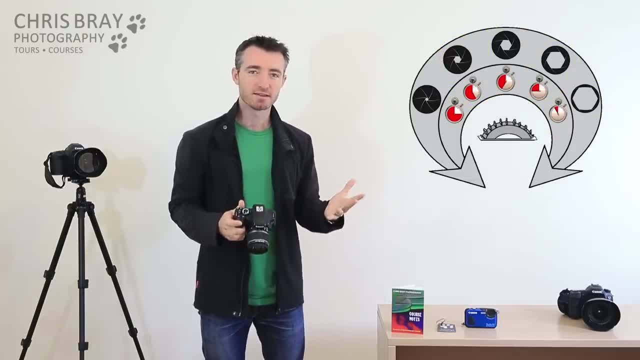 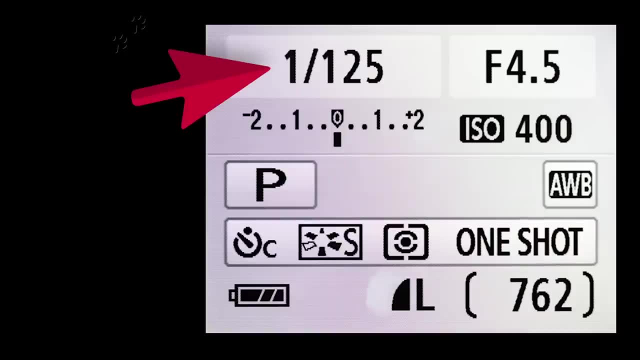 shutter speed gets faster, but it's still giving you the same total amount of light in the end. So this is typically how it works. You touch your shutter button, the camera wakes up, suggests those middle default sort of values for you. that's the shutter speed: 125th of a second. 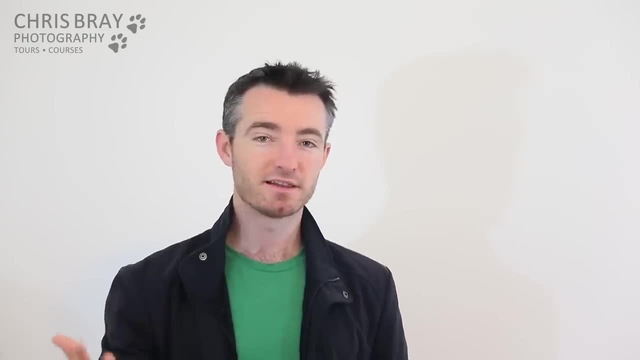 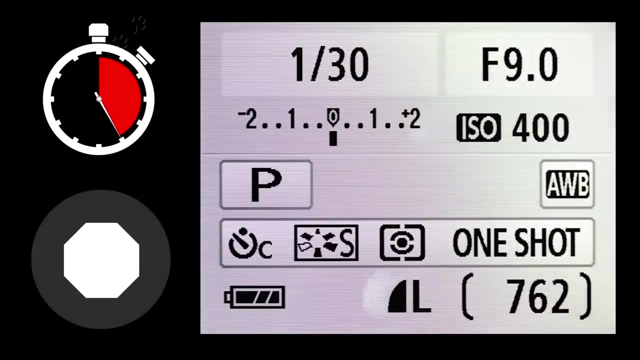 And over here that F4.5, that's the size of your aperture, but we'll learn later on about what that actually means And how that links to your depth of field. But as you scroll around now you'll find that the aperture hole is getting smaller. 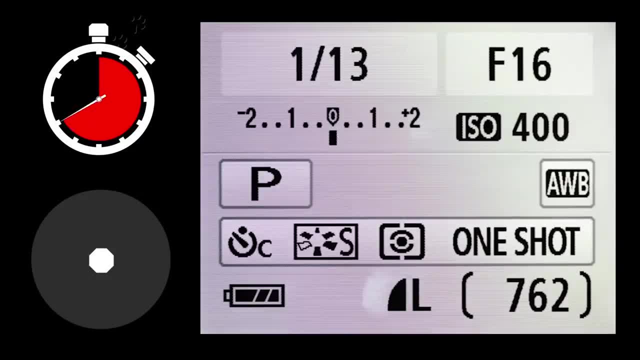 and because the hole is getting smaller, the shutter has to stay open for longer and longer. so we're still ending up with the same total amount of light. So the brightness of your photo is not changing. you're just choosing how you want that light. 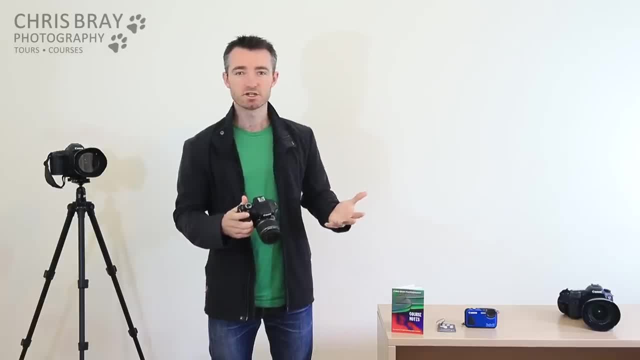 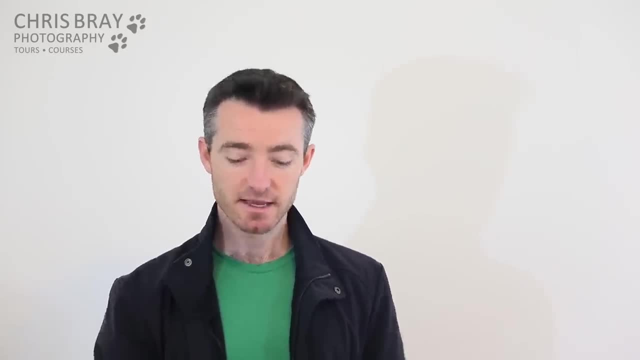 to come in and having different creative effects now for different apertures and different shutter speeds. Now the great thing about P mode is you're entirely safe. It won't let you scroll off the edge of the earth and start getting incorrectly exposed photos. 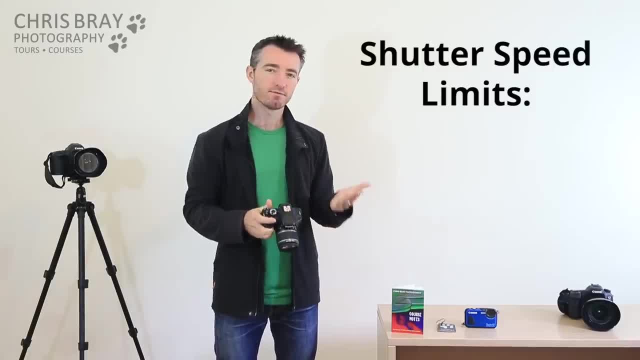 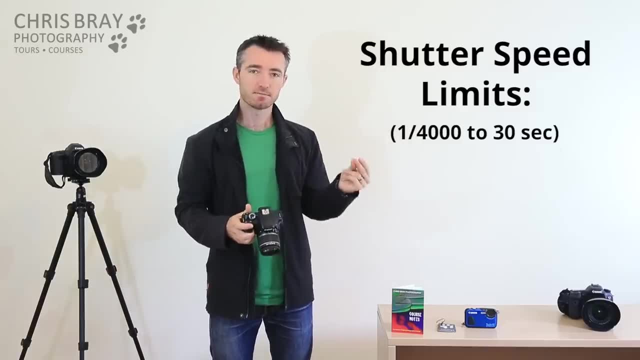 It'll always keep you within certain limits, either a shutter speed limit. you'll find that the fastest photo your camera can probably do is about 4,000th of a second. some cameras can do 8,000th of a second, but that's a physical limit. 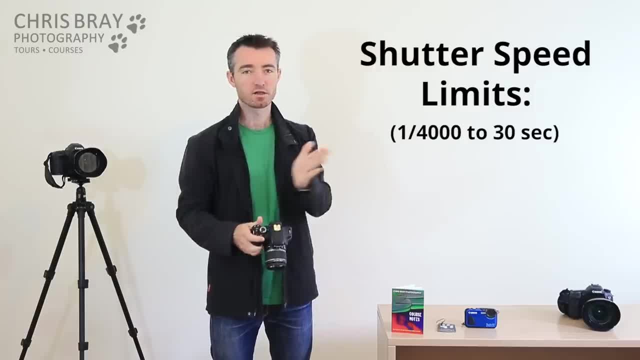 The camera just can't take a photo quicker than that. So if you were scrolling around and got to 4,000th of a second, you just wouldn't be able to scroll anymore. Fair enough. Or if you're going the other way, the slowest, longest shutter speed most cameras can do. 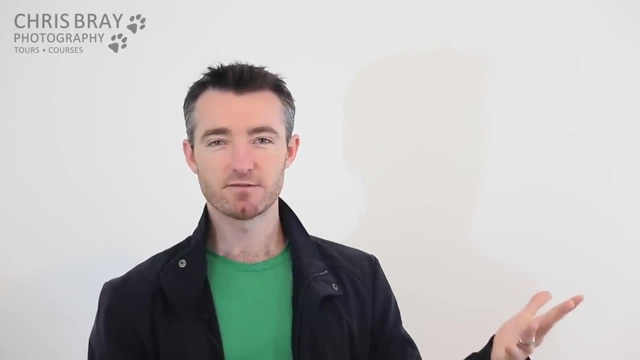 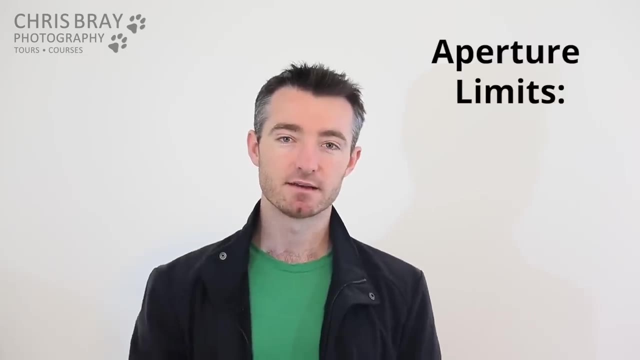 is 30 seconds. You can take a longer 2 hour star trail photo, but to get longer than the 30 seconds, you do need to start plugging in external devices. More commonly, though, you're going to come up against an aperture limit. 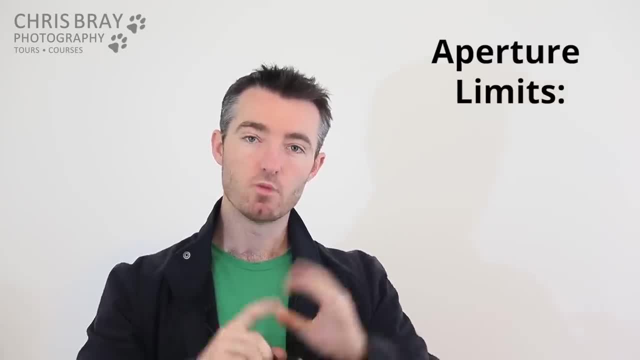 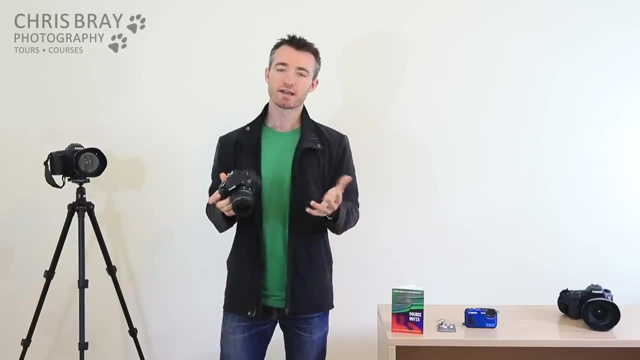 Because whatever lens you've stuck on the camera, the aperture hole can probably only open this big or go down this small. So you'll be scrolling around and your f-numbers will just stop. Fair enough. So how does your camera work out? how bright you want the photo to be? 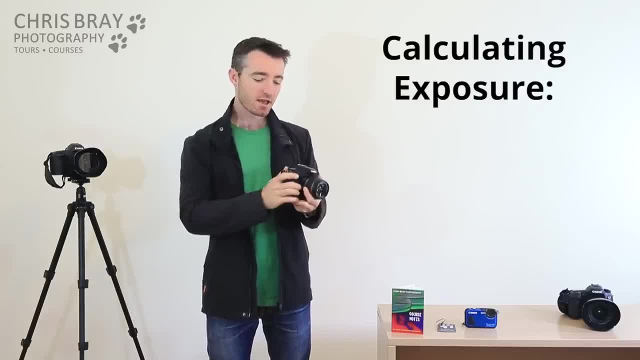 Well, it's actually very simple. Inside here there's a thing called a light meter and when you half touch your button it's trying to find something to focus on. it's also looking at how bright the world is out there and it just decides how much light it needs to collect to give your photo. 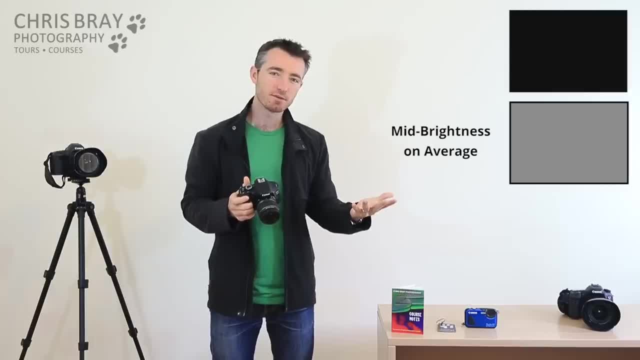 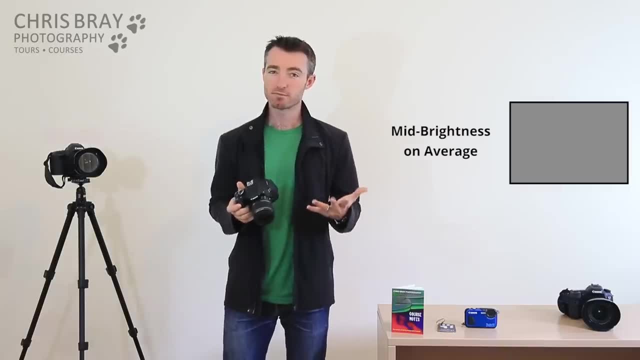 on average mid-brightness, Halfway between being totally black and underexposed or totally white and overexposed, Just on average mid-brightness. But a lot of cameras have different metering modes in them: matrix metering evaluative. 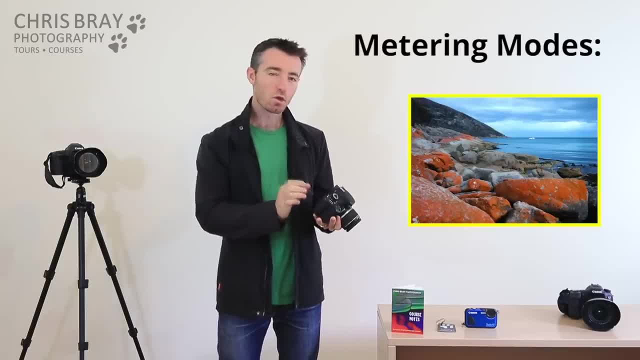 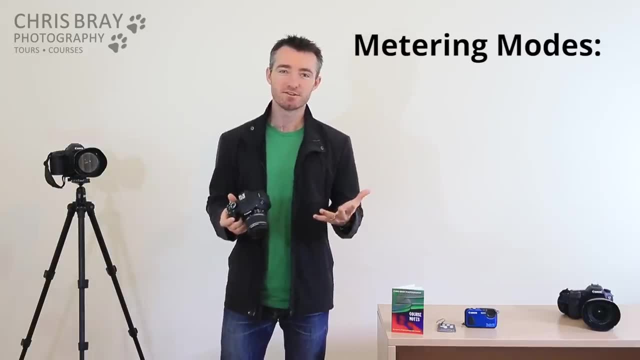 metering and so on. All those things are doing is just telling the light meter which part of the photo to look at, which part will come out being mid-brightness or whatever you tell it to be. So let's take a look at the one that I recommend you use, which is for a Canon evaluative metering. 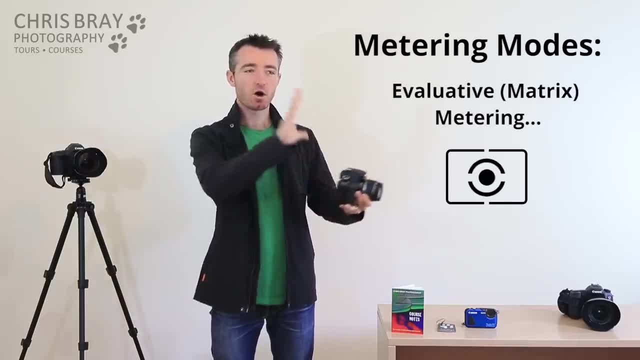 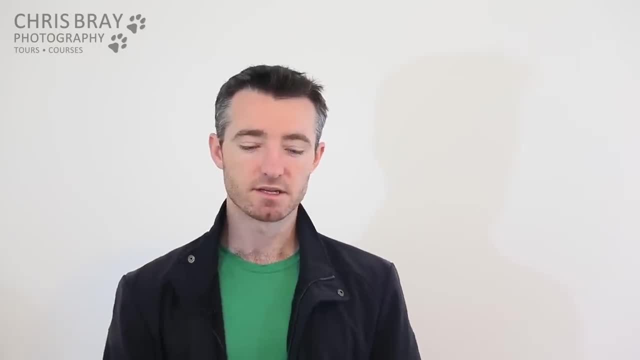 or Nikon calls that, matrix metering. Now that's where the light meter is: looking at the whole picture overall and making sure it comes out mid-brightness or whatever you tell it to. Now that actually works out quite well for most photos, because your typical scene actually. 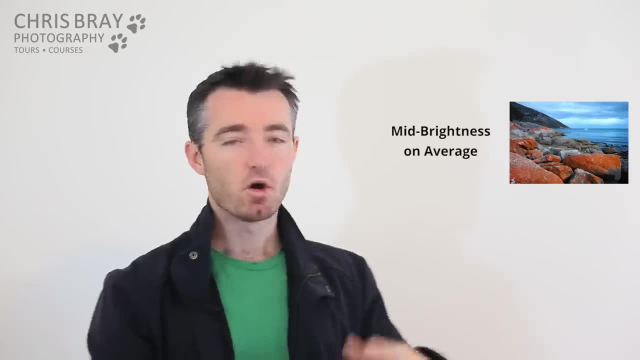 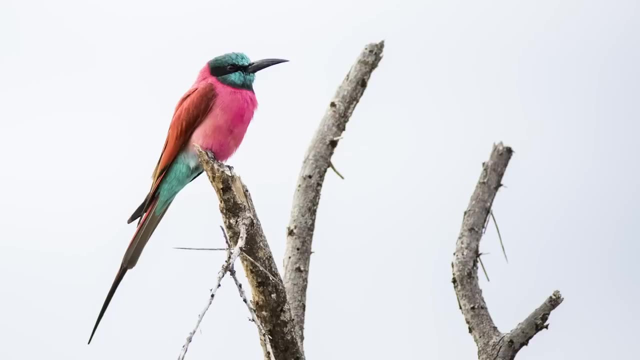 has about as much dark stuff as it does bright stuff, and on average it's mid-brightness, But of course it's not going to be perfect for every situation. Take a look at these examples. So here we have a bird in a tree. that's correctly exposed, but it is actually quite bright, isn't? 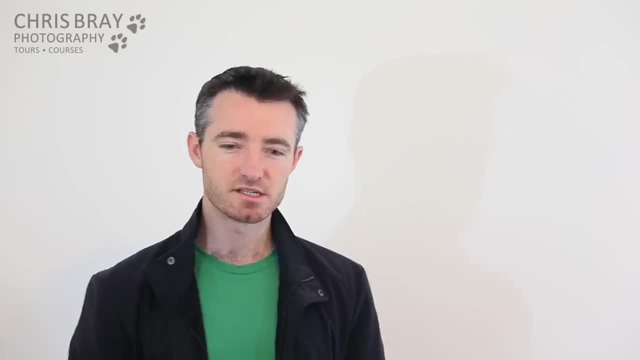 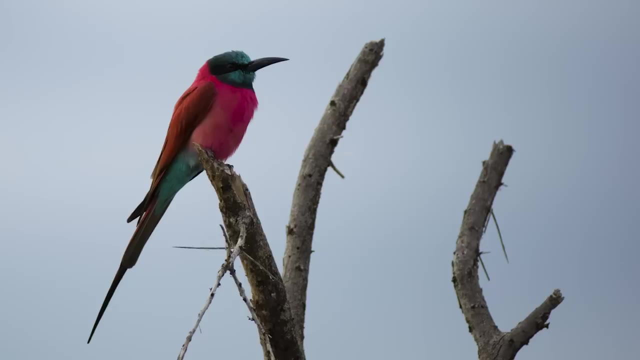 it. There's a lot of bright sky back there, So what tends to happen in these situations is that your camera looks at the scene and goes: well, I'm going to collect enough light to be mid-brightness overall, and your photo ends up looking a little bit like this. 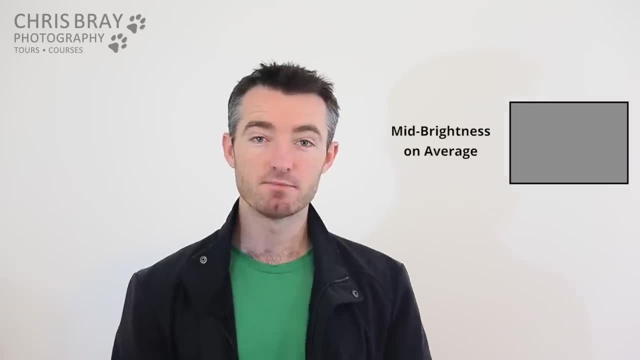 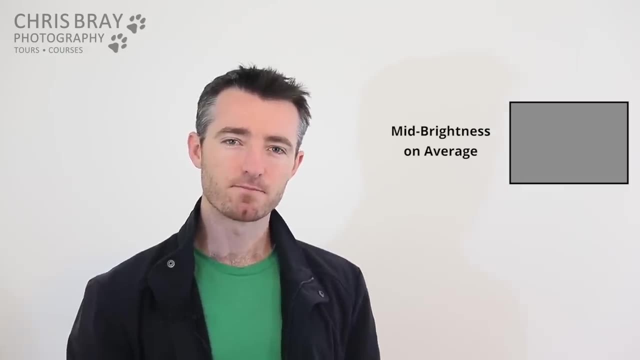 Quite dark and drab compared to what you actually wanted. That's because it's giving you a mid-brightness photo, but actually what you wanted the real world was quite a bright scene, So you'd need to find a way to tell your camera to make that photo brighter. 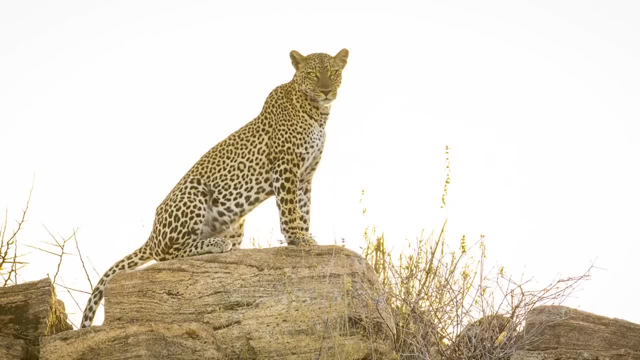 Another classic problem is when your photo is backlit like this one. There's so much bright light in the background that the camera just goes. well, I'm going to collect enough to make it a mid-brightness photo for you, and you end up with a shot. 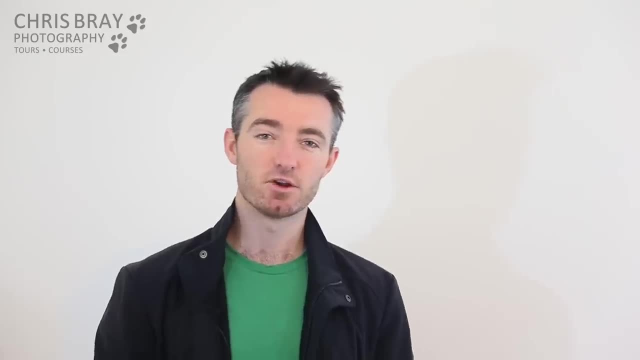 a bit like that. Your subject just looks like a silhouette. We've all done this before, you know. when you accidentally catch a window in the background of your photo And your subject is just a dark, If you think about it, that photo is still mid-brightness overall. half the photo is. 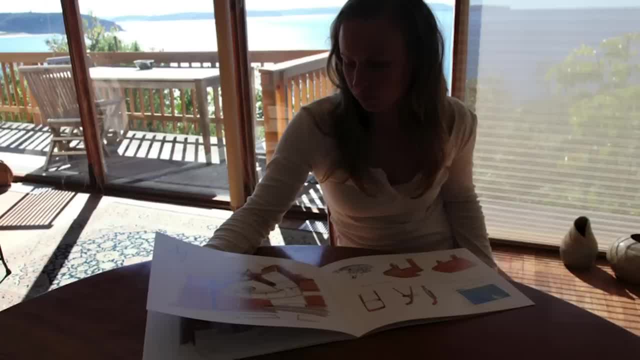 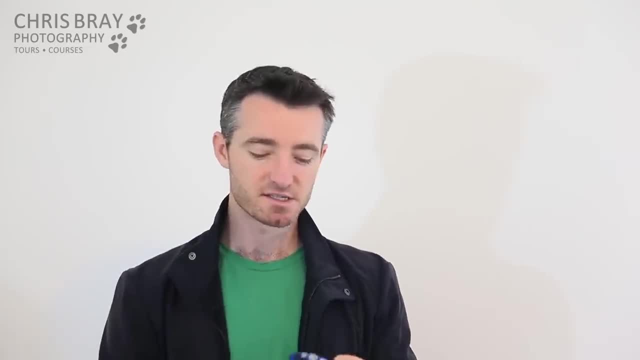 black and the other half is white, but the thing we're interested in, our subject, is way too dark. So again, we need to find a way to control this exposure brightness. Quick little detour onto a compact camera. You might have noticed these things just have so many different scene modes these days. 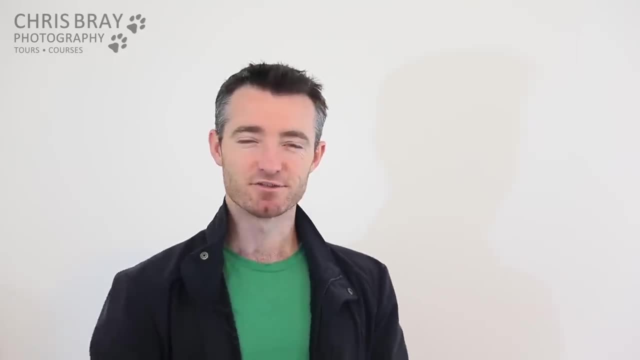 There's like pet mode, underwater mode, snowman mode, and I never used to really use those modes because I didn't really understand what they did. But I've since learnt that a huge amount of programming have gone into those different modes. It's totally worth scrolling to the different setting if you're taking photos of fireworks. 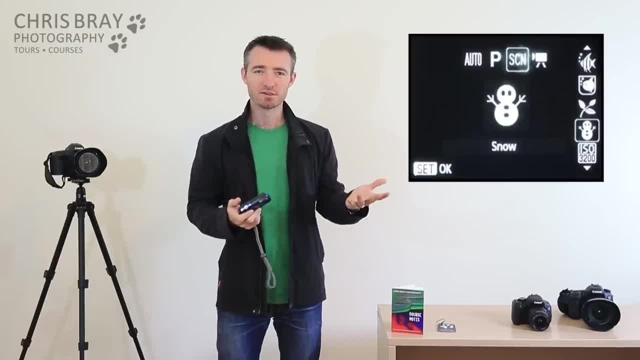 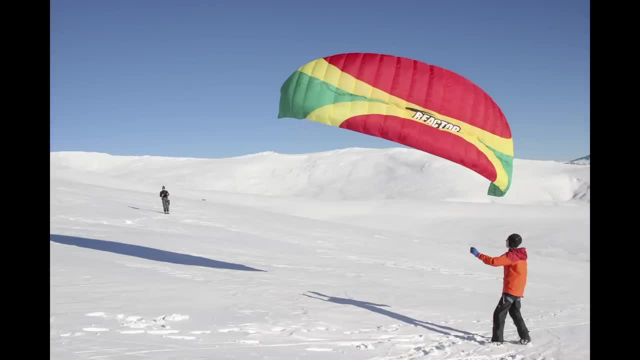 go to fireworks mode Or snowman mode. What snowman mode is doing is just saying: hey, I'm in the snow, I expect a lot of bright white stuff around. collect more light than you were going to give me a nice bright white. 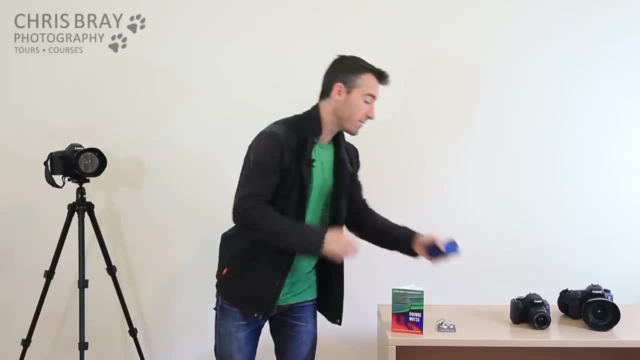 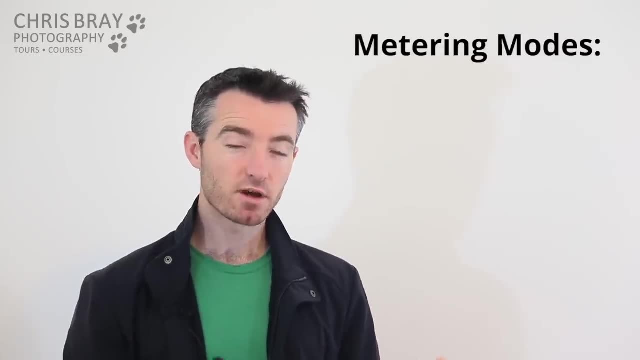 photo, not a dull grey snow, But back on a real camera. maybe you're supposed to use different metering modes Now, different brands, of course, and different cameras offer different things. but basically you've got quite a few options there normally, but we'll go through them all, so you know. 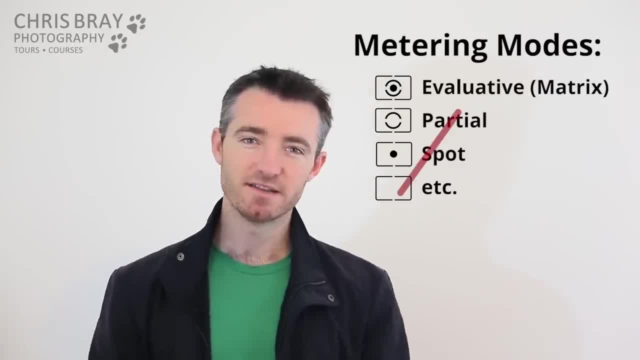 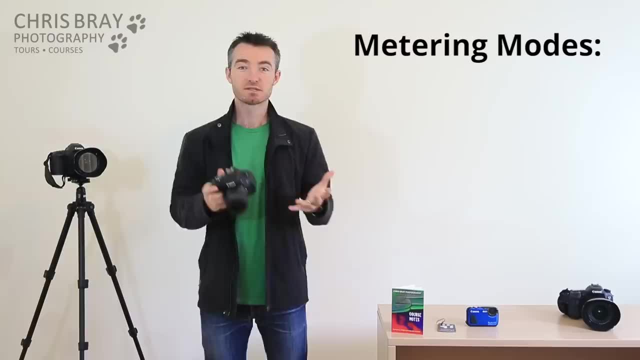 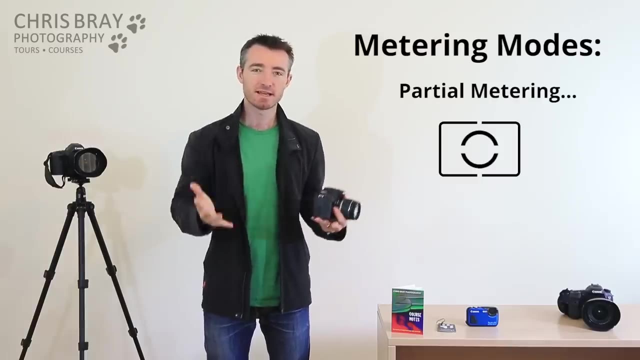 what they are. So let's take a look at partial metering. That's where the light meter just looks at the middle region of the photo and makes sure that comes out mid brightness, and it doesn't look at the outside stuff. So in a situation like this that would kind of work, because it doesn't get blinded by 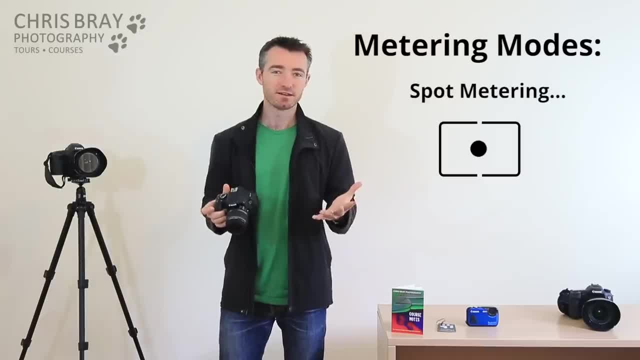 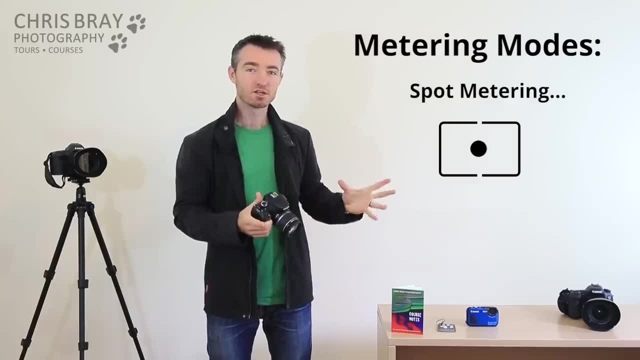 all this extra bright stuff on the outside, What about spot metering? Now, spot metering is lethal. It's one tiny little point, That's all the light meter is allowed to look at And it bases the whole image off, making sure that little point comes out exactly mid brightness. 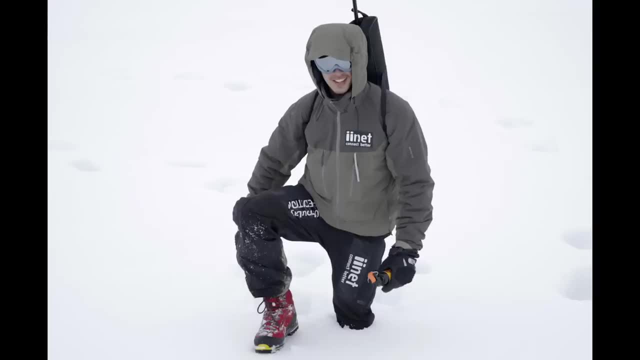 So that's great if you're pointing at something that's supposed to be mid brightness. So for a photo like this one, maybe that would actually come out alright, because that dot is supposed to be mid brightness. But what if you missed and you pointed over here instead? 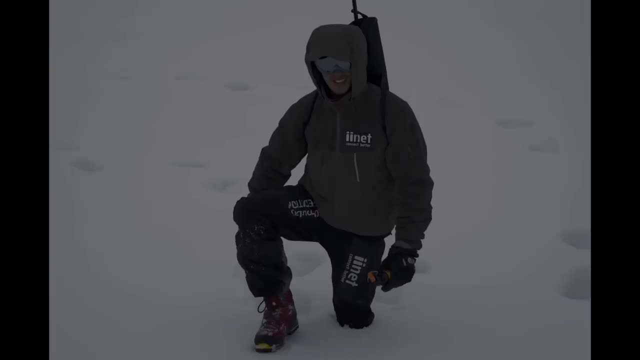 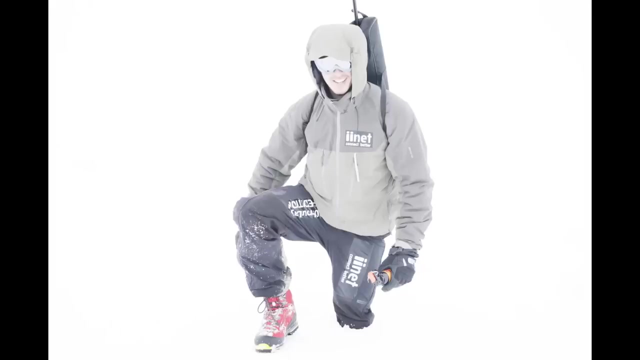 The camera will make sure that that part comes out exactly mid brightness, which just looks terrible. Or if you point it over here, something that's supposed to be quite dark, then the camera is going to make sure that dark thing comes out being mid brightness and you end up with 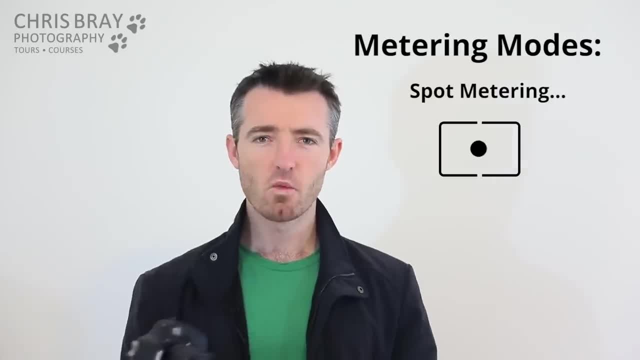 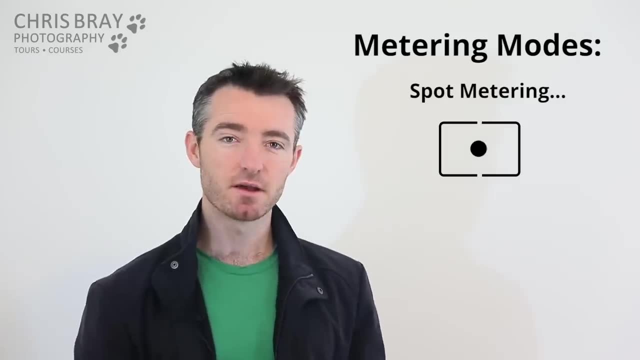 a massively overexposed shot. Most of the time, you're just left wondering going. why do they give you such a crazy over the top setting that ends in disaster most of the time? Well, it does have a use, but it's designed for in a studio setup where, just before you, 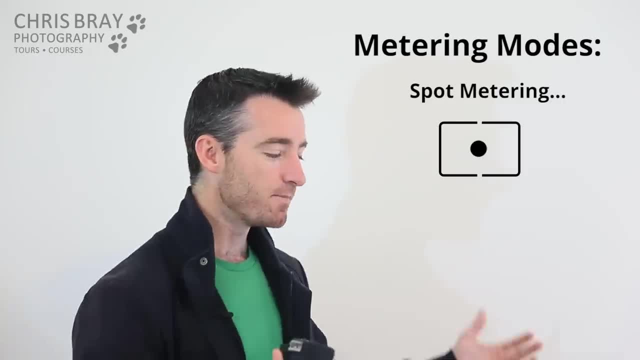 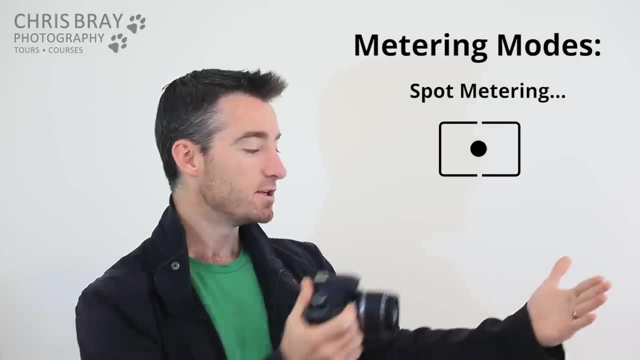 take a picture of a model or a pack of cornflakes. whatever you're photographing, you'd quickly hold up what's called a grey card in front of your subject. you know a bit of cardboard or perspex that is exactly mid brightness. 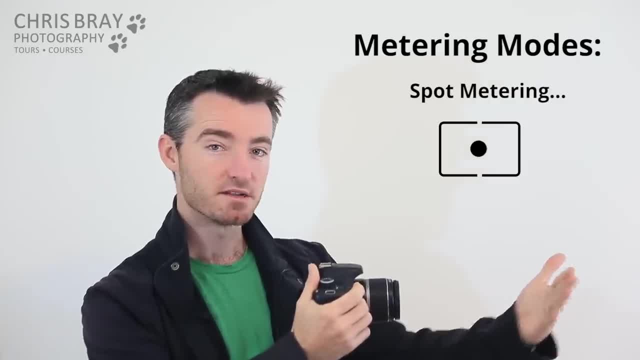 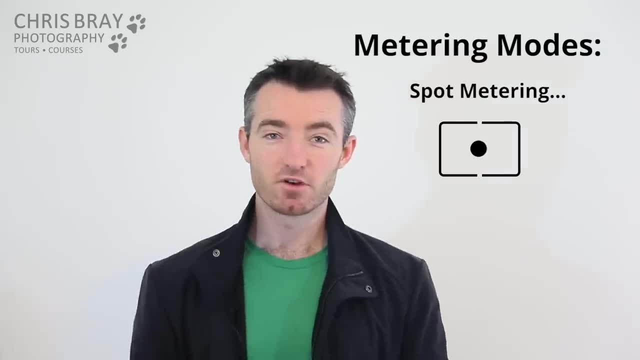 And you'd spot, meter off that and go, beep, make sure this comes out exactly mid brightness. because it is mid brightness, beep, take it away, take the shot and, lo and behold, you end up with perfect exposure every time. Now, that's great if you've got a grey card in a studio, but out in the real world it's. 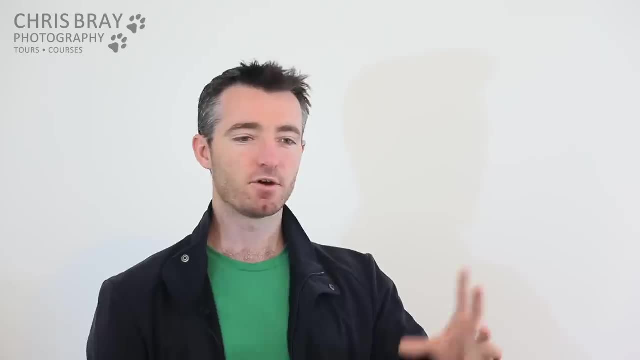 just impractical. Some people will usually say about now that they find that if they're photographing a bird in a tree and it normally comes out being silhouetted, if they change to spot metering and then try it, then it might come out better. 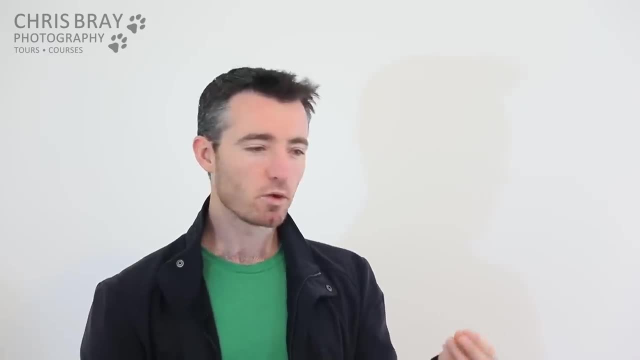 Yeah, it probably will come out better, but the problem is it still won't be right. What happens if now it's too bright Or it's too dark? Are you supposed to then change to centre weighted averaging metering? No, There is a whole system in your camera, everyone's camera, designed to help you control your 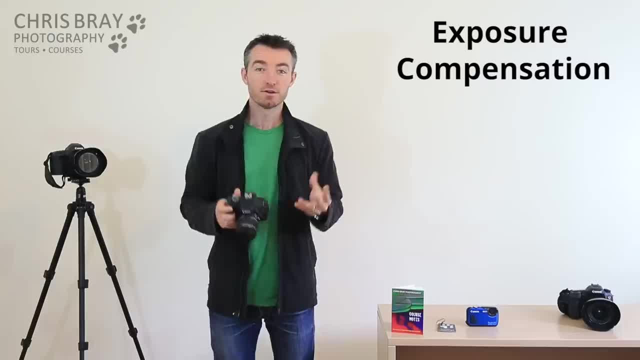 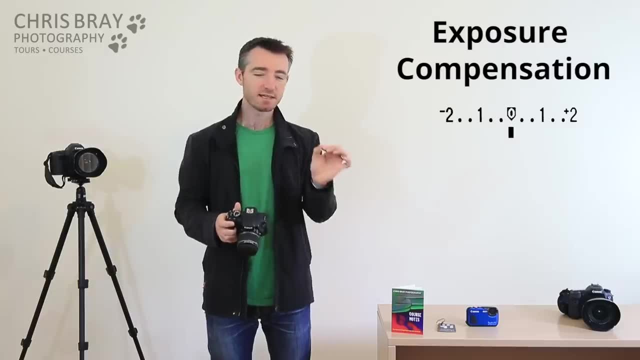 exposure Minus brightness. Exposure compensation. You've all seen this little slider indicator before. it's often on the back of your camera, even inside the viewfinder, when you're looking through. it's really important. If you leave it in the middle on zero, that's when your camera is going to collect enough. 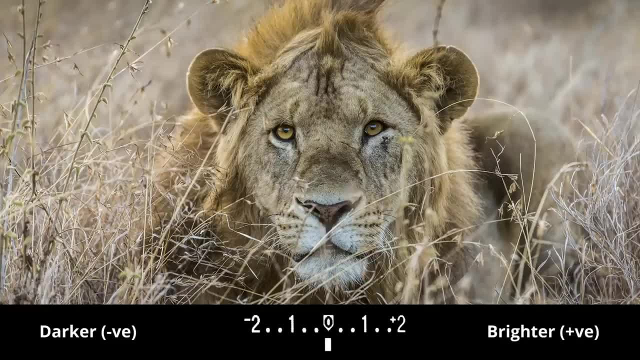 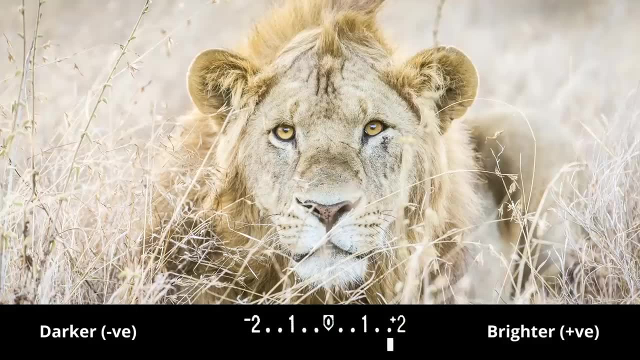 light for your photo to be mid brightness on average. But if you move it down minus one, minus two, it's going to collect less light, your photo will come out darker. Or if you go plus plus one plus two, then your photo comes out a predictable amount. 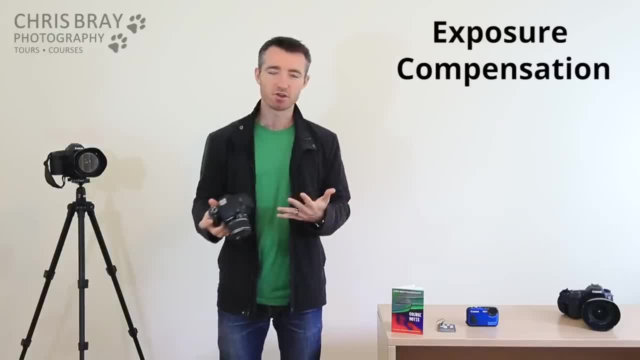 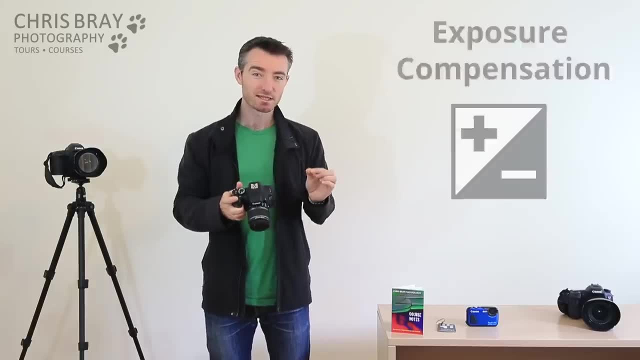 brighter than mid brightness. Obviously, how you change it depends on what camera you have, But most of the time you'll find your camera has a little plus minus brightness button on it, Just like that. Don't get confused by one that looks like that: a little plus minus brightness with. 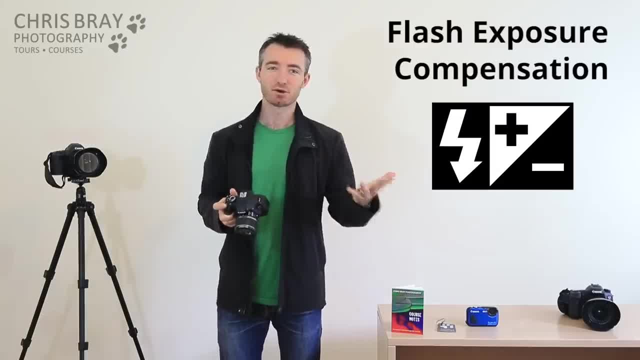 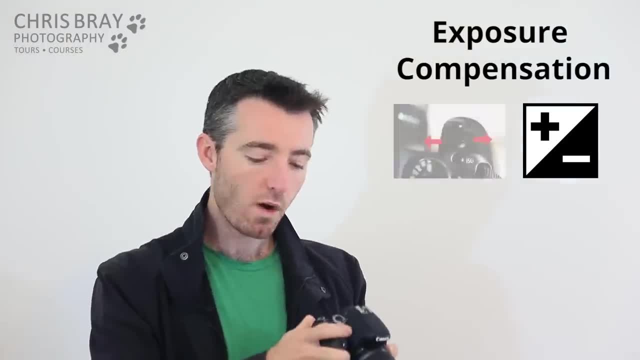 a lightning bolt next to it. that's changing the exposure of your flash something totally different. But you're just looking for a little dedicated plus minus brightness button. You'll have to press that button in and keep it held in while you scroll one of these wheels. 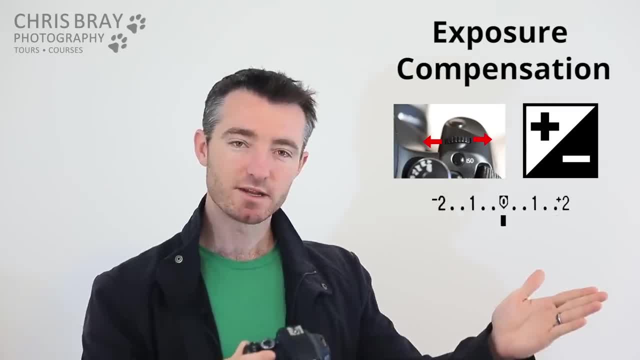 and then you'll find that little marker will move up or down and then, wherever it is when you let go, it'll stay there And the next photo will be really dark, and so will the next one, in fact, even if you. 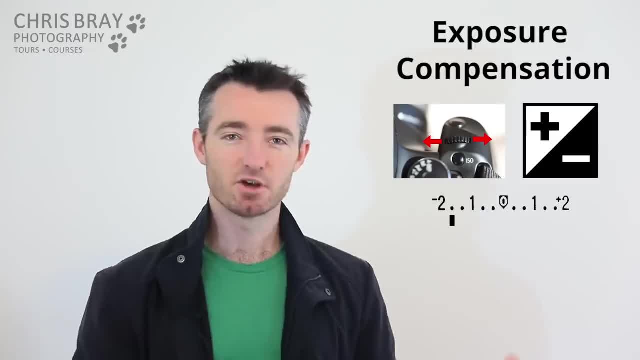 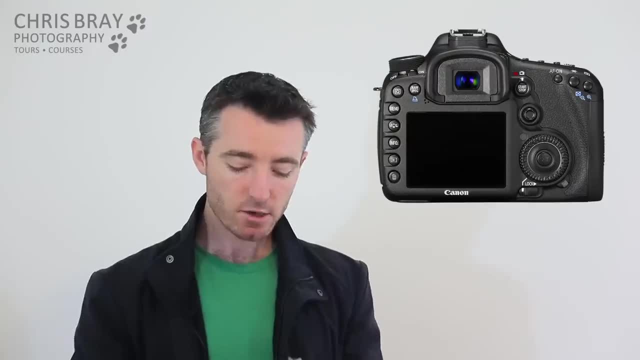 turn your camera off And pull it out again next week and take a picture. it'll still be on minus one or whatever you put it on. So you've got to get in the habit of checking where you've put it. For some other Canon cameras, about half way up their range or better, you don't have to. 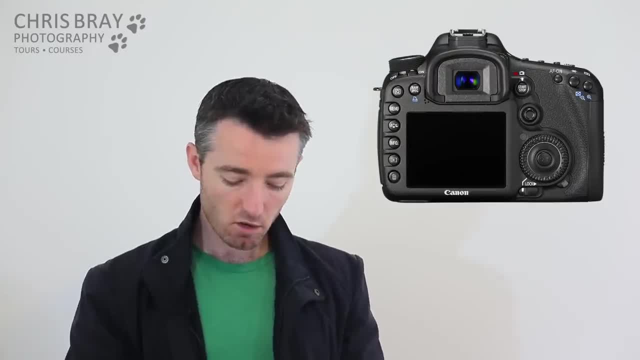 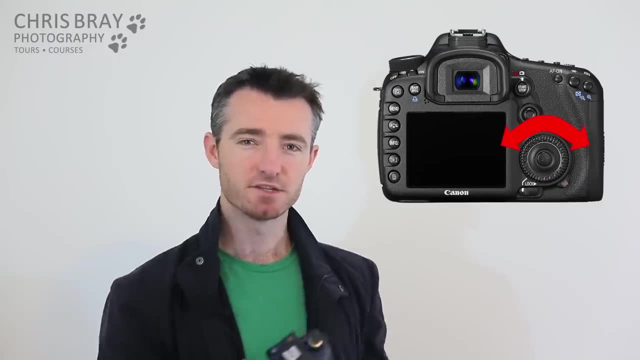 press and hold some awkward button in. while you scroll On these ones, there's a whole wheel dedicated to it right next to your thumb, And any time you bump that wheel, the photo becomes brighter, darker. It shows you how often you're supposed to be doing this exposure compensation there's. 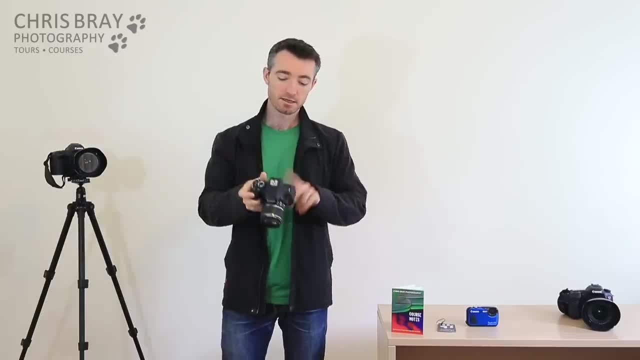 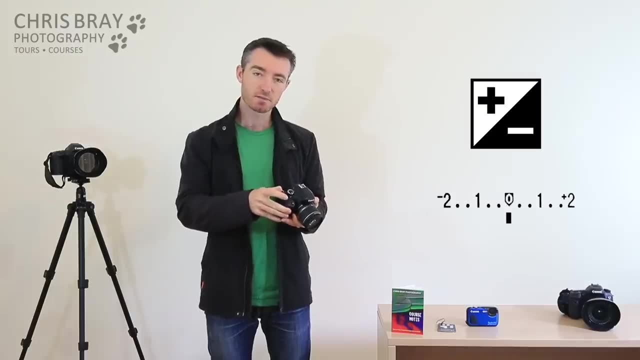 a whole wheel there right next to your thumb. So generally you take a picture, you look at it on the back of the screen and you say I think it's a little bit too dark, So then you need to brighten it up. so you'd go hold the little plus minus exposure compensation. 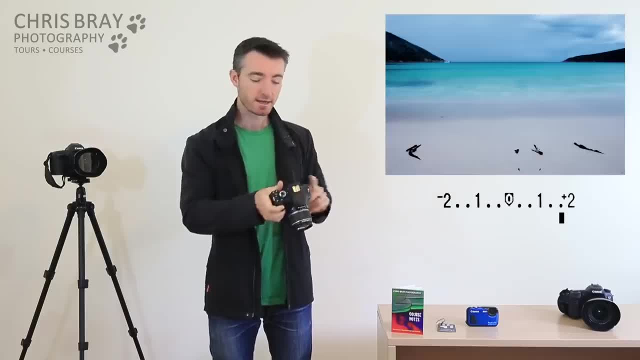 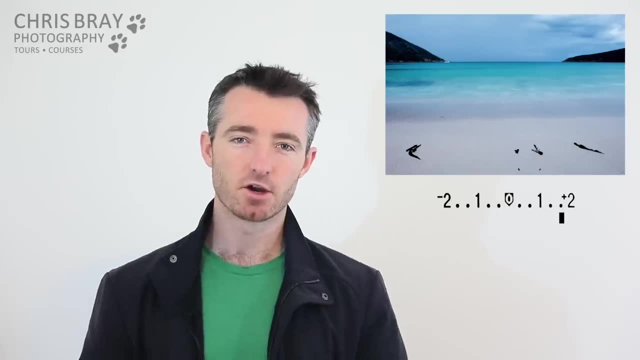 in, plus one, plus two, take the photo again and then hopefully it comes back looking better. I know that sounds like a little bit of trial and error, but you'll get a whole lot better at judging it and you won't need to take the incorrect photo first. 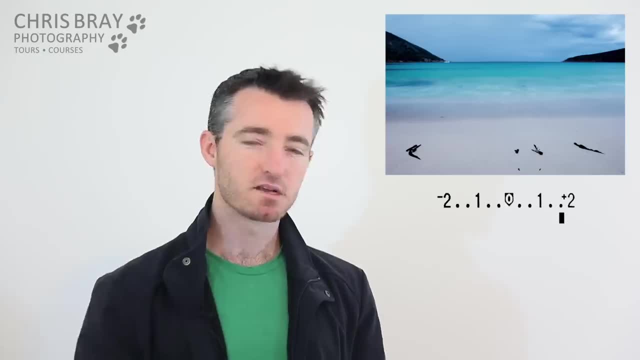 You'll be able to say, oh, I'm in the snow, it's quite bright. I already need to have it on about plus one and two thirds or plus two or whatever it is. So it's really important to be able to control the brightness of your image, not only because 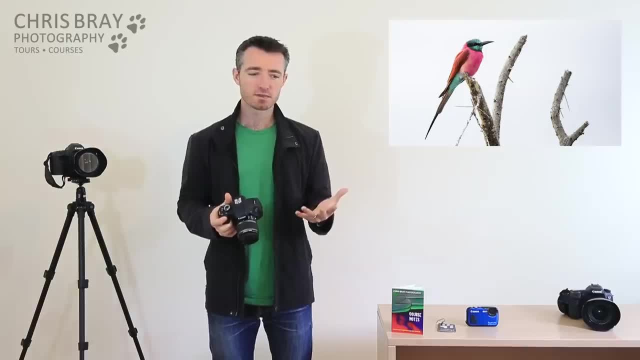 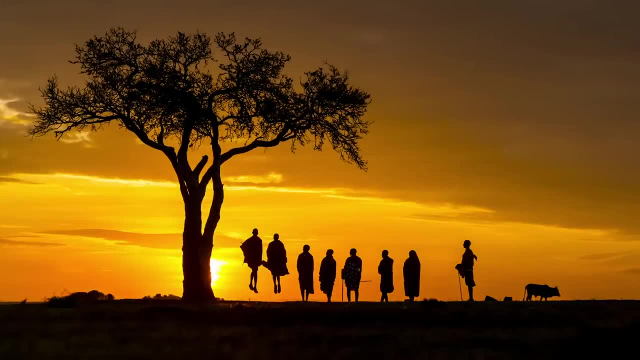 the camera gets it wrong sometimes and you need to be able to correct it, but also because it opens up creative options for you to deliberately make a scene much darker, maybe for a good silhouette and rich up the colours in the sunset or something, or to really overexpose. 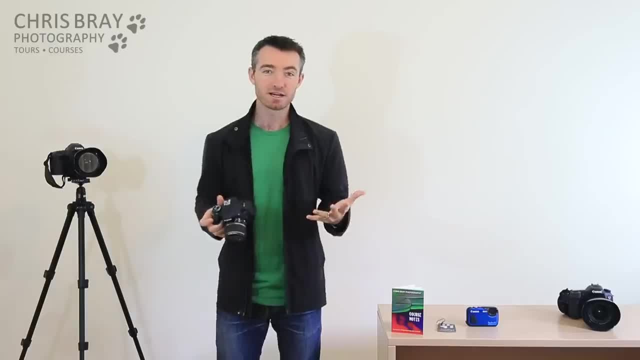 the photo deliberately and end up with this really bright washed out effect. But a lot of the time, of course, you actually want to get perfect exposure and if you want to be really sure, looking at the photo on the back of the camera, it's really hard. 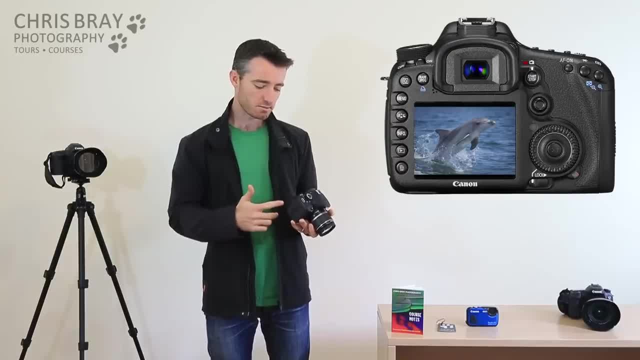 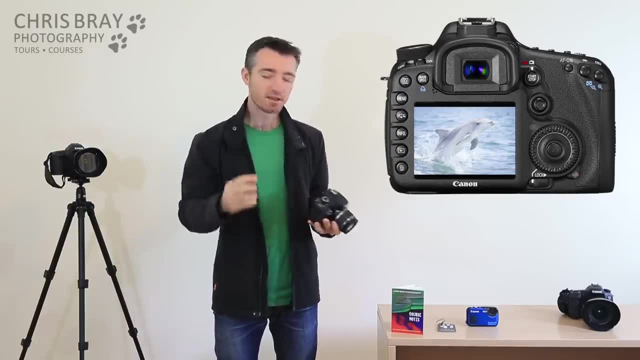 to tell which one is correctly exposed. Is it this one? Maybe it's that one, Who knows? And to make it worse, you can change the brightness of your LCD screen on the camera. If you put your screen brightness on plus ten, all of your photos are going to start. 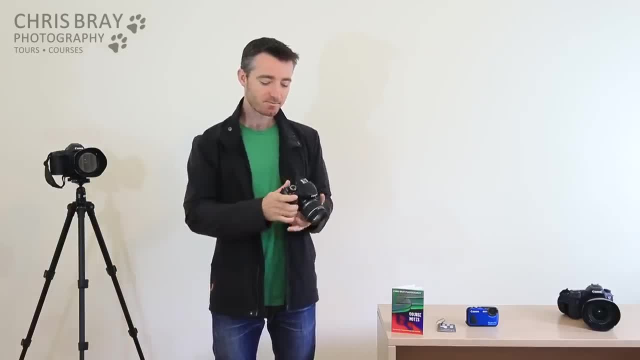 to look really overexposed. You know they're not. your screen brightness is just too high. Also, you know, when there's sun shining around and everything's reflecting and glaring off there and you can't even see what's on the screen anyway, 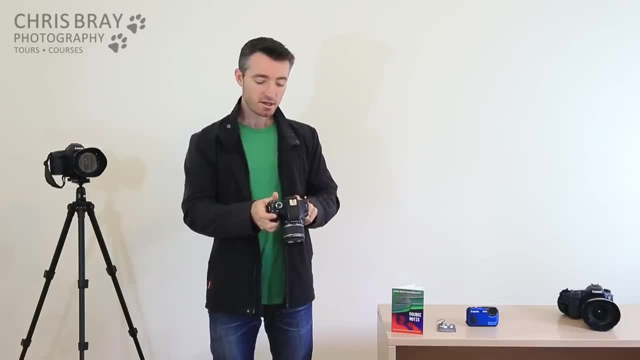 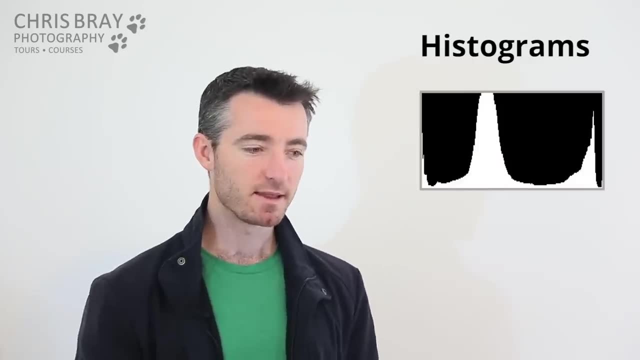 There's plenty of times where you just can't trust what's on that back screen. So these are the situations when histogram graphs can come in handy. Now, you've probably seen these little graphs. from time to time They just pop up and people are like: what is that and how do I get rid of it? 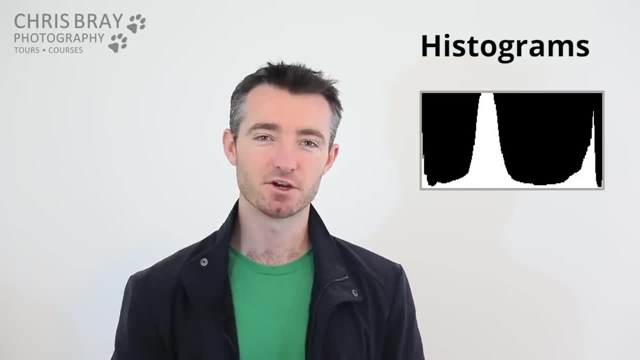 But it's actually very simple to understand and really very useful, and it's the only thing we show you in the entire course. so bear with me. A histogram graph just tells you how much of different brightnesses you have in your picture overall. 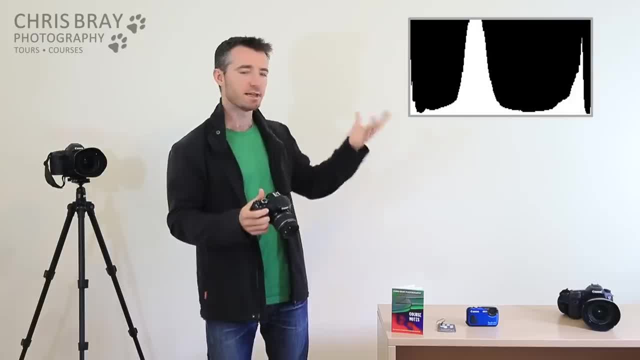 You know, a spike on the left hand side of the graph doesn't have anything to do with the left hand side of your picture or anything like that. It's an overall brightness scale. So going across the bottom, that's your brightness. Going further to the right is getting brighter. 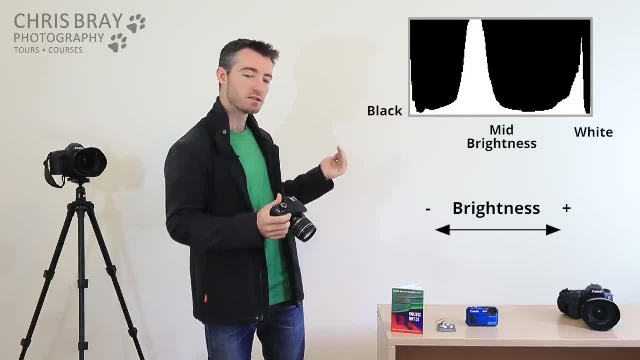 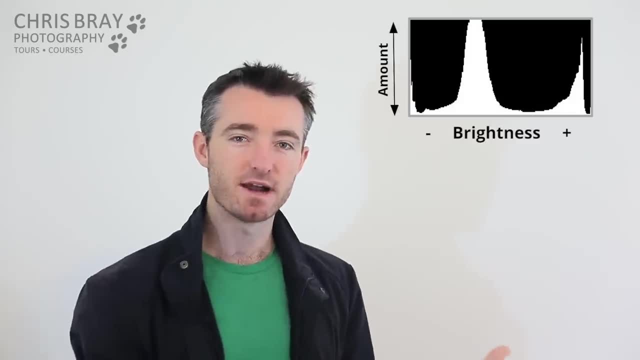 And coming back this way to the left, is getting darker. So pure black is at this end on the left and pure white is at the far right hand end, And the height of the graph at any point is just the amount of that particular brightness. 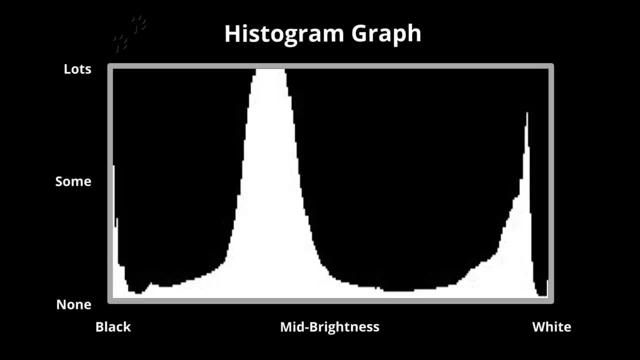 So we can look at this one and say, well, how much black does this photo have? And you look at it and go, black is at that left hand end. oh yeah, there's a fair bit of black there. And then there's nothing, really, until we get to the mid brightnesses. there's a huge amount. 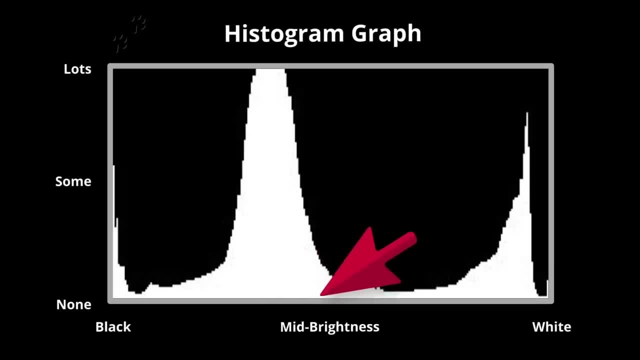 of mid brightness stuff- in fact slightly darker than mid brightness- that big spike, And then there's nothing until we get to the bright stuff. there's a fair bit of bright stuff there, And then there is a tiny little bit of pure white there as well. 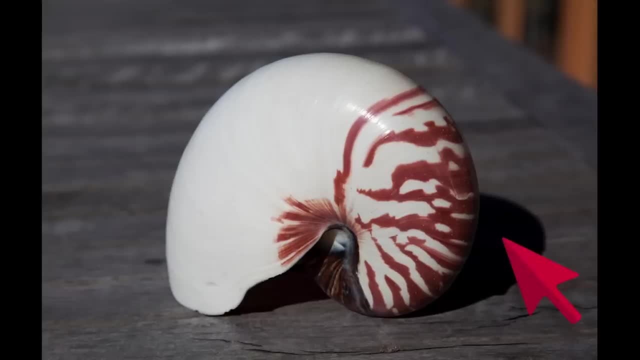 Now looking at the picture that came from, that makes sense. You can see we've got some black there, We've got a huge amount of slightly darker than mid brightness stuff and we've got some bright stuff and we do have that little bit of white in the highlights, just there. 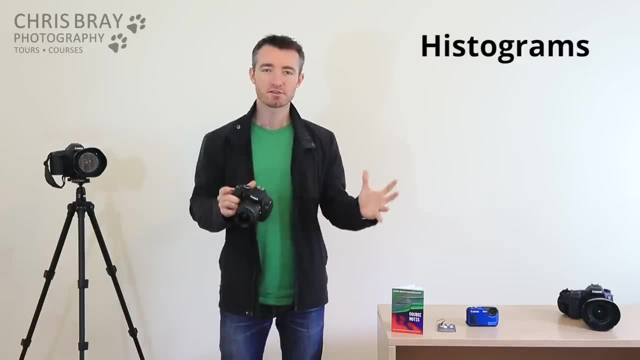 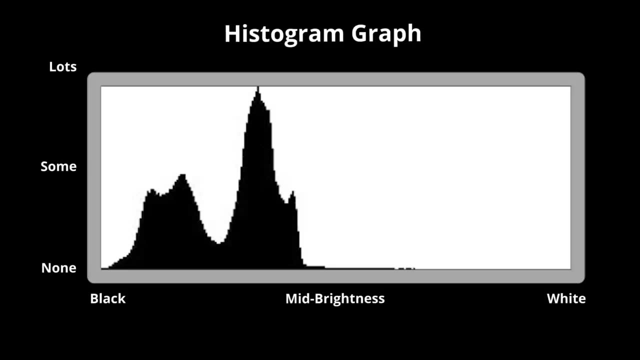 So why this graph is useful is: at a glance, you can see the true brightness of your image, irrespective of what you might have your screen brightness set to, or if there's sunshine around and you can't tell. You can just look at a graph like this one and say, well, look, all the information is. 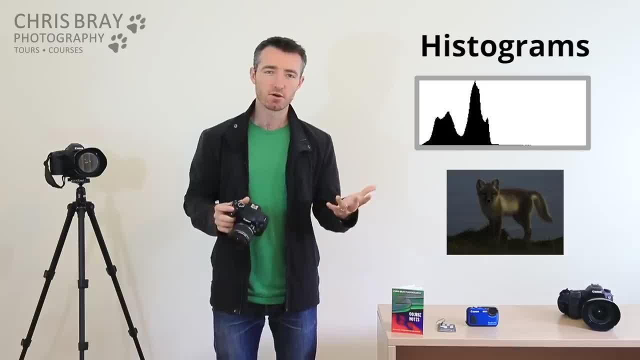 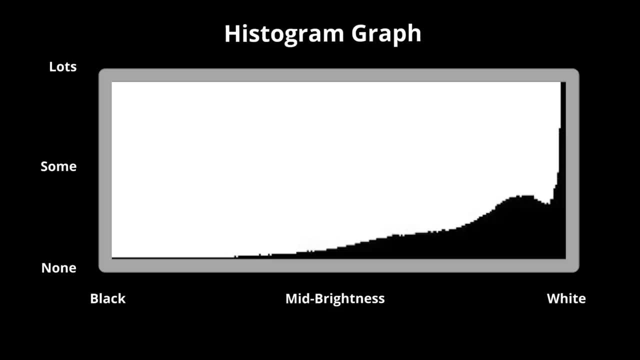 shoved down the dark end of that graph. Unless you wanted a very dark photo, that's probably underexposed. You need to brighten it up and take it again. What about this graph You can see here there's a huge amount of white. 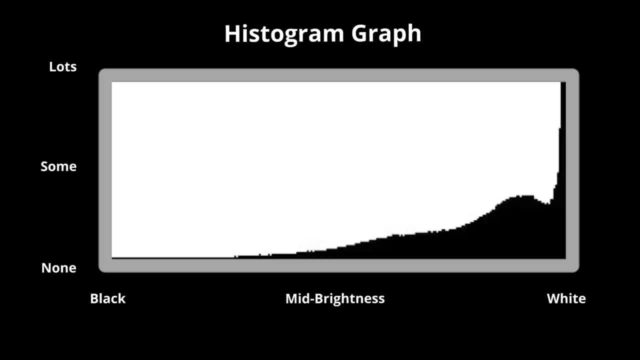 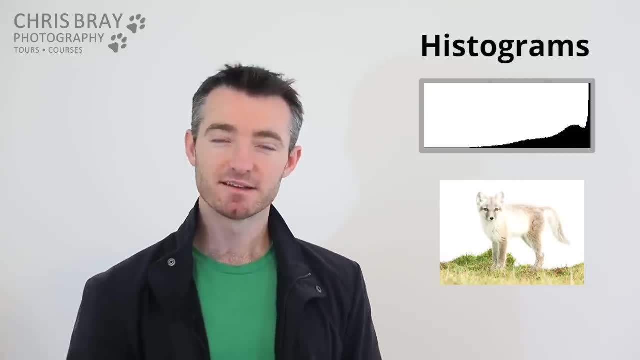 Lots and lots of white and lots of bright stuff and then the graph kind of peters off. You've got no mid brightness stuff, no blacks, no dark stuff. So that is a very bright photo. So unless that's what you wanted, that's probably an overexposed picture. 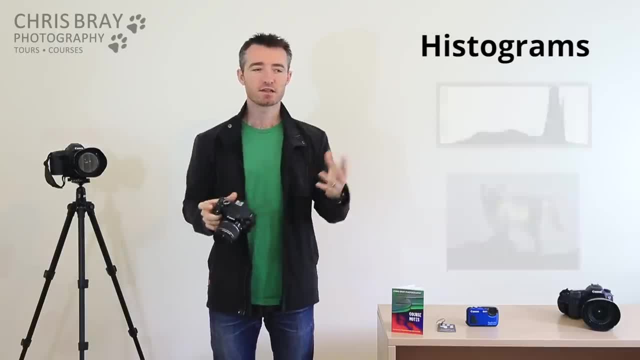 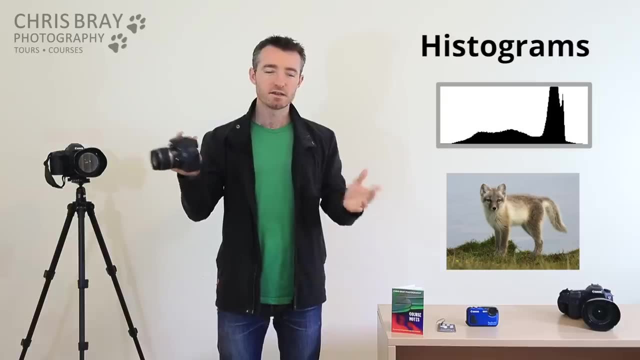 What you're after with your typical histogram graph is just a good spread. You know, they say most photos should have a little bit of black in the darkest part and the brightest part of the photo in the highlights is probably just supposed to be white. 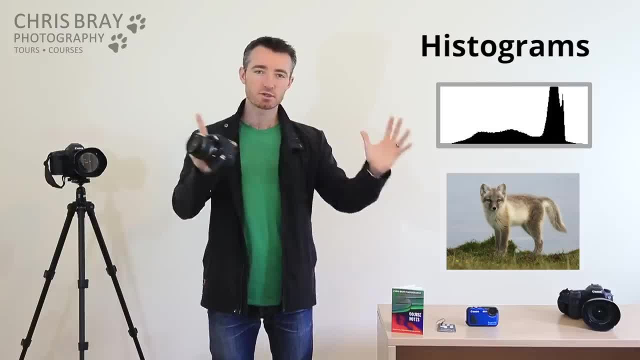 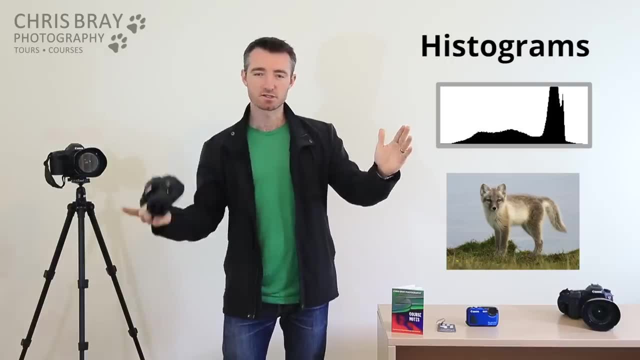 So it's okay if it kind of gets to the two ends of the graph. What you want later in the graph you want between the two ends. You can think of it as a goal post if you like. You want all the photos safely between the two ends, not so dark that it's still black. 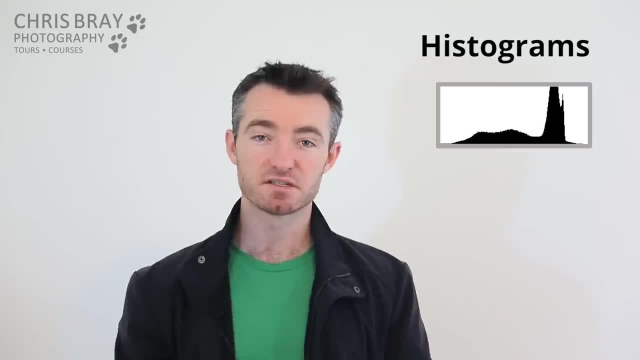 or not, so bright that you've just blown it out and it's just become white. Don't worry about spikes. People often freak out about that. All a spike is saying is that you've got a lot of that particular brightness in the picture. 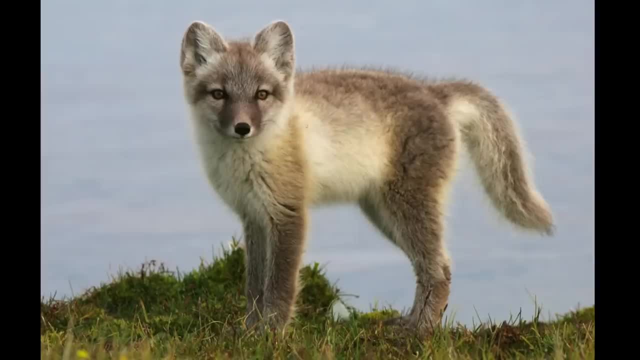 In this example. there's a fairly big spike there towards the bright end. That's just the water in the background. It's quite bright and there's a lot of it, so you get a bit of a spike building up in that part. 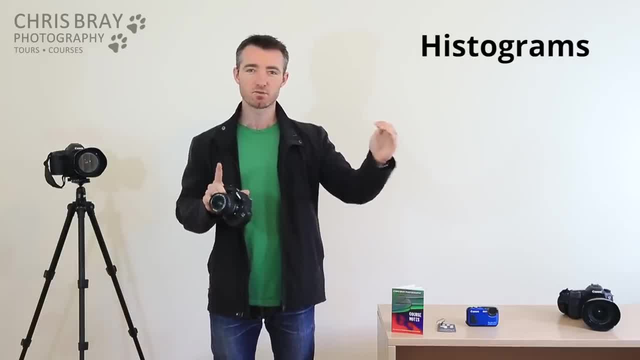 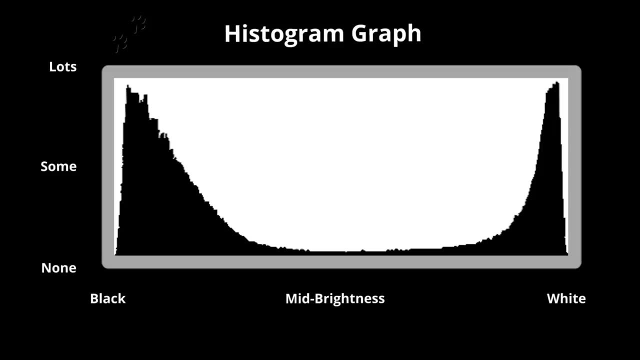 So what do you think the histogram graph would look like if you took a full frame photo of just a zebra skin, So black and white? Obviously, the graph's going to look a little bit like this one where you've got a whole lot of black and then kind of some shades near black, but then nothing until you get. 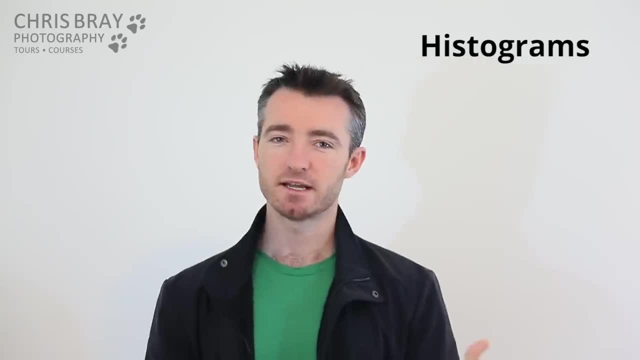 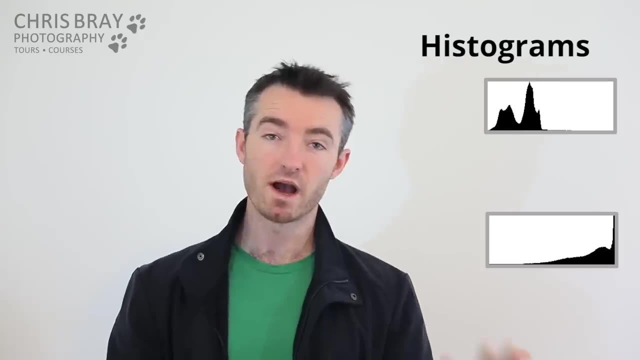 to the bright stuff: Some bright stuff and a lot of white. Now you can't just look at a histogram graph on its own and say, oh, that photo's underexposed or overexposed, because it depends on the image. Maybe it's supposed to be a very bright white subject. 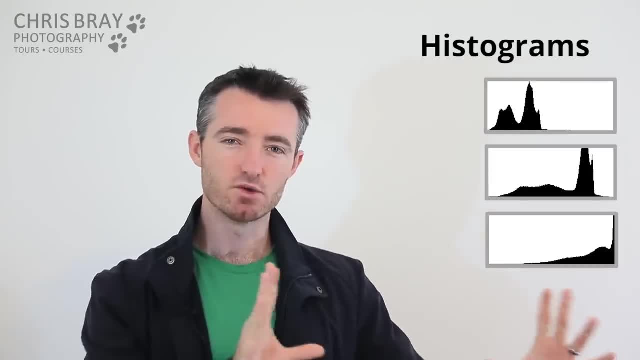 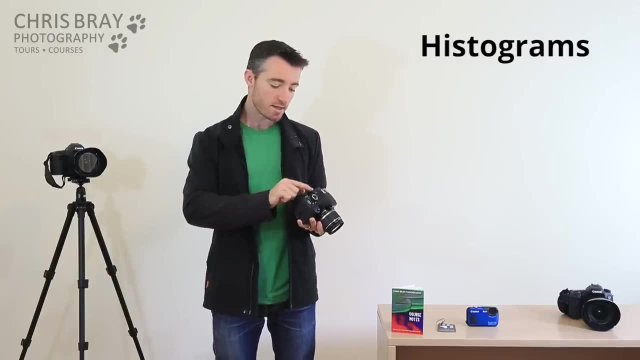 But generally speaking you just want your histogram graph safely between those two ends. So to look at your histogram graph, you've normally got a bit of black and white and that's probably in review mode, playback mode, looking at a picture you've taken. 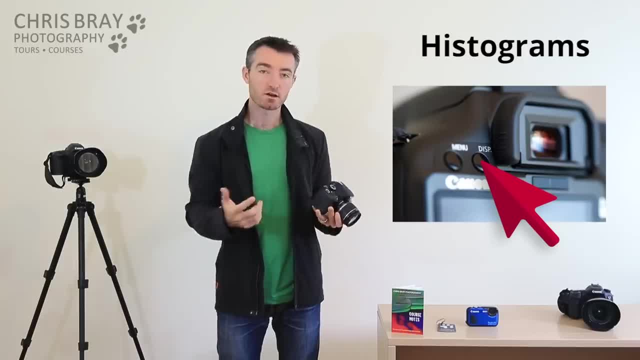 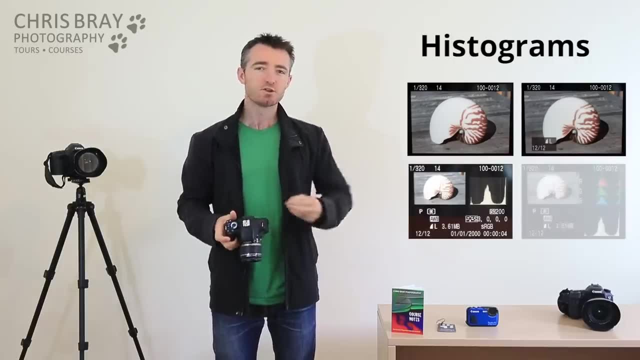 And then you either hit info or display a couple of times, or for a Nikon it's up or down And it just cycles through different pages of information and one of them will finally bring up your histogram. Don't worry about the one with all the different colors, you're just looking at that white. 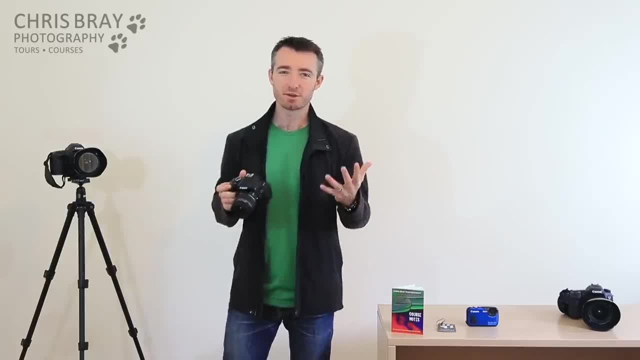 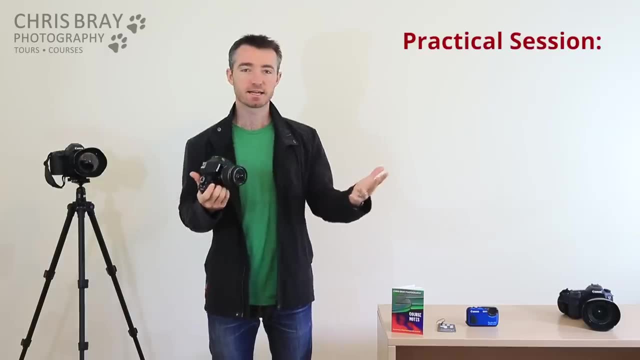 one. That's the overall brightness graph. Okay, so now's probably a good time to go outside and do our first prac session. So pick up your camera, make sure you're in P mode and then just go and find something to take a photo of- doesn't really matter what it is. 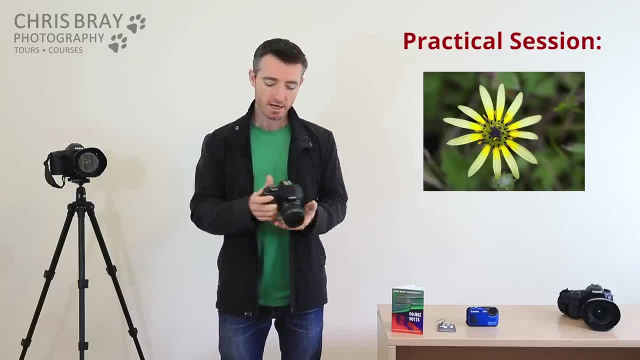 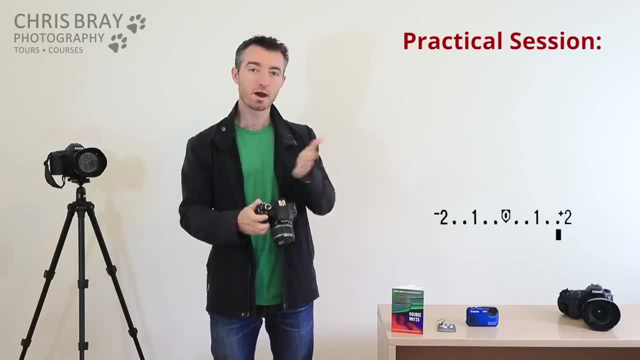 Take a picture- initially it should come out being mid-brightness on average- And then work out on your camera where that little plus minus brightness button is. press and hold it in scroll. do something quite dramatic like plus one or plus two. take the. 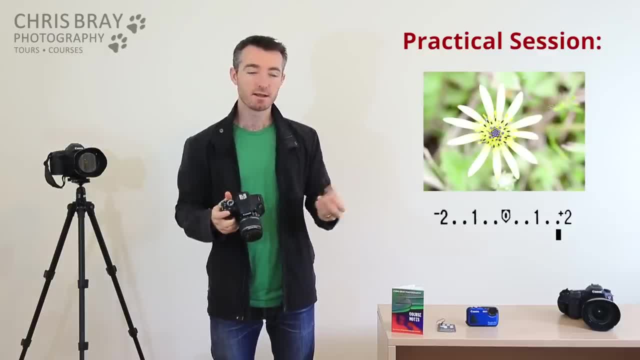 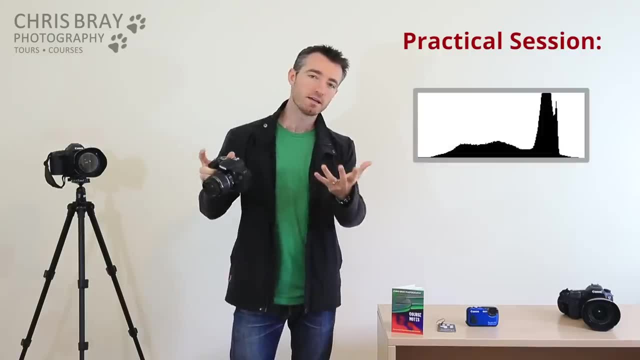 same picture again, and you should definitely see. the picture then looks a whole lot brighter And do a darker one as well. you know minus two, minus three. check out that. Maybe bring up your histogram graph as well and watch all that information shove down. 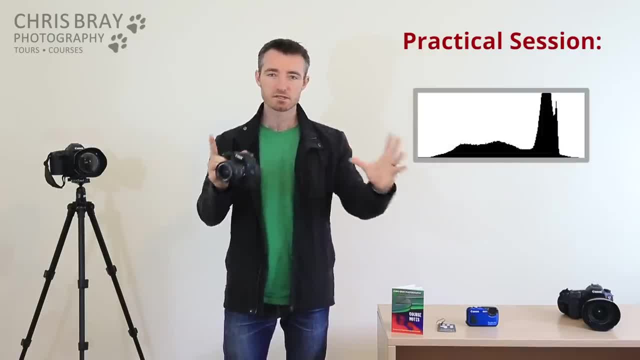 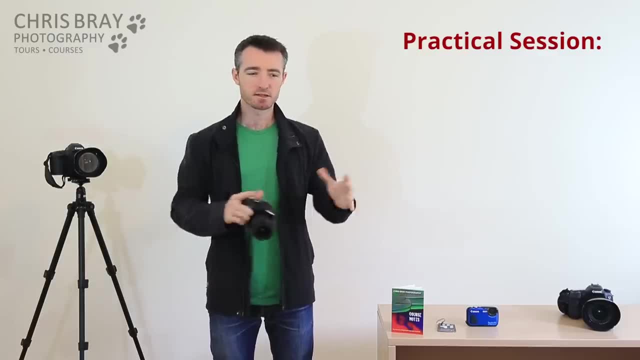 the dark end or move up to the bright end and try and get it at just about right, safely between the two. If you think that's all too easy and you've done all that before, a good extension can be to try and take a photo of something that's mostly white, like a sheet of white paper. 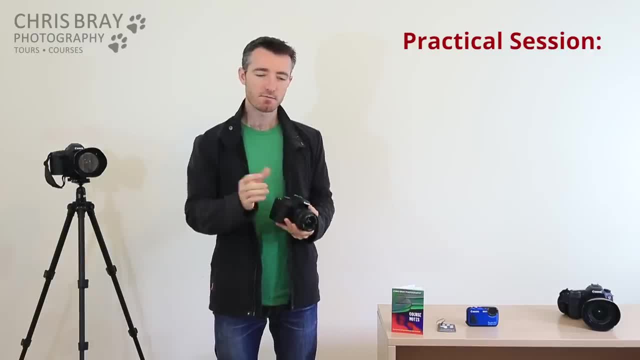 or something. If you take a photo of that, initially it's going to come out being a mid-gray sheet of paper, mid-brightness, And you'll be able to look at it on the back and just say: math's too dark, I'll go plus. 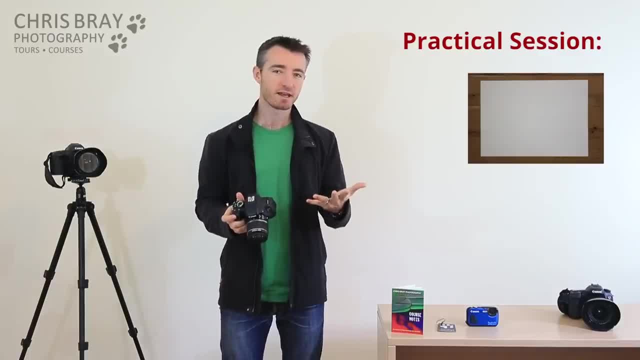 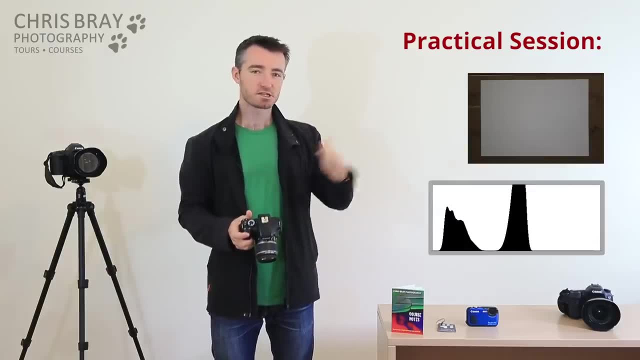 one take it again and then it comes back looking brighter and you might think that's okay. But actually if you checked your histogram graph, you'd probably find the first photo, the mid-brightness, that spike. The histogram will just be basically one big spike in the middle, lots of grey. 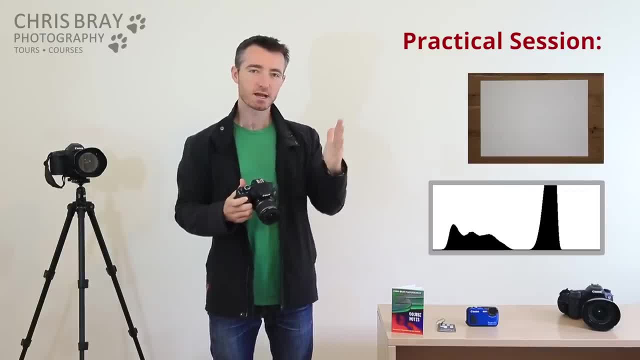 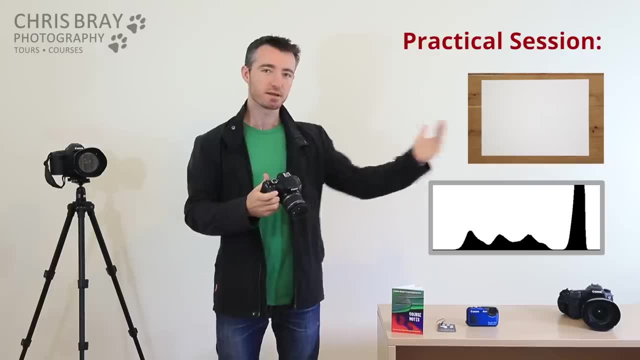 And you'd say, okay, so you go, plus one, take it again. That spike will move towards the white end, but it won't be anywhere near it. So you'd have to go, oh, plus two, take it again, and the spike would move even further. 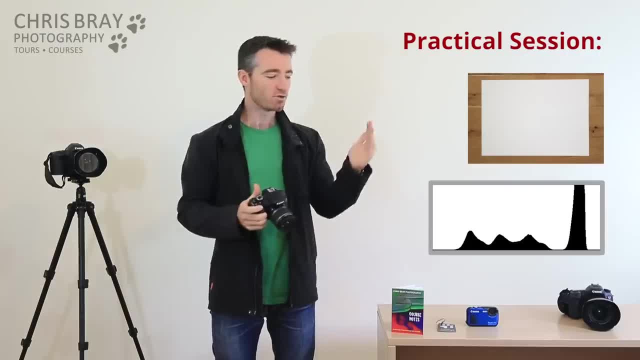 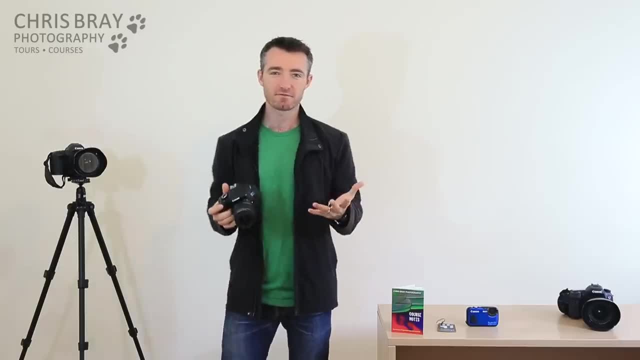 And you'd probably surprise yourself how far you actually need to scroll to bring that spike near the white end, which is where it's supposed to be if what you're photographing is white. So give that a try When you come back from that prac. it's time to move on to the next lecture, which is all. 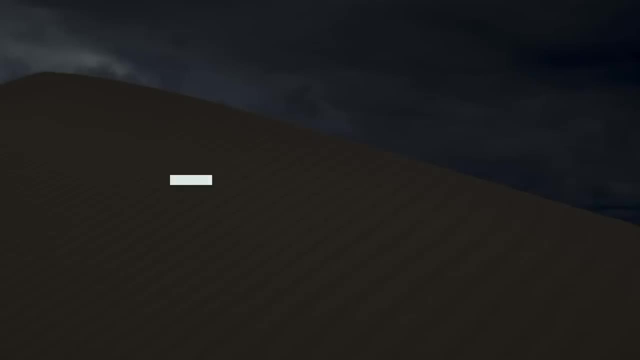 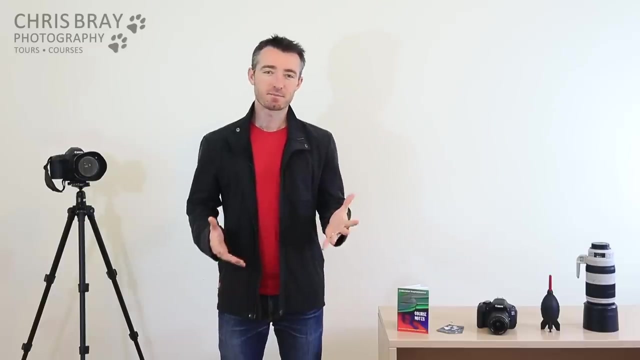 about aperture And how that affects your depth of field. So aperture and depth of field: Now, a lot of people think this is about the most confusing part in photography, But that's only because people insist on teaching it in a really stupid way. 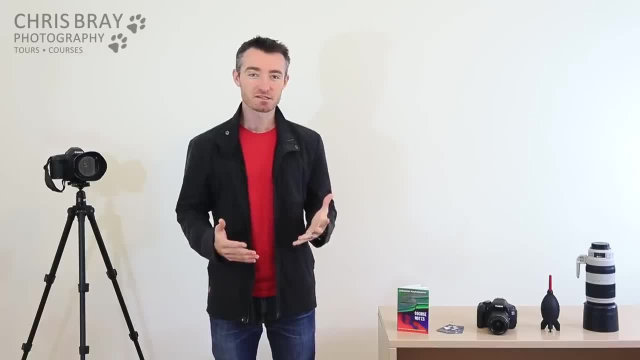 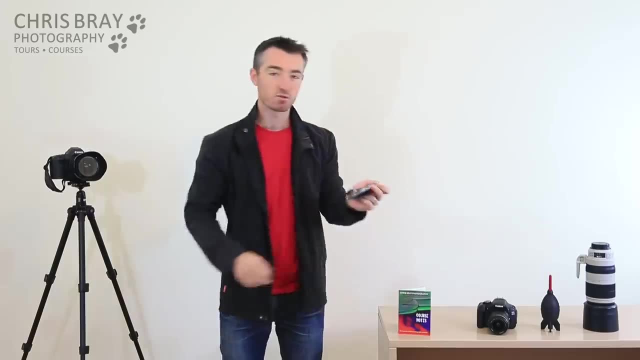 There's a very easy way to understand aperture and it'll make perfect sense, I promise, And just a reminder, that this is all covered in the aperture section of our course notes booklet as well, that you can buy online, And also the plastic summary clip cards. 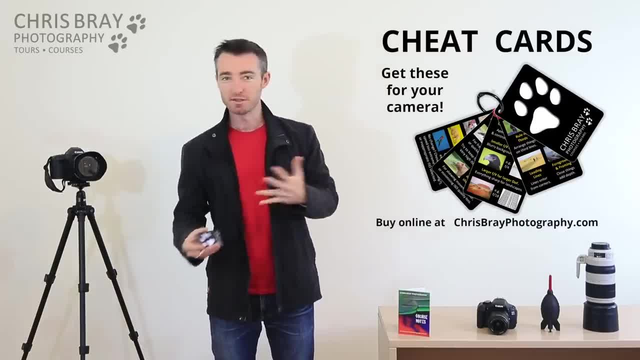 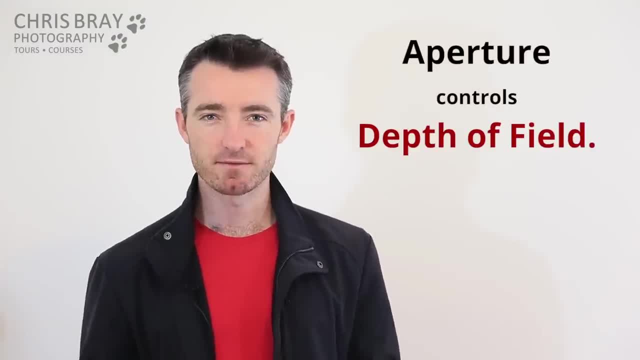 There's the aperture section there, Which tells you which way to move your f number, to do what with your depth of field and all that kind of stuff as well. Pretty handy. So, as we already saw in the basic lecture, aperture controls what's called your depth. 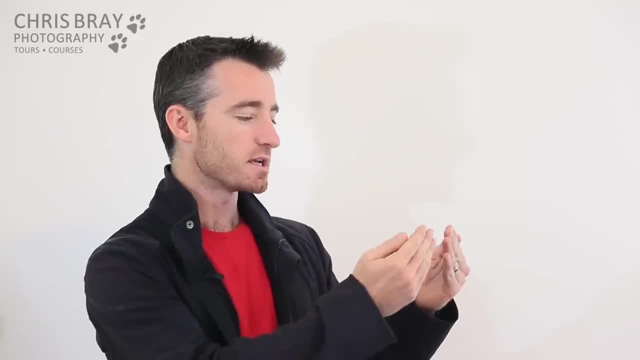 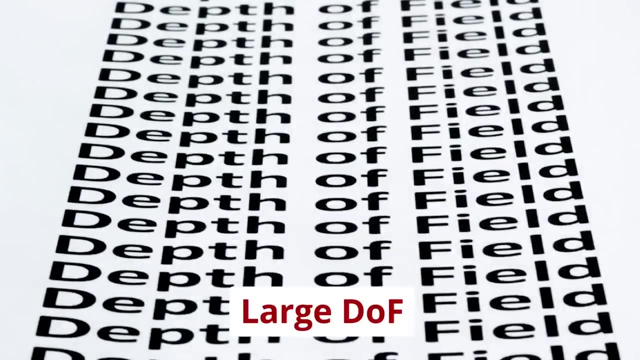 of field, And depth of field is just the amount of stuff that's in focus, in front of and behind the point that you actually focus the camera on. So this is a very small or shallow depth of field, And this one is a large depth of field where much closer is still in focus and way into 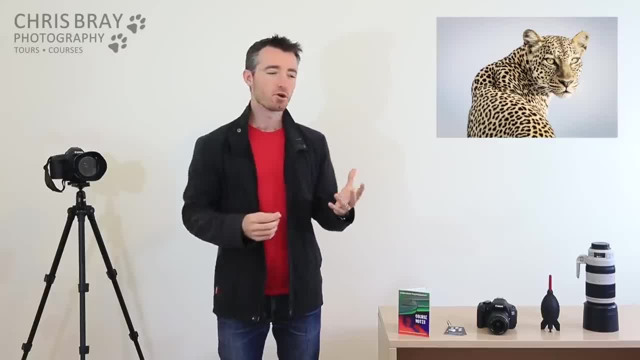 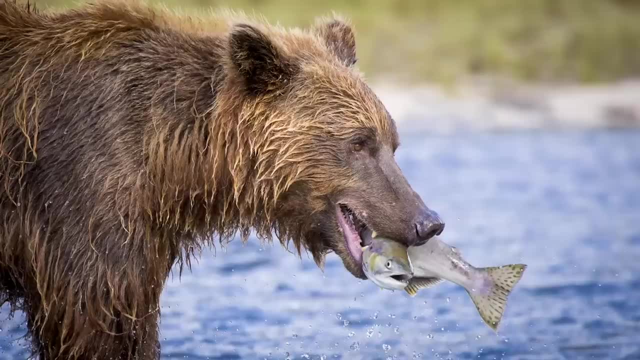 the distance is still sharp as well. So typically for a portrait type photo, where there's only one thing you're supposed to be looking at, You want the softest, blurriest background you can to make your subject stand out against it. look more 3D. 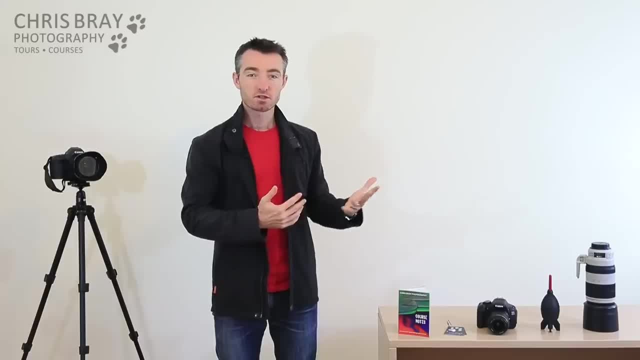 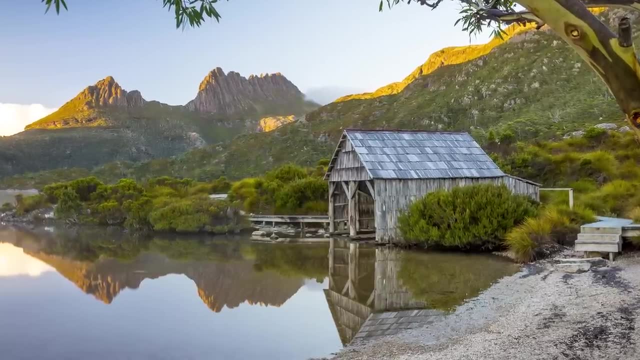 So you want a small depth of field for that blurry background But, contrast to that in a landscape, you actually want a big depth of field Because the close up plants and flowers and the distant mountains and clouds- everything is interesting and you want the viewer's eye to be able to travel everywhere in the scene. 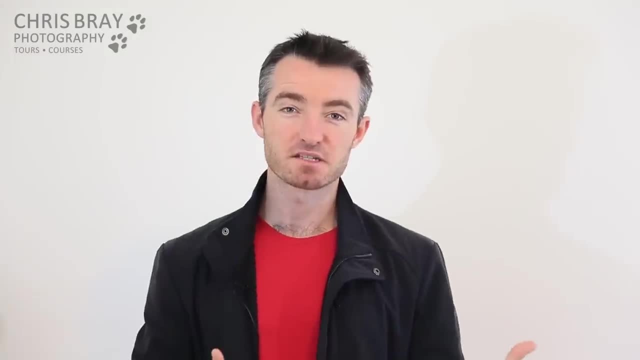 So for a landscape, you want a big depth of field And, as we already saw in our basic photography lecture, using a bigger or small depth of field to affect the background has a pretty significant effect. So you want a big depth of field. And, as we already saw in our basic photography lecture, you know using a bigger or small depth of field to affect the background has a pretty significant effect. So you want a big depth of field And, as we already saw in our basic photography lecture, you know using a bigger or small. 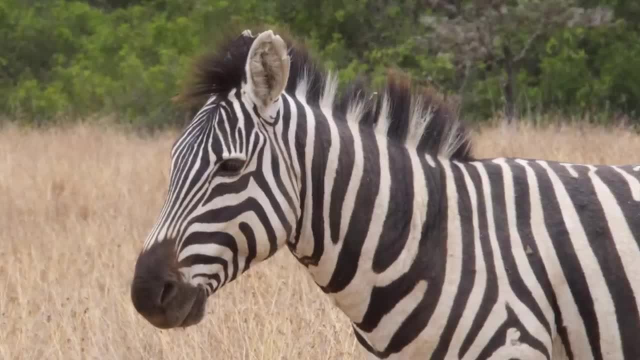 depth of field to affect the background has a pretty significant effect. So here's a shot of a zebra using a fairly large depth of field. So the zebra is kind of sharp, the background is kind of sharp. It all feels quite flat and stuck together. 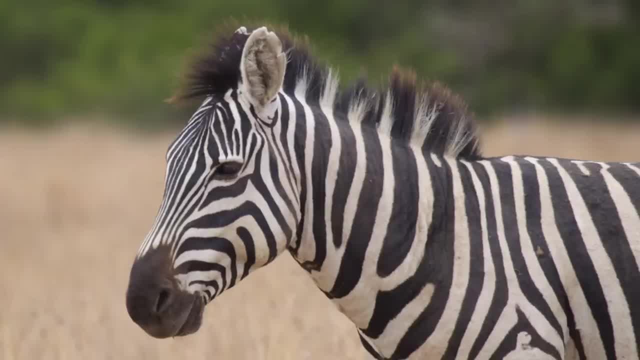 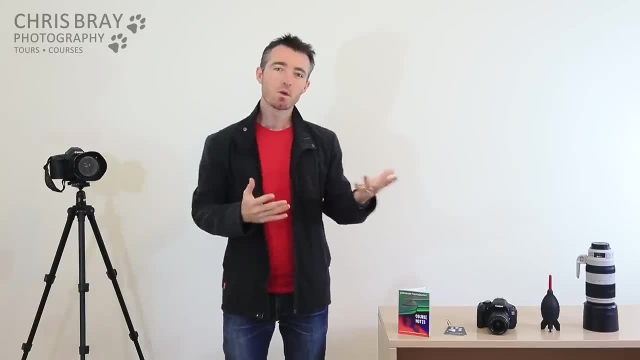 As opposed to using a smaller depth of field where you can see now beautiful blurry background. The zebra just leaps out. against that, You can see individual hair detail on the mane. So what actually is aperture? Well, inside your lens it's this variable sized hole. 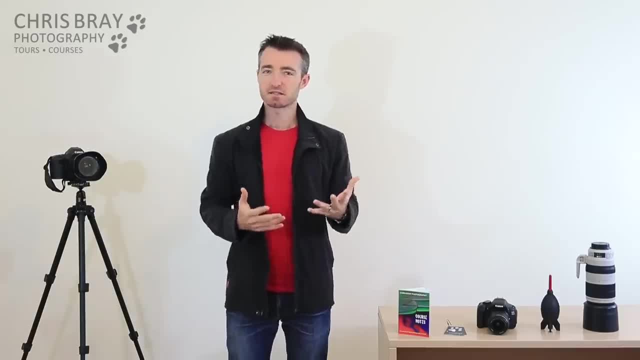 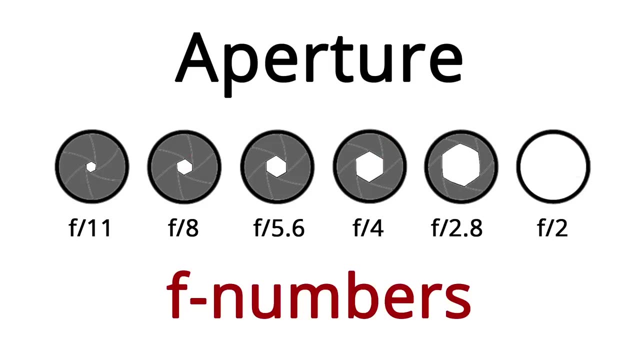 And you can just set that to be whatever size you want. And it's defined in these things called F numbers or F stops. So you can see here that's F8,, F4, F2, and then you go: oh, hang on a minute. 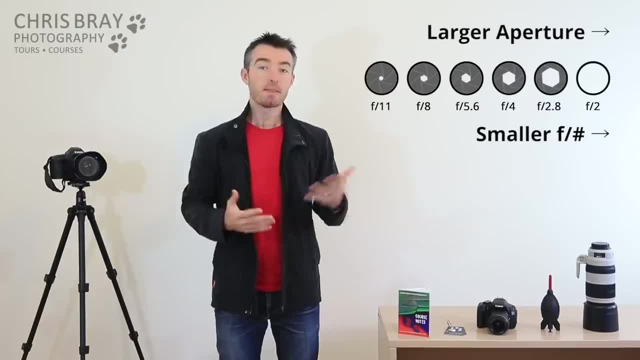 The F number's getting smaller but the hole's getting bigger. And that's about where most people get to trying to understand aperture. They suddenly realize there's this whole mental gymnastics you've got to go through to work out what on earth you're trying to do with your F number, to do what with your hole. 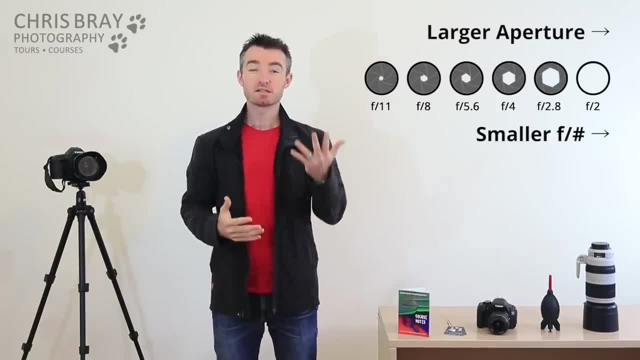 and what does that do to the depth of field anyway? and it's all just way too confusing. But that's only confusing because for some strange reason everyone insists on talking about the size of the aperture hole instead of the F number. You know, you live in a world of F numbers. 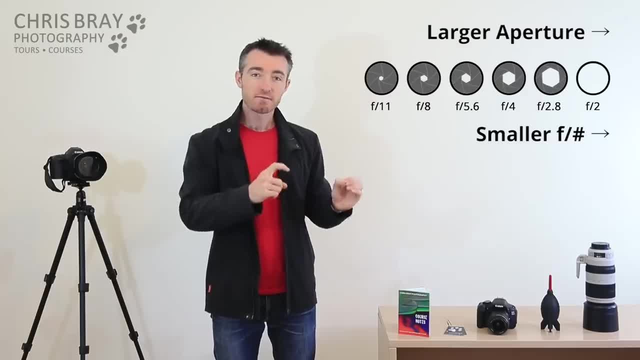 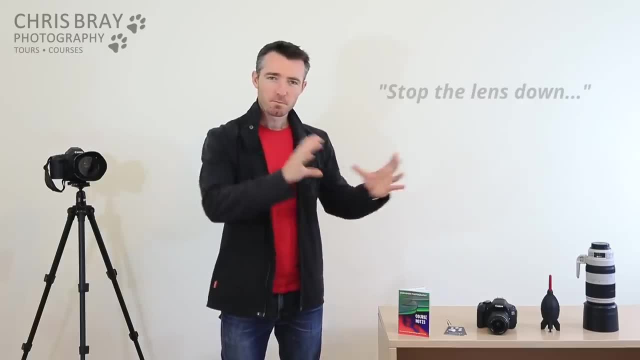 If you're setting your camera up to take a shot, you're scrolling the F number. You're watching the F number get bigger or smaller. You're not watching the size of the hole inside the lens. You hear phrases like open the lens up more or stop the lens down. 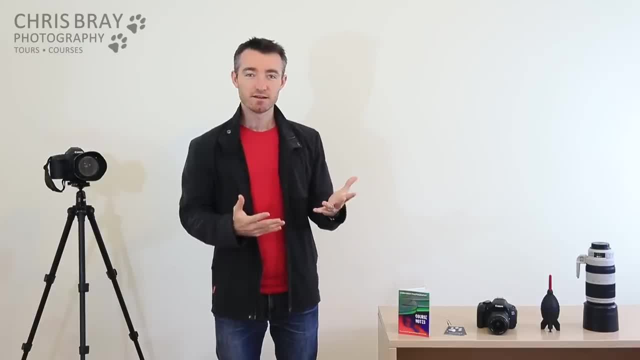 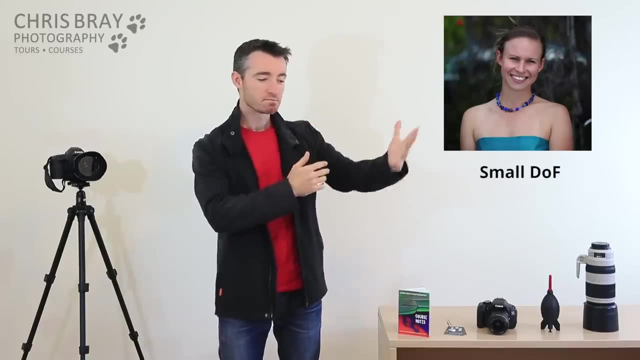 Use a bigger aperture. This is what, apparently, is supposed to go through your head. if you're trying to take a photo of a person or a portrait shot, Obviously you want a small depth of field for a small amount of stuff in focus. a nice 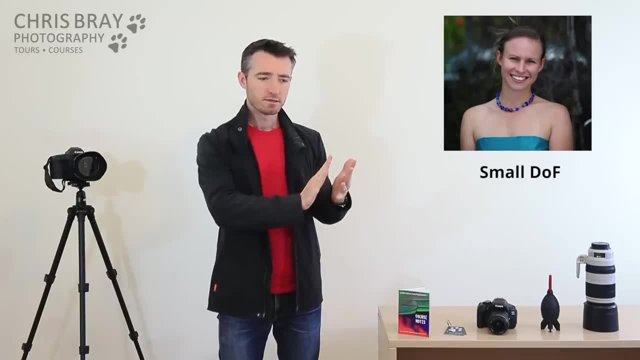 blurry background. So you go: okay, we need a small depth of field. Well, it turns out You get a small depth of field with a large aperture hole. So you go, right, So I've got to flip it All right. 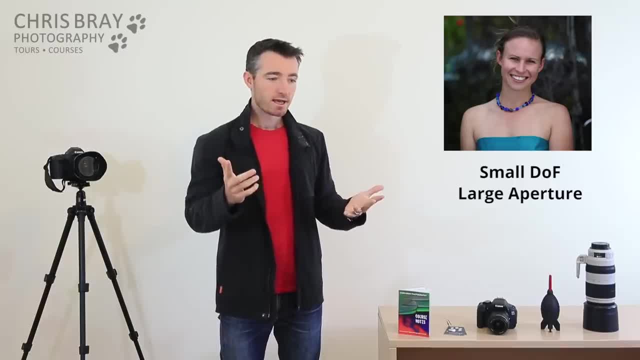 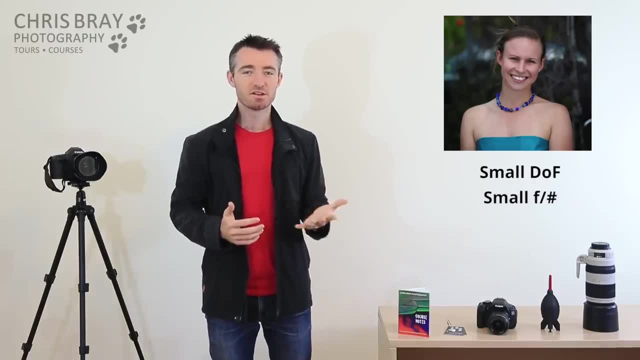 Large aperture hole. How do you take a picture with a large aperture hole? Well, you've got to remember: actually a large aperture hole is a small F number. So you flip it again. Well, clearly that's just stupid. So if we just stick with F numbers, it turns out aperture is incredibly easy. 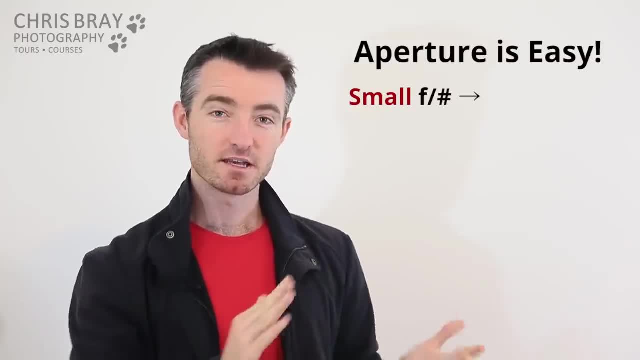 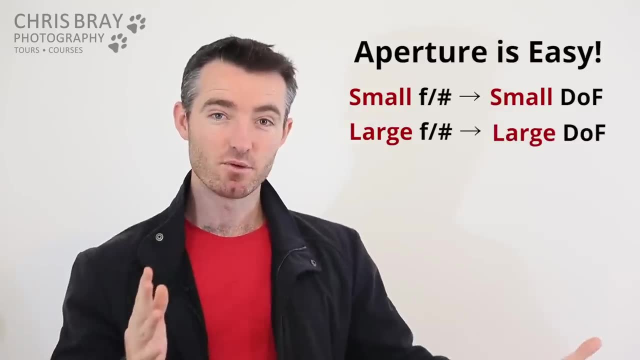 Let's have a look. If you use a smaller F number, guess what? You get a smaller depth of field. If you use a larger F number, you get a larger depth of field. It's pretty straightforward. Now. the actual range of F numbers you can scroll to depends on what lens you have. but 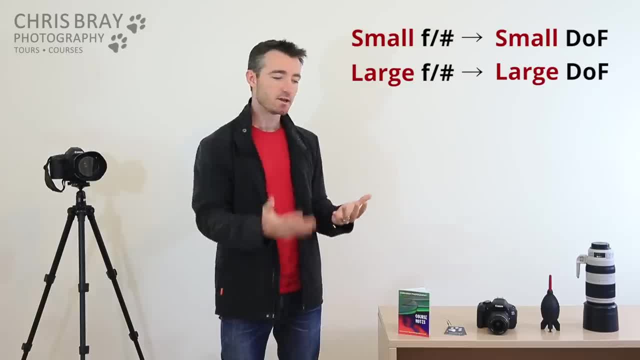 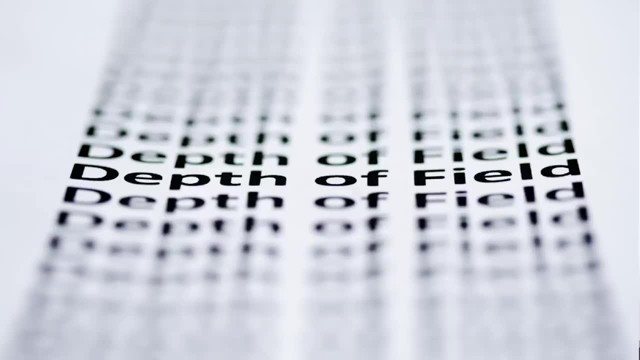 some of them will go up to numbers about F40-ish and down to about F1 point something. So let's pretend F numbers go from about 1 to 40. So this photo was taken at F2.8. So as far as F numbers go, that's a small F number gives us a small depth of field. 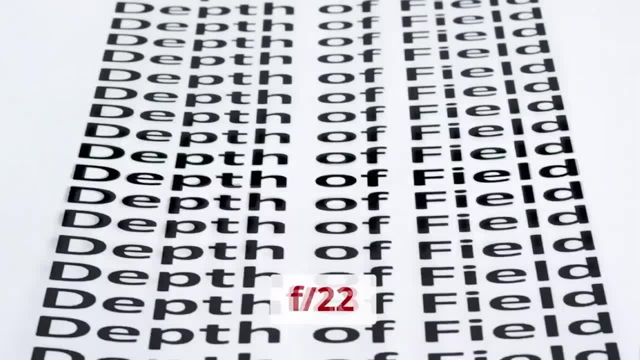 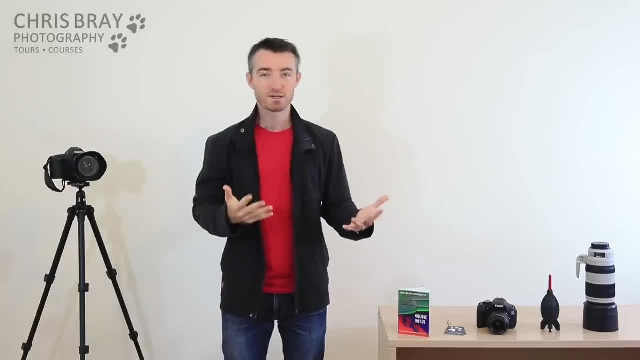 a small amount of stuff in focus. But if we used a bigger F number, like F22, that's a big F number, big depth of field, big amount of stuff in focus. Another example you can see here: this photo was taken at F2.8.. 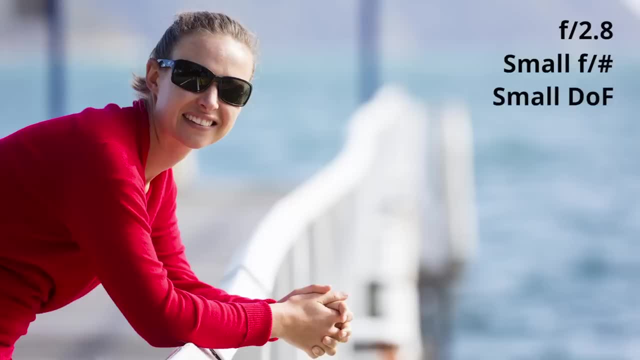 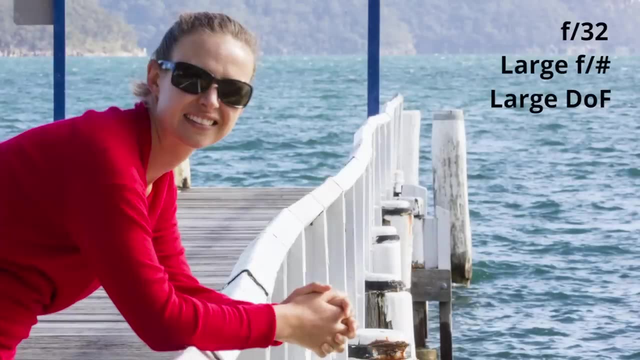 So that's a small F number, small depth of field. You can see the background is blurry and just Jess is sharp there in the front. If we used a large F number though, like F32, you can see the difference there. 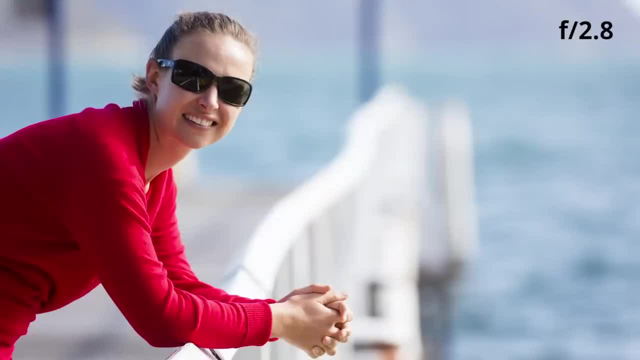 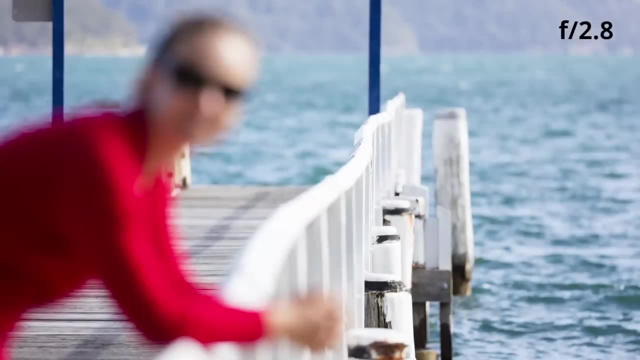 The background. everything is sharp now. But back on that small F number, small depth of field. of course. if I'd focused on that bollard halfway back or something, then that bollard would become in focus and the ones behind it would be blurry and the ones in front of it. 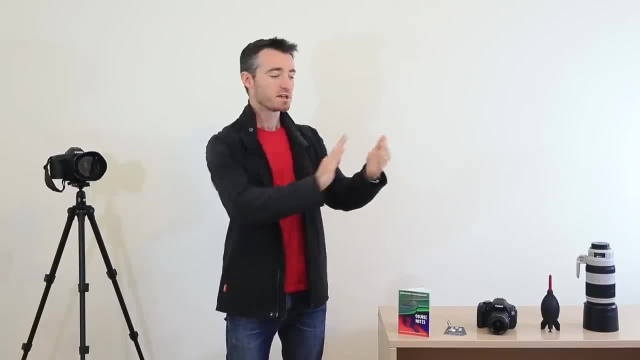 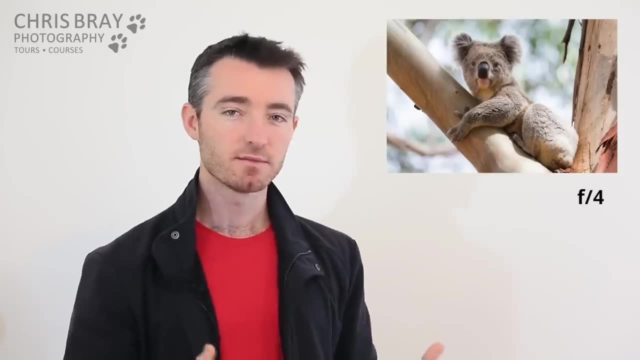 Jess, would be blurry. Obviously, whatever you focus on is going to be in focus. The F numbers just scroll up or down that depth of field around that point. So if you're taking a photo of a thing you know- a person, an animal, a subject you want. 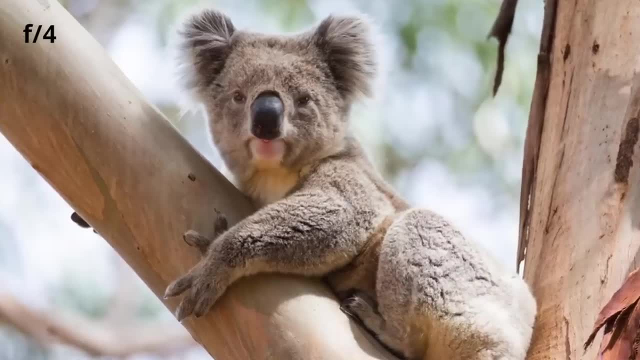 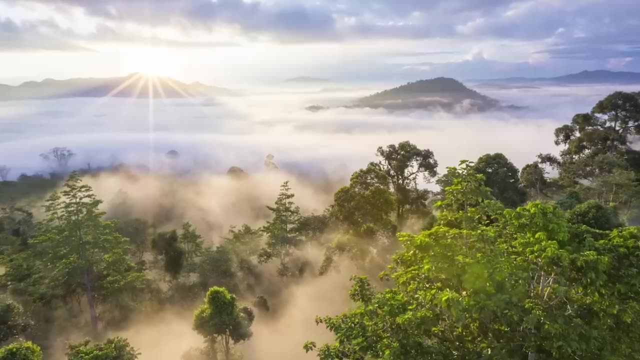 to use a small F number for a small depth of field- nice blurry background to help it stand out. But if you're taking a photo of a landscape shot where you want a big depth of field, you just use a big F number, like this one: F18.. 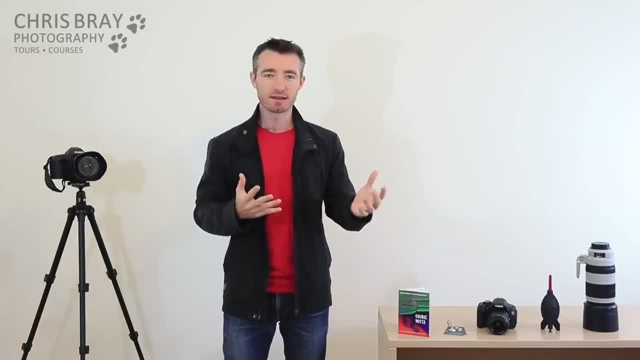 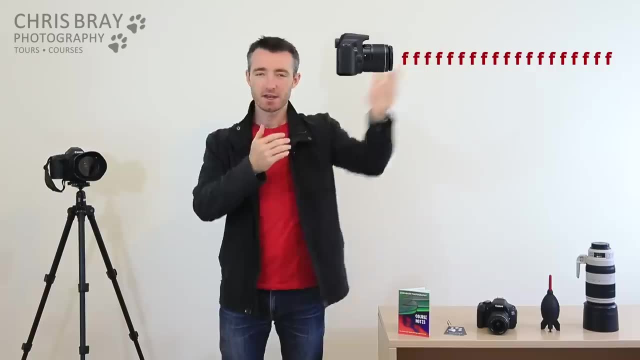 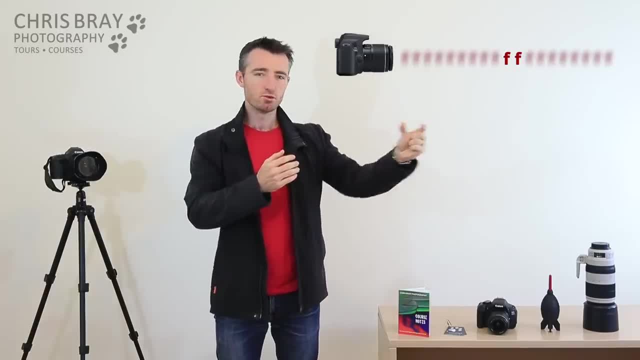 Now, if you only wanted two of those Fs to be in focus, doesn't matter which two- whichever two you focus on, I guess- but if you only wanted two Fs to be in focus, you'd pick F2.. If you wanted 10 Fs to be in focus, you'd pick F10.. 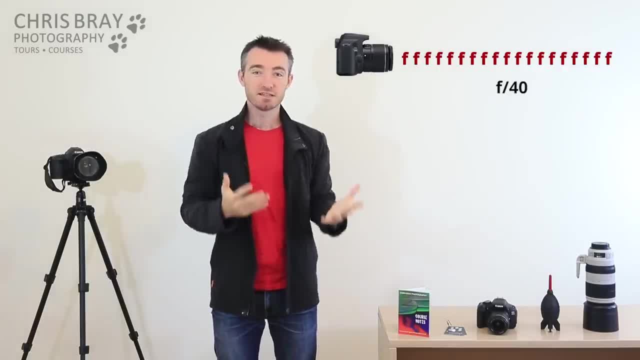 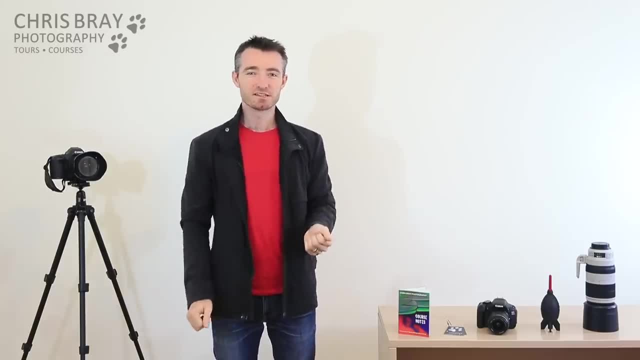 If you wanted all 40 Fs to be in focus, you'd just pick F40.. Basically, you can boil it down to the more things you want in focus, the more Fs you want. Aperture doesn't get any simpler than that, and it really is quite easy. 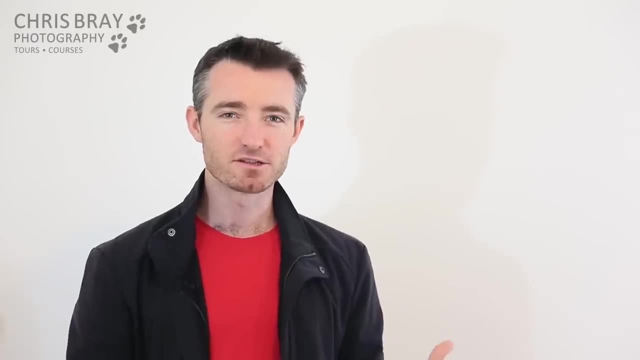 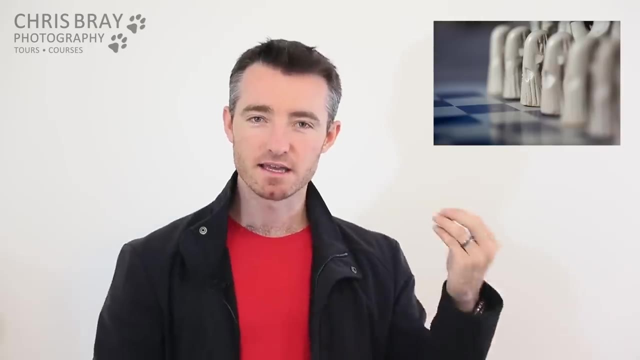 Aperture really is your most powerful creative tool for making your photos look much more professional. You know, using a small F number for a small depth of field is a really powerful way of directing the viewer's eye exactly where you want them to look. 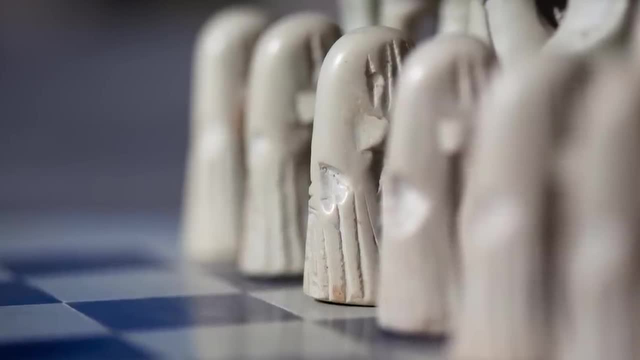 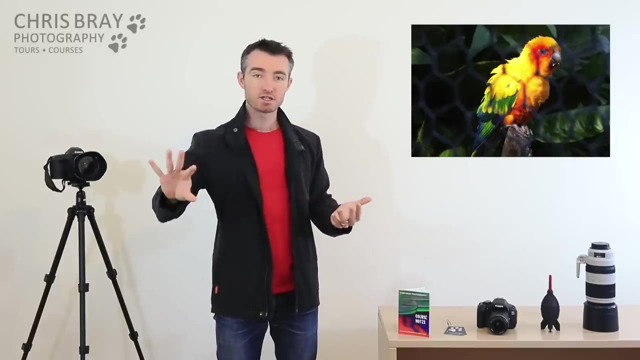 Like in this photo. you can't look anywhere else. really, your eye is just drawn straight to that one chess piece. Also, blurring stuff out that you don't want is incredibly useful In a zoo. you might have mesh- cage mesh in front of what you're photographing. 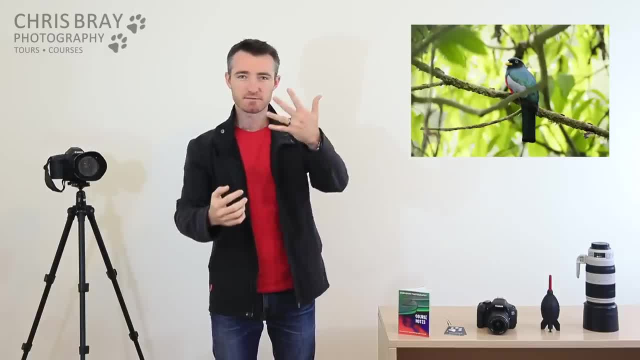 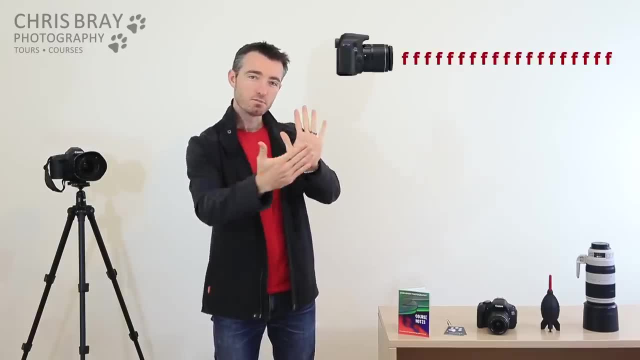 In the real world, you're going to have a bird deep in a tree somewhere and there's little sticks in front of it. There'll be bits of grass popping up in front of your lion. If you can actually focus carefully on your subject, though, and use a very small F number. 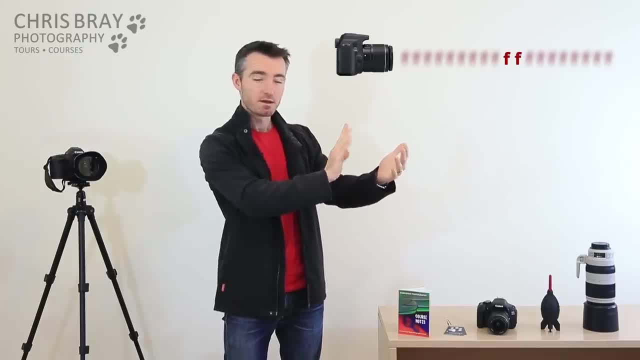 for a small depth of field. you can make your subject nice and sharp, but anything in front, like these little sticks, start to become blurry. And if you use a small enough F number and you can get close enough to that thing, you're. 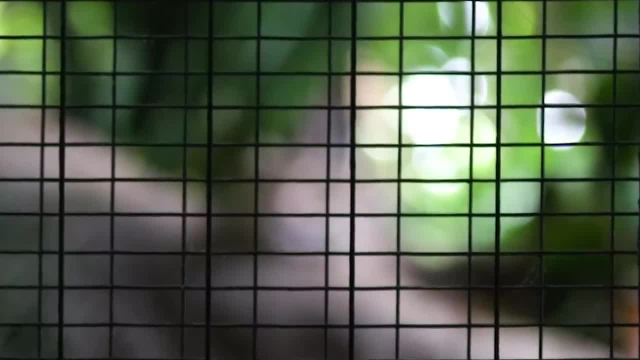 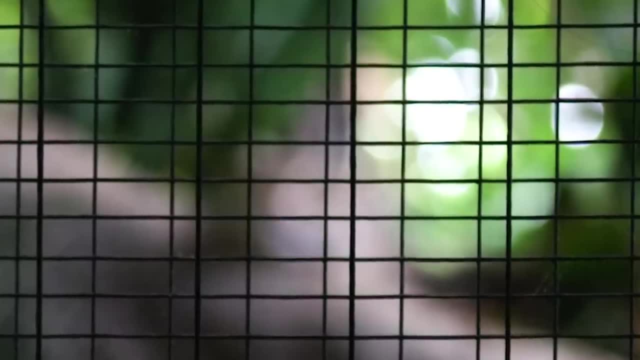 trying to blur out, you can actually make it disappear. Look at this example. This mesh here is a one centimetre mesh, so there's no way I could hope to poke my camera through there and get a nice clean shot. But if I carefully focus on the cat inside there, 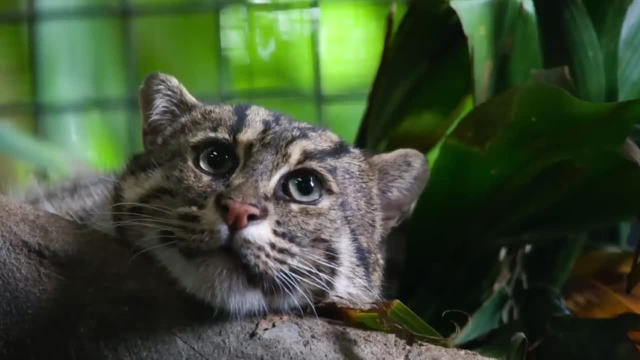 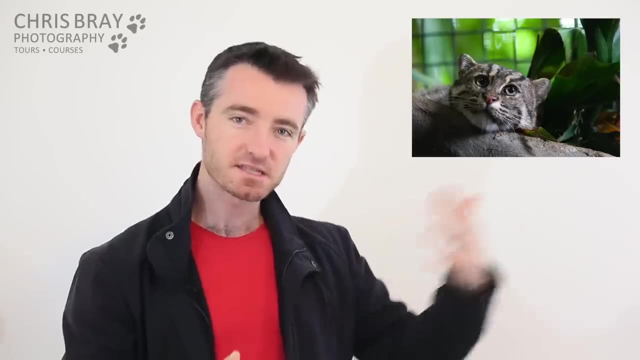 That's a cat in there And then use a small F number, then anything in front of the cat becomes blurry and the cage wire, as you can see, has completely disappeared. That mesh you can see in the background there, that's the other side of the cage, behind the 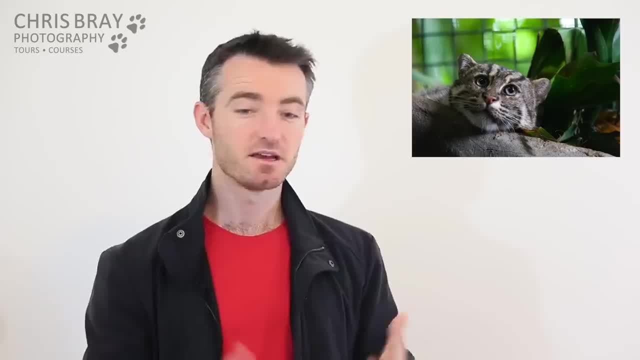 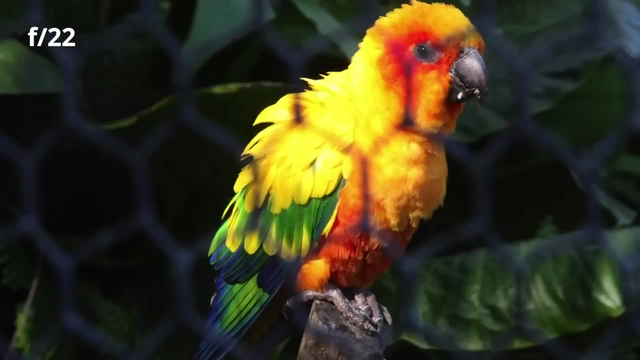 cat, But there's literally six or seven wires going across in front of its face, but you just can't see them because they've been blurred out Pretty amazing. Another example: bird on a stick, So F22, that's a fairly big F number, big depth of field. so the bird is sharp, the 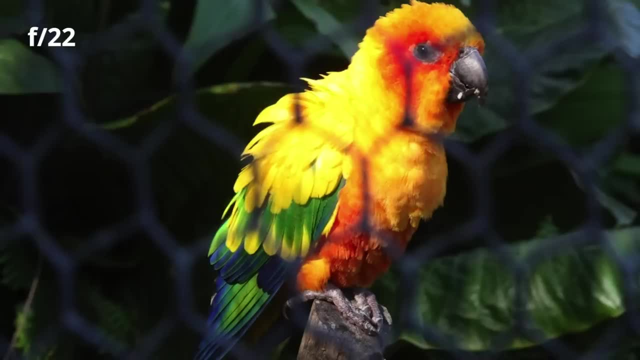 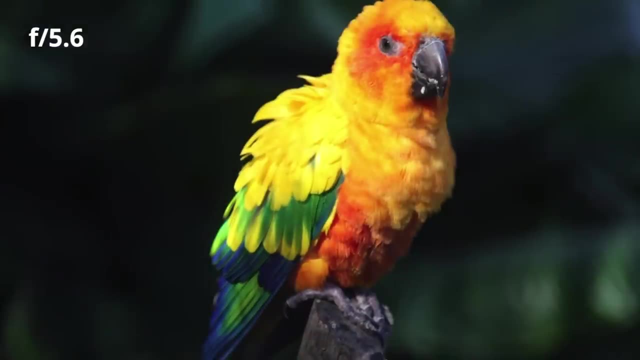 background leaves are quite distracting there and obviously the chicken wire in front is really annoying. But if instead we just scroll down to a smaller F number- F5.6, and take the same shot again, then look at the difference. there. The background is now a nice soft pastel-y kind of background and the chicken wire's 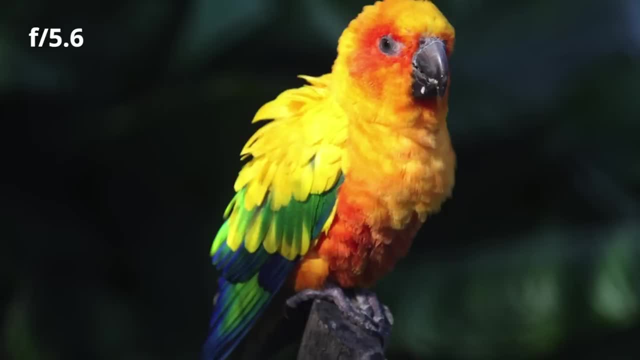 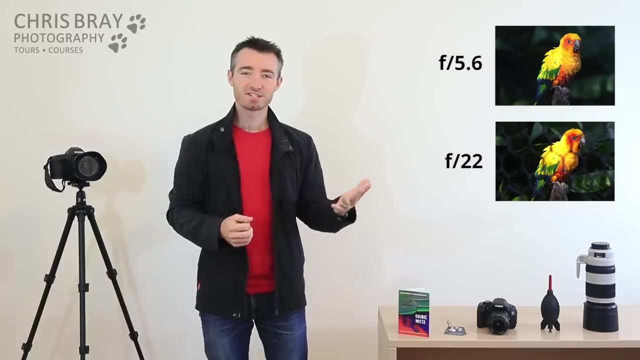 gone Fantastic And don't think that that is something you can only do with really expensive incredible lenses. I deliberately took that pair of photos with the cheapest, crappest lens money can buy. But even with really cheap dodgy lenses you can do amazing things with your depth. 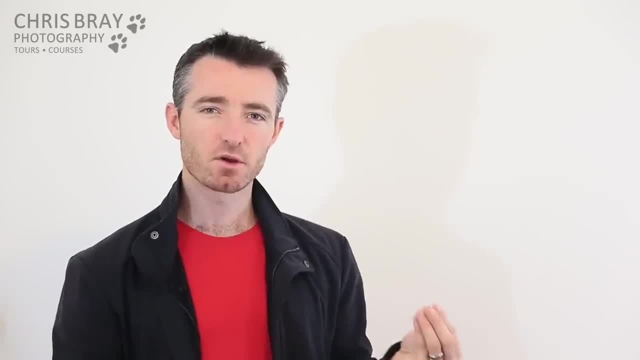 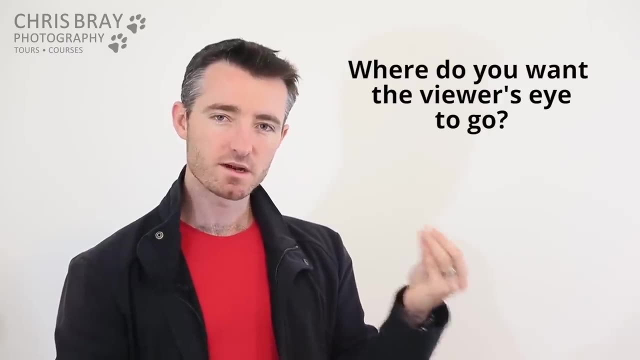 of field. So you're supposed to be thinking. now, before you take a photo, ask yourself the question: where do you want the viewer's eye? What are we supposed to be looking at? Is there only one thing of interest? One subject? 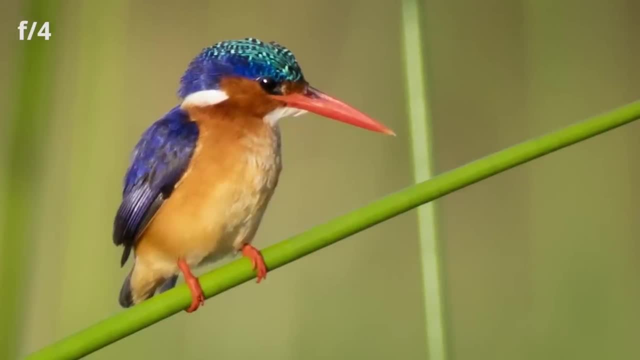 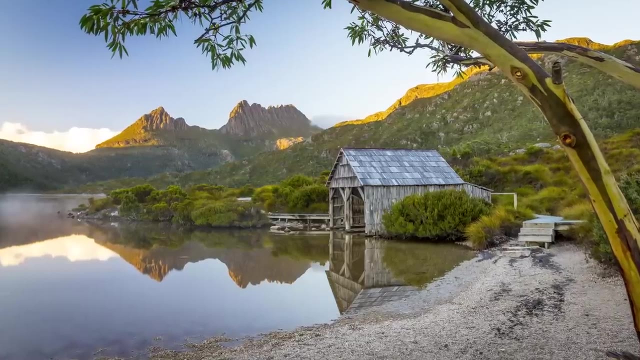 Then you probably want a small F number for a small depth of field, nice blurry background to make it stand out. But if there are multiple things at different distances, like a landscape, then you want a big F number for a big depth of field and make them all come out nice and sharp. 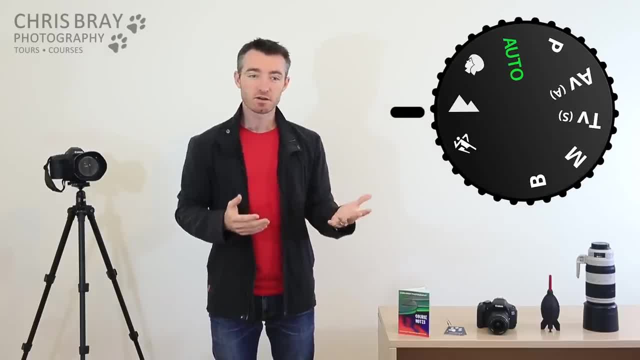 Incidentally, if your camera has a landscape mode, basically that's just telling the camera to pick a larger F number for you so you get a larger depth of field, Or a portrait mode, That's just telling the camera to use a small F number so you can get a larger depth of. 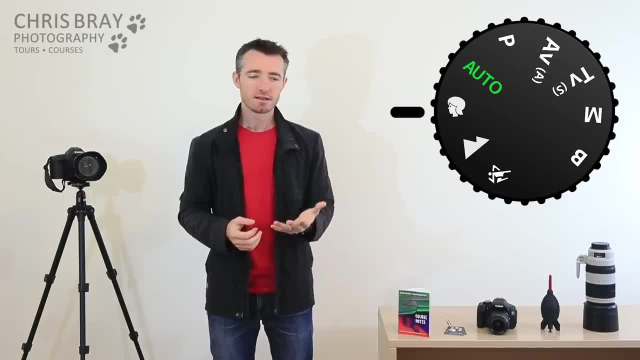 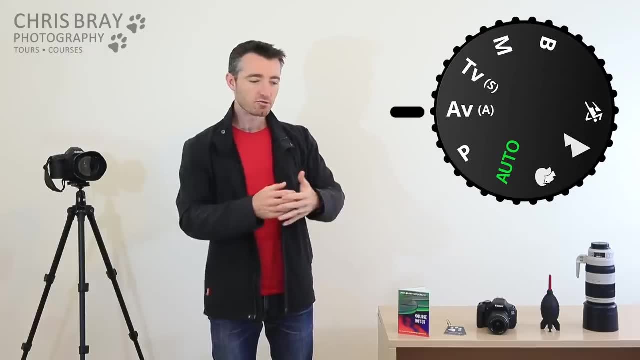 field give us a bit of a smaller depth of field. nice blurry backgrounds. Now. that's definitely better than auto mode, for sure, but it's nothing like as powerful as going over to aperture mode- like we're going to have a look at in a second- to really 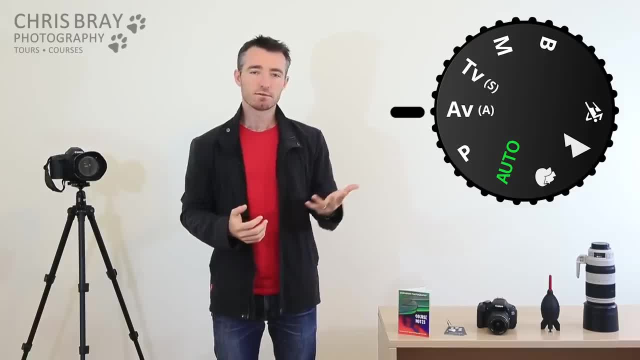 drag that F number exactly where we want, Because often you know landscape mode doesn't pick a very big F number. it might pick about F7 or 8, whereas you could probably drag your F number all the way to F20 if you wanted. 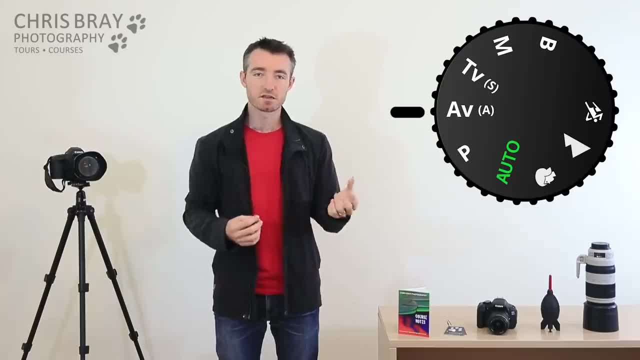 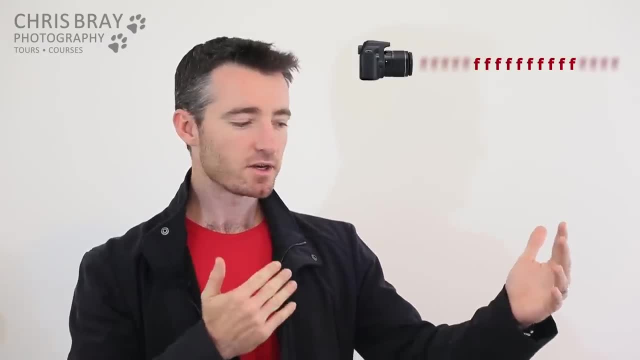 to. So you can just get much more control and more exaggerated effects by going to aperture mode and telling the camera exactly what you want. It's worth realising that the region of stuff that's nice and sharp is not actually centred around the point that you focused on. 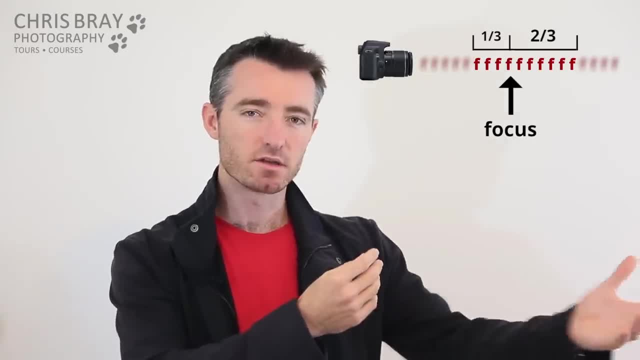 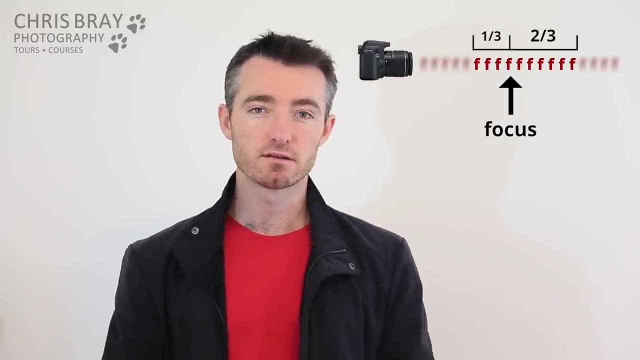 Turns out that about two thirds of the in focus stuff is behind where you focused. only one third of it comes forward And you might think who really cares about that? seems a bit pedantic, but it's actually really important, particularly for a landscape shot where you're trying to maximise your. 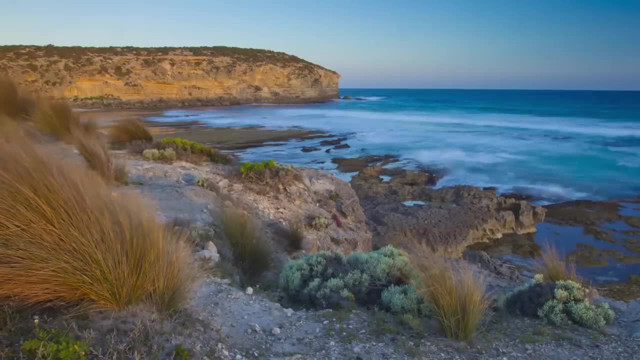 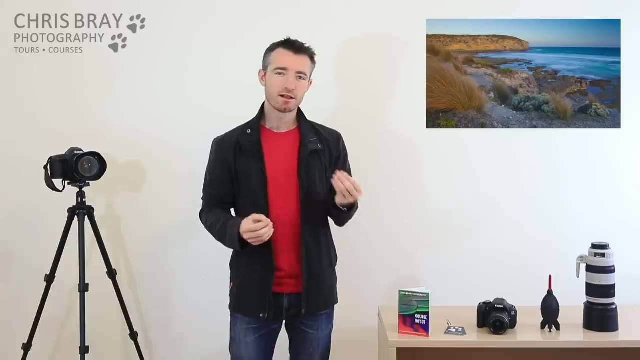 available depth of field. So a situation like this one: we want a huge depth of field, so we're going to use a big F number like F22 or something great, But then where do you focus? A lot of people make the mistake on their landscape photos of focusing on the distant. 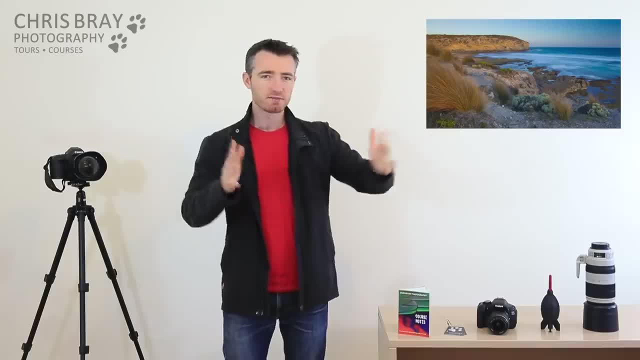 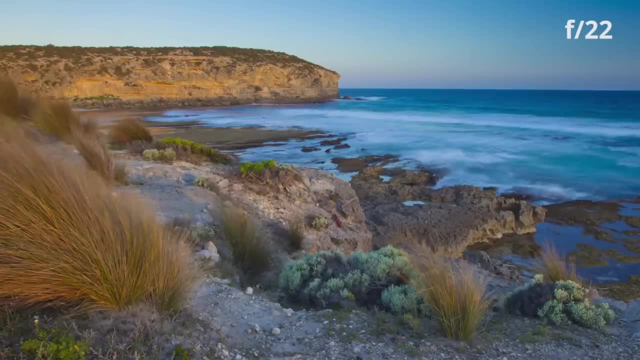 mountains, And the problem then is: sure, you've got a big F number gives us a big depth of field, but if you focus on those mountains, two thirds of that depth of field is now wasted behind the mountains. only one third of it comes forward and your foreground rocks and pebbles. 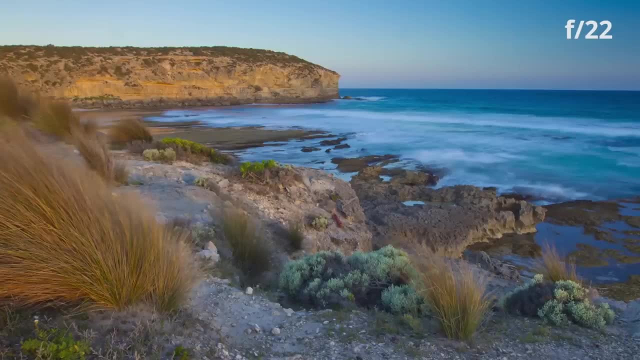 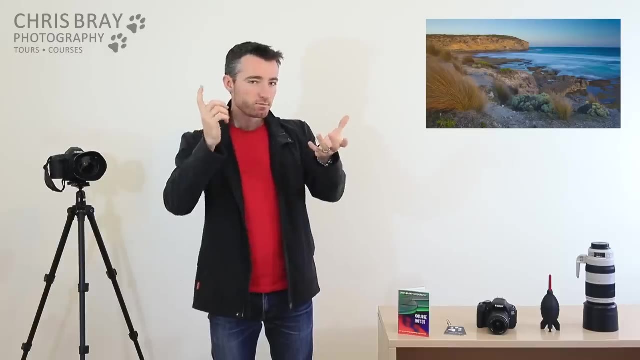 and stuff are still going to be out of focus. So the actual answer is: when you're photographing a landscape scene, you just try and arbitrarily focus about a third of the way into your shot. So you just briefly point the camera down about a third of the way in. 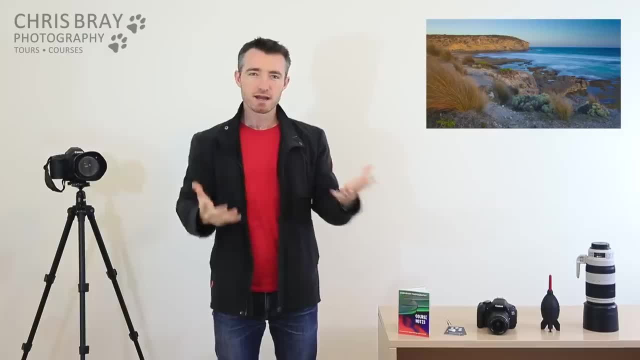 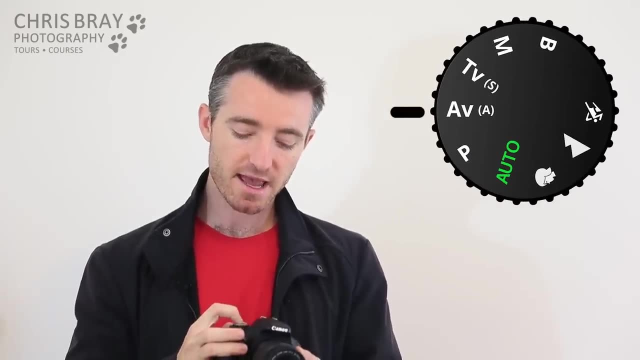 Beep Focus, Lift it back up And take the shot, And that's just maximising the use of your available depth of field. Okay, so let's take a look at aperture mode. So aperture mode on a Canon is AV and for every other brand it's just called A. So in 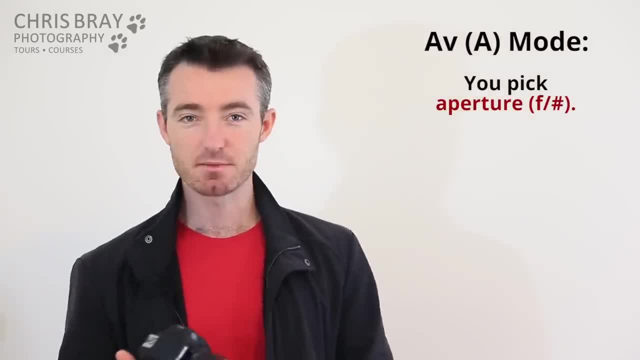 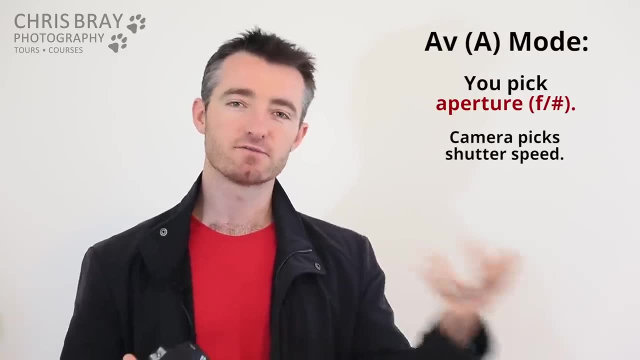 aperture mode. you can pick whatever aperture value you want, as long as the lens is capable of it, and the camera will pick the right shutter speed to match up for it, so that you get correct exposure or whatever exposure you've asked for. if you've asked for a darker, 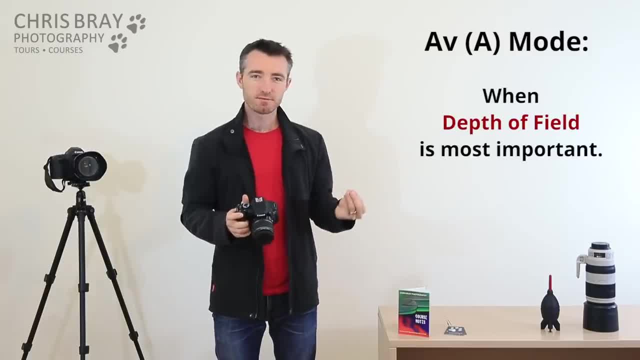 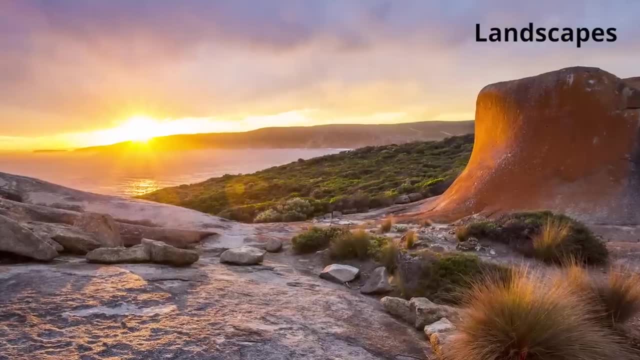 or brighter photo, So you'll be using aperture mode whenever depth of field is your most important. So if you're taking a portrait shot or a landscape shot- which to me is most of the photography you ever take- so I actually stay on aperture mode almost all the time. 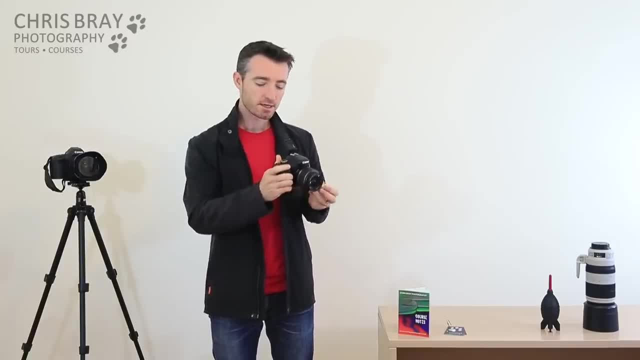 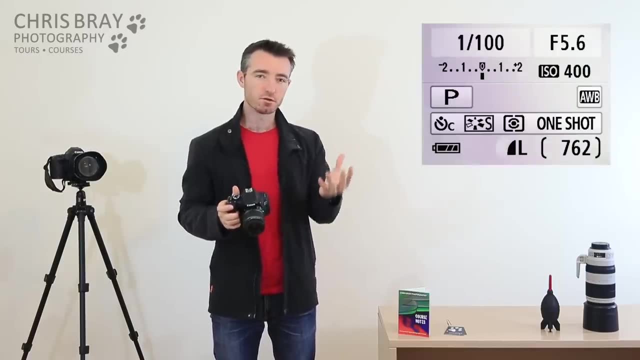 And this is typically how aperture mode works. You wake your camera up by pressing the button and it comes up with the last f-number that you used. Now that's quite different to p-mode. remember how p-mode always gives you that default auto-mode. 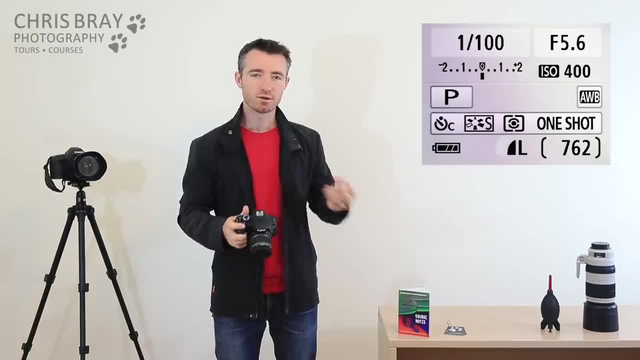 middle kind of value. You could always scroll to the same f-number if you wanted to, but it rapidly gets pretty repetitive in p-mode. If you're taking a bunch of landscape photos, for example, in p-mode, you go beep and it. 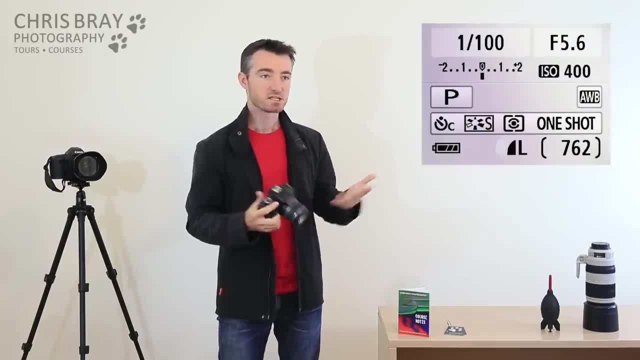 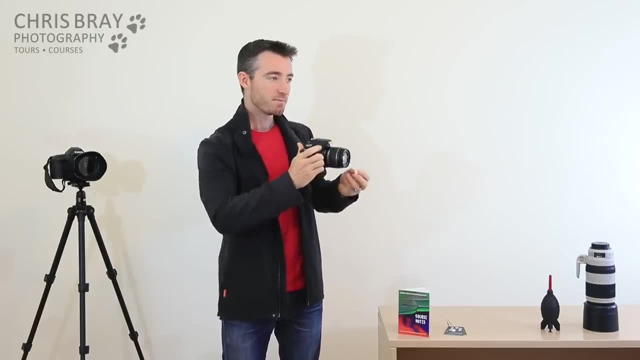 comes up and says how about 5.6, and you go: how about f-16, for a big depth of field? Scroll, scroll, scroll, f-16, take a shot. Then you try and take your second photo and you half press beep and it goes, how about. 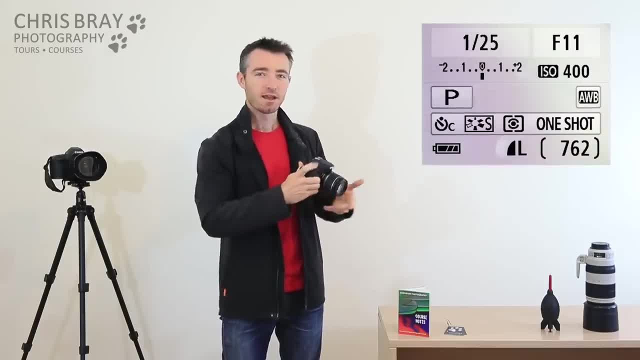 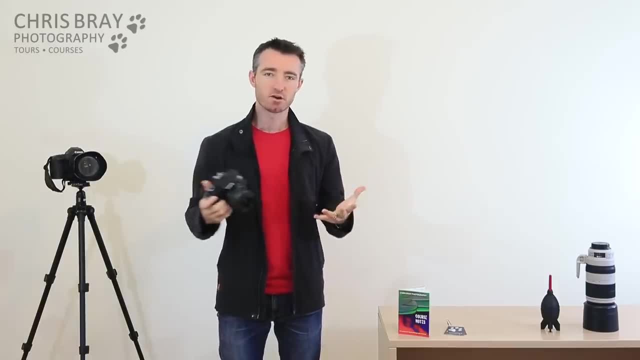 5.6? And you're like, ugh, how about f-16 again? And you have to keep moving it, or if the lighting changes or you point somewhere else In p-mode, you're not really nailing anything down. everything keeps kind of shifting around. 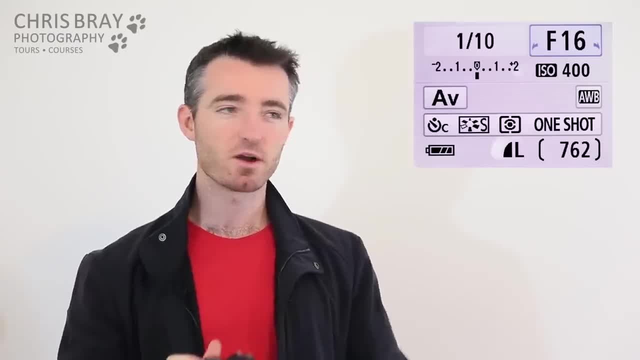 But in aperture mode, if you put in f-16, it'll stay on f-16. No matter what the lighting does or where you point the camera, the shutter speed will just keep being updated for you. so you end up with whatever exposure you asked for. 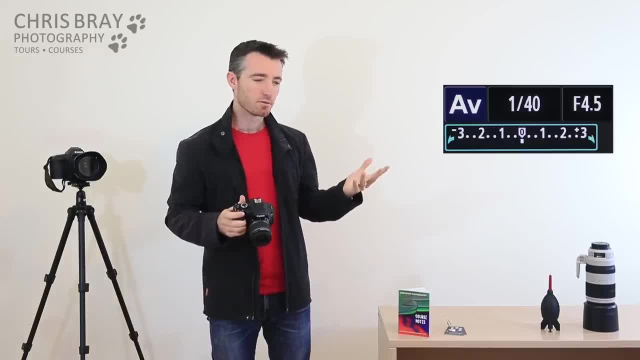 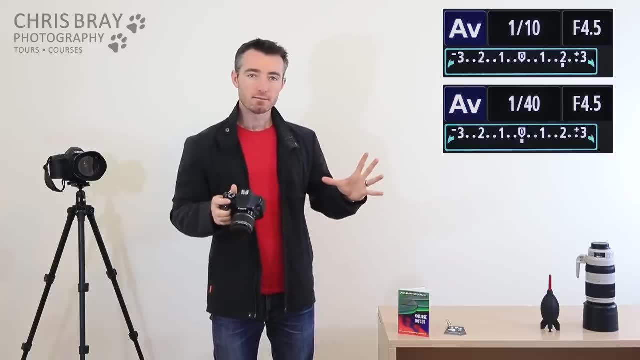 Let's say you make the photo brighter, so you use your plus minus exposure compensation and you say plus 2, so now it's got to be a lot brighter In aperture mode. it's not allowed to open the hole up anymore, because you're still. 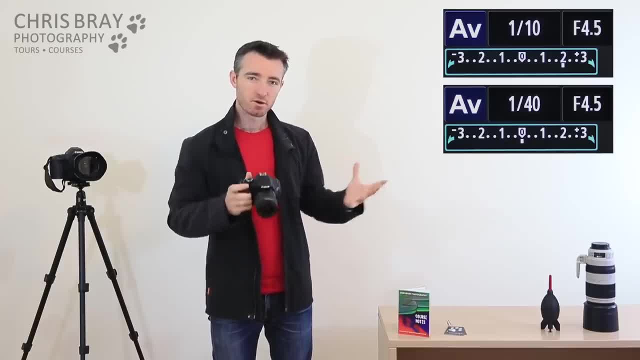 saying the same f-number, but somehow it's got to let more light in so your photo is brighter. So you'll just find that it leaves the shutter open for longer so more light comes in. Or if you asked for a darker photo, you could say: how about f-16?? 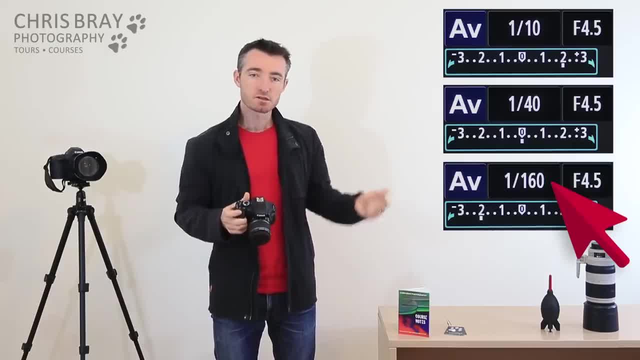 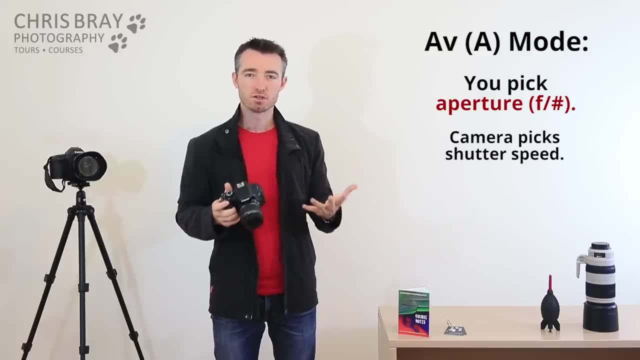 You'd find it would just be using a faster shutter speed for you so that not so much light got in. Basically aperture mode. you pick your f-number, it works out the shutter speed so that you end up with whatever exposure brightness you asked for. 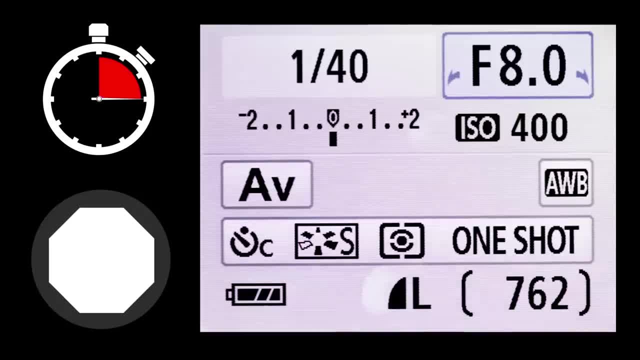 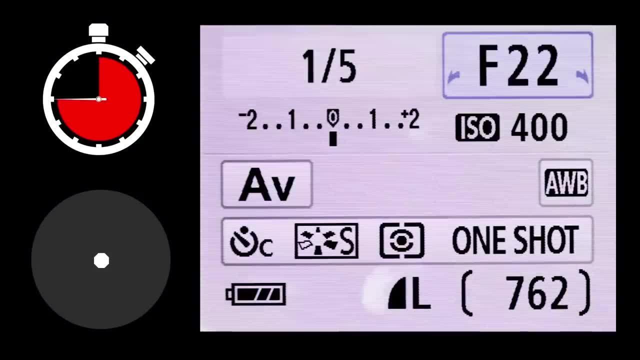 So, looking here, obviously, as we scroll our f-number up bigger and bigger, getting a bigger depth of field- good for landscapes and so on- you're noticing the aperture hole is getting smaller and therefore the shutter has to stay open longer and longer. so we 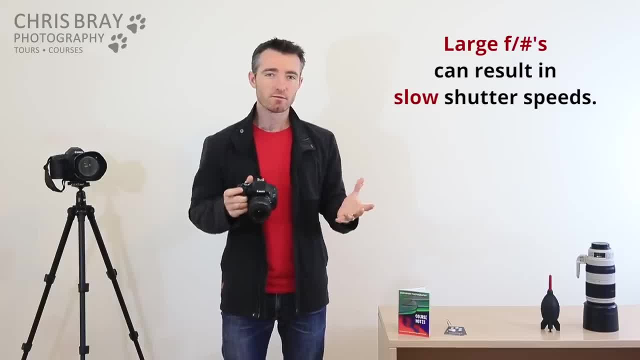 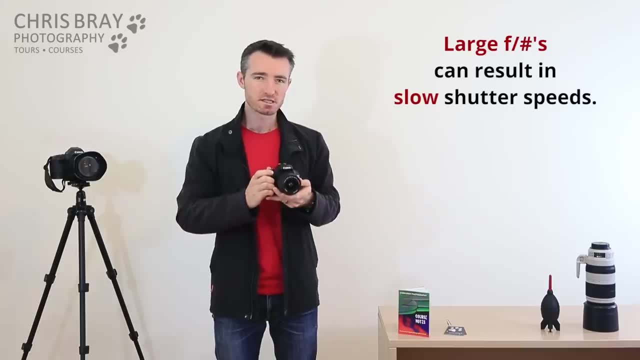 still end up with that same correct exposure. That's something to be aware of. Really large f-numbers, Really small holes. They often end up requiring quite a long, slow photo. so you've got to hold the camera really steady or put it on a tripod or something. 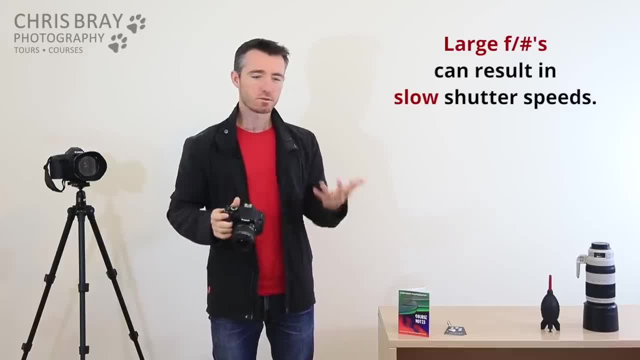 That's why landscape photographers and things always bother to bring a tripod where someone else can just walk past with a happy snap and go click. didn't need a tripod, But no, they're using such a big f-number for such an amazing depth of field that the 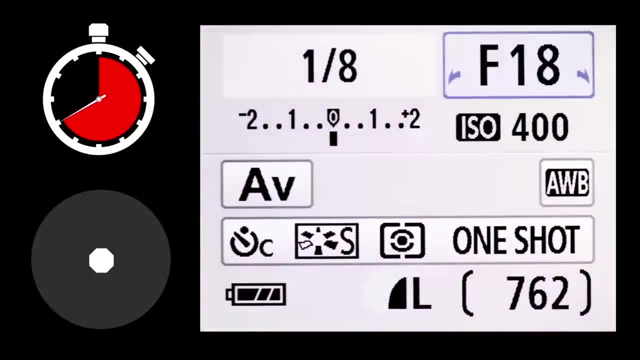 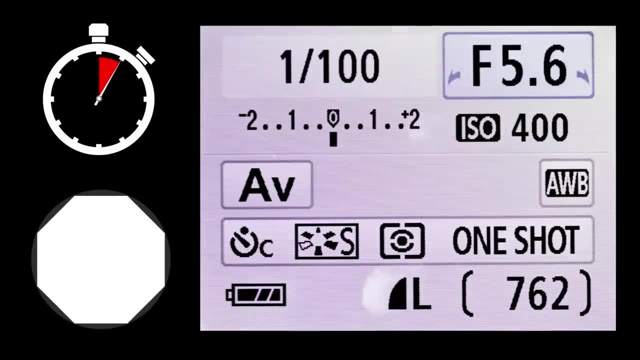 photo is going to be quite slow. Going the other way then, scrolling smaller and smaller f-numbers, getting smaller depth of field- good for portraits, nice blurry backgrounds and conveniently also nice fast photos at the same time. Just a point to note: don't expect to see the depth of field change when you're looking. 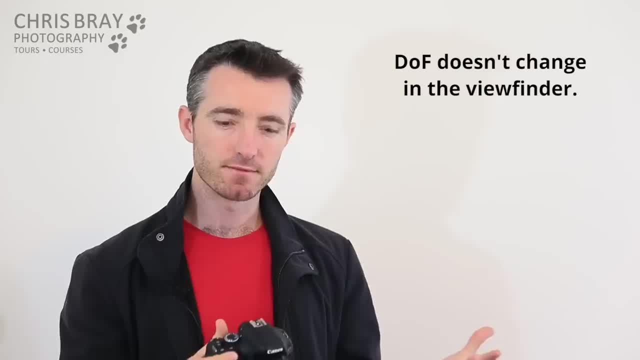 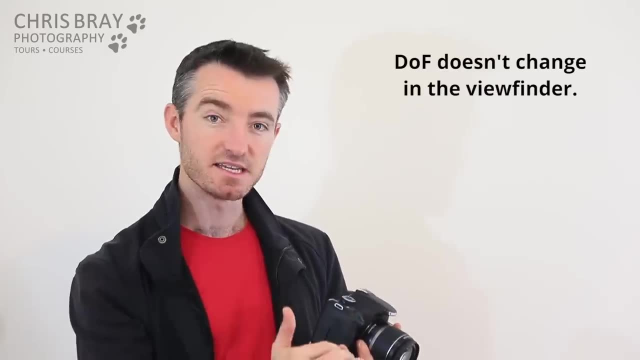 through your viewfinder. It's not actually until you get the photo back that you'll see the depth of field, Because when you're looking through the viewfinder in a DSLR, in fact, the lens stays open to the largest hole it can so you can see. 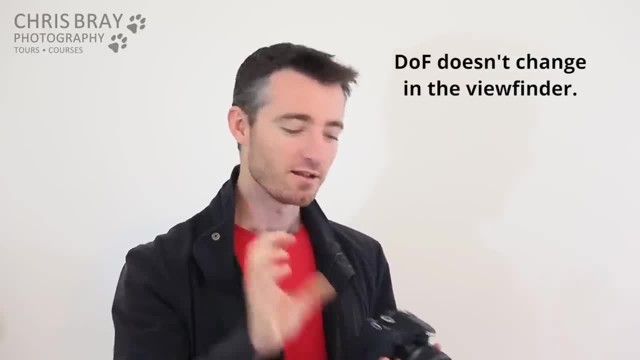 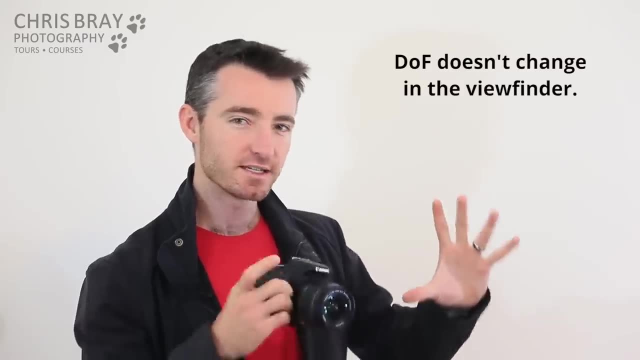 It wouldn't be much good if you'd asked for f-22,, which is a really small hole, and the lens just shut down. you wouldn't be able to see through your camera anymore. So in fact, it stays open, no matter what f-number you ask for, until you actually take. 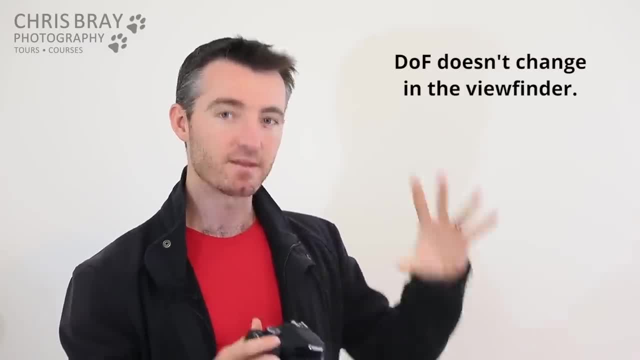 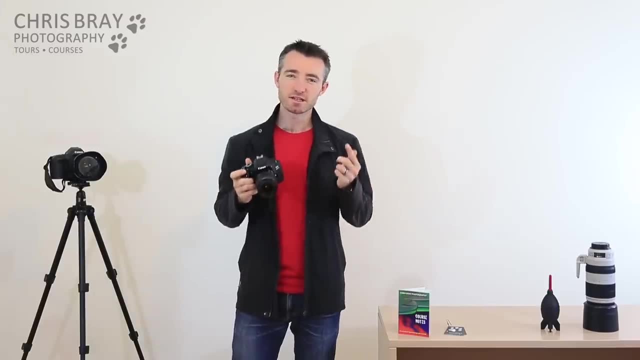 the shot and then it briefly jumps down to a different size. That's it. It takes the photo, then it opens back up again, so you can see. It just means you can't see the depth of field changing in real time. The other thing to remember is you're not entirely safe anymore in aperture mode. 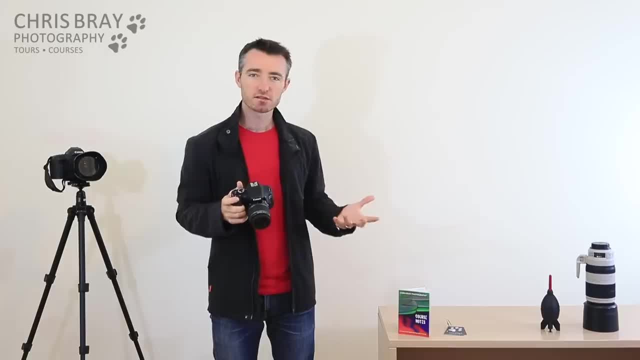 It won't stop you selecting an f-number even if there actually is no shutter speed to match up to it. for that current lighting condition Maybe it needs more than 30 seconds, or maybe it needs faster than the 4,000th of a second. 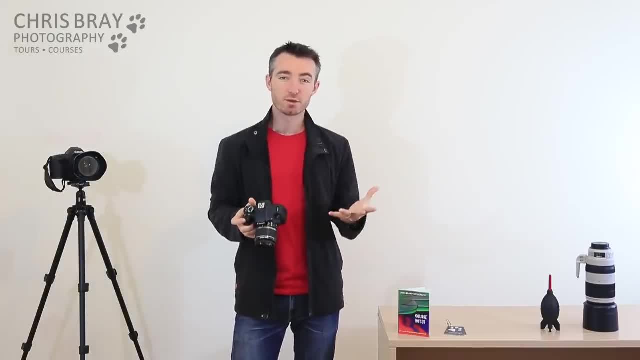 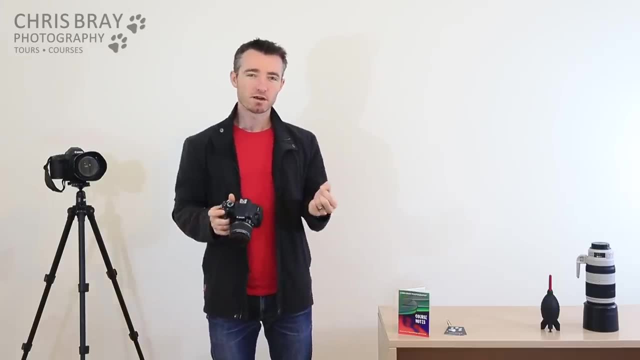 limit that the camera can do. So you can pick whatever f-number you want, as long as the lens can do it, but there just might not be a fast enough or a slow enough shutter speed to match up to it. So you've got to be aware of that. 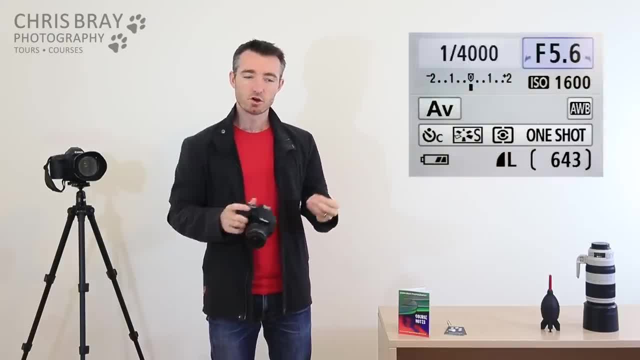 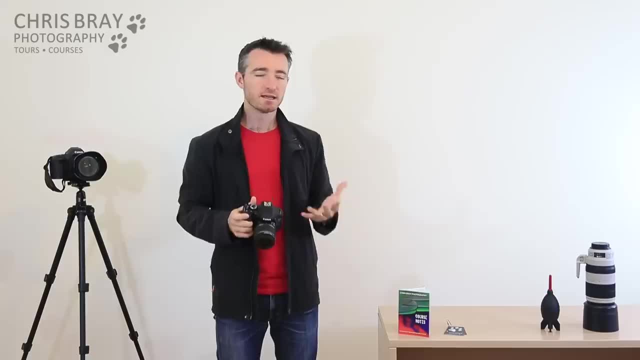 The camera will warn you. it'll sit there flashing the f-number at you or it might go red, or Nikon's normally say high or low. there'll be some warning there letting you know that the f-number you've picked is basically out of range for the current lighting conditions. 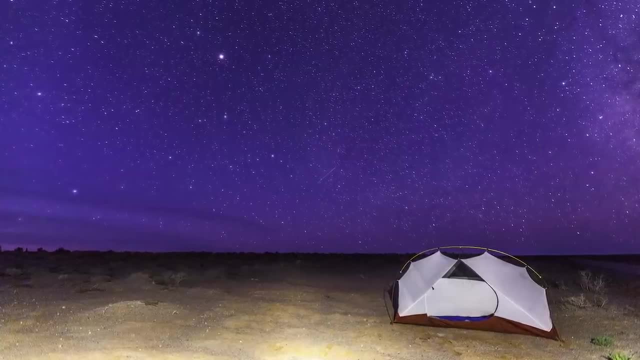 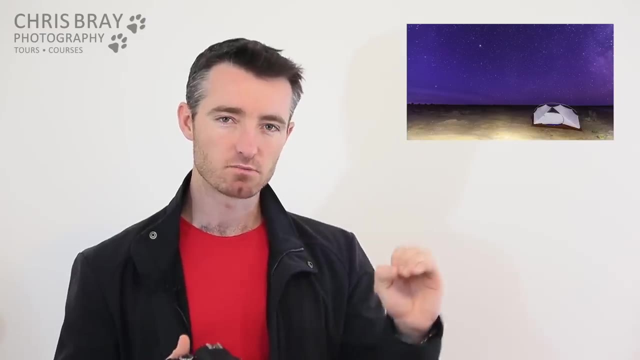 It'll sometimes happen in a situation like this. let's say you're trying to take a photo in the dark and you make it worse by using a large f-number. Now, when I say you're making it worse, that's because a large f-number is a small hole. 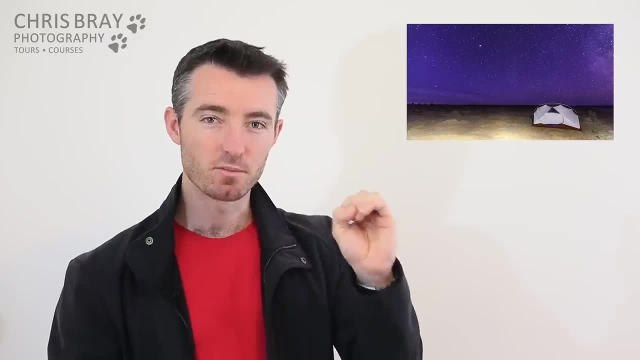 so there's already almost no light out there And you're forcing it to come in through a pinhole. It's going to take forever to get enough light in there for the photo, well and truly more than the 30 second limit that the camera can do itself. 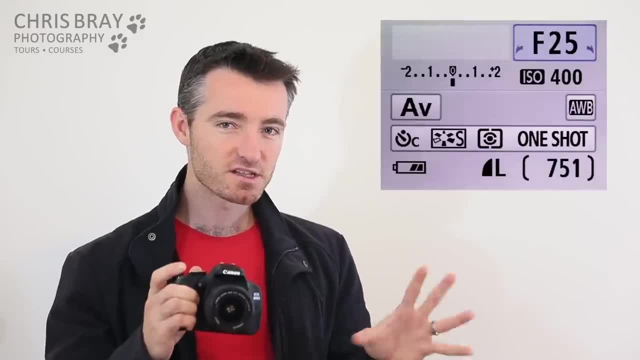 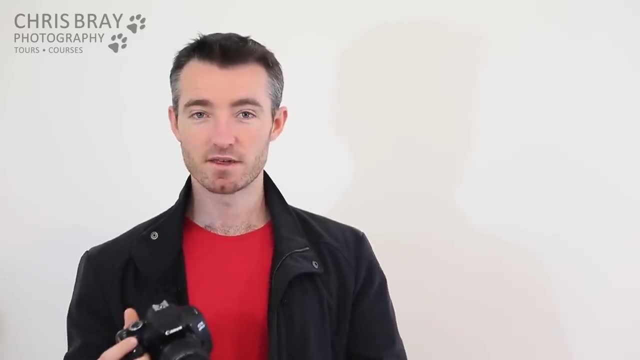 But it won't stop you taking the picture. it'll just flash 30 seconds at you, basically saying: don't do it. if you take this photo, it's your own silly fault. It'll just stay open for as long as it can, which is only 30 seconds, and then it'll give. 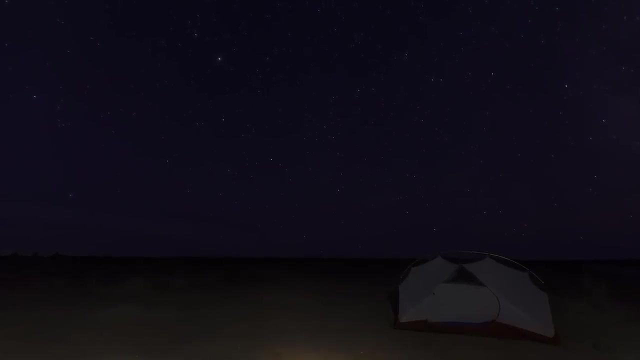 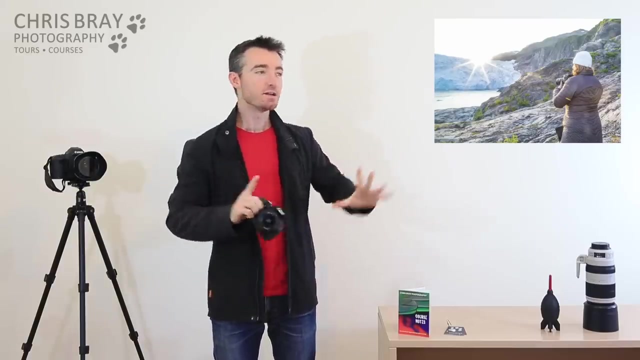 you a photo back that just looks dark. It's just it couldn't stay open long enough to give you the correct brightness. The same thing can also happen at the other end, if you use too small an f-number, so too big a hole, and you're pointing straight at the sun or some really bright light source. 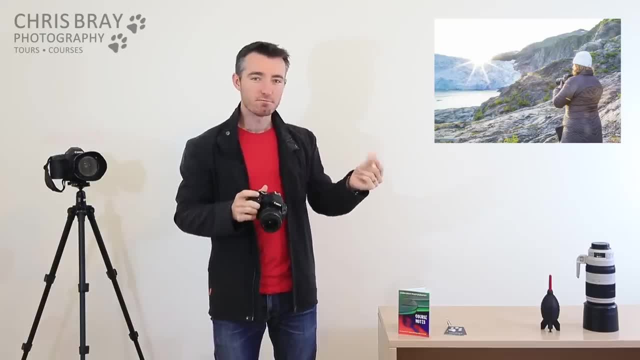 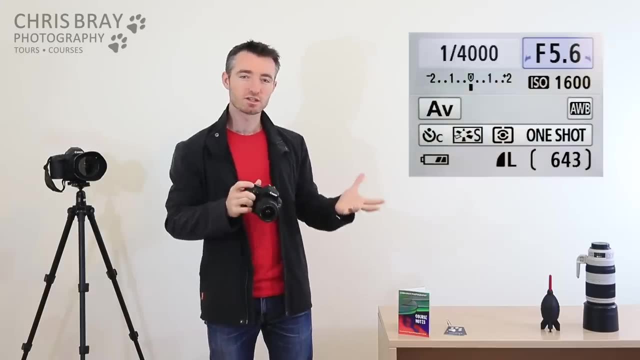 Then so much light comes gushing in there, the camera only really needs to be open for a millionth of a second to get the correct exposure. But the quickest photo it can do is maybe four thousandth of a second, and still too much light's going to get in and you'll end up with an overexposed photo. 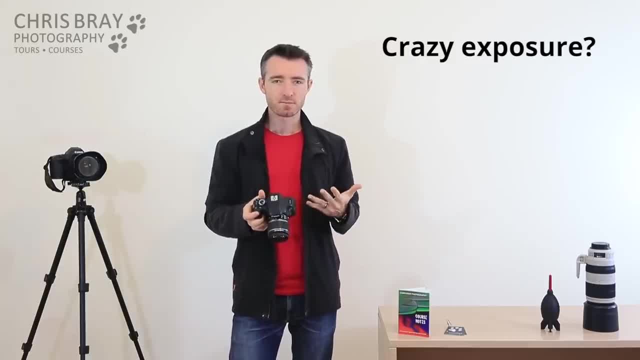 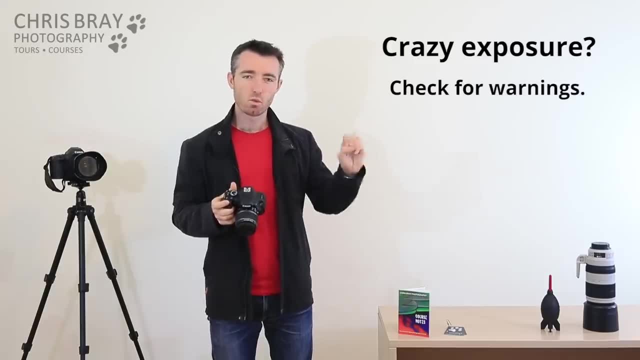 So that's a bit of a telltale. If you're looking at a photo and you just seem to be getting inexplicable exposure, like I asked for it to be brighter and it's not getting brighter, or something like that, it probably was telling you that there was something warning, something flashing at you. 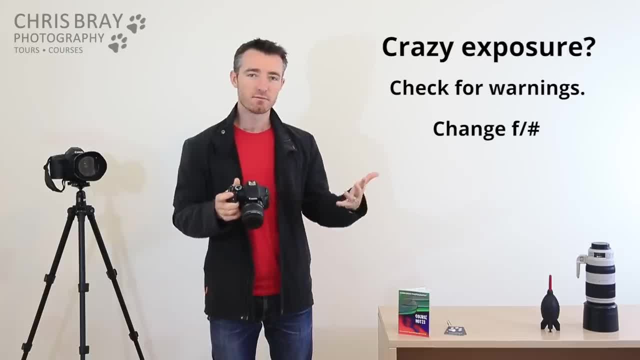 and you just missed it. So just don't use such a large or such a small f-number until it kind of calms down and doesn't have any flashing warnings at you. Another thing you can do to combat that is change your ISO. but we'll leave that to. 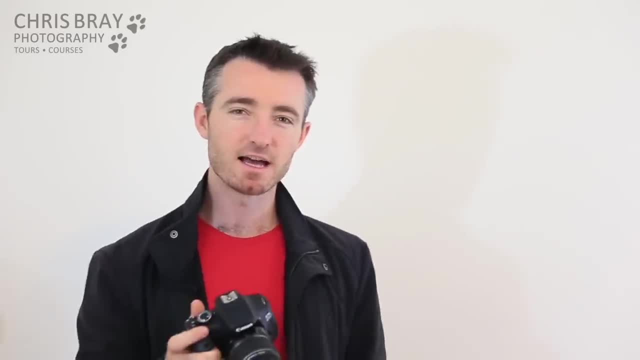 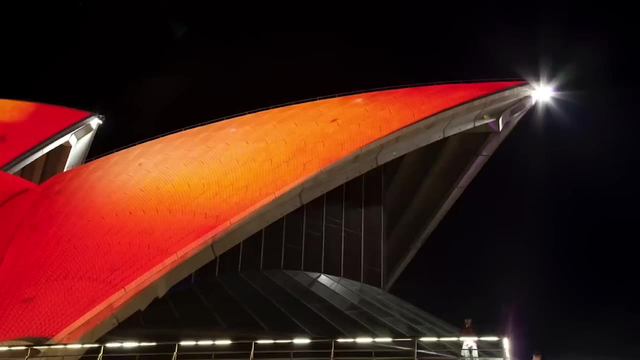 the ISO lecture. An interesting side effect you can get with using a large f-number. apart from having a large depth of field, it actually tends to make any point. light source turn into a bit of a star, a bit of a starburst. 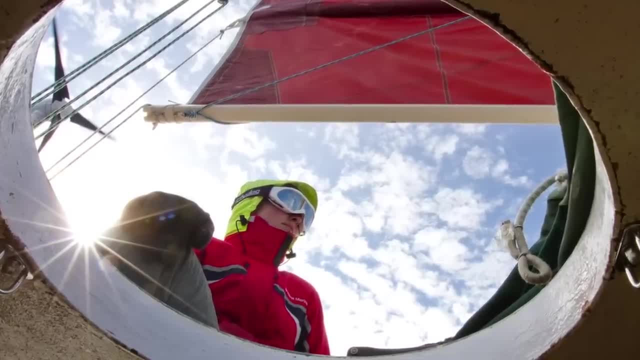 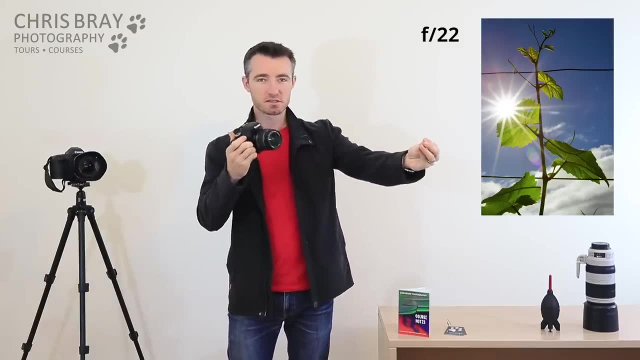 It can look really cool. Some people hate it but I think if it's used properly it can be quite nice. So to get that effect, you have the sun actually hiding behind the leaf or the building or whatever it is, while you half press and set the exposure and focus and all that kind. 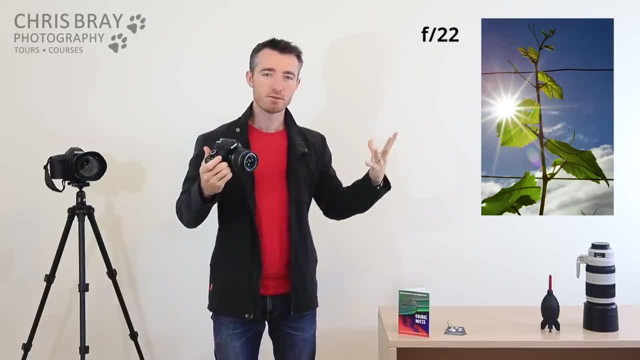 of stuff. Because, remember, if you have the sun already in the shot, it might throw out your metering and you'll end up with a silhouette. So you have the sun hidden half, press beep and then just move to the side just until. 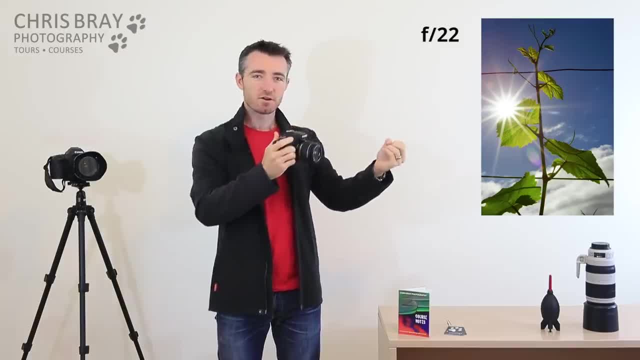 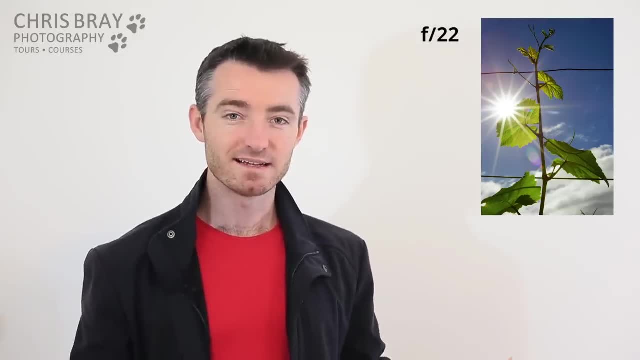 the sun just starts bleeding over the corner of the building. Take the photo just before you go blind. basically, Obviously, don't look at the sun with a really long lens. This effect works better anyway with a very wide lens. If you look at the sun through a long lens, you actually risk going blind. 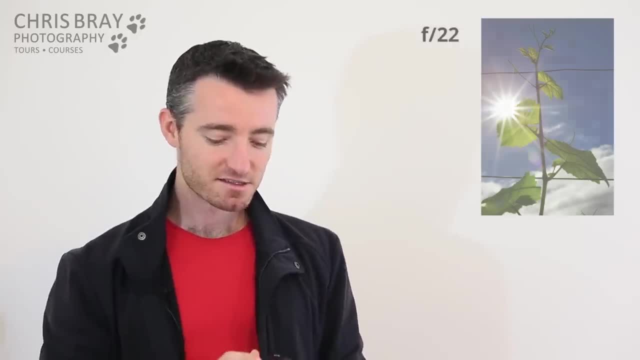 It's like looking at it through a telescope. You can just burn a hole through the back of your head, So try not to do that. Alright? so it's time to go out for your aperture prac, which is actually a pretty straightforward prac. 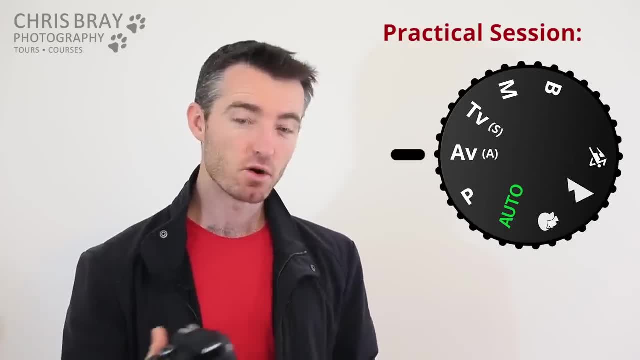 You just pick up your camera, make sure you're on aperture mode, AV mode or A mode, and then you just want to find a subject and take two different pictures of it: one with a big F number, one with a small F number. 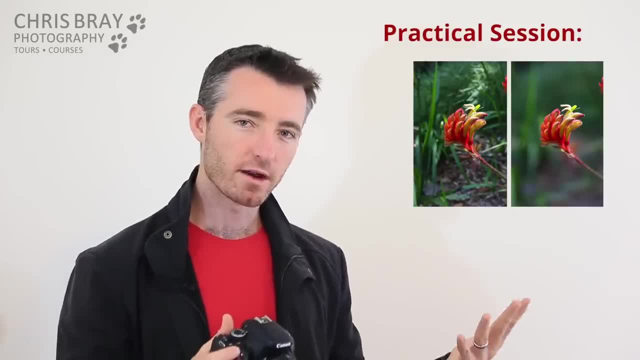 And then just compare the two and you should be able to see the background blur out in one of them and become sort of sharper and more distracting in the other one. Like, look at these two photos. Which one of these has the smaller F number? 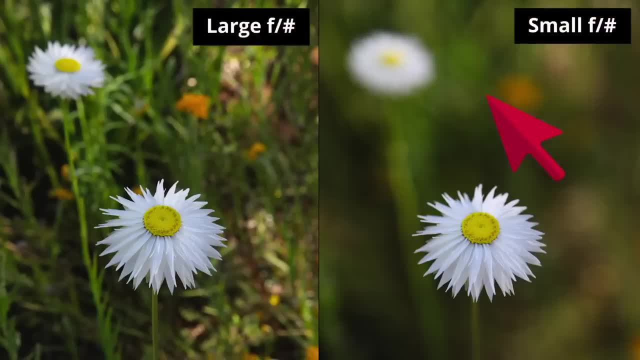 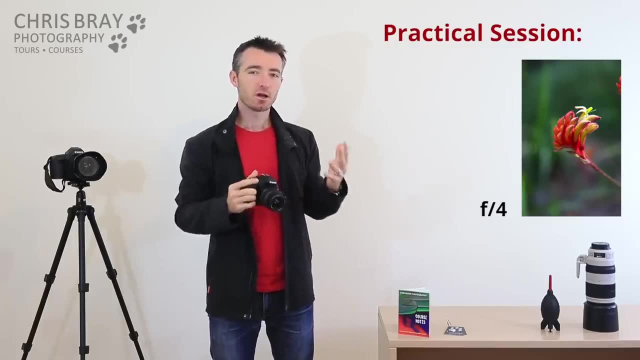 The smaller depth of field. Definitely it's this one. In fact, the closer you get to your subject and the further away the background is, and the more you zoom your lens in, that'll all help to give you a nice blurry background. 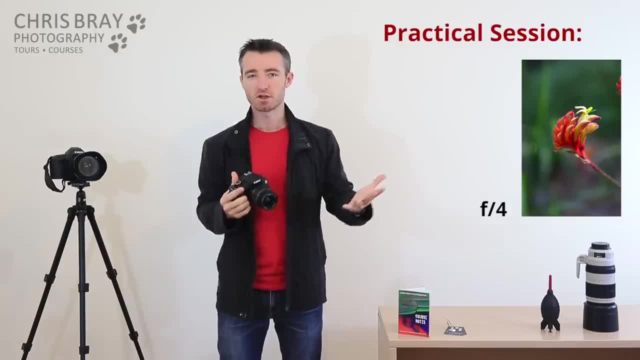 If you're really not able to see any difference between your big F number and your small F number shot, you just probably didn't pick a good example. You know you've got to get closer or find something that's not so many different things. 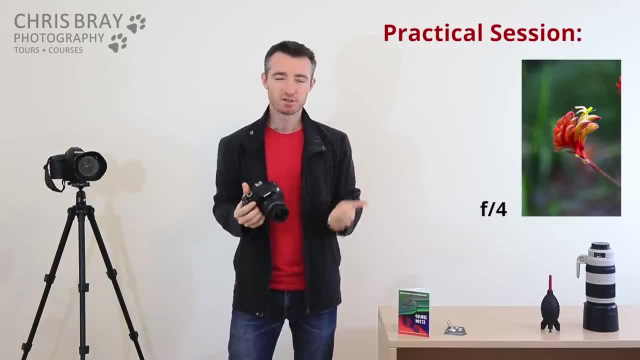 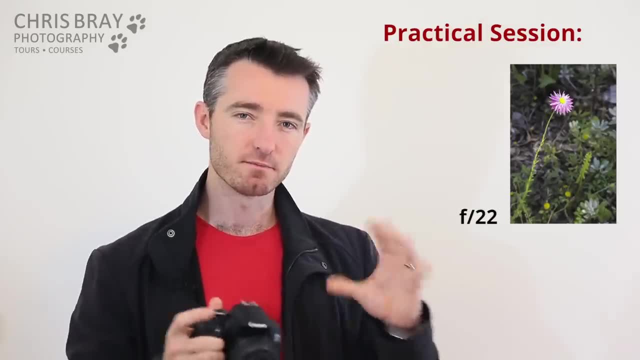 at a similar distance away. Just get closer, You'll get there. in the end. You should be able to see a fairly dramatic difference. Another common problem you might have with this project is that you're not able to see anything. The problem with this project is if you're using your large F number. so for the big 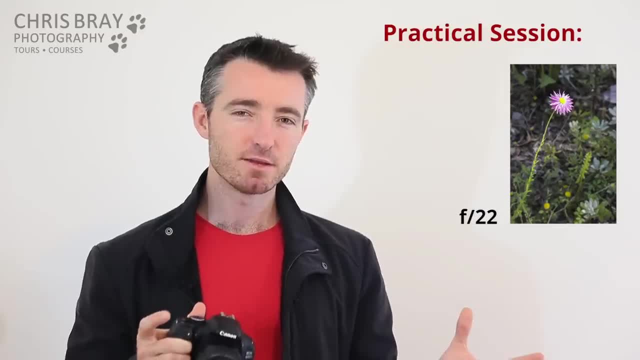 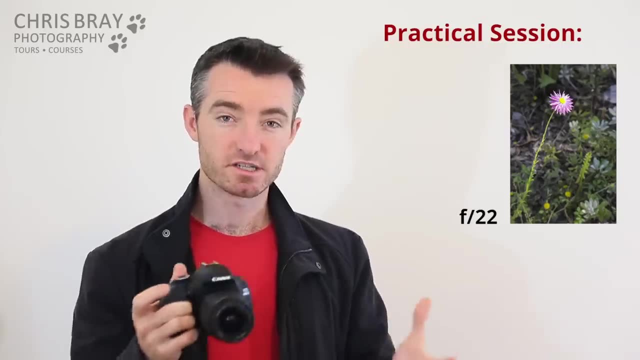 depth of field. you expect the whole thing to be nice and sharp, But you might actually have a problem where the big F number makes your photo so slow that you get camera shake and in fact the whole thing goes blurry just from subject movement and camera shake. 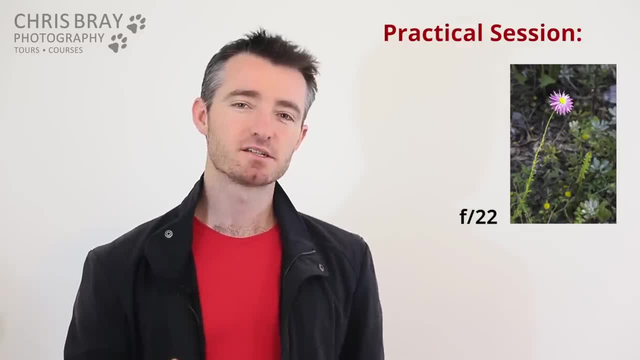 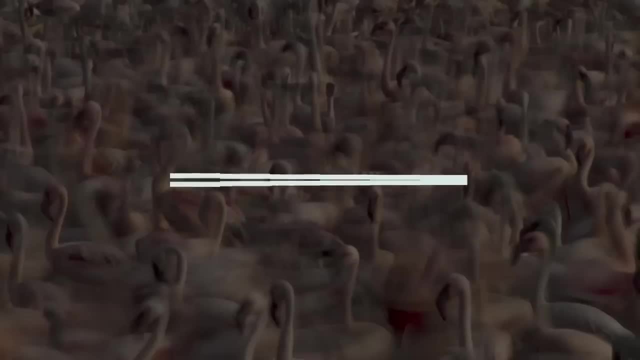 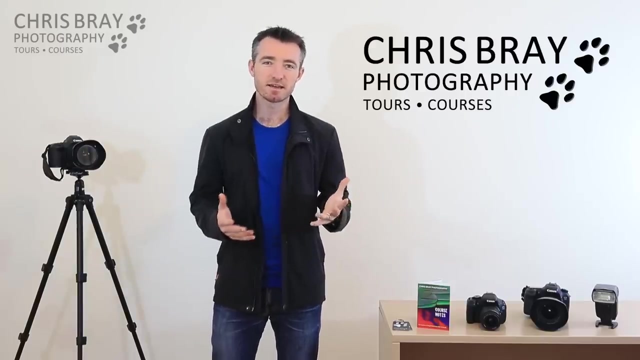 Nothing to do with the F number. So if you're getting camera shake problems, then just turn your ISO up more. Then come back in and look at the next lecture, which is exploring shutter speed. So in this lecture we're going to look at shutter speed and the effect that has on. 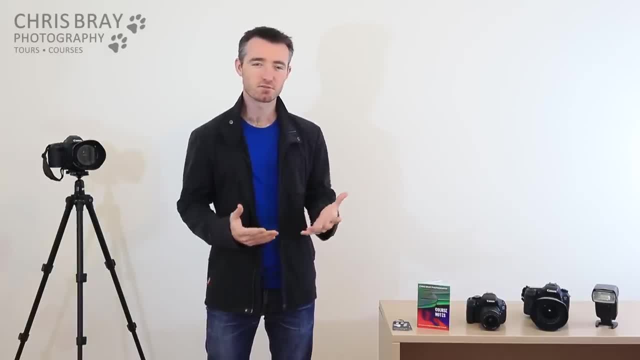 things that are moving in your photos. It's nothing like as long or involved as the previous lecture on aperture, because it's pretty obvious really: The longer the shutter is open, the more things can move, the more you get movement blur and so on. 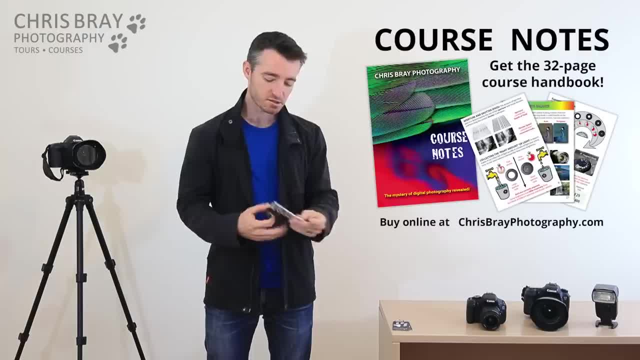 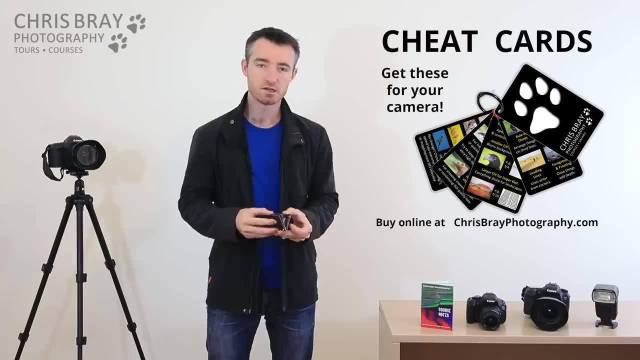 But you might still pick up a few interesting little tips. And don't forget, this whole section is also covered in our course notes booklet that you can buy online, and also those little plastic summary clip cards as well. There's a section there on, you know, using shutter speed to freeze or show movement, and 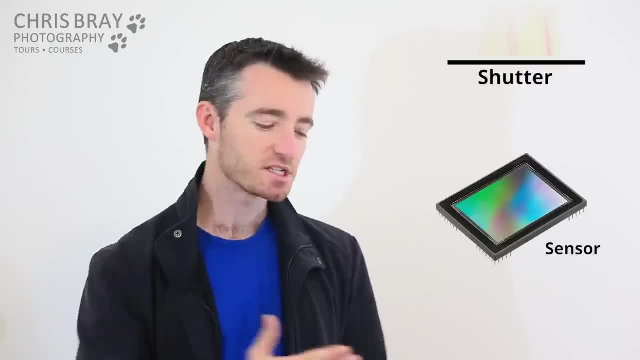 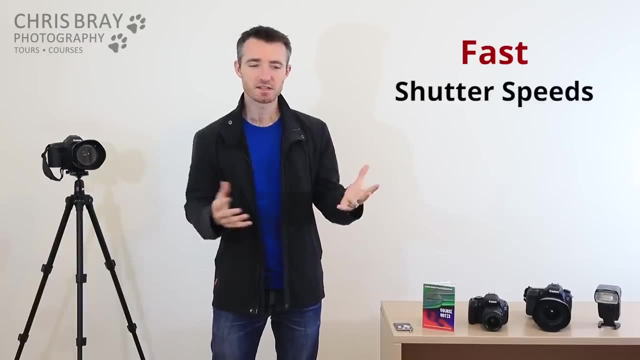 how you do all that kind of stuff. So what is shutter speed? Well, as you know, it's just how long that shutter is open, for how long the light is allowed to shine onto the sensor for. So if you use a very quick shutter speed, then nothing's had a chance to move anywhere. 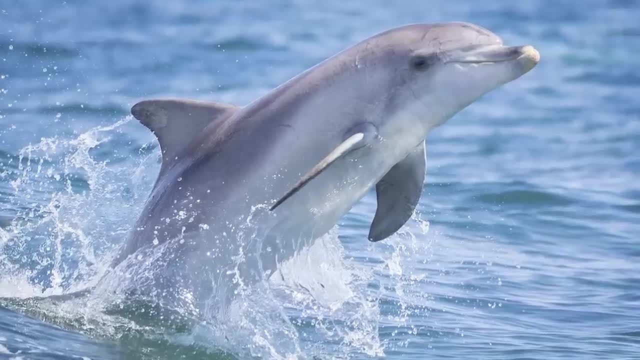 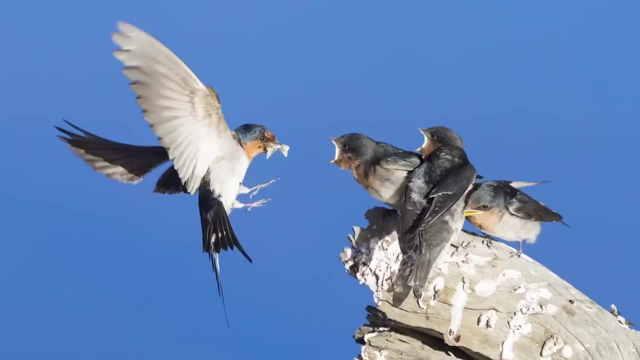 while a photo is being recorded, so you end up being able to snap freeze- even quite fast- subjects like these ones. You know it's worth knowing that almost all of your cameras should be able to do four thousandth of a second. You can all snap freeze photos like this if you know how to control it properly. 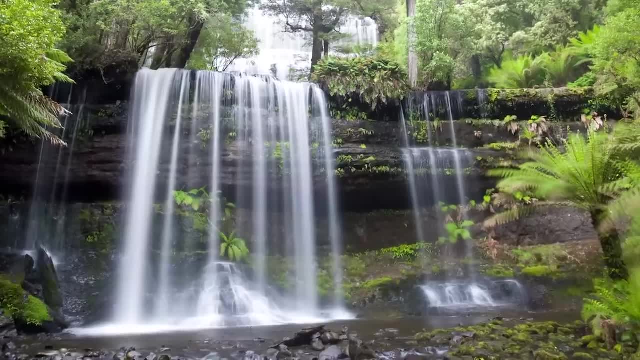 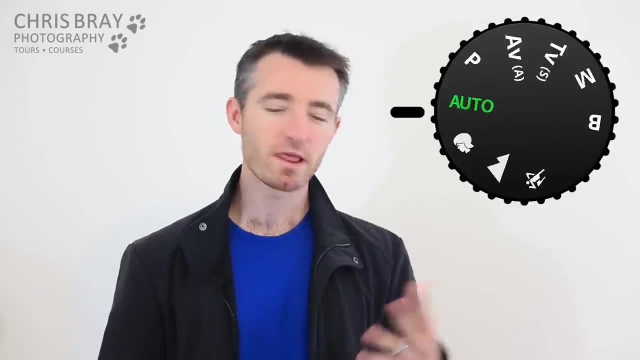 And slow shutter speeds, on the other hand, show movement blur, so anything that's moving becomes streaked across your image And you can create some really beautiful effects. Incidentally, sports mode. If your camera has a sports mode, one of the things that sports mode tries to do is give 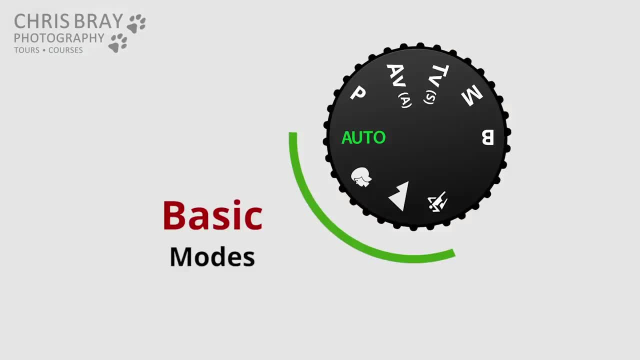 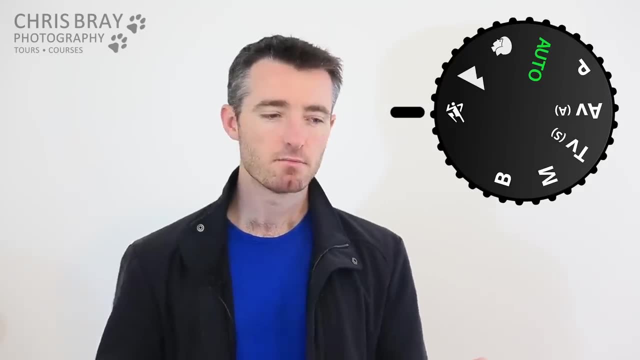 you a nice fast shutter speed so you don't have blurry people running around. But the problem with all of these basic modes are that you can't change anything yourself. So sure, it might try and give you a fast shutter speed, but what if you wanted to brighten? 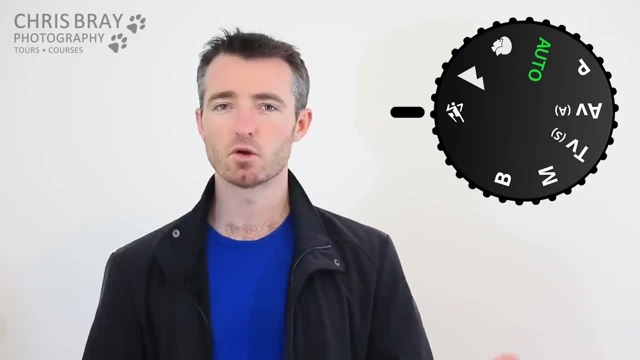 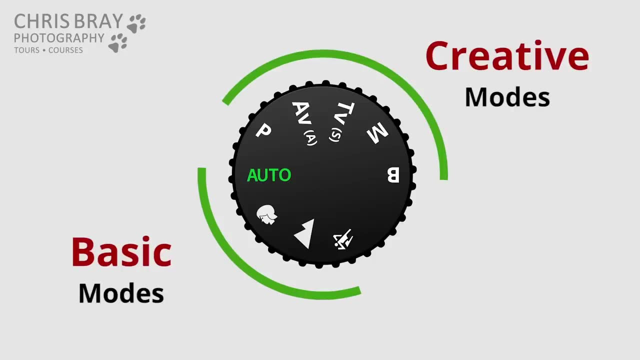 the photo with your exposure compensation or you know, use a different autofocus point or something. You can't do any of that kind of stuff. Yeah, they're incredibly limiting modes to be in. You may as well be in aperture or shutter speed. 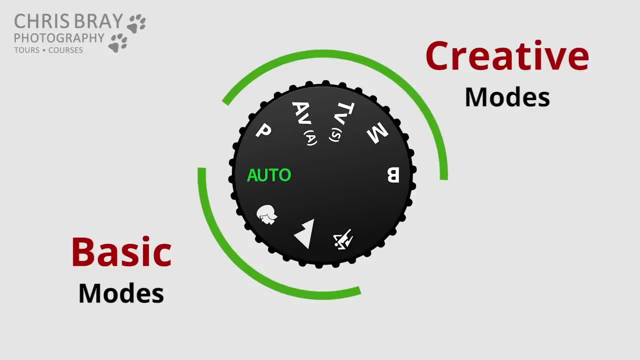 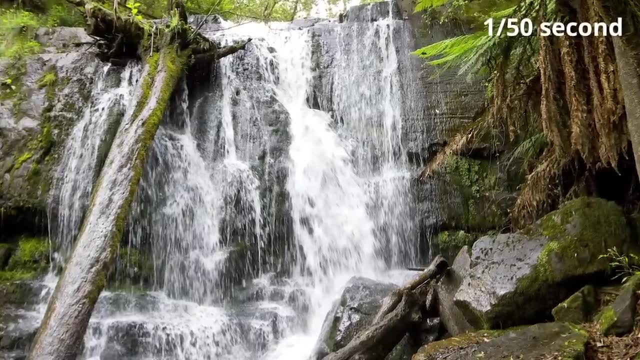 Here's a photo of a waterfall taken in auto mode And, for whatever reason, the camera thought that 50th of a second would be about right Now. 50th of a second is not particularly quick or particularly slow, so we haven't frozen. 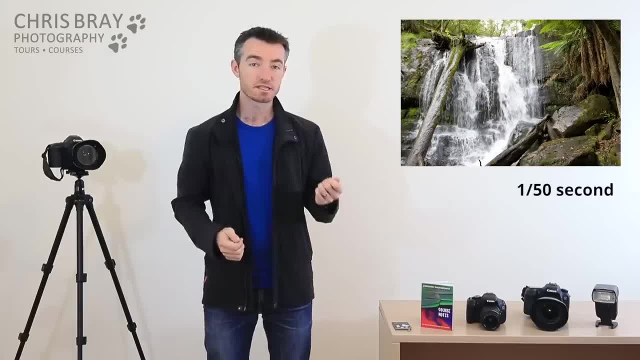 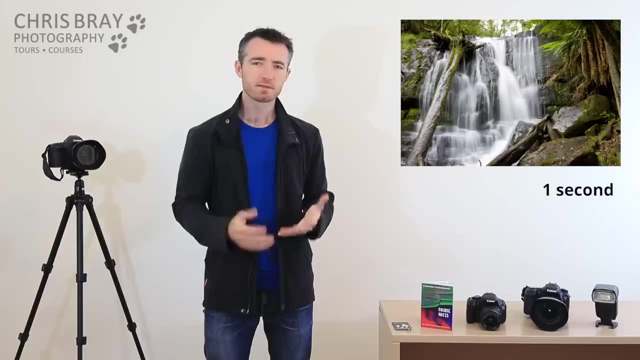 the waterfall or shown that nice flowing movement. But if instead we ask for a one second photo, then now you can see that lovely flowing cascade effect that looks so beautiful in waterfalls. There's a lot of situations where showing a bit of movement in your photo is a good. 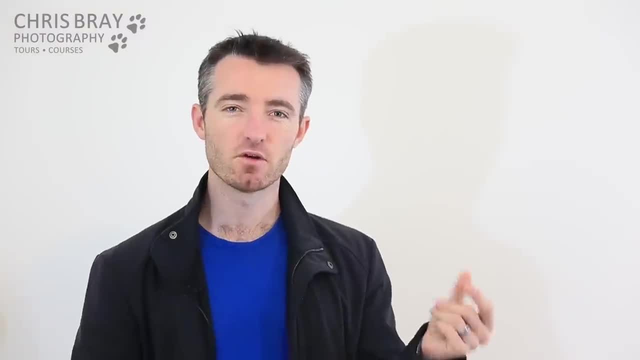 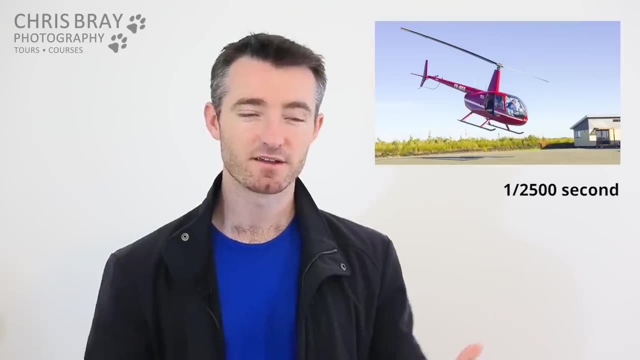 way to add a bit of life. You know, if you take a fast photo of a helicopter, normally you end up with a really fast shutter speed and the blades are just frozen there in mid-air and it kind of looks like the engine's turned off and it should just be falling out of the sky. 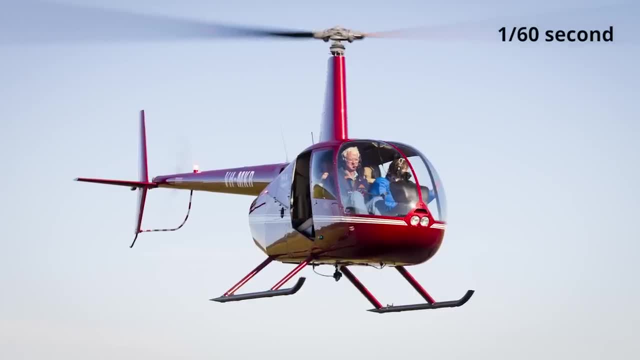 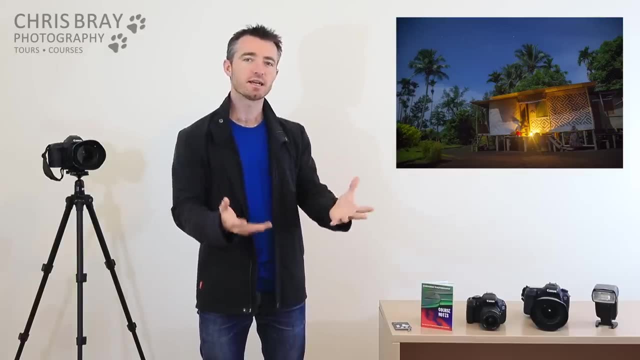 But if you allow just enough shutter speed that the blades can turn a little bit, it just looks more natural like the engine's still going. Most low light photography has to be quite long, slow photos, just because it takes a long time for the camera to get enough light in there to record the image. 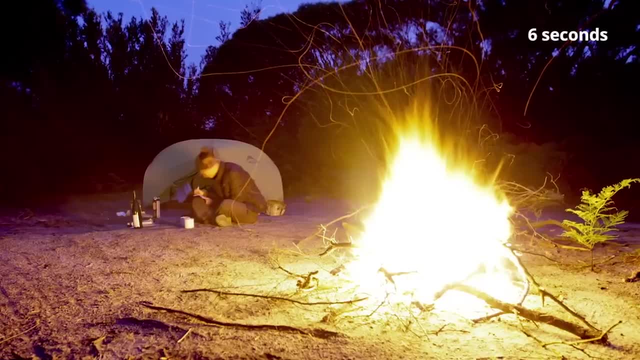 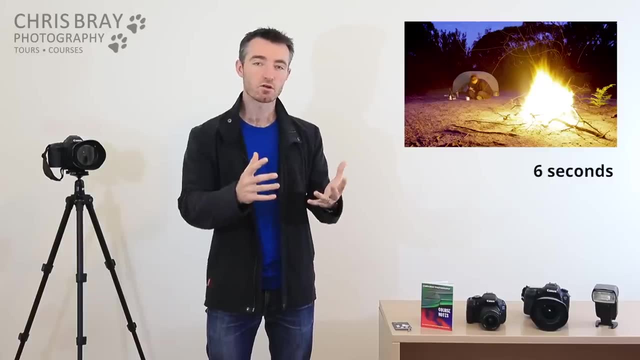 But this is some of the most beautiful creative photos you can do, I think Like this one: 30 seconds. So obviously the camera has to be absolutely motionless, so ideally on a tripod or at least sitting on a rock or something where you don't have to touch it. 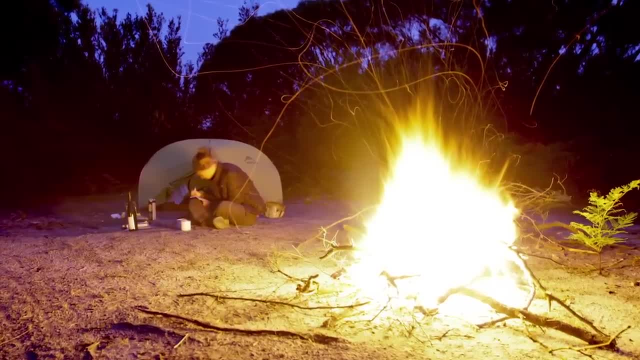 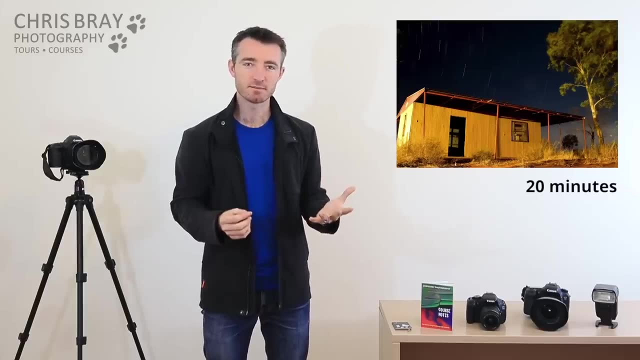 But not only does the camera have to be motionless, of course your subjects do as well, And you can see. actually she has moved, so she's blurry there. but it would have been alright This one 20 minutes. So now we're getting beyond the 30 second limit that the camera can do by itself. 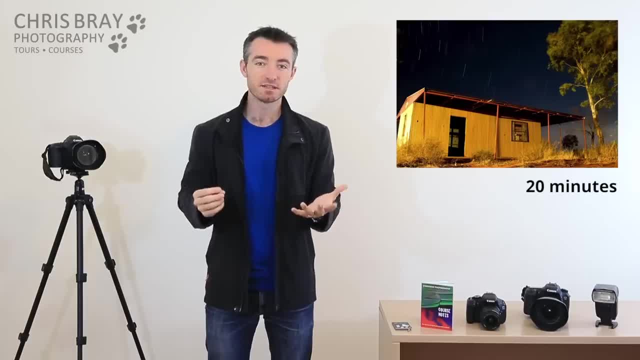 So to get this kind of shot you've got to plug in some external timer. So after 20 minutes obviously the earth has started to rotate and the stars get dragged past the sky there And I'm beginning to get a bit of a star tracking. 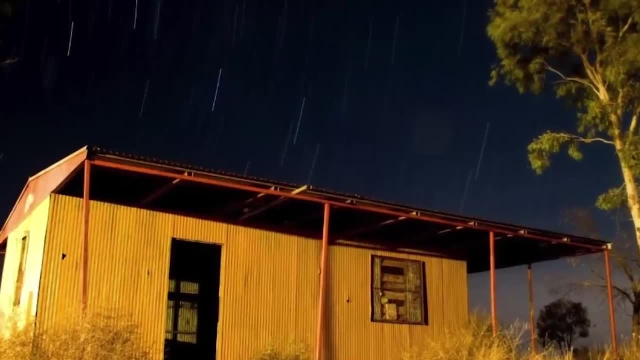 So I'm going to go back to the camera, But it's cool to see the star trail is not actually a straight line, is it? It's a bit of a curve, And if you can work out where the centre of that set of circles are, you get a photo like: 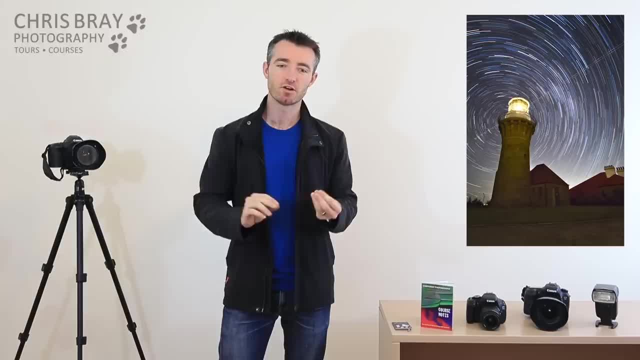 this one. So to work out where that point is, where all the stars are spiralling around in the northern hemisphere, it's a bit easier. There's a giant star there called the North Star, and if you can recognise that it's. 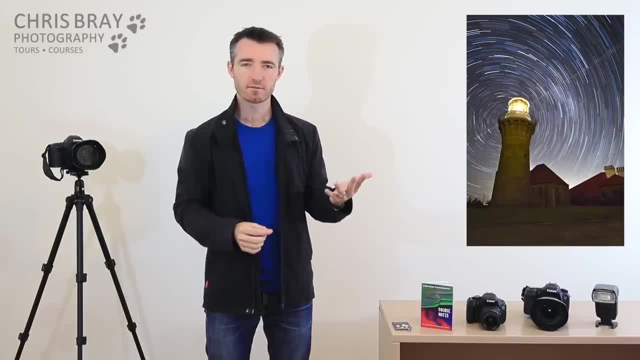 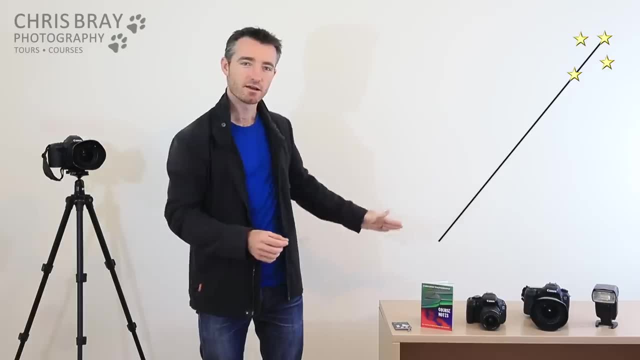 easy In the southern hemisphere though it's a bit more complicated, But you can work it out from the Southern Cross. So if you find that constellation and you just draw a line down through the middle of the Southern Cross, like a string coming down from the continent, 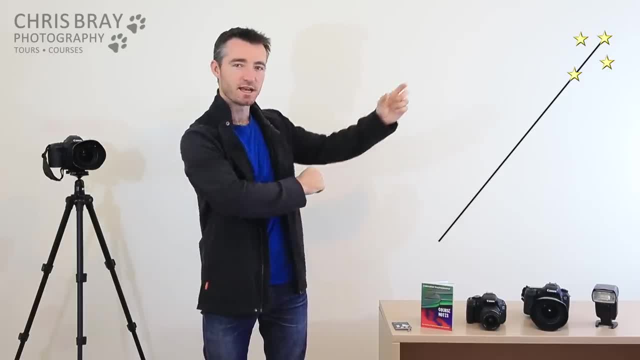 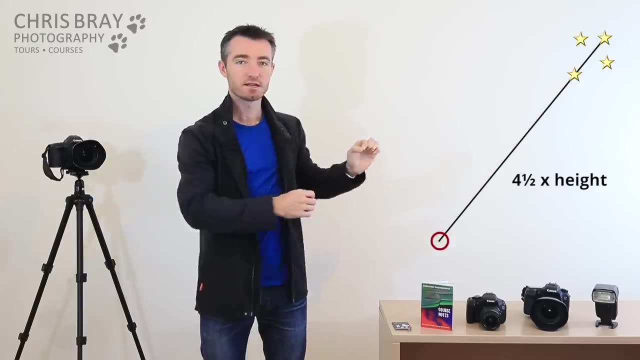 And if you just extend the axis of the Southern Cross down by about four and a half times the height of the Southern Cross, so you just kind of go there. it is one, two, three, four and a bit. that's the same point. 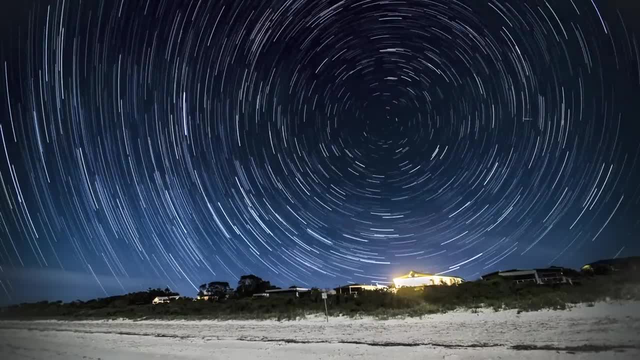 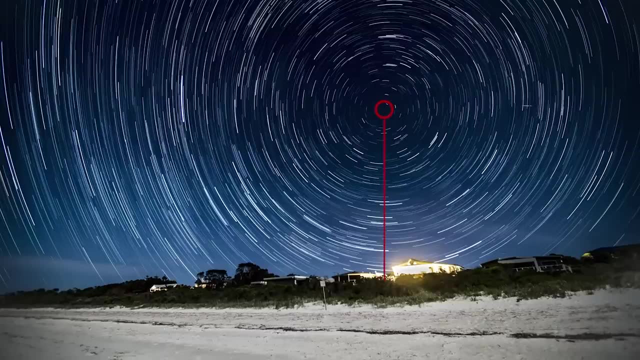 That's where it's all spiralling, So you can put that somewhere for good composition in your shot. And also, if you're lost and you're trying to work out where south is, find that point and then directly down the nearest bit of horizon straight underneath. that'll always 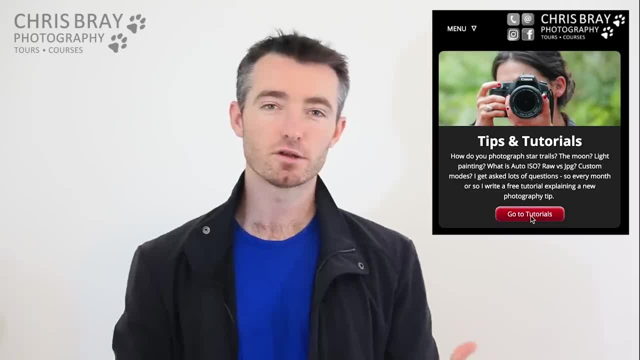 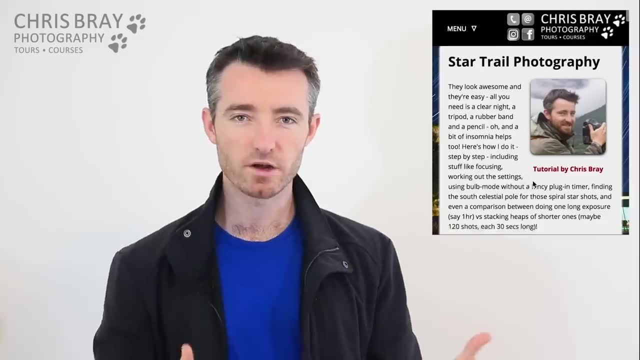 be due south, So that might come in handy as well. We've actually got a whole lot of really good tutorials on our website, including one on Star Trails. It's quite popular. They look quite long, these tutorials, but it's just because I've worded them in a way. 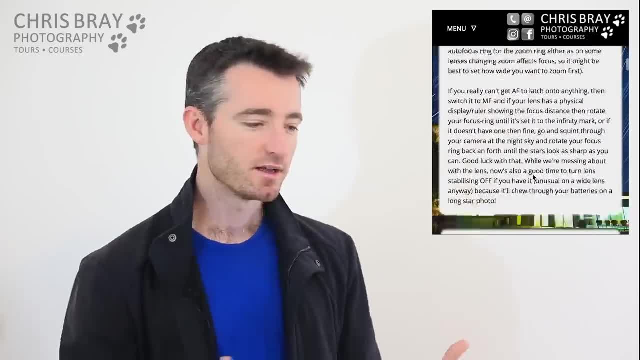 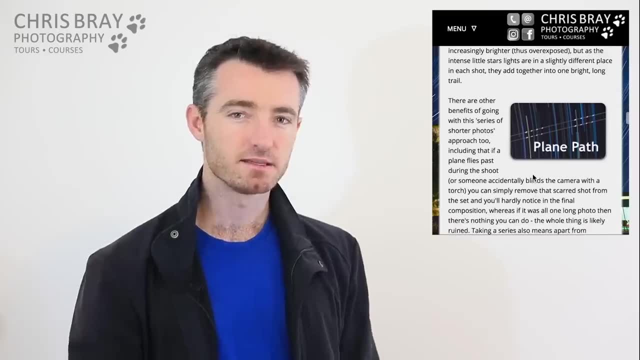 that they're really easy to understand and they don't assume any prior knowledge. So it goes through everything, like: what lenses are you going to use and how do you focus, because it's in the dark? What are the common problems you might come up against like a plane? 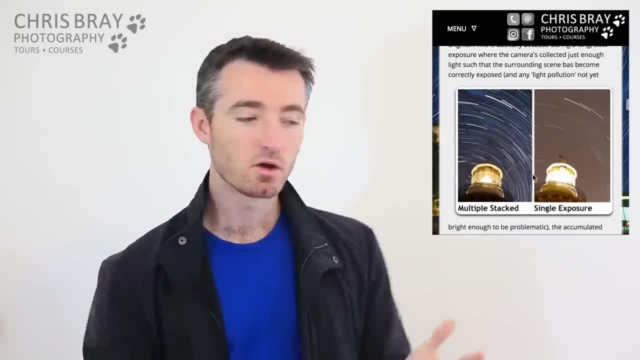 What are your different ways of being able to do it? You could do one really long exposure, or you could do a whole lot of short ones and then stitch them together using free software. There's a whole lot of different options out there and it's really worthwhile having a. 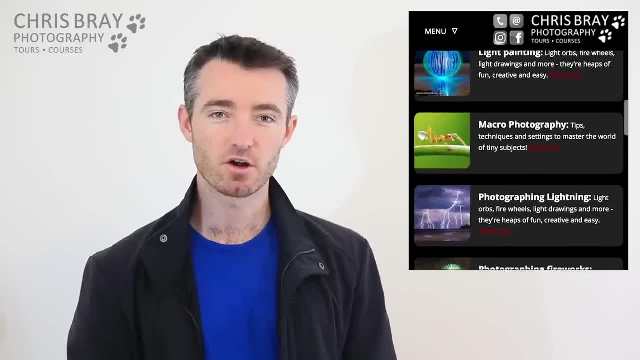 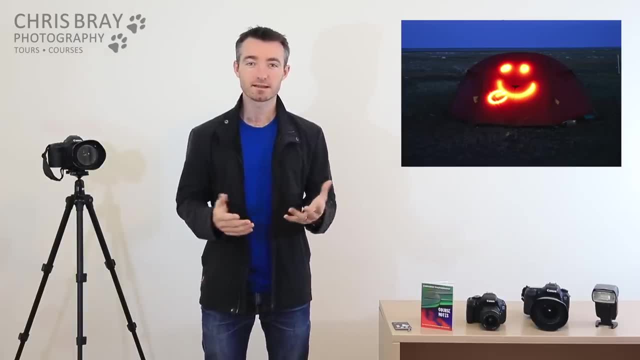 look at these free tutorials. So go to the website crisprayphotographycom And have a look there. There's so many different tutorials Now, longer, slower shutter speeds. they give you time to be a bit more creative with light. 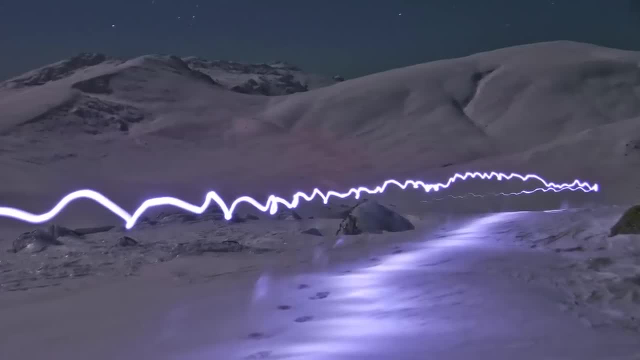 and come up with some really cool photos, Like this one. it's a photo of someone walking through the snow carrying a torch. You can't really see the person in the photo because they've kind of smeared themselves across the whole image. 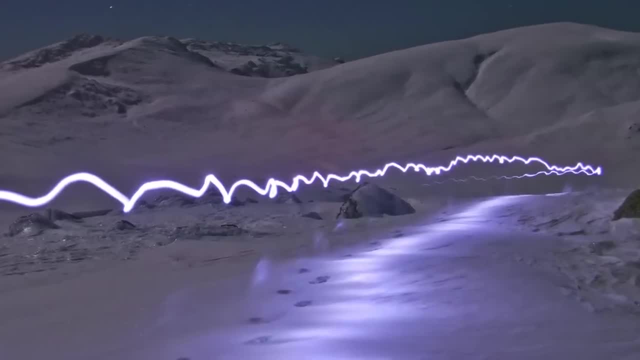 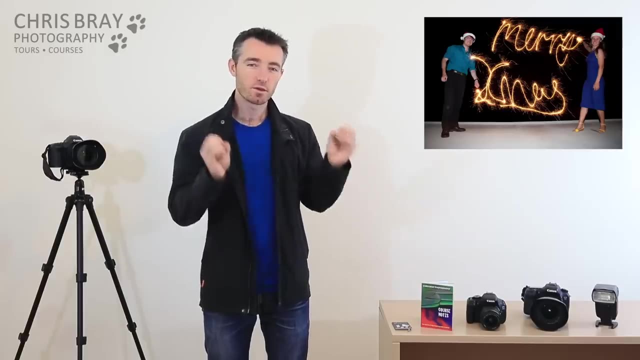 But the torch was bright enough that wherever it went, it really left a mark on the sensor. This was our Christmas card photo a couple of years back, so there's no fancy Photoshop or anything going on here. It's just a 10-second photo with a flash at the end of it. 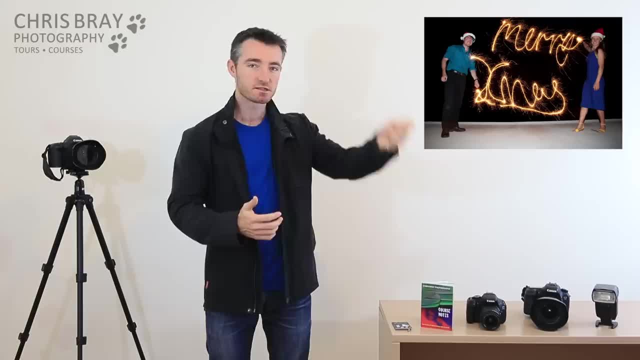 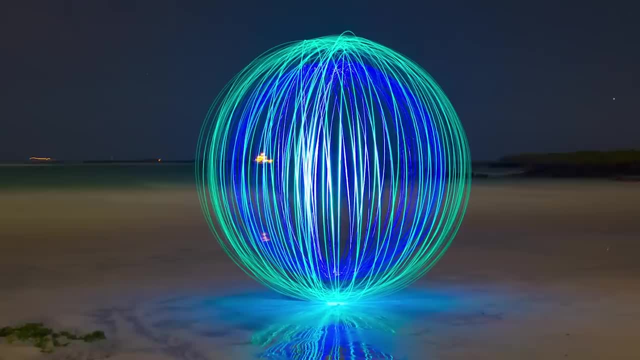 So initially all the camera can see is the light. It's just black. And then the sparklers write Merry Xmas, And then we stand to the side and then the flash goes off and fills us in there. It's pretty cool what you can do with these kind of things. 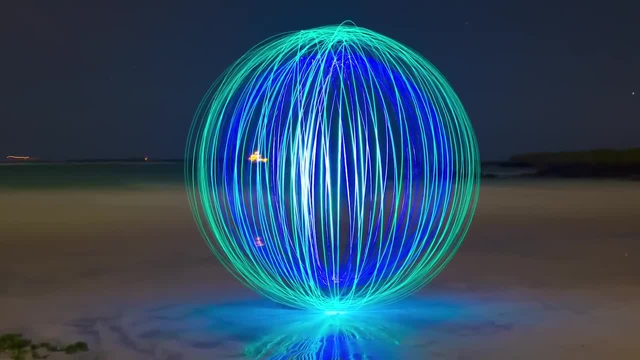 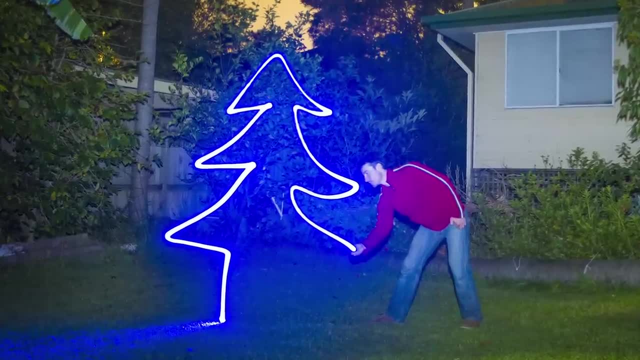 Or this one: you can tie a light to a string and spin it around while you walk in a circle and you end up with a light orb. Looks pretty cool. You can draw pictures just in free space. You just use these little torches to draw shapes or symbols, and then the reflection. 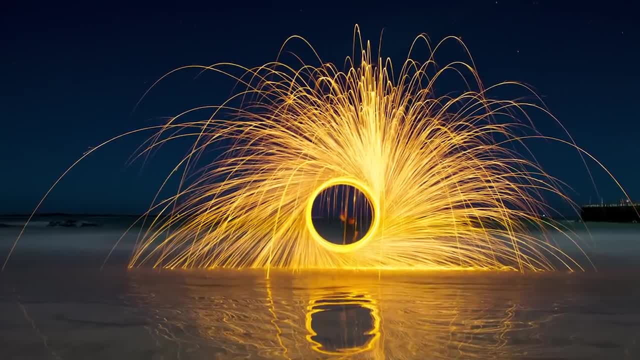 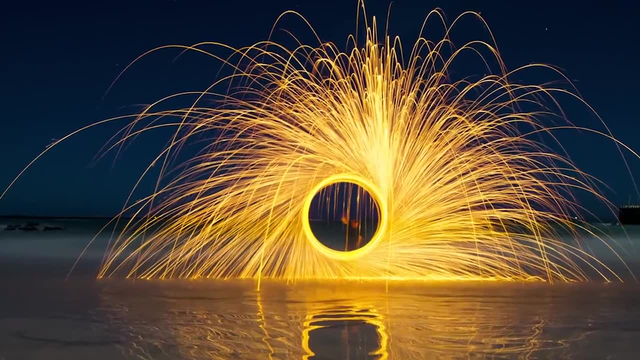 there is because we've done it on a wet beach And if you haven't tried a photo like this one before, you really have to. It's great fun. It's actually steel wool. You wouldn't think steel wool would burn, but it just sort of smolders a little bit. 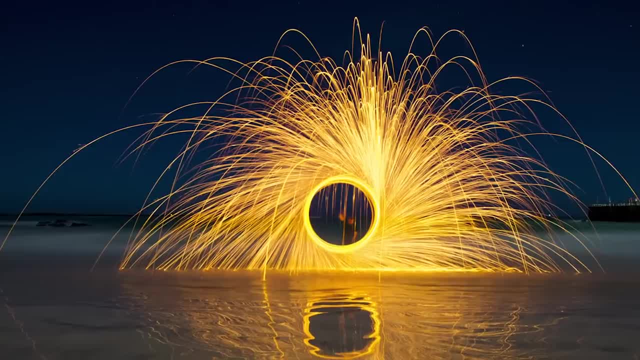 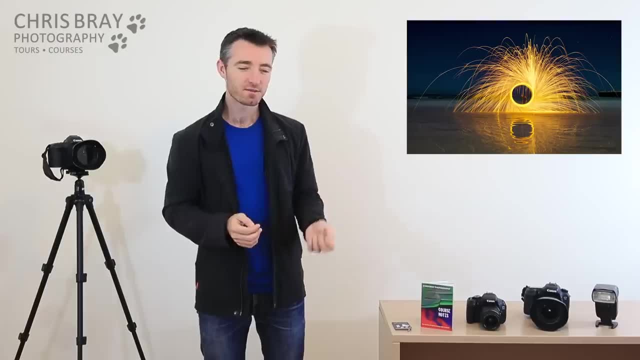 But if you tie it onto a bit of string and spin it around absolutely, it burns and it just sends these beautiful shards of molten metal up in these wonderful arches and it just looks amazing. You've got to be careful, though. 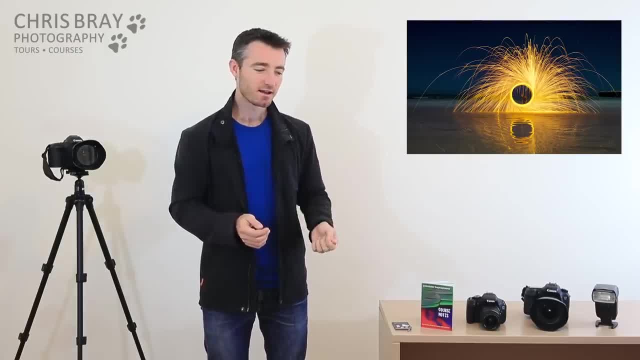 There's a few tips you probably don't want to learn by trial and error. like some of the bits of steel wool go straight up in the air and come down and land in your hair. So good plan to wear a hat And best not to just tie the steel wool directly onto the string, because otherwise you'll. 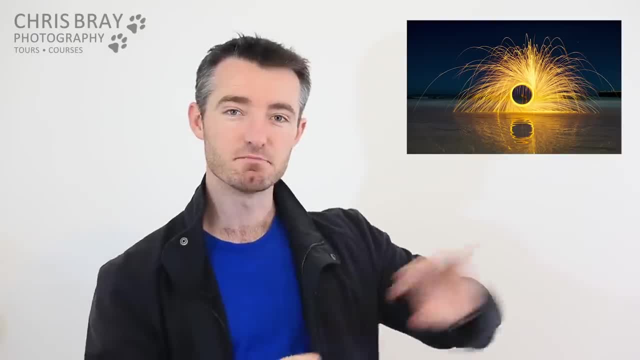 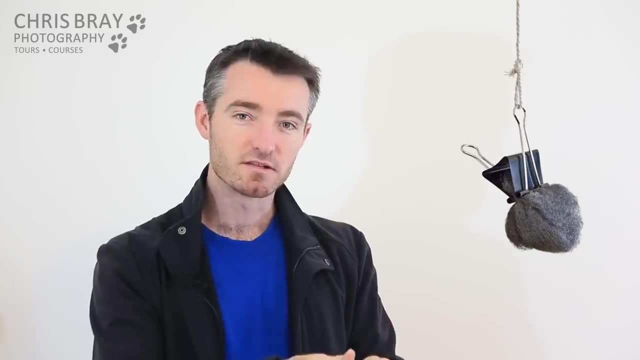 find partway through. It just burns through and you just send this burning meteor onto your neighbour's roof. That's not good. You're better off actually using a bulldog clip, clipping the bulldog clip onto the steel wool and tying the string onto the bulldog clip. 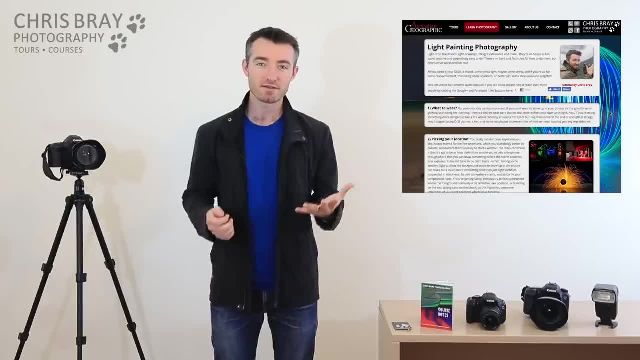 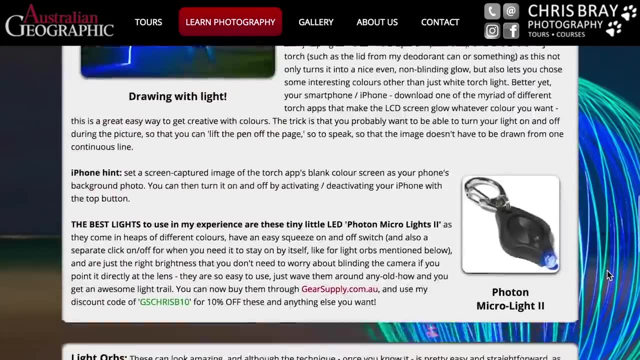 You know a few little tips like that that might just save you a little bit of embarrassment. We also have a light painting tutorial on the website and that just goes through. all about how to take these long, slow exposures where you can draw things with the light. 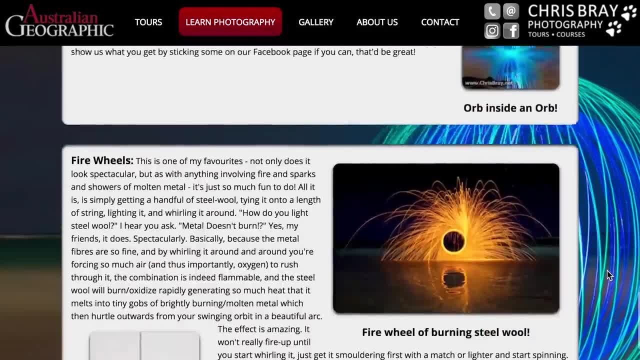 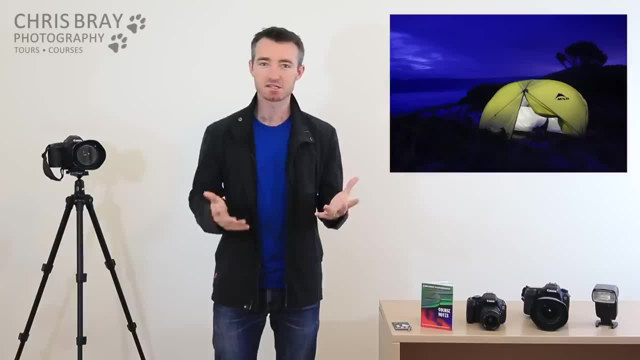 like the light orbs or drawing pictures or the steel wool. So you have a read through that as well and have some fun. But what about this photo of the glowing tent? Now, as much as MSR would like us to believe that tents are wonderfully warm, glowing havens. 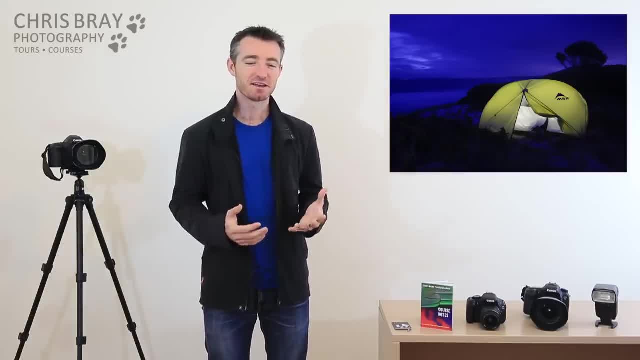 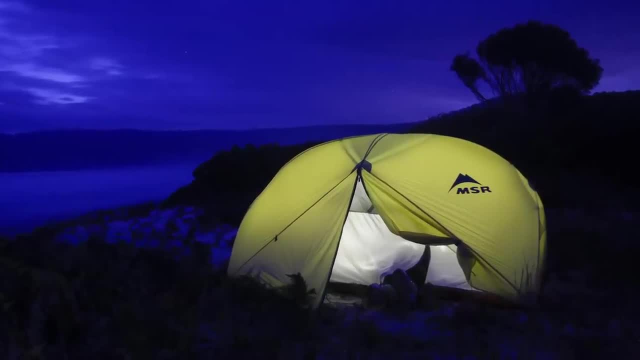 they're not. They're miserable, cold, horrible, wet, dark places. But to make it glow like that you've just got to do whatever you can do in 30 seconds with light. So I've actually just dived inside the door of the tent. there you can still see my legs. 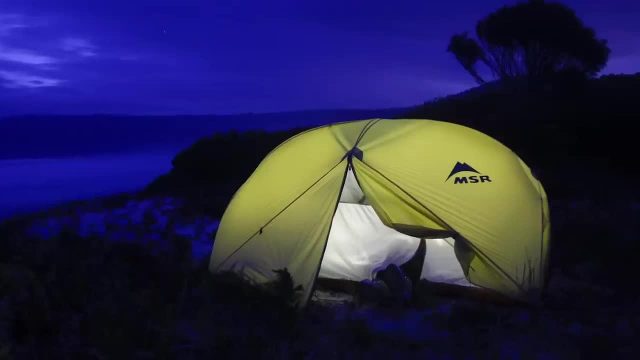 hanging out and the little white lines in there. That's just me waving the torch around trying to give it an even spread of light from the inside. But the thing about all of these low light photos: you can't even begin to do them unless. 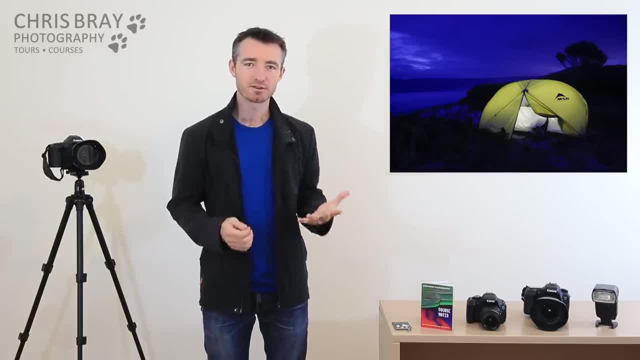 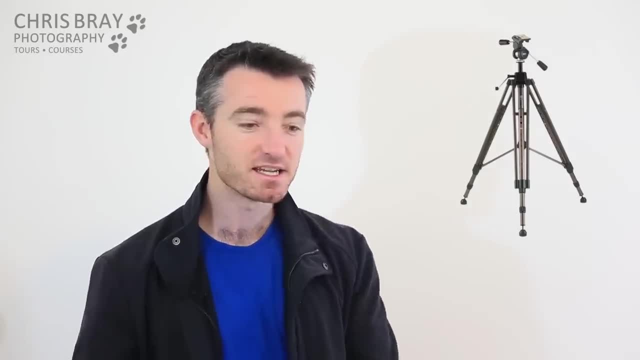 you have a tripod Now. I think that's the main reason why it's worth it. It just opens up this whole world of photography for you. Don't get an enormously giant, heavy one. you know lots of people have that, but they just. 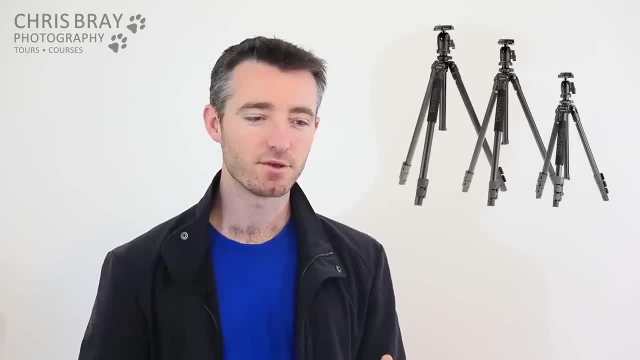 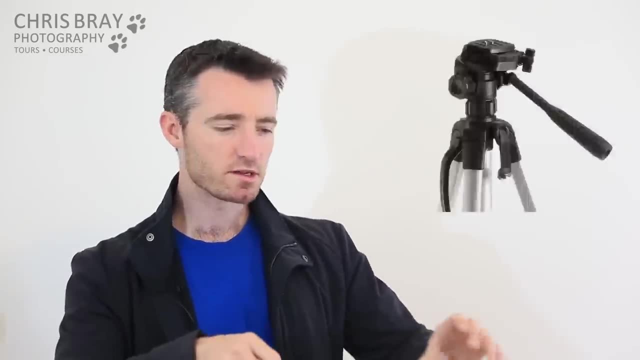 never take it with them anywhere. Get one that's small enough that you can be bothered to take it with you. When you're buying a tripod, I'd consider getting one that's with a ball head. that's nice and easy, easy to move around. you know the old ones where you have to kind of adjust. 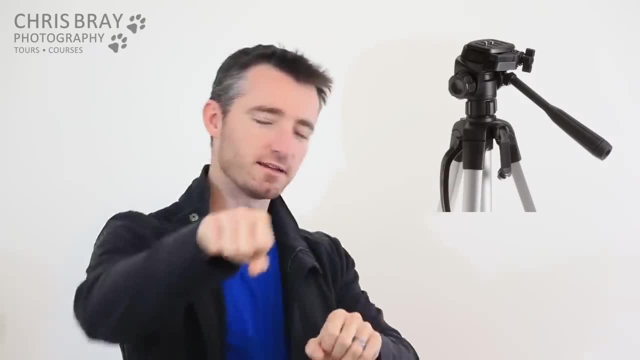 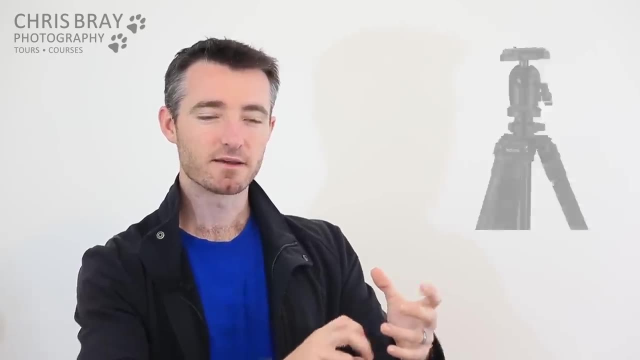 one lever this way and then some other adjustment here to go vertically- and it's quite awkward to use A ball head is what I like, where you just undo one thing and you can point it wherever you want And then it's nice and quick. 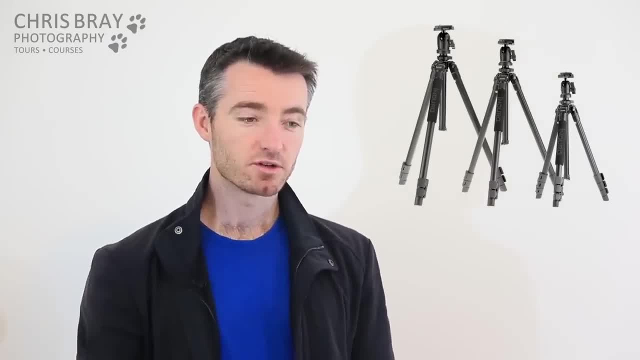 And all tripods have a load limit that they're designed to support. so you've got to make sure your tripod is strong enough to support your camera and your heaviest lens, But don't go and buy one that can support ten times as much, because it's just too heavy. 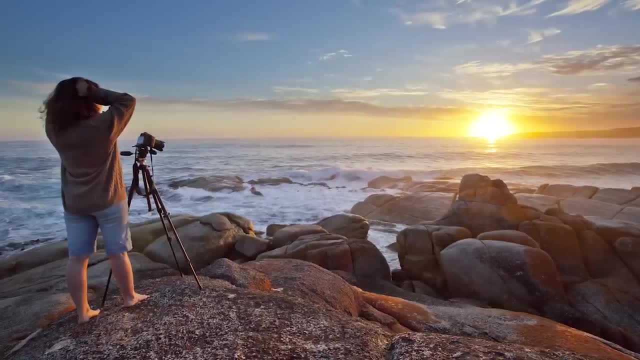 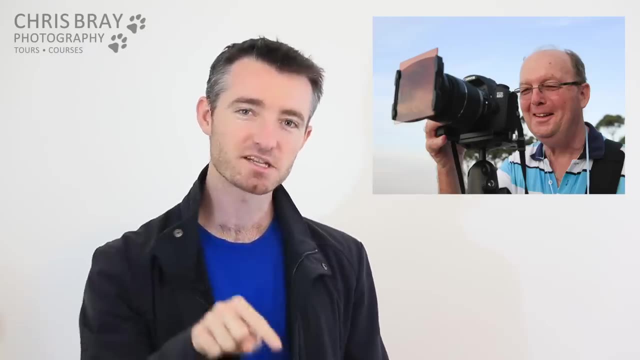 and too expensive, and you'll never bring it with you anyway. Now, even if you've got a tripod, sometimes you'll find these long exposures are still blurry, And normally what's happened there is you poked the camera. It's you pressing the button that started the whole thing wobbling. 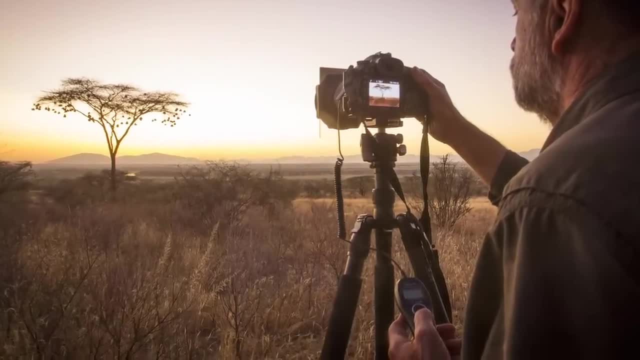 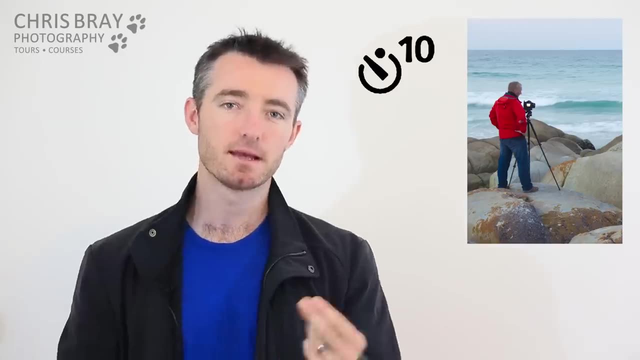 So you could use some fancy timer remote, But you're better off just using the inbuilt self timer you've got on your camera. You know that ten second countdown, beep, beep, beep, and then it takes the photo. If you're ever using your camera on a tripod, you may as well turn that delay on. 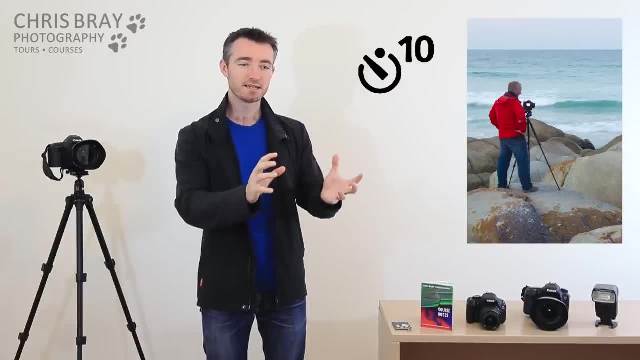 It just means you can press the camera all you want and it'll wobble a little bit, But after ten seconds it'll be perfectly still and it'll take it for you. Also, it's a good idea if you're shooting on a tripod and you know, everything is nice and 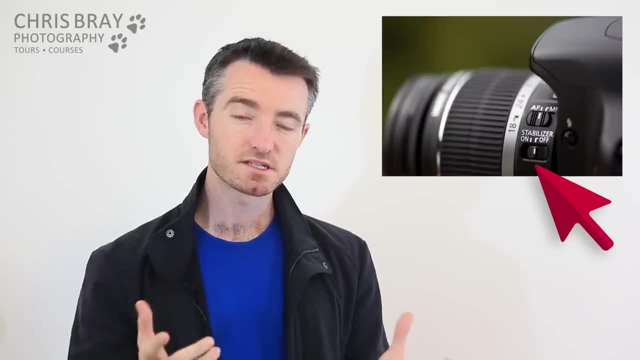 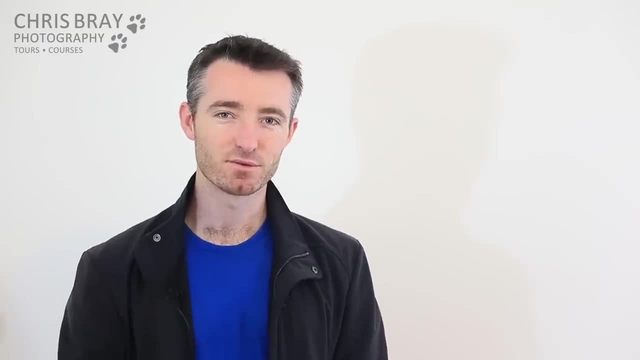 stable, you should turn the stabiliser off on your lens, Because some stabilisers actually end up introducing camera shake if the camera is really steady, So turn that off. Just remember to turn it back on again afterwards. Let's have a look at the different drive modes you might have in your camera. 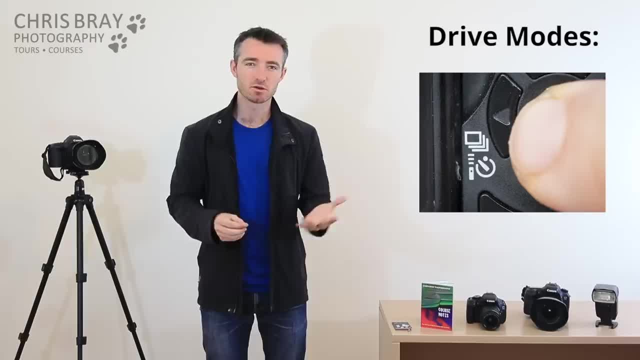 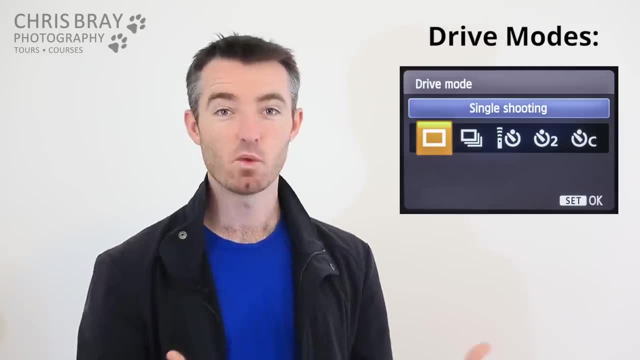 So you either have a button that's called drive or a button that has these kind of symbols next to it, or you'll find your way there. But you get options like these ones: Single shooting- that's what you normally want. That's when you press the button once and you get one picture. 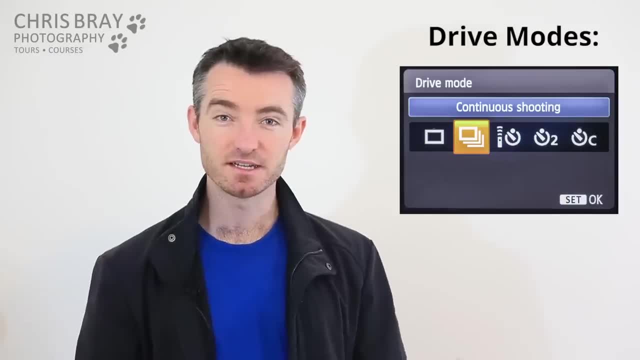 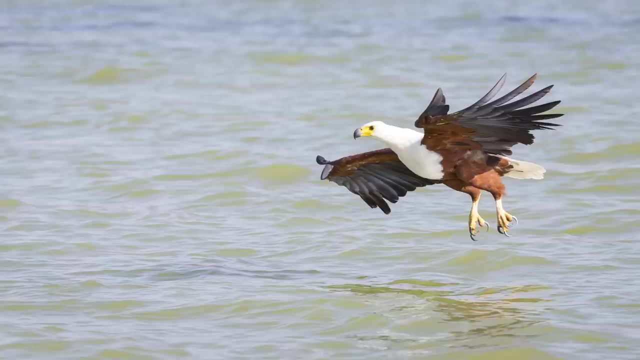 That's normal. Or you've got rapid fire, continuous shooting, high speed, continuous- And that's when you hold your finger down and the camera just takes as many photos as it can, as quickly as it can, until you take your finger off. 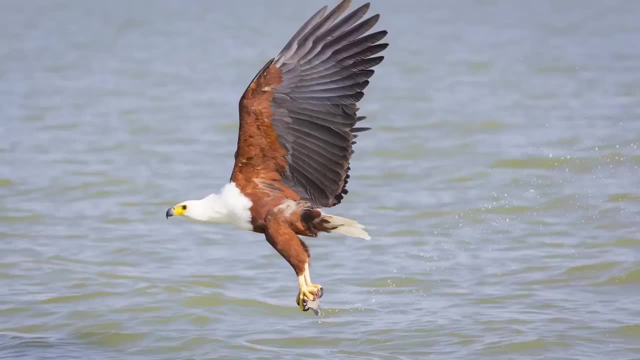 And that's good for a situation where there's something rapid, Something rapidly happening in front of you and you don't know quite when to get the perfect moment. So you just leave your finger down and get all of them and then go back and hopefully. 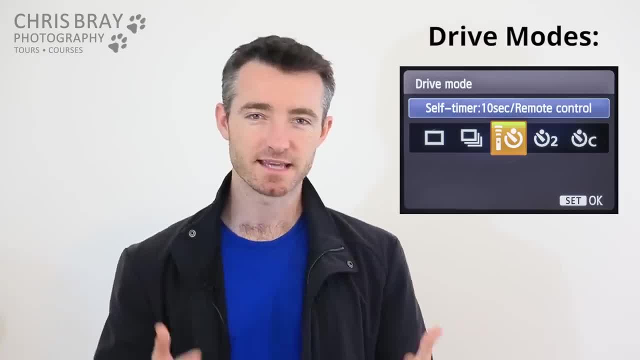 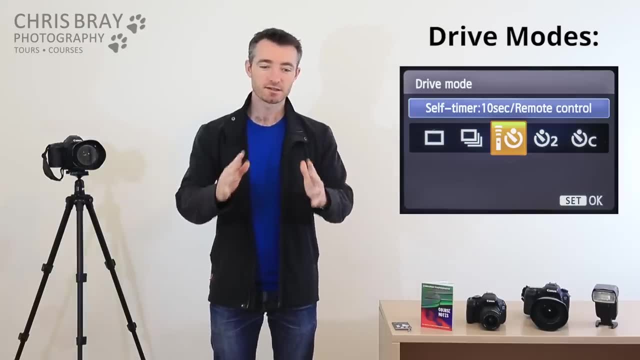 find the perfect moment in there somewhere. This one is the 10 second delay, the countdown timer, Normally good for with your friends so you can run around and stand and be part of the photo, But, as I said, it's also good for if your camera's on a tripod to keep it nice and steady. 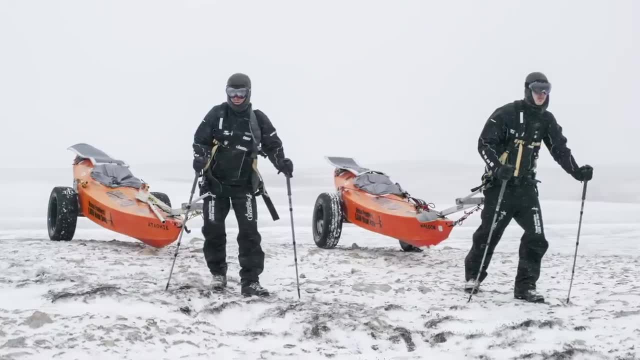 so it's not wobbling anymore by the time it actually takes the photo. Funny story: getting this photo though up in the Arctic. So I didn't have any fancy timers with me or anything during that trip. All I had was 10 seconds. 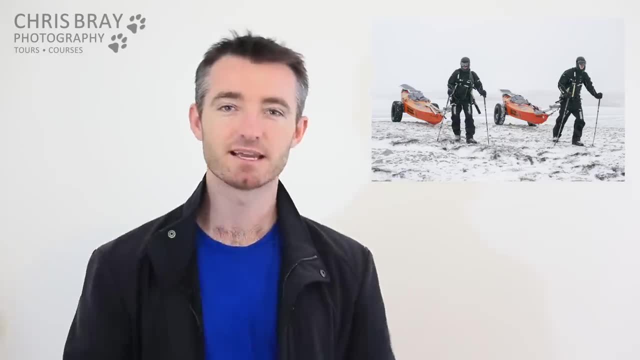 To run around from behind the camera, pick up my hiking poles and pick up the harness and make it look like I just hauled the kayak up the hill. I actually had to take this photo 7 times because the first couple of photos were of 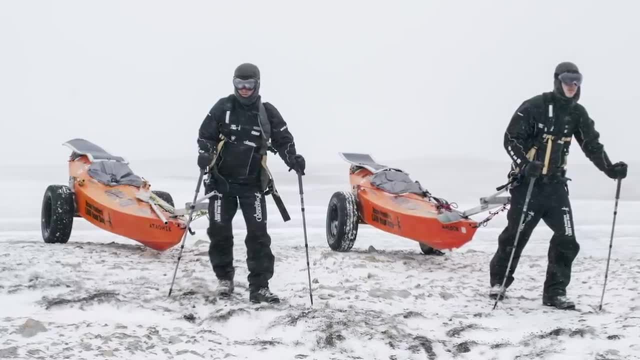 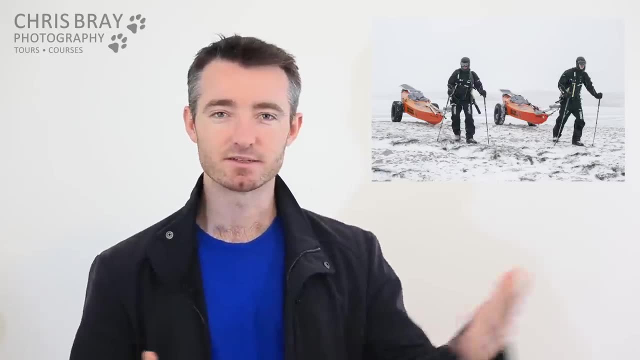 me just sprawled on the ground somewhere, slipped over. you know, it's just ice. When we actually finally got home, I did talk to Canon and say: why don't you make a variable time limit on these things, like out to a minute or longer where you could calmly walk? 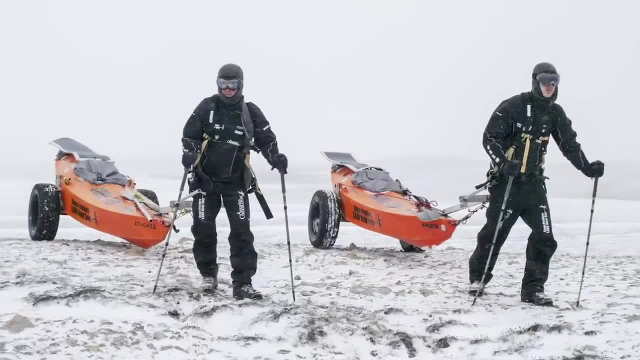 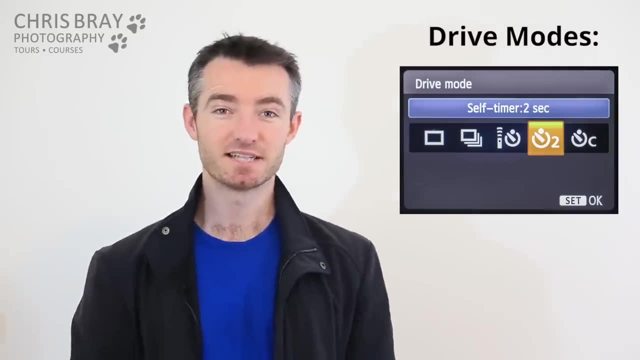 into the distance of your own photo And they basically said: yeah, but then no one would buy any of our little timers, would they? So that's the two second mode, which is actually five times less useful than the 10 second one. 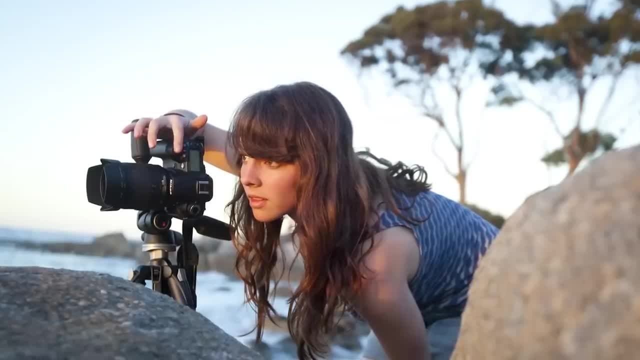 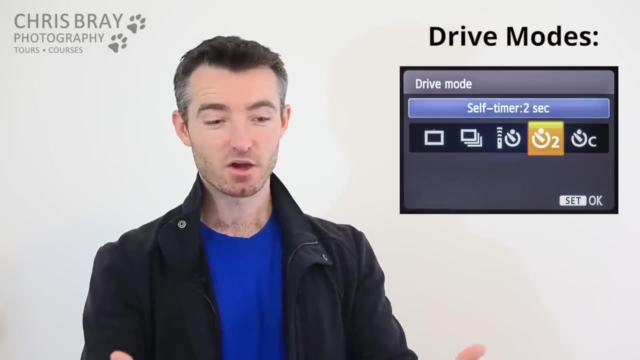 But I gather it's more useful for when the camera is on a tripod and you want to press the button and step away. the camera will have stopped shaking after about two seconds, So it saves you a little bit of time. And, yeah, I guess it's good for coastal exposures or something where you're photographing a. 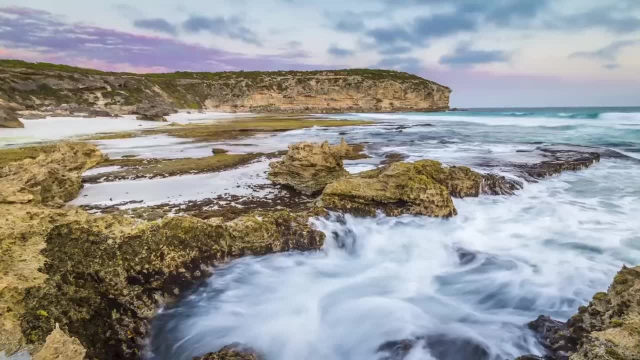 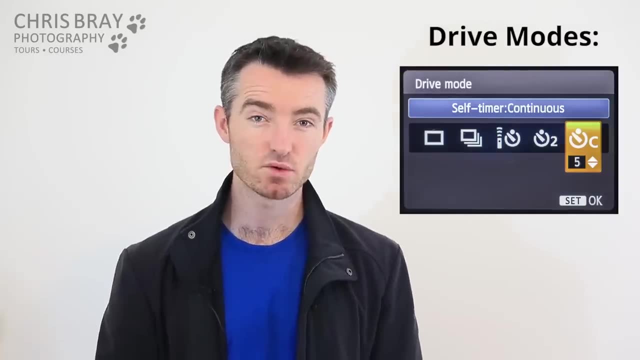 wave coming over a rock. It's hard to predict 10 seconds out when the wave is going to come, So two seconds are a little bit easier to use, but it's basically for when the camera is on the tripod. Some cameras have a self timer continuous mode, like this one. 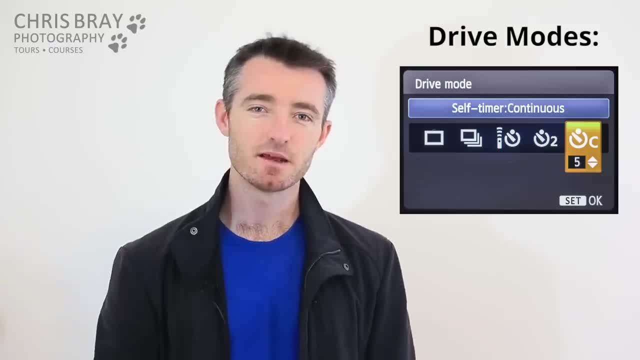 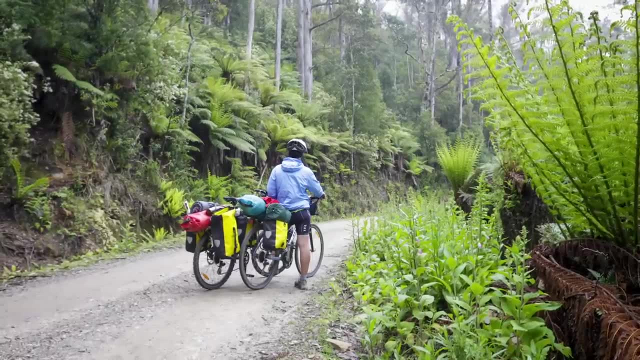 It looks like a variable time limit, but it's not. You're still stuck at 10 seconds, But that's the number of photos it'll take after 10 seconds, normally with a one second gap between them. So that's useful in a situation like this, where maybe Jess can hang on to the bikes. 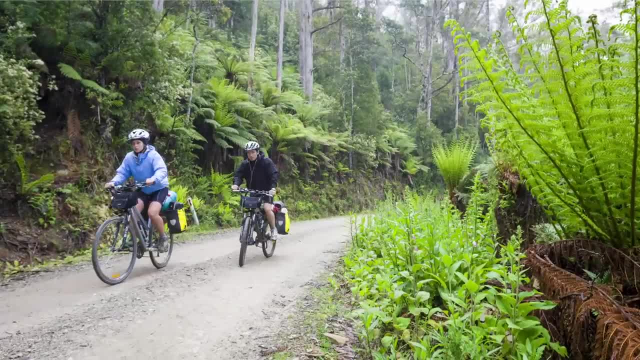 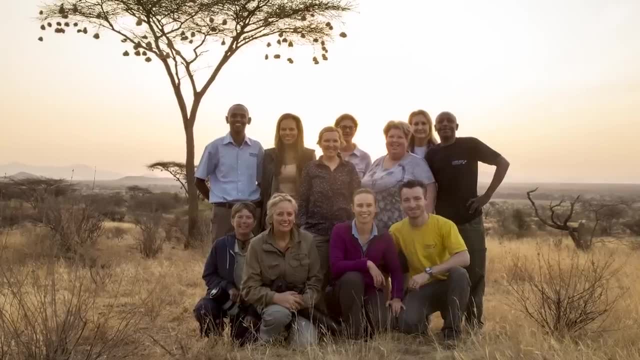 I can set the camera up, press the button, run back and then it'll take a bunch of photos as we slowly cycle towards And then you can go back and pick the best one, Or more commonly useful, for a group photo. Normally you take a group photo, then you have to run back and check and then you find 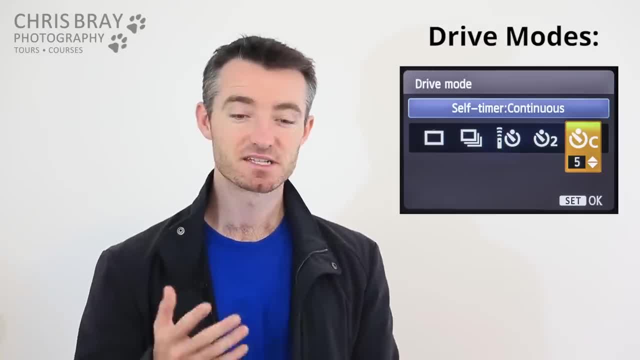 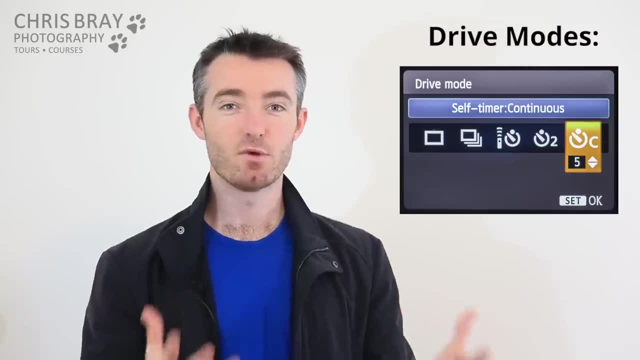 out that someone was blinking and you have to go back and do it again. So instead You just tell it to do the 10 second delay. you run around and join your friends and then it'll take a whole series of photos afterwards and hopefully one of them everyone's eyes. 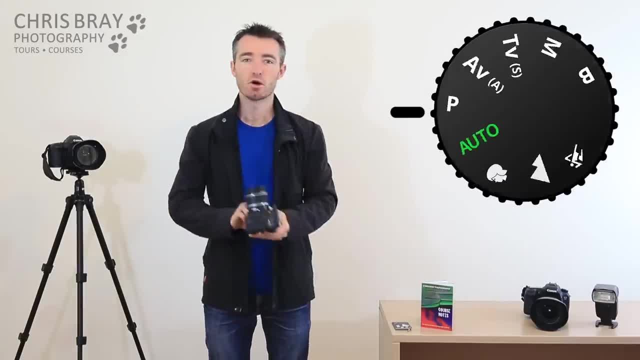 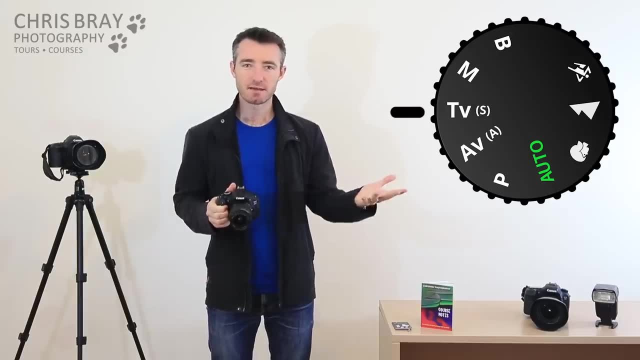 are open. Okay, let's have a look at time value mode, TV mode on a Canon or S mode for every other brand, And in time value mode you can choose whatever shutter speed you want and the camera works out the aperture to go with it. 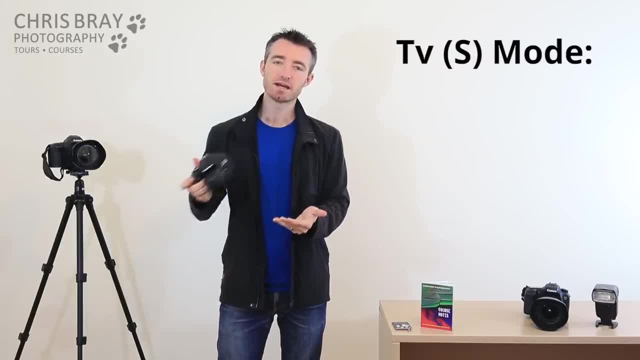 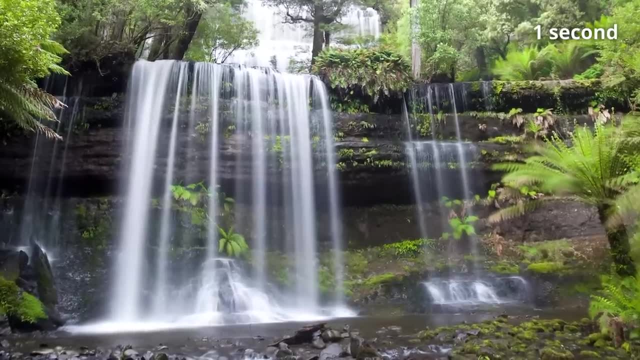 It's just like the opposite of aperture mode, So you'd be using TV mode or S mode when getting a particular shutter speed is what's creatively most important to your photo. So maybe you really want a one second photo to get that waterfall, Or maybe the most important thing is to have a four thousandth of a second photo to be. 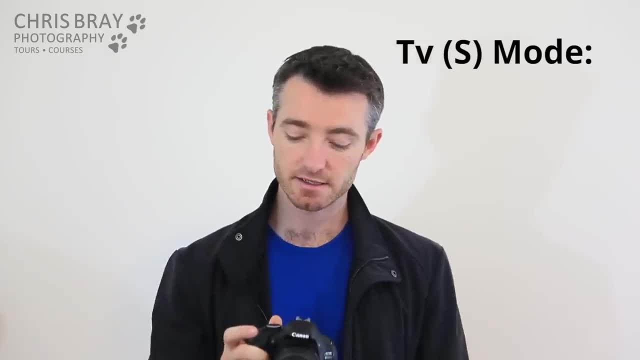 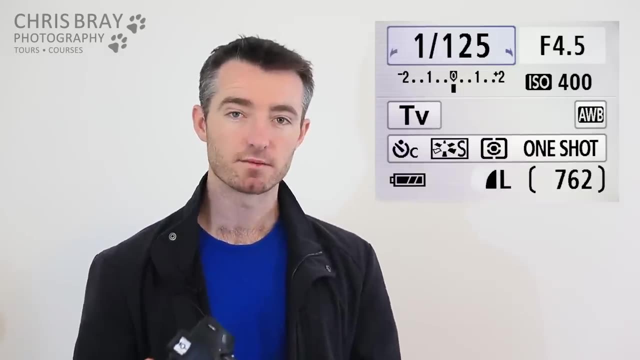 able to freeze a bird or something like that, And it works just like you'd expect. You touch the button, the camera wakes up and it starts with the last shutter speed that you used and you can scroll around and pick whatever value you want. 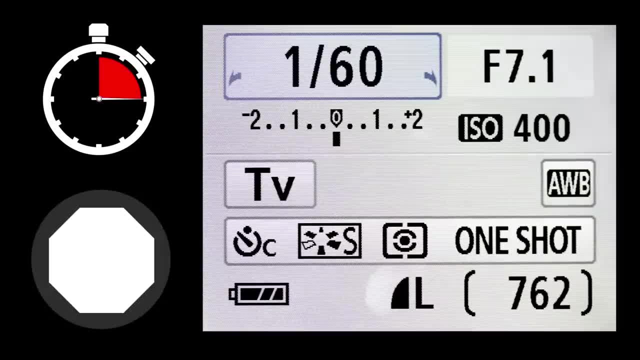 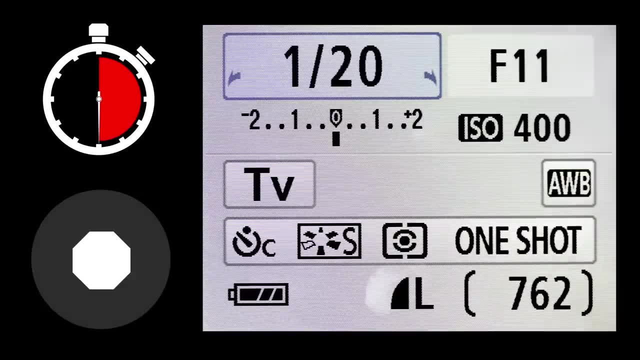 You can see, here we're scrolling to slower and slower photos and to prevent more light coming in, the camera's automatically using smaller and smaller holes for us at the same time. But you can see, we're going to run into the same kind of limit in the end that the camera. 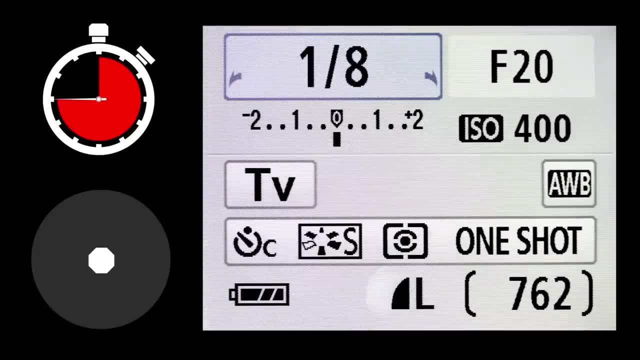 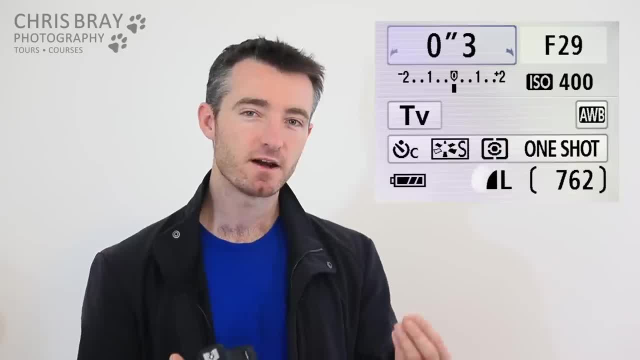 just can't make the hole any smaller after a while. So as we ask for longer and longer photos here, sixth of a second, 0.3 of a second- that seems to be okay, But if we try and go any further, you find the camera just can't shrink down that hole. 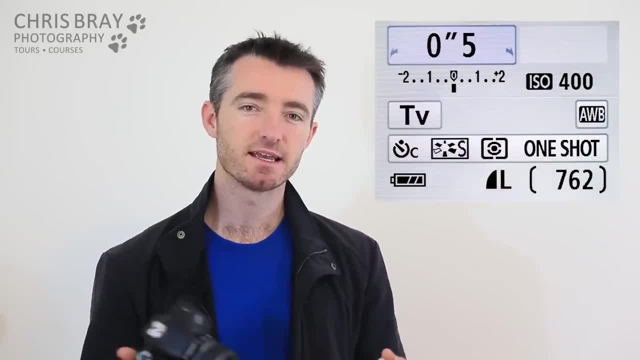 anymore, so it can't stop any extra light coming in. So then you're going to get into that same situation we saw in the aperture lecture, where it just starts flashing warnings at you saying: you know, the value you're picking is inappropriate for the current lighting condition. 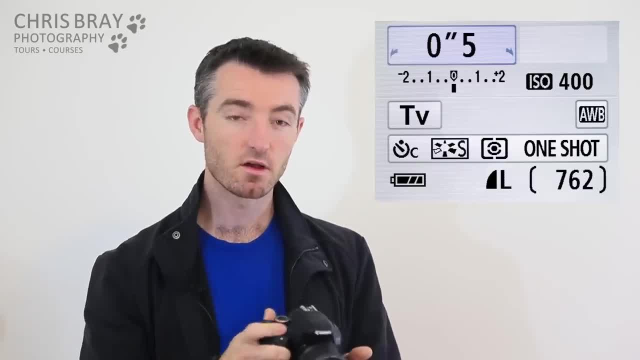 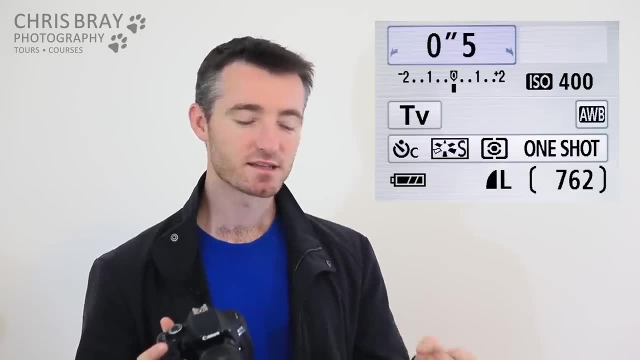 But again, it won't stop you taking the picture. So if you really wanted to, you could scroll all the way to 30 seconds or something during the day And it will try and warn you. but if you ignore those warnings it'll just take a full 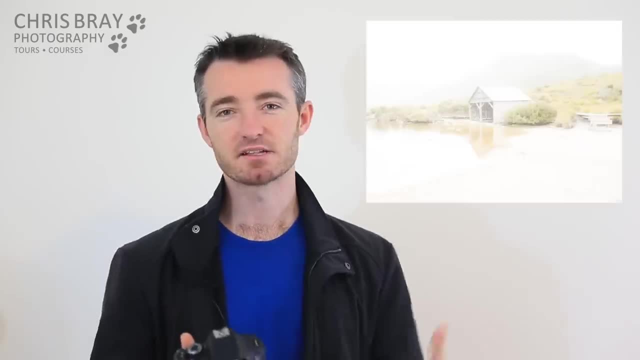 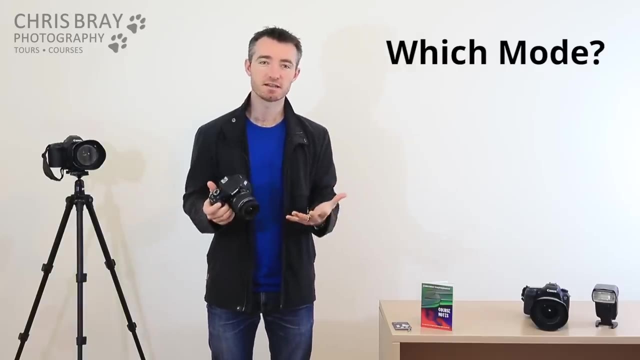 30 second photo for you and it'll come back and it'll just be massively overexposed. So just watch out for those flashing warnings again. And just a reminder: you can always get to the same photo, exactly the same settings. 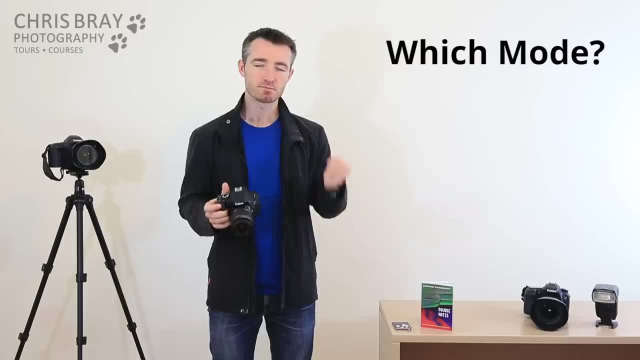 on any of these other modes, like aperture mode. it's just which variable do you want to make sure you keep at the same value? If you really want a particular shutter speed all the time, then you'd want to be in shutter speed mode. 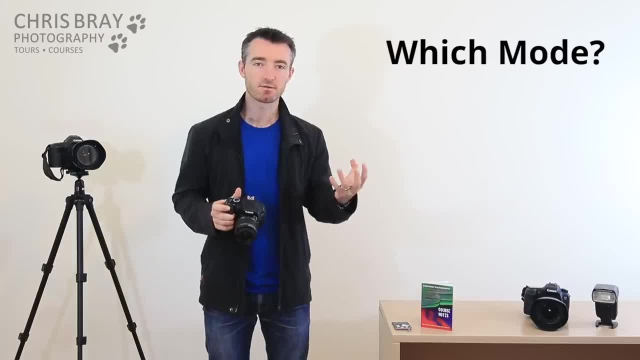 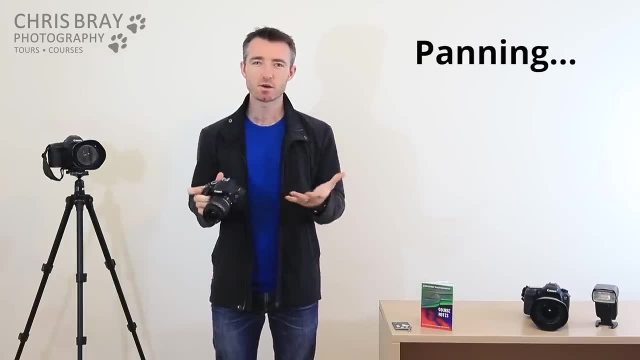 If the most important thing was to have a particular F number the whole time for a certain depth of field, Just stay in aperture mode. So some cool tricks with longer shutter speeds. The panning shot is a good one to practice. That's where you want to show movement in a subject, but rather than just holding the 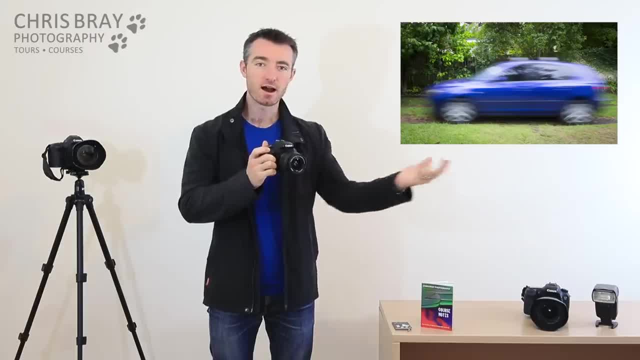 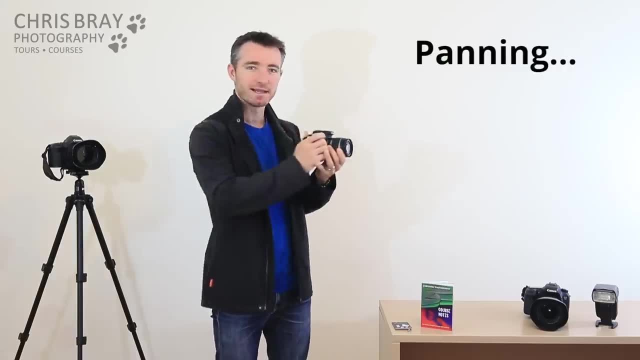 camera steady and having a long shutter speed and letting your animal or your car, or whatever it is, move past, because that wouldn't look very good. you'd just end up with a blurry subject. Instead, you can actually follow the subject with the lens as it goes past. 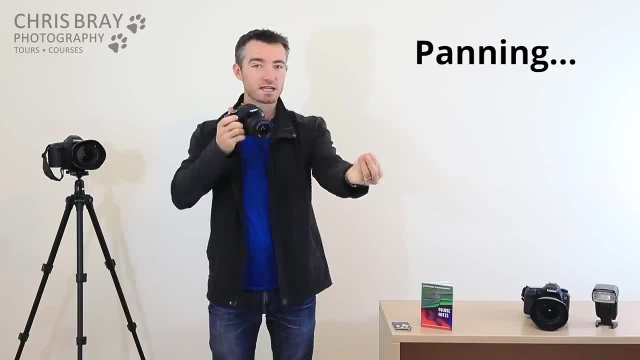 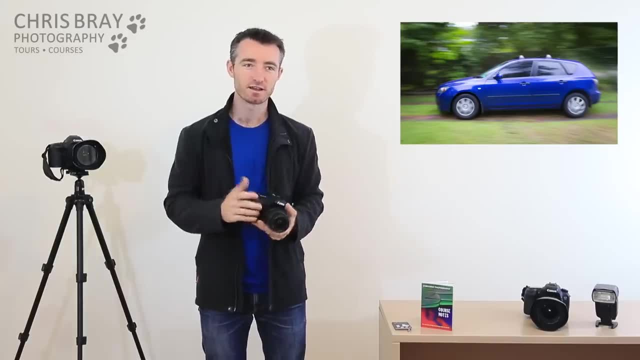 And if you can keep your subject in exactly the same part of the photo, it stays nice and sharp, but the background click becomes blurred and streaked past. It's a much nicer way of showing your subjects moving than having a blurry subject. 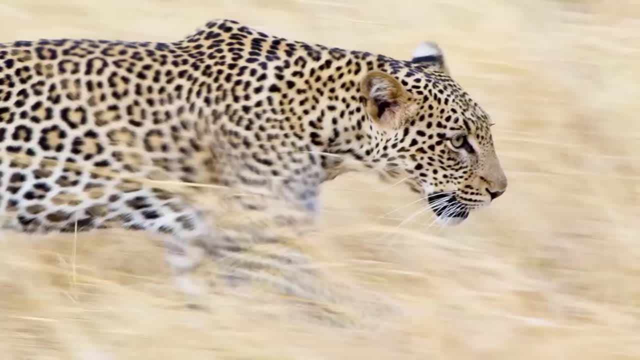 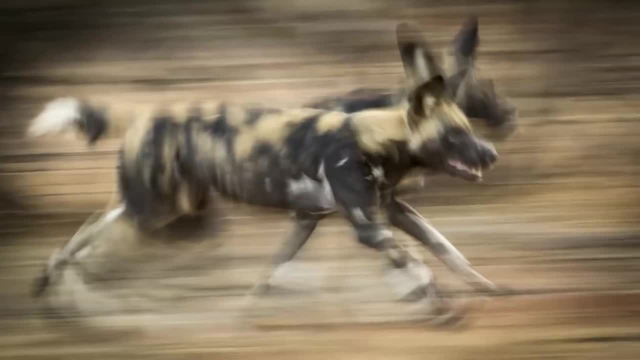 Experiment with different settings, Start off with about a tenth of a second or a twentieth of a second- So that's still fairly slow- And then just look through and follow it as it comes along, click and take it when the animal or the car is right perpendicular in front of you, and you should end up with a. 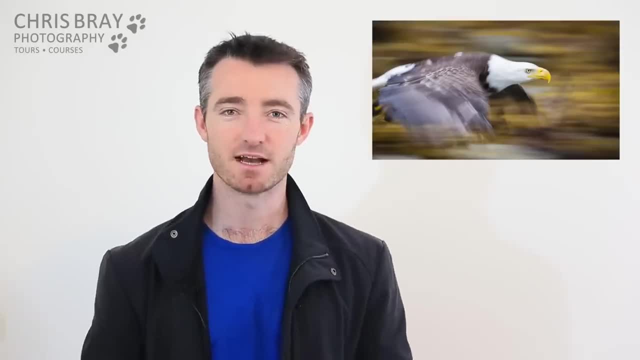 pretty cool result. It's just practice. You'll get a lot better, even in the first couple of times you try The zooming in shot. Try and imagine what your photo would look like if you zoomed in while you were taking the picture. 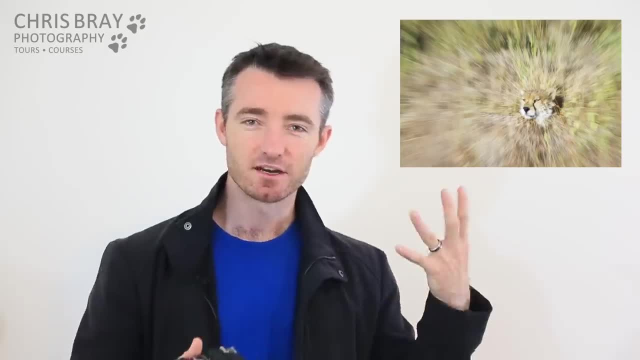 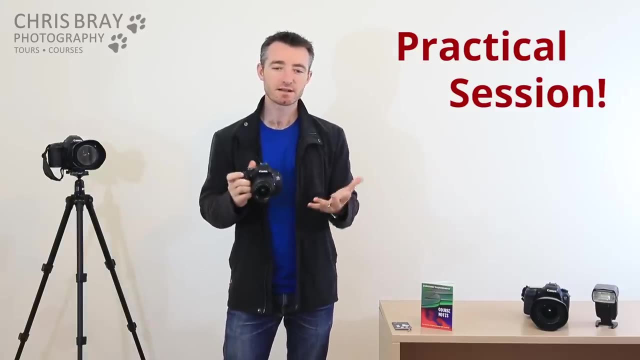 Kind of weird, But it is kind of cool. It creates all these leading lines, kind of pulling your attention into the subject, which can be a nice creative effect. Now for our shutter speed prac. what you want to do is just go outside and find something. 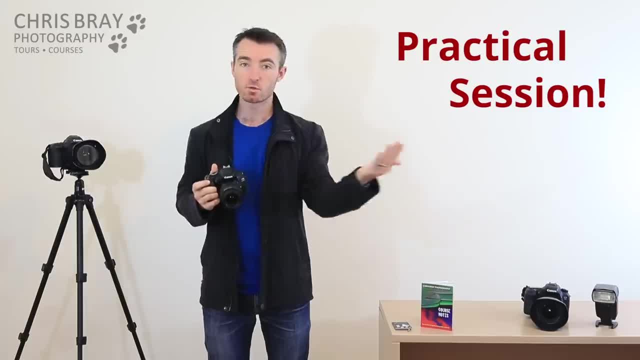 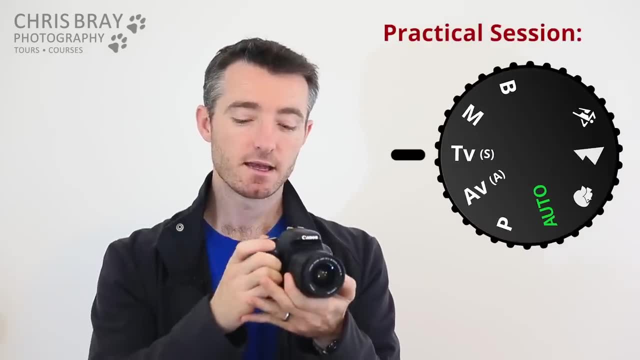 that's moving. You know. it could be a car driving past, it could be a friend walking back and forwards in front of you. Ideally it might even be a waterfall or a fountain. So then set your camera up on a tripod, ideally, and then wake it up. 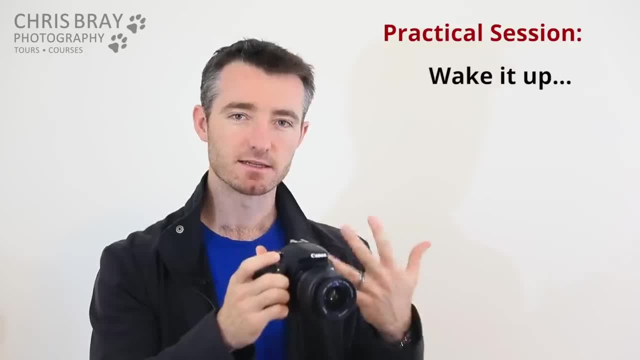 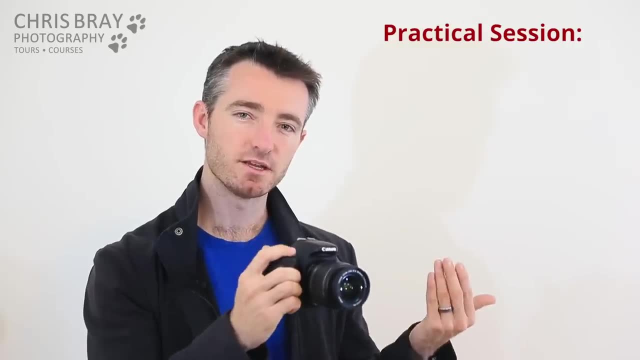 That's an important step. You've got to always remember to wake up your camera so that it's alert and looking at the lighting out there and stuff- Otherwise you wouldn't know if it was trying to flash warnings at you or not- And then try and scroll down to the slowest shutter speed you can. 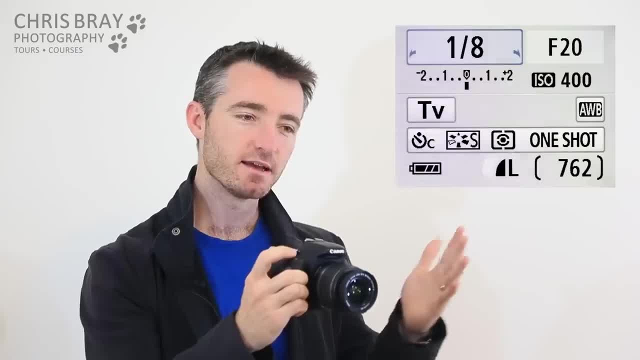 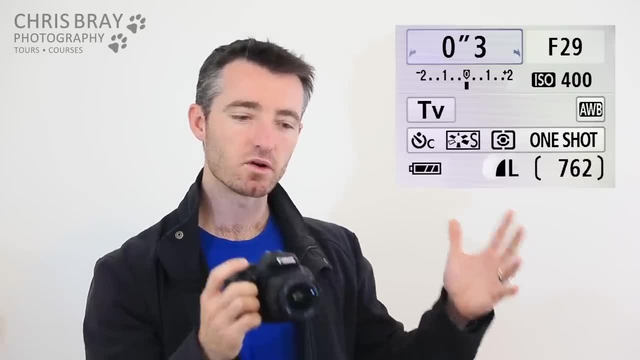 So you wake it up, scroll slower and slower, watching your shutter speed, and eventually you'll get so slow that it'll start to flash warnings at you. So then come back one, and then it should calm down. That's the longest, slowest photo you can take. 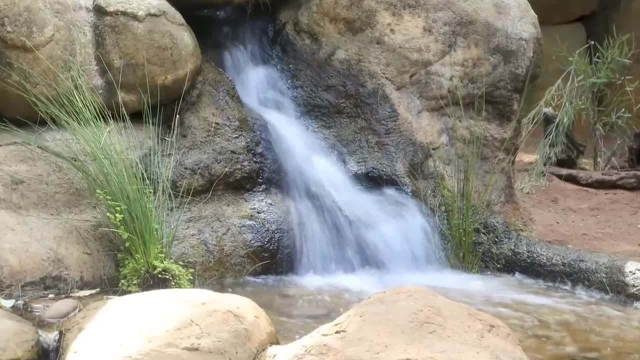 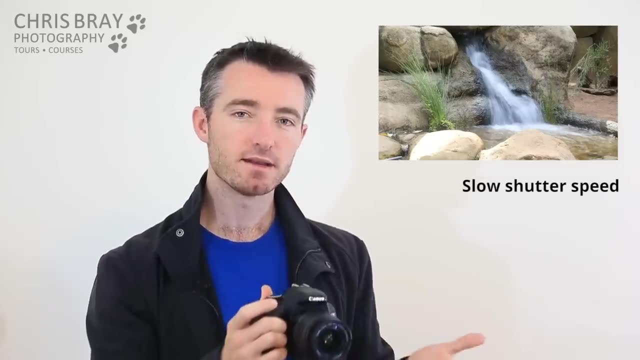 So go ahead and take that one click and you'll probably see that shows the movement in the fountain or the waterfall or the car going past. That'll show movement blur. And then take the same photo again, But now with a fast shutter speed. 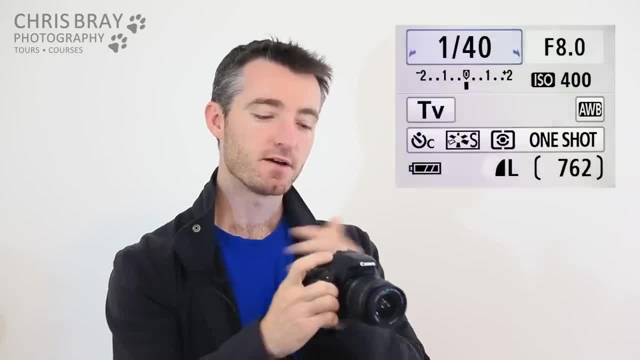 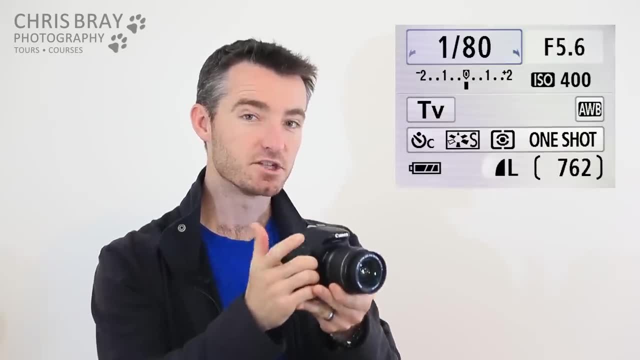 So you'd wake it up and then go the other way, faster and faster, And then finally it'll get too fast. it'll flash warnings at you. come back a bit. okay, Then that's the fastest photo you can take in that situation. 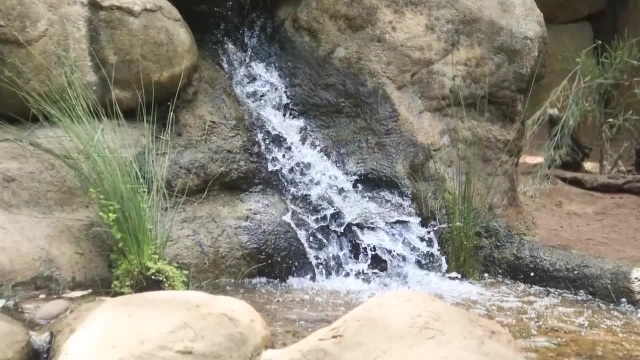 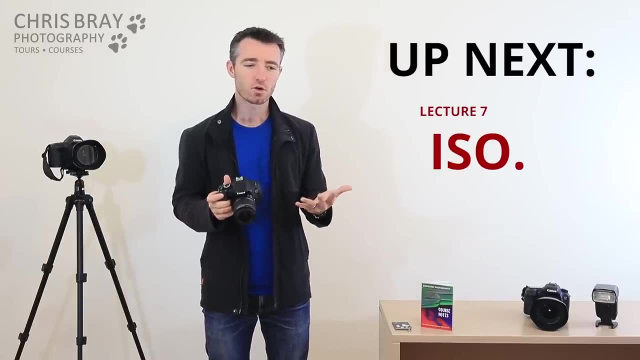 So take it and you should find that the movement has been frozen, or at least less movement has occurred Now, because we haven't really covered ISO yet. that's in the next lecture coming up. for now, just put your ISO on a middle sort of value, like ISO 400, that'll be fine. 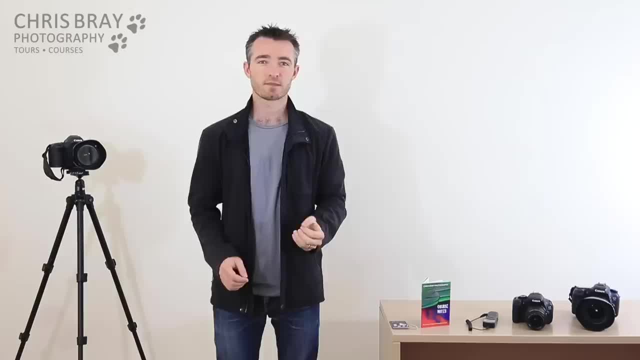 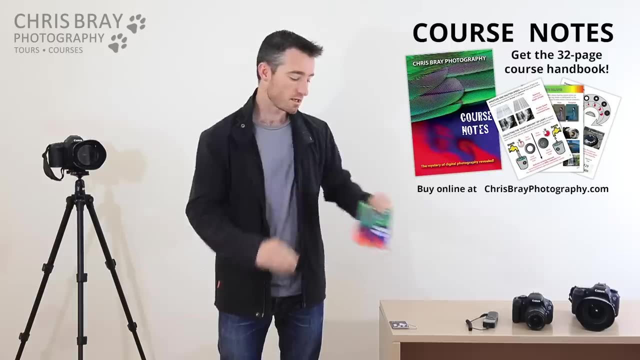 Okay, we better have a look at ISO and how that all fits together. And just a reminder: there's an ISO section in the booklet that goes with this course, as well as a little summary set of plastic clip cards. got a handy little reference there. 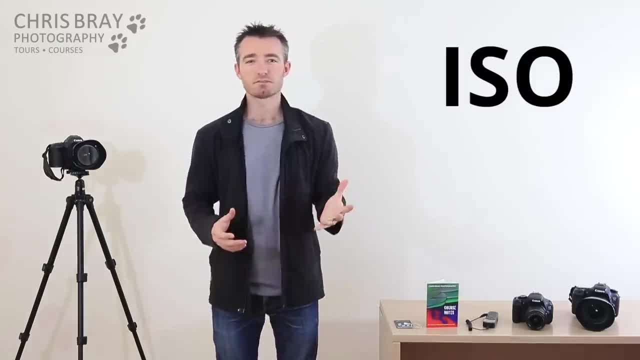 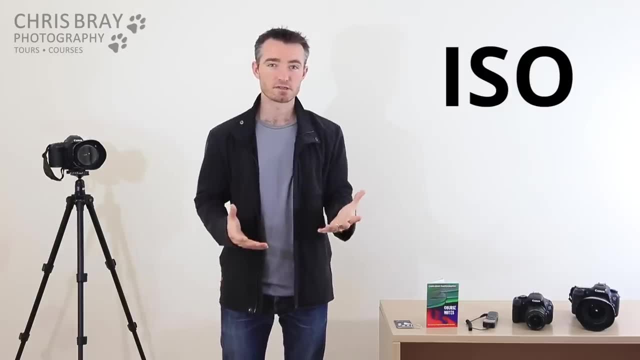 if you ever forget any of these key tips. So ISO is basically a variable setting for how sensitive your camera is to light, how much light it needs to collect to be able to give you a correctly exposed photo. Now, ISOs go from about as low as 100.. 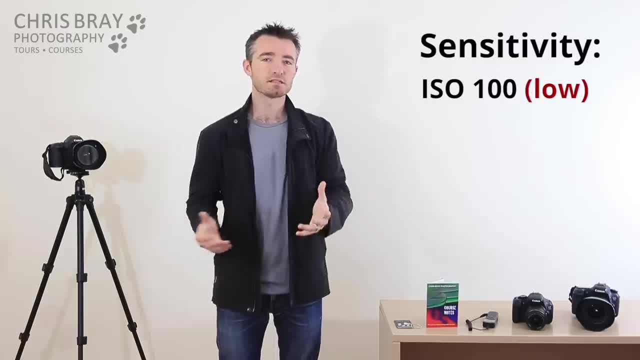 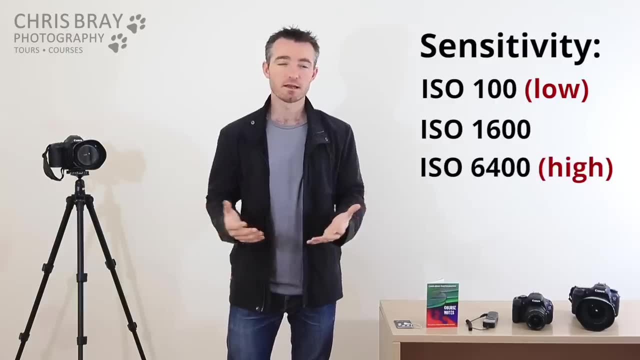 That's a fair bit. ISO is a fairly low value. unsensitive- that means it needs to collect an awful lot of light to be able to get you a picture. Or you could crank your ISO right up to 1600, several thousand, and then it's very sensitive. 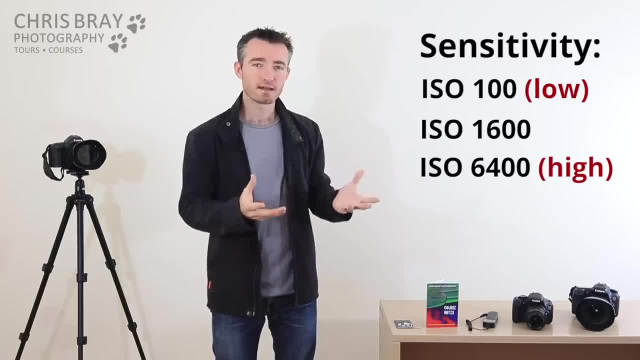 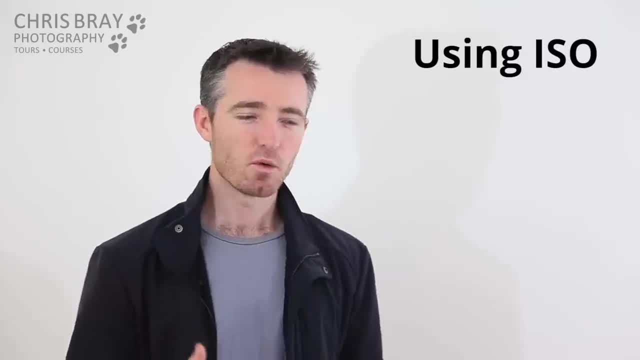 it doesn't need much light at all, even a little brief amount of quite faint light, and the photo's already finished and give you a correct exposure. Now there's all kinds of ways people have managed to get themselves confused about ISO, what it is and how you use it. 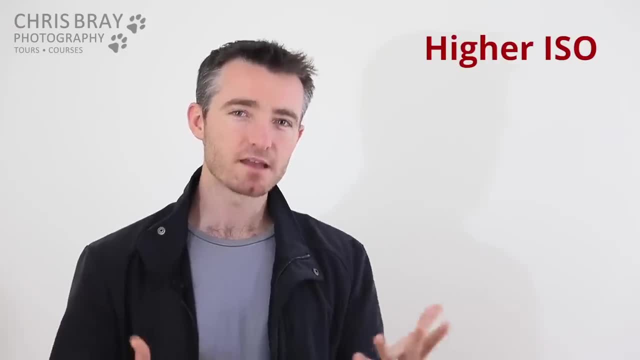 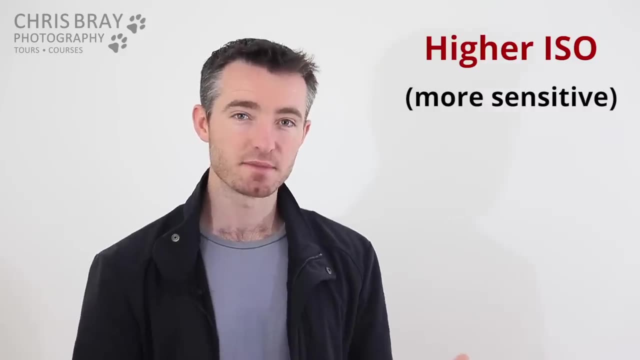 Basically, this is the simplest way to understand ISO. The higher you turn your ISO, the more sensitive your camera is to light, So it doesn't need to collect so much light anymore to give you exactly the same picture. So, instead of having to leave the shutter open for ages and collect this huge amount, 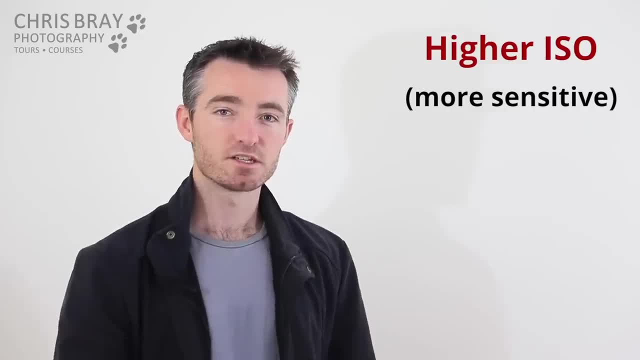 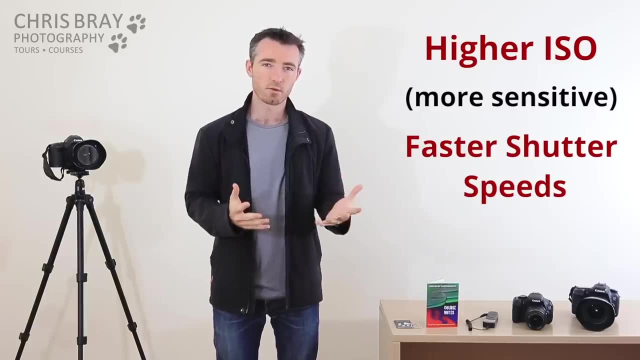 of light. even just the first little bit of light coming in is enough. the shutter finishes, and that means you're able to get faster shutter speeds than you otherwise could. Now that's a real advantage to be able to have faster shutter speeds than you otherwise. 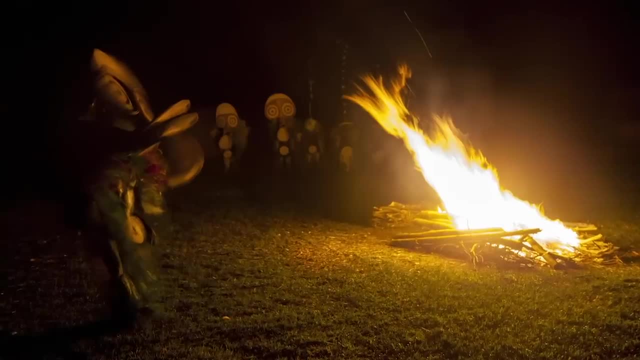 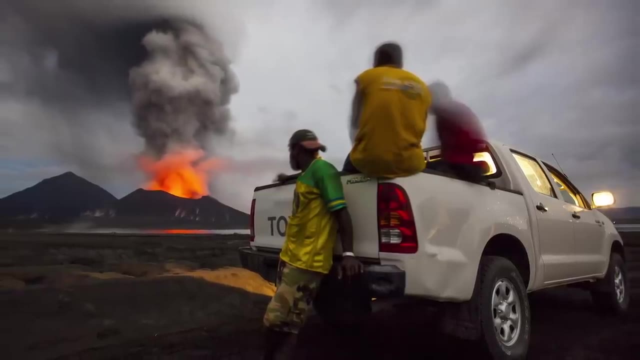 could, particularly in low light, when otherwise the photo's just too long and slow and you end up with a lot of camera shake and you get blurry photos even if you have your camera on a tripod, Whereas you can have a fast photo- great, you can handhold it. no one has moved anywhere. 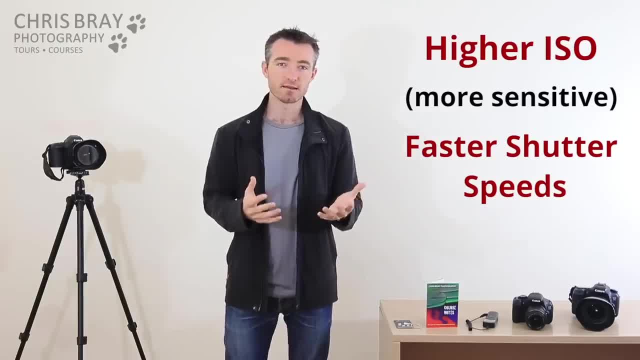 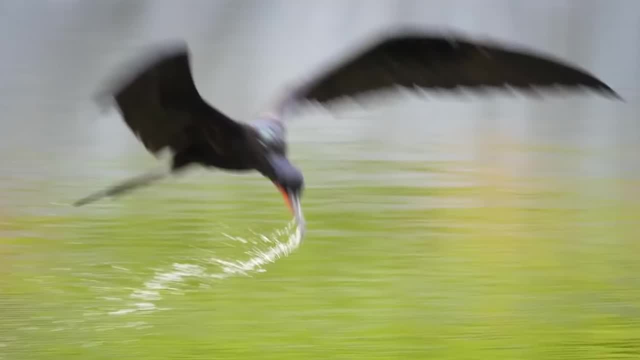 and that's great, Or even just for extra fast photos during the day, Like if you were trying to freeze a bird in flight. maybe the fastest photo you could normally take would be about 500th of a second. That's pretty quick, but it's not quick enough to freeze the wingtips on the bird. 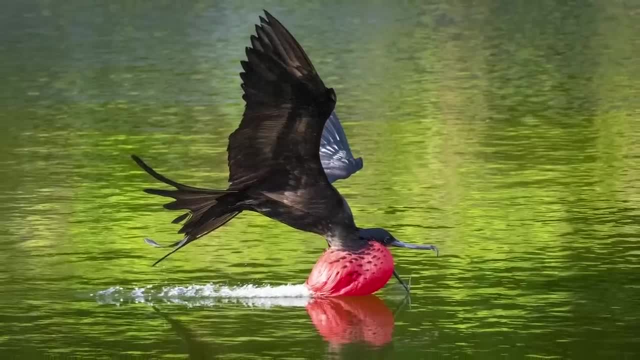 So if you turned your ISO up, you might then be able to take 4,000th of a second and absolutely freeze those wings. It's the same thing if you think about it. by turning the ISO up, we've been able to. 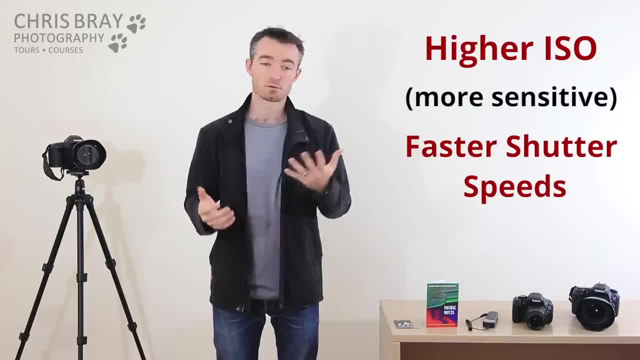 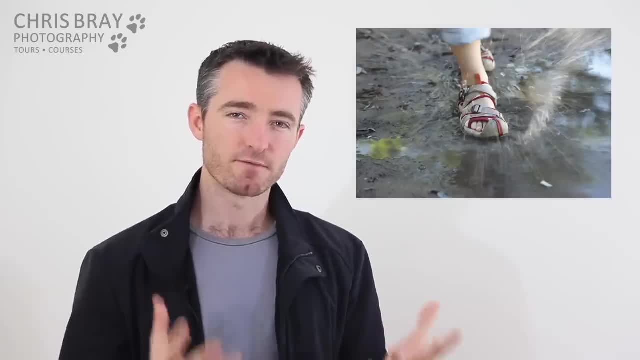 take faster shutter speeds than you otherwise could, either in low light or just because we want an even faster photo during the day. So here's a little example to help that sink in. I wanted to try and freeze these water droplets, so with a very fast shutter speed. 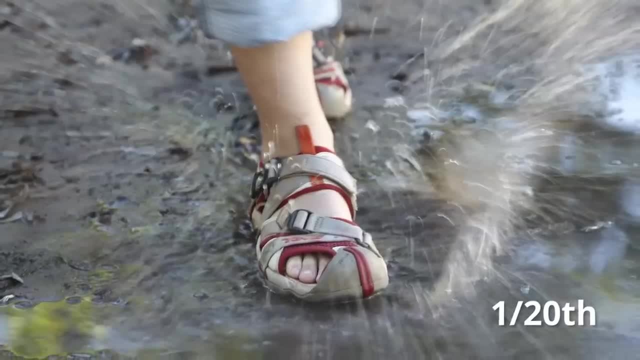 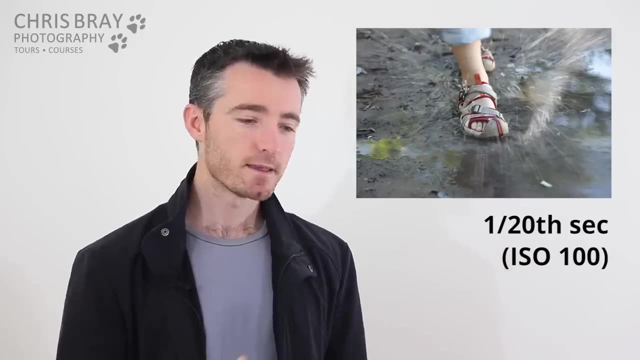 But because it was early morning there wasn't much light around. the quickest photo I was able to take was only 20th of a second. Now, when I say that was the quickest photo I could take if I was in P program mode, 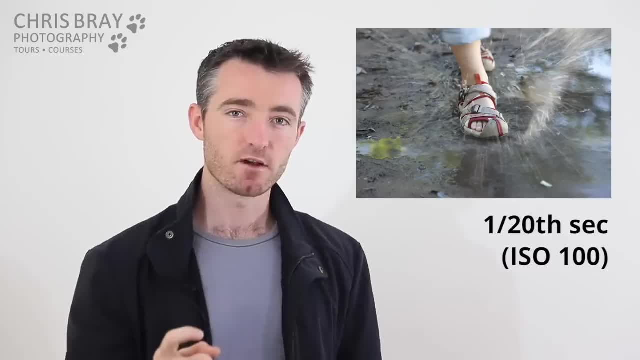 then that means all I could scroll to was 20th of a second and it wouldn't let me scroll any further. Or if I was in shutter speed mode, That means I could happily scroll to 20th of a second, but if I tried to go any faster, 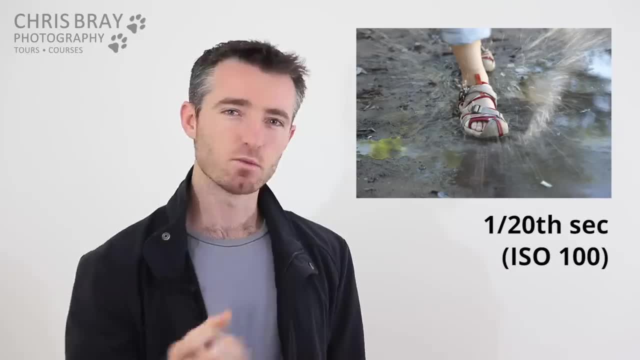 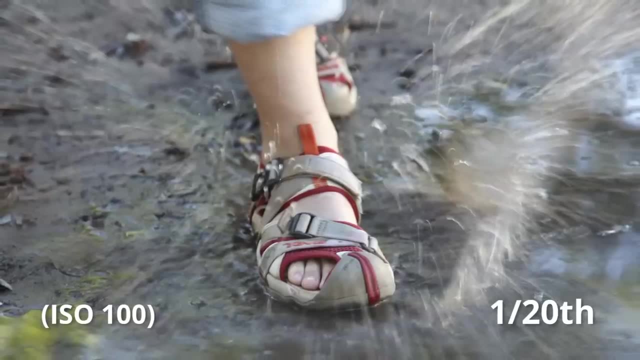 like 50th of a second or 100th of a second. it would have just sent flashing warnings at me saying, no, it would have had to have come back anyway. So, no matter what, I couldn't get a faster photo than 20th of a second. 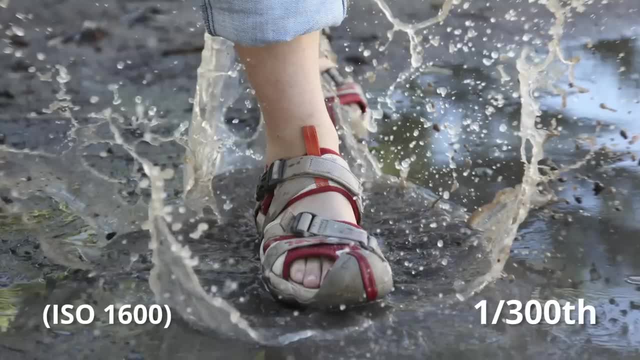 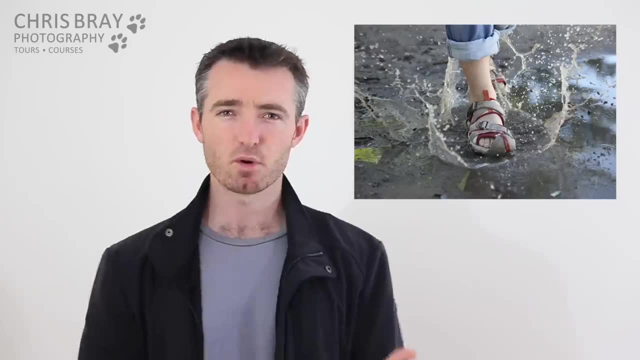 But if I crank my ISO up to ISO 1600, then all of a sudden I'm able to scroll all the way to 300th of a second to get that creative effect. I wanted to freeze the water droplets, But it's important to realize that other than that, the photos look the same. 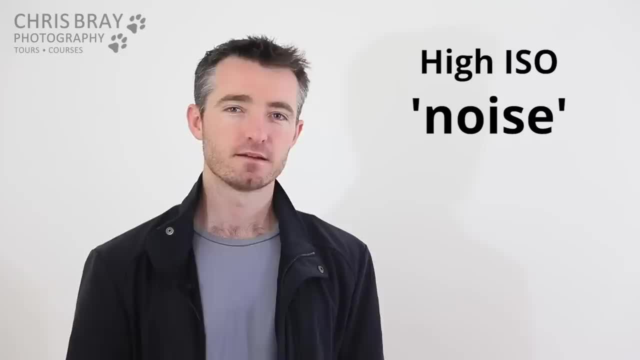 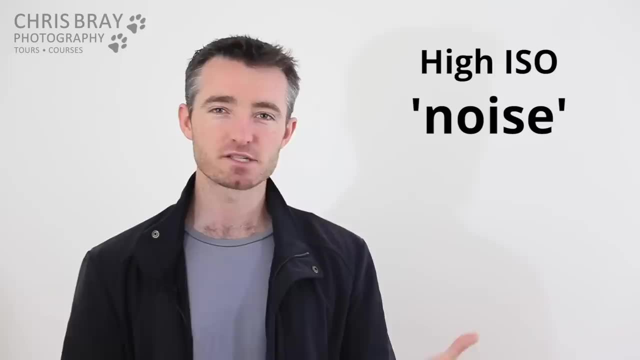 It's just by turning your ISO up You can get away with faster shutter speeds. Now, if you crank your ISO too high, you do have the downside of losing a little bit of quality in your image. It's called ISO noise. The same thing used to happen with film, due to a totally different reason, but it looked. 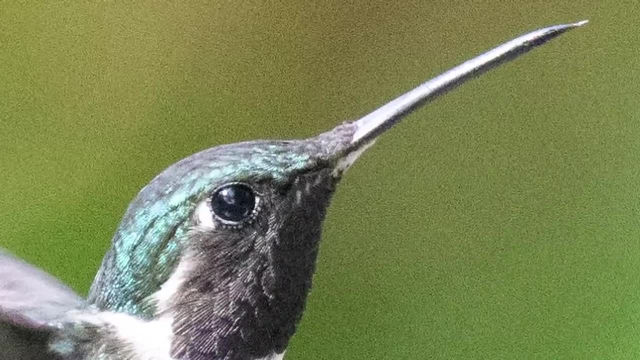 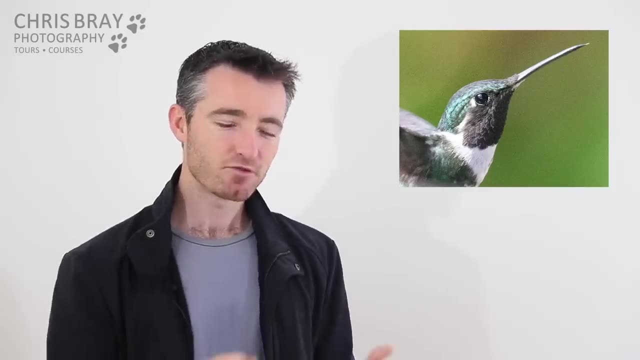 similar. When you zoom right in on an image, you see it looks a bit gritty and grainy. You get these kind of random speckles of color. Now, this is nothing like as big a problem as people make it out to be. 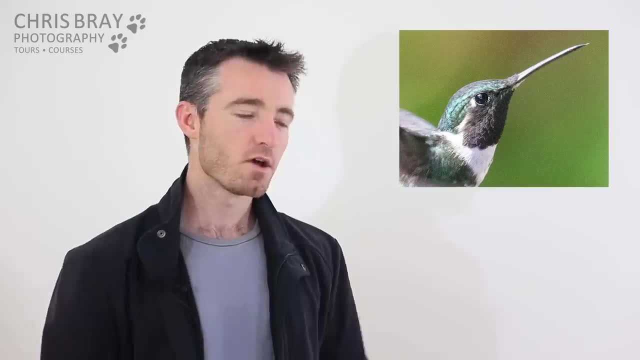 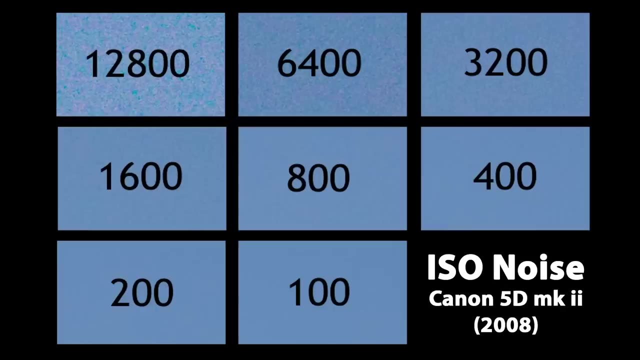 You really only see ISO noise if you zoom really a long way in or if you blow the picture up really huge. Let's take a look at a series of photos. This is taken of the same patch of blue sky at different ISO levels, and you can start. 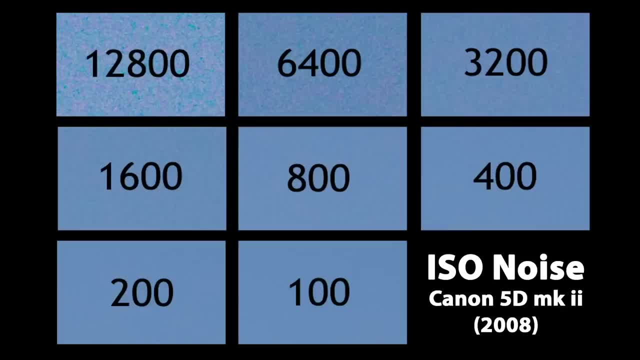 to see: the higher you crank your ISO, the more we're starting to get these random little speckles of color in there. But this technology is getting better and better all the time. This example is a Canon 5D Mark II. 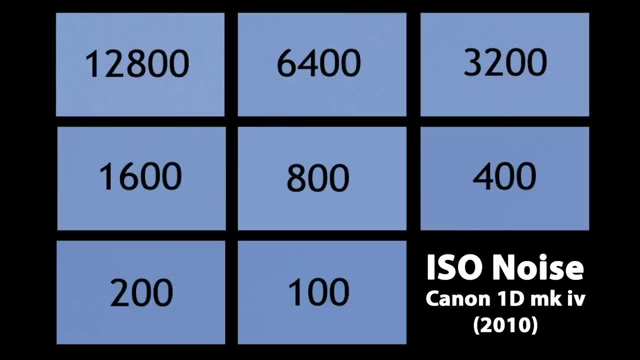 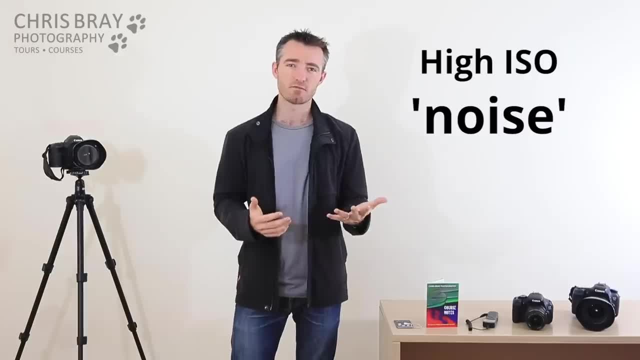 That's ancient in terms of cameras. So the same example again now with a 1D Mark IV. So even that's a good couple of years old, And now you can see the ISO is much better. Unfortunately, you still have people going around saying, oh no, don't turn your ISO. 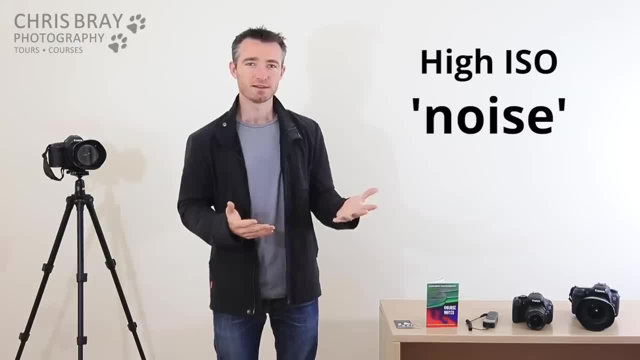 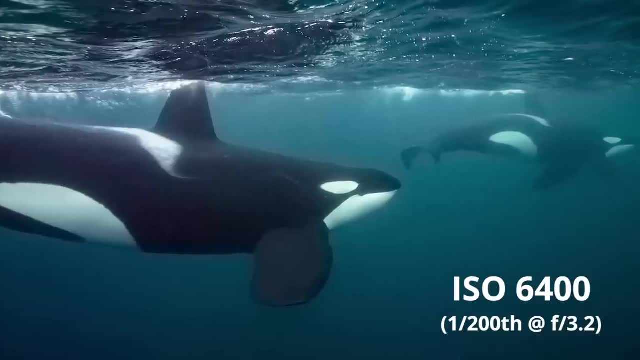 up At 800, it'll be unusably noisy. It's just completely not true. These days you can crank your ISO to ridiculous values and you can. it basically unlocks photos that were previously not even possible. I'd much rather have a little bit of speckly noise in my photo because I've used a bit 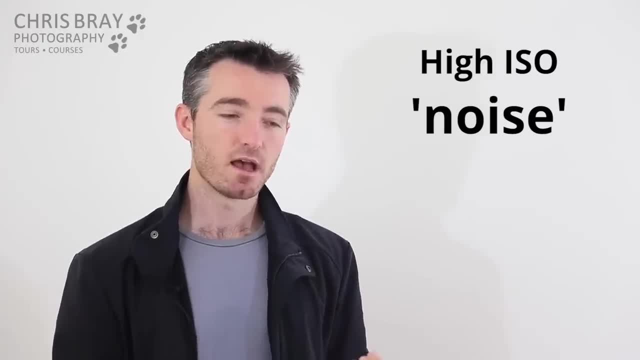 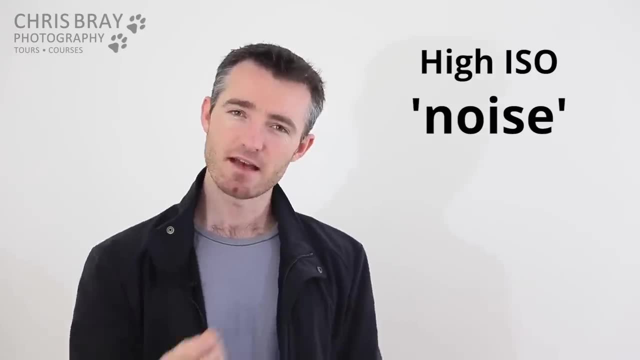 too high ISO than not having used high enough ISO and end up with the shutter speed being too long and slow and have a blurry subject. You know, a blurry subject is really obvious and it ruins the shot. Having a little bit of ISO noise. it's not the end of the world and, in fact, post production. 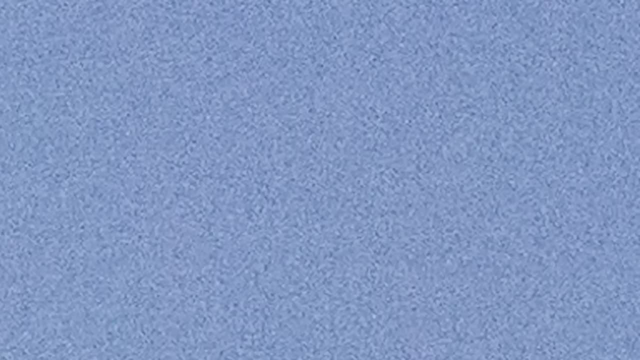 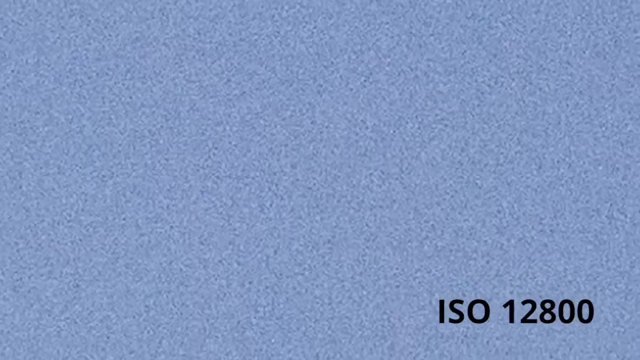 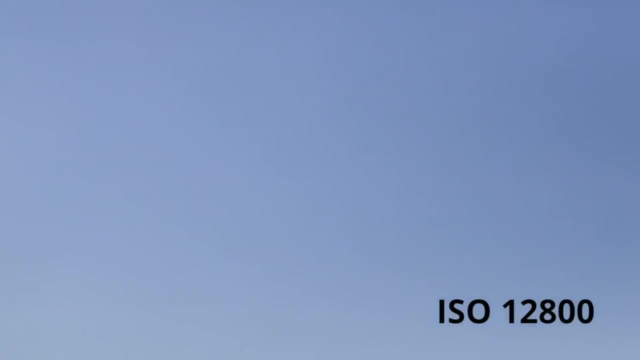 is getting better and better. Let's zoom out this photo. This is the example photo of the really ancient camera, the 5D Mark II, at the 12800 ISO, which was the worst that camera was prepared to offer us, And by the time you zoom all the way out, it just looks nice uniform blue sky. 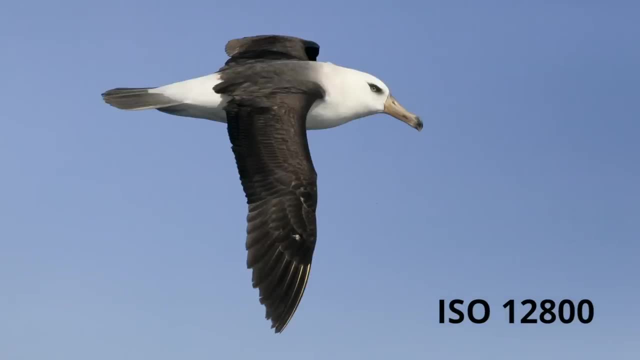 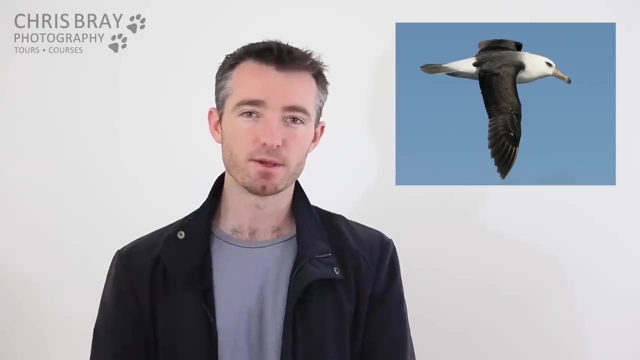 If that was a full frame photo of a bird, that would be fine. So I actually err on the side of safety by having slightly too high ISO than too little. Now, all this has been about turning your ISO up to help you get faster photos, but the 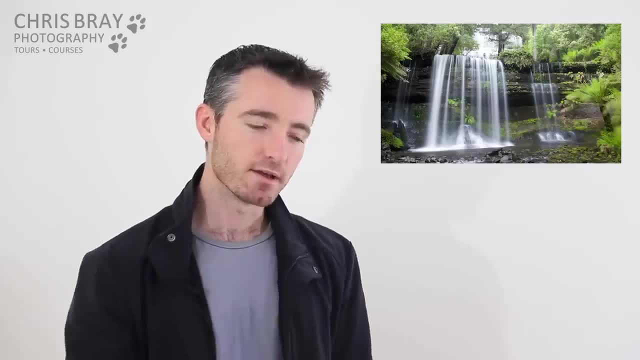 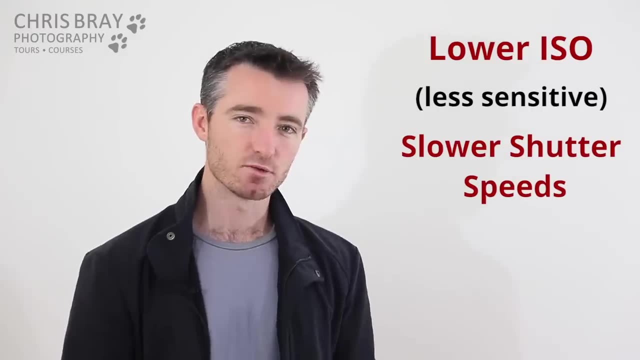 reverse is also true. If you wanted to slow your shutter speed down and get really long slow photos with lots of flowing movement in there, it helps to turn your ISO down. So if you dropped your ISO down to ISO 100, something like that, you'll find you might. 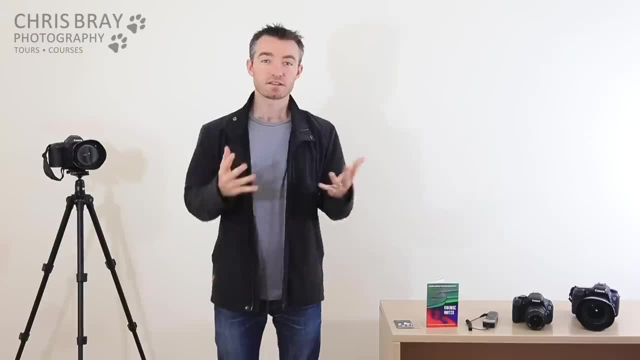 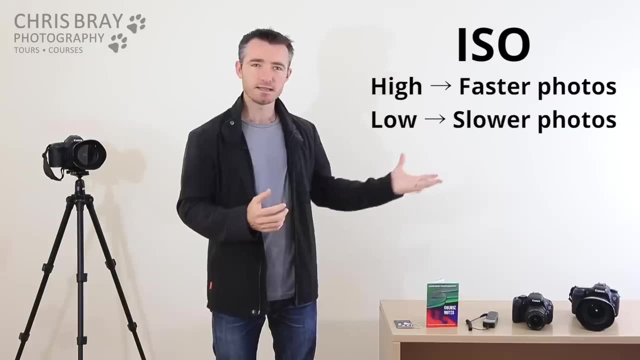 be able to access much longer slower shutter speeds than you could before. So the take home point for ISO, if you like, is basically to treat it as an extension tool for your shutter speed. It's something you can completely forget about and ignore, really, until you find yourself. 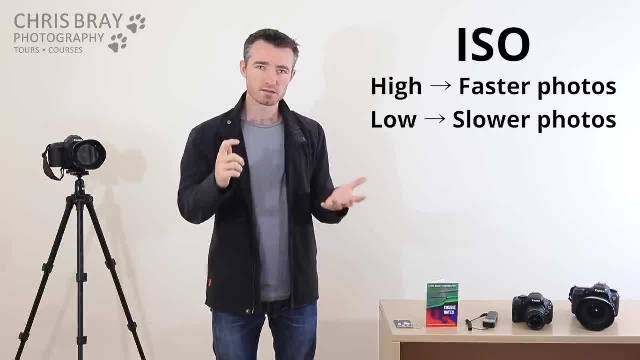 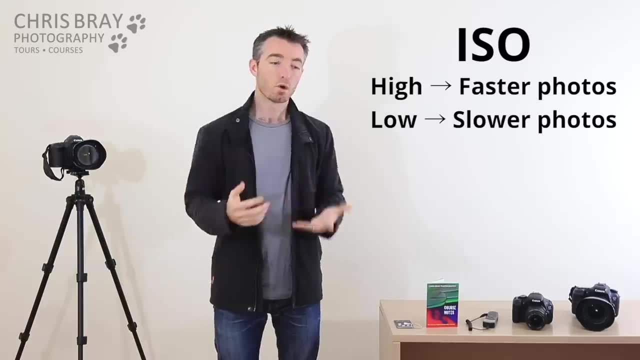 going. gee, I just can't get a fast enough photo. You know the bird's way too fast. The wings are still blurry, or whatever it is. then, oh, turn your ISO up, then you'll be able to access much faster photos than you could before. 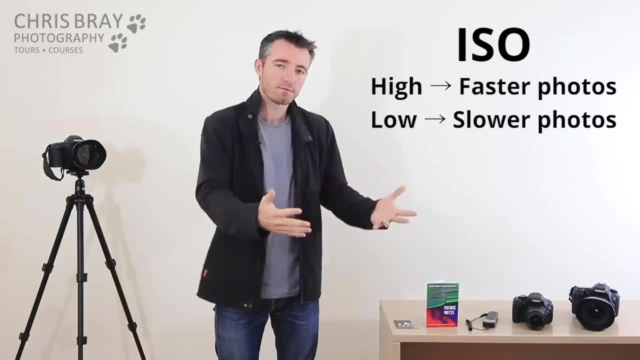 Or if you're like: oh, I wanted to get a slower photo than I seem to be able to get, I want a longer photo for more movement blur, then drop your ISO and you might find you'll be able to access much longer, slower photos. 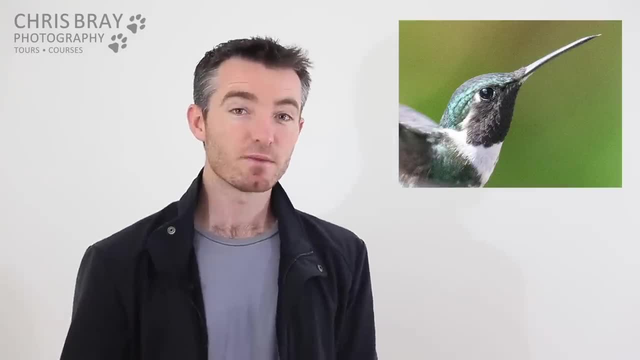 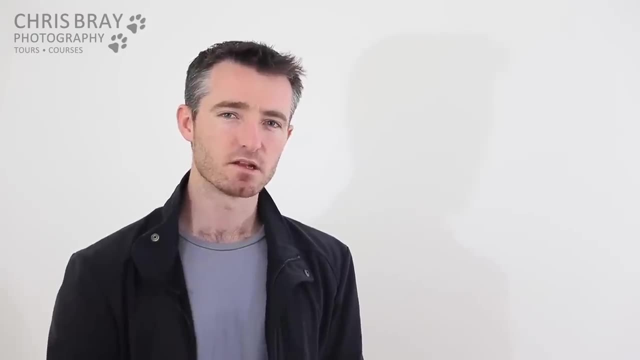 But to avoid noise, the idea is just to keep your ISO as low as you can. There's not much point having your ISO super high and getting really fast photos if you didn't need to, because you're also going to get that little bit of noise quality loss. 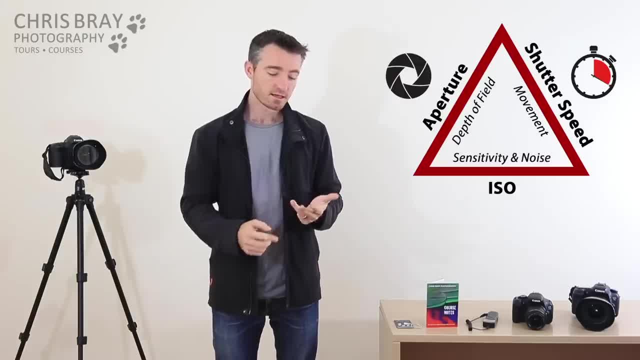 So that's it really for ISO. You've already covered aperture and shutter speed, and together those three things form what's called the exposure triangle. They're the three variables you can control to affect the way the light ends up in your photo, You know. so your shutter speed is how long the shutter is open, for how long the light's. 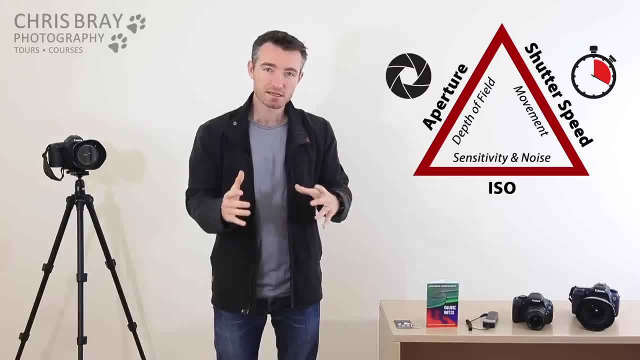 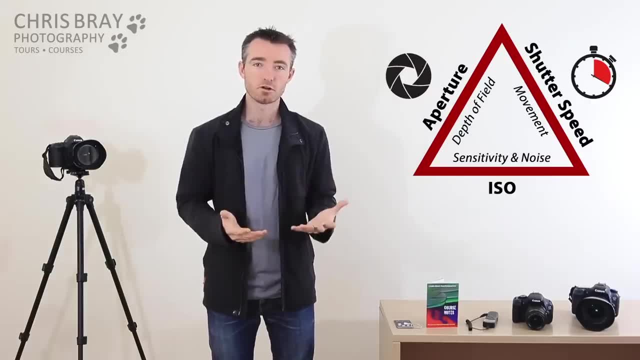 coming in, for Your aperture is the size of the hole, sort of how much light is coming in, And then your ISO is basically how much light it needs. So by varying all of those three things, you've got complete control over your camera. 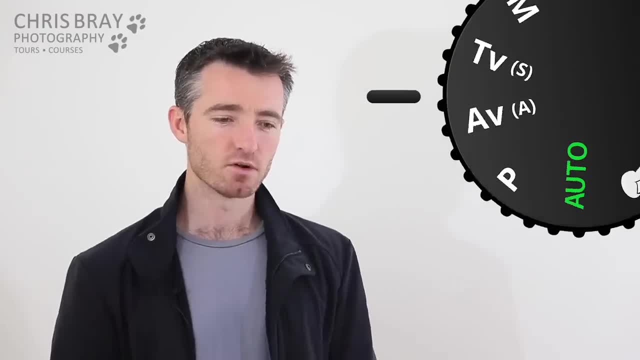 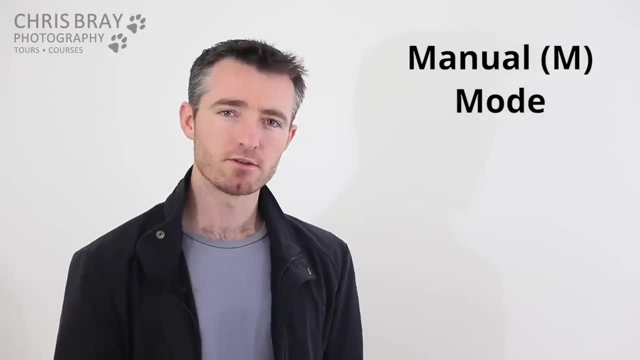 Now, before we go out and practice ISO, I just want to touch on a couple of other cameras, camera modes, Things like manual mode. Now, unfortunately, there's a real misnomer around with manual mode, in that people think unless you're shooting on manual mode, you're somehow not getting the full creative control. 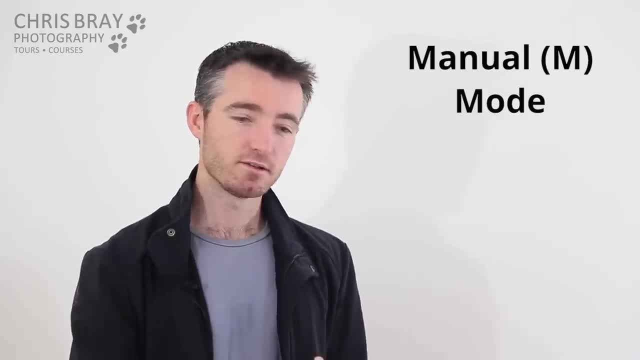 out of your camera. That's just completely not true. Values, like you know, aperture mode, shutter, speed mode- they're still giving you complete control. You can still get to every setting you could imagine. You've still got exposure compensation, so you can still get the photo brighter or darker. 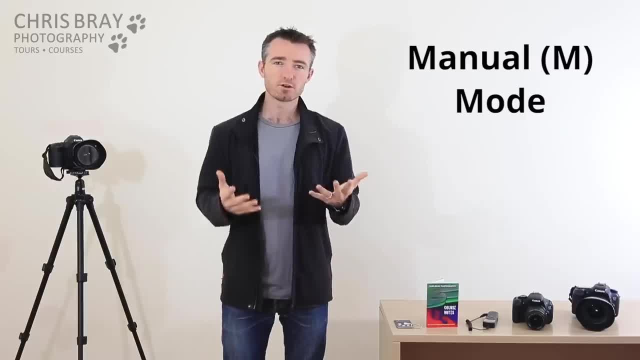 A lot of people think you need to go to manual mode for that. In manual mode you've got to do everything yourself. You've got to pick your own aperture, Your own shutter speed, Your own ISO, And it doesn't help you match them up. 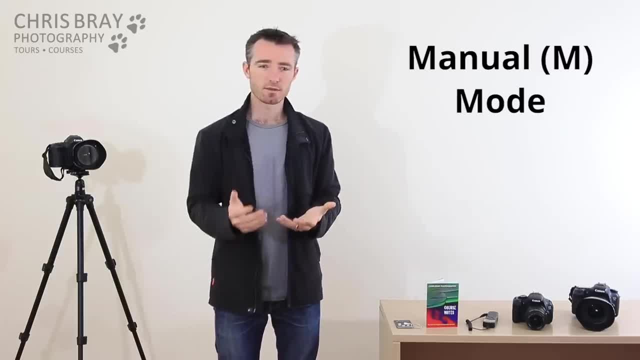 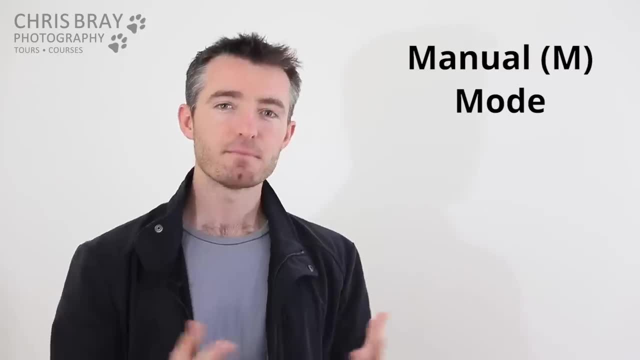 So if the lighting changes or if the scene changes, you just end up with incorrectly exposed photos all the time, unless you're forever watching that little light meter and balancing all these values and juggling them around. Now, manual mode is useful in situations like in a studio where you want to be able to set. 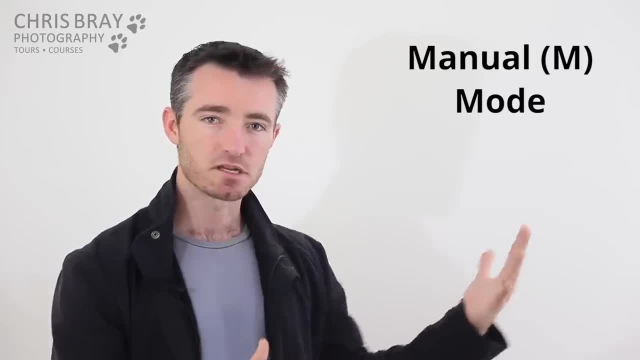 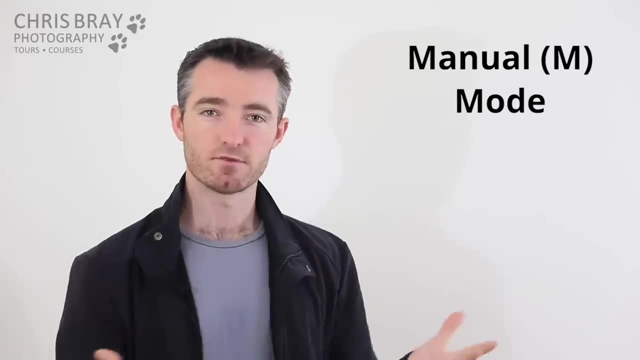 your values up once and you don't want anything to change depending on you know different subjects moving in front Or complex flash work. you don't want your camera to respond to the ambient light because you're going to change the whole world with different flashlights. 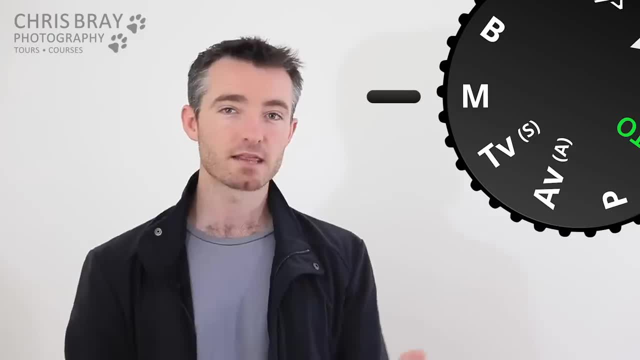 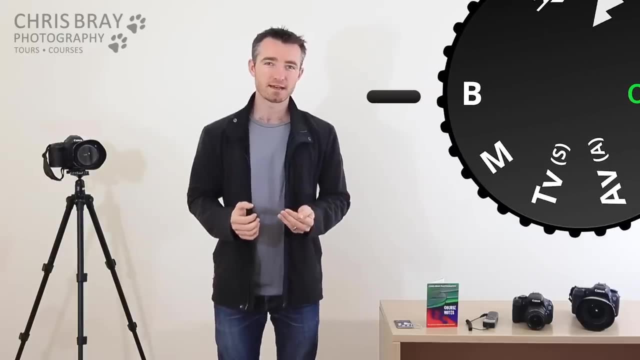 Things like that, Then manual mode has a use. But normally out in the real world running around where the lighting's changing and that kind of stuff, it's just slowing you right down. Bold mode is another mode that's worth looking at. 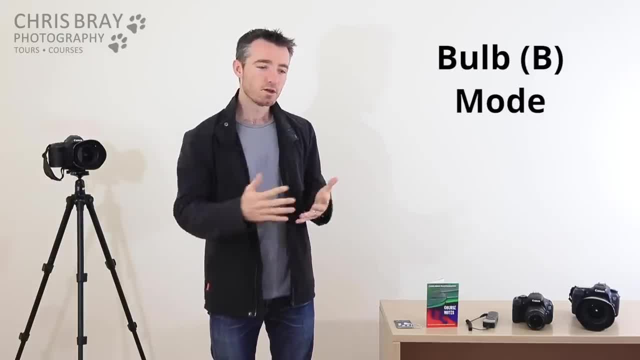 This is how you can get beyond that 30 second limit and start taking longer. you know, two hour star trail photos or something like that. If you don't have a bold mode, don't worry, it'll be hiding inside your manual mode. 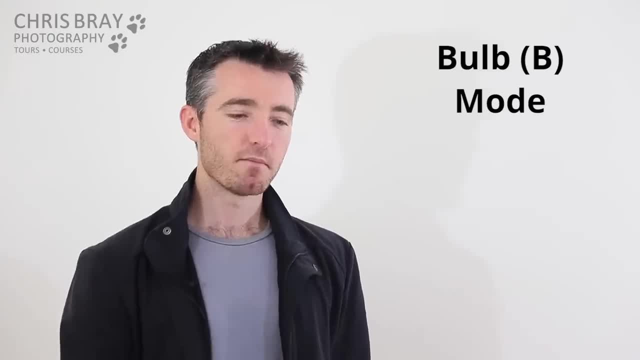 So in bold mode, you can pick whatever aperture you want, But then with your shutter speed it's determined by how long you leave your finger on the shutter button for. So you could actually hold your finger on there for an hour and get an hour star trail. 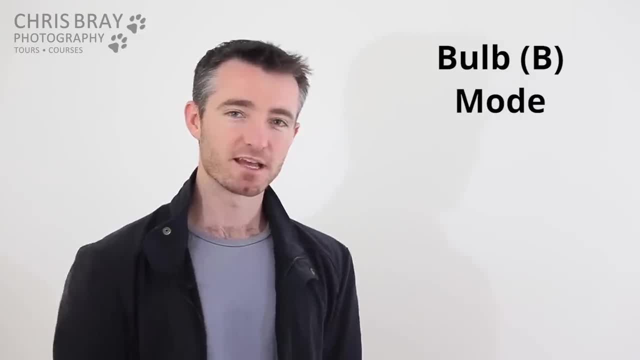 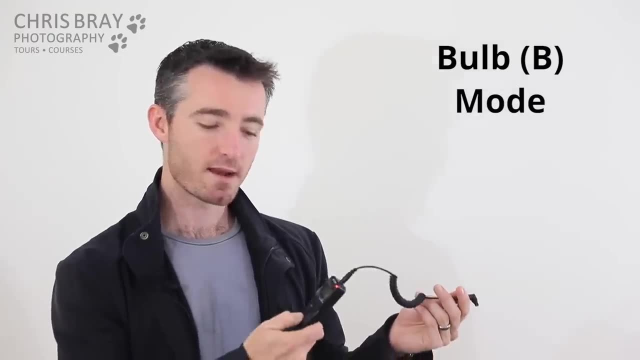 photo or something. Obviously, it'd introduce a lot of camera shake and your finger would get a bit sore. So that's when you're actually designed to plug in one of these external timers. So that's the same as pressing the button on the camera and that's the same as leaving. 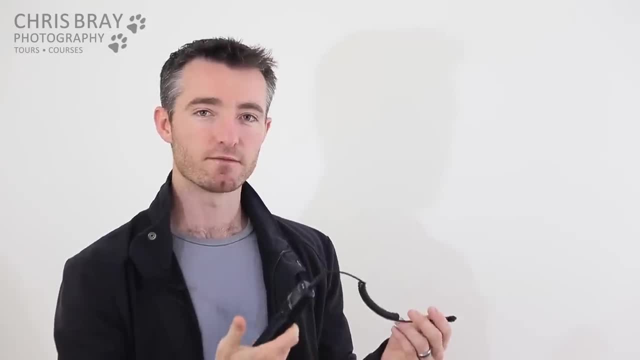 your finger on the button And then you could come back later on and turn it off. Now, if you don't have one of these fancy timers, that's alright. You know, on our photo safaris we go out to these beautiful places where the sky is. 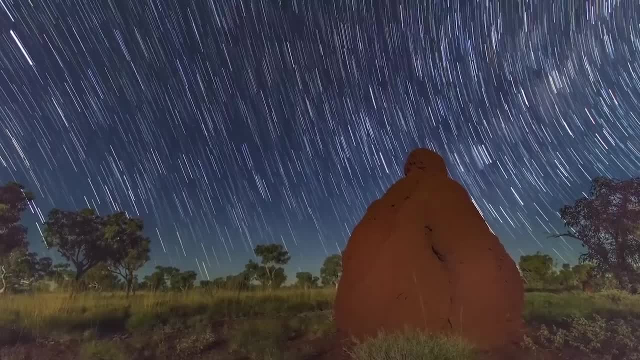 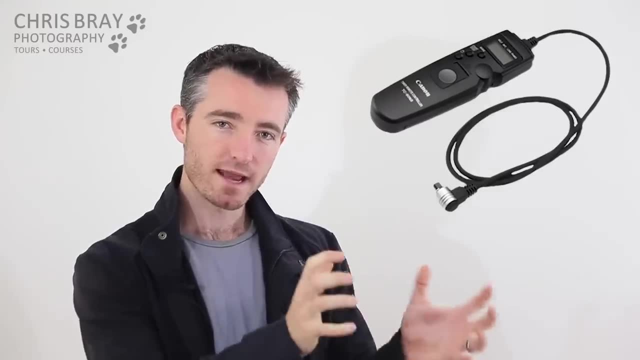 super dark and the stars are so rich. Everyone wants to take star trail photos. Not everyone has those timers, but you can still experiment just by. you need to find a way to hold that button in without hanging onto the camera. The best way is just to hold it in with a bunch of rubber bands. 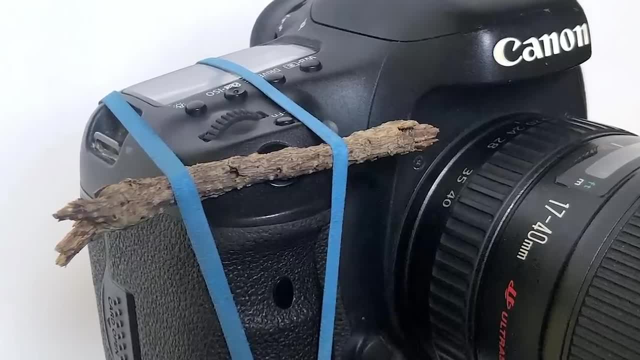 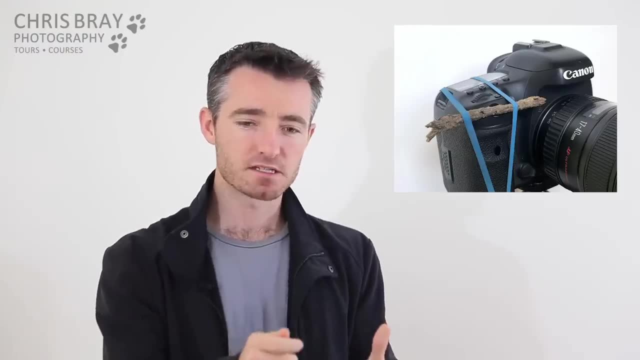 You might need to put a little stick, or, and just that'll hold the button in there And then you can step away and the camera starts taking the picture. You come back an hour later. Don't worry about it. you might be wobbling the camera for the last hundredth of a second. 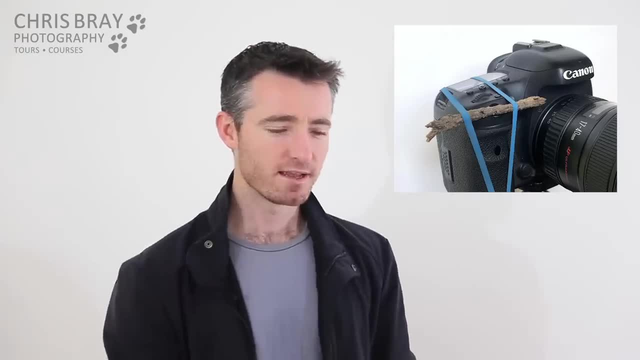 as you pull the stick out. That doesn't matter. Think about the ratios involved. If it's taking a whole hour for that faint light to register in your picture, the last hundredth of a second of wobble isn't going to make. 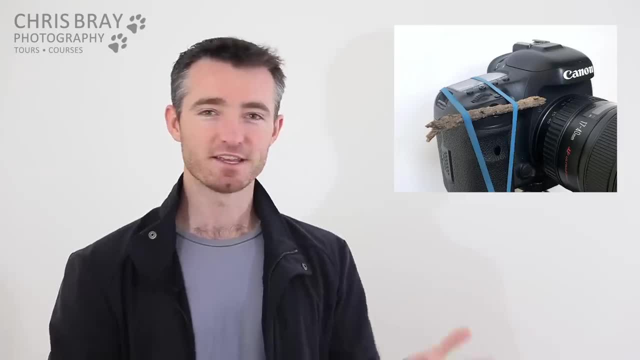 any difference. Obviously it's more convenient to have a fancy timer and you can get one eventually. But just to start with, it's good to know that you could go out tonight and take a star trail photo, just to see if you like that kind of thing. 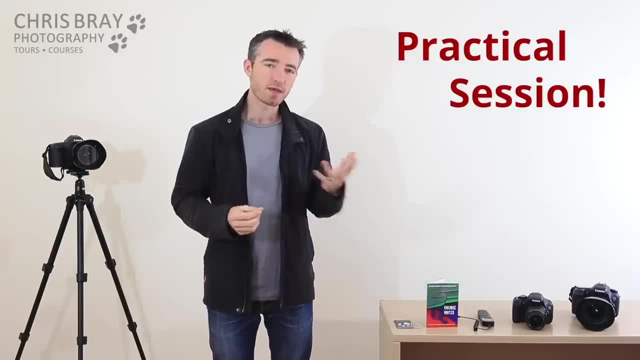 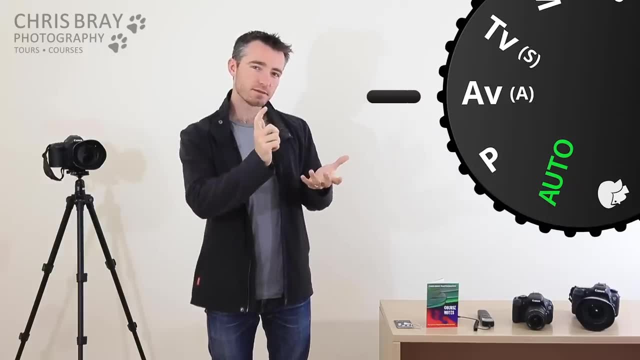 So for our prac session on ISO you should test out how it affects both aperture mode and shutter speed mode. Start off in aperture mode and then just pick whatever f-number you want And then look at the shutter speed that the camera is going to use. 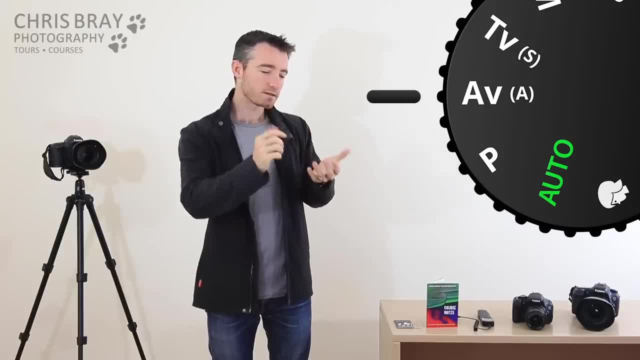 Either take a picture and look at it, or just look through the viewfinder, touch the shutter button and just look at the shutter speed it's suggesting. there, Let's say it was going to use, you know, 50th of a second. 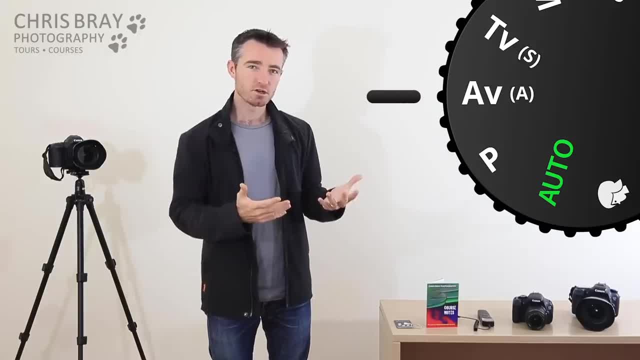 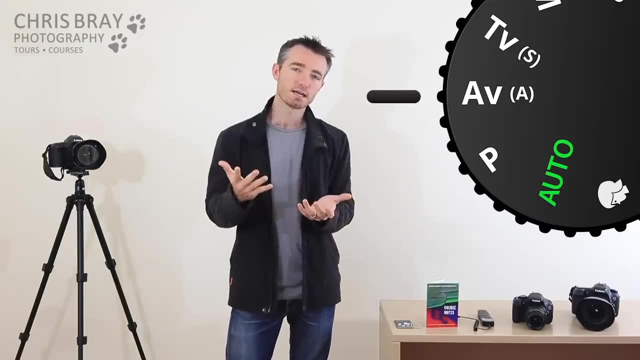 You'd find if you turned your ISO up, you'd find the shutter speed it's going to use is quicker. So if you doubled your ISO, it's going to double your shutter speed, So that's convenient. If you're ever remember when we were taking the large f-number photos- and they were quite- 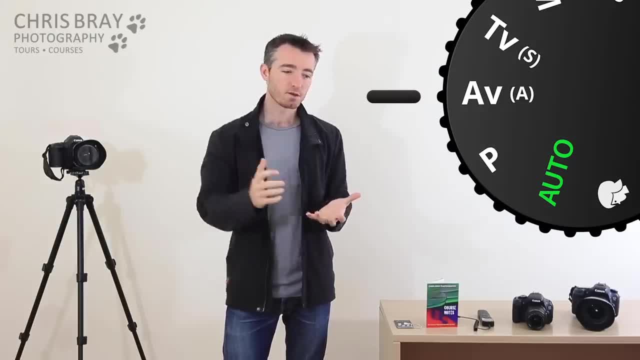 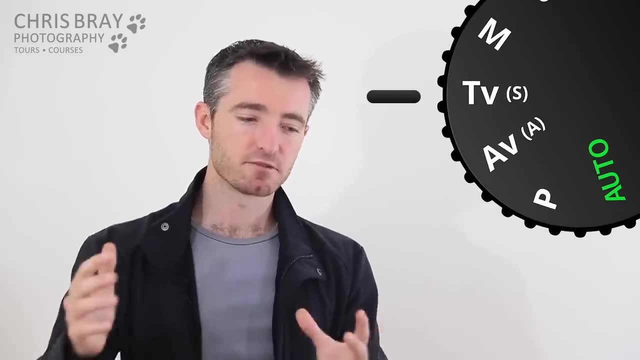 slow, A lot of camera shake involved. If you crank your ISO up, you'd find then the shutter speed becomes faster again and you'd be able to hand hold it without that camera shake. Changing your ISO in shutter speed mode just affects the range. 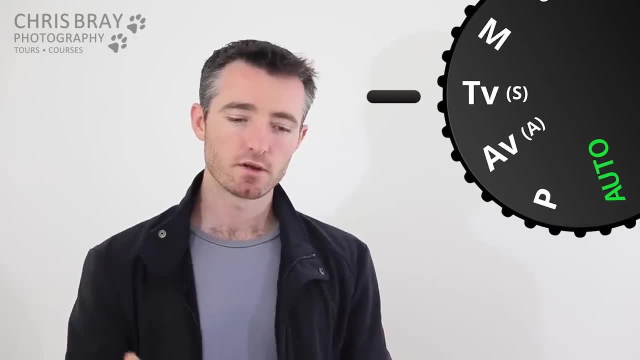 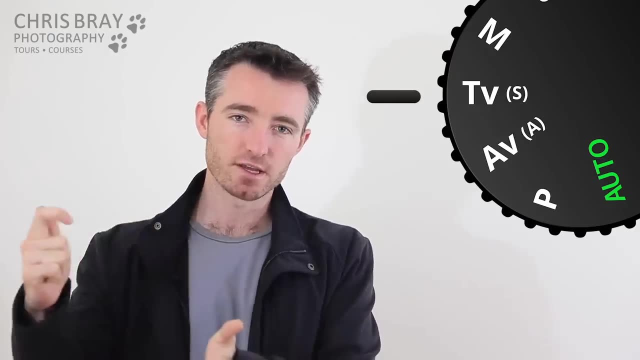 The range of shutter speed values you're allowed to operate within. So you know, let's say, if you're in shutter speed mode, so TV or S mode, you wake your camera up and you try and scroll and find the fastest photo you can get to. 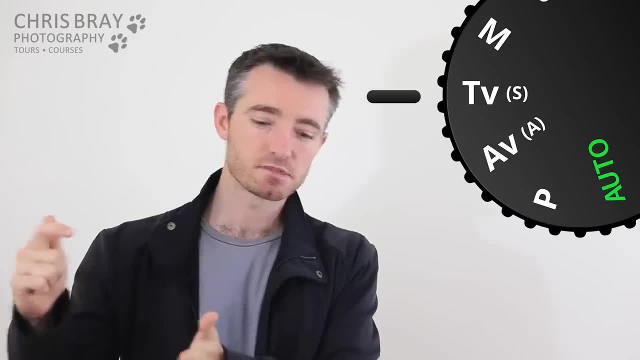 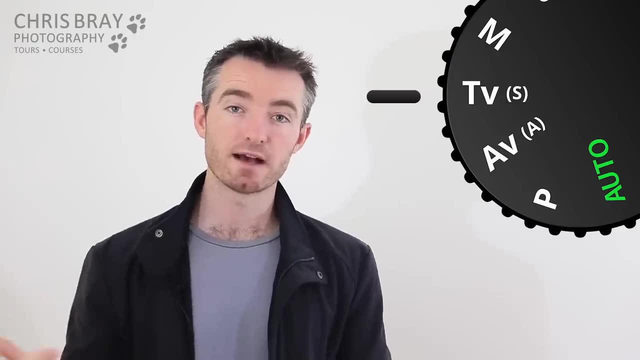 It might be 500th of a second or something, before it starts flashing warnings. so you come back a bit. But if you turned your ISO up, you'd then be able to keep scrolling to much faster shutter speeds. you know, 2 4,000th of a second. 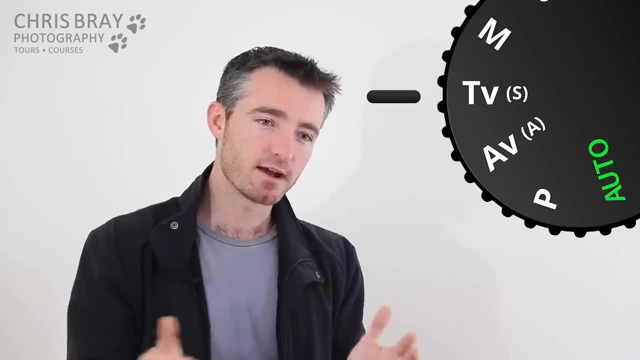 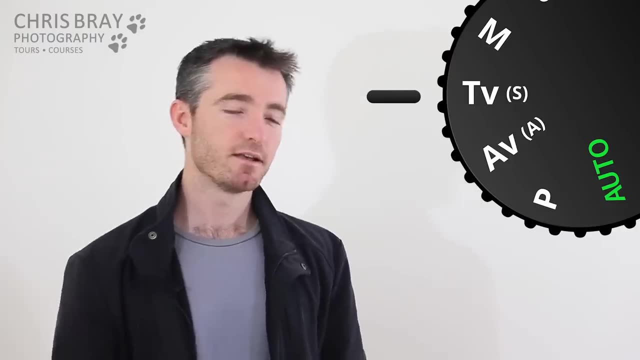 Or if you wanted to get longer, slower photos. initially you kind of scroll down and you go, oh, All I can get is 50th of a second or something. But if you drop your ISO all the way down, like ISO 100, then you might find you could. 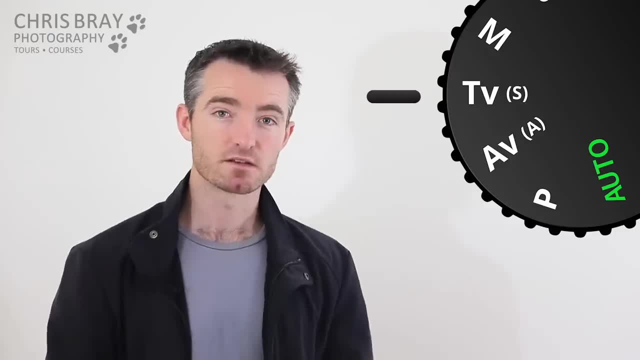 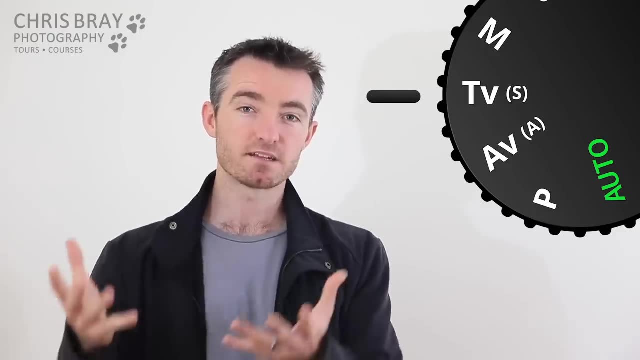 scroll to an even slower shutter speed- 20th of a second or 1 second or something like that. The same thing is actually happening in both situations. if you think about it, By turning your ISO up, we're either able to get to faster shutter speeds in shutter 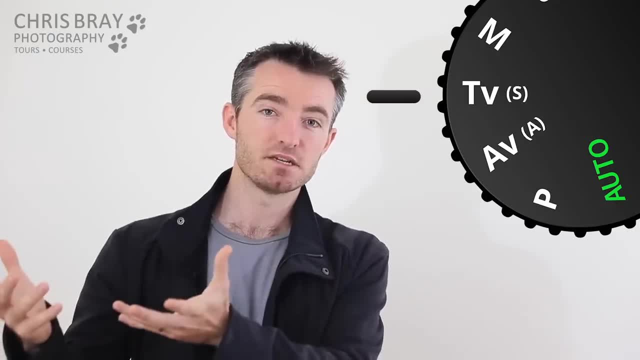 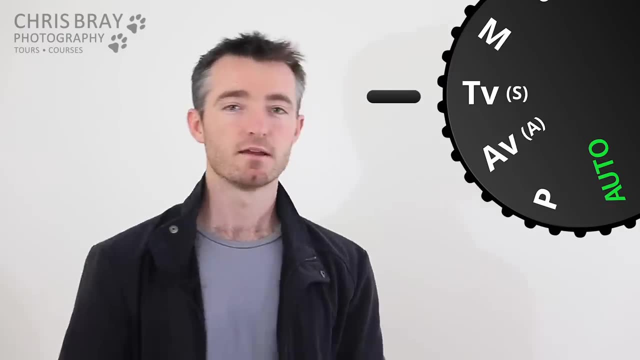 speed mode or in aperture mode, it's automatically picking faster shutter speeds for us. And if you turn the ISO down in shutter speed mode, you can get to slower photos. you just still need to scroll there In aperture mode, turn your ISO down, it'll automatically pick slower photos for you. 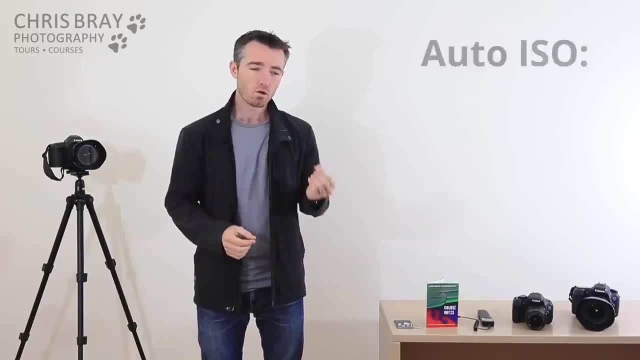 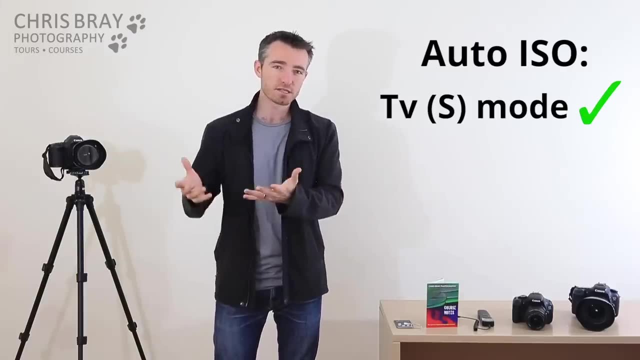 Now, what about auto ISO? A lot of people ask about that. Now, auto ISO in shutter speed mode, TV or S mode, that's actually quite handy, because then the ISO will only ever lift up just enough so you can get whatever shutter speed you're. 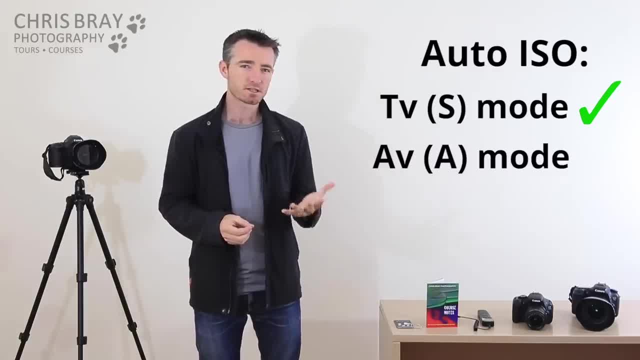 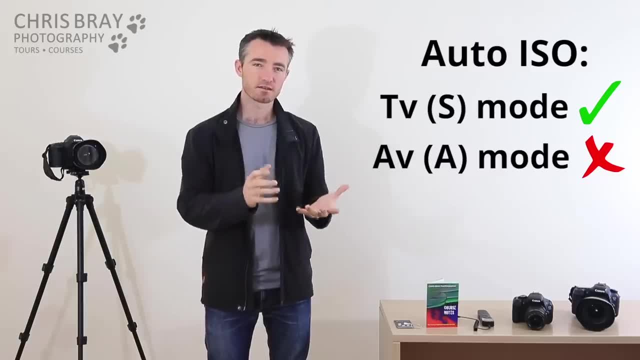 after. But auto ISO in aperture mode is actually not that good because all it ever does is lift your ISO enough that you're getting enough shutter speed not to have camera shake. That's basically all it's trying to do. So it's giving you a quick enough photo. 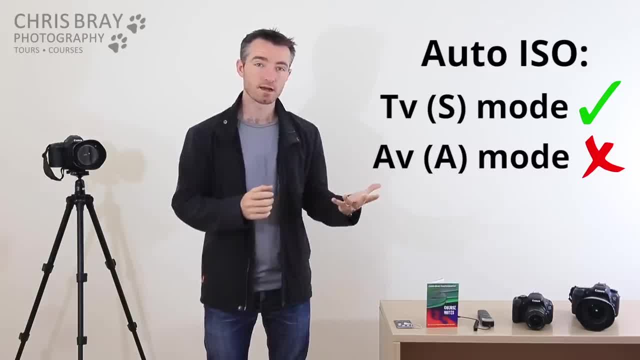 A photo that you're not shaking around. Often it's nothing like quick enough to be able to freeze the animal or the bird or the person walking around. you still end up with blurry photos. So I don't use auto ISO for aperture mode, but I use it quite a lot in time value mode. 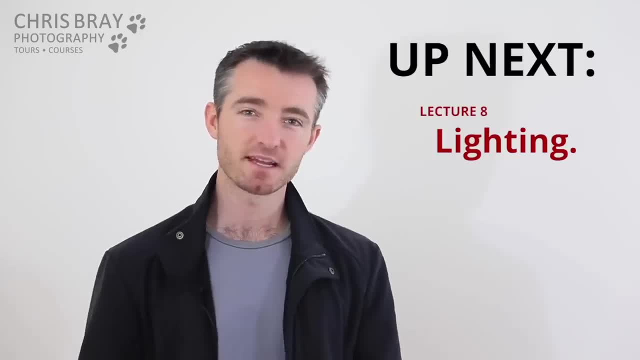 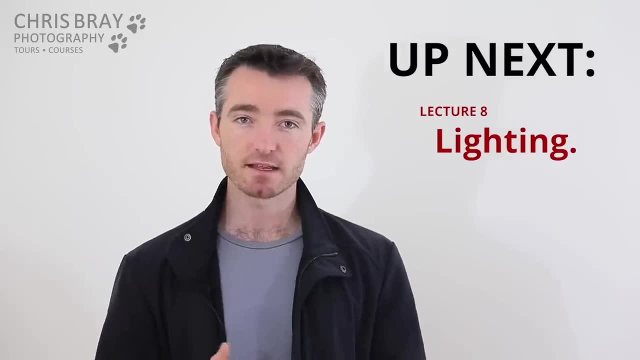 shutter speed mode. So after you've done that practical session, make sure you come back and find the next lecture in the series, which is on lighting. There's so much you can learn about lighting- just the simple stuff like the different types of lighting and the different directions of lighting, how that affects your photos. 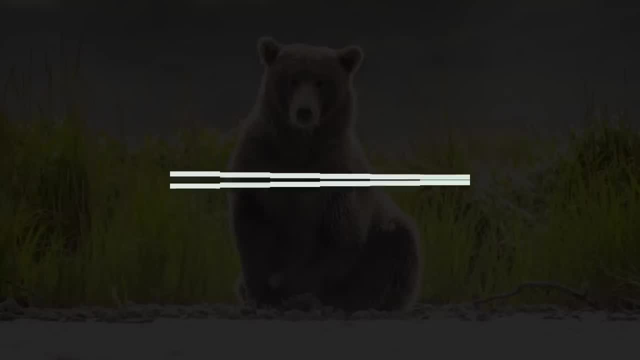 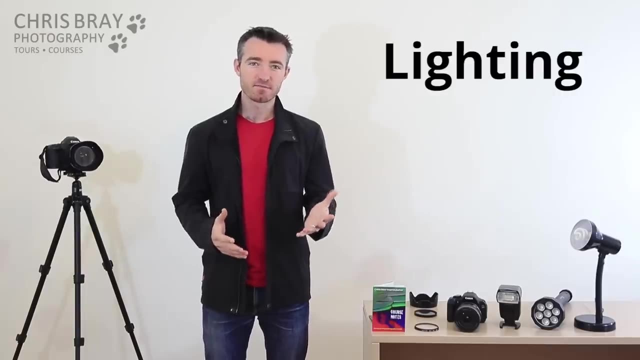 It's a really powerful thing to know. So in this lecture we're going to look at lighting. Now, I know that sounds like a fairly broad topic, but at least being able to understand the different types of lighting and the different directions of lighting and how that affects. 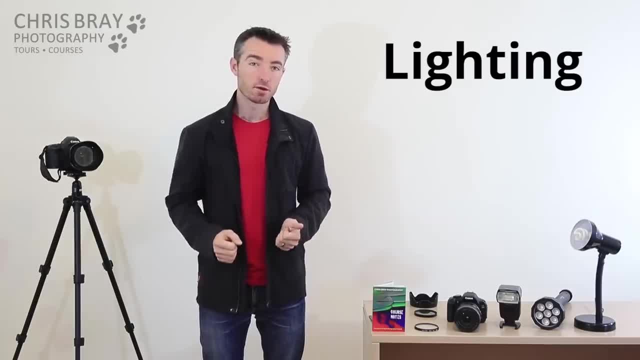 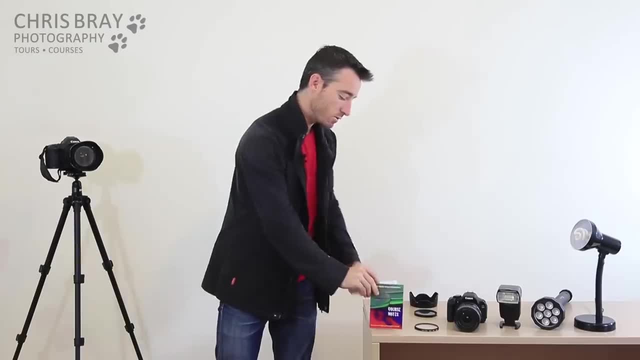 your photos and flash and things like that. that'll put you a lot further forward in what you can get out of your photos. And just a reminder that in the course notes booklet as well there's the same lighting section that matches up And with the little summary clip cards there's a section there that tells you about the directions. 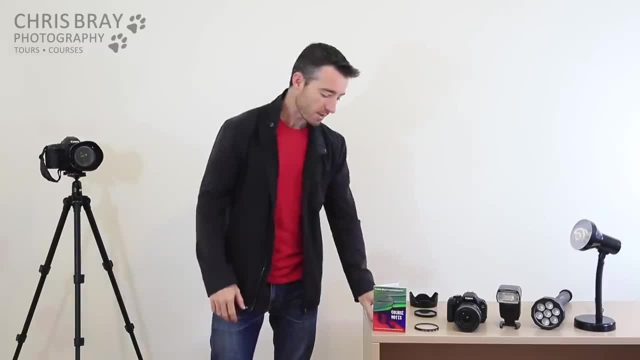 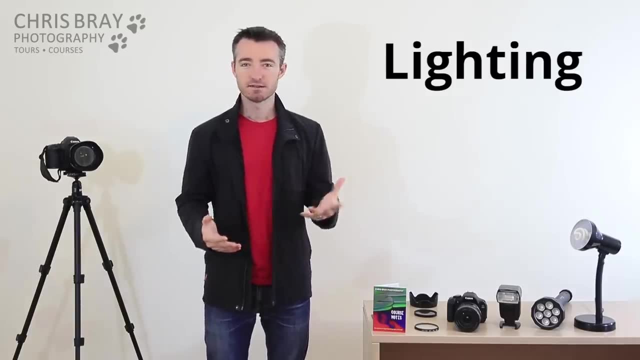 of lighting That puts your shadows and so on, So that's pretty handy, But in many ways, lighting is probably the most important part in photography. really, You know, you can do as much as you want with your aperture and shutter speed and blah. 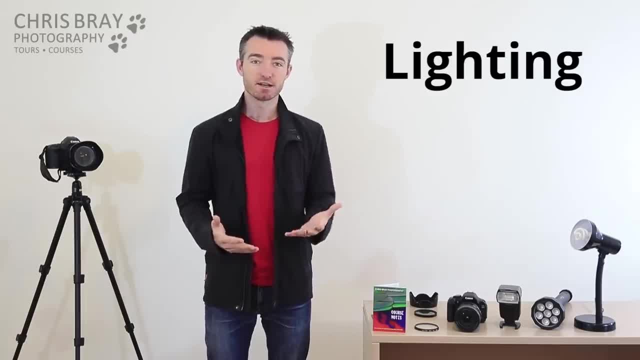 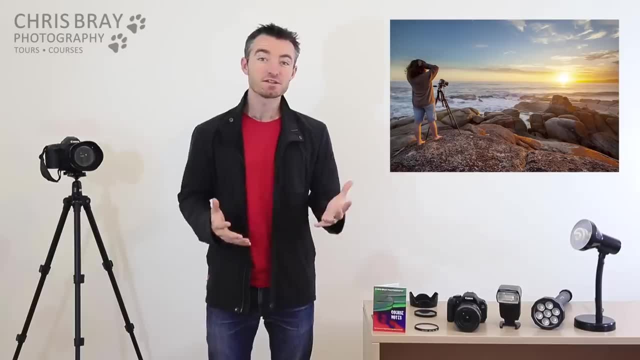 blah blah, But if the lighting is terrible, there's almost nothing you can do to get a good photo. Let's just look at the various types of lighting you get in your average day, starting with lovely golden morning lighting. Now, as you know, morning lighting is beautiful for photography. 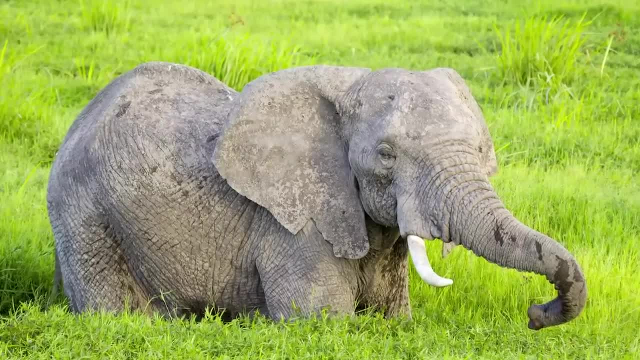 You know, the sun is low in the sky, so it's nice and soft. You don't have that contrast problem, The shadows are not too dark And it has that nice warm glow to it as well. It's a really beautiful time for taking photos. 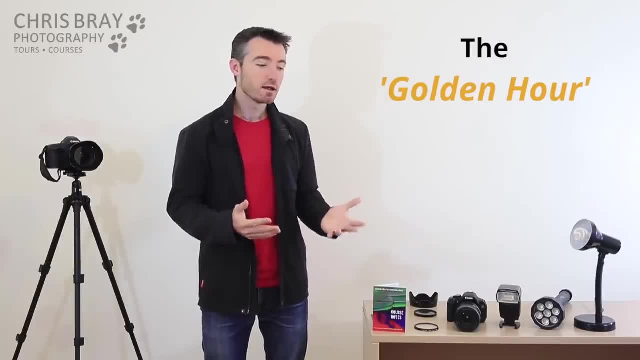 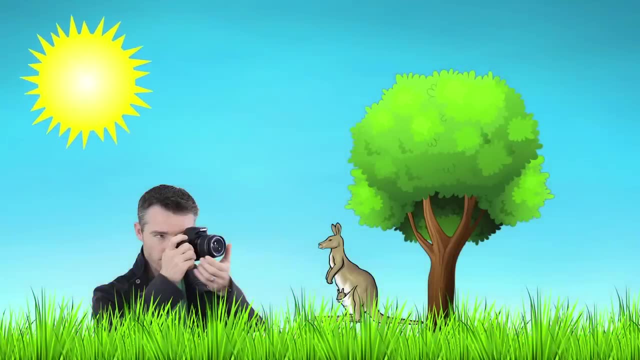 While you can certainly take beautiful photos before the sun comes up as well, you've got about an hour afterwards- That's what they call the golden hour- when the lighting is just perfect. After that, pretty rapidly, the sun starts to climb higher and get stronger, and you. 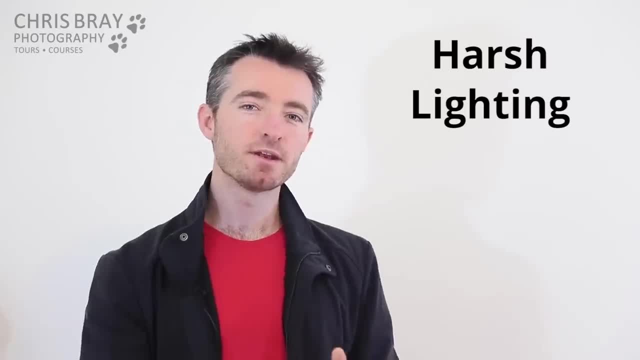 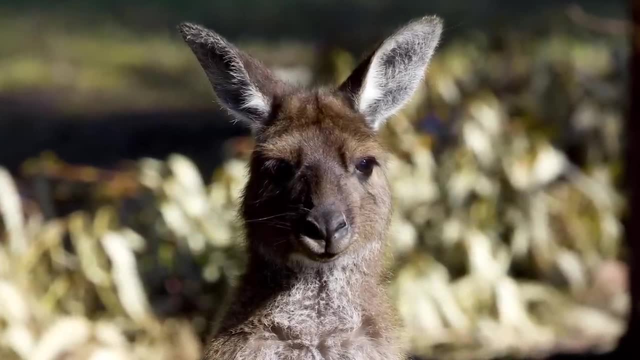 end up with harsh lighting. When the sun gets too strong, then you end up with contrast problems. So the bit in the sun is a million times brighter than the bit in the shade next to it. So the shadow just becomes jet black or you end up blowing out your highlights. they become too bright. It's just not a good time for taking photos. Also, middle of the day the sun is quite high, so you end up with top lighting, which means you get shadows in the eye sockets of people and you know photographs of animals and things. 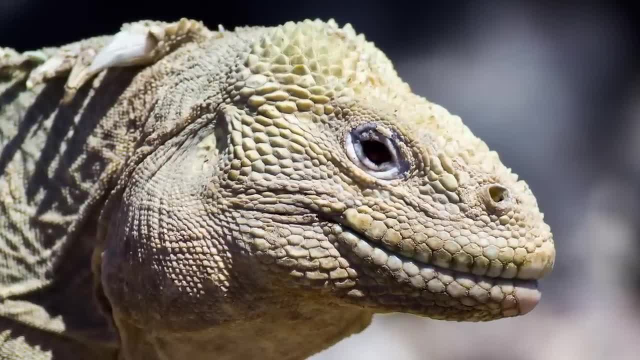 They kind of become very bright on the top and very dark underneath. It's not a very nice direction of light either Not a good time for taking photos. If you have to take photos in the middle of the day, in the sun, you're better off going. 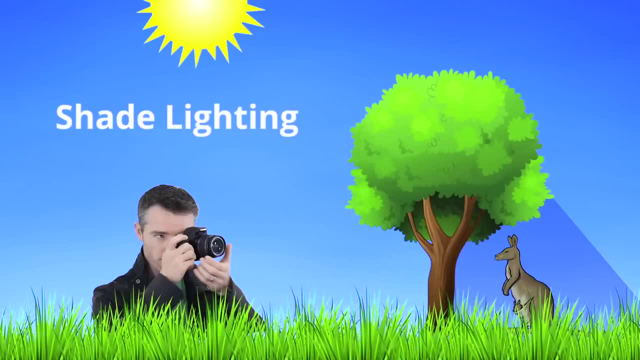 and finding some shade, Literally going and standing behind a building or something where it's just total shade lighting, Because the light that gets into the shade is out of the way. It's not a good time for taking photos. It's actually really beautiful. 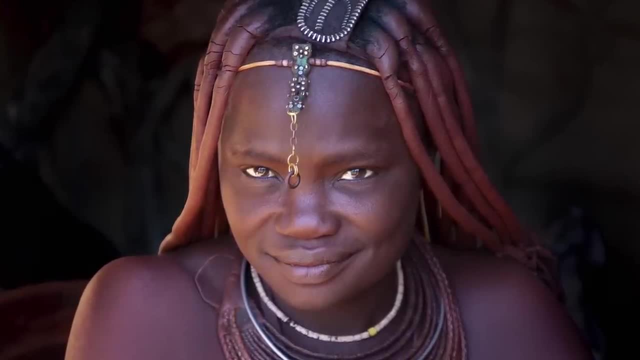 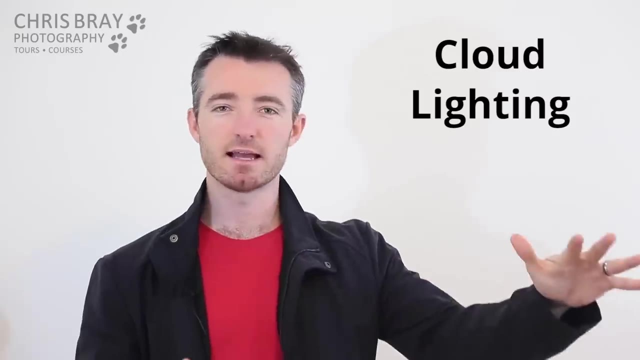 You don't have any contrast problems because you're already in the shade, so there's not going to be any shaded side of your subject. It's just nice, and even It's the same with cloud lighting. You know, if you wake up and it's just a blanket cloud cover day, you might think what a boring. 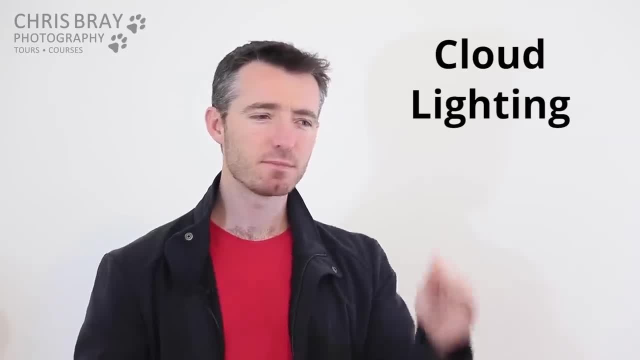 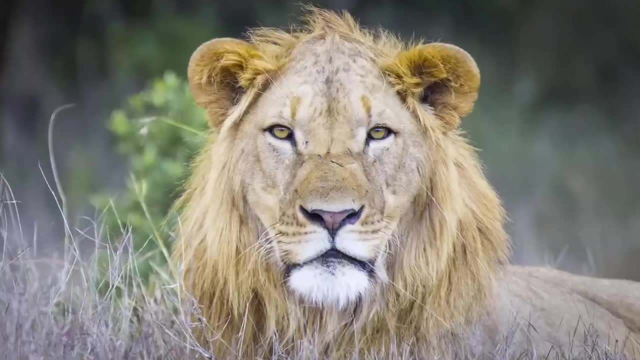 day for taking photos. Sure, your landscape photos might look a little drab if there's too many clouds, but photographs of things like people and animals- fantastic. Cloud lighting is beautiful. It's just such a soft light and the light has bounced off from everywhere. 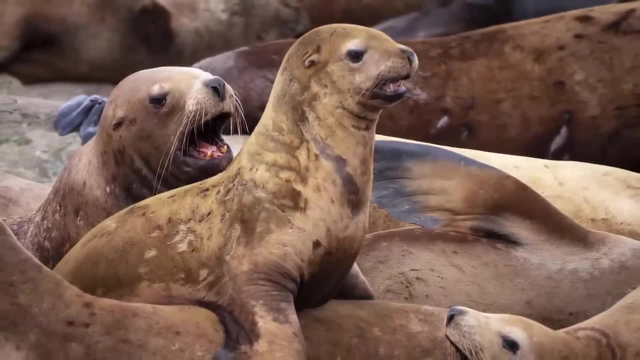 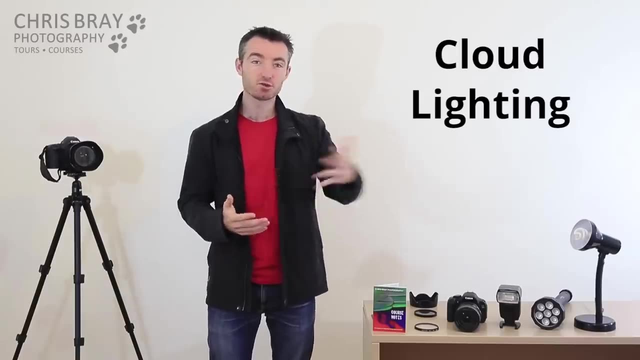 So it's coming from every direction at once So it fills every little nook and cranny evenly. It's a very flattering kind of light for portraits. Wrinkles and things don't really show up. It's a great time for taking photos and it means you can shoot all day long because 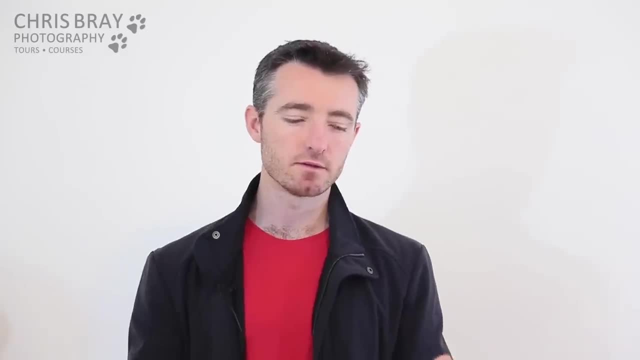 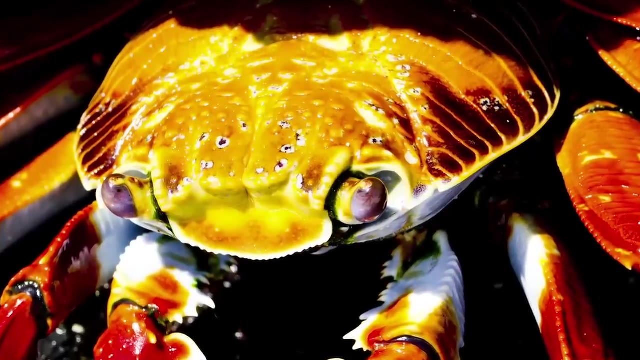 there's never any harsh sunlight. Here's a good little tip: If you're photographing an animal that's sitting in the sun like a little crab or a lizard or something, if you could actually shade it with your body, sort of move yourself between. 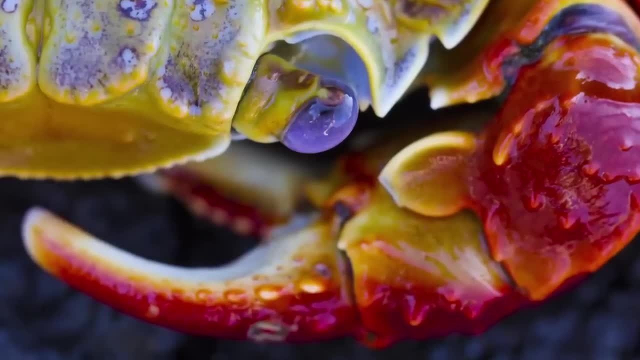 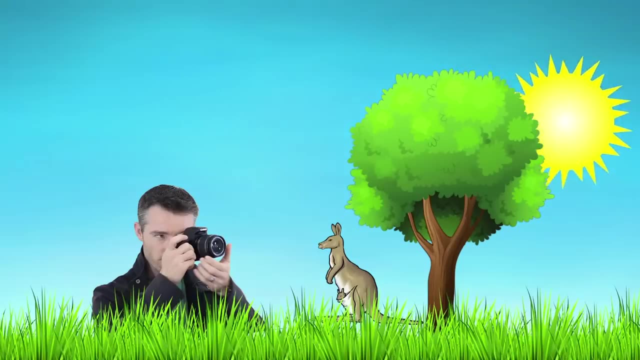 the sun and your subject cast your shadow over it, then you've got it in nice soft shade lighting and it'll look beautiful. All the colors will look nicer and it won't be so contrasty anymore. Moving on, then you get to evening lighting, much like morning lighting, I guess. 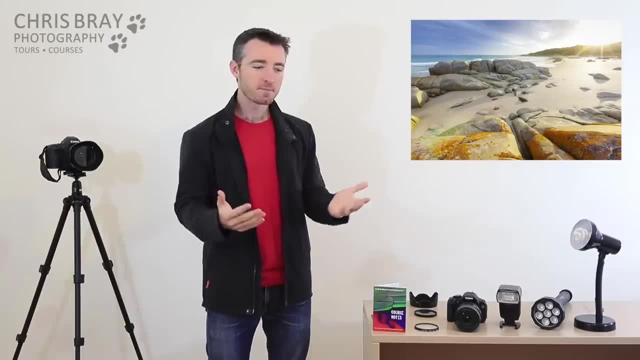 The sun is low in the sky and you get that nice warm orange glow again and the contrast problem is not there anymore. You can see in this photo you can see the shadows, but they're not too dark at all. 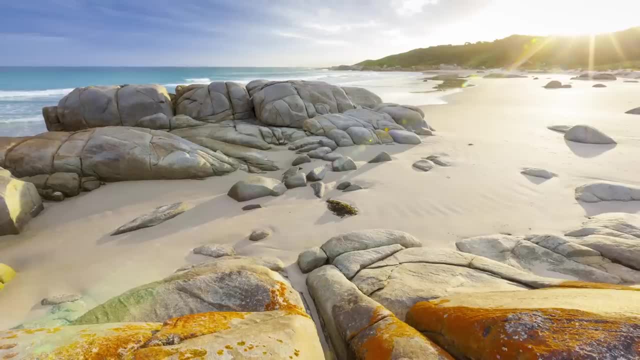 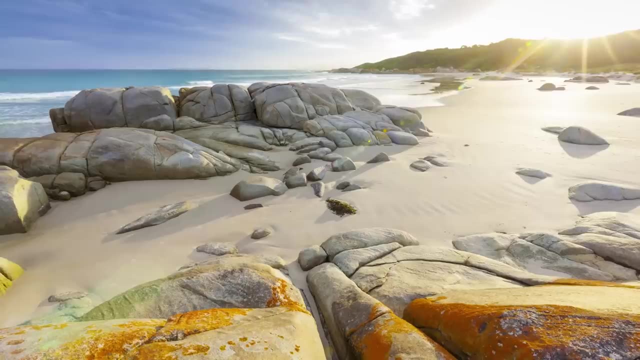 They just provide a bit of interest. It makes it look a little bit more 3D. You can still see into the deep crevices in the rock and obviously this photo is taken with a large F number. You can tell from the large depth of field. so everything is in focus, but also the sun. 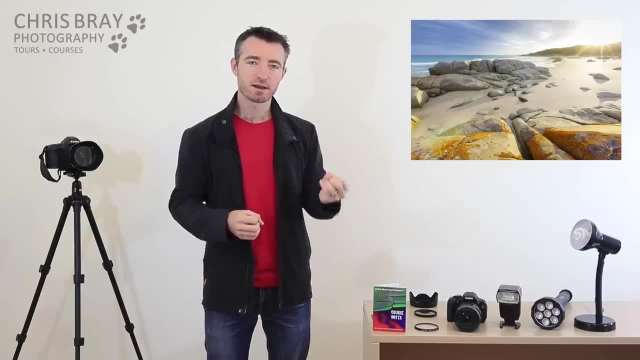 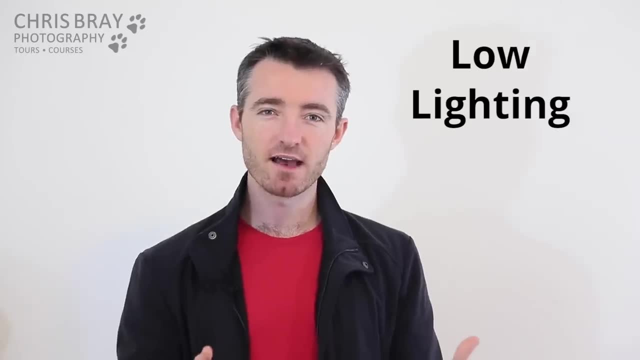 has done that, starburst, which remember in the aperture lecture. you get that with the large F number. And finally, moving on to low lighting. Now, low lighting is tricky to deal with just because there's not much light around. 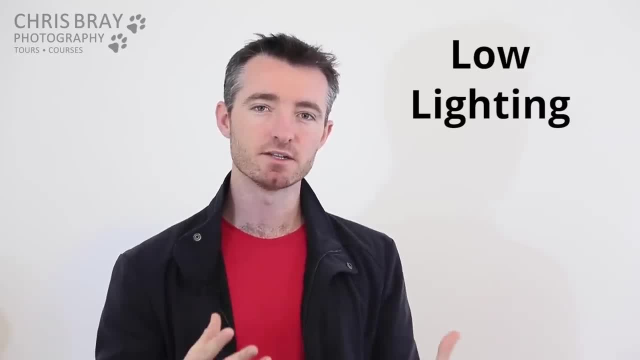 and it's going to take the camera quite a long time to collect enough of it to give you an image. So you're going to have to expect to have quite long slow shutter speeds. so you're going to have to hold the camera really steady or put it on a tripod or turn your ISO up. 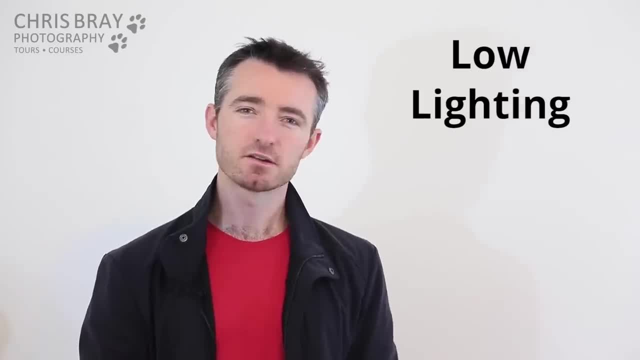 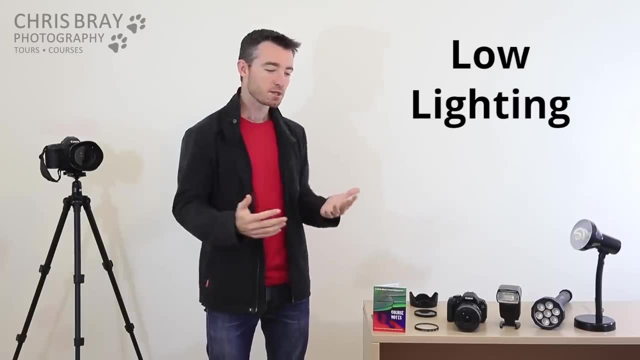 or a few other things. It's a little trickier to deal with, but it's worth persevering because you can get really beautiful results. Don't always let your flash pop up. It's worth knowing that in all the camera modes we've been using on this course. so 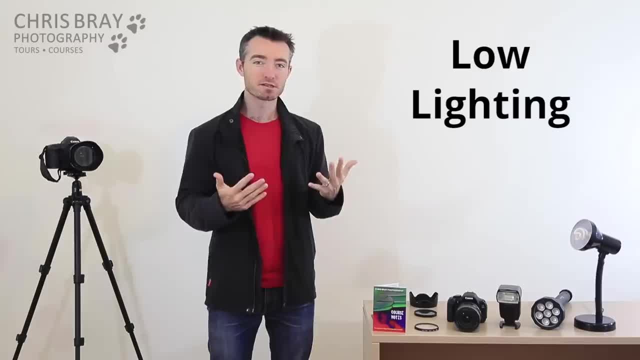 program mode and everything better than that. the flash will never pop up on its own. If you actually want to use the flash, you have to press the little flash release button next to the flash and then it'll pop up. but if you leave it down, then you're forcing. 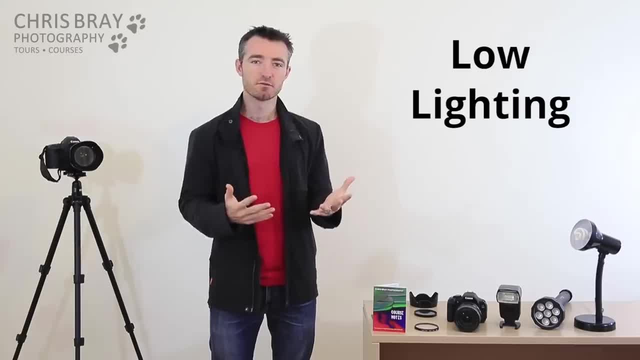 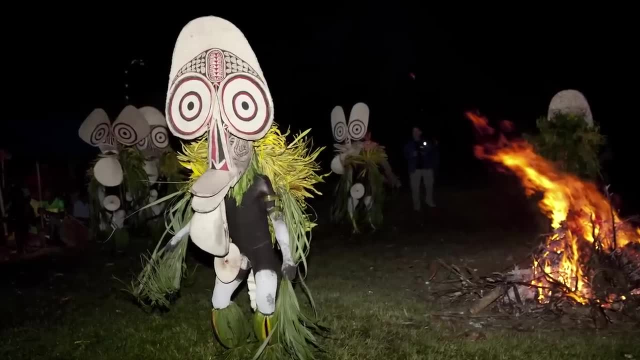 the camera to use that natural ambient light and you can get such beautiful results. All of these sort of photos would have just been ruined. in auto mode The flash would have popped up, bam, and you'd lose all that delicate lighting of the fire. 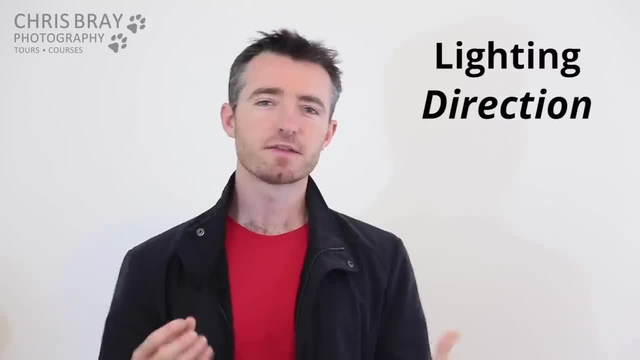 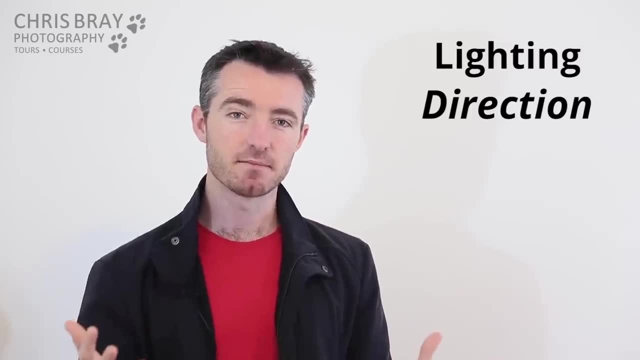 or the head torch, whatever it is, so persevere. So the other important factor of the lighting is not only the quality of the light, but the direction that it's coming from, because that affects the shadows, as you'll see. So let's start with front lighting. 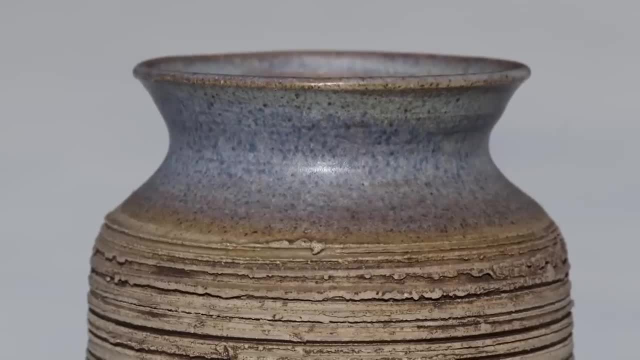 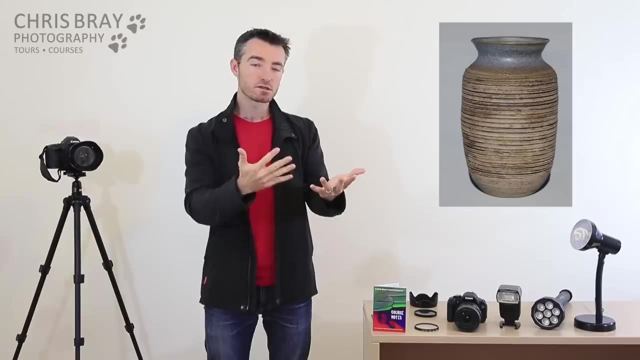 That's where your subject is lit, from the same direction that you're looking at it. So there's some pretty tell-tale signs of front lighting. Your subject ends up being completely illuminated, so you don't have any shadows on it, of course. 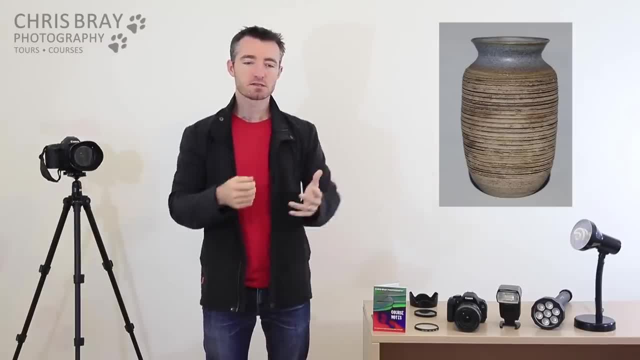 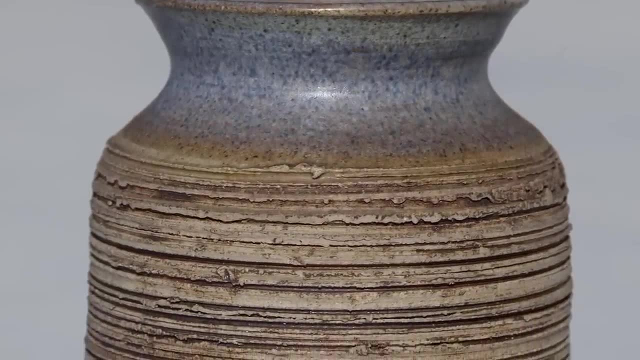 because if you're shining the light on the front of it, all the shadows are around the back. So it's great if you want to be able to see every detail, like for a product photo, for a catalogue or something, And there's a lot of drawbacks to front lighting. 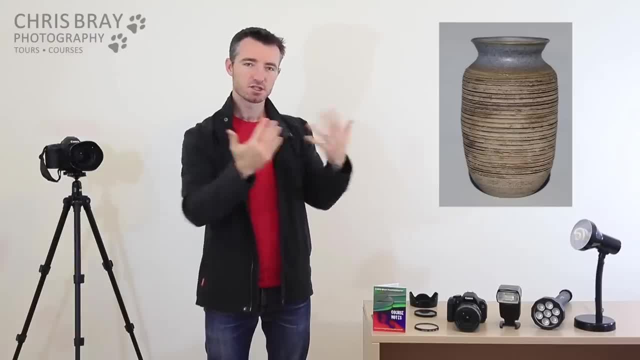 If your subject is at all reflective or glossy, it's not going to look as good as it does. The light just sort of shines straight back into the camera and you get that nasty glare. Same on the skin of people, or if they're wearing glasses, or if you're trying to shoot. 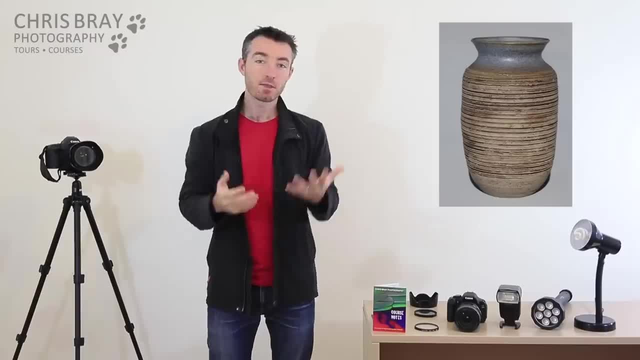 through glass. It just bounces back at you, so it's not that nice. And the worst thing about front lighting is it tends to make your photos quite flat and two-dimensional. You can't really see the shape of things. You need some shadows for that, and that's where side lighting comes in. 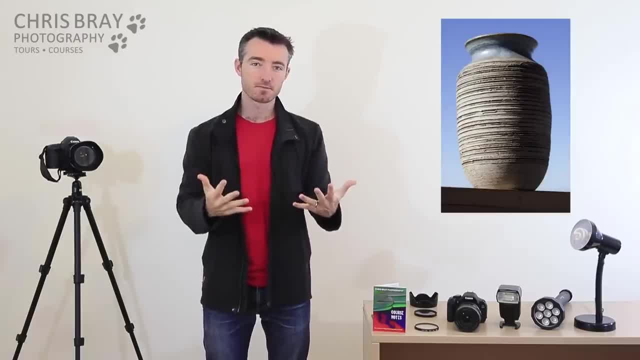 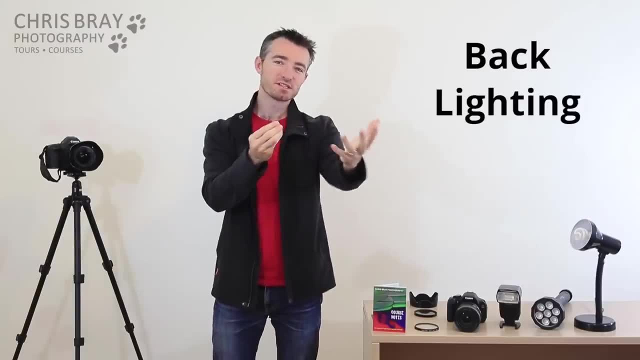 So side lighting reveals shape and texture through the shadows. So side lighting is good for portraits or anything where you just want to make it look a little bit more 3D. Now back lighting, when you're starting out in photography, people often try and avoid. 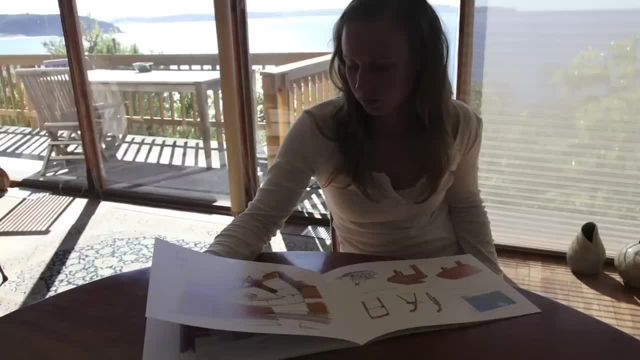 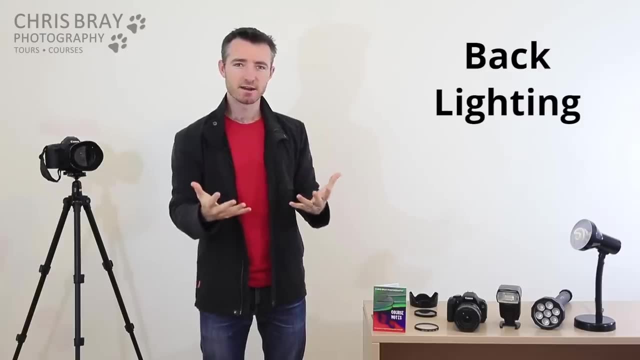 it because you end up with dark silhouettes and things like you saw in the exposure lecture, when you accidentally have the girl in front of the window or if you get the sun in the background of your shot and your subject just comes out as this really dark figure. 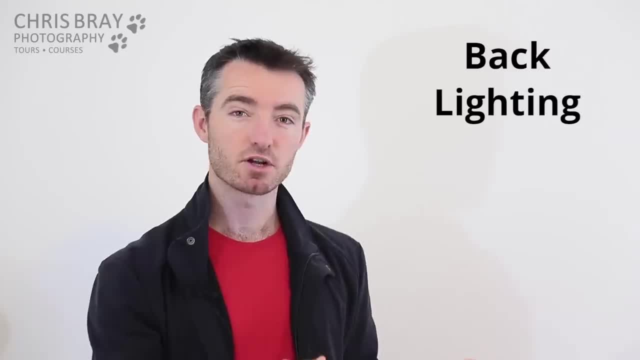 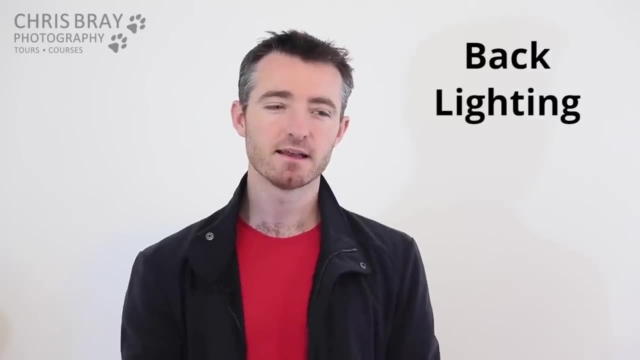 But in that exposure lecture we learned how to fix those kind of problems using exposure compensation. So you could just go plus two, brighten the photo back up and then great. So after you've learned how to deal with the problems of back lighting, it can give you. 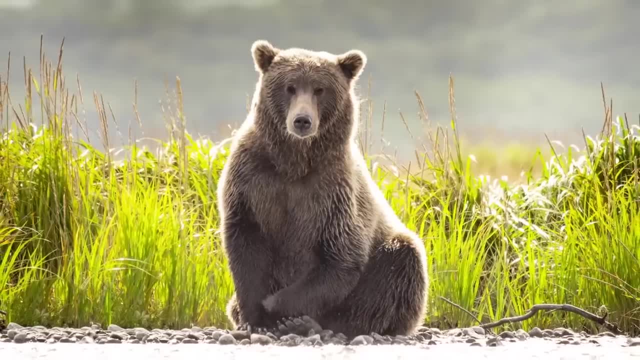 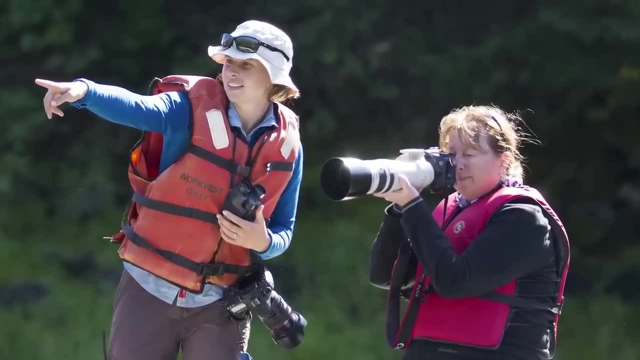 some really beautiful results. It can give you a nice glow or halo Around the edges of things, Rim lighting. It can give you really nice silhouettes And for people it gives you nice highlights in the hair. So back lighting can be a really beautiful light to use. 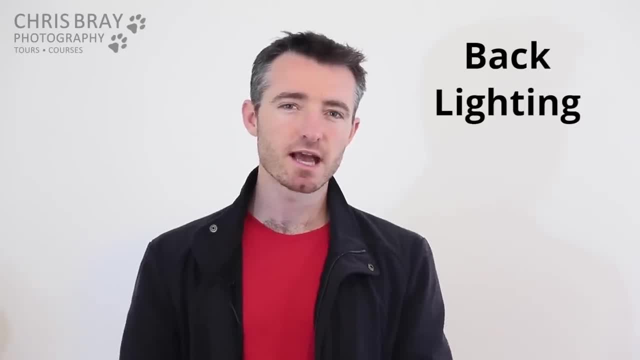 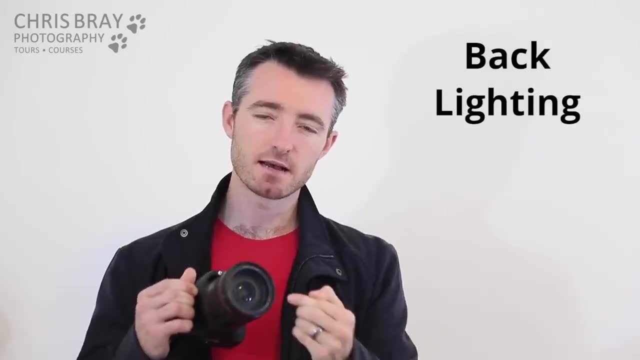 You might just find you need to overexpose the shot sometimes And you've also got to look out for lens flare. You've probably seen these little splashes of light that come across your photo from time to time. That's caused by direct sunlight coming into the front of your lens and reflecting off 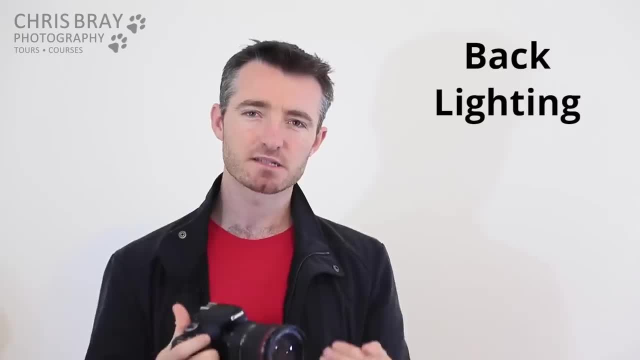 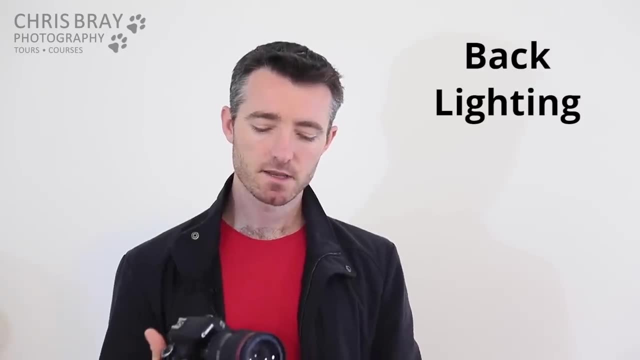 every bit of glass inside your lens. Now, getting direct sunlight in your lens is a problem for several reasons. Not only do you get lens flares, But you also lose some of the saturation of your colors, And if you have little bits of dust or something on your lens, they tend to show up more. 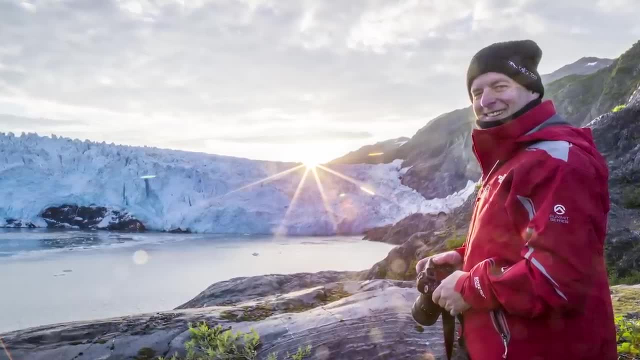 Autofocus can struggle. Getting sunlight in your lens is not a good thing. Now, if the sun is actually in your photo, then you're going to get sunlight on the front of your lens. Clearly There's not much you can do about that. 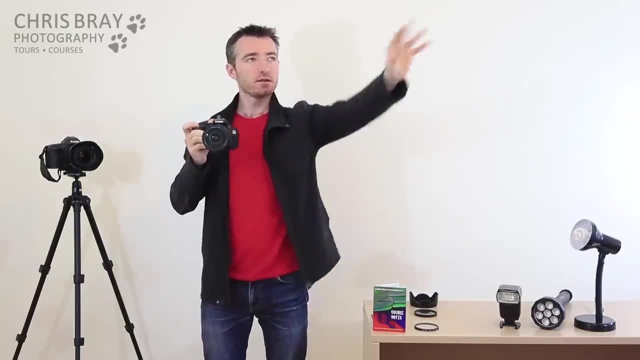 So you'll probably have lens flares and all the other problems. But often the sun is not in your shot. Maybe it's up here somewhere You wouldn't have even really thought about it. maybe You wouldn't think it's backlit at all. 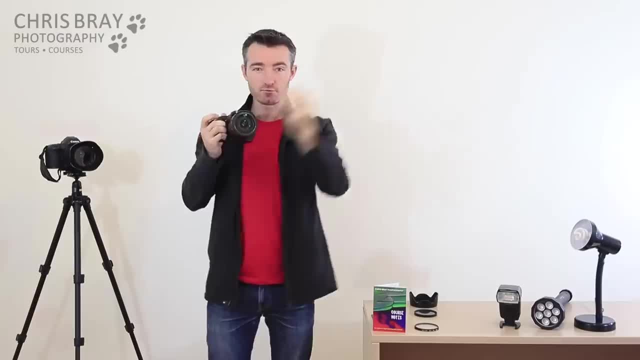 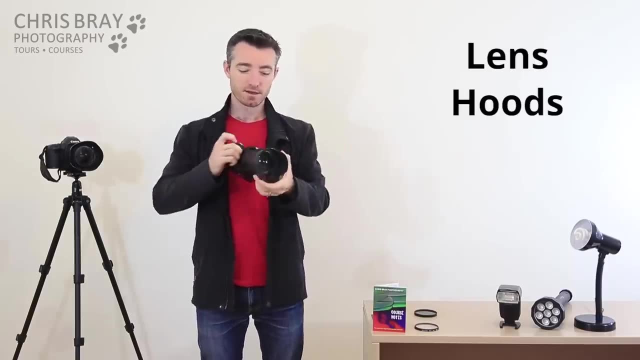 But in fact the sun can still see directly into the lens, So we're getting direct sunlight spilling across the front of your lens And we're still getting all those problems. So that's what these things are for: Lens hood. The whole point in life is just to shade the front of the lens. 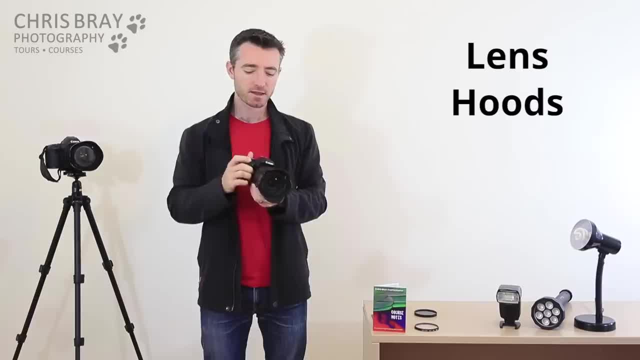 So you don't have lens flares, So you get to keep your nice rich colors, and so on. Now most lenses come with lens hoods And often times people just tend to forget about them Or they just leave them on backwards all the time. 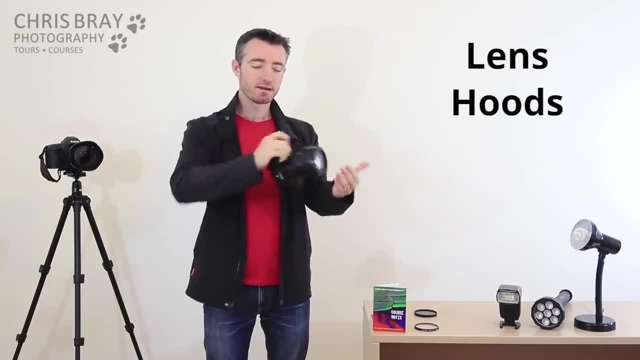 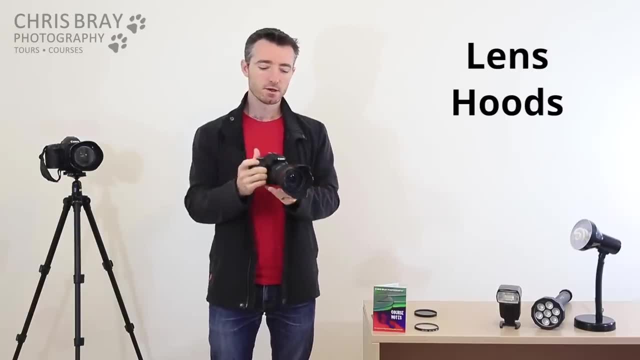 Which is a bit silly. That makes it smaller so you can put it into your camera bag, But every time you're photographing you really should get in the habit of getting it out and putting it on. It's almost never a problem. 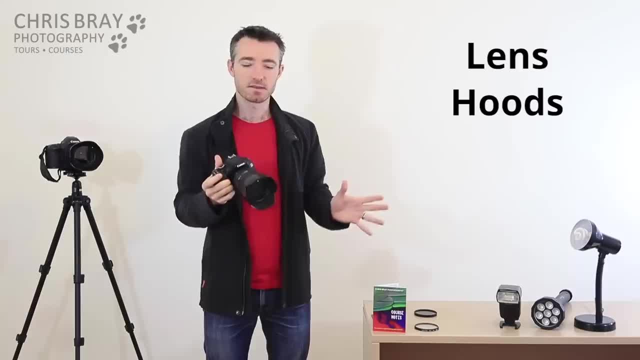 People think, oh, it's cutting out light and you might need that in low light or something. It's not true. It's only ever cutting out light that you don't need to photograph. It's just cutting out stray light coming in from the edge. 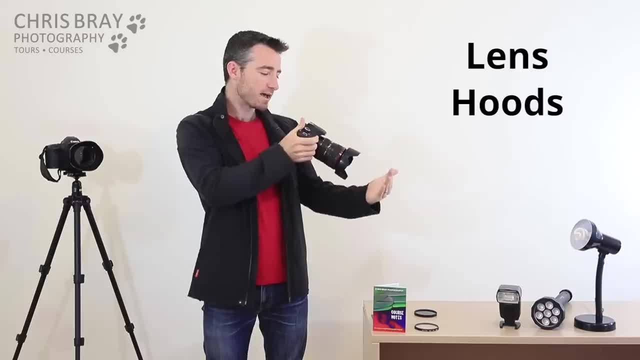 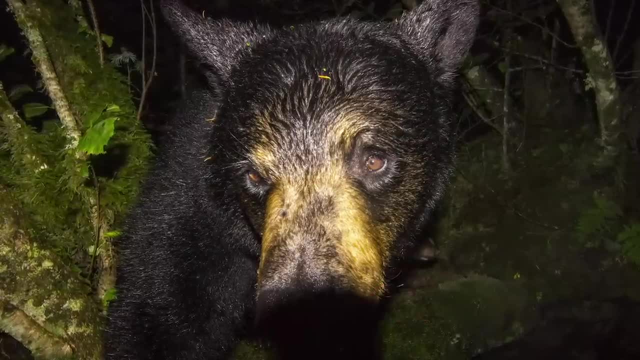 The only times you might ever want to take it off is if you're doing really close up flash work and you popped your little flash up and it couldn't quite see past the lens hood, So you end up with what's called a hood shadow on the bottom of your photo. 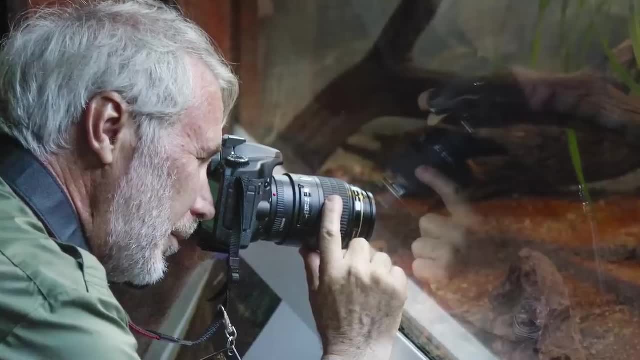 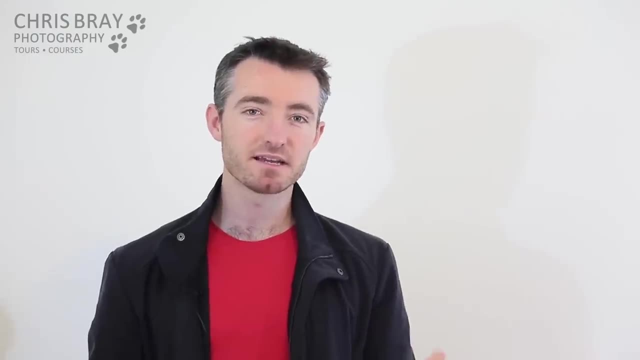 Or if you're trying to get that much closer to a window or something, then sure, then you can take it off, But in every other situation You should get in the habit of using it. So it's worth taking just a couple of seconds to think about lighting before you start taking. 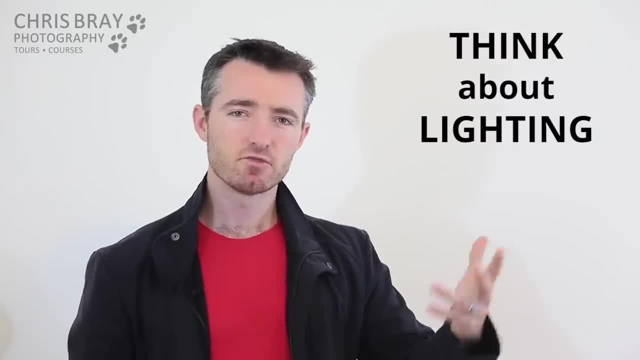 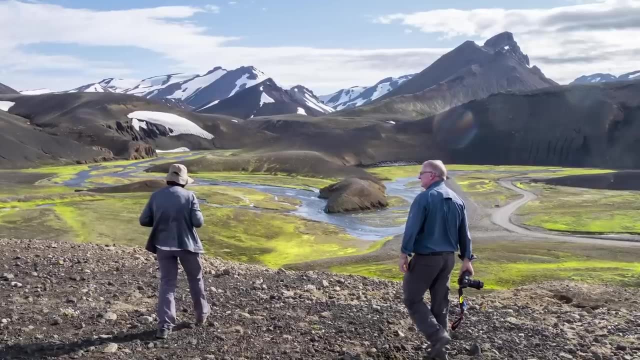 photos. You know, if someone asks you to take their photo in the sun, realize that they're going to be really harsh shadows. Go and find somewhere in the shade Or maybe, if there's no shade, look up in the sky and you might find that the only reason. 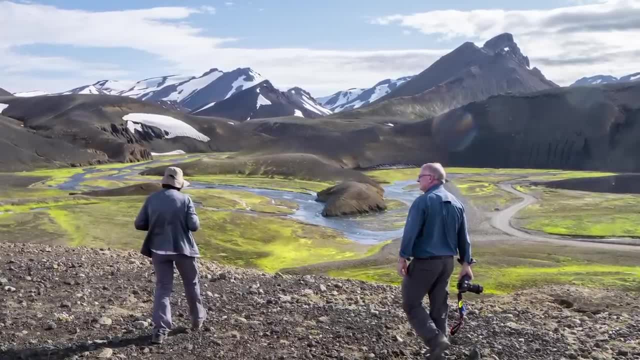 it's harsh sunlight just now is that there's a hole in the clouds, But it looks like if you wait about two minutes, there's going to be a big bank of clouds roll in front of the sun and then you'll be with nice cloud lighting. 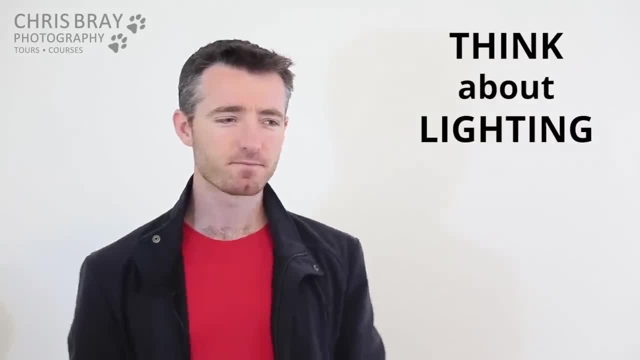 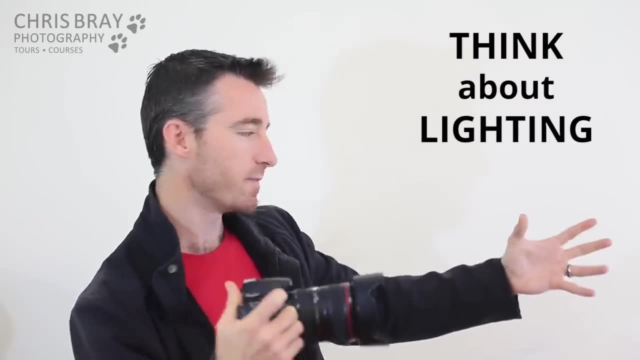 Totally worth waiting two minutes for some nice cloud lighting before you photograph, Or at least think about the direction of the light as well, Rather than having the sun over there and getting lens, flares and things, maybe bring it around here and shoot from that way. 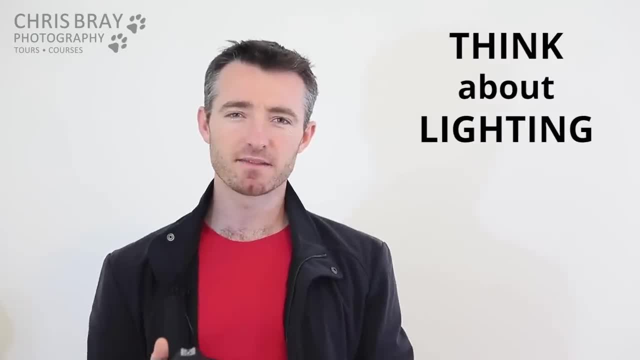 Then you get some side lighting, It looks more 3D. It doesn't take long to think about these things, but it can make a really big difference in how your photos look. Look at this example of a little beetle on a leaf. 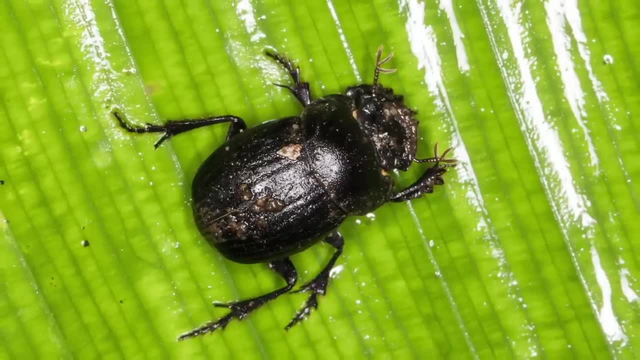 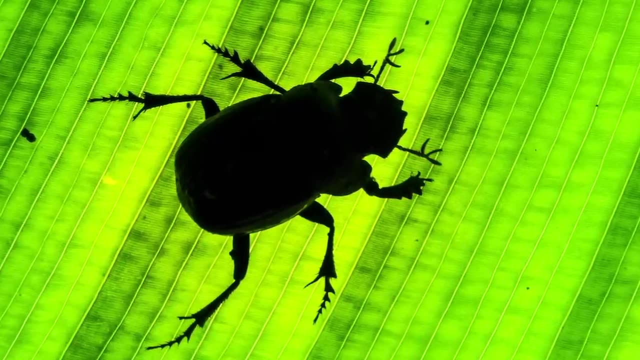 You can see that's just fairly boring top lighting. But instead if you turn the leaf up to the light and had the light coming through it, then you get beautiful colors coming through the leaf and there's a real silhouette of the beetle and it looks fantastic. 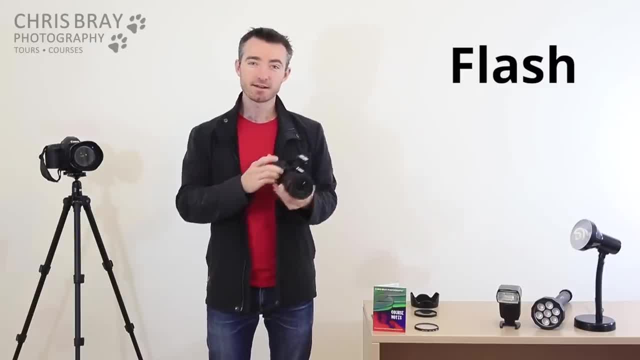 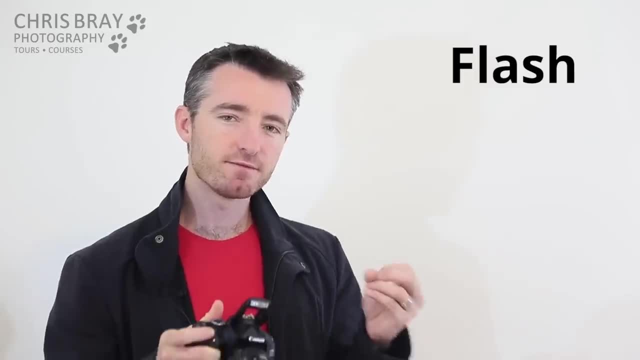 Okay, Let's take a look at photos. Let's take a look at flash. Definitely not just for nighttime use. In fact, I use my flash a lot more during the day than I ever do at night, Because if you use it during the day, you can fill in those harsh shadows caused by 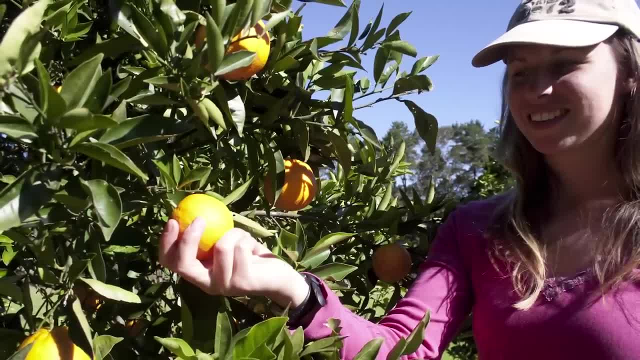 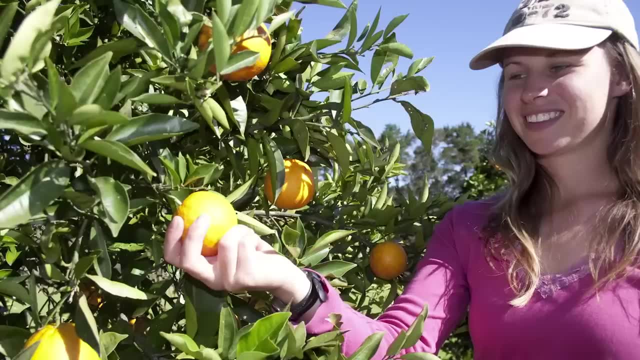 strong sunlight. This example is crying out for some fill flash. Look at those harsh shadows under the hat and it's just all so contrasty. But if we just pop the flash up, take the same photo again, that looks much better. And the great thing is it doesn't even look flash, does it? 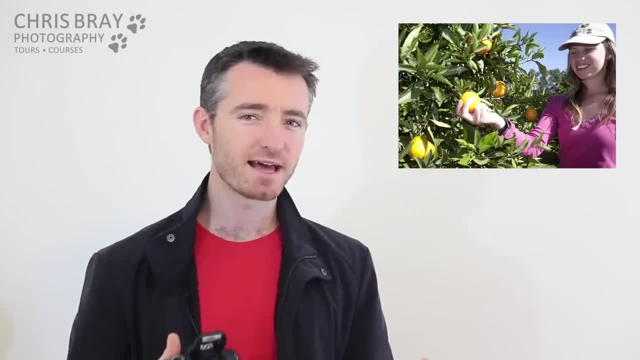 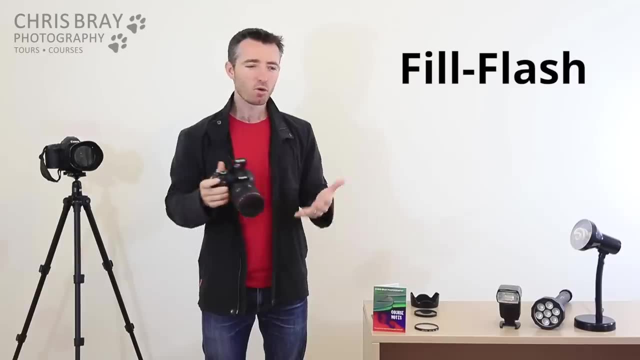 Looks quite natural. If you take a flash photo at night, normally it looks pretty flashed, But during the day you can just slip some light into the shadows there. When you're doing that, it's a technique called fill flash, And all of your cameras can do this. 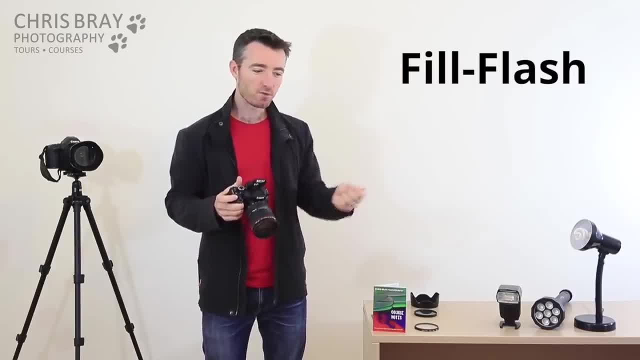 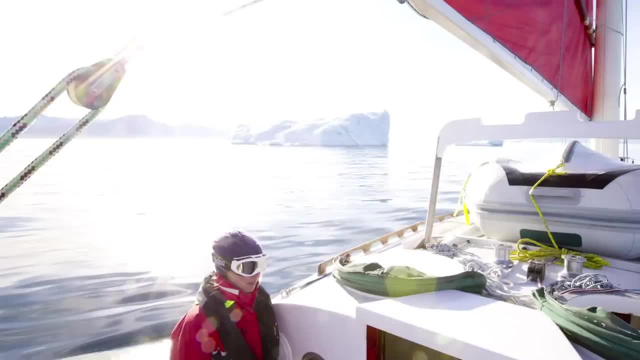 Even your compact cameras, even your smartphone cameras, you can normally force your flash on. Now you could just try and lift up the overall exposure until your subject was nice and bright, But by then the background would be completely blown out. So you're better off just popping your flash up, throwing some light in there and filling. 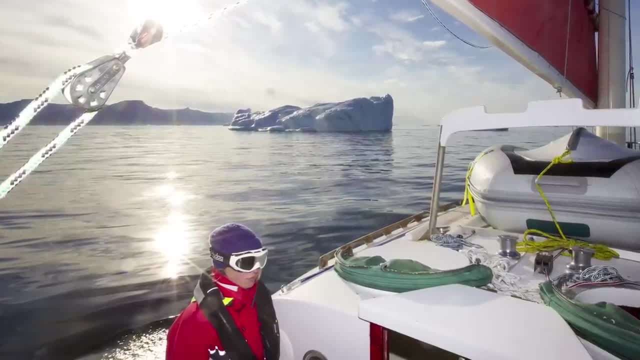 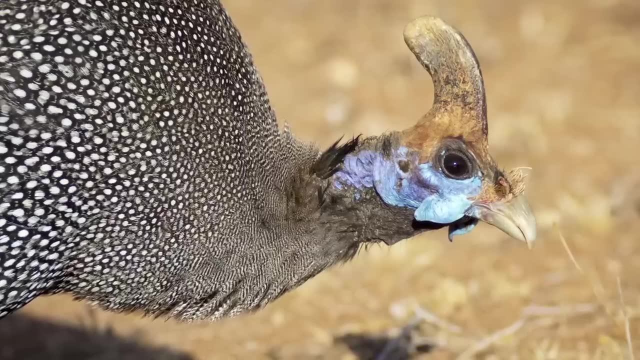 in those shadows to being the same brightness as the background, and then it all looks great. You can also use your flash to add a little glint or a sparkle Into the eyes of people or animals. It's called a catch. light Makes a big difference. 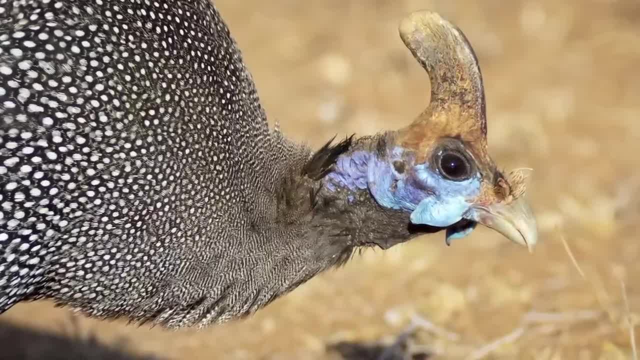 Just brings them to life a bit more. It doesn't have to be a flash, You just need to be able to see the reflection of something quite bright in their eyes. Could just be a window or something like that, But a flash is an easy way to try. 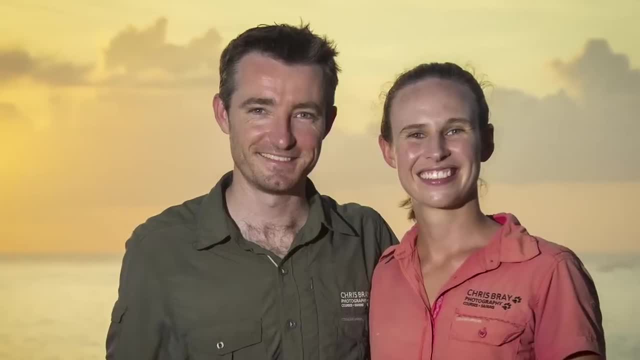 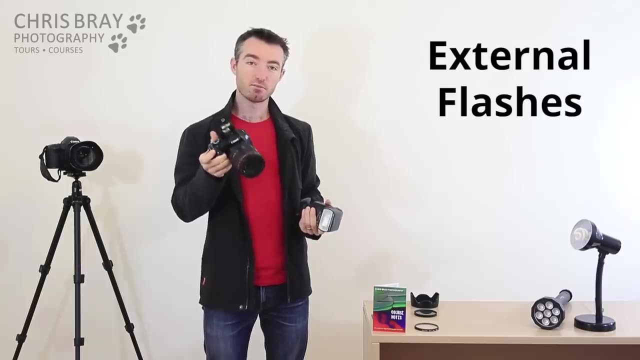 So maybe in the last of a batch of photos you've taken, pop your flash up. Just see the effect you get. Okay, we better have a look as to why on earth you'd buy one of these giant external flashes if you already have a little inbuilt or pop-up flash in your camera. 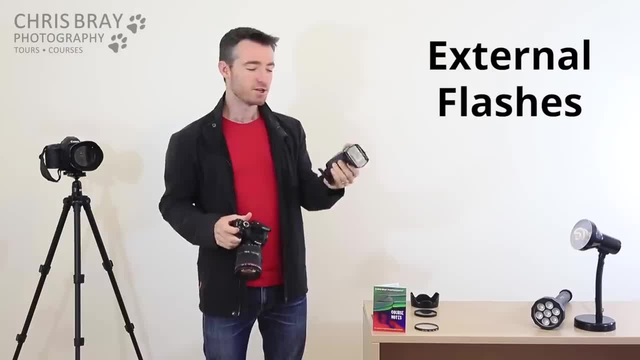 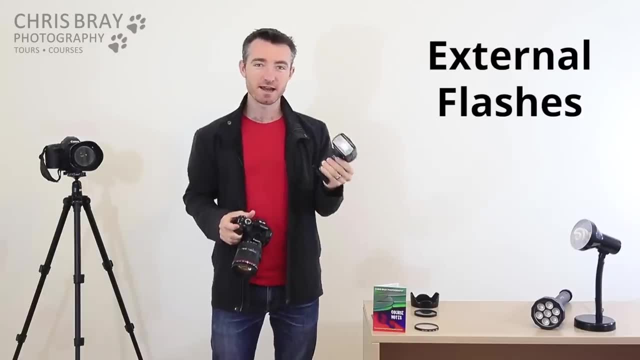 Most people just assume it's because these are obviously bigger, More powerful. You can penetrate the dark further. That's true, But that's actually not the main reason you'd buy one of these. It's because of the amazing creative lighting options these kind of things open up to you. 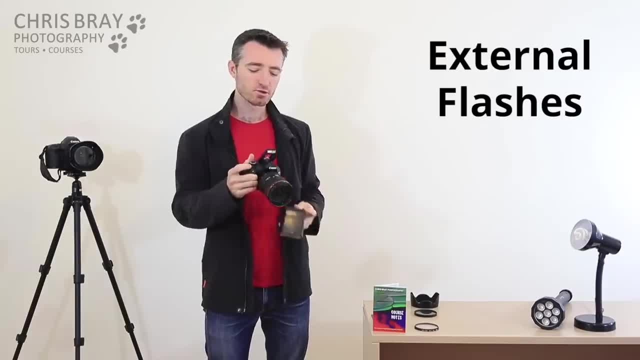 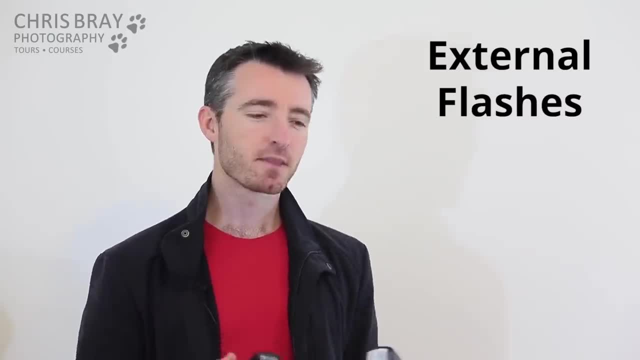 Because with a pop-up flash or an inbuilt flash, all you've ever been able to do is just harsh front lighting, And we saw before there's nothing nice about harsh front lighting. You know you get reflections and glare and it makes your photos look very flat and two-dimensional. 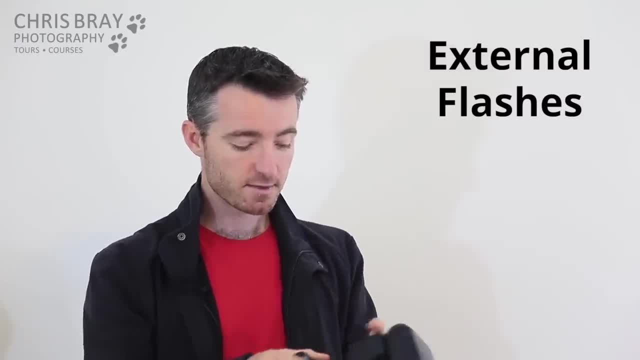 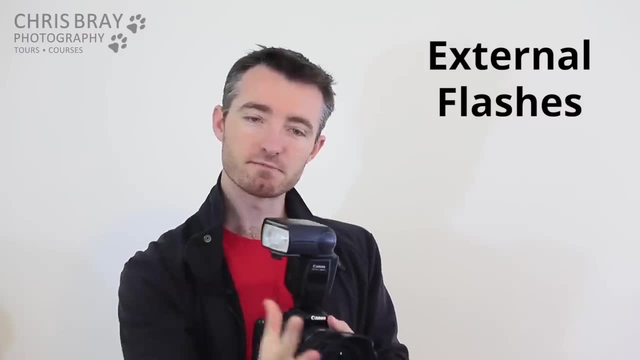 That's all you've ever been able to do before. But if you put one of these on instead, Then instead of harsh front lighting You can turn it to the side and get bounce flash. You bounce it off a wall and it drifts back, and then you've got soft side lighting. 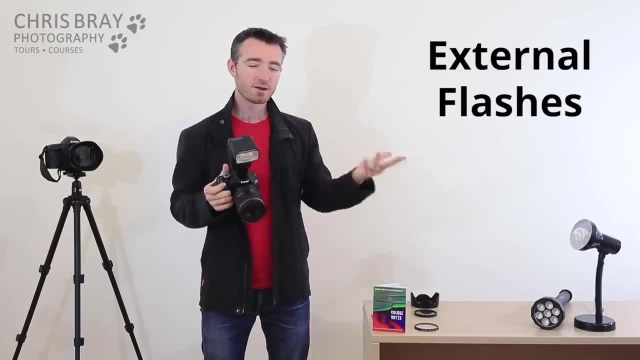 Of course you do need a wall or something to be able to reflect the flashlight off. No much good being outside and turning the flash to the side and hoping you're gonna get some light back, But in those situations you just take the flash off the camera. 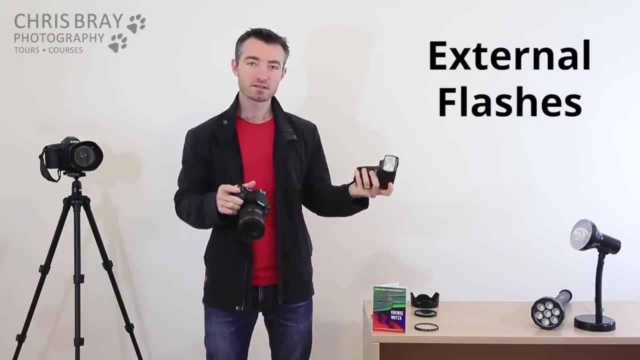 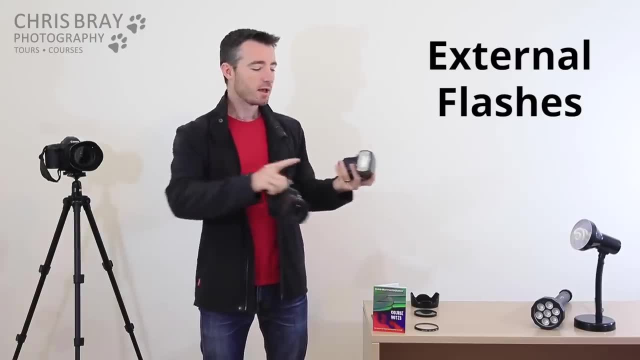 You know you connect it via a hot shoe extension cable or a lot of flashes are wireless now And that just lets you get the flash to the side a little bit to give you some side lighting, So your photos look more three-dimensional. Of course it would be fairly harsh because you've got a flash gun pointing straight at 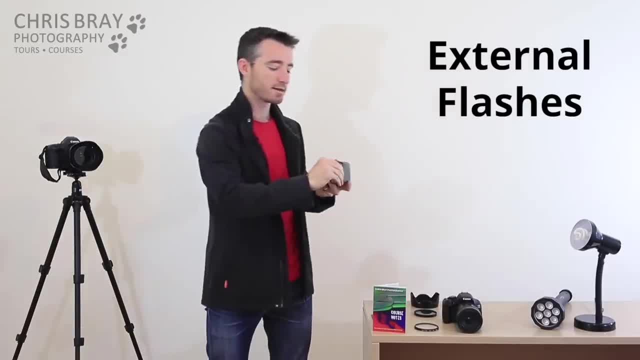 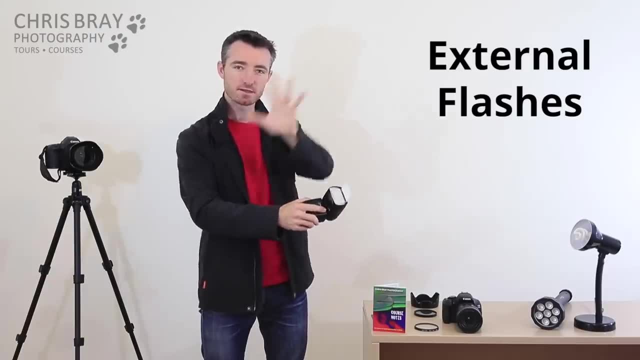 your subject. But what you can do in those situations then is just pull out a little flash diffuser or in fact a lot of flashes. you can buy big external plastic diffusers and they just make the light come from a softer, more gradual kind of area. 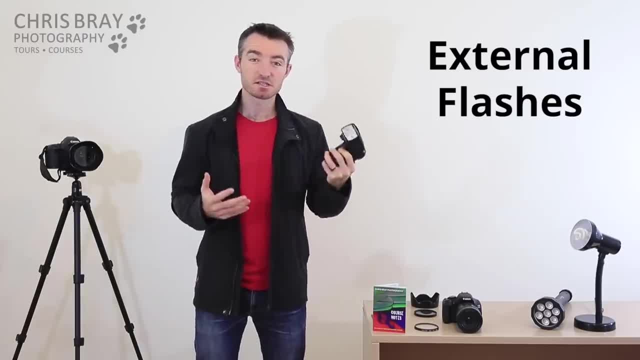 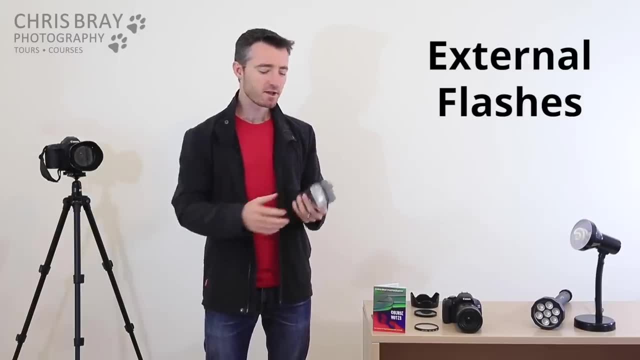 And you just end up with more three-dimensional photos. Using flashes these days is just so easy. It used to be quite complicated. You have to learn about things like inverse square laws and guide ratios and that kind of stuff, But these days it just does it all for you. 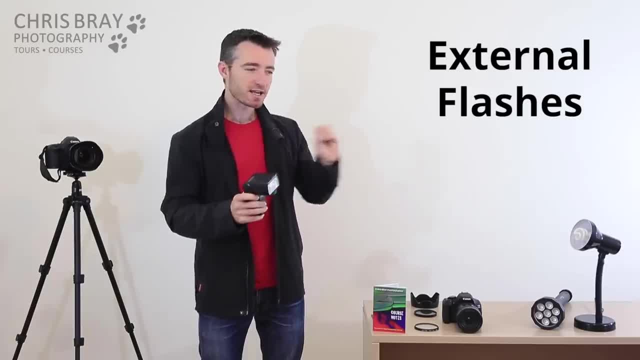 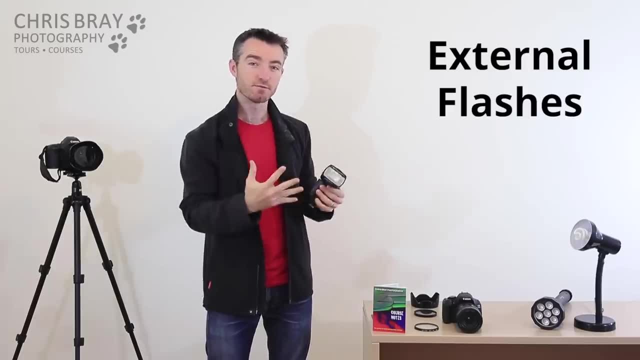 Modern ETTL flashes. In fact, when you take a picture, the flash actually sets off a little pre-flash first, and the camera looks at how bright that's made your subject and then adjusts the power of the flash for the real photo. So you end up with exactly whatever brightness you've asked for on your flash exposure compensation. 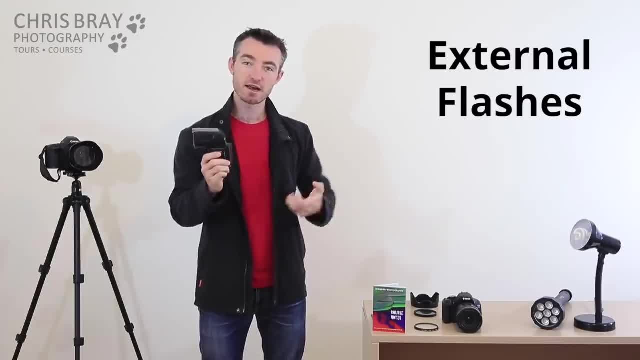 It's just so easy: Bounce flash, you know, you just turn the camera to the side and take the photo again and you'll still end up with the correct amount of light. Look at this example. So this is classically front flashed. 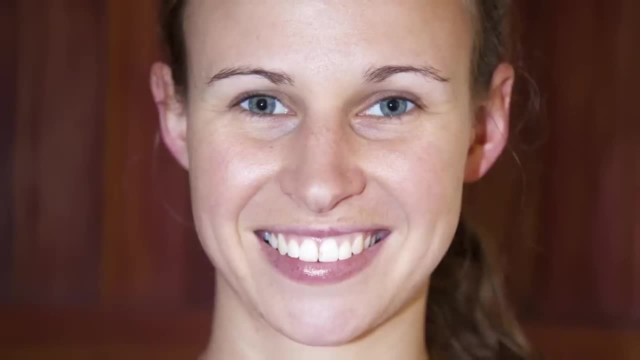 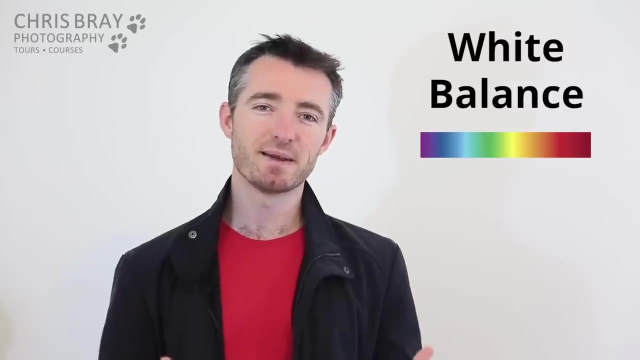 Looks like a stunned rabbit and looks a bit two-dimensional. But now just turn the flash to the side, Bounce it off a wall. You get nice soft side lighting. It just looks so much nicer and more 3D. Let's look at white balance. 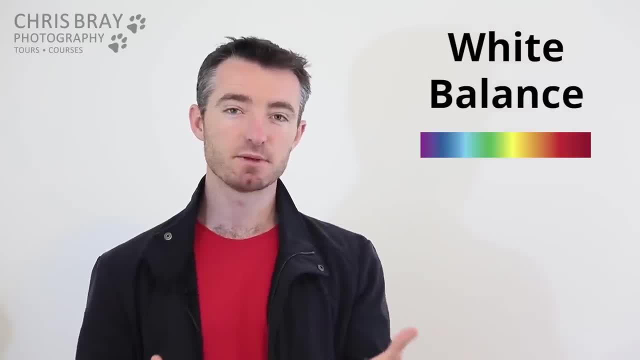 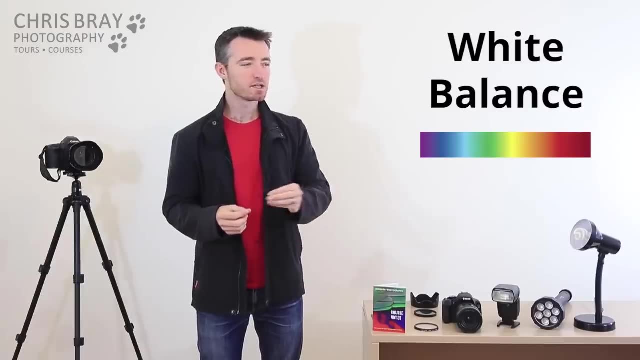 White balance is about making your colors come out correctly, Making things that are supposed to be white, making them come out looking white, not slightly blue or slightly orange. It's quite a tricky thing that your camera's got to do for you, actually because you're. 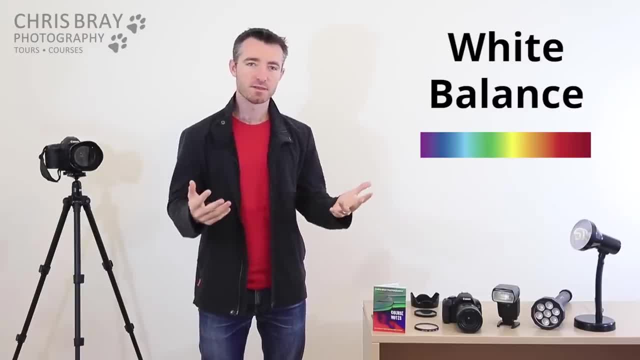 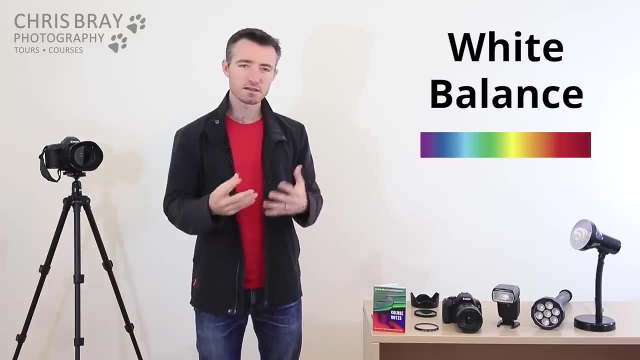 never photographing under pure white light with the entire spectrum in there. You know, most indoor lighting is a little bit orange Shade lighting is a little bit blue And if you use the wrong white balance setting, your colors just come out a little bit off. 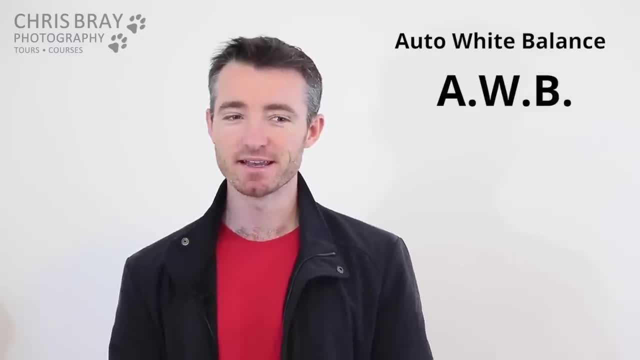 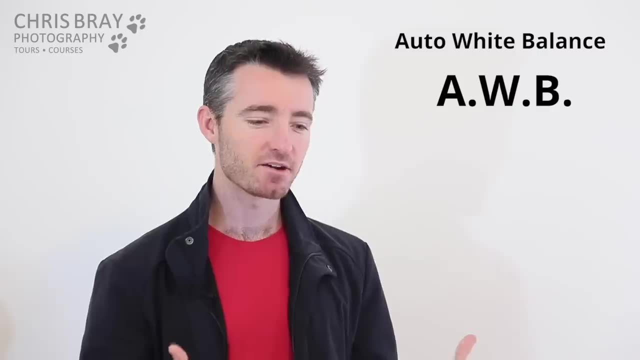 Now, thankfully, You have auto white balance AWB And honestly, that's the one you want to leave it set on almost all the time. Not only does it do a really good job at working out what kind of frequencies are lighter out there and adjusting it properly, but the main thing is it'll remember to check it every. 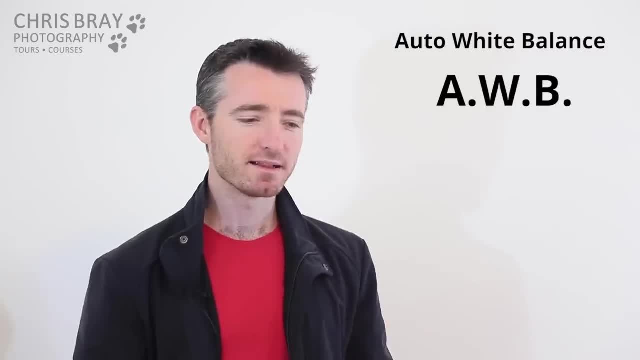 single time. You know you see people running around trying to set their own white balance and most of the time they just forget and you end up with photos with weird colors. But the reason you need to know about white balance is because eventually, your photos 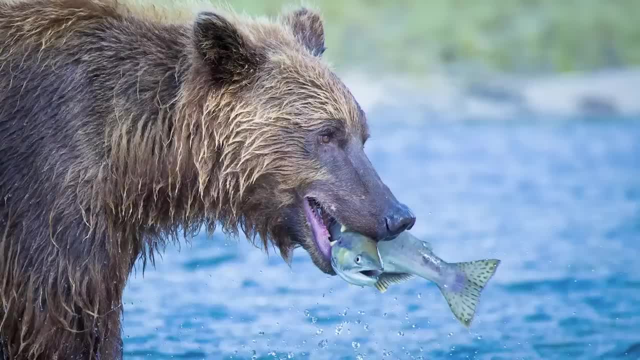 might start looking like one of these, If you ever find yourself thinking, gee, there's something weird in the color department. you're going to check your white balance setting and you'll probably find you've just accidentally slipped off auto white balance and you're on shade or tungsten or something like that. 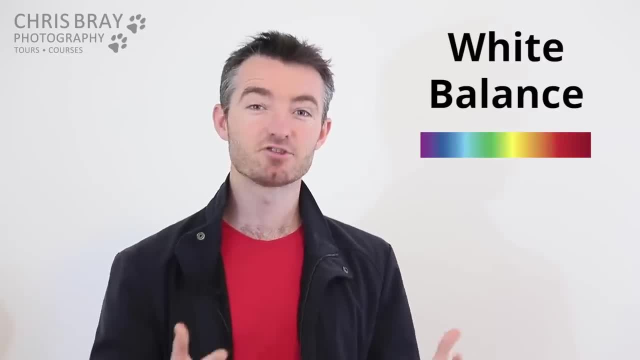 Put it back on auto, it'll probably fix it right back up If it doesn't. if you're literally on auto white balance and the colors are still weird, it's a pretty unusual situation. maybe the camera got tricked because there were two. 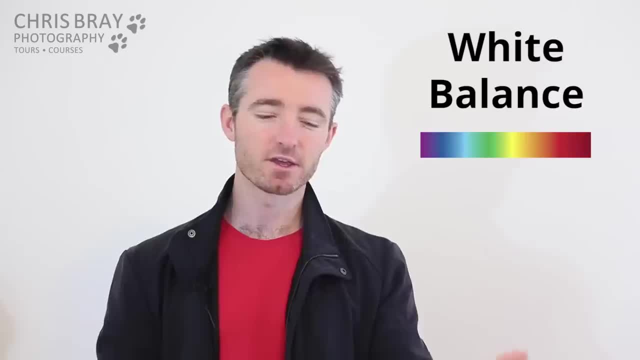 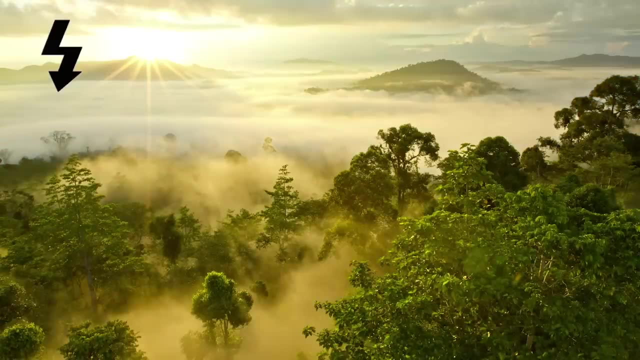 types of light around or something. then, and only then, would you bother going into your white balance setting and actually choosing one of those values: Tungsten, Daylight, Fluorescent Flash, Cloudy Shade- And if none of them are right, there's even a custom white balance in a lot of cameras. 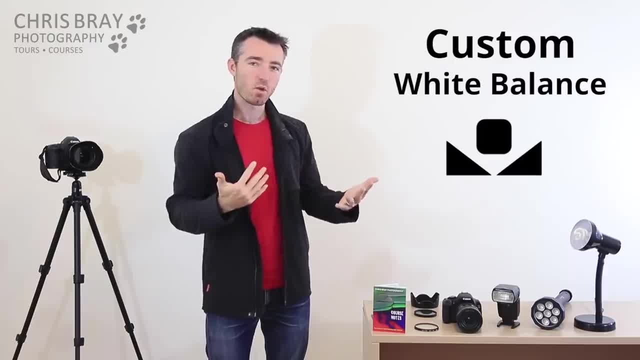 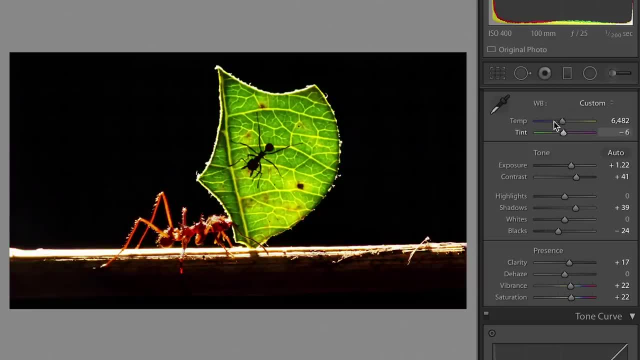 where you can just photograph something that's white and tell the camera to make that come out white and then it'll correct it for that. But I've never even really had to use that. You can tweak your color later on in post production as well, and if you're shooting. 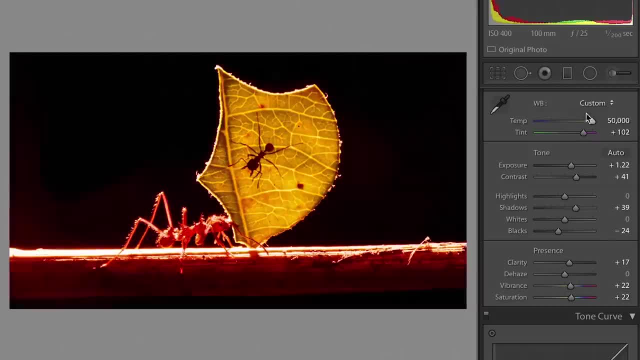 a raw file. it really doesn't matter. White balance is entirely an afterthought. you can choose it from a drop down list later on, So don't worry about it. just leave it in auto white balance most of the time and that'll. 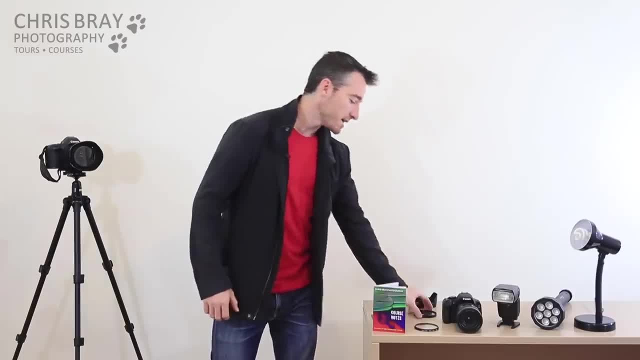 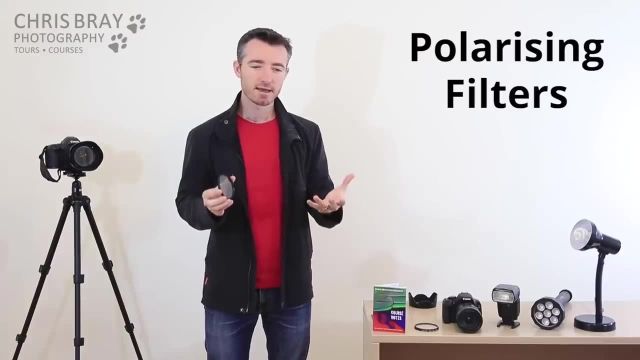 keep you out of trouble. Okay, let's take a look at filters now, Starting with polarizing filters like this one. Now, polarizing filters- just like polarizing sunnies. they help to cut out glare and reflections and things like that. 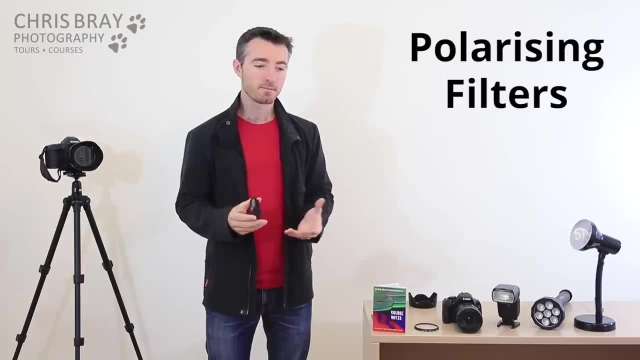 Can make the sky look a darker, richer blue clouds look better, leaves and things. Leaves are quite waxy and if you can get rid of the glare you end up with a deeper, richer green leaves in your landscapes. Really cool bit of kit to have, particularly for your wide angle lens, but you've got to. 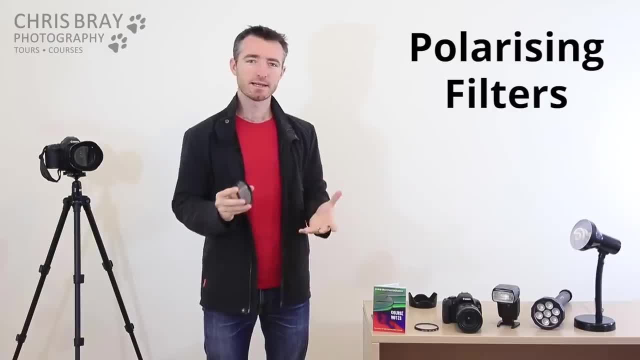 realize how they work. A lot of people buy them and just screw them onto the end of the lens and then forget about them. There's nothing wrong with leaving a polarizer on the end of your lens, it's not even funny. Firstly you screw it on, but you'll find the actual polarizing filter then keeps spinning. 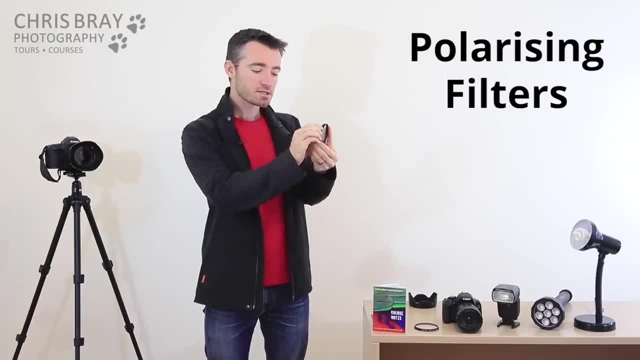 and you've got to set that every time you're taking a picture, Because as you twist it you'll find all the reflections disappear and then they come back again. And you've got to choose it because the lighting is different in every situation. 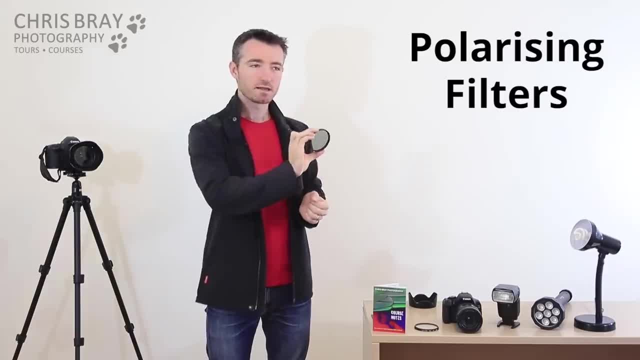 The other reason why you shouldn't leave it on is because it does make the world quite dark out there and your camera is forever going jeez, it's quite dark. the shutter will have to stay open longer to collect more light, So you end up with longer shutter speeds, more camera shake or you'd have to turn your. 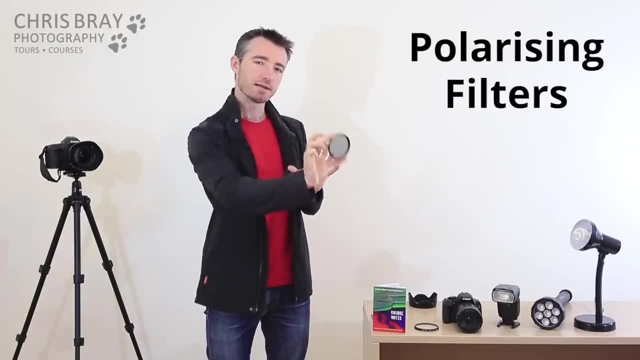 ISO up more And also every bit of glass you put in front of your lens, you're potentially reducing the quality of your lens. So you get what you pay for, particularly with polarizing filters. If you buy a really cheap one, take a photo, zoom right in, you might find your lens is. 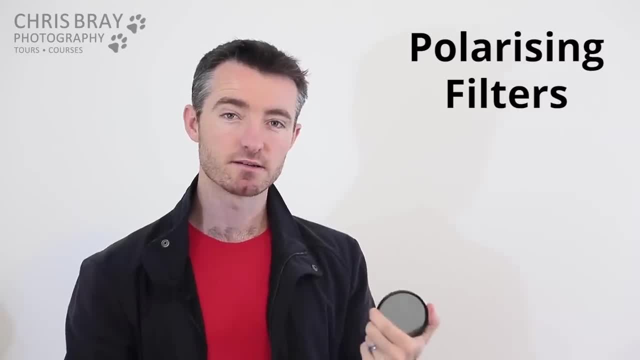 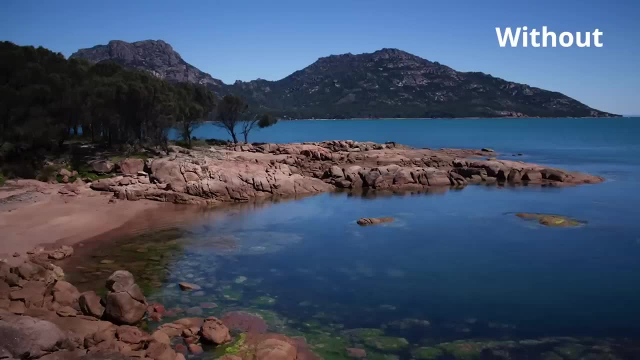 just not sharp anymore, So only put it on when you actually want to use it. but you can get really beautiful results. Have a look at this one. So here's a photo taken with and without the polarizer. When I say without, it is on there. I've just twisted it, so there's not much effect happening. 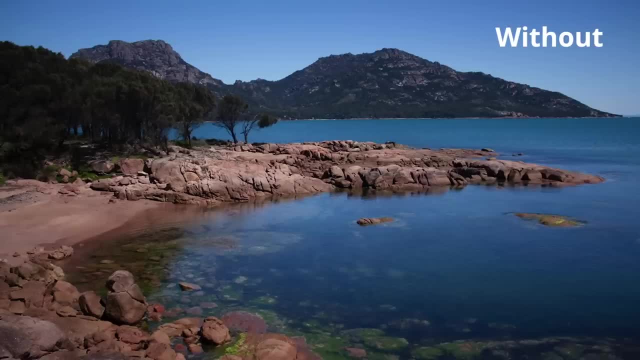 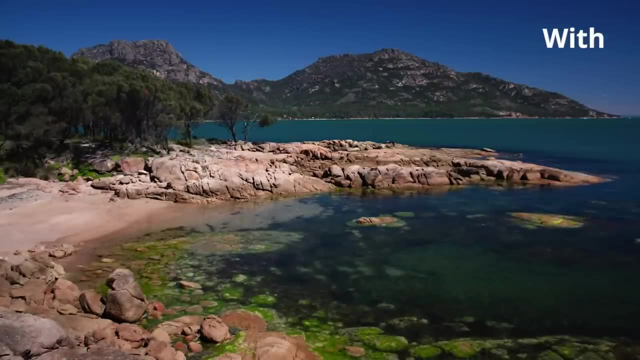 So you can still see all the reflection of the sky onto the water. so it's hard to see into the water. there There's a bit of that white haze in the sky, But if we turn the polarizer so the effect is more visible. now have a look. 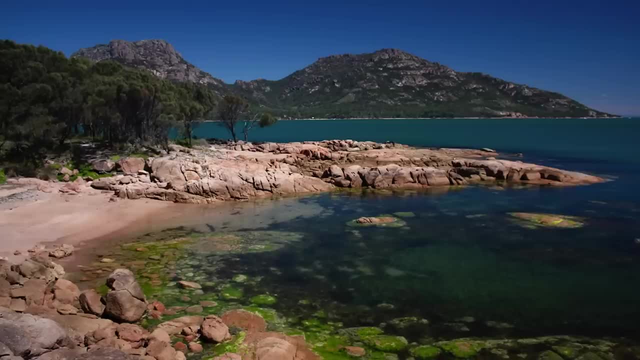 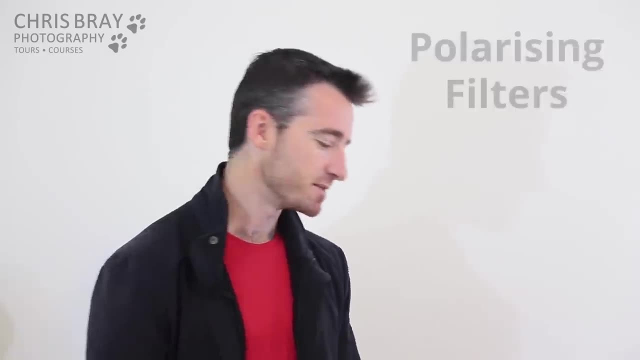 All the reflection disappears on the water so you can see straight in there And you're left with a darker, richer blue sky which looks great. Really cool bit of kit to have, but, as I said, only put it on when you actually want to use. 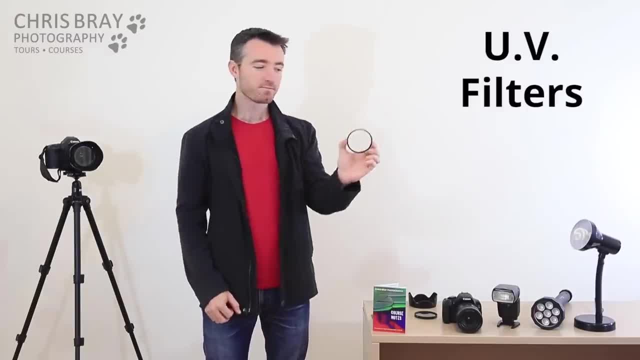 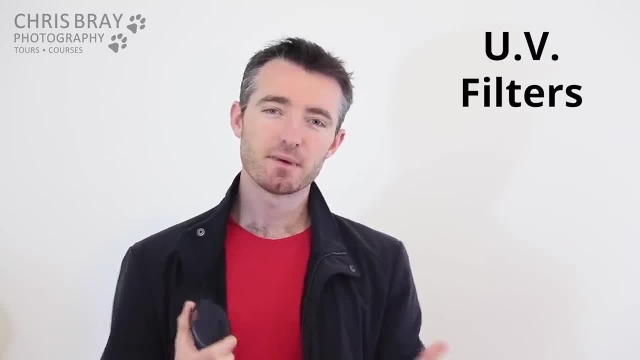 it, As opposed to these filters, the clear UV filters, These ones should be on your camera all the time. Now, a UV filter, not surprisingly, filters out UV light, But actually all of your digital cameras have a UV filter built into the sensor these days. 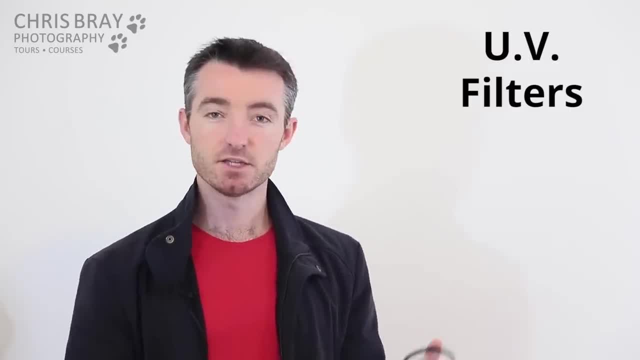 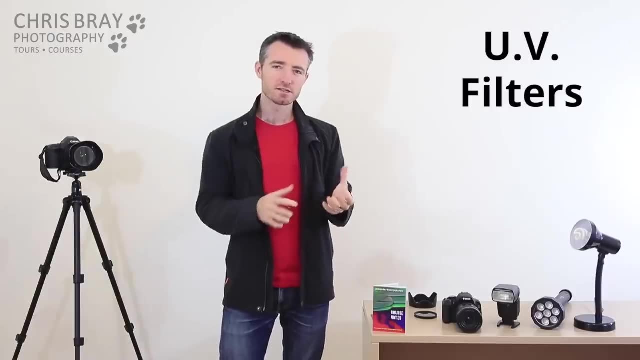 so the fact that this is filtering out UV light too, is a completely useless bonus, But the real reason why you should still all have one of these on is just because they protect the front of your lens. The front of your lens is actually really delicate. 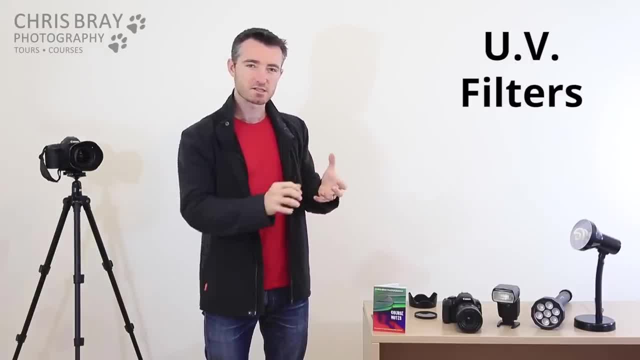 It's got very fine anti-reflective coatings on them that are very easily scratched And if you put your fingerprint on there it's quite hard to see. It's a bit of a pain in the ass. It's hard to clean the front surface of a lens. 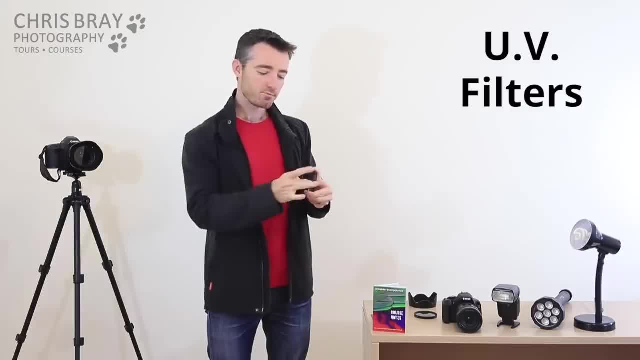 But if you put one of these things on there, not only are they very easy to clean, but they're pretty well bulletproof. It's actually quite hard to damage a UV filter, And if you do, chuck it out and buy another one. 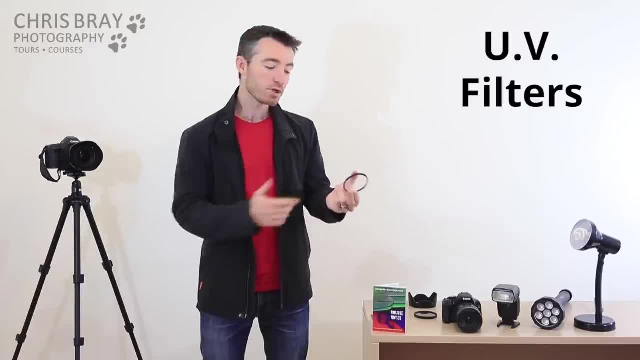 They're replaceable. They're much cheaper than the front of your lens, But again, you get what you pay for with these things. so if you've spent a lot of money for a really nice sharp lens, spend a bit of extra money and get a good quality UV filter. 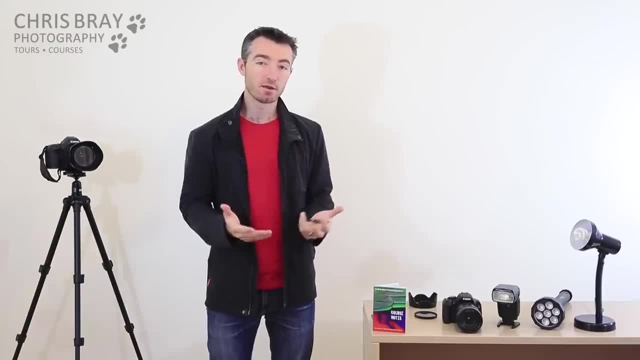 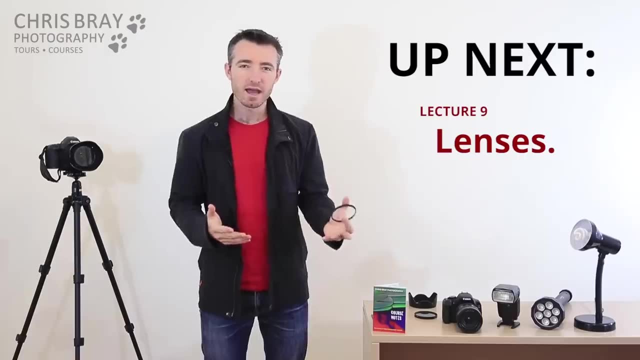 Otherwise you're just going to lose all that clarity again. So that's it for lighting. Next lecture is all about lenses: A bit of a handle on how you classify these things, what you're paying for, what the different features are, what they do and so on. 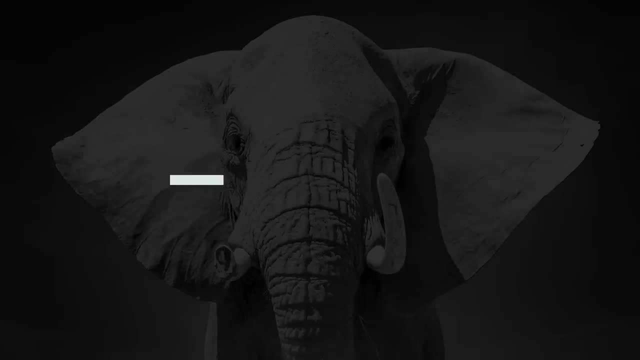 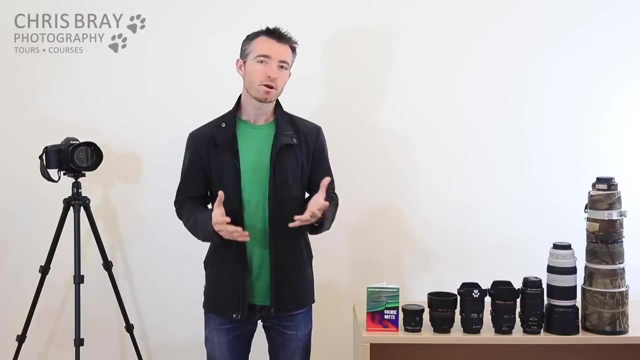 So thanks very much for watching this one and I hope you enjoy the next one as well. Alright, in this lecture we're going to look at lenses. There's obviously a million different types of lenses and it's a good idea to have a. 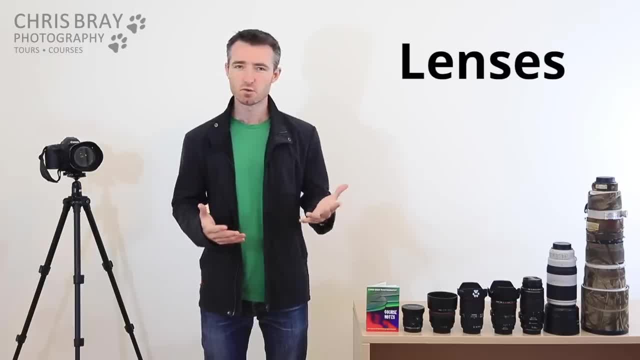 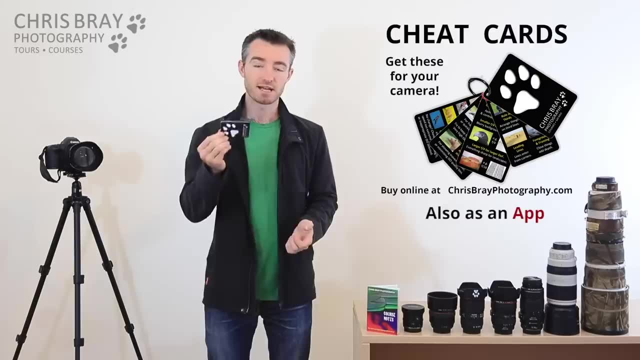 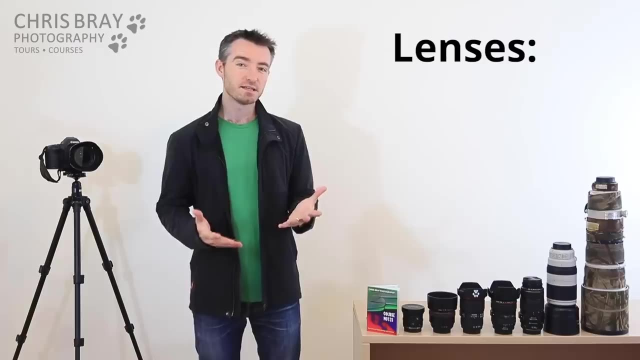 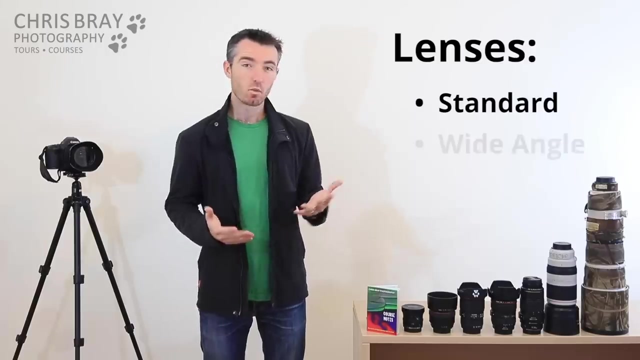 bit of a handle on how you classify them, what the different types do and so on. And just a reminder that there's a whole lens section in our course notes booklet as well that you can get online. Thanks for watching And I'll see you in the next one. 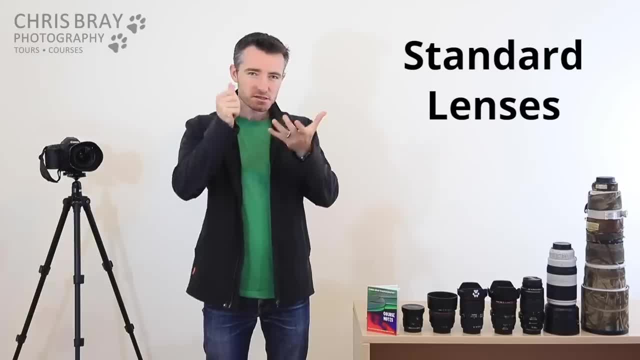 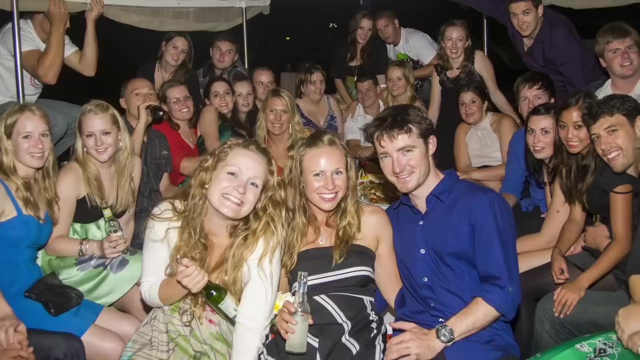 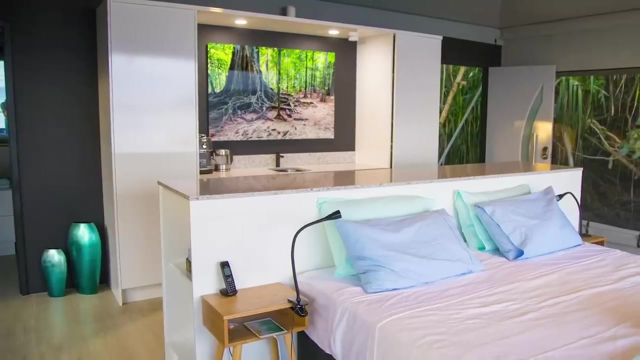 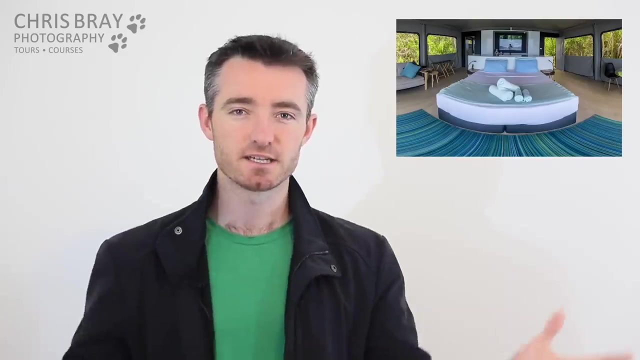 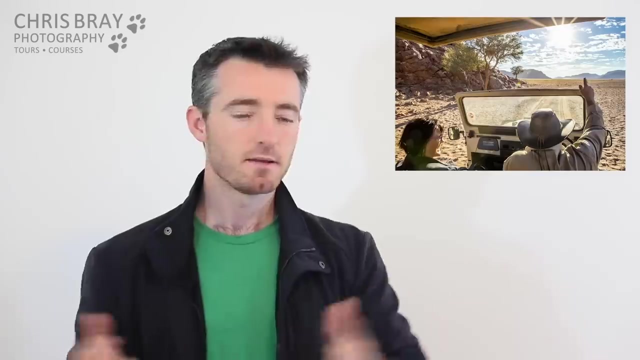 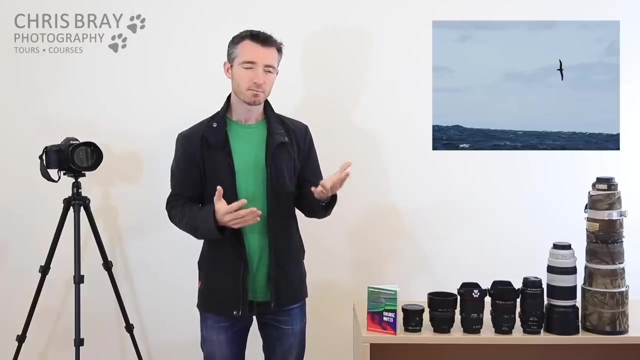 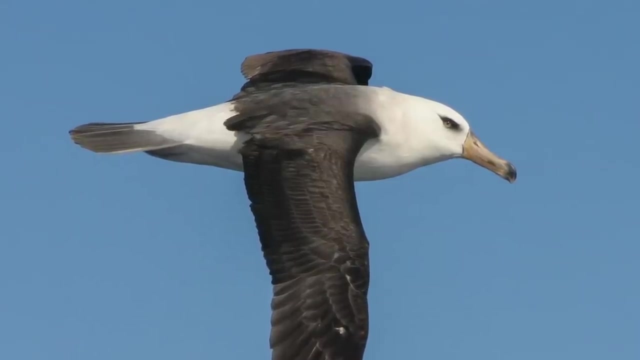 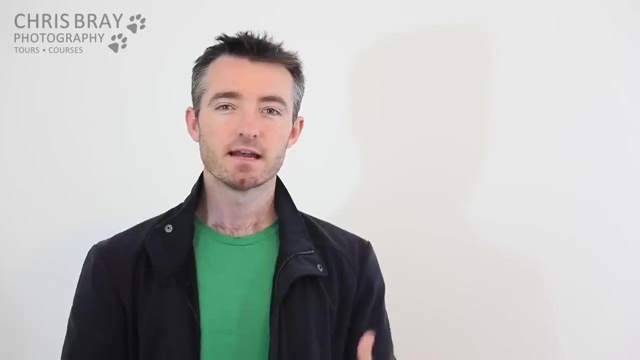 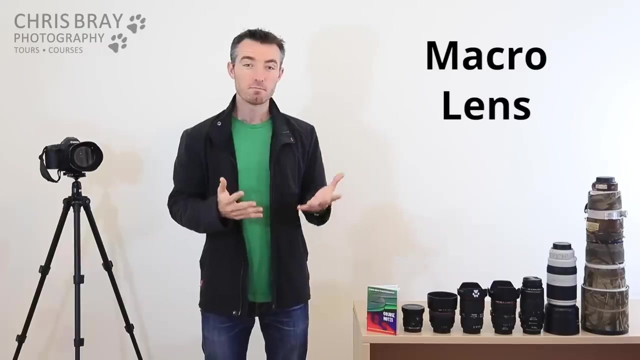 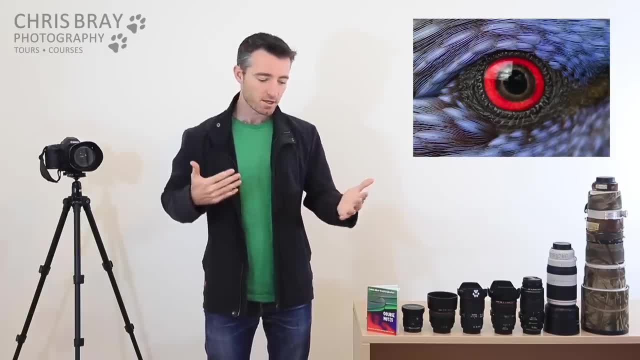 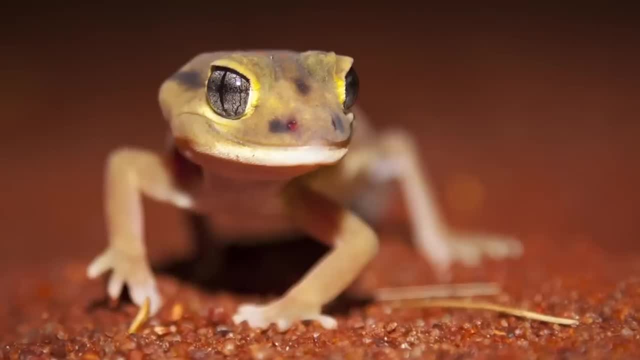 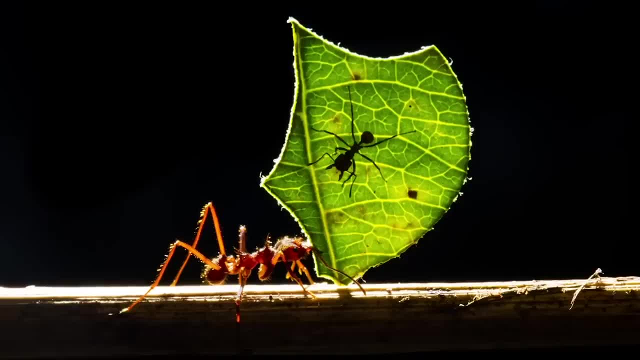 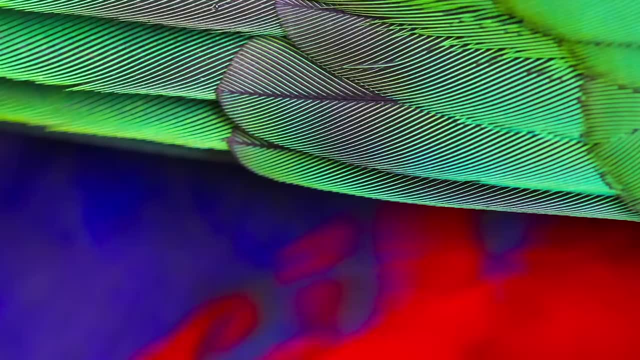 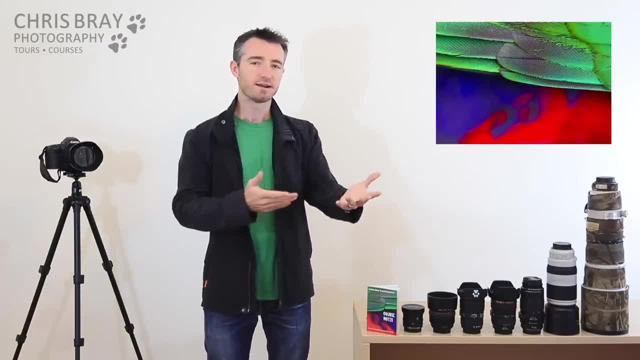 to buy next? you've got- maybe you've already got- a wide and a fairly long lens. what are you going to buy next? it's basically either a bit wider or a bit longer than you've ever had, but it's sort of more of the same. but really, a macro lens will open up a whole new world that you've never. 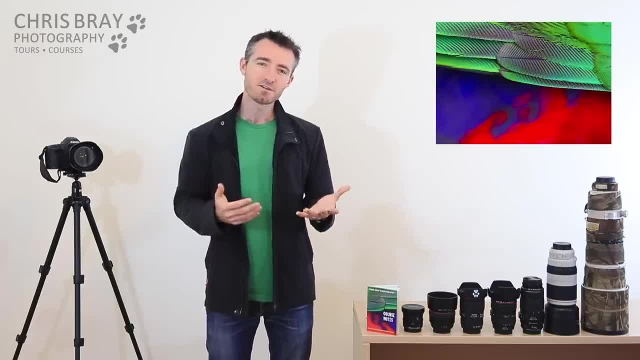 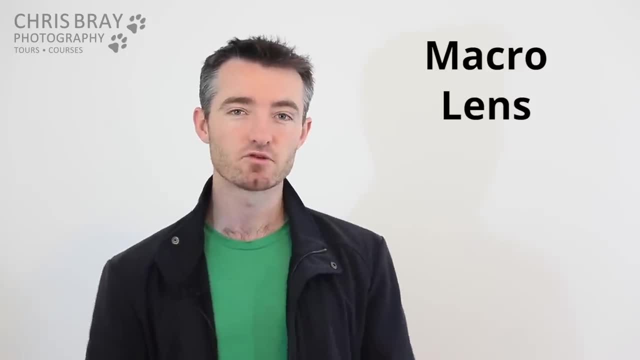 been able to experiment with before. i'd really recommend doing that. and don't forget, they don't only focus up close, it's a normal lens in every other regard. you can focus a long way away as well. in fact, they're excellent portrait lenses, because normally macro lenses go down to a nice small f. 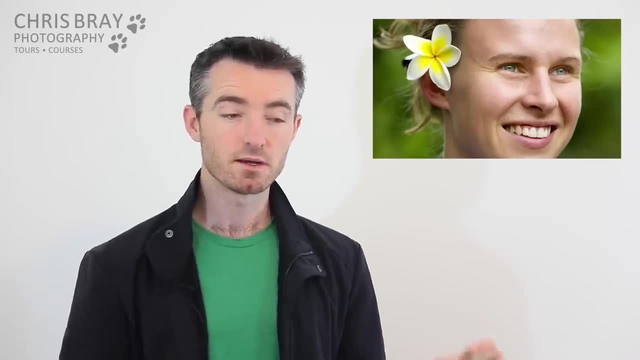 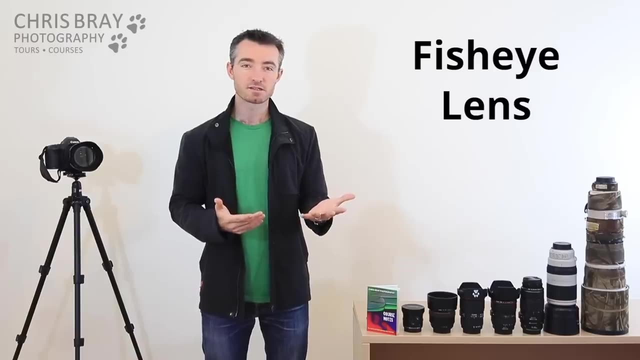 number about f 2.8, so that's great for portraits as well. small f number, small depth of field, beautiful blurry backgrounds. they're really nice lens to have. other interesting creative lenses would be fisheye lenses. they just give you a really wide angle of view, almost 180 degrees. 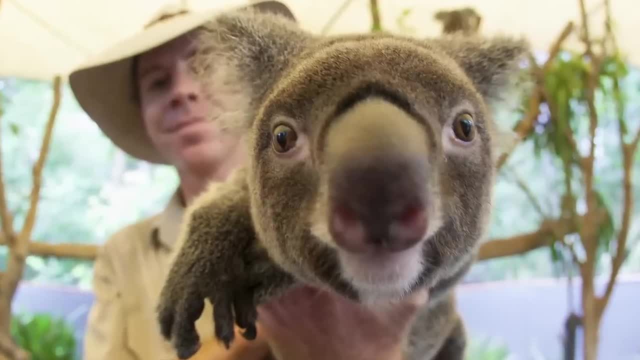 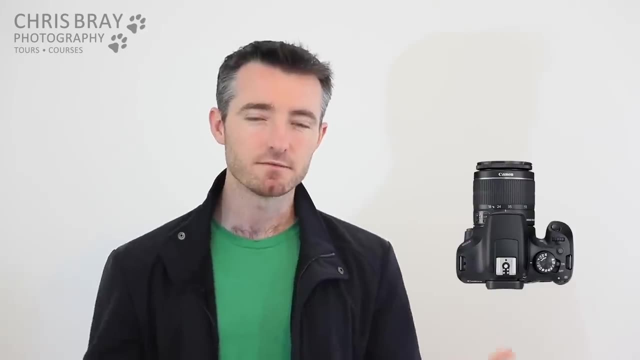 they kind of have a bit of a distortion or a bow on the horizon as well. tilt shift lenses- there's all kinds of other lenses that just do creative things really, but really it all depends on the angle of view that the lens can see. so if that was wide angle, that, 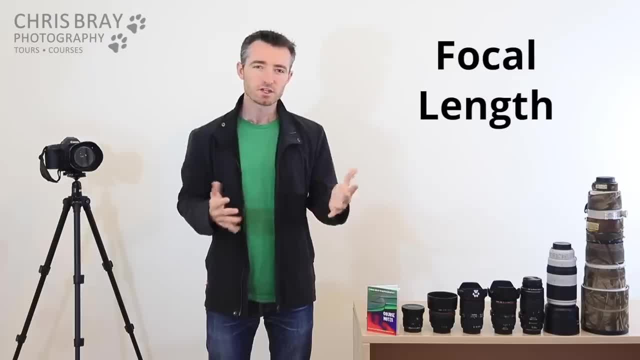 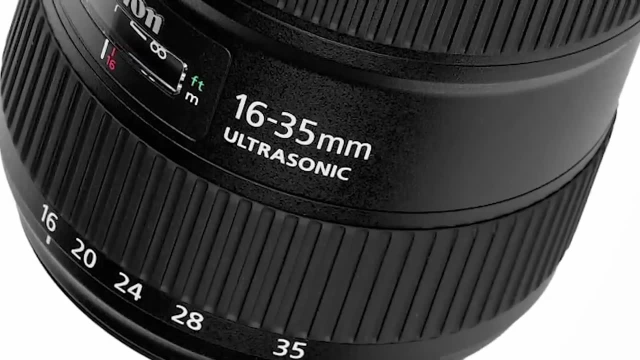 might be standard and that might be telephoto. but the way you measure the angle on the lens is with what's called the focal length. so if you pick up a lens it'll have a measurement written on there. it might be 16 to 35 millimeters and you'll see they're going 16 to 30. what does that? 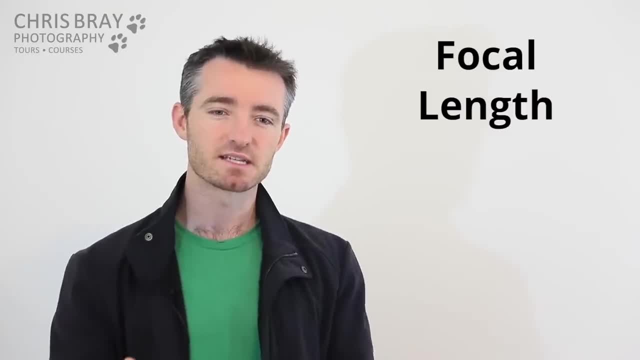 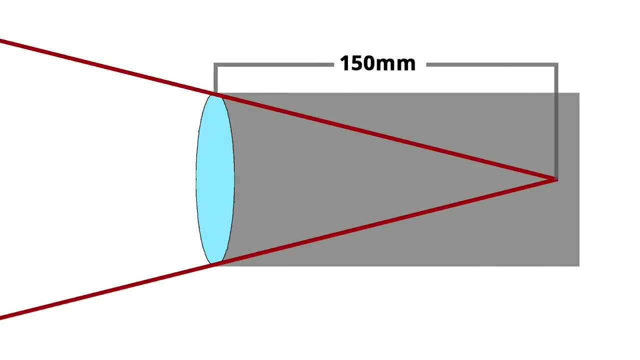 even relate to. focal length is just a measure of how the light is focused inside the lens. you can see, if this was a 20 mil lens then maybe this would be a 50 mil lens and that would be 150. but you get the idea. the longer the focal length, the kind of narrower the field of view, the more 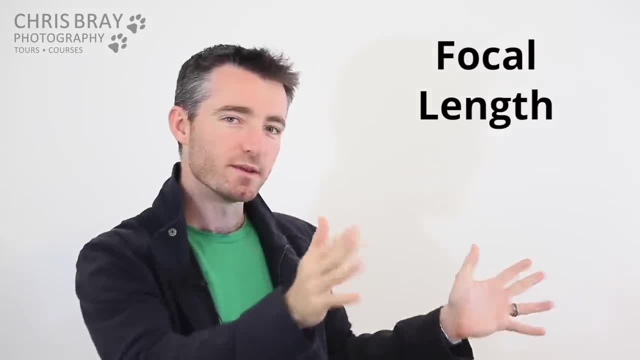 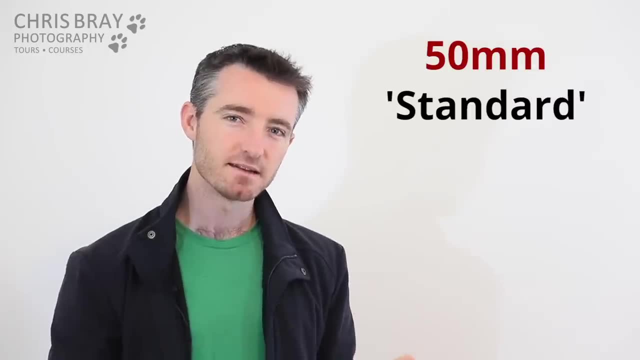 like a telescope, and the shorter the focal length is, the wider the view becomes. but it's the only thing you really need to try and remember is that it's all centered around 50 millimeters. that's standard, that's the normal value. so 50 millimeters, that's what the human eye sees. 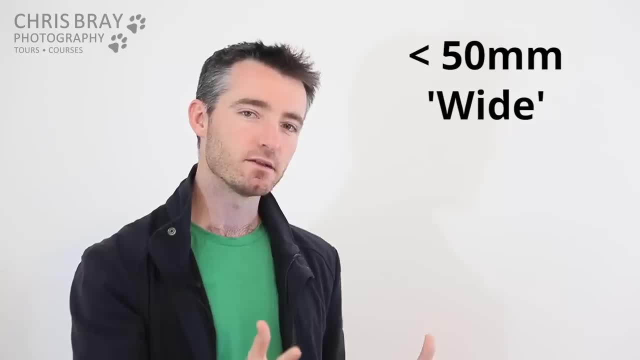 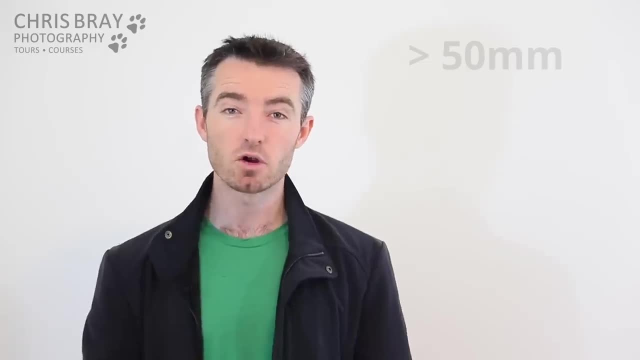 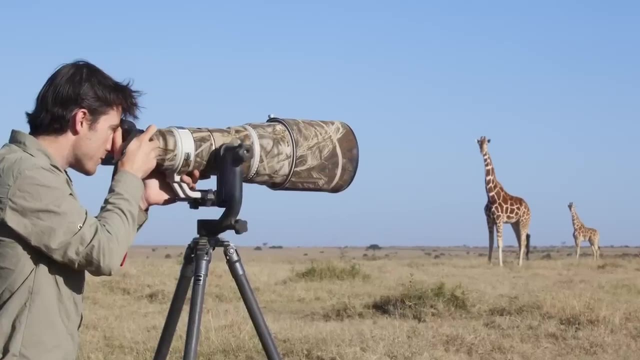 so anything shorter than a 50 mil lens becomes a wide angle lens. 24 millimeters, that's a wide angle lens, 10 millimeters super wide. anything longer than 50 mils is then a telephoto lens. so 100 mils a telephoto. 200, 400, 600 millimeters is a super. 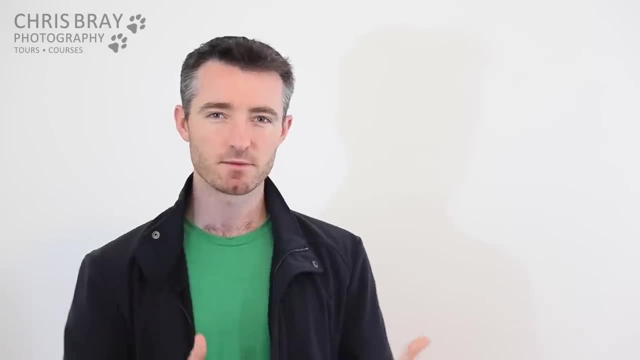 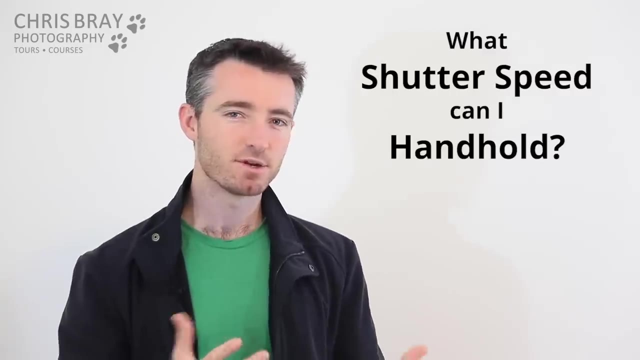 telephoto lens. so this brings us to a useful little rule of thumb that some of you might find useful. people like to know what shutter speed can you get away with hand holding you know? when do you really need to dig out a tripod? no one likes tripods. there is no one flat answer for it. it. 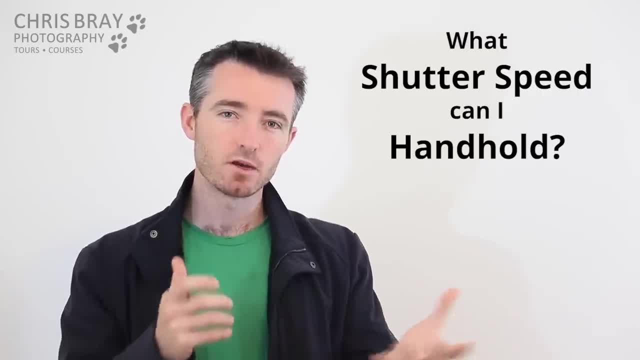 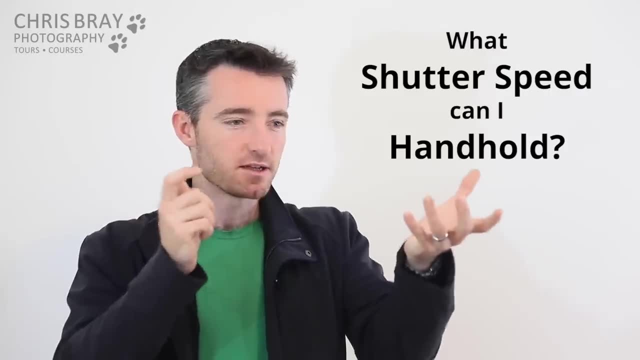 depends on your focal length of the lens, depends on how much you've zoomed in, which kind of makes sense if you think about it. if you've ever used a really long lens or a telescope and tried to hand hold it- your own handshake is just sort of jumping around everywhere and to get a sharp shot. 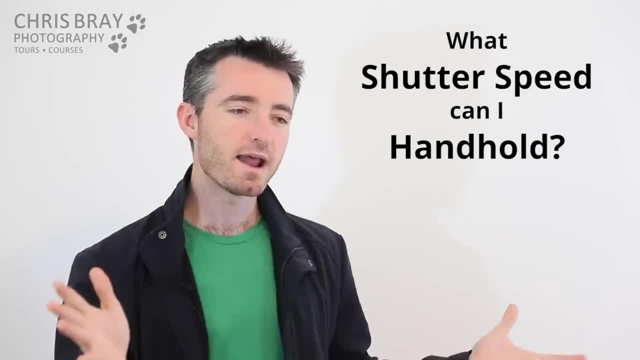 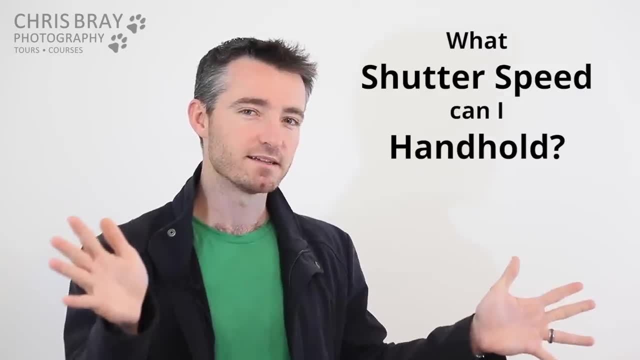 with that you need a super fast shutter speed. but if you have a really wide angle lens you can wobble around and you barely see anything change. so you can actually get away with quite long slow photos for a wide angle lens. so basically the rule of thumb is try not to hand hold anything slower. 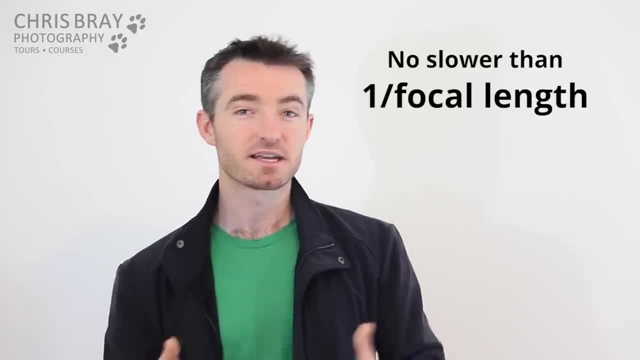 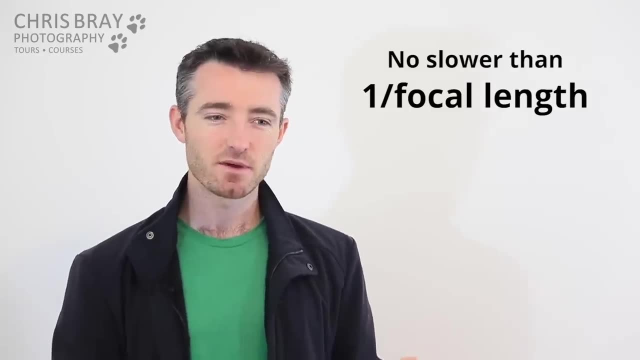 than one on the focal length of the lens. now, i know that sounds like an einstein equation and people tune out as soon as they see a fraction, but it's actually really easy to use- and it's not exact science anyway, because things like stabilizing comes into play as well- and whether 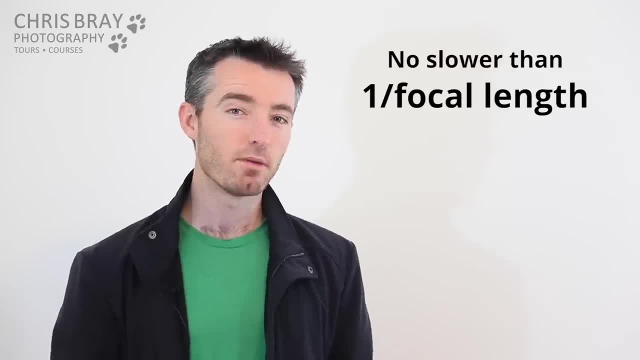 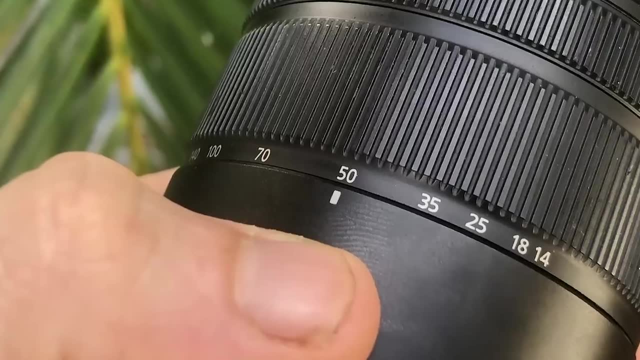 you've got a full frame or a crop body, all this different stuff, but it's still a good ballpark gives you an idea. so it's saying, if you're using a 50 mil lens or you've zoomed your lens in until it has about 50 on its focal length measurement, there you'd want about a 50th of a second to be. 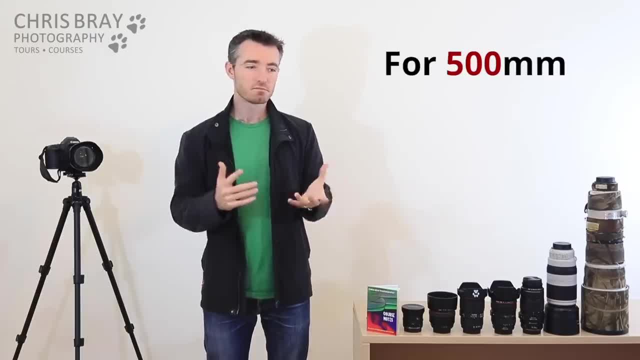 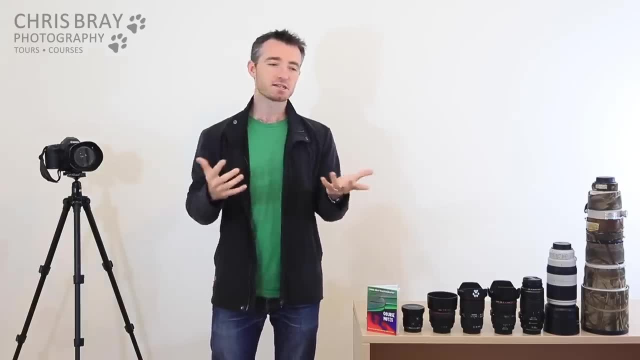 able to get away hand holding it. but if you're using a 500 mil lens, so a telephoto lens, then you'd want about a 100th of a second, otherwise you're going to have camera shake. it makes sense. it's just saying the longer the lens is, the more it's going to be wobbling around, so the faster you. 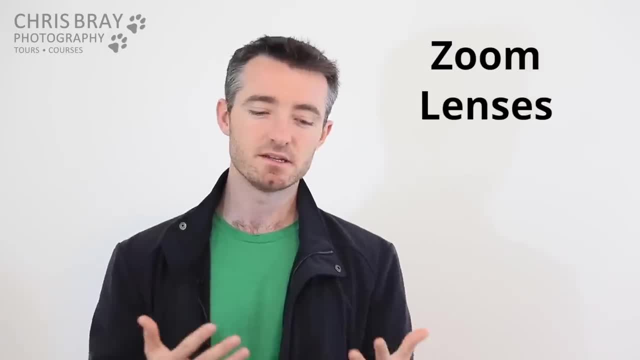 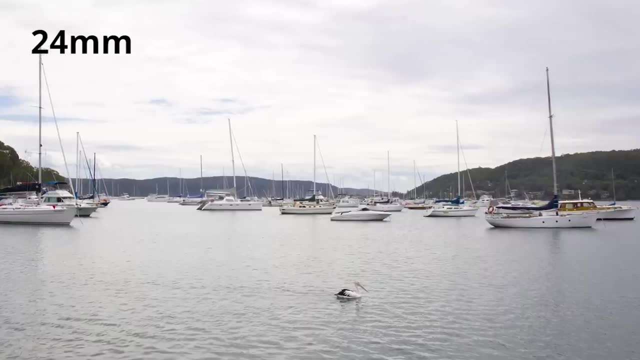 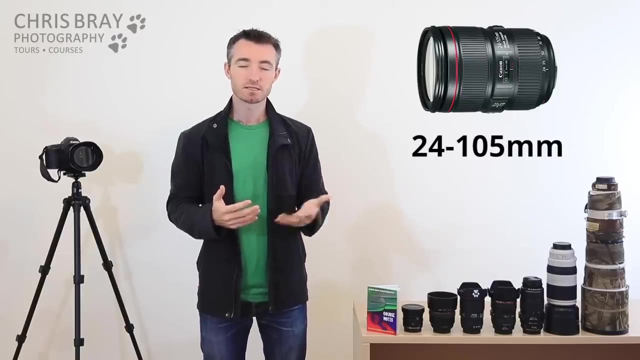 need to be if you're going to try and hand hold it. so what are zoom lenses? zoom just simply means you can zoom between different focal lengths. so this one, for example: 24 mils to 105, 24 being wide angle and 105 being a bit telephoto. so that's quite a versatile lens. i leave that lens on my 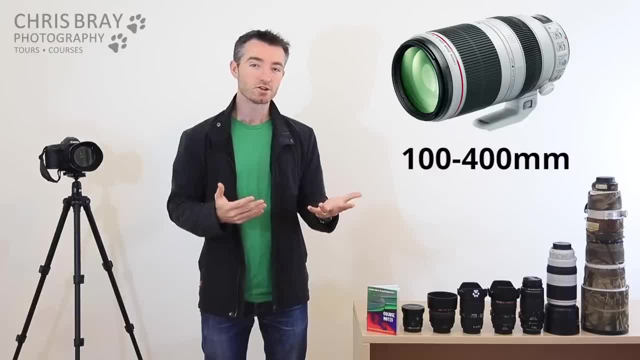 camera a lot of the time until i've got a reason to put something else on, like this lens, which is a 100 to 400 millimeter lens. so that's telephoto to super telephoto. that's an excellent lens for sport or wildlife. it's really convenient. a lot of guests will take this kind of lens on on photo. 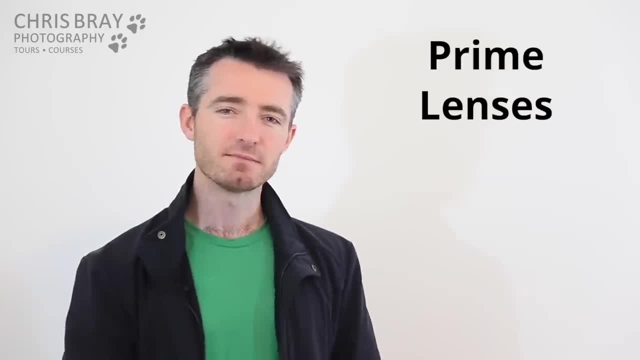 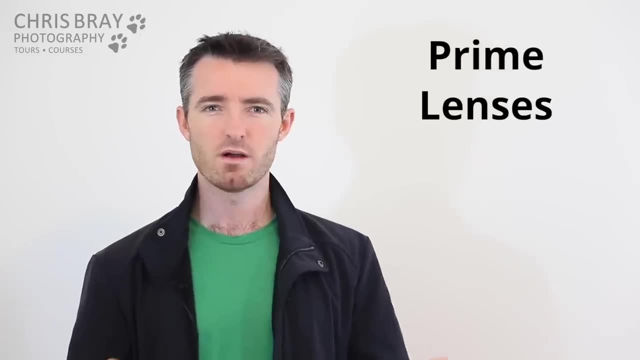 tours with us. what about lenses that can't zoom at all? they're called prime lenses or fixed focal length lenses and often confusingly, they're even more expensive, and i used to think: why would you pay so much more for a lens that you can't even zoom? what's going on? well, it's basically because 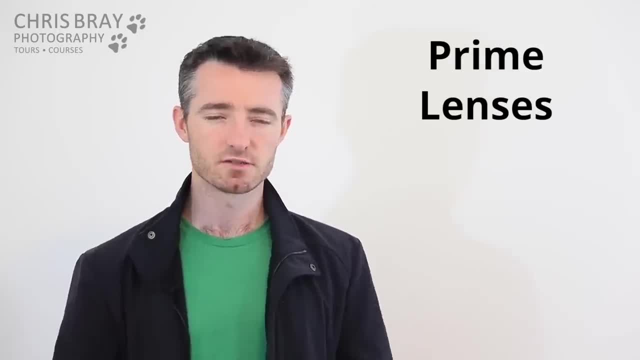 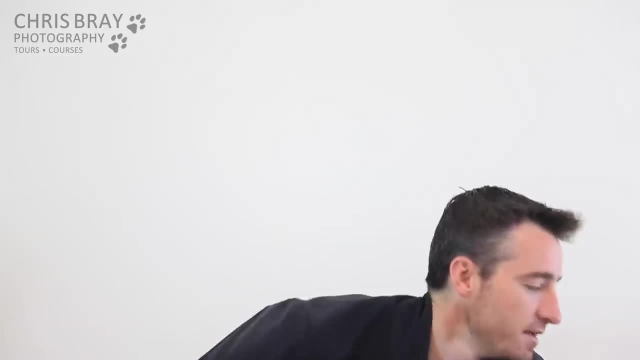 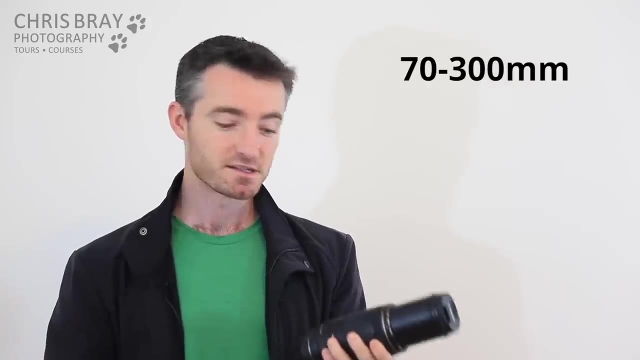 as soon as you allow a lens to zoom, you introduce all kinds of problems. you know, the highest quality lenses are the ones that are designed to do just one job and do it perfectly. take a look at this one. so this lens is trying to be a good 70 mil lens. it's also trying to be a good 300 mil lens. you know they're completely. 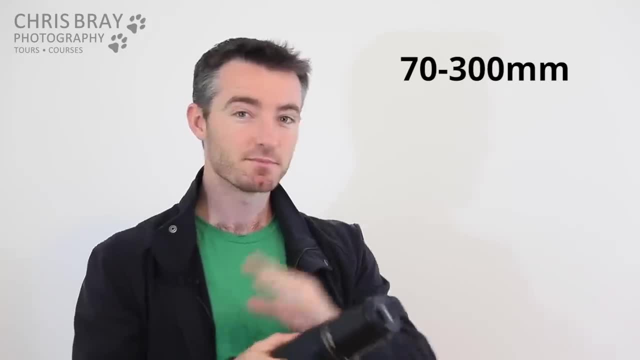 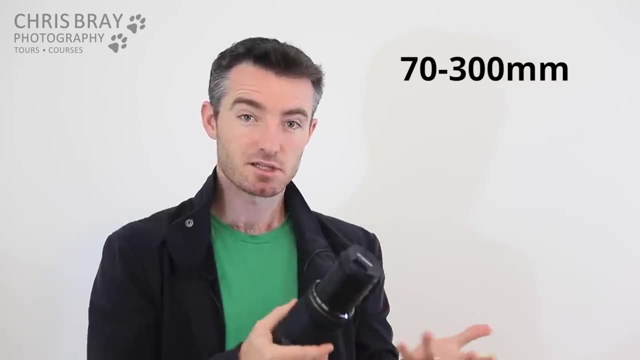 different lenses, really they should be. each bit of glass in there should be shaped completely differently to do those two jobs and also see how it's got to slide in and out. that means there's got to be slop in the system. you can see it wobbles. that's why it's got to slide in and out. 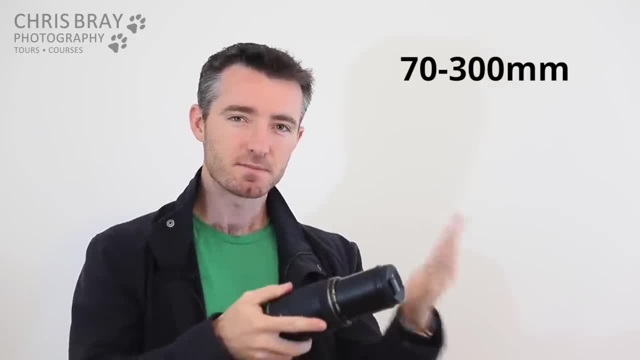 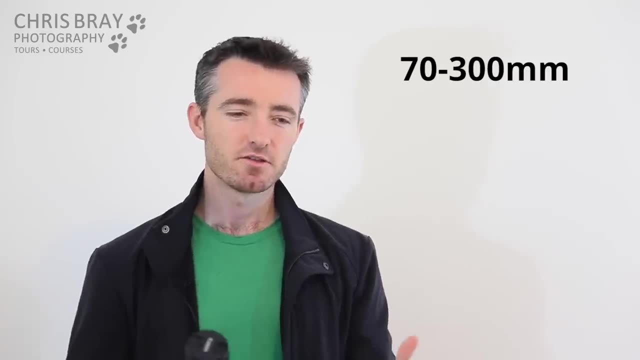 it's no good. so you zoom out and sags down a little bit so all the optics aren't perfectly aligned. so you get little chromatic aberrations and rainbows and just not very sharp photo. so in many ways, the more a lens tries to do, the less good it is at any particular point along the way. 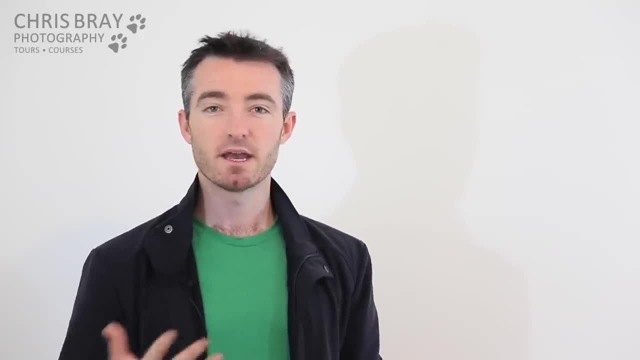 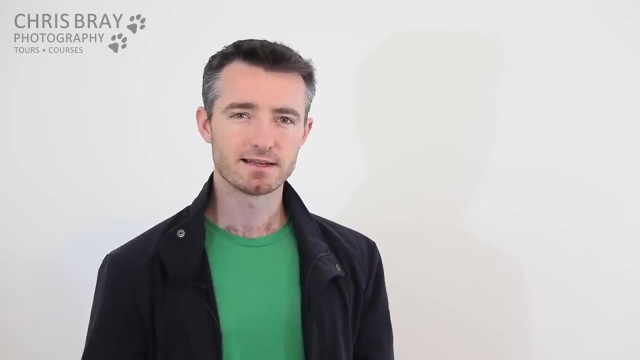 becomes a bit of a jack of all trades. now, that's not always true. you can pay a fortune and have lenses that actually do a really good job, even though they're quite versatile. but it's just a general rule of thumb. you know, you find lenses that do all the way from, you know, 18 millimeters. 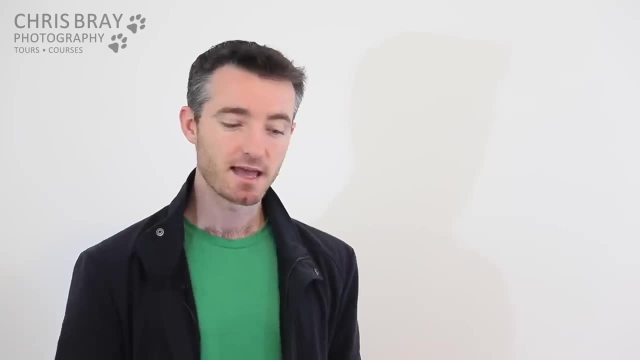 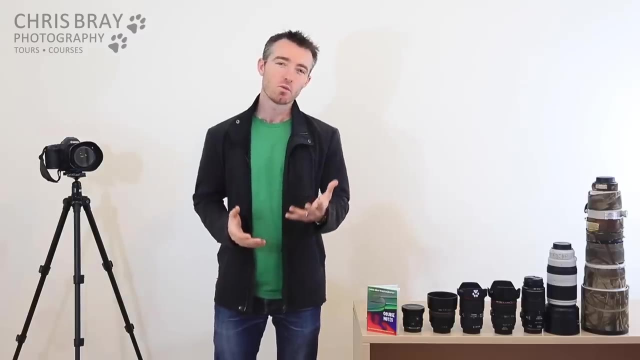 incredibly like versatile. you never have to change lenses and it's lightweight for traveling. so they've got their pluses as well, but it's also not going to be the highest quality lens. okay, the last bit of jargon. what is the speed of a lens people talk about? oh, it's a fast lens. what does? 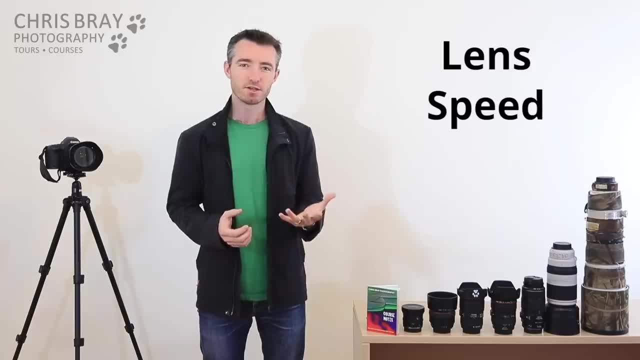 that mean the speed of the lens is just the smallest f number you can get to remember back in the aperture lecture it was all about scrolling down to really small f numbers which gave you beautiful blurry backgrounds and nice fast photos. well, that's, a small f number, is a fast lens, it's. 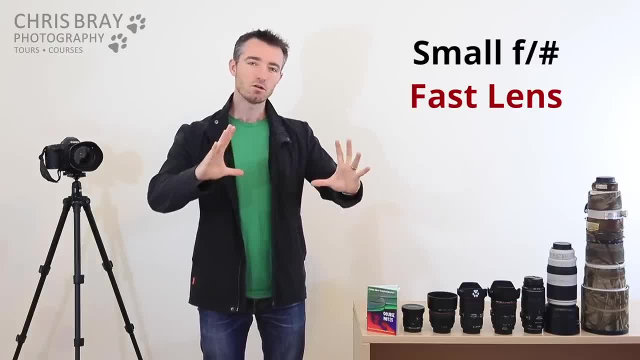 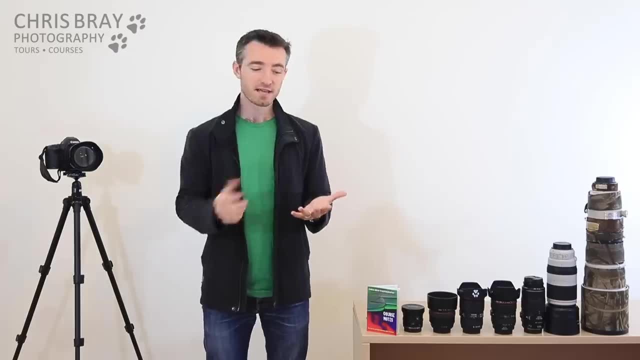 called speed just because you imagine a small f number being a big hole can let lots of light in quickly and you can take quite fast photos even in low light. so that's it. we can now understand the naming convention that they write around the end of lenses, either around the edge or inside the 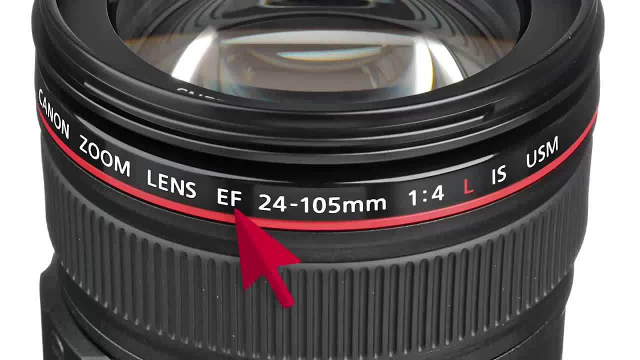 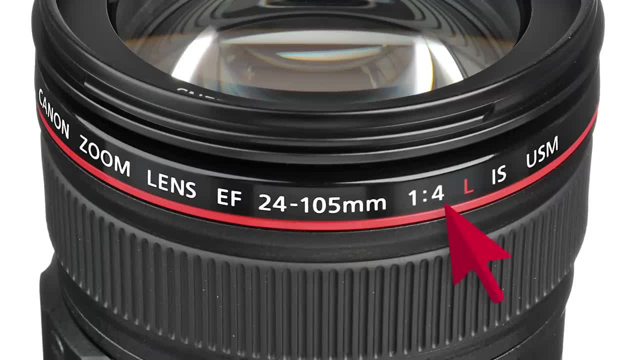 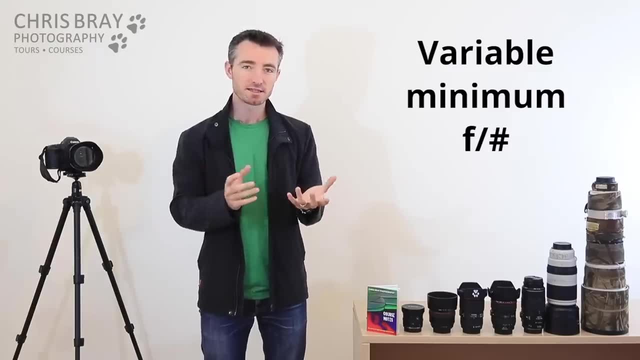 bit. telephoto great f4. that's the speed of the lens. that's the smallest f number you'll be able to scroll down to. some lenses have different minimums depending on how much you've zoomed in. so you might see a lens that says, you know, f 3.5 to 5.6 and if you zoomed all the way in the 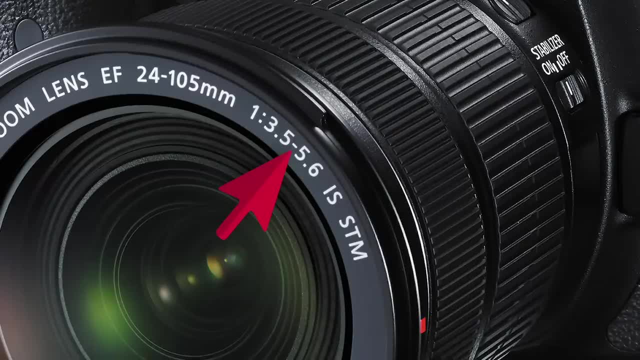 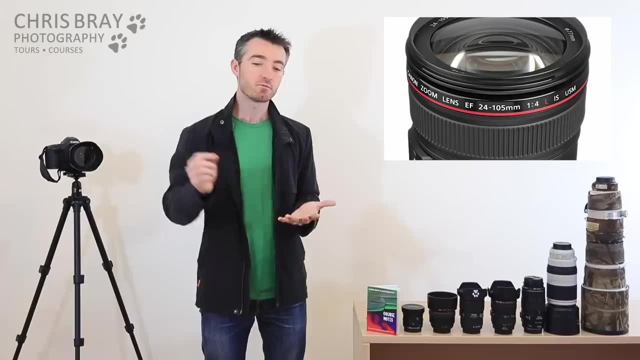 smallest you could get is 5.6, but if you're out nice and wide maybe you can scroll all the way down to 3.5. l in canon lingo just means luxury. they could equally replace that with a dollar sign and that would mean exactly the same thing. 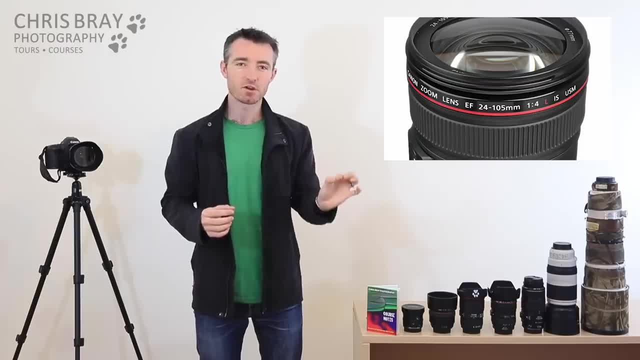 uh, they also mark these ones with a red stripe around the end, just so you know not to drop these lenses. but they're just basically higher quality, more professional. they cost a lot more but they've got better glass in them so you get sharper results. they've often got better anti-reflective. 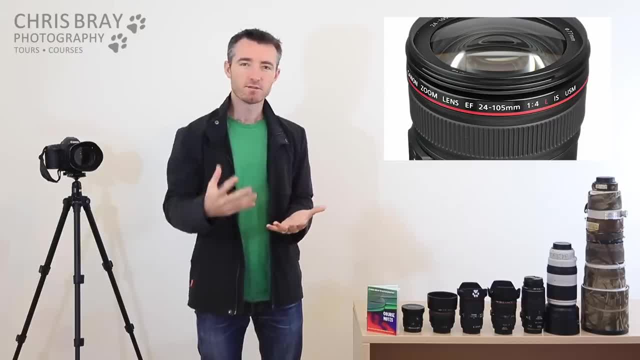 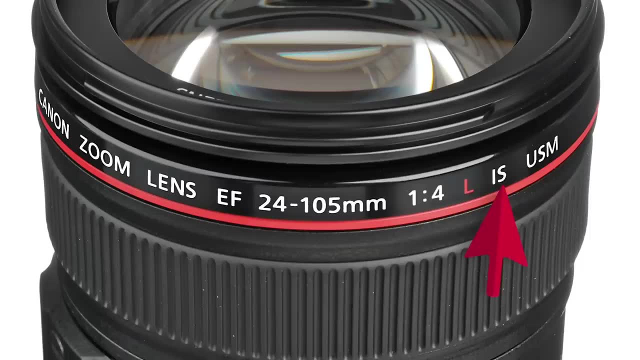 coatings on the front so you catch the colors better. they've got better environmental seals so if it rains you might be able to still use. it is that's just canon's wording for image stabilization. so in lens stabilizing- and it's incredible, different brands call it different. 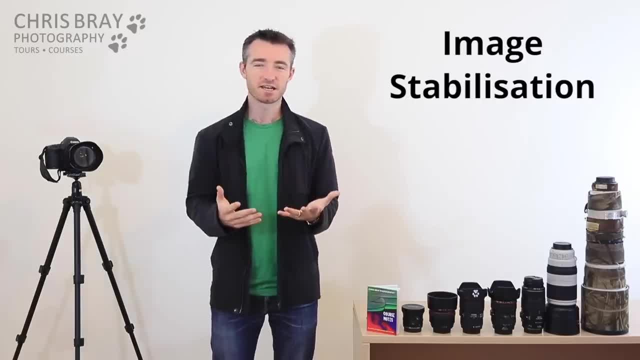 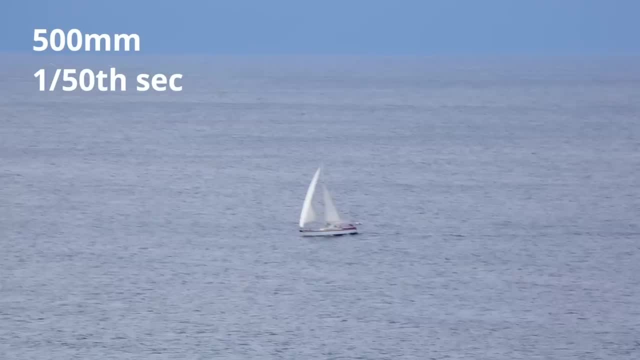 things. you know- vr os, but it's the same thing with the camera shake. you can kind of see it in the lens stabilizer. it's a little bit different than the camera shake, but this technology is getting amazing. now you can hand hold photos where there's just no way you should have been able to do it without a tripod. take a look at this. 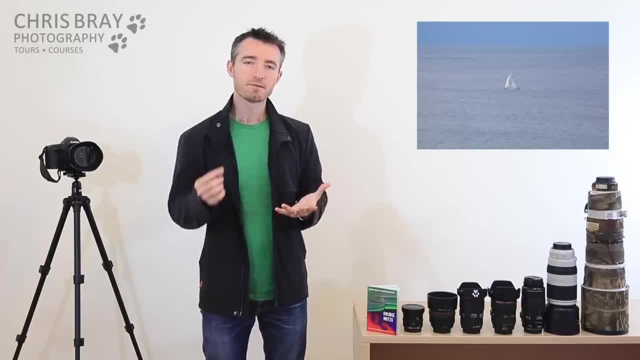 kind of example. this is hand holding a 500 mil lens, so a super telephoto lens, without any kind of rest or anything, trying to take a photo of this little sailboat going past at 50th of a second. now, thinking back to that rule of thumb just before, if we're using a 500 mil lens, we should be using about 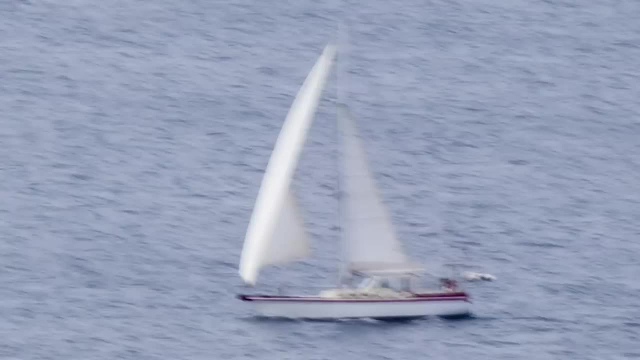 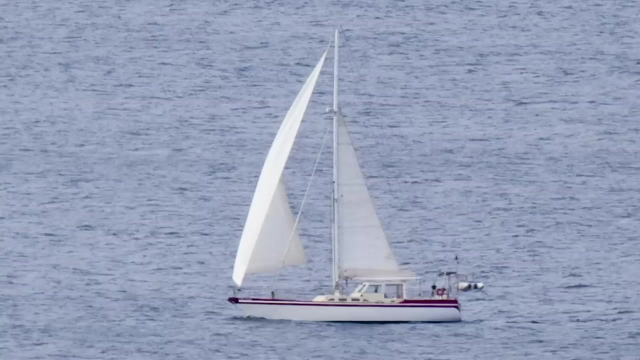 With stabilizing turned off, zoomed all the way in. that's about as good as you could hope for, But if you turn the stabilizing on, how much better is that? That's amazing. There's no way I should have been able to take that photo. 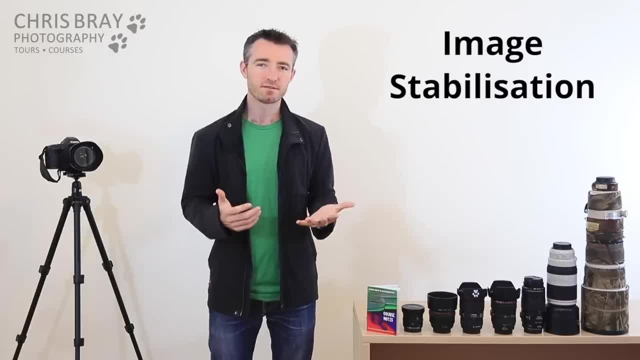 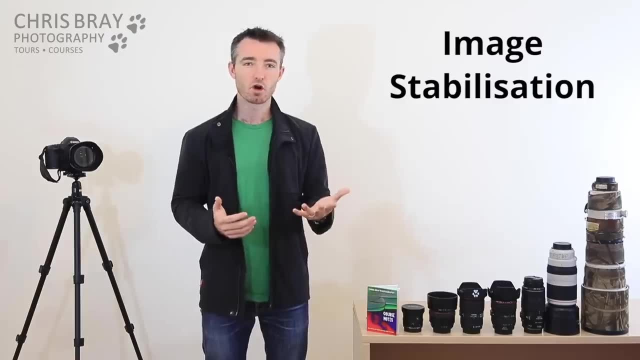 And stabilizing has come a lot better since that. even Sure, it costs a bit of extra money. Normally it's an extra 20 or 30% of the value of the lens to get a stabilized option, But it's becoming more and more commonplace. 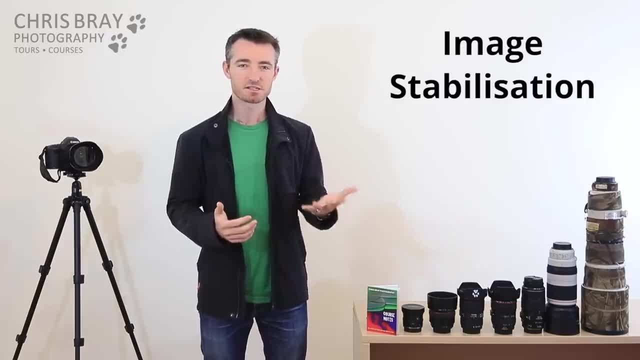 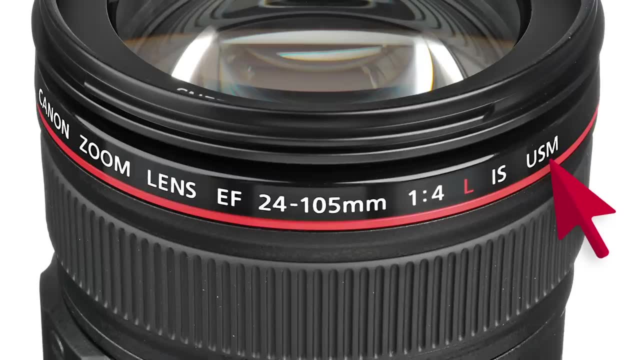 They just don't have the unstabilized option these days for a lot of them, because it's just so invaluable. The last bit, USM. that's just a measure of the speed of the autofocus motor, Which sounds a bit obscure, but it is kind of important. 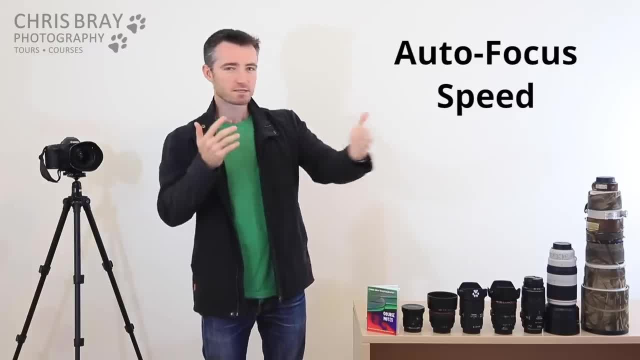 It tells you how quickly it can focus. You know some old lenses just kind of hunt forever, and if the animal's moving quickly it kind of almost never finds it. You'd have to search your own, whatever lens you're looking at. 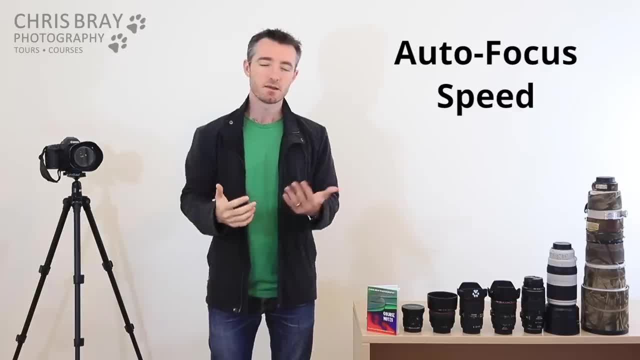 You'd have to look up whatever those letters mean for yours because there's so many different types. But USM ultrasonic motor, it's pretty quick, That's good. What about manual focus? When would you ever use manual focus? 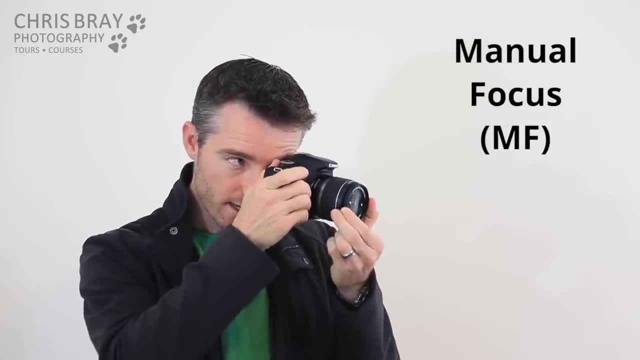 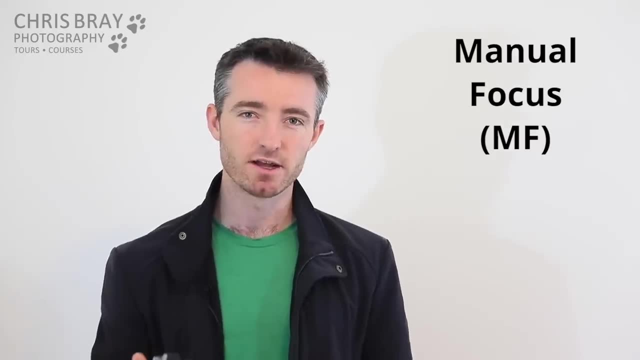 Because then you've actually got to peer through the video And twist the focus ring back and forwards and try and decide when you think it's sharper. You know autofocus is way more accurate than manual focus could ever be. It's just, unfortunately, there are times when autofocus will fail you. 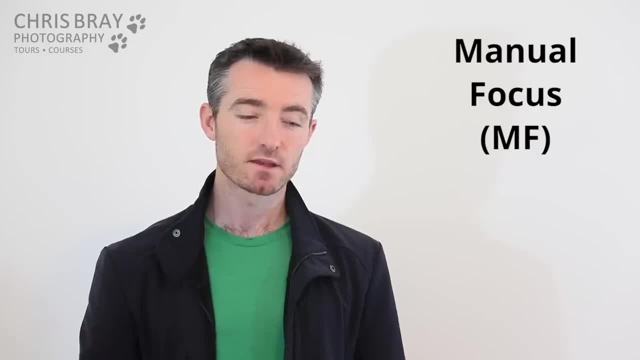 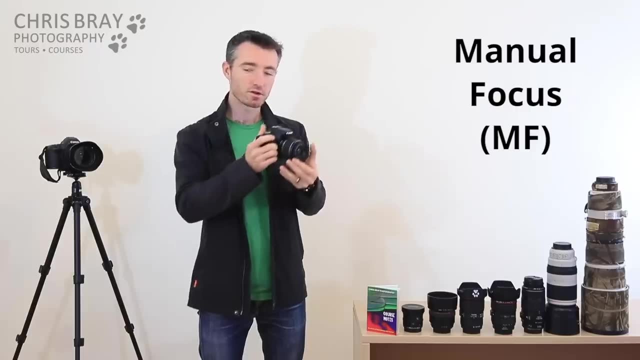 And then you've got to resort to manual Times like low light. I'm sure you've all done that. You try and take a photo in the dark and the camera just goes and can't see anything. So you could switch it over to manual focus and try and guess it about right yourself. 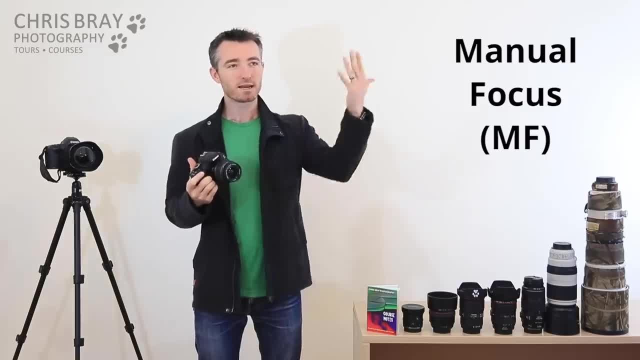 Another situation where autofocus will normally fail is on a very plain, uniform surface, or like the clear blue sky, with no clouds or anything. The lens can't really see anything to lock onto. It's looking for contrast, really an edge, so it just sees straight through it. 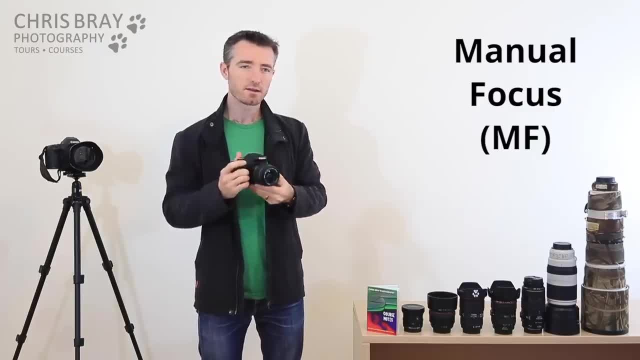 So you could switch over to manual focus and try and get it about right, But instead I'd actually stay on autofocus but just point the camera briefly at something that's a similar distance away, like a tree on the horizon or something, and go beep and then bring it back and take the photo. 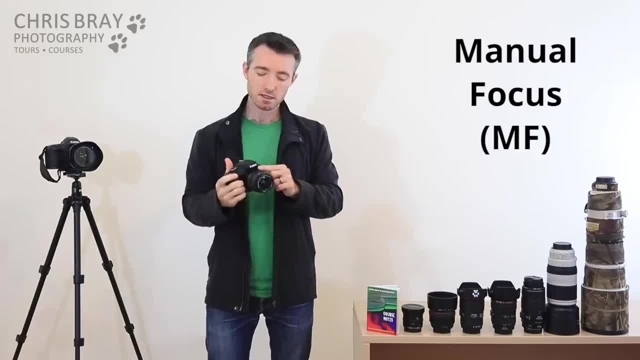 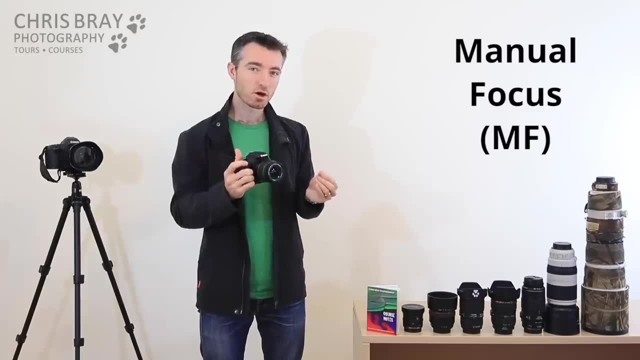 The time I'll actually use manual focus. quite a lot is to lock in the focus. Maybe it took me quite a long time to get perfect autofocus because it was low light or something, But after it's finally got it like maybe on the tenth time. 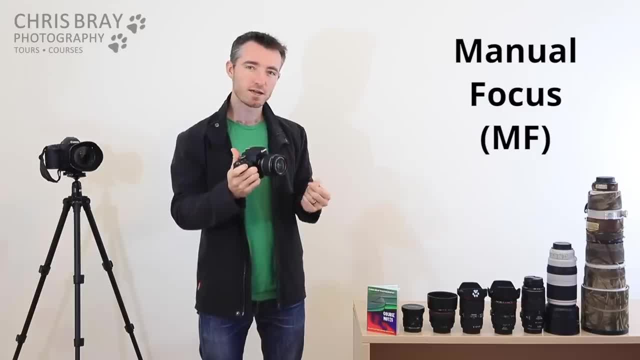 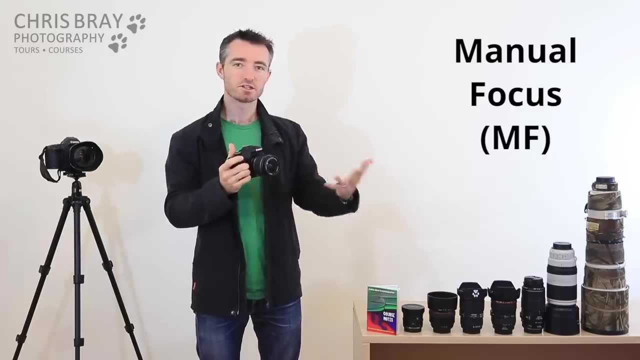 hmm, hmm, hmm, beep. great, then, if you switch your lens back to manual focus, as long as you don't bump that focus ring, from now on you can go and take as many photos as you want and it doesn't start hunting for it each time. 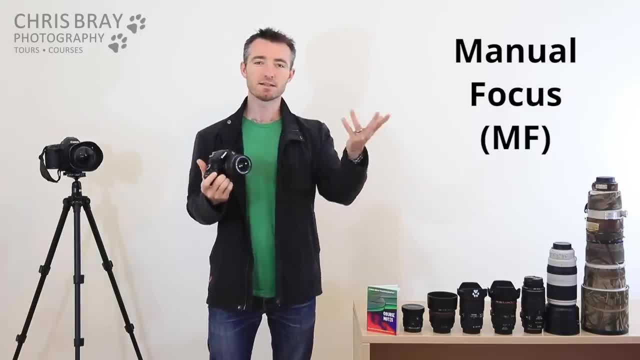 So that's a good little tip, Say, if you're photographing some little animal in a tree or something at night time, so it's pitch black. you can't autofocus, you can't manually focus either, because you can't see what you're doing either. 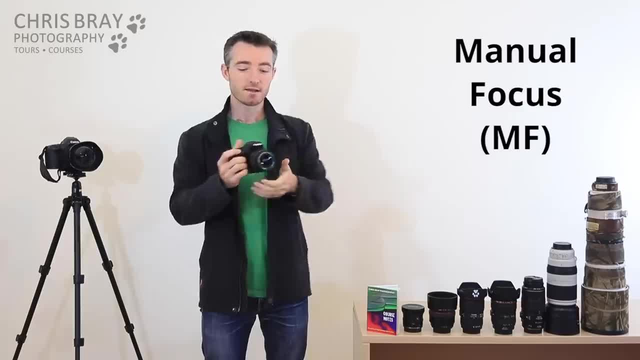 a good tip is to shine a light on it. light it up, then you'll be able to autofocus on it, no problem, way better than you could have with manual. So beep, and then with your camera on a tripod, you can then go and turn your autofocus over to manual focus. 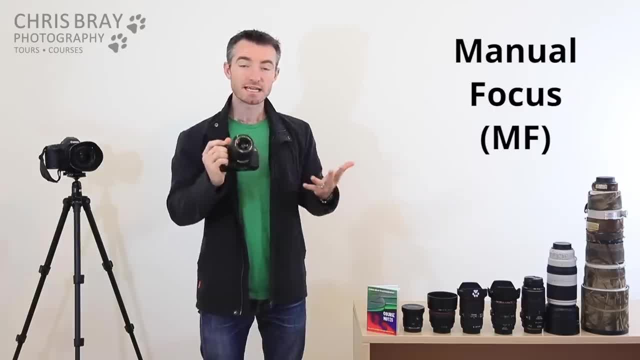 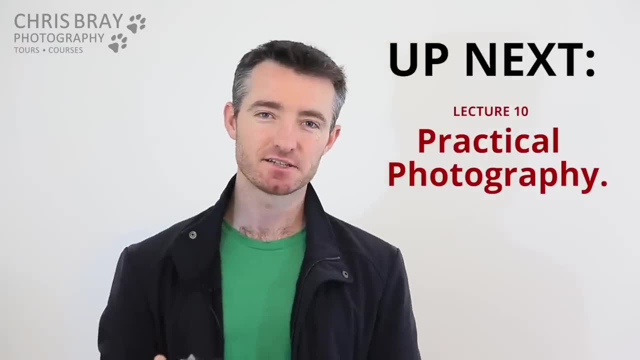 turn your torch off and then you can go ahead and take a full, you know ten second night time photo, knowing that the focus has already been locked on at that perfect distance. So next up we have one last lecture on practical photography. 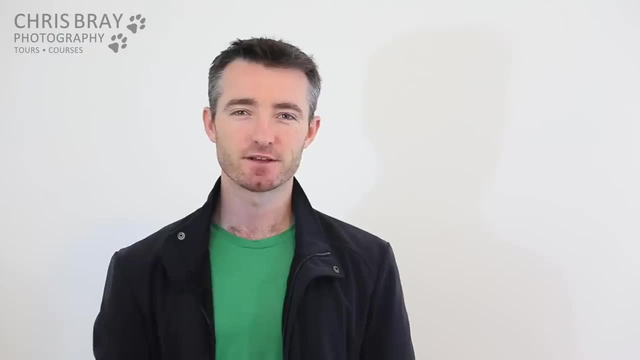 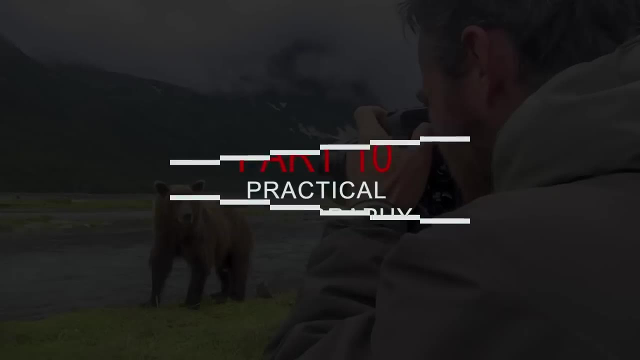 Just bits of advice, really- that I'd hate for someone to be able to do a photography course and not be told, So don't miss out on that one. For this final lecture in the online photography course, we're going to have a look at practical photography. 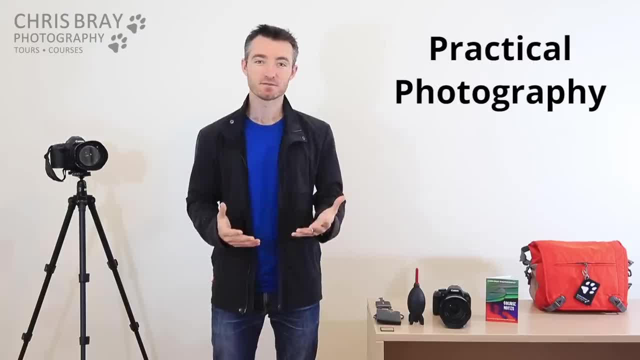 So it's just an eclectic bunch of things. I'd hate for someone to be able to finish a photography course and not be told Things like keeping your camera clean, trying to break into the industry, a little bit of post-production and so on. 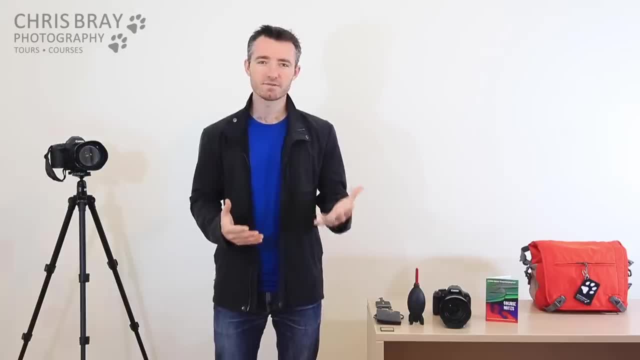 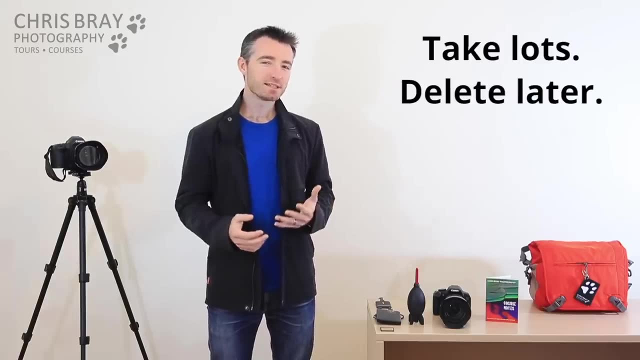 But, to start with, you've probably all got to agree with me that one of the big advantages of digital photography is that you can just take so many photos and delete all the bad ones later on, right? Well, deleting them later on is something I'd encourage, rather than at the time. 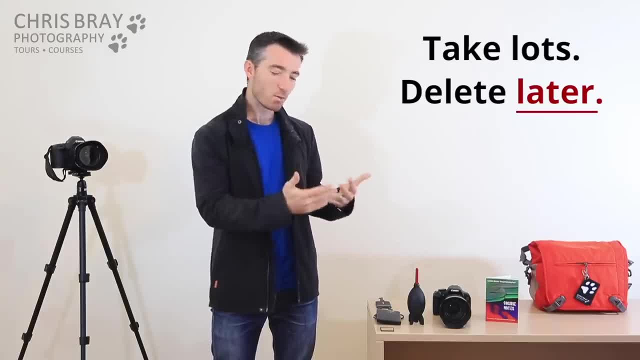 Some people have this urge to sit there going through the photos then and there, while they're taking them and working out which ones to delete, and so on. I think that's a bad idea for several reasons. First of all, you're going to run out of batteries before you know it. 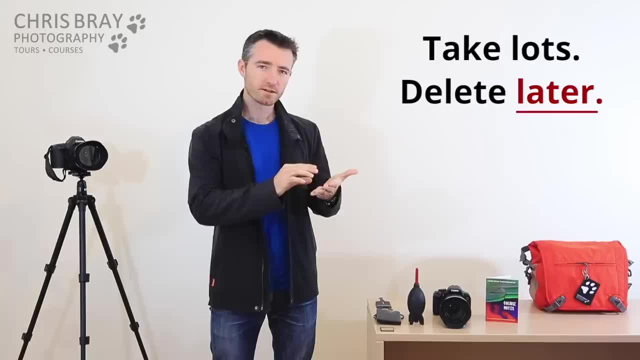 Next, it's just too hard to work out if a photo is perfect or not, looking at that tiny little screen on the back of the camera. Two photos that look identical. they never are. One of them's better, one of them will be sharper. 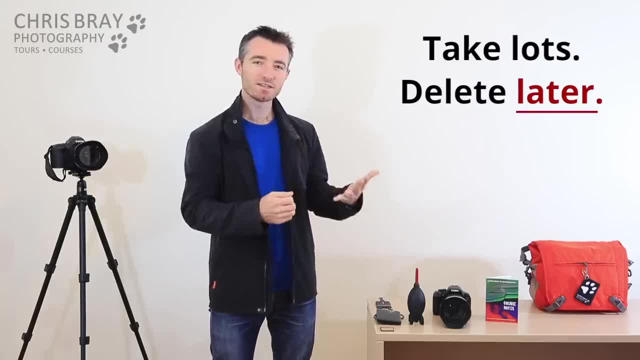 or maybe there's a little bug flying past in one of them or something. Wait till you can get home and put it on a big screen. make a proper, informed decision. It's also just too easy to accidentally delete the wrong photo. I've seen it too many times on our photo tours. 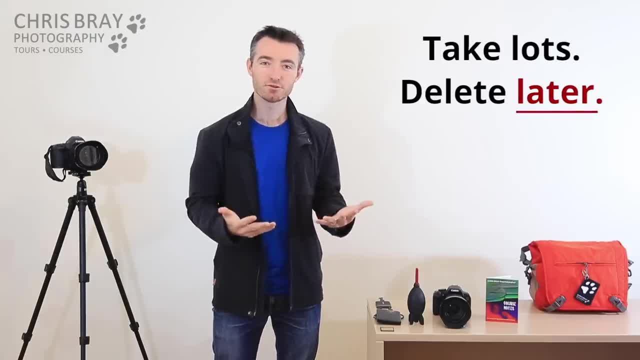 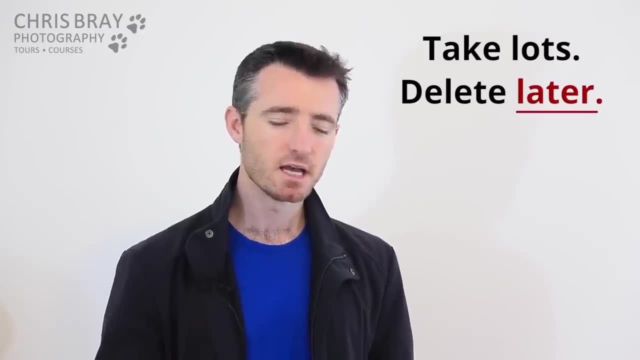 People would just be deleting. oh, that was the wrong one And there's no undo on the back of your camera. The only time you ever really need to start deleting photos out in the field is when you accidentally fill up your memory card and you forgot to bring a spare with you. 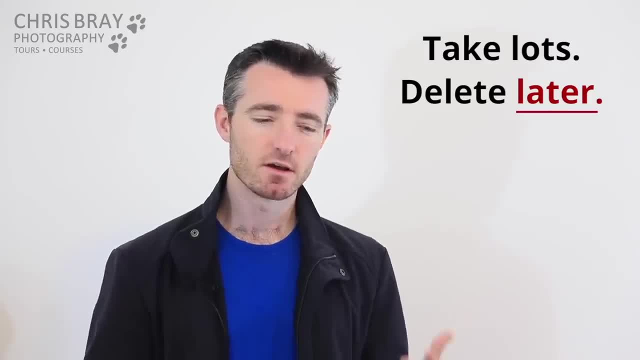 And this normally only ever happens if you just don't get into the habit of clearing your memory card after each holiday. You know, of course, if you never empty your card it's going to fill up, But you should just get in a good habit of every time you come back from a photo session. 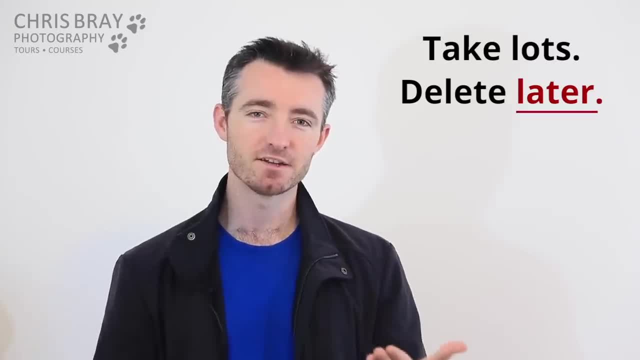 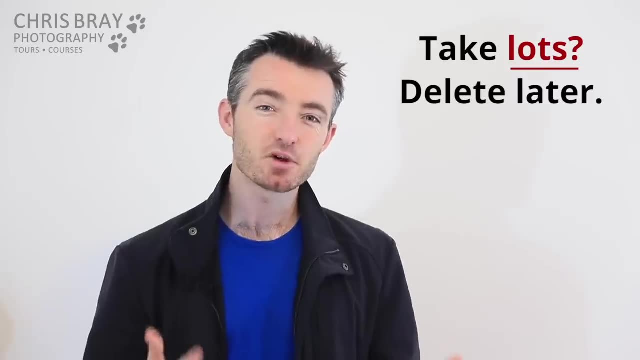 just download all your photos, back them up and then format your memory card in your camera and start fresh. Then hopefully, you'll never run out of space in the field and you won't have to start frantically deleting photos. Being able to take so many photos is mostly a good thing. 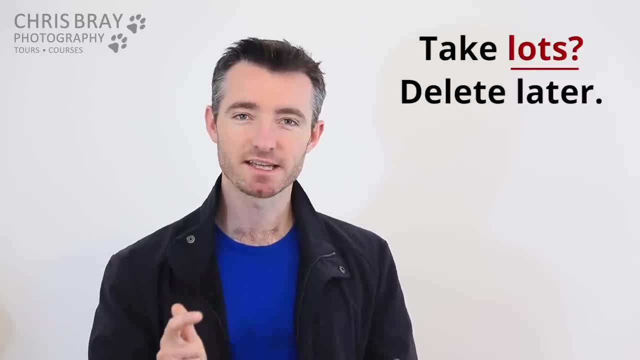 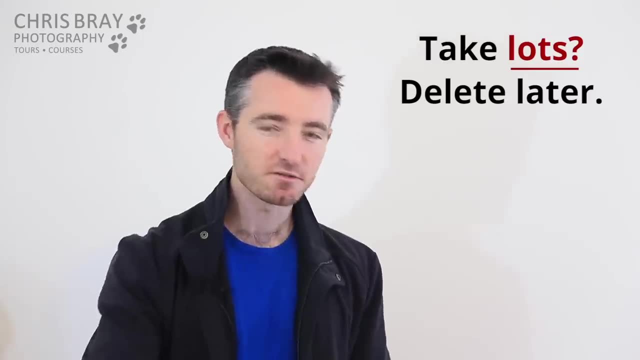 It means you can hold your finger down and rattle off 70 photos and get that perfect moment that you would have almost never been out of time with film. And because each photo is free, it doesn't really matter. You can try different angles and weird settings. 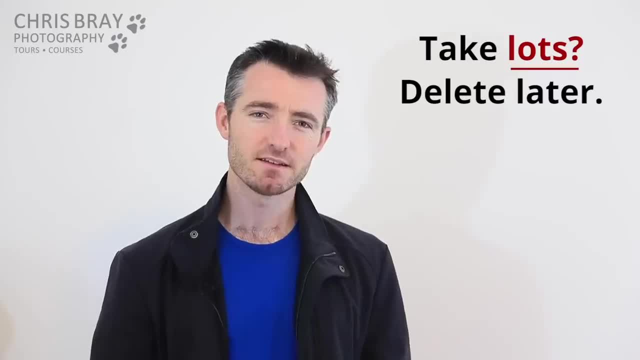 and you know, fluke some really great shots. But the fact that you can take so many photos now is not always a good thing, because it kind of means that people put less effort in. You know, if you went away with a roll of 36 exposures on a bit of film. 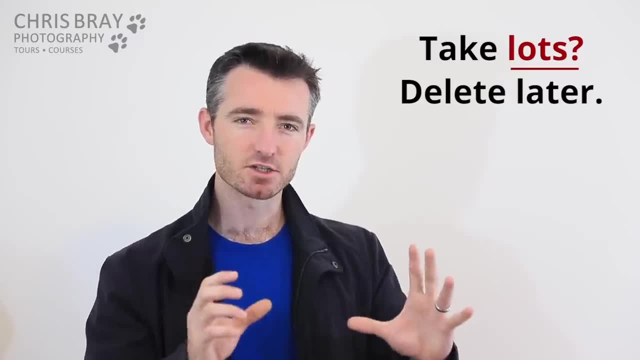 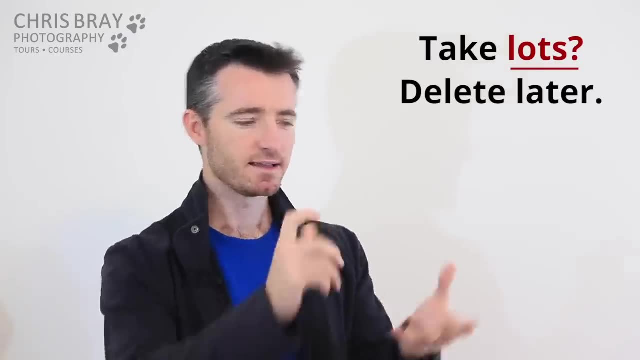 you used to put the time in and think long and hard about how you'd frame up the shot, and even if you didn't know anything about theory, you'd still make sure people were smiling properly, and so on. But now it's a bit like: ah, yeah, whatever. 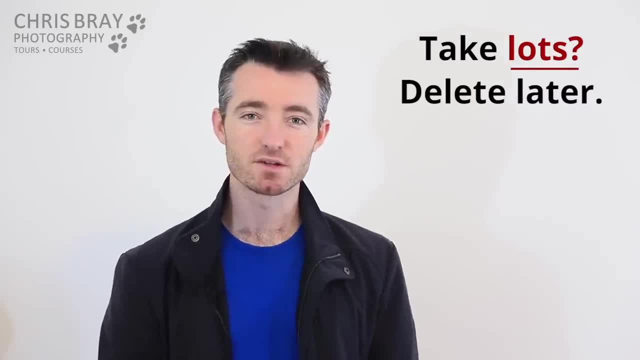 And you probably spend the same amount of time. you know a minute to take a photo or something, but you take 60 photos in that and actually none of them are any good, because you didn't put any thought into it, because it didn't feel special. 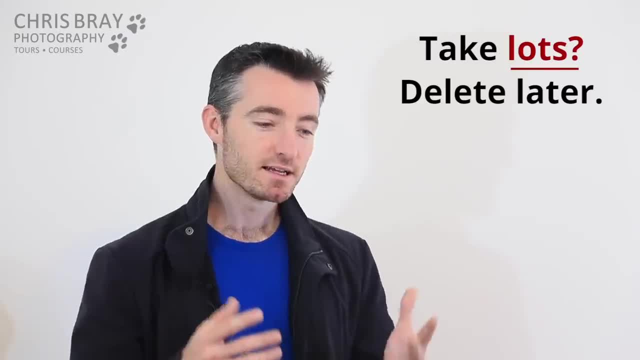 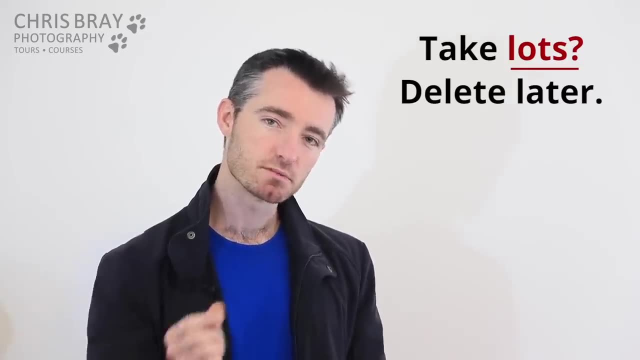 So that's often the mark of a good photographer- is someone who actually takes a bit of time initially to think about lighting. you know the direction of the lighting, the background, what kind of settings do you want? small F numbers for blurry backgrounds. 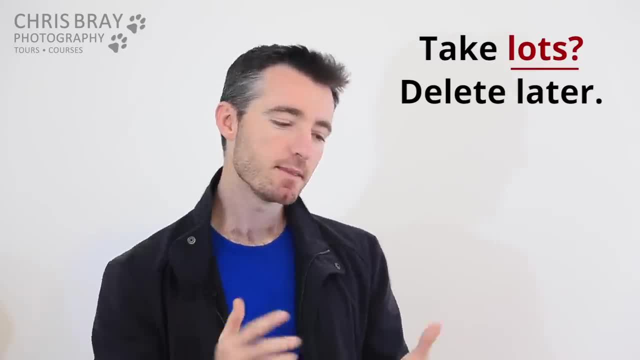 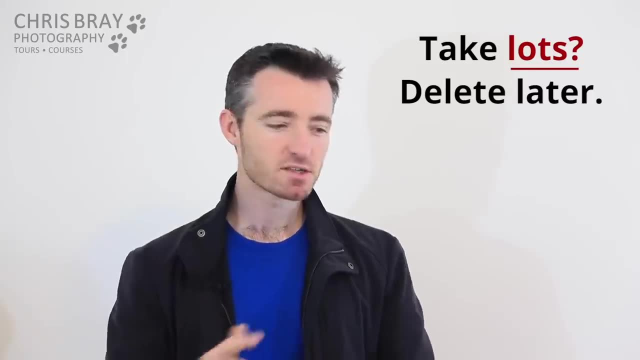 all these kind of things, and then you just take a couple of photos, and then maybe a couple from a different position as well. Don't just take one, Because chances are there'll be something wrong with it. Take a couple, But don't just go nuts and take lots. 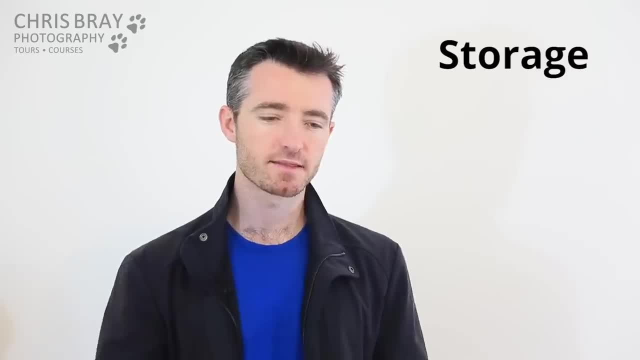 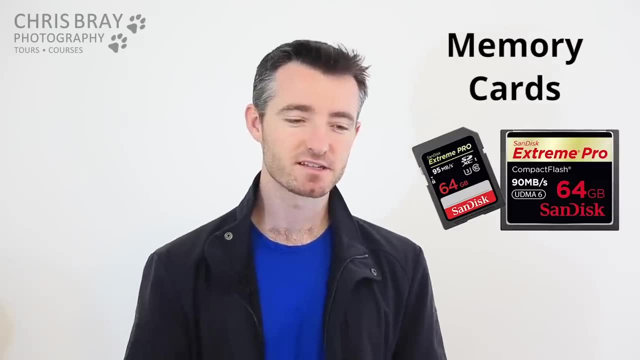 I just want to touch on storage of your photos on memory cards and things like that. I don't think it's a great idea to buy the largest memory card that exists, you know, 100 and something, gigabytes, whatever's up to you these days. 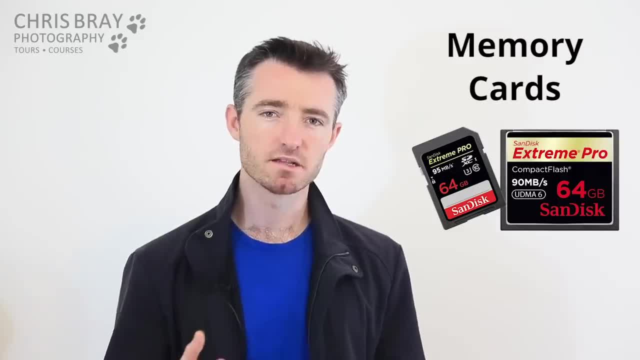 because it just means you're putting all your eggs in one basket. risk-wise, You're better off splitting it between a couple of cards because they can fail. Obviously, you get what you pay for and good brands like SanDisk and things seem to fail less than the really cheap alternatives. 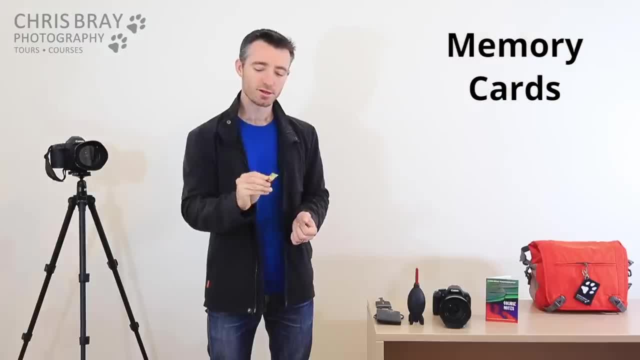 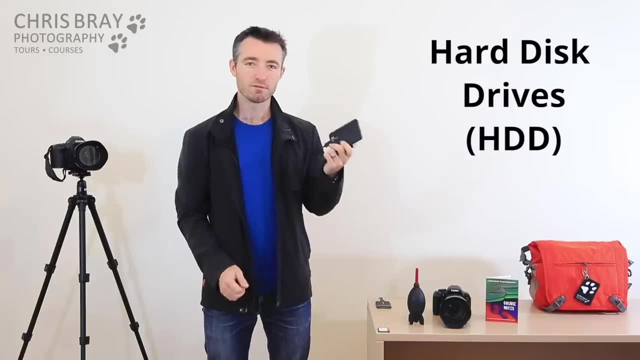 But even SanDisk cards can fail, But they are pretty durable. You know, you can normally put these things through the wash and they're still okay. As opposed to these things, the USB-powered- you know, portable-powered hard drives, they're pretty easy to break. 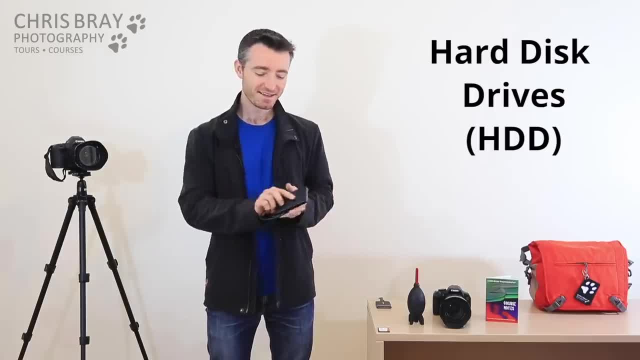 And if you haven't broken one yet, just count yourself really lucky. You should always have two copies of anything on a hard drive like this, because it doesn't take much of a bang for them to stop working And because they're so huge, you know two terabytes or something. 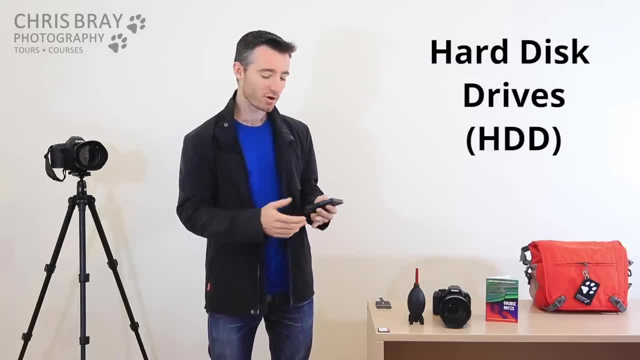 it can be catastrophic: the number of photos you could lose, The number of photos you could lose in one go. So if you're using these sort of things- and we all do- just make sure you have two of them And you always have the same data on both of them. 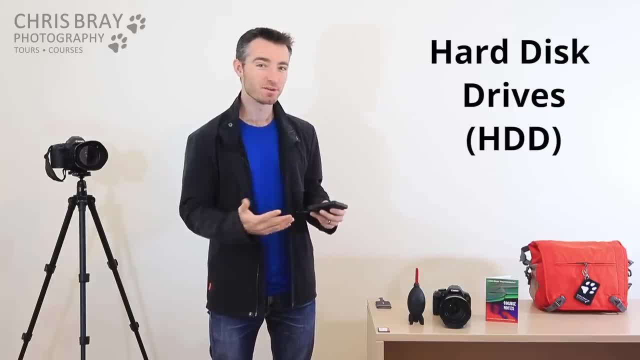 so that when one fails, treat it like it's going to fail at any moment, because it probably will. You've then got time to go and get another hard drive and then copy it across. These days it's starting to get more and more affordable. 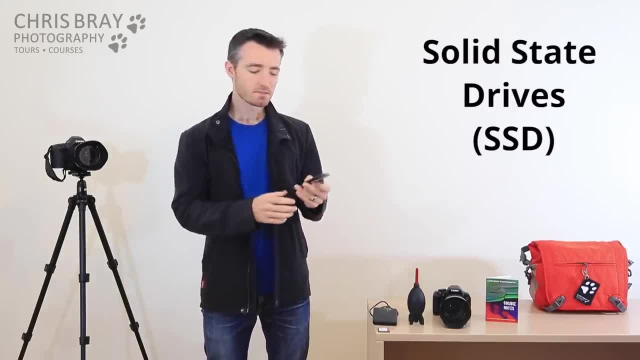 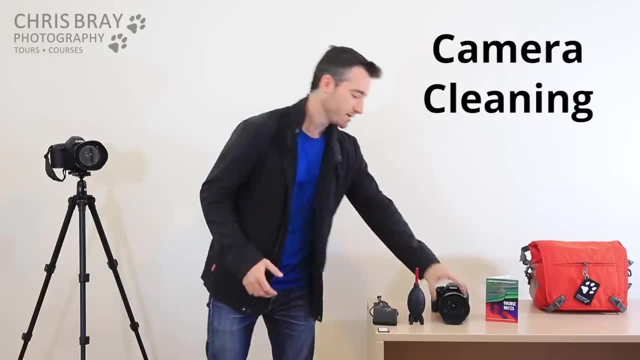 to be able to use these solid-state hard drives, And that's great for when you're traveling, because they're small, they're durable and they don't use too much power. What about keeping your camera clean? Now? the outside doesn't matter so much. 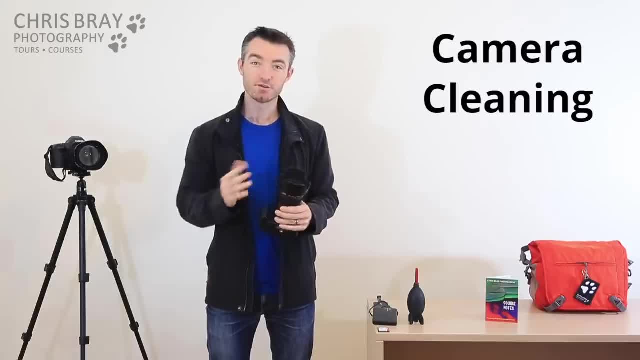 The front of the lens. yeah, use a lens cloth or a tissue if you can, But if you have to, you can still use your shirt, Particularly if you've got a UV filter over the front. it's pretty easy to clean. 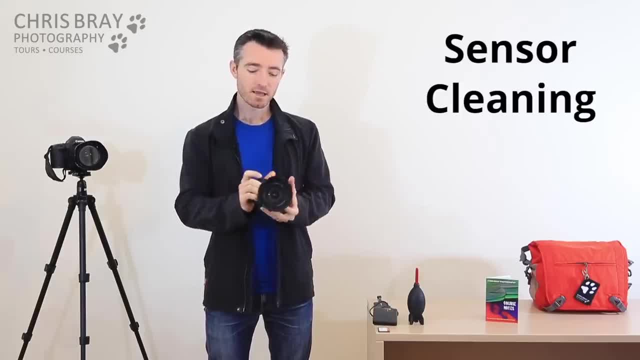 But the important part is obviously inside the camera sensor And if you get dust in there it'll just find its way down and sit on the sensor and it just blocks light from getting to that part of your photo And you'll just have a little black dot on your image from that photo onwards. 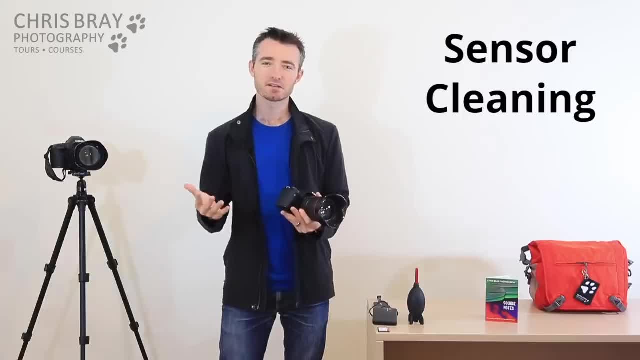 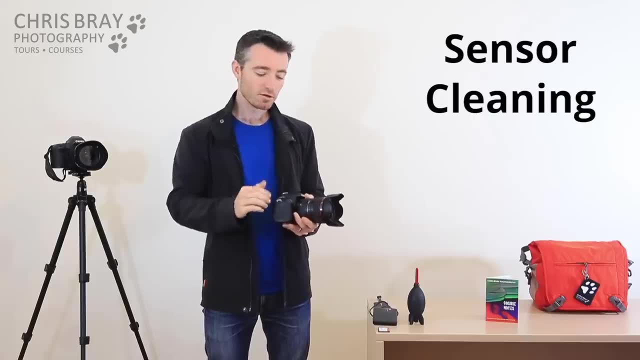 every single photo from then on. You know, back in the days of film it didn't matter so much if you got a bit of dust in there, because each new photo was a clean piece of film pulled out of the roll. But with a digital camera, 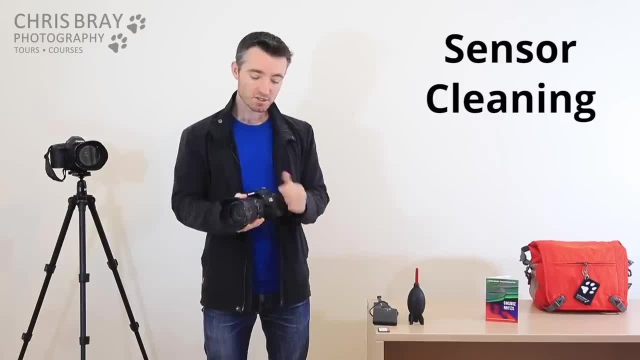 it's the one sensor back there for the entire life of the camera And eventually you will get dust in there and you'll start to get little spots and you've got to work out how to clean it. I actually take a test photo every couple of days or weeks. 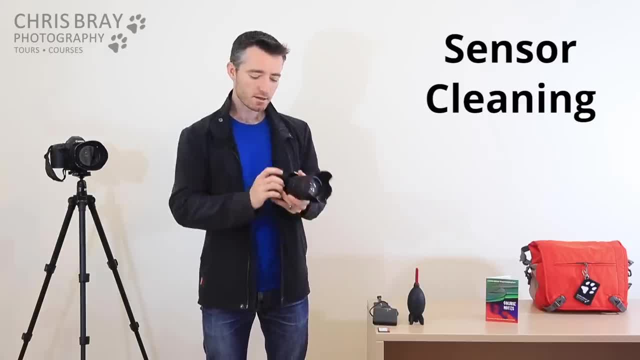 depending on how dusty the environment is, that I'm in just to check. So I go on to aperture mode and use a really large f-number. Think of it as a big f-number for a big depth of field. It'll show up all the dust. 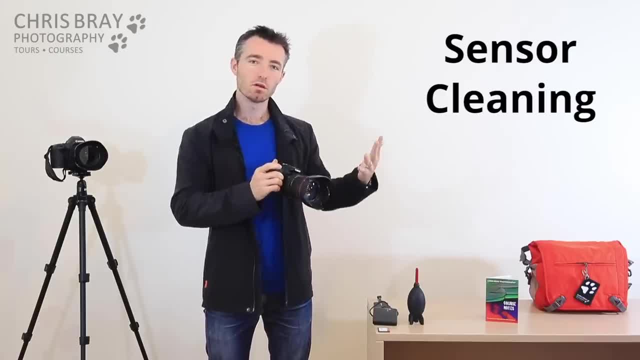 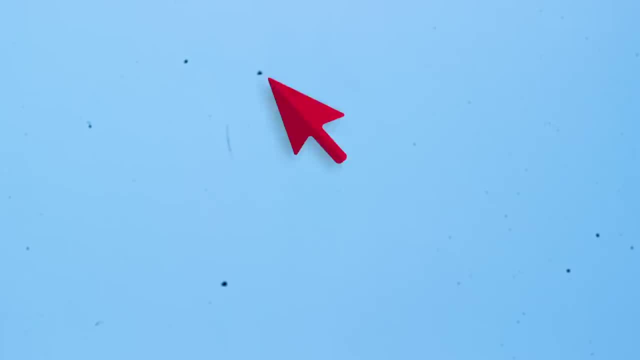 And then you take a test photo. that should just be empty, like a plain wall or blue sky or something, And then zoom right in on the back of the camera, Move all around, Just check you don't have any of these little black spots. 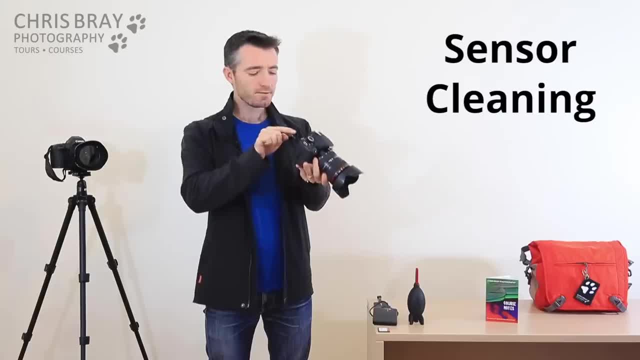 These are all bits of dirt sitting on the sensor. If you can see them looking through your viewfinder, then they're not on the sensor. They'll be on the eyepiece up inside the eyepiece. You can clean that if you want to. 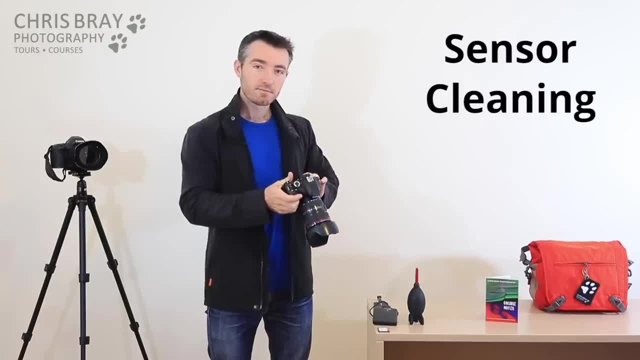 I don't generally bother, Mine's covered in dots, But if it's turning up on the picture then it's on your sensor And you've got to work out some way of cleaning it. Now. most manual cleaning options are pretty scary. 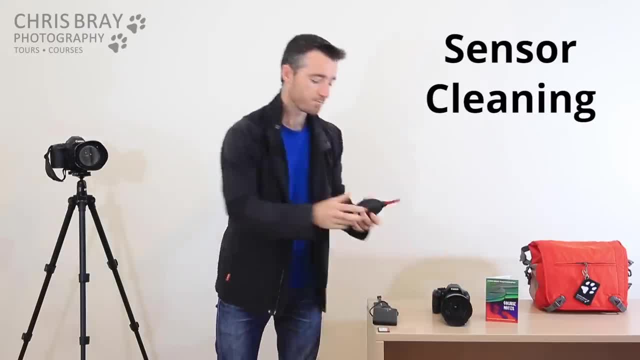 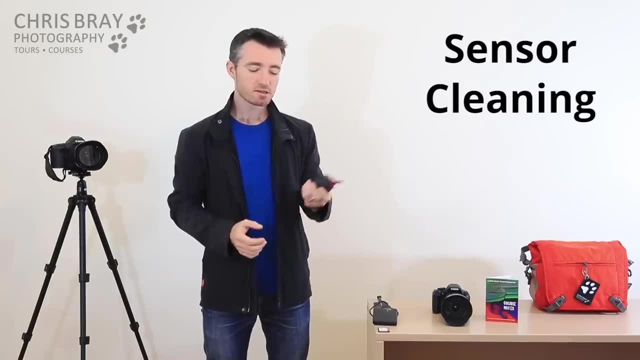 But there is one kind of option that you've got which you can do yourself. That's these little air puffers. You know, normally you just take your camera to your nearest camera shop and get it cleaned, But this will be cheaper than getting it professionally cleaned once. 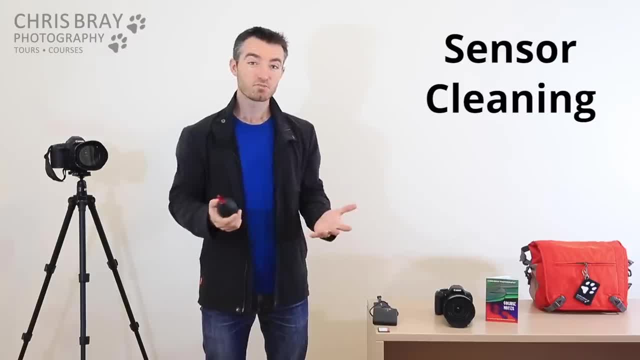 And now you can clean it as many times as you want, wherever you are. It's pretty easy to do: You just go into the camera, go into the menu and go to sensor cleaning And say you want to manually clean your sensor. 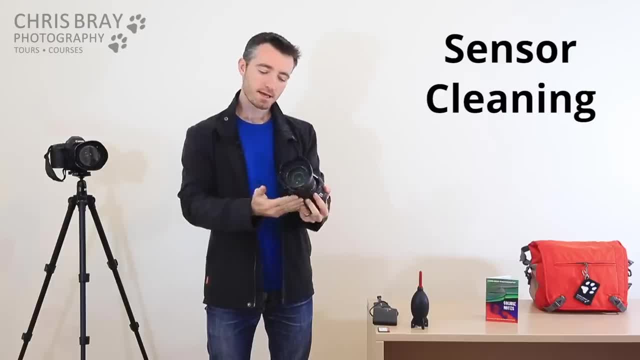 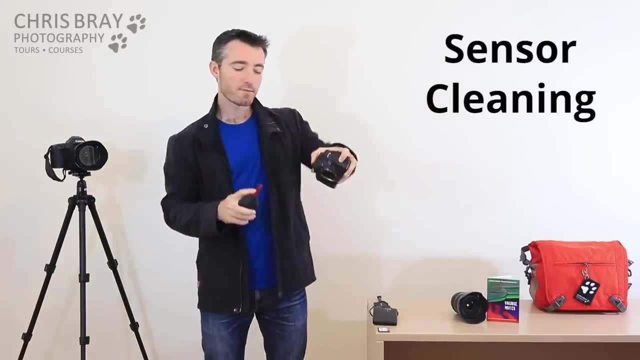 OK, And then it'll lift up the mirror and it'll pull open the shutter and you'll just be able to see the sensor sitting there, And ideally you hold the camera upside down, so any dust you dislodge tends to fall out. 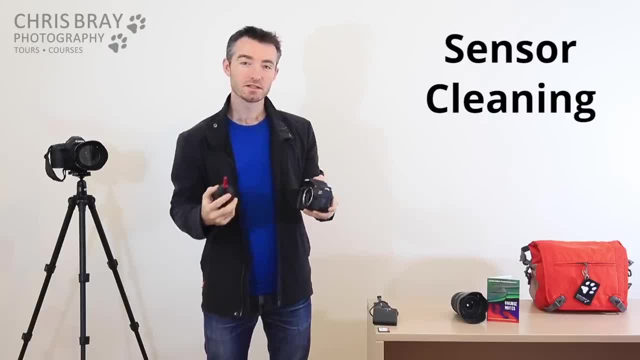 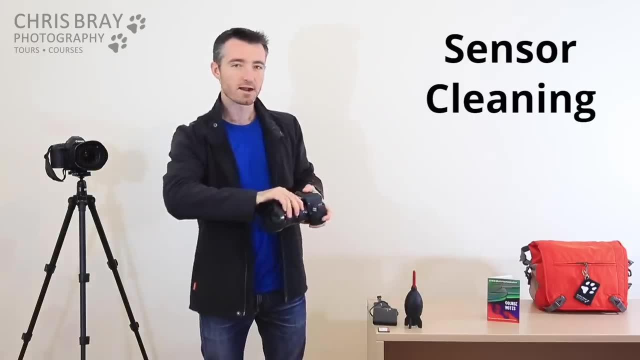 And you stick that in there, give it a good blow and that will clean the sensor Something like 90% of the time. you'll get it spotless with this And you really can't damage the sensor by carefully puffing air at it like that. 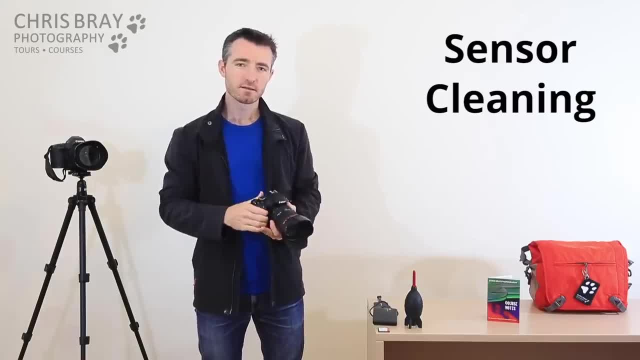 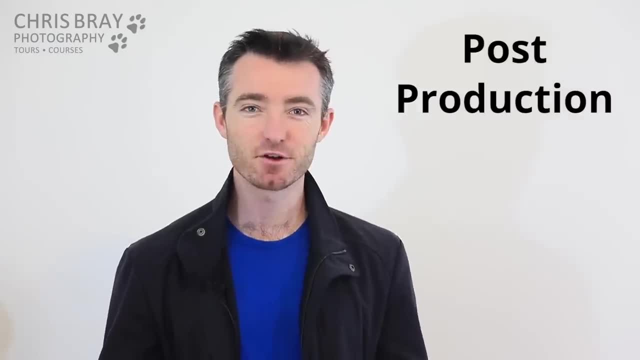 Don't use a spray can of compressed air or anything like that. But it's pretty easy and now you can just do it whenever you want. OK, Let's take a look at post-production. Now I'm not going to try and teach you Photoshop. 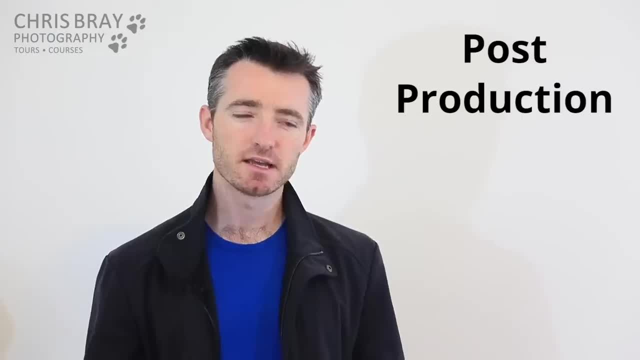 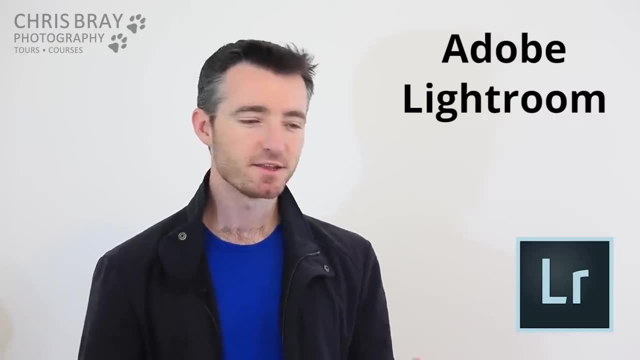 in the next two minutes, but I just wanted to touch on the program that I use and sort of how much I get involved in all that. I recommend a program called Adobe Lightroom. It's pretty much industry standard now. There used to be a bunch of other programs around. 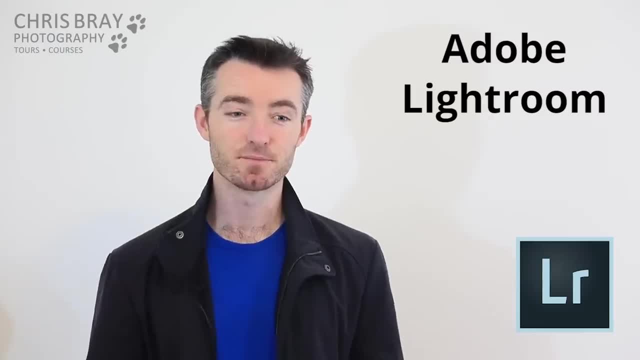 and most of them have fallen by the wayside because Lightroom is just so good. It's about $12 a month and it's just the best money you could spend on your photography each year, for sure. It basically does two separate things. 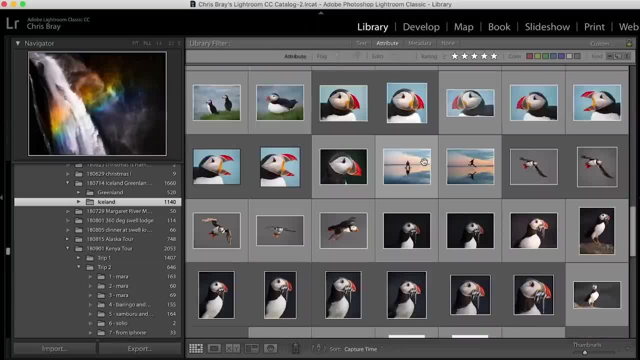 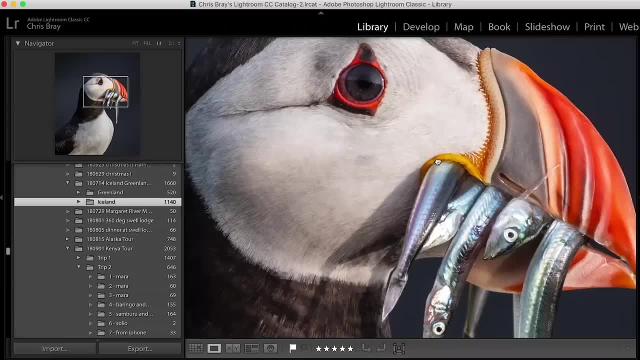 Half of the program is about keeping your photos organized, so it helps you with that logical workflow progression of downloading your photos onto your computer, giving them logical file names, putting them in a logical date folder structure so you can find things, tagging them with keywords and ranking them. 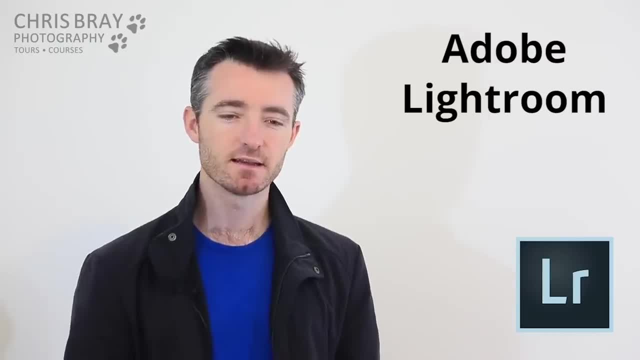 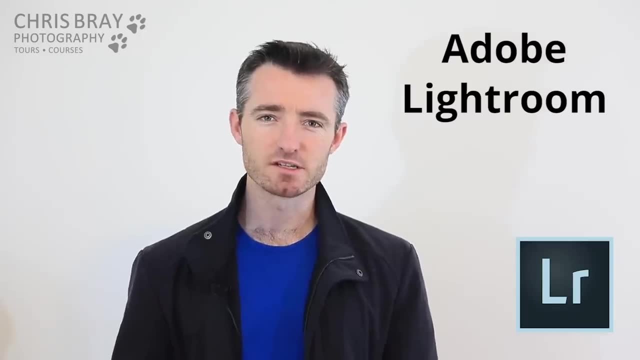 and pulling them into little albums so you can kind of access them all conveniently. But the other half of the program is actually tweaking your photos a little bit, Not to the level of Photoshop, but you don't need to do that most of the time. 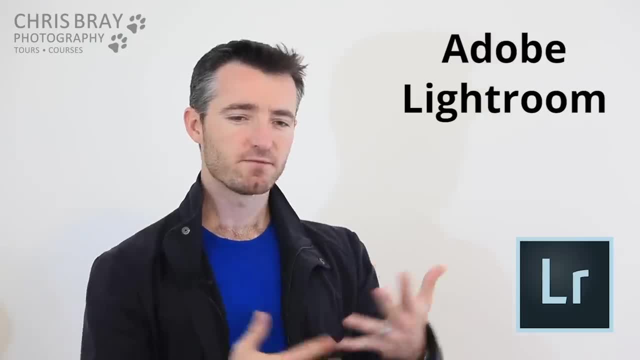 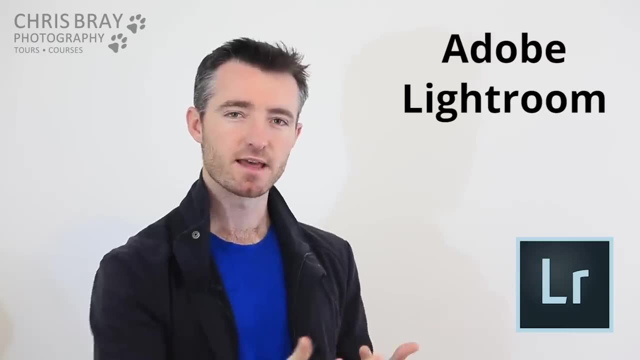 Photoshop is more about opening up these four different images and completely creating something new: stretching the girl's legs and bringing in a different person in the background and getting rid of that and coming up with a new digital image. We don't need to do that most of the time. 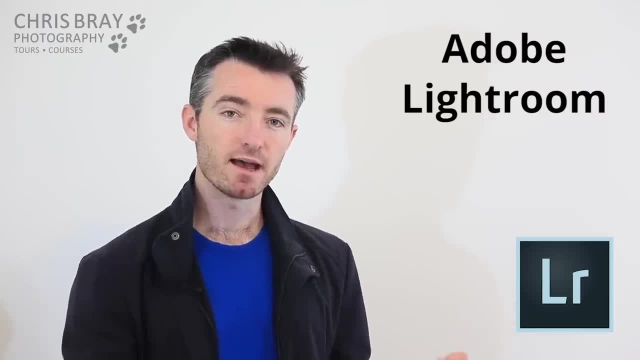 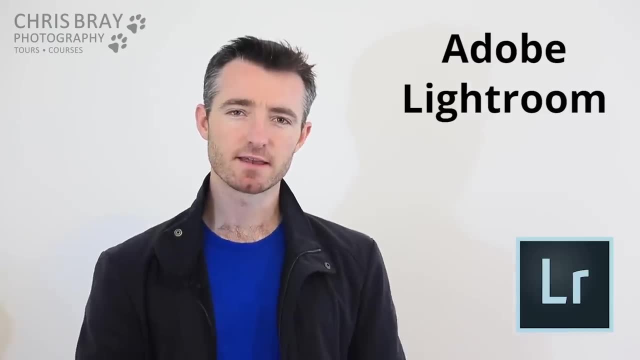 We just want to be able to fix up the problems with the photo you have: make it brighter or lift out the shadows or, if it's wonky, fix it up, square it up a little bit. Simple stuff like that, I mean Lightroom, is quite powerful. 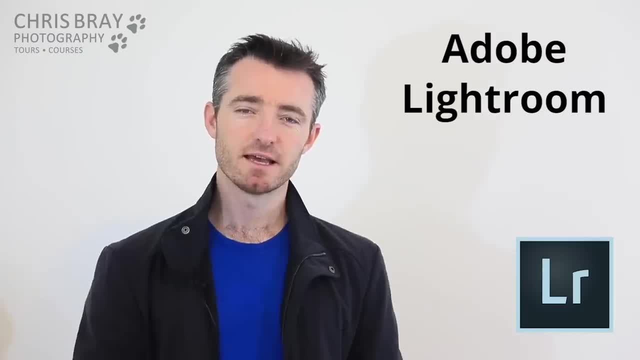 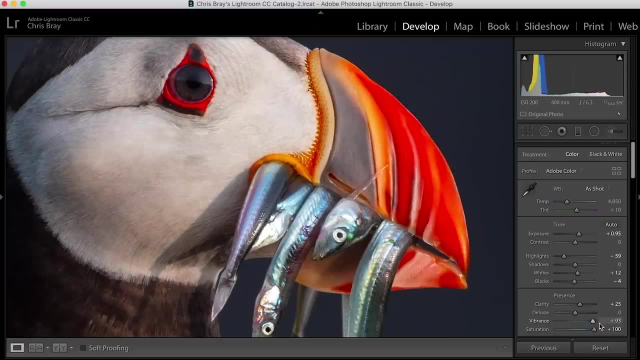 You can do a lot beyond that, but just the simple stuff and it makes it very easy. It's normally as hard as grabbing a slide bar and sliding it left or right and going, wow, that looks amazing, That looks incredible. 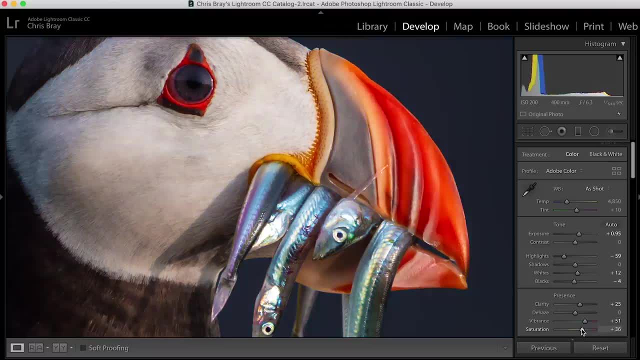 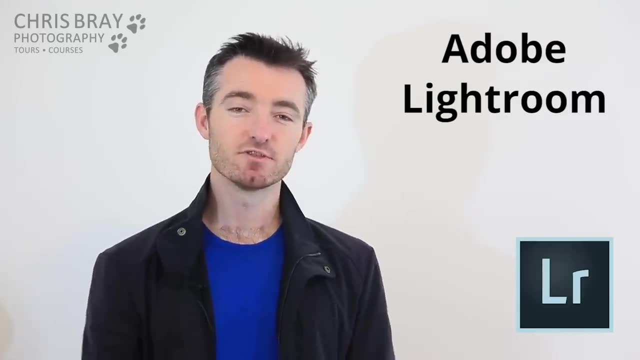 A little bit too unbelievable. maybe I'll pull it back to about here. Great, You can teach yourself Lightroom in a weekend- really. There's so many free videos online about how to use it, but it's just a really good program. 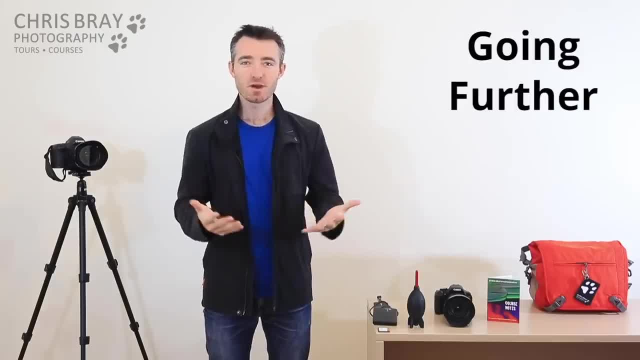 So where to from here? Well, it depends on where you're trying to go, I guess. but if you're trying to get your work published because you're trying to make a career out of photography, well then, even just starting with your local paper. even free of charge if it has to be. I wouldn't do that for long though, because that just devalues your own work. But initially, sure, Inside the front page of every newspaper, you'll find the email address there for the editor. 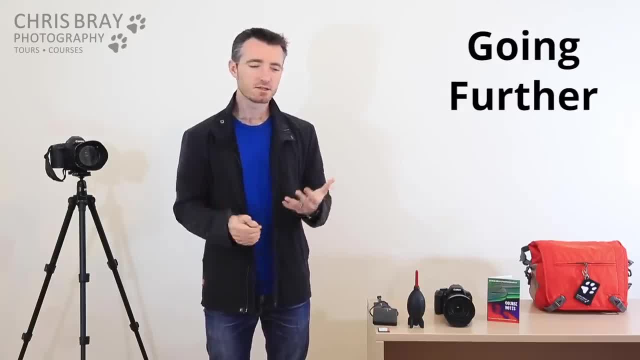 so you could send them a photo of some topical event that just happened. Don't do that kind of stuff to magazines, though. If you send your top 40 photos to something- geographic magazine- the editor's not even going to have time to look at it. 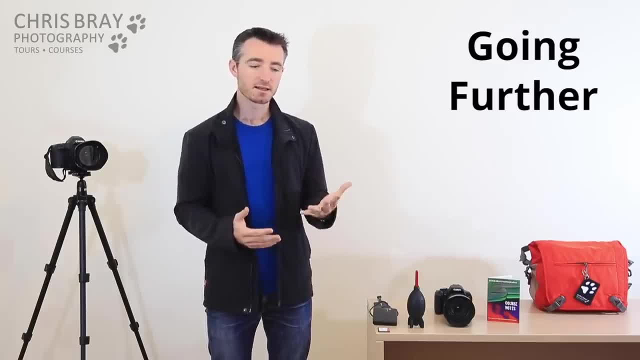 That's not their job. The best way to get into a magazine like that is in the front couple of pages or the back. there's often a section there of readers' photos and I know that sounds like you actually want to get paid for your photos. 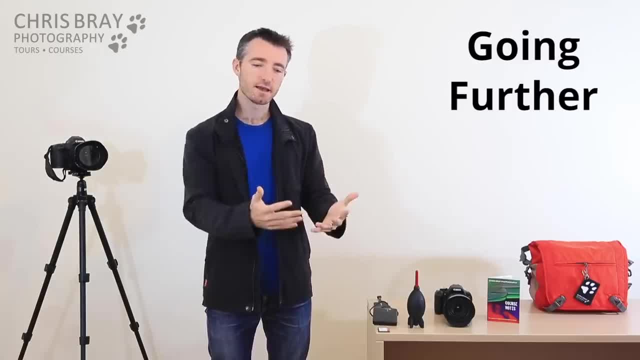 but it is still a good way in, because if you send your photos there, someone's job it is to go through all those photos and pick the ones that are the best and then, if they like yours, then they'll contact you And then you've got your foot in the door. 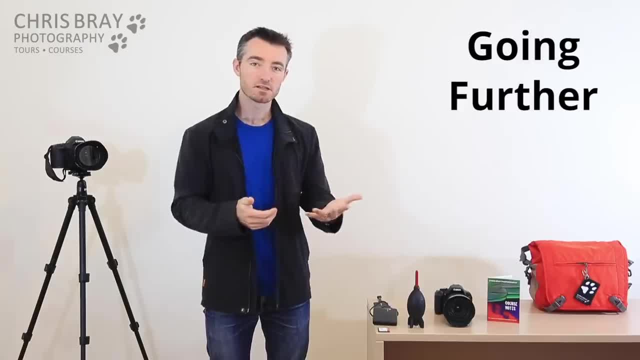 You've got a contact there And then, while you're talking to them, sending them the higher-res version, you can say: oh, next weekend I'm going to this colorful climbing festival up in the mountains. I'll take some photos and give you my best ones. 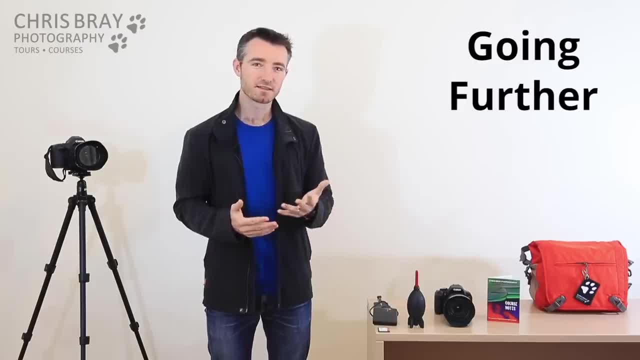 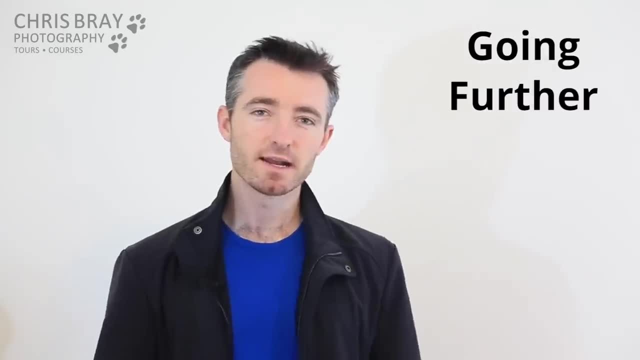 And you might have a bit of an in there. I know people who have got into magazines like that through the free readers' photos section and then submitting an article. It's worked quite well Entering competitions. that's a great way to get better with your photography. 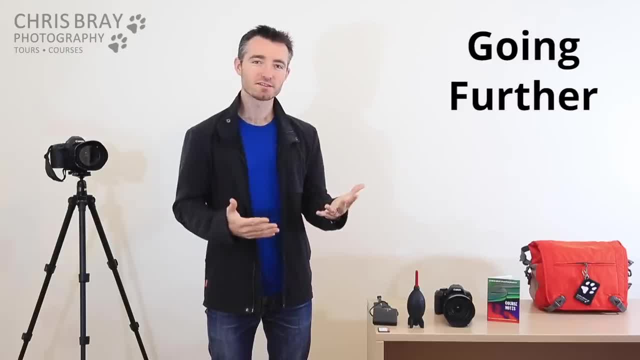 basically because it makes you practice. It's all about practice. now, Having done this online photography course, you've got more than enough theory you could possibly need to know. It's just about getting quicker at using it and how to apply it in different situations. 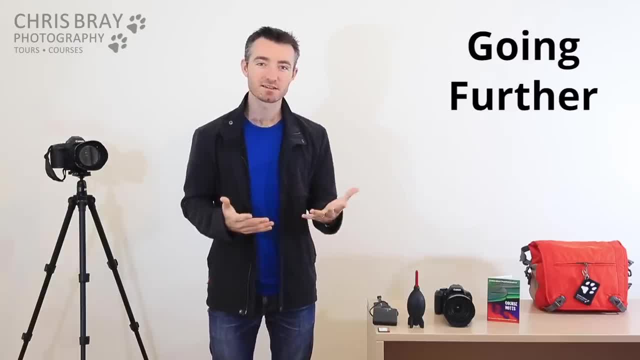 without having to think too much and so on. And that only comes with practice. So competitions give you an excuse to get out there and take photos. Often it's outside your comfort zone. You have to use some particular technique, or it has to be taken at night or something. 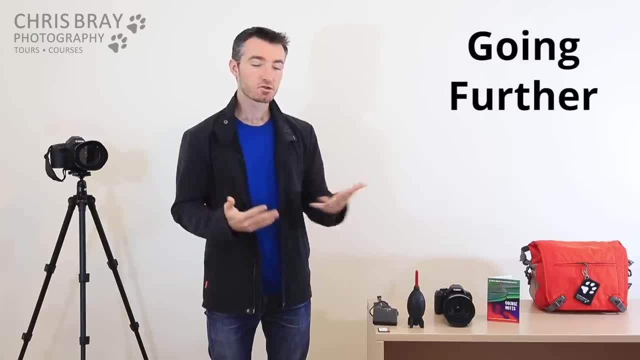 And great. that just extends your skills. Sooner or later you start winning stuff. That's great. You become an award-winning photographer. Stick that on your website. If it's a good competition, you probably win camera gear. It might even be linked to a publication. 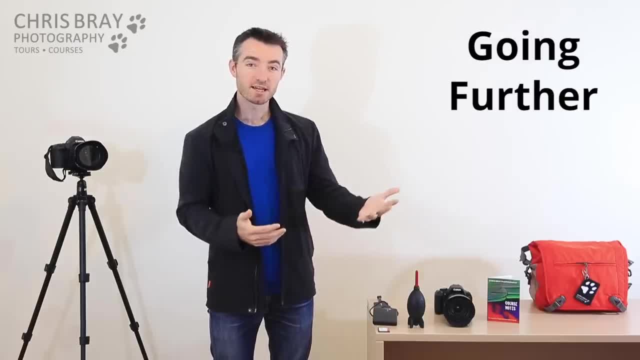 So then you get your photo published somewhere as well, So you get a contact in the industry there as well. It can all start happening at once for you if you start winning competitions, So If you don't, it's just about practice. 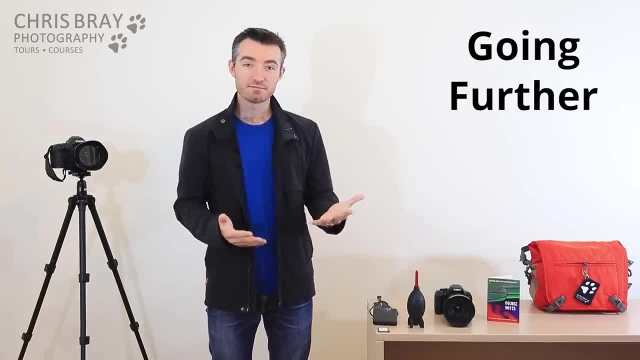 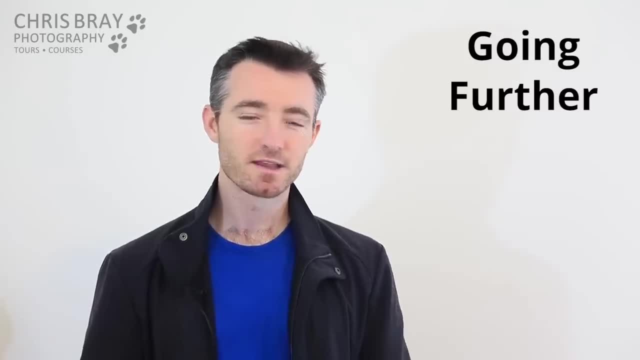 So go and find some competitions, Make a website. It's getting incredibly easy to make websites these days. You can do it yourself for free if you've got any sort of computer mouse at all. Otherwise, you can get someone else to do it pretty cheap these days. 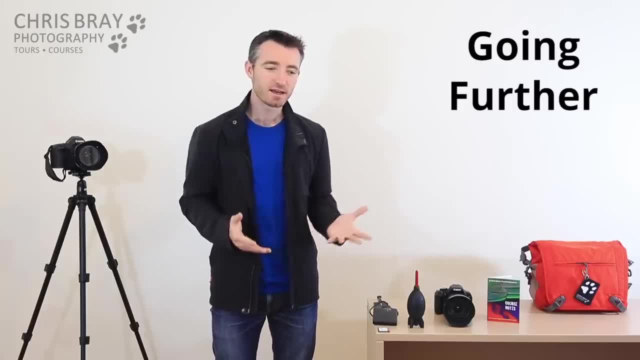 And then do go learn a bit of post-production. You do need to do that to be able to get the best out of your photos. Some people think that post-production is just cheating. They think if you touch the photo at all after it comes out of the camera. 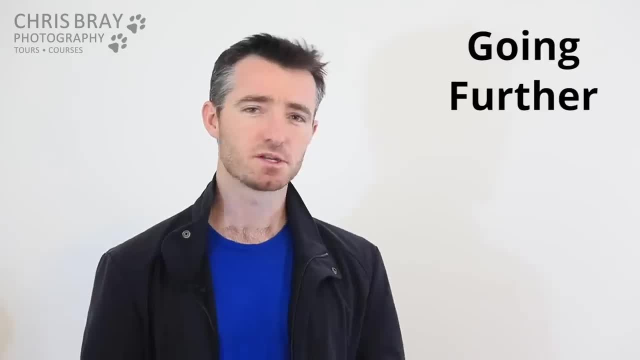 then that's cheating because you couldn't do that with film. But of course you could do that in film. You could do quite a lot of tweaking. You know just how long you left the lamp on for when you're exposing the paper. 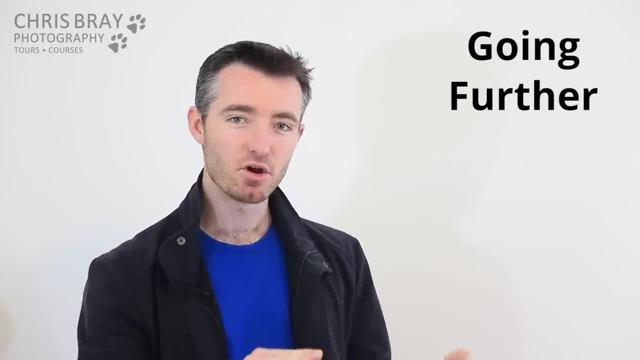 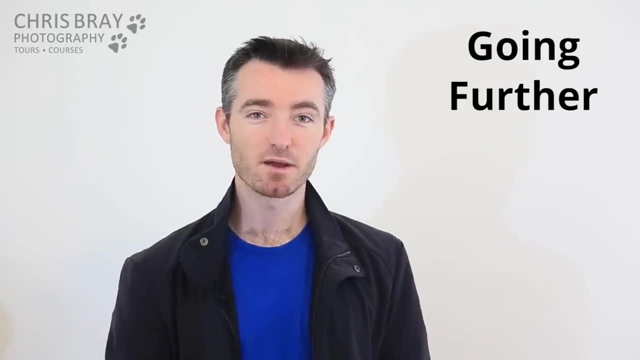 that was like changing your exposure. You could dodge and burn, cover up this bit for a while and then let the light come through. So you could be doing basically local adjustments and that kind of stuff. And that was just black and white. You could do even more with color. 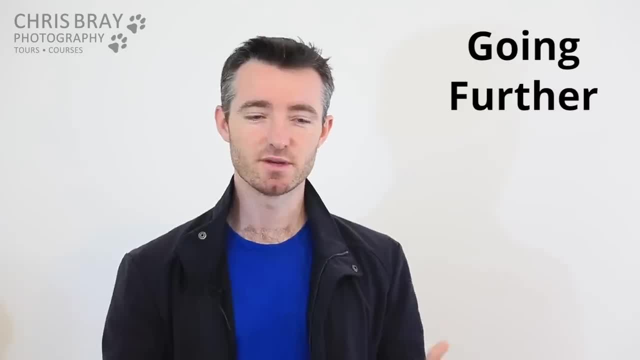 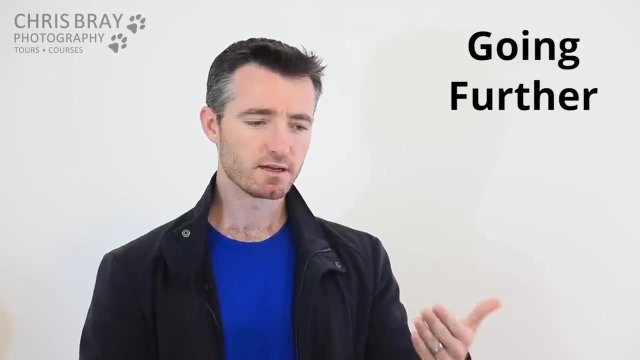 So it's a bit silly to say that, oh, just because it's digital now and it's too easy, you shouldn't be allowed to do anything. I don't think that's true. But then some people say, oh, I'm pretty sure it's okay to get this photo of a ship. 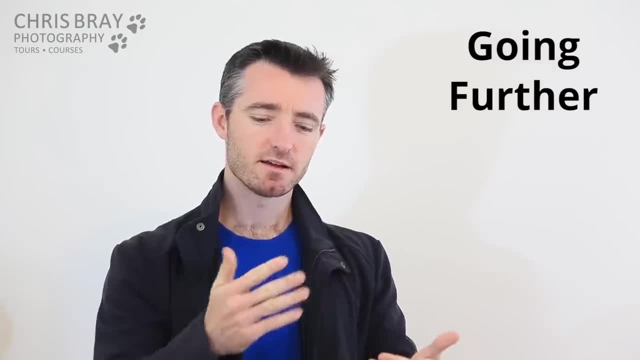 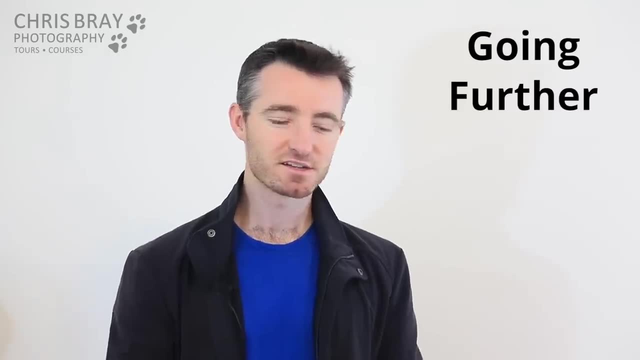 and this photo of a dolphin and then and merge it together and clone the dolphin, And now we've got two dolphins jumping over the ship. That's well, they're both digital images, right? So it's still digital photo. No, I don't think so. 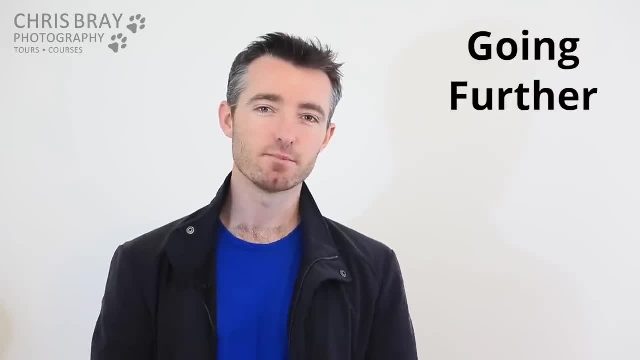 It might be a digital image as its uses, but it's not a photo anymore. But it's important to realize that even the strictest magazines around, like the Geographic series, and really strict competitions like Wildlife, Photographer of the Year, that whole. 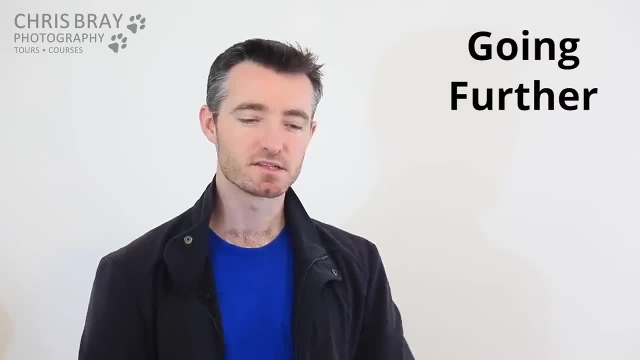 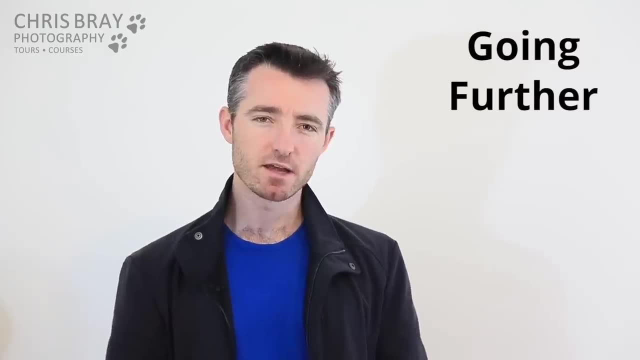 you know, huge cash prizes and whole careers are built off this thing. Any image you've seen in there in the last couple of years, they've all been digitally manipulated. But they basically try and draw a fairly clear line in the sand. Different competitions have different rules, of course. 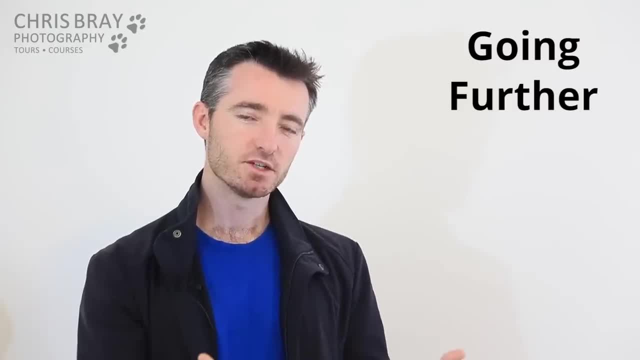 but basically they say you can do whatever you want to the image, as long as you do it to the whole image. So if overall the image is too dark, you can brighten it up. If the colors are a bit flat, you can increase the saturation. 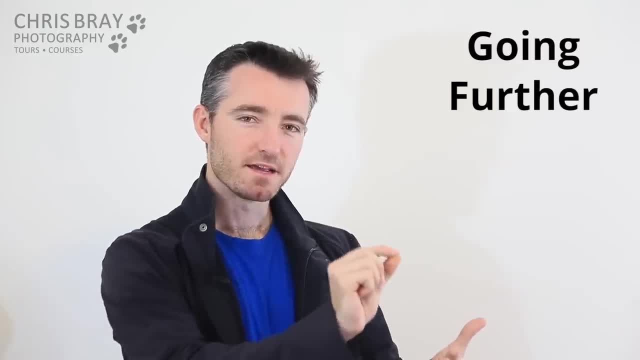 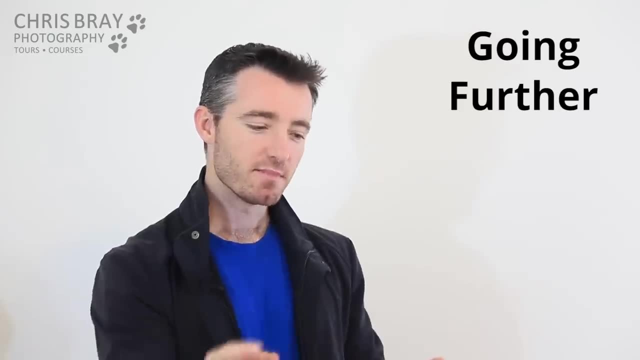 But you can't just go and get the girl's eyes and make them go green, or get rid of the person in the background or bring in a seagull. You know if you start actually changing one area and making it look like something completely different. 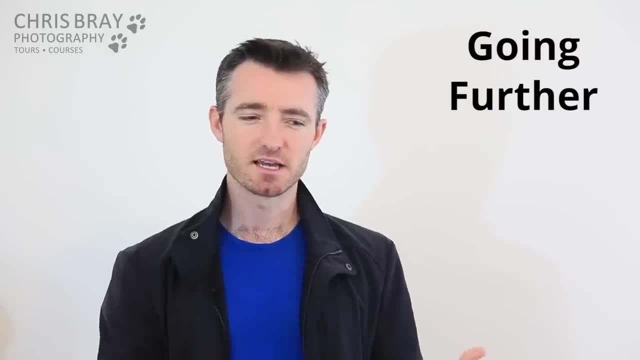 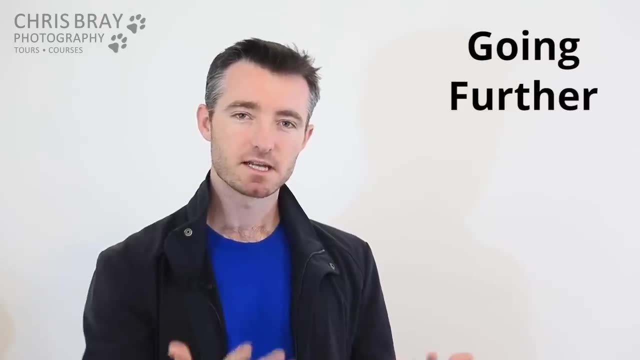 not at all like it did at the time, then that's pretty universally accepted as cheating, or at least creating a digital image anyway. But you shouldn't feel bad about going and tweaking your photo up a little bit, fixing up the colors and so on. 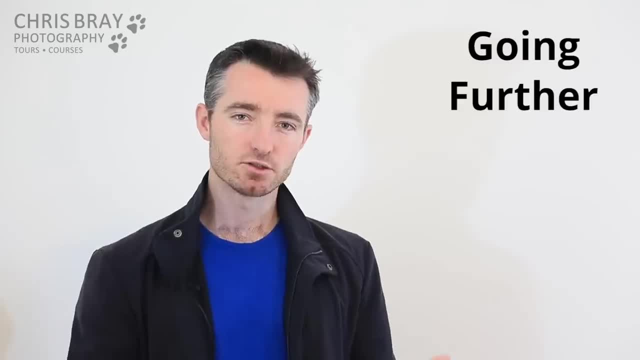 because that's the whole point of shooting in RAW. You know, when professionals shoot RAW files, it's because you get to slide the colors and everything around to more accurately represent the scene, Because otherwise you're leaving that to the camera. So in a normal camera, 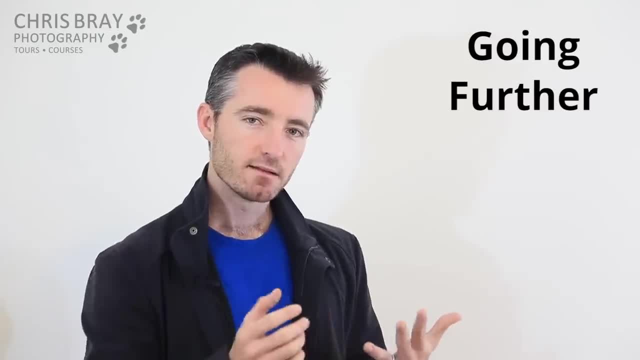 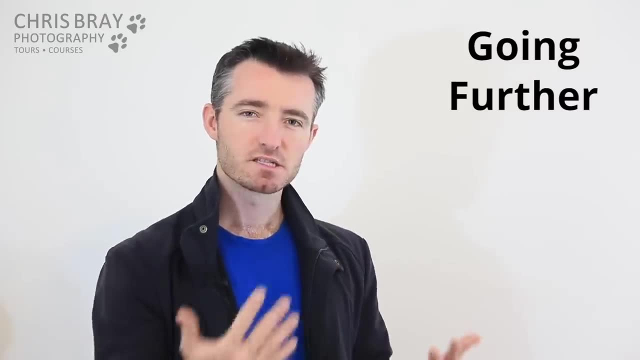 all that light comes in and they start off as a RAW file and then the camera works out how blue is this normally and how bright and dark the shadows, and it ends up with this kind of passes it through an onboard averaging algorithm and you end up with a picture. 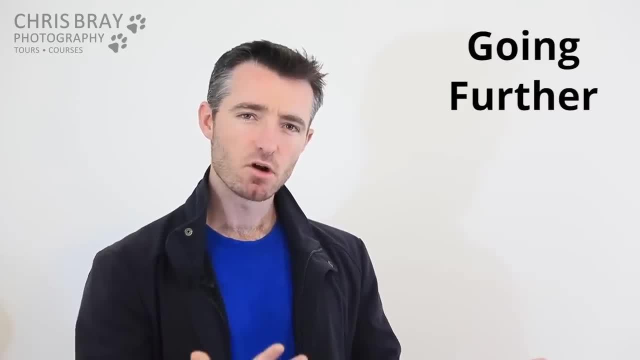 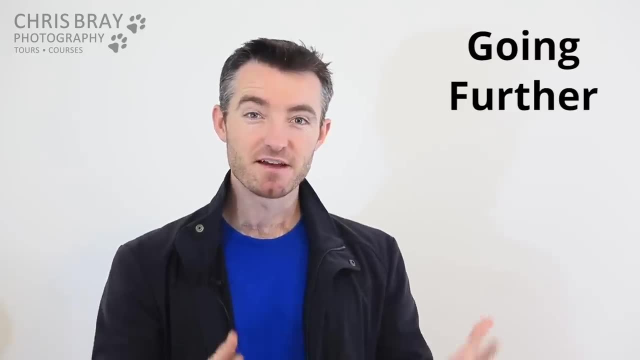 that it thinks is the best representation of the colors And it's not quite right. So if you're out there and it's a particularly vibrant blue day out at sea and the ocean is just that amazing sapphire blue color and you take a picture of it, 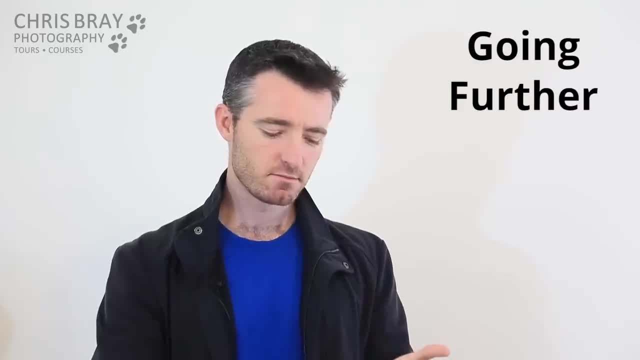 and you look at the picture, you probably think I swear it was bluer than that And it was. It really was. It just passed it through an onboard averaging algorithm and given you a JPEG. So you should go back there and punch up the vibrance of the blue. 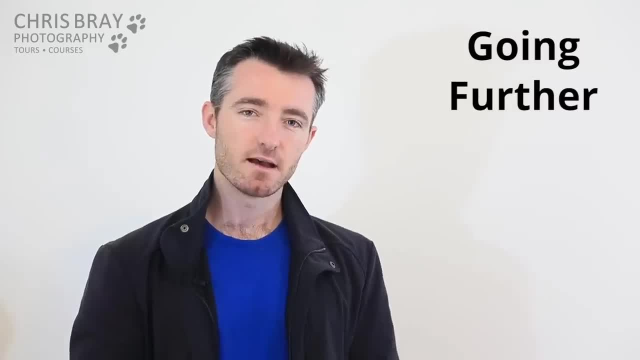 make it look nice and vivid again, just like it did at the time. Now some people have particularly vibrant memories, I think, and when they go and tweak their photos they come back looking a little bit unbelievable. Don't do that Of all the photos I've judged in competitions and things. 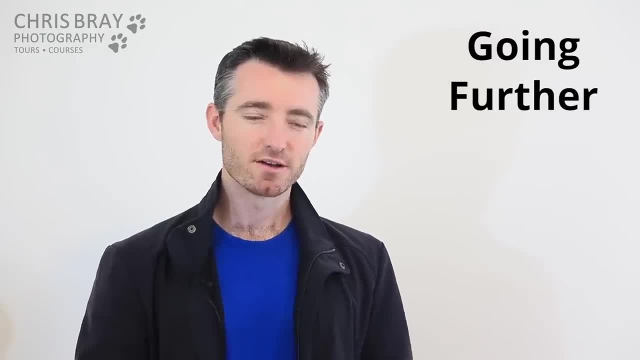 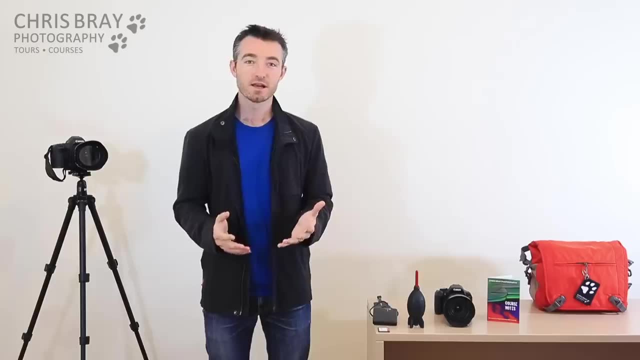 that's. the easiest way to ruin an otherwise great photo is just to oversaturate the colors and things like that. You're just trying to make it look like it did at the time, and that should be totally acceptable. So if you've got any questions or anything, 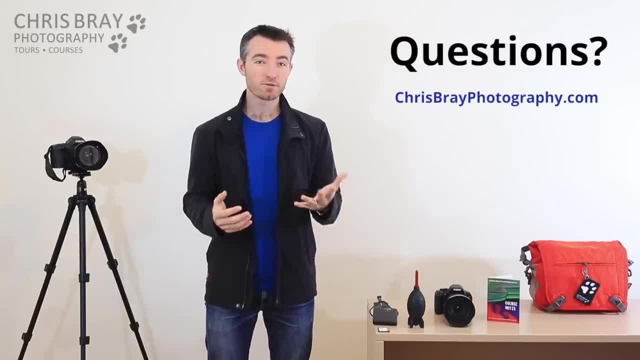 you can send them through our website, chrisbraephotographycom. or, if you're on Facebook, have a look for us on there, Chris Brae Photography. We've got a group there of more than 10,000 people. 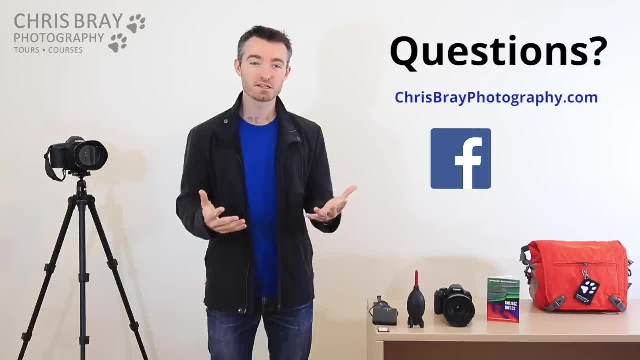 Most of them have done the photography course, so it's just a great knowledge base of photographers there. You can ask questions If you want feedback on your photos, or should you buy this lens or this one rather than asking me. I will reply. 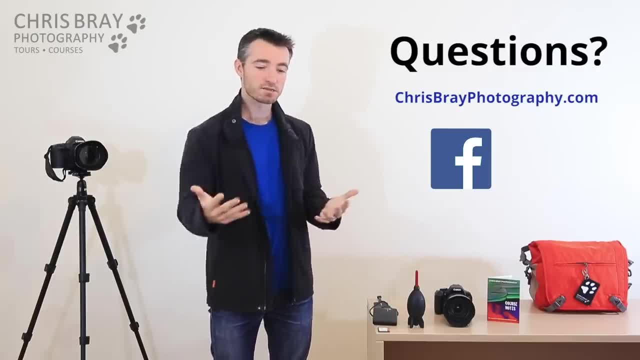 but my answer's not necessarily correct, even. But if you've got a list of 10 things or if you've got a list of 10,000 people there who are giving you feedback, the average of that probably is about correct, So it's a good resource. 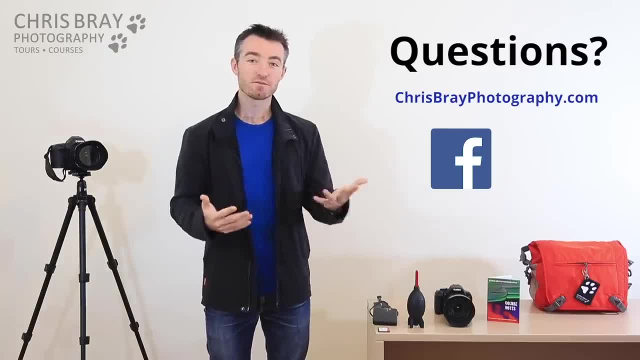 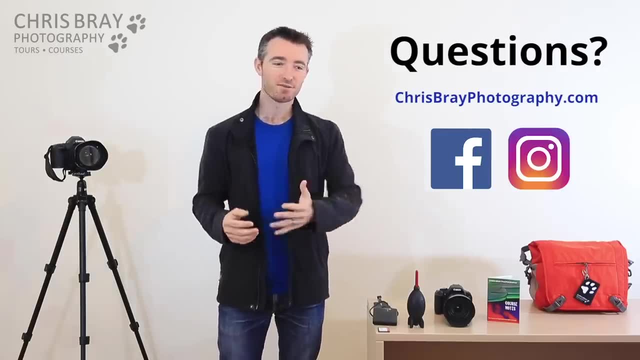 We try and keep it current with news, photography news, new cameras that have come out or competitions you might want to enter, So go and have a look for us on Facebook. We're also on Instagram If you want a beautiful photo sent to your smartphone every day or two. 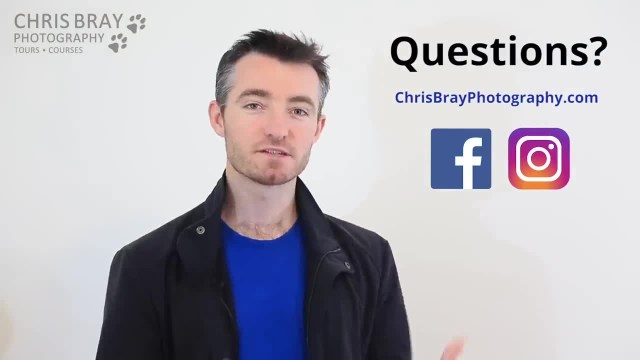 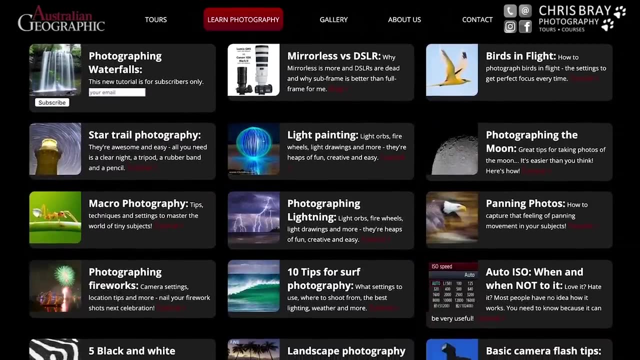 go and sign up on there And then go to our website and look at all those free tutorials. As I said, we've got so many free tutorials there covering so many different topics, from things like light painting and star trails to photography, Photographing, fireworks and lightning. 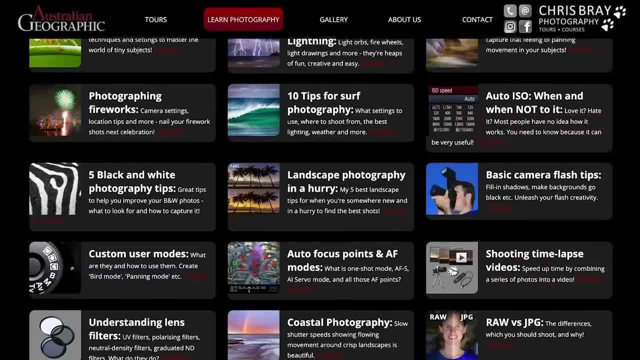 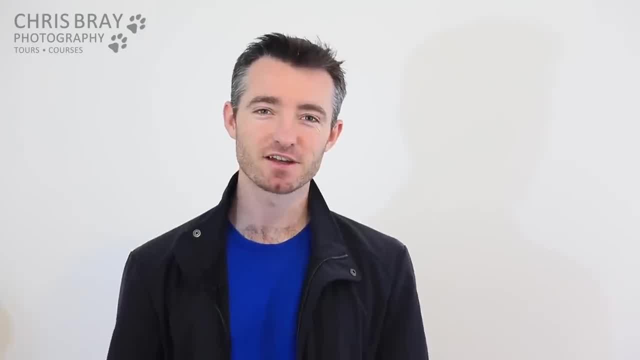 using custom modes, flash basics, the moon and more advanced stuff. like you know, the real difference between JPEG and RAW. Okay, now that you've finished my photography course online, if you enjoyed it, I really recommend you go and take a look. 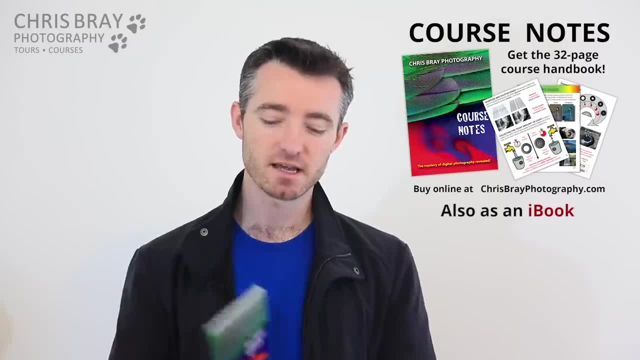 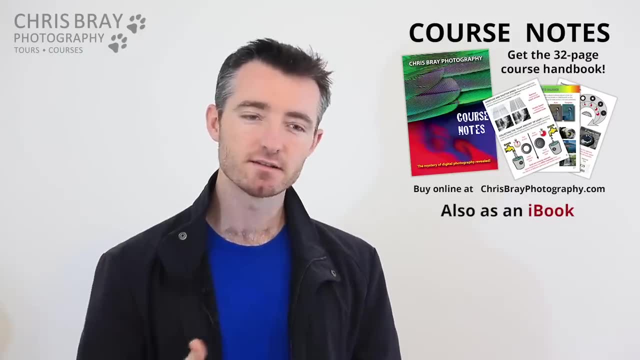 at the course notes booklet that goes with the course from the website. It's just a handy little refresher of everything in the entire course, one little section at a time And you can just sit there and re-read it until it all makes sense.